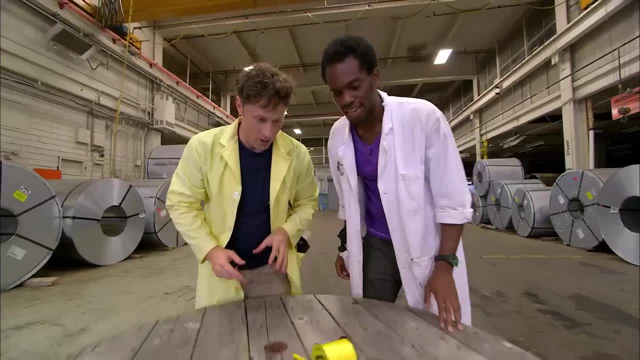 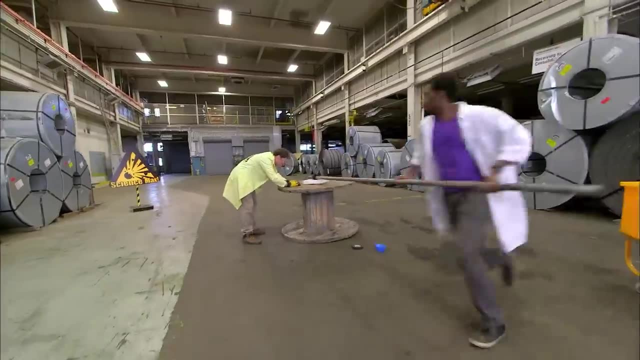 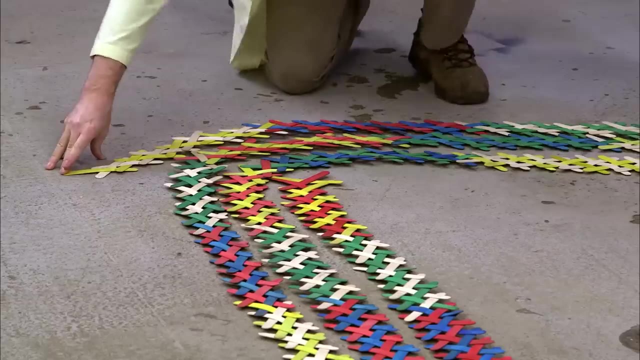 Science Max. This episode of Science Max is all about storing energy and releasing it. Yeah, let's try it out for real: Storing it in a giant spool racer Plus a domino chain reaction, mouse trap chain reaction, popsicle stick chain reaction. 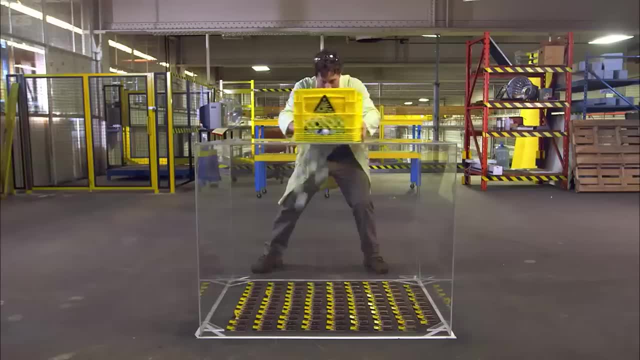 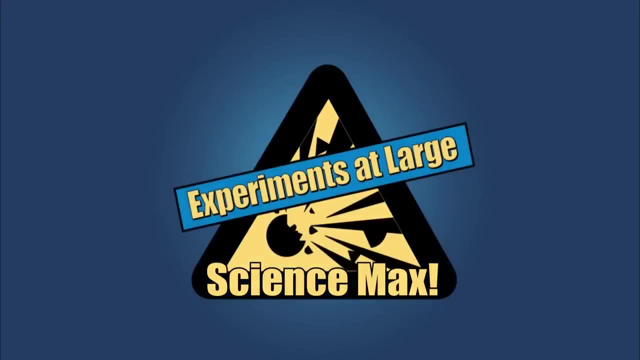 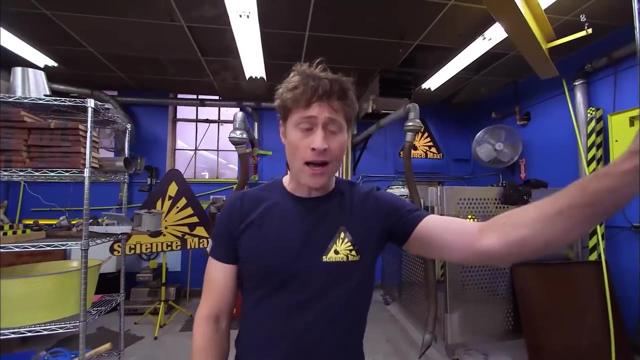 and more All on this episode of Science Max Experiments At Large. Okay, three, two, one go. Greetings, Science Maximites. Welcome to Science Max Experiments At Large. Wow, I really need some more energy. Fortunately I have some saved up. 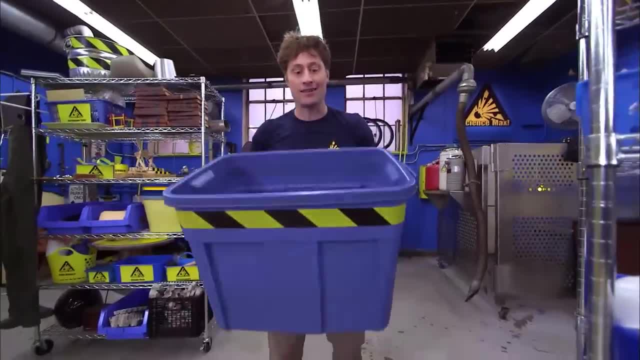 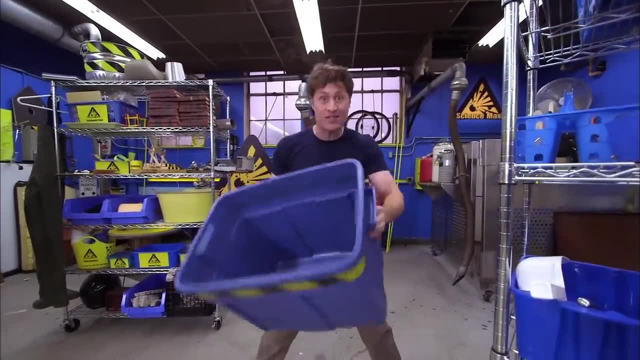 Ah, that's better. Yeah, I know what you're thinking. Storing energy like that doesn't make a whole lot of sense. But you can store energy and that's what this episode of Science, Max Experiments At Large, is all about. 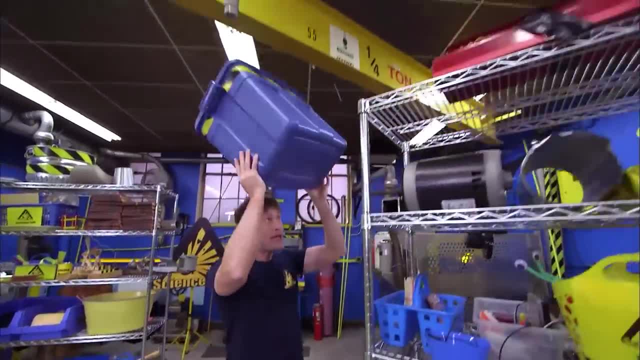 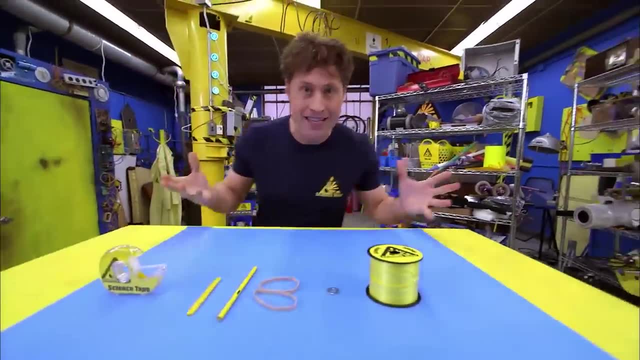 In fact, I'm going to store some energy in this container simply by putting it up here on the top shelf. More on that later, But right now let's look at another way that you can store energy and release it in a really fun way. 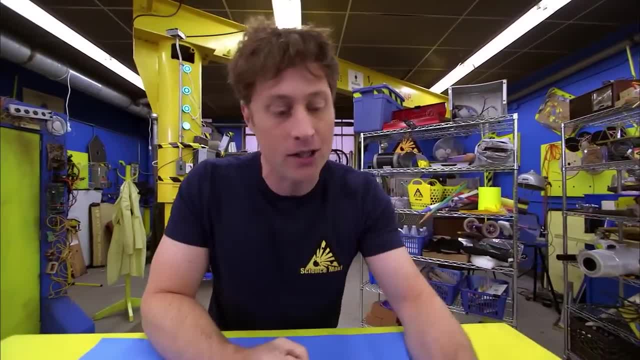 We're going to make a spool racer And it's pretty simple. Here's all you need. You need some science ribbon. Now, if you don't have science ribbon, you can use regular ribbon, But the ribbon really isn't important. 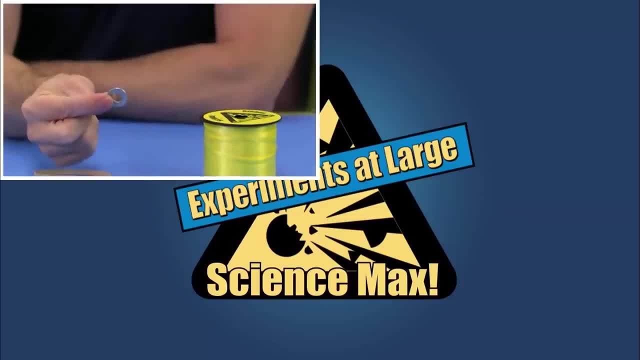 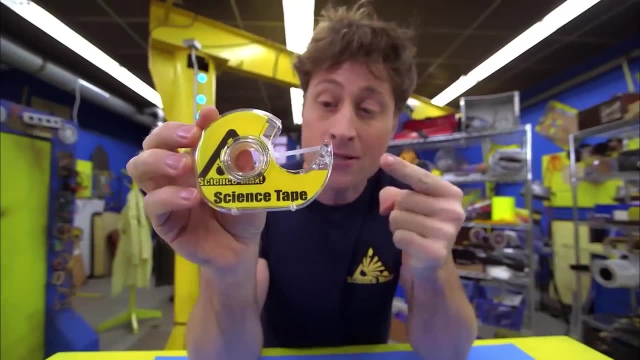 It's the spool that's important. You'll also need a washer elastics pencil or pencil crayon, a popsicle or craft stick and science tape. Science tape is the same as invisible tape, except I use this one only for science. 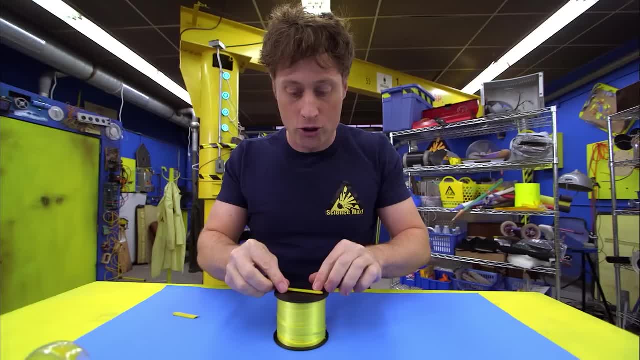 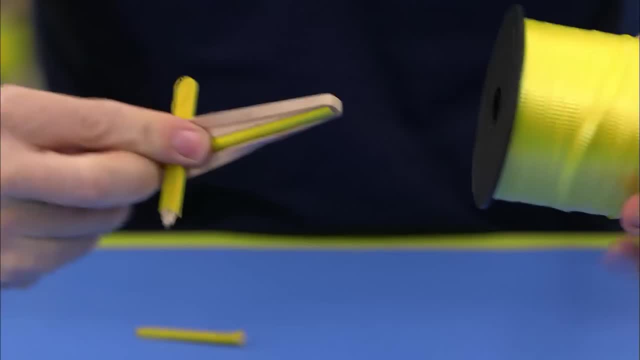 Here's how you build it: Break the popsicle stick so it's smaller than the diameter of the spool. Then put the elastics on top of the pencil and pull them tight. Thread the popsicle stick through and feed it all through the hole of the spool. 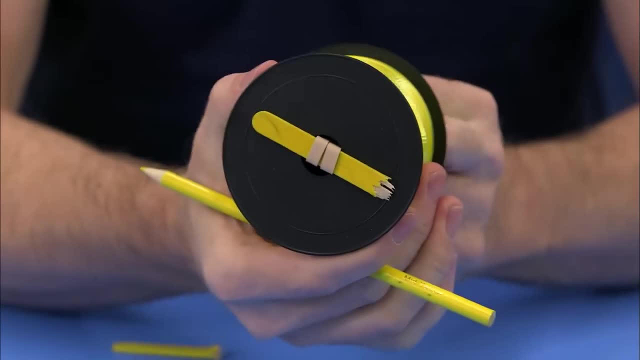 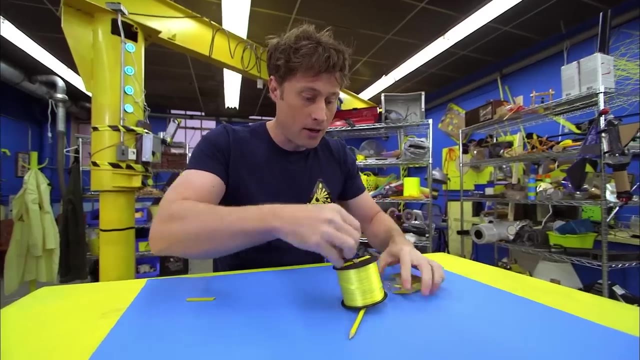 Grab the elastics on the other side and pull out the pencil and everything will be threaded perfectly. Then stick on the washer and thread the pencil through. Finally, tape the popsicle stick down so it doesn't move. And if any of these steps are a little too fast, 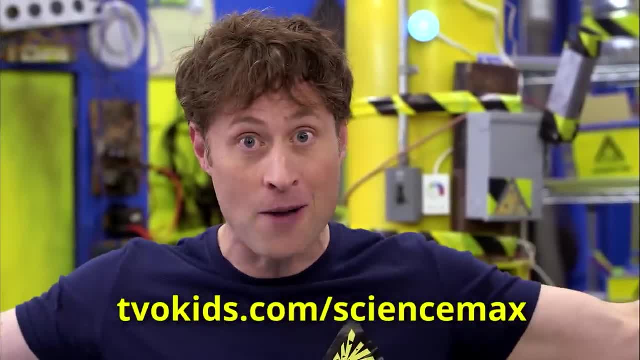 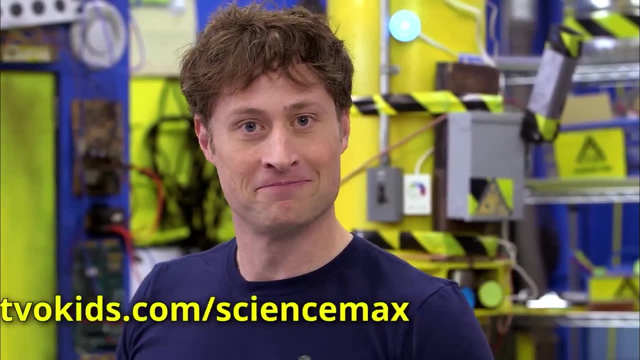 don't worry, All of the instructions are up on the website. That was cool. I can't make it go away, I can only make it come up. So there you go, A spool racer, And here's how it works. 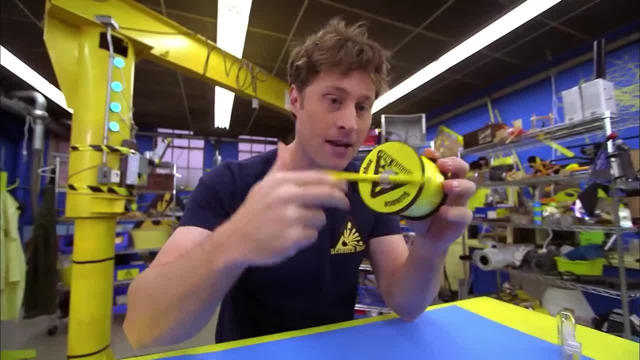 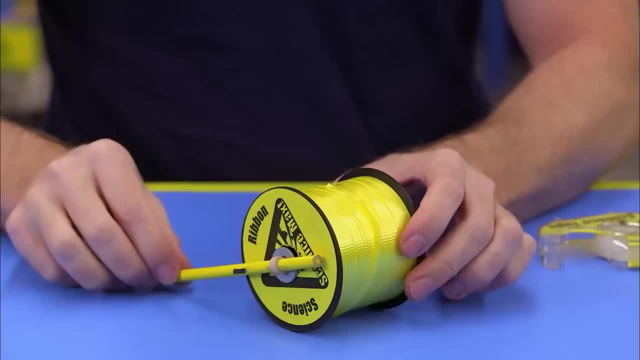 You spin the pencil around and that twists the elastic. Now that elastic is going to want to unwind, right? So just keep spinning that pencil around until it's good and tight, And then, when you put it on the ground, the pencil's going to want to unwind. 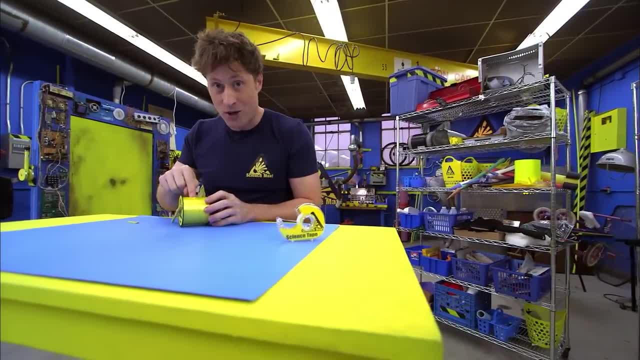 but it can't, because the table's in the way now, which means that the energy is going to transfer to the spool, which is going to turn Whoa And it's going to drive away. Yeah, Let's try it out for real. 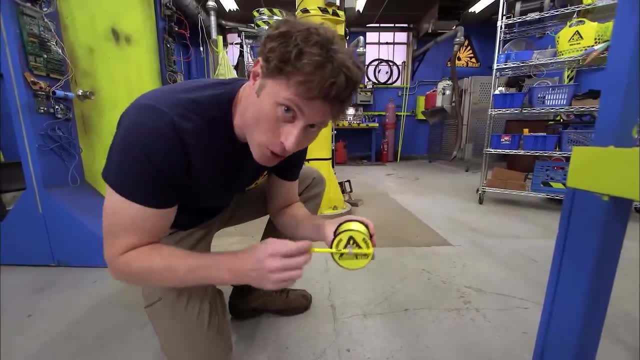 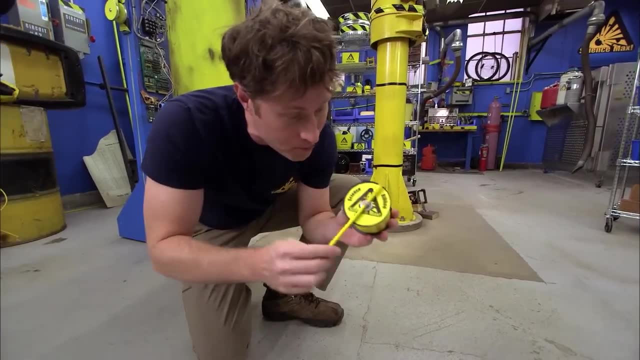 So why does this work? It works because the elastic is coiled right. Yes, and because I'm putting in the energy to twist it. You see, I'm putting in effort to spin this pencil crayon around and then, when I've finished, 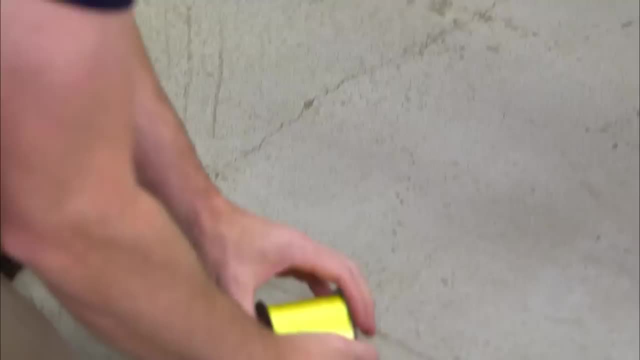 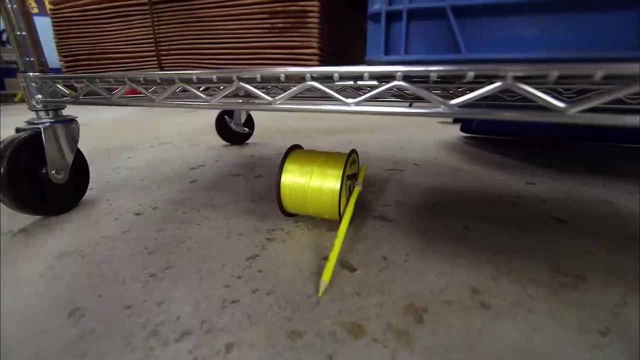 all of my effort has been stored in the elastic. When I let it go, my energy transfers into movement. So that's Uh-oh. That's what we're going to do today. Science Maximites: We're going to max out the spool racer. 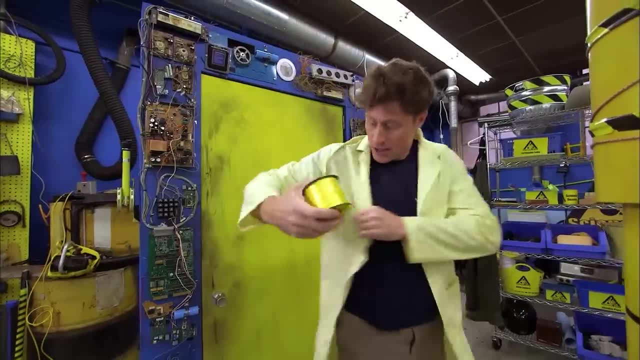 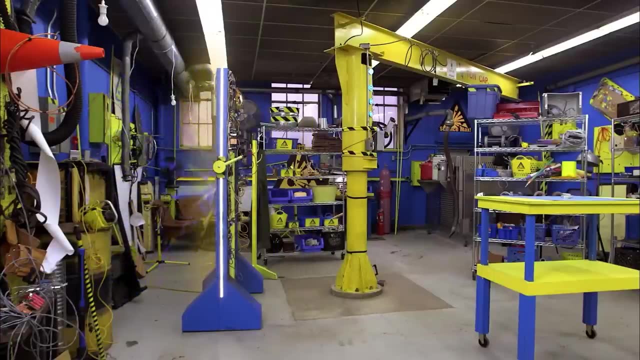 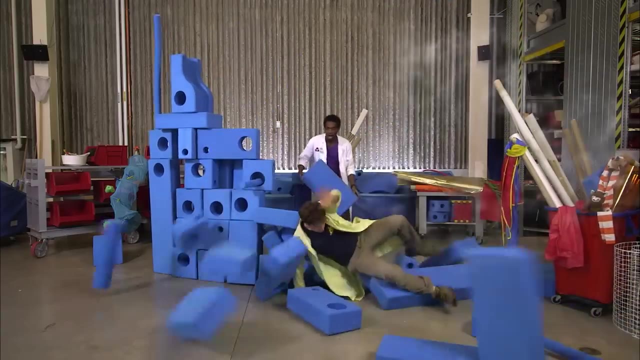 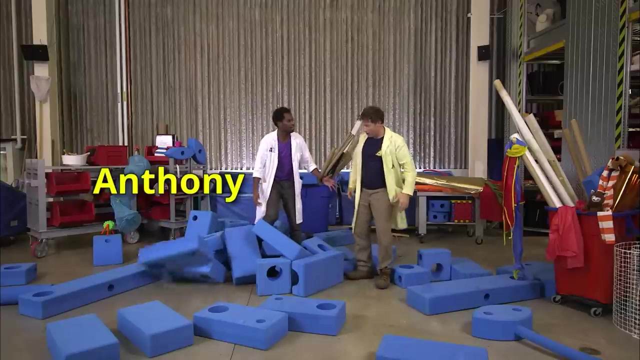 I think Anthony would really know how to help me with this. So I'm off to the Ontario Science Centre. Come on, Let's go, Phil. What happened Phil? What happened You? okay, Anthony, Hi, Oh, were you in the middle of something? 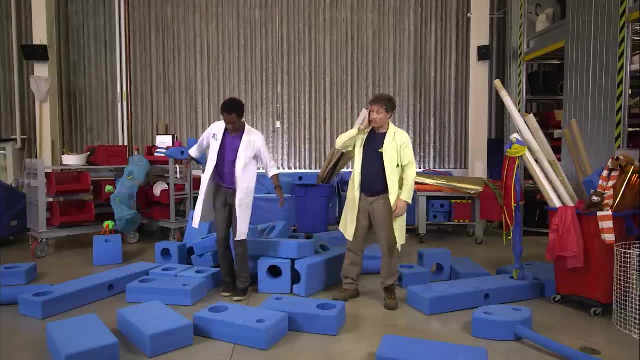 I don't worry about it. yeah, Oh, okay, Sorry about that. You know what I was wondering If I could get your help with something. Sure, yeah, Yeah, One word: Spool racer. Actually, that's two words. 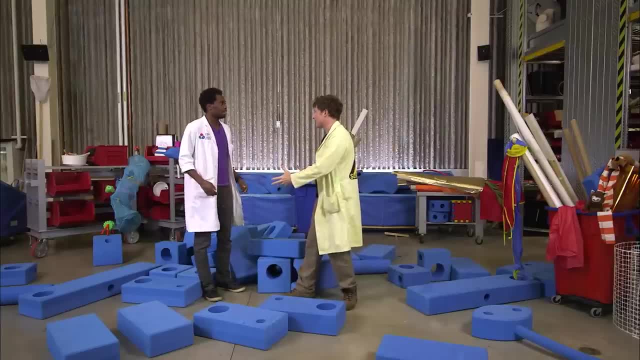 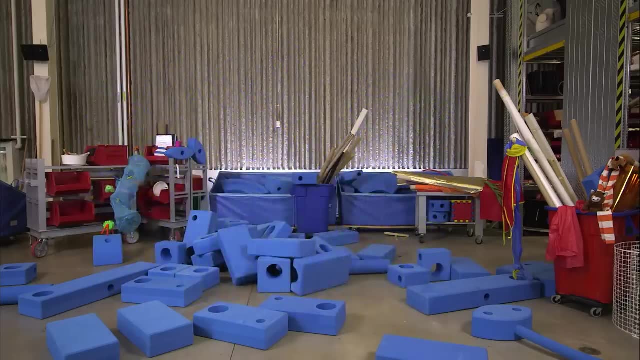 Spool spool racer. Yeah Yeah, Do you want me to max out a giant spool racer? Uh yeah, Awesome, let's go back to Science Mat 10 quarters. Okay, Anthony, today I want to max out the spool racer. 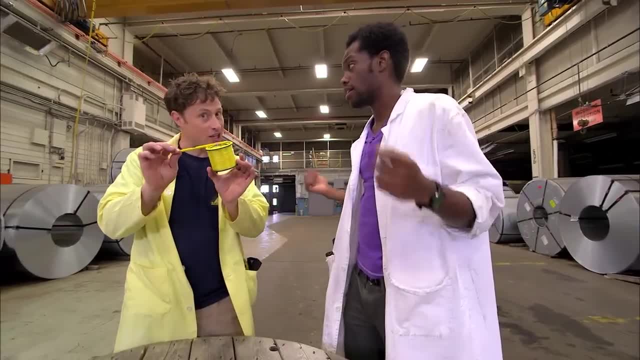 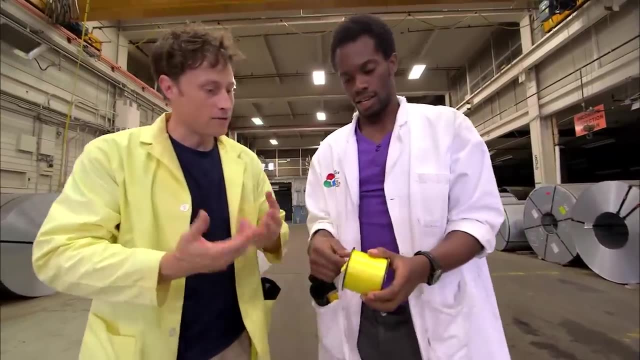 Awesome, Right, so you twist up the elastic and it goes from potential energy all stored to kinetic, kinetic energy. Whoa, there we go. That's awesome, So not too hard to design. should be fairly easy to max out. 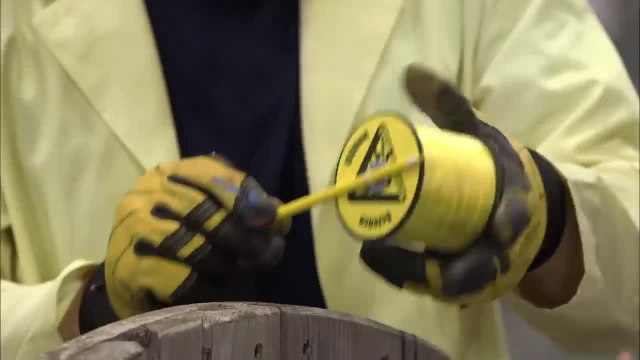 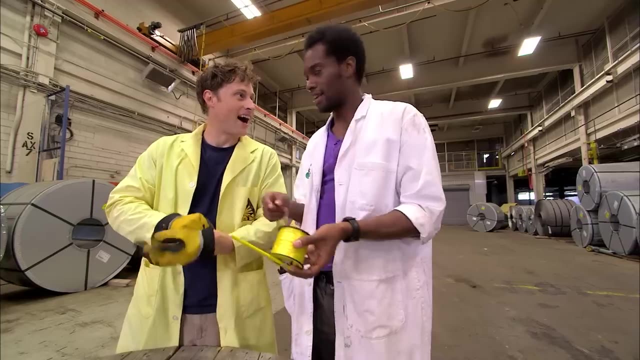 Yeah, really simple couple of parts here. We just got elastic band inside and then this big long pencil to store the energy and then release it. And the most important part, Ah, is spool. Is the spool, Exactly? And I know where we should start. 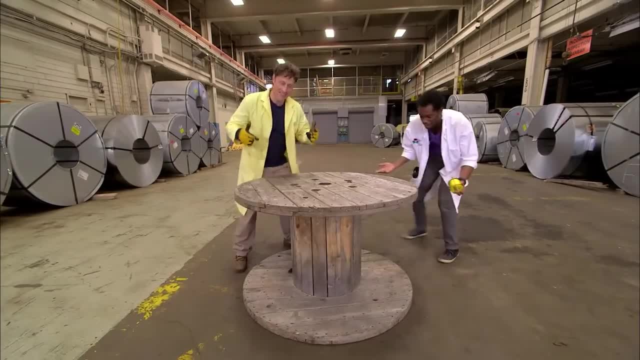 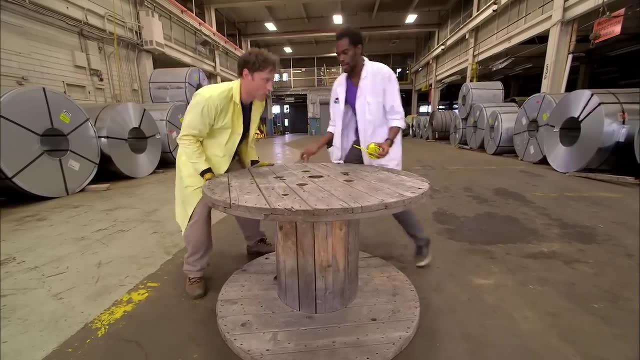 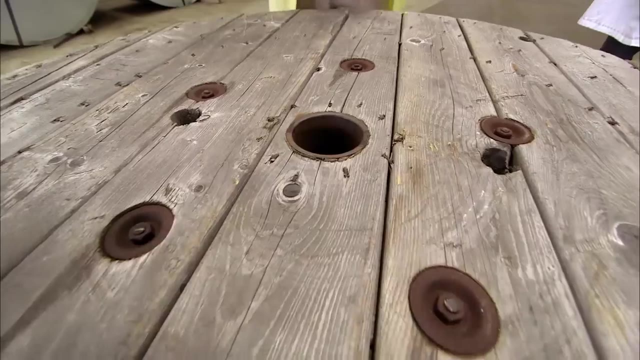 Where's that Right here? This is an industrial cable spool, so the big thick electrical cables they come wound on this thing. Yeah, okay, So we start with this. Got it, And the good news is that it's got a hole already. 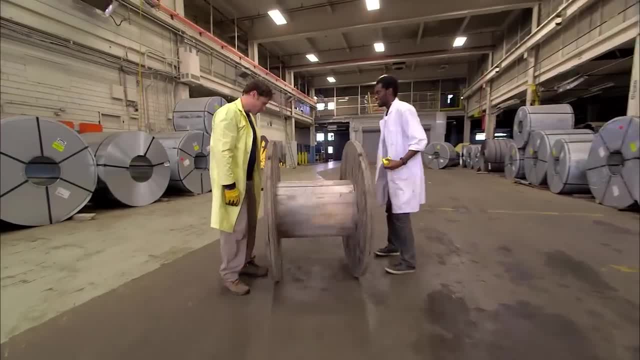 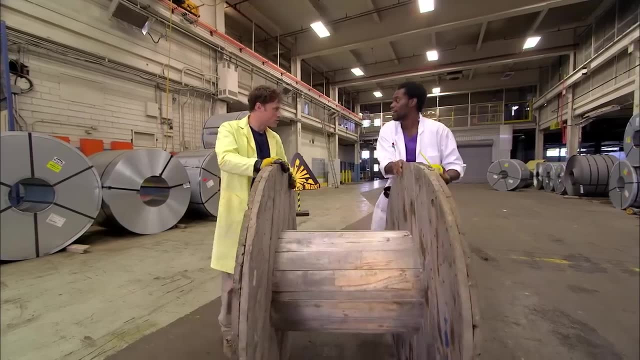 And check it out. it rolls. it rolls really well, right? Uh-huh, Okay, cool, Okay, okay. So bungee cord, Yep, And long pole or something, Yeah, And we're ready to go. 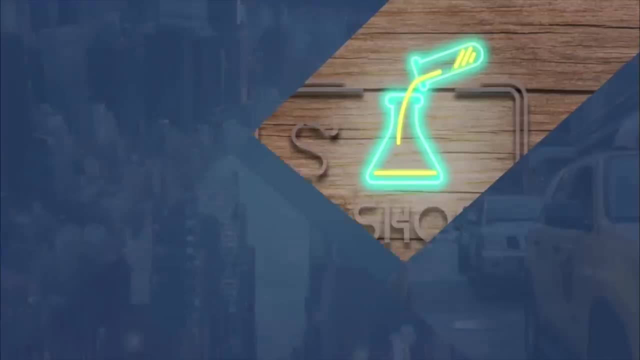 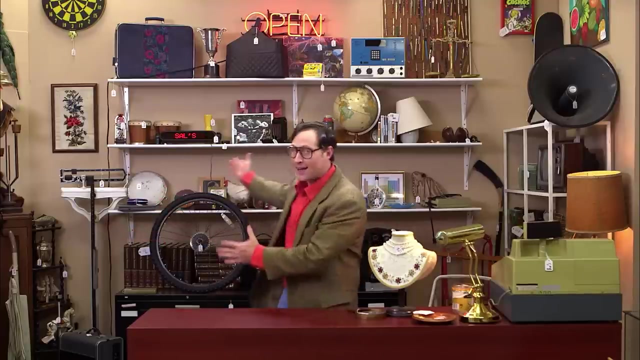 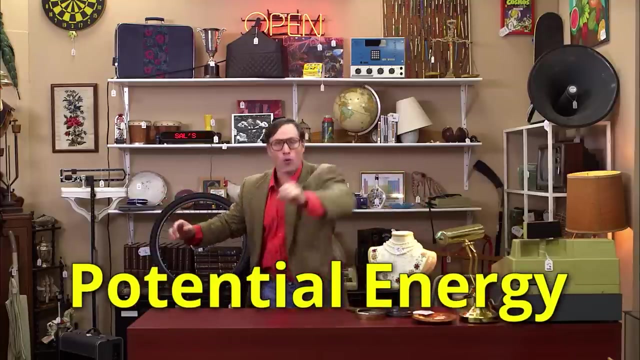 I guess let's get some parts, Okay, Okay. Oh, hey, how you doing? You wanna buy something? I got a lot of stuff here and I got a special today, only Potential energy. huh, I will throw in some potential energy. 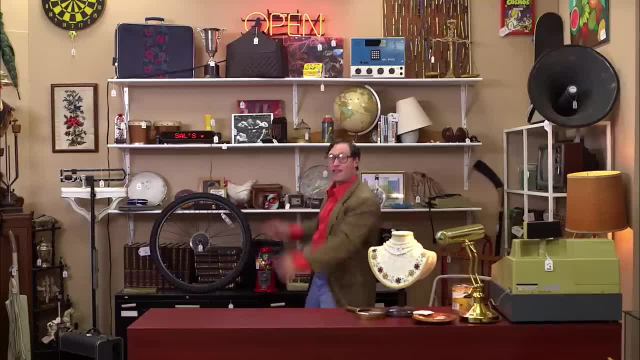 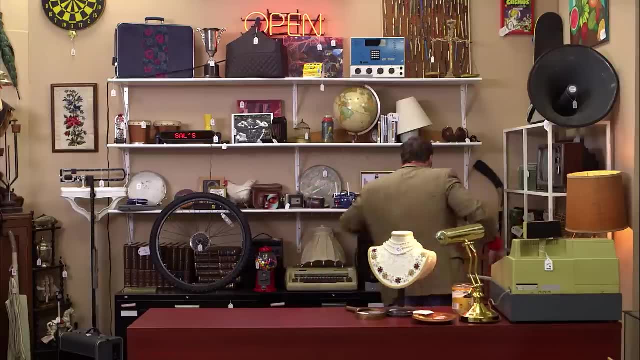 with any order. You see this stuff on the shelves here. This stuff on the higher shelves has more potential energy than the stuff on the lower shelves. Don't believe me Here? hold on, hold on. Look at this state-of-the-art traffic controller. 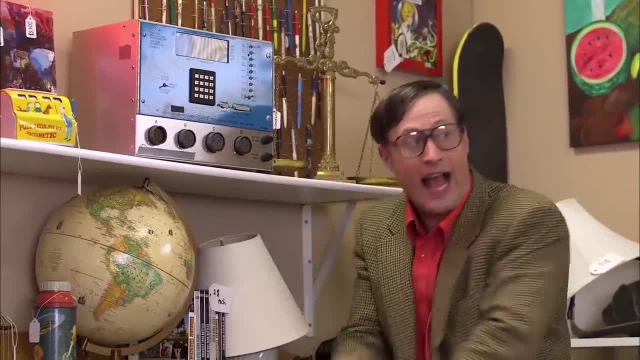 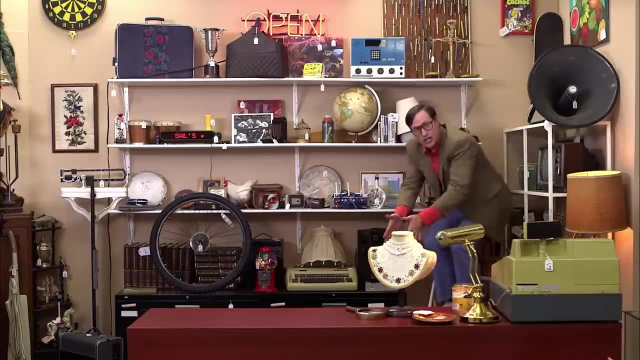 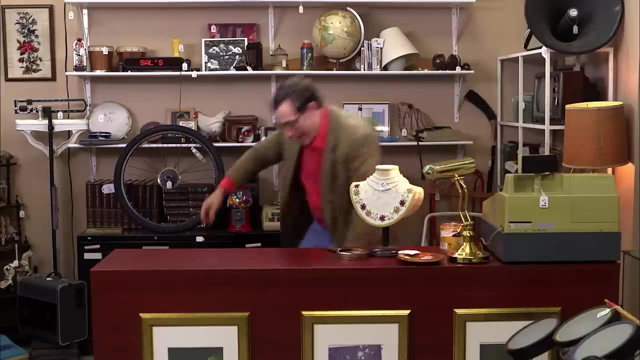 Right now it's sitting up here on this high shelf. Now, if it were to fall, it would be going fast, which means it would have a lot of kinetic energy. You see, when it fell down, it had enough kinetic energy. 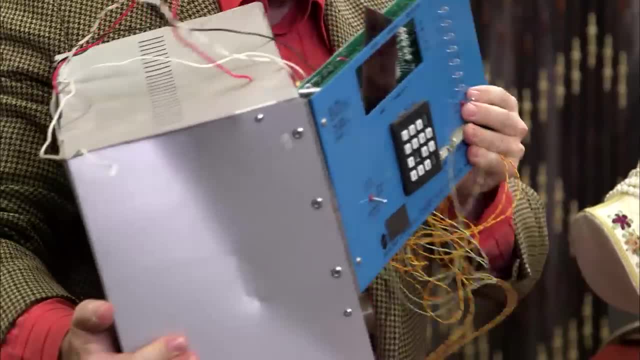 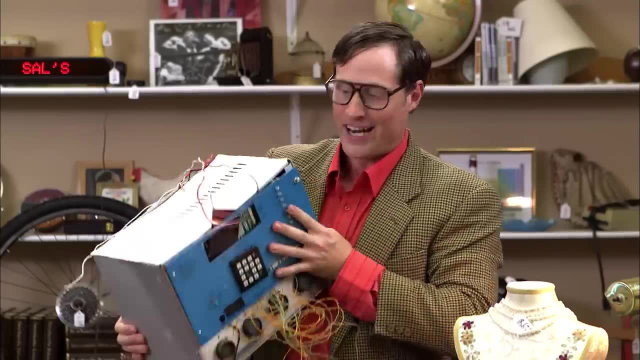 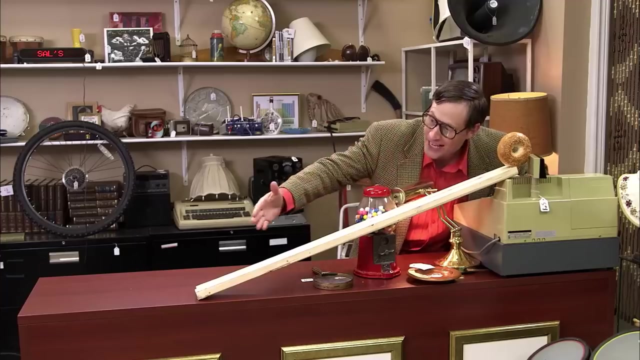 to completely break itself apart. Um yeah, Well, that's the difference between potential energy and kinetic energy. Look at this bagel just sitting here, not moving, minding its own business on top of this ramp. It's all potential energy and no kinetic energy. 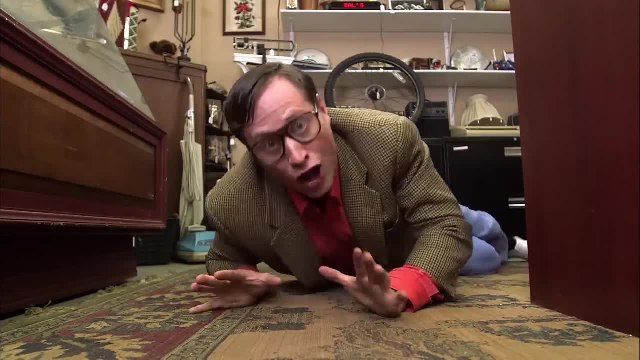 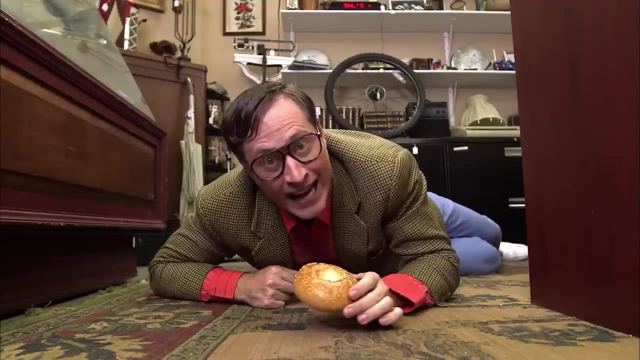 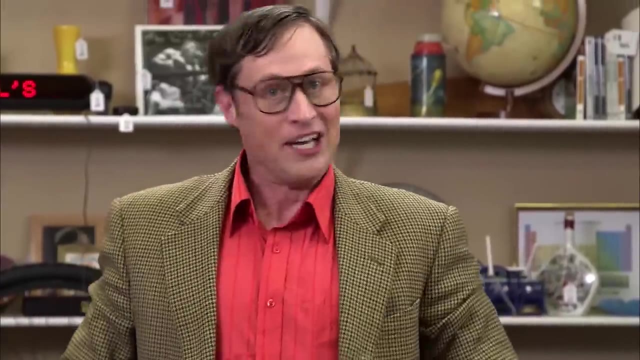 And when it gets to the floor, it's all kinetic energy and no potential energy. Whoo-hoo. And now it has neither, because it's on the floor and it's not moving. Ha, five-second rule, And now you know your energy. 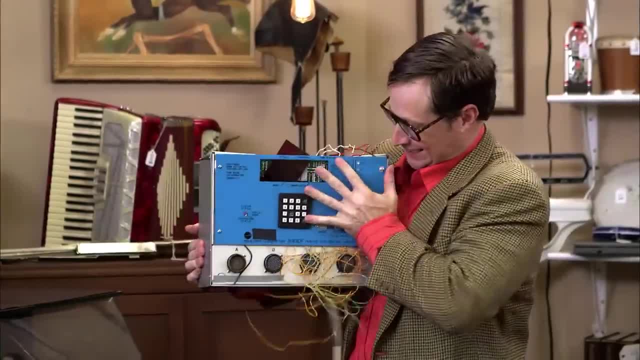 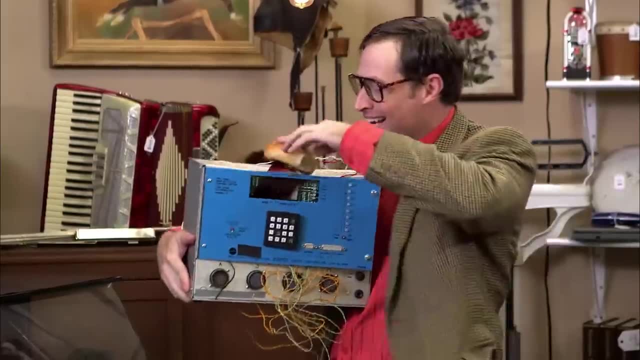 So what do you say? You want this thing. Uh, tell you what. I'll give you a discount because you know it's gently used. Hey, I'll even throw in this bagel, huh, Alsogently used. 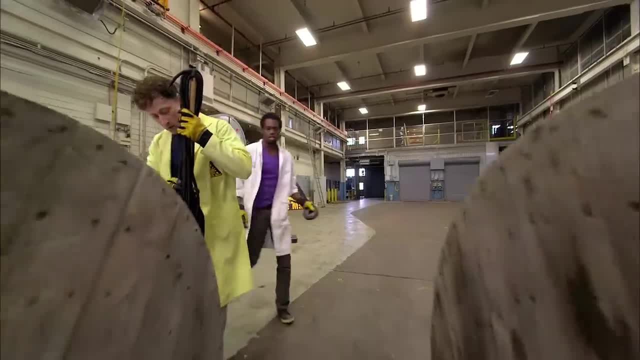 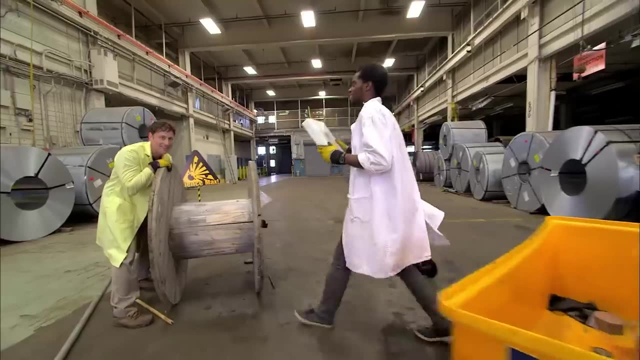 Anthony and I are maxing out the Spool Racer. We start with a long coil of bungee cord which is kind of like a giant elastic and feed it through the spool. Then we put on a big piece of plastic. 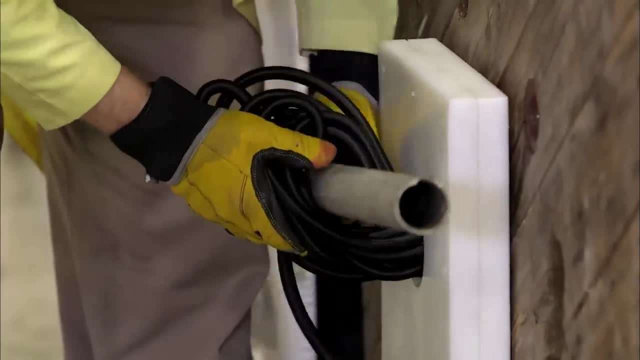 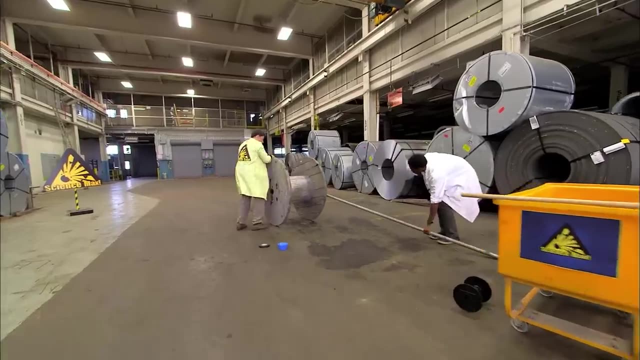 to act as our washer and use a long pole as the pencil. We flip the spool on its side to wind it up, Then we flip it back and it's ready to go. All right, so we have it all wound up. 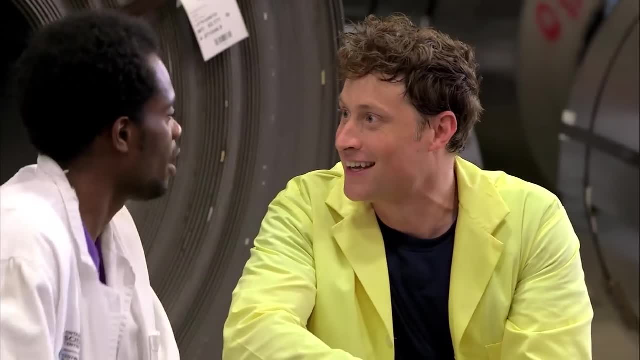 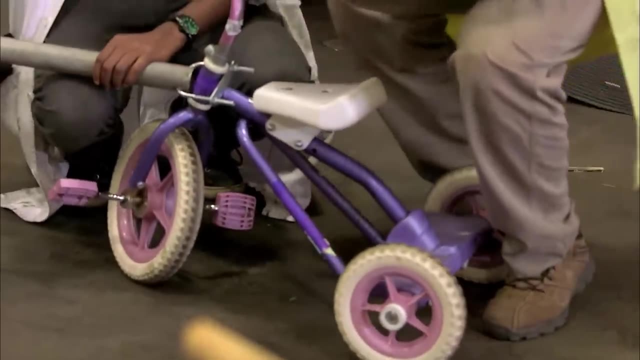 and we're ready to try it again, but with one change. Uh, Phil, Yeah, What's with the trike? I ride the trike. It's like I always say: What's the point of building something big if I can't ride it? 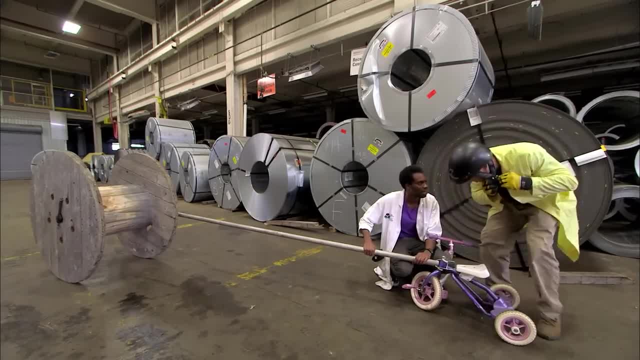 There's no way you're gonna fit on this thing. No, no, I don't put my feet on the pedals, I put my feet here on the back, right, Okay, yeah, I get it. I get it, You got it. 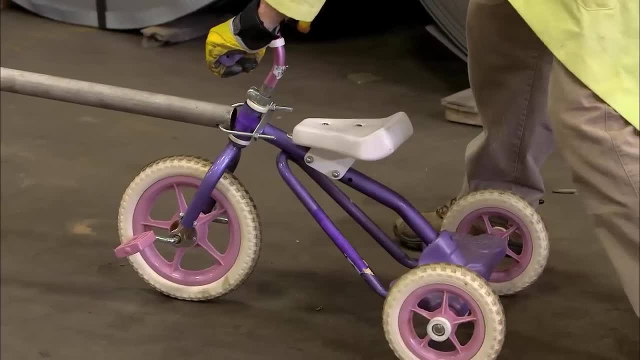 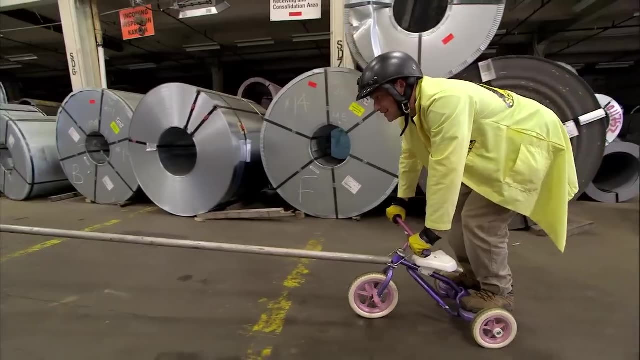 Uh, hold on, I gotta do my helmet up, Safety first. You ready, I'm on it. Okay, three, two, one Go. Oh, it's working. It's working. Amazing, All the stored energy in the bungee cord. 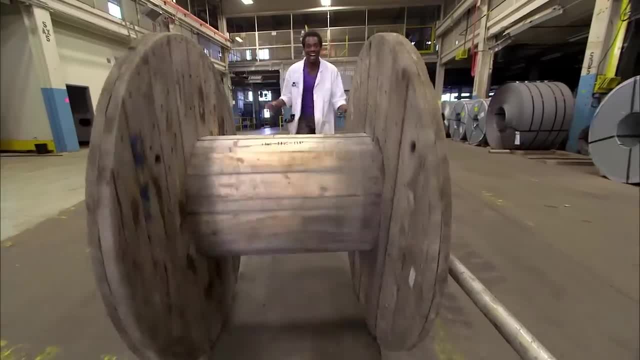 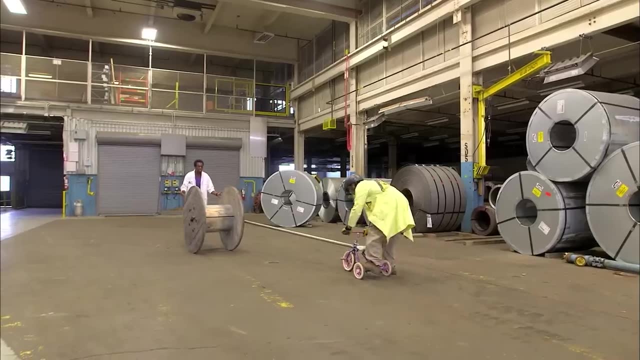 is being released and the spool starts to turn, There's even enough energy that I can get pulled along behind it. It's not going that fast, though It's pretty good, though It still pulls me Right, Yeah, pretty good. 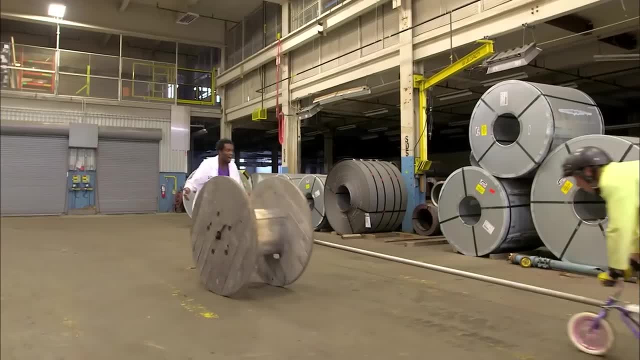 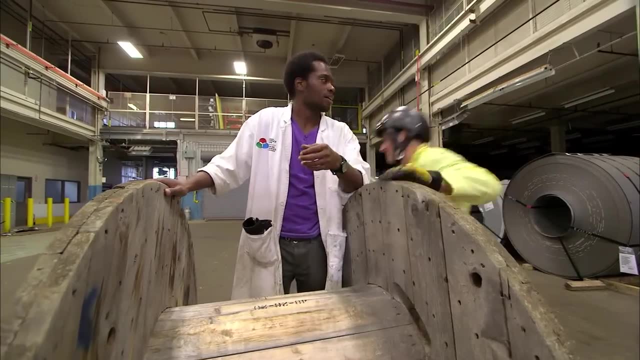 So spool racer actually able to get pulled by it. Yeah, You know what? I think we can go even bigger, Bigger, Yes, Well, what did you have in mind? I'm glad you asked. I'm glad you asked. 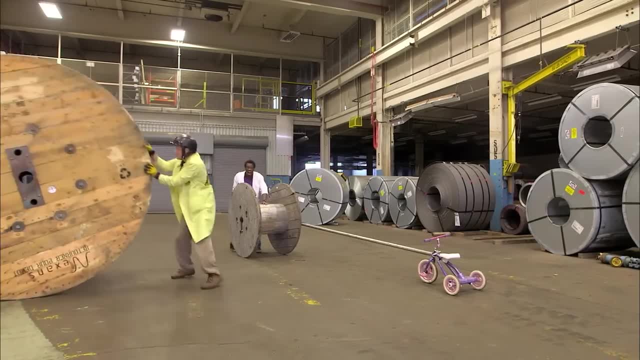 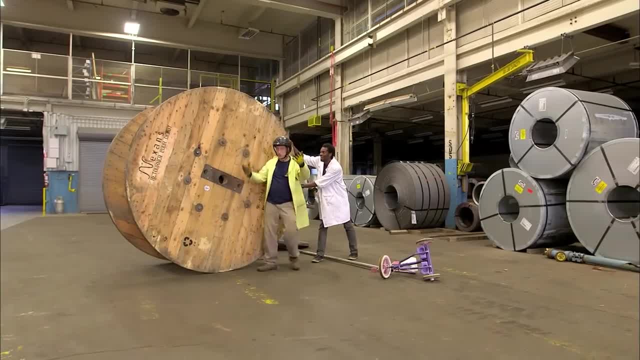 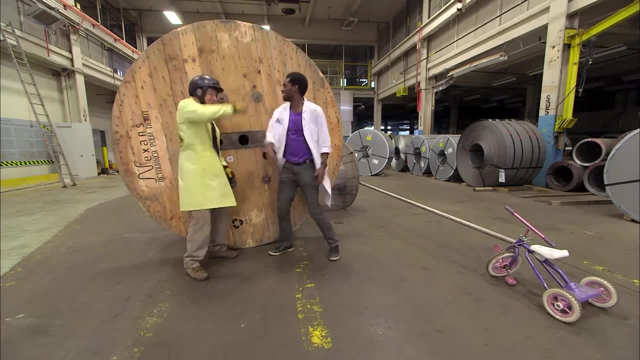 And I thought we would do the same thing with this. What do you think? I think this could generate a huge amount of energy. Okay, so all we gotta do is just build it, just like we built that other one- Just bigger, Except way bigger. 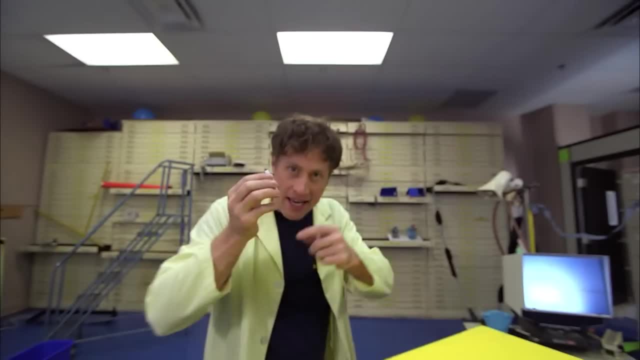 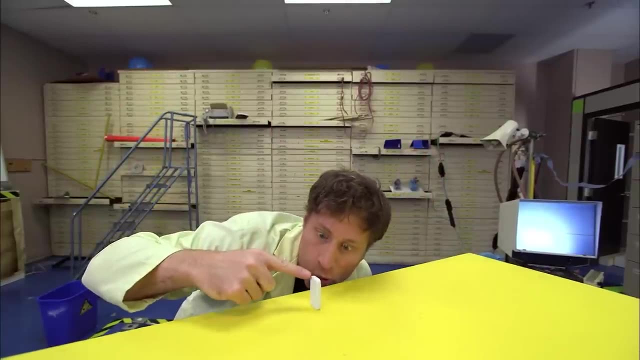 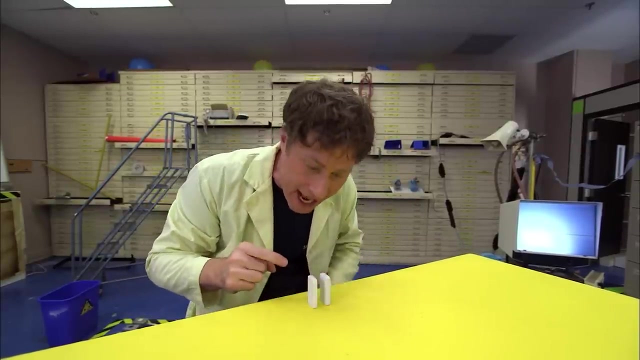 Let's do it. Yeah, Let's do it. When you set a domino on its end, you're giving it potential energy because it can fall, Ooh. And when you put two dominoes together, you can start a chain reaction because that one. 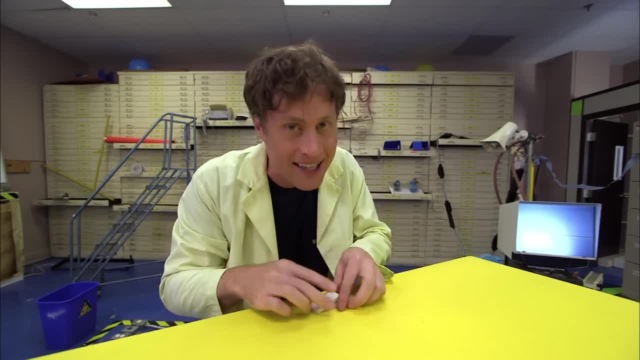 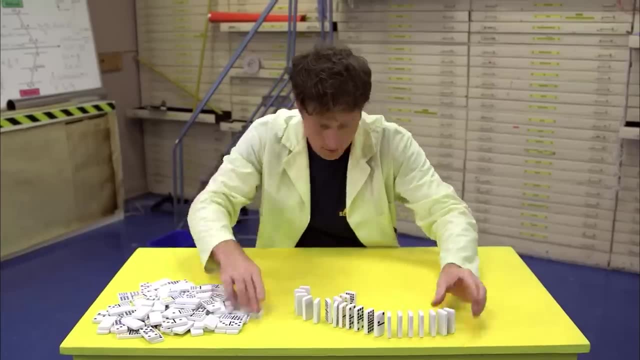 will fall into that one, but it's a lot more fun with more dominoes. Setting up a run of dominoes is a lot of fun, but it takes a flat surface and a steady hand, And if you want to do it yourself, add gaps so if one part falls, it doesn't take out. 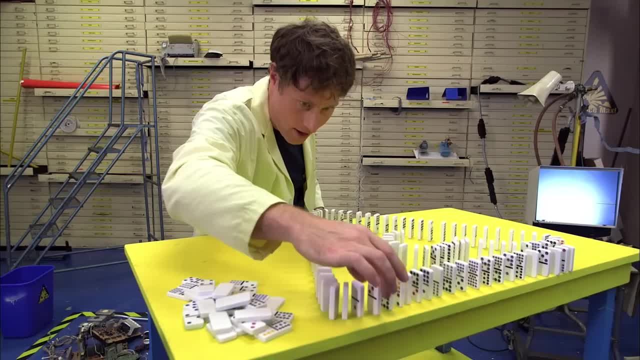 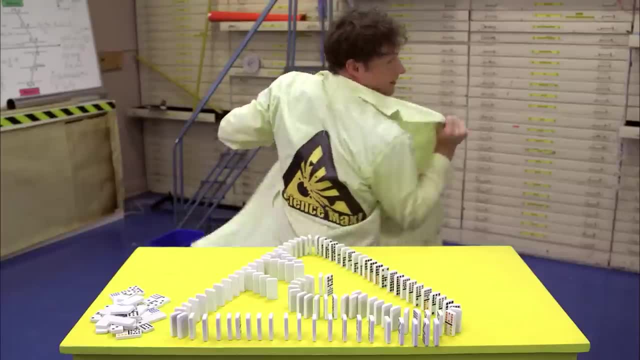 the whole run. Last one: There I had some dominoes left, but I did it. I made the Science Max logo- See Science Max Right, Sort of Let's see how it works. Ready, Yeah, Now it's time to max it out. 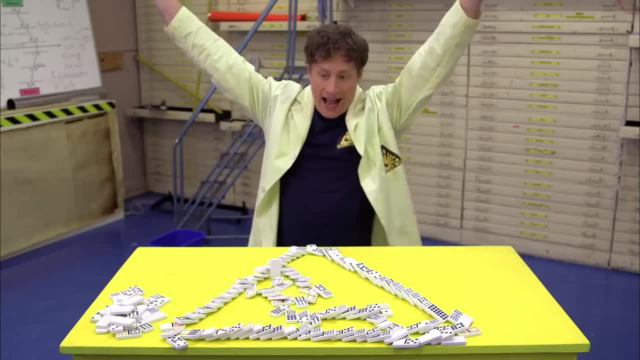 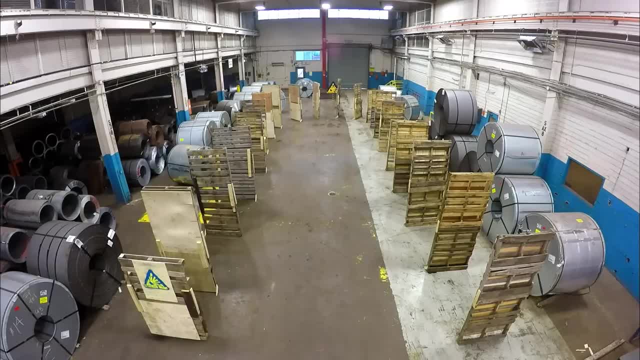 Oh my gosh, Giant maxed out dominoes, Woo-hoo. Even though these dominoes are giant, they're still going to work the same. They're standing up on their ends, which means they've got some potential energy. and when? 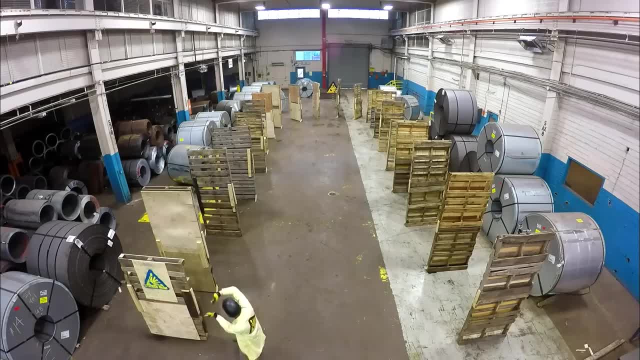 I give this one a push. that potential is going to turn into kinetic energy and it's going to knock the next one, and the next one, and the next one. I hope I don't know what's going to happen, but let's find out. 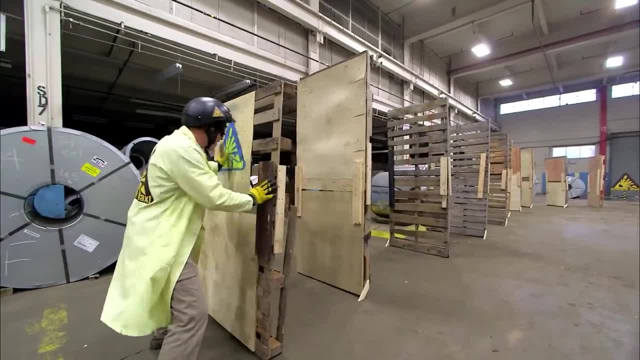 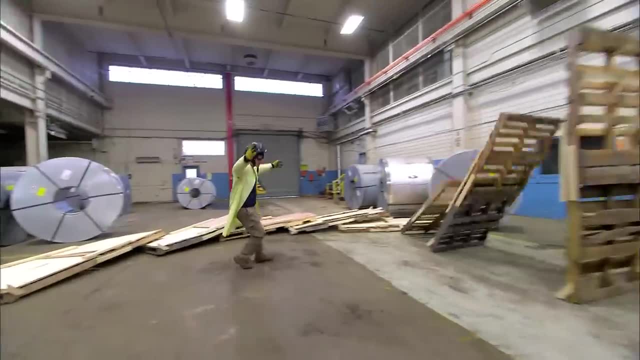 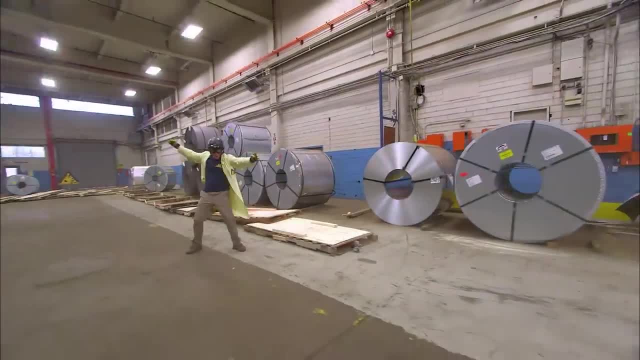 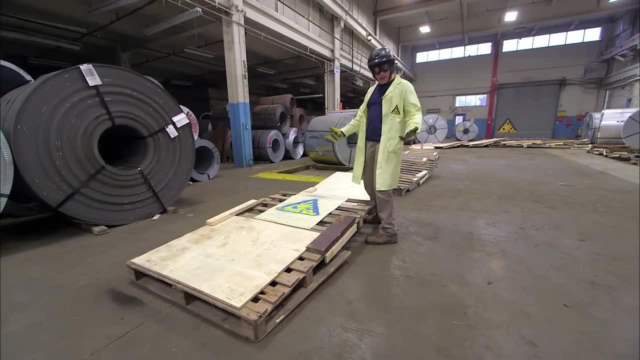 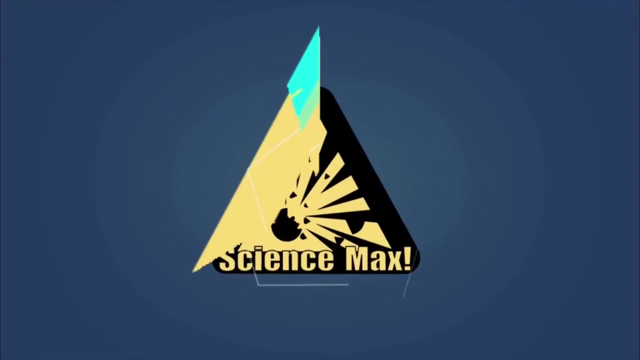 Oh my gosh, Oh Giant dominoes. Yeah, science. The problem is when you use dominoes this big, setting them up again is a real chore. Ugh, This is a mousetrap, but don't worry. 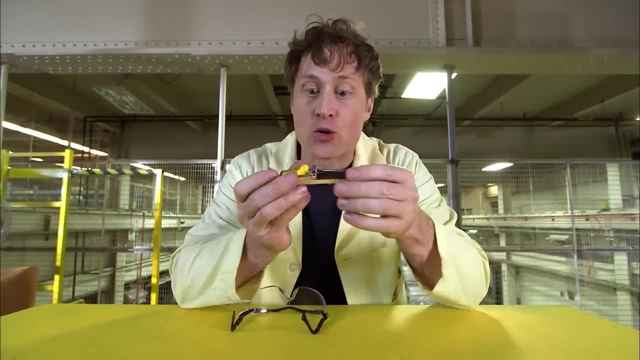 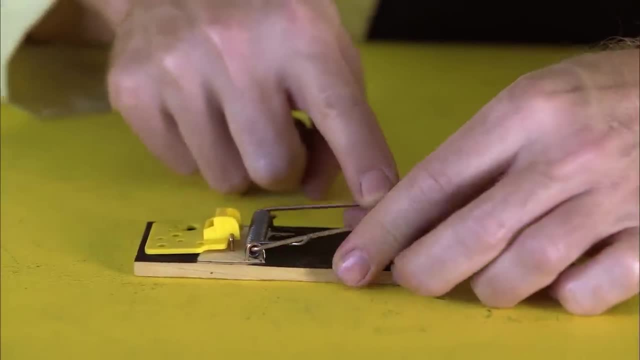 No mice are going to be harmed in the making of this episode. Mousetraps are a great example of stored energy. You see, in order to set a mousetrap you have to push this bar back, and it's hard to do because the spring holds it. 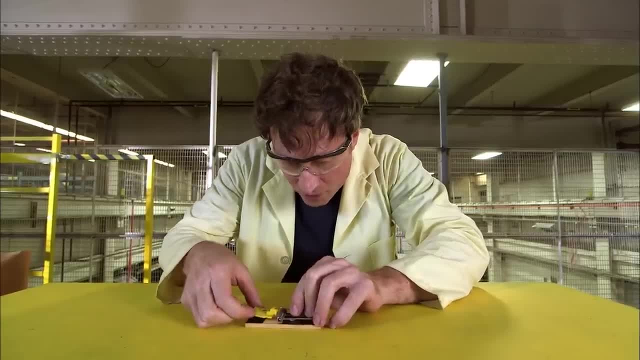 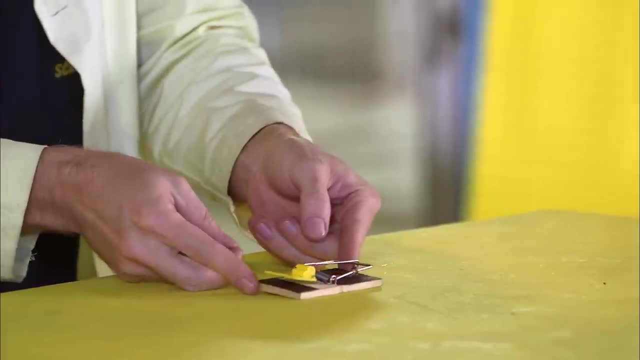 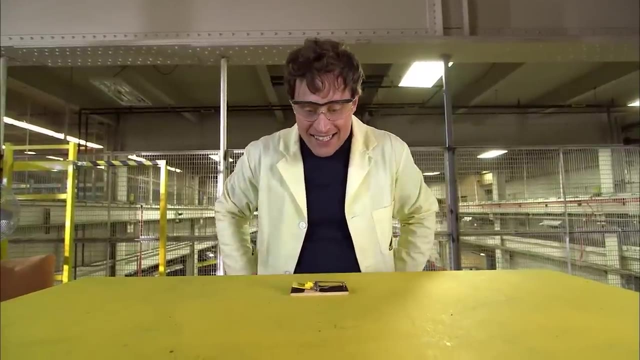 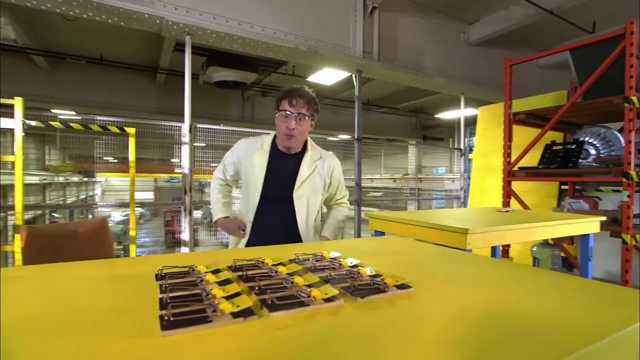 and then you set the mousetrap by putting this little lever underneath this very sensitive trigger and once you have it set, all that energy is stored as potential energy, but it'll go off with just the slightest touch releasing the energy. So what if I had a number of mousetraps? 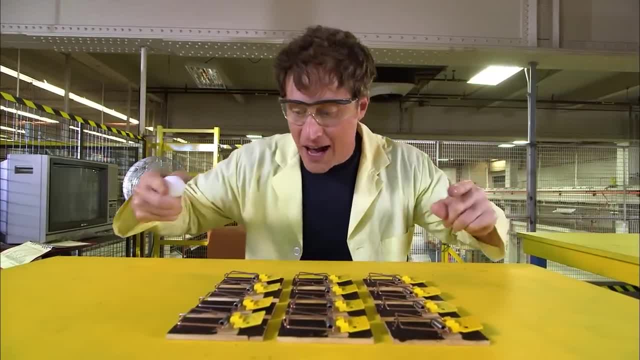 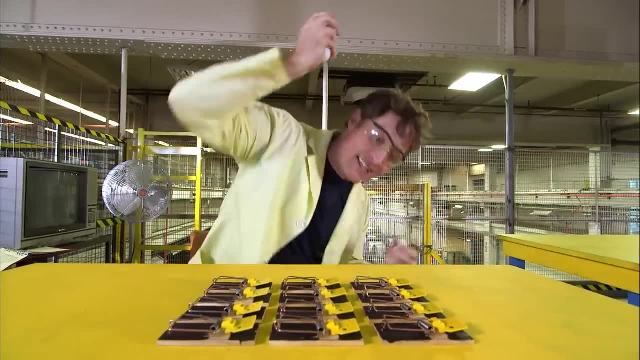 and they're all set and all of that potential energy is stored up, and I dropped a number of ping-pong balls on them. Well then, I could set off a chain reaction where one mousetrap flies and hits another mousetrap. 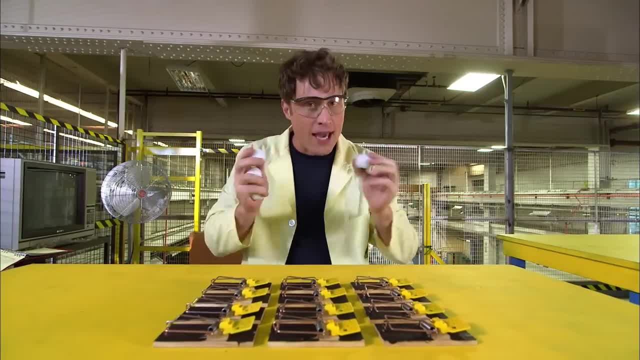 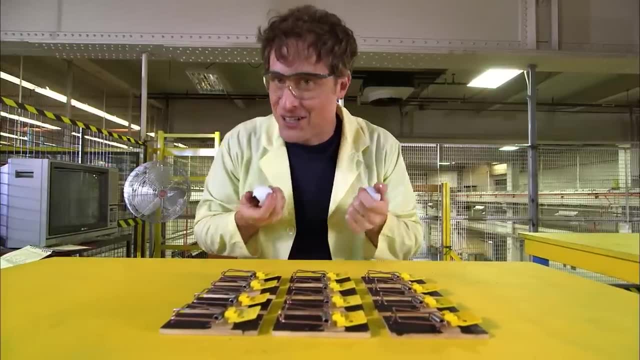 then hits a ping-pong ball and then they all go. Now, this is something you can try at home, but do not set the mousetraps yourself. It can really hurt if it snaps on your fingers, so you should probably ask an adult. 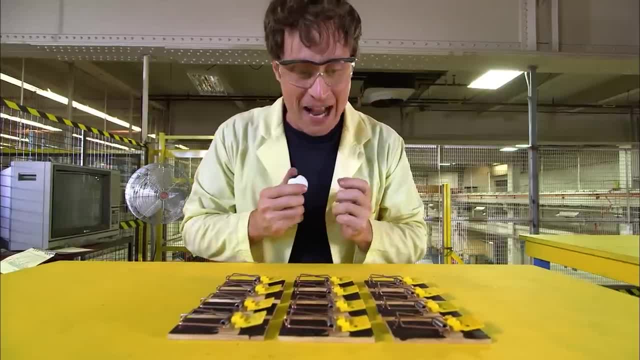 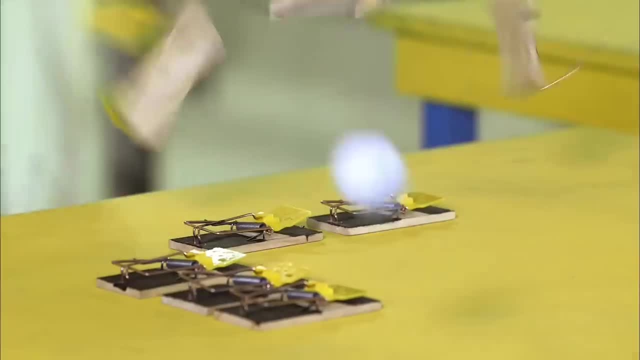 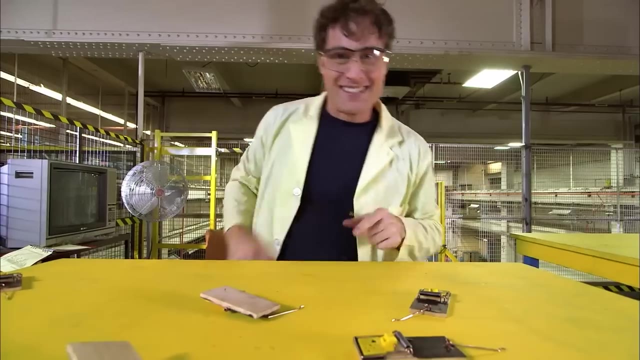 to help you, and then you can see how brave the adults in your house are. Okay, you ready, Here we go. Mousetrap chain reaction. And last one. There we go. And now let's max this out. Let's do it with 90 mousetraps. 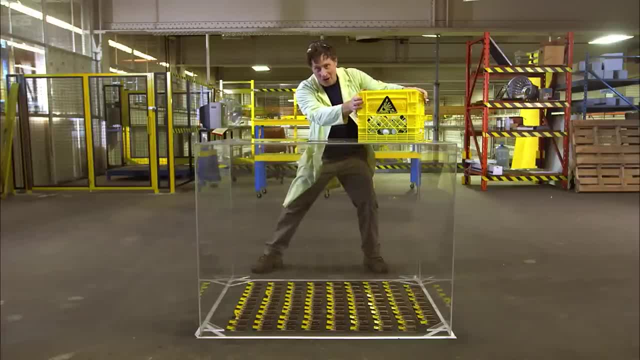 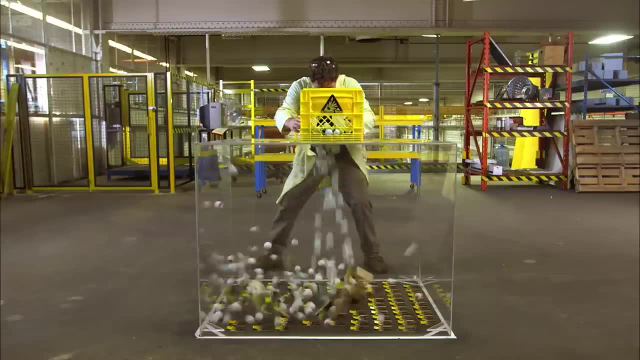 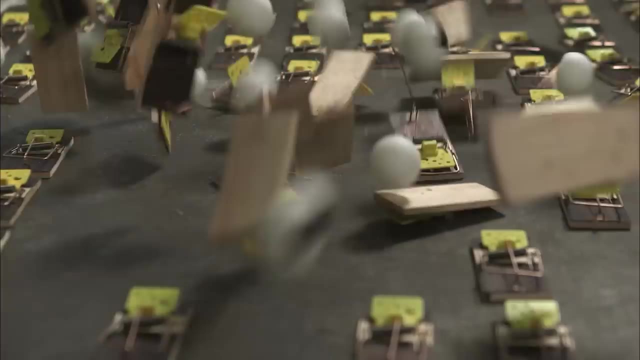 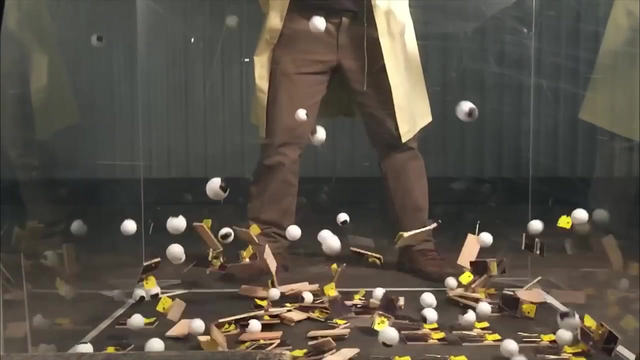 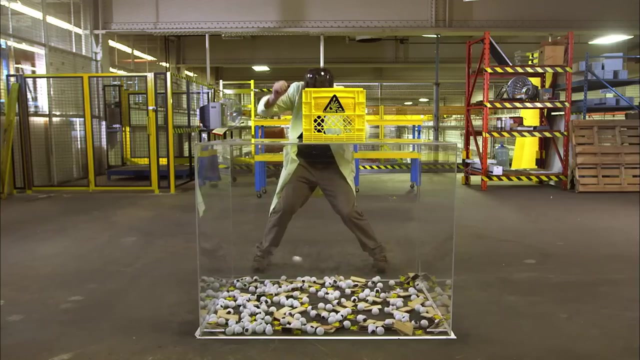 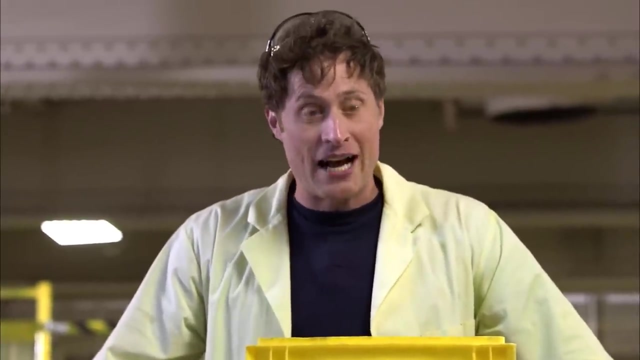 And this is a crate of ping-pong balls. So Let's see, Let's see what happens when we put them together. Ha-ha-ha-ha-ha-ha, There you go, Maxed out, Ping-pong ball, mouse trap, chain reaction. 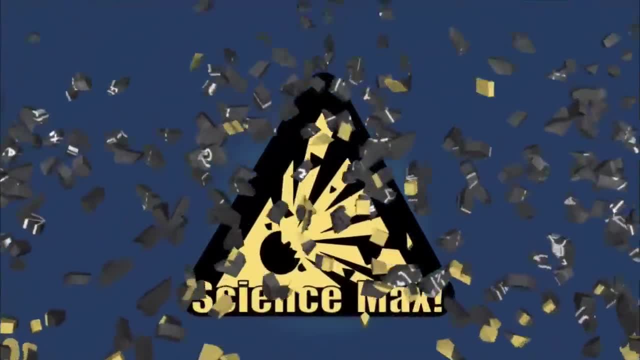 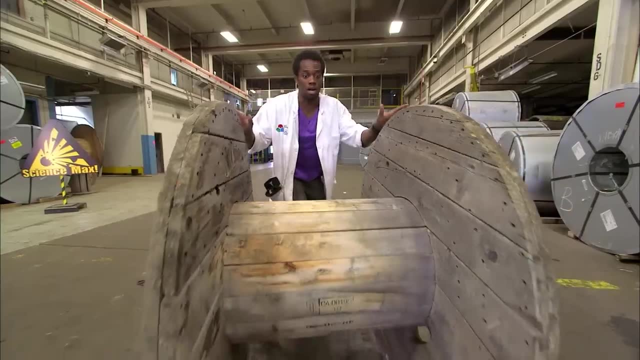 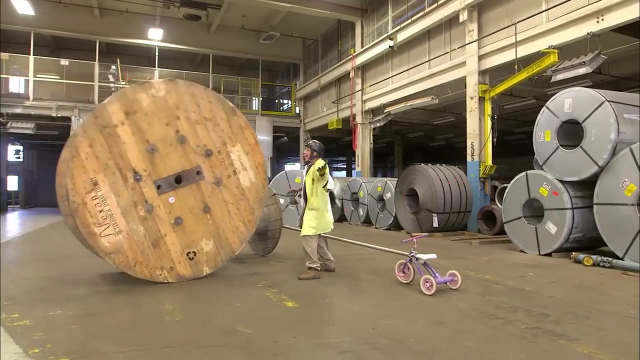 Awesome, Ready, I'm on it. Anthony and I have built a large spool racer. Oh, it's working. It's working And it worked so well. the only option was to go bigger. What is this? This is an industrial cable spool. 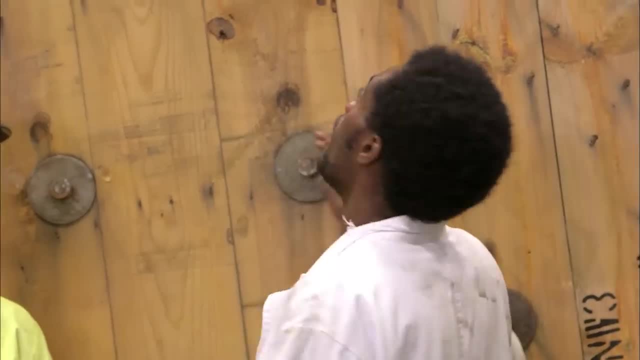 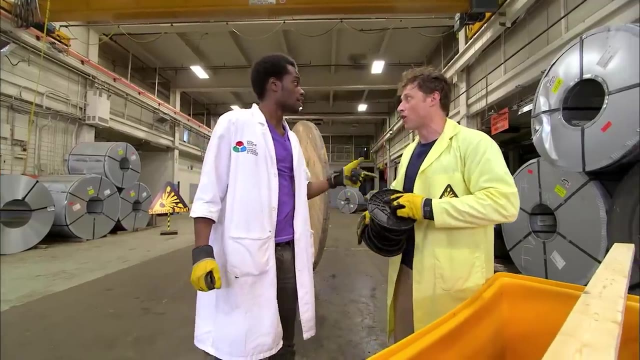 and this is the biggest size that they make. I think this could generate a huge amount of energy. Building our giant spool racer is the same process as the other builds, So the steps are exactly the same, but on a larger scale, And this time we're gonna use, obviously, the large spool. 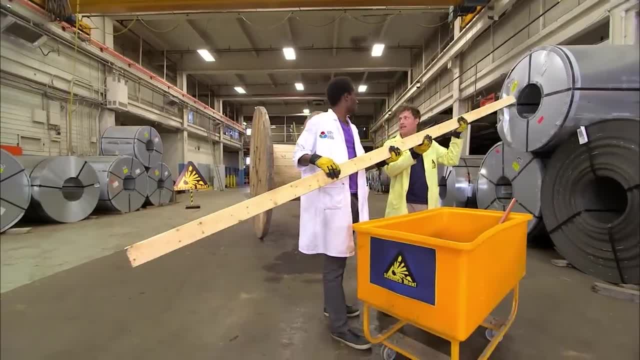 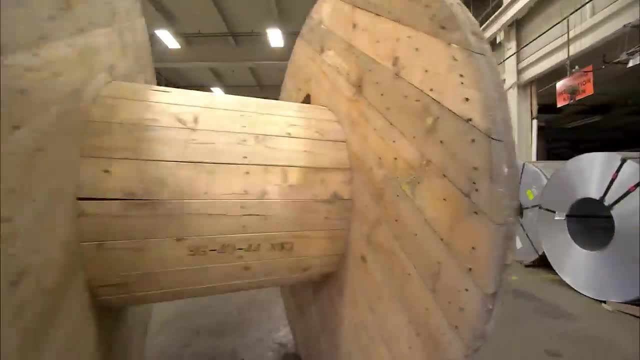 and we're gonna use this two by four as our pencil windy thing. Coil some bungee cord, feed it through Ready Yep. Okay, Here it comes, There we go, Got it. Ha ha, yeah, Add a washer and a long. two by four. 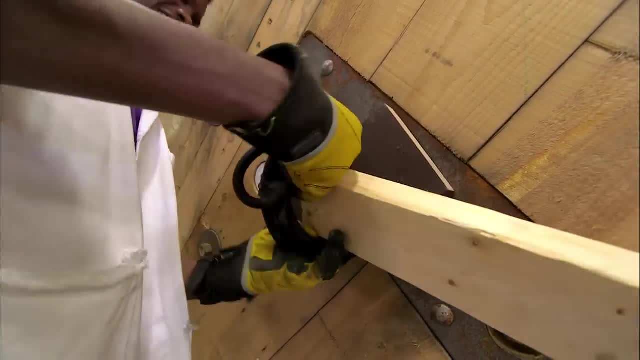 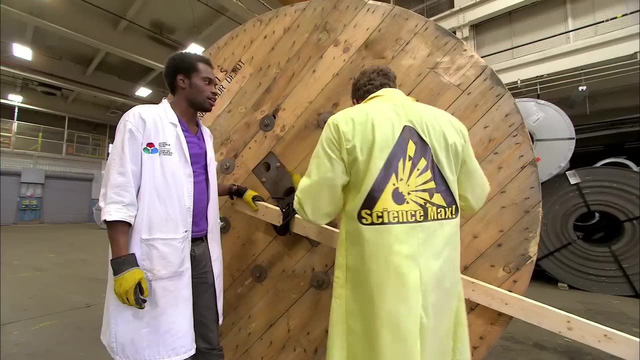 to act as our pencil. And now we stick the giant two by four inside the coil, just about: Yeah, we got it, There we go, And we're ready to try it out. So it looks like we're ready to go. 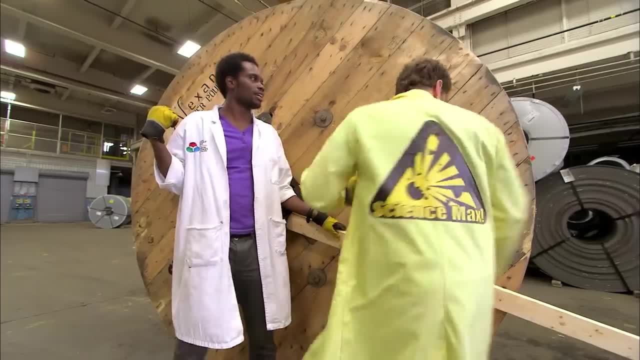 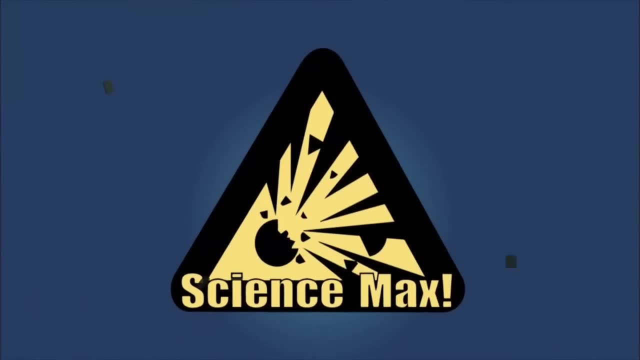 Yeah, exactly. Do you wanna do it in here or you wanna do it outside? Oh, definitely outside. Okay, let's go. Yeah, okay, cool, Yep. Oh, it's heavy, All right, Batteries are great at storing energy. 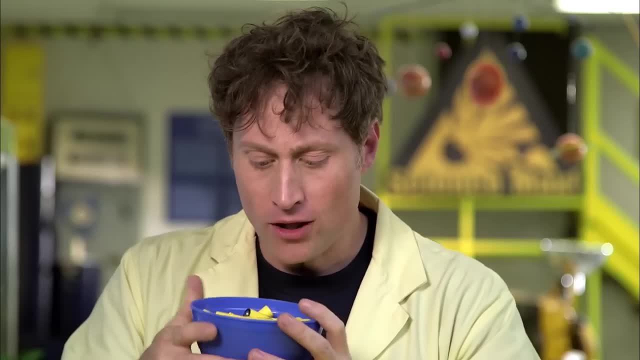 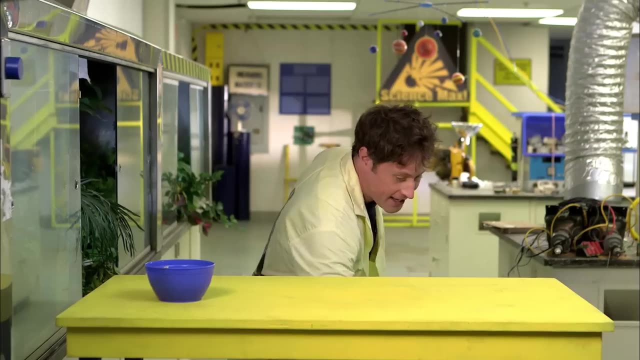 They store electricity Batteries. But if you're like me and you have a whole bunch of batteries and you don't remember which are the good ones and which are the dead ones, there's a trick that you can use to find out. Get a frying pan or a brick or a concrete floor. 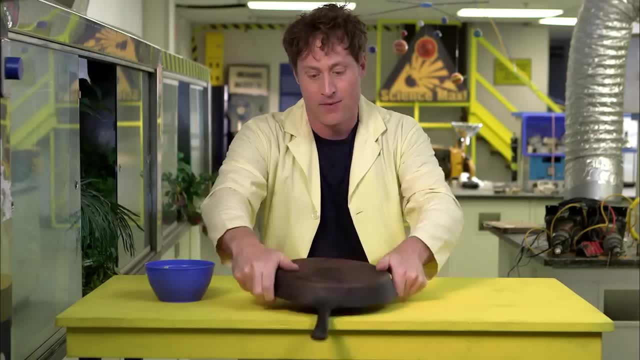 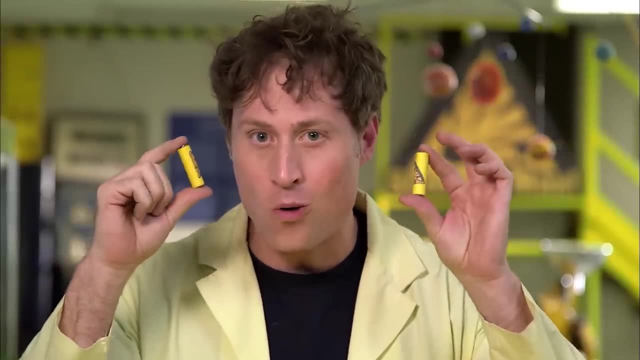 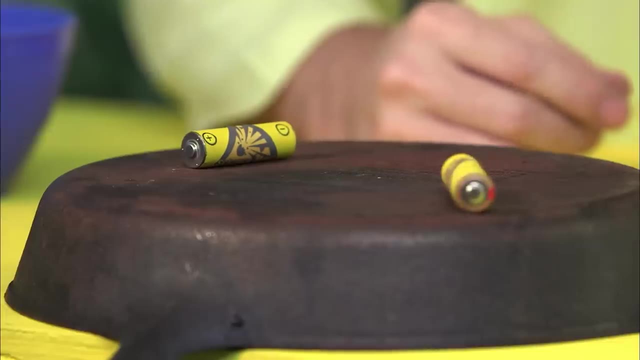 or something else. that's very, very hard and an adult's permission. Here's the secret: Dead batteries will bounce, and batteries that still have some life in them won't Watch. Good battery, Dead battery- Now it's a little hard to see. 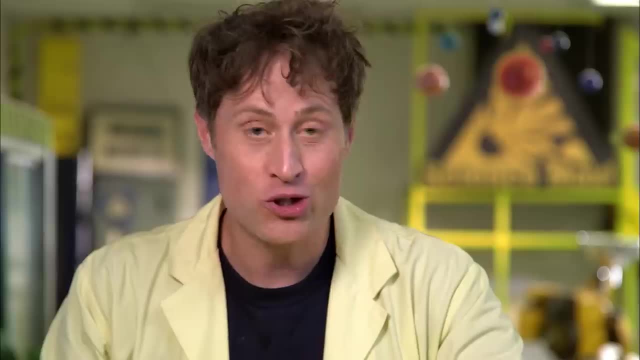 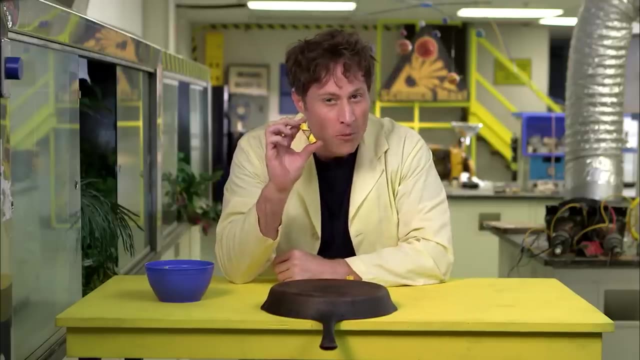 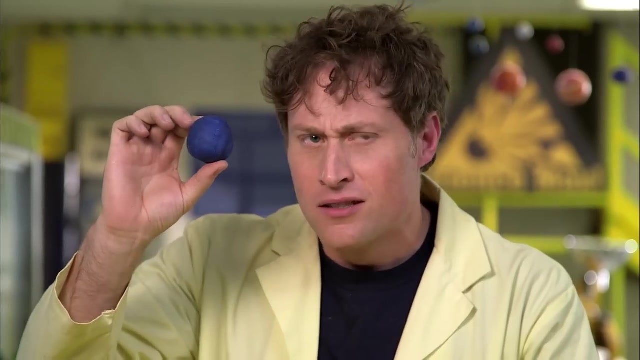 but listen. One hit, Two hits. Here's what's going on. See, batteries store electricity in the form of a gel, sort of like modeling clay. This is modeling clay, fresh from the fields where the pits, the mine. 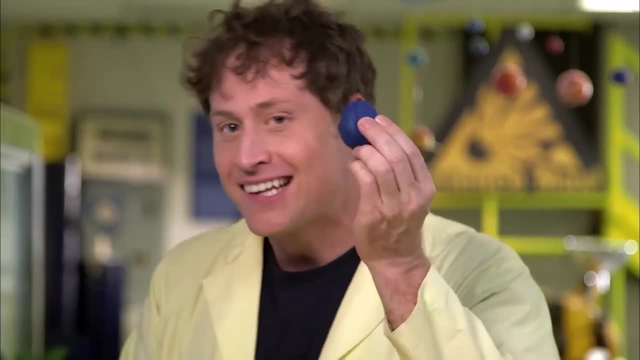 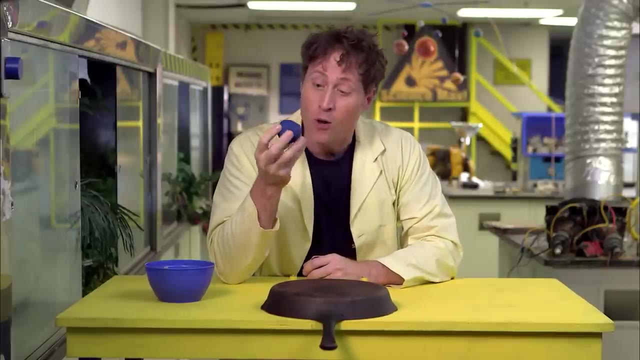 wherever modeling clay comes from- and this is modeling clay I've left out for about five days, so it's all dried up and hard. Now, when modeling clay is new, it's all wet and soft and when you drop it it doesn't bounce very well. 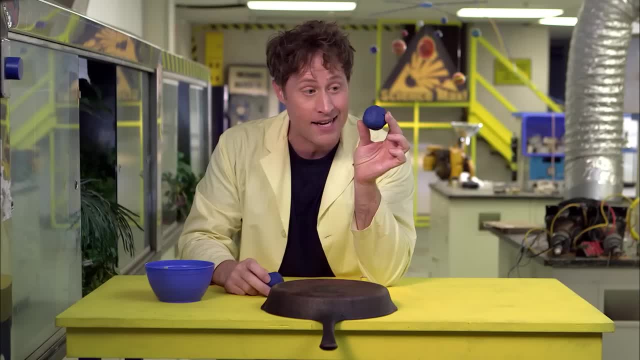 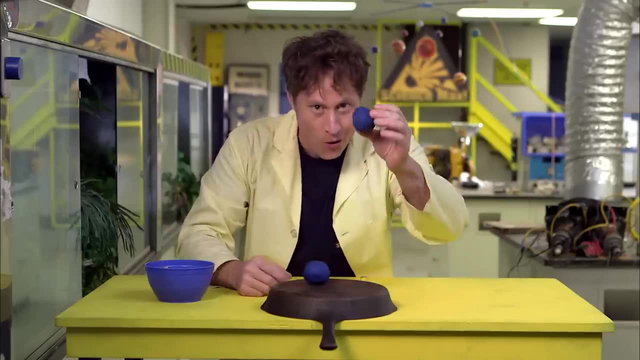 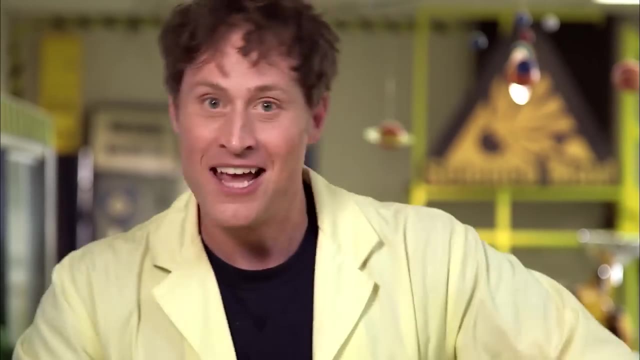 I've left this piece of modeling clay out to dry for about five days Now. it's all dried up and old and it bounces- New, Old. So same thing with the battery: Good batteries won't bounce and bad batteries will. 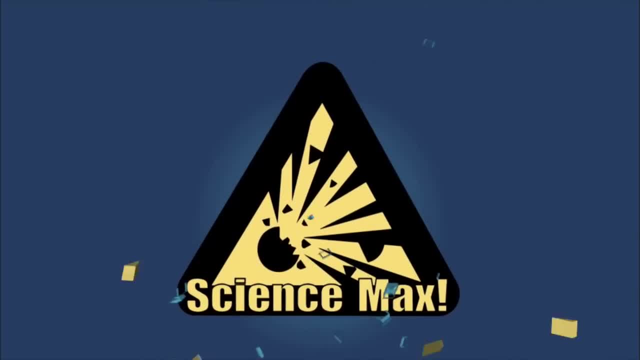 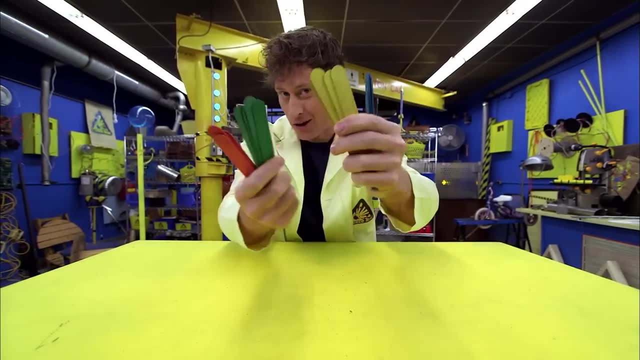 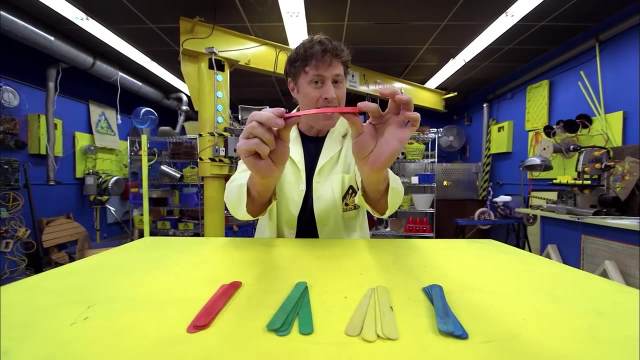 Science. Here's a fun chain reaction. You can do with popsicle sticks or craft sticks, because these ones are a little bit wider than popsicle sticks. It is because these kind of sticks are slightly bendy, and when you bend them and put them together in a pattern, 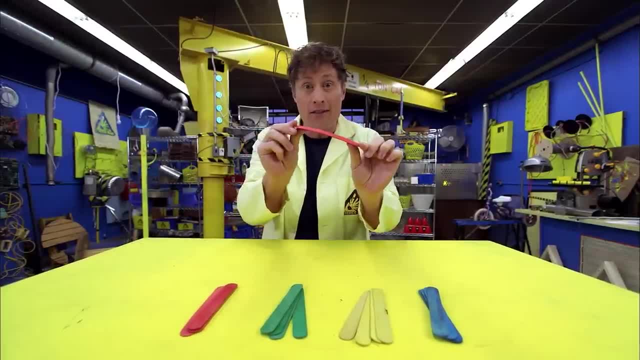 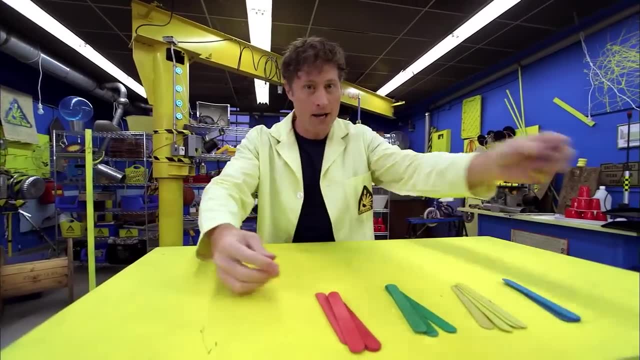 in a certain way you can keep them under tension, and then they want to snap back and then they'll fly. So here's how you make the pattern Ready: You take a popsicle stick or a craft stick and you put it down on the table. 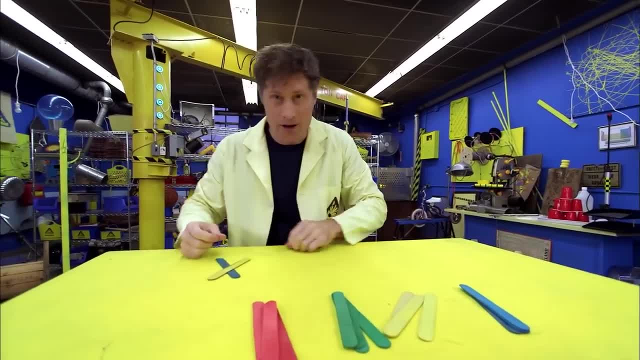 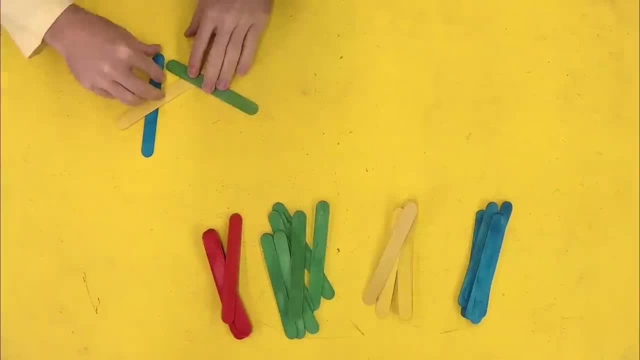 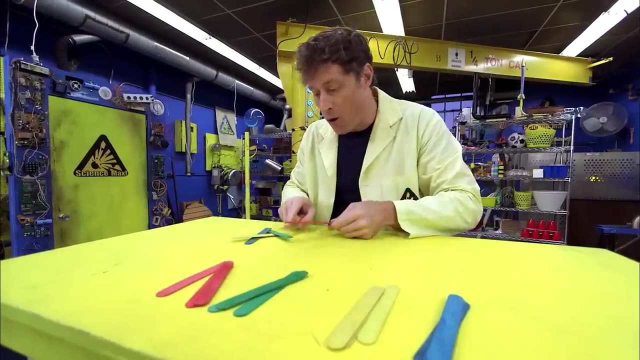 I know, okay, It's a slow start And we take another one and put it across. Now comes the secret. The secret is over and then under. You want to put it over one and then under another, Like that, And then this one over under. 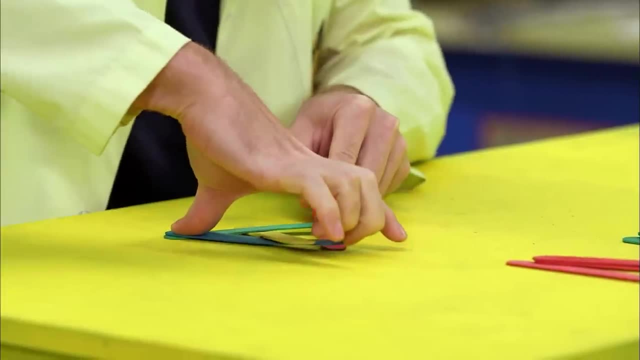 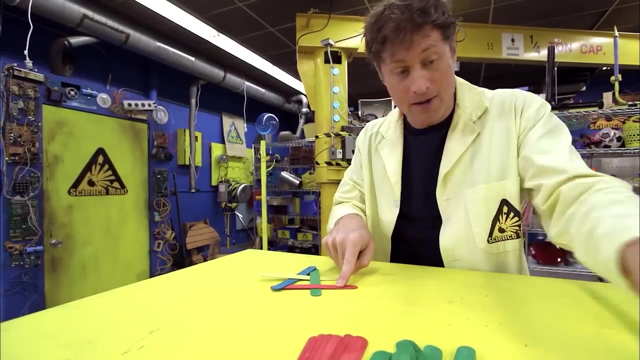 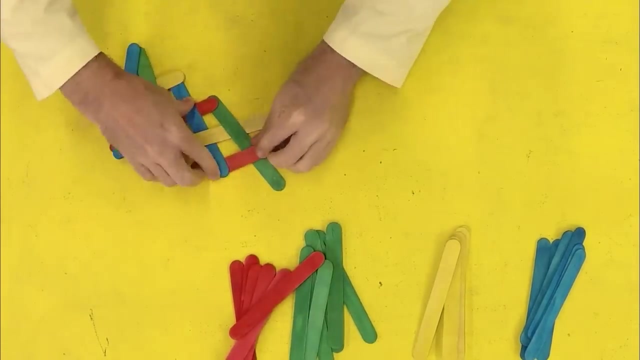 Put it over the one that looks like it's the top stick and under the stick that looks like it's the bottom stick, And then it starts to hold tension. It starts to hold the potential energy. It's a nice pattern. Each stick goes over and under the two sticks at the end. 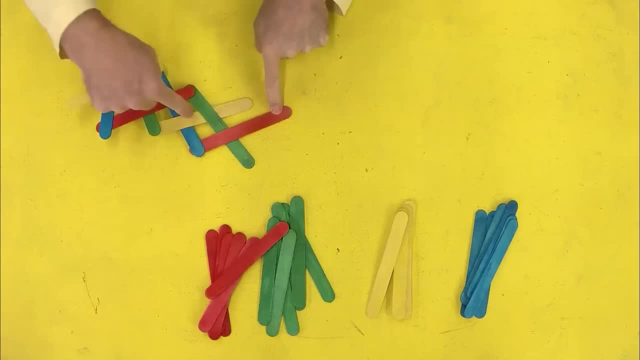 Now here's the trick: Soon as this one lets go, then that one will let go, then that one, then that one, then that one, and that's how you get the chain reaction. They all start flying up. So you have to build it with never letting go. 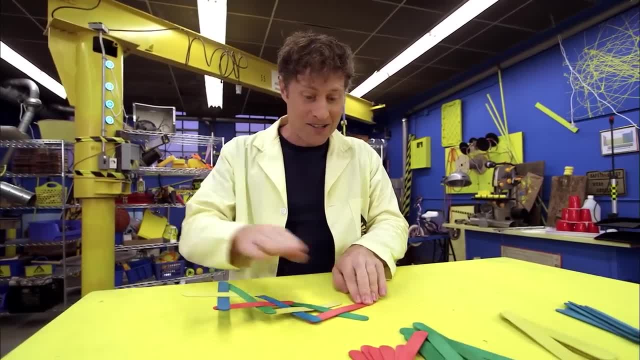 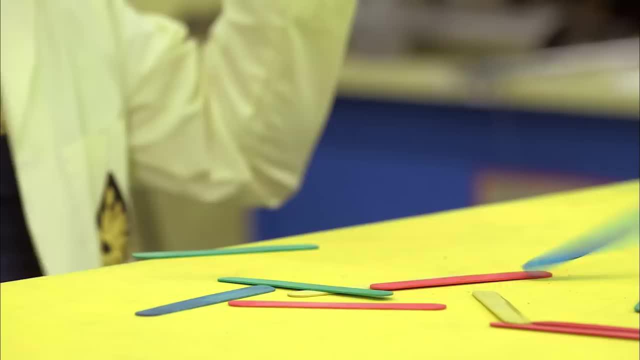 of that last stick. You've got to always remember to keep a hand on it, or else you'll have to start again. Okay, so you ready. You want to see me? let it go? Here we go. I know that isn't so great, because it's better. 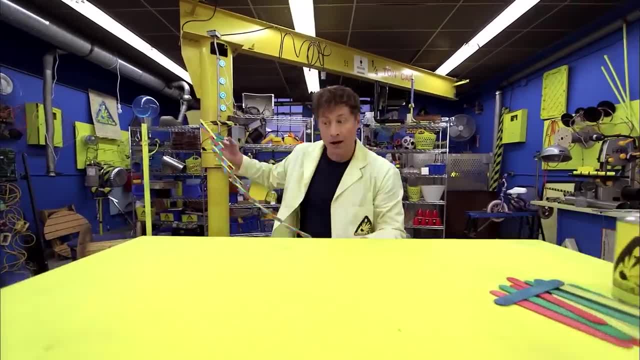 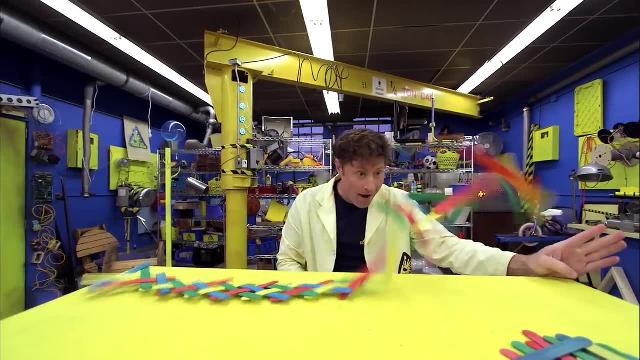 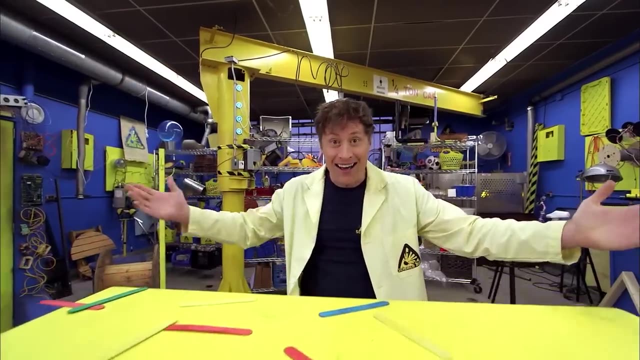 if it's a longer chain, I have a longer chain. I've got a binder clip on this end. keeping the craft sticks together. Ready, Three, two, one Wah. Release of kinetic energy from the potential energy of winding. all the craft sticks together. 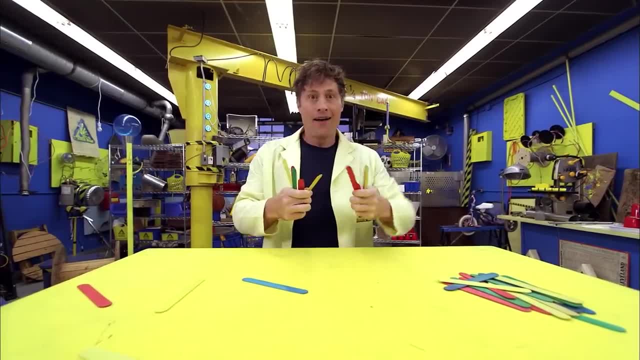 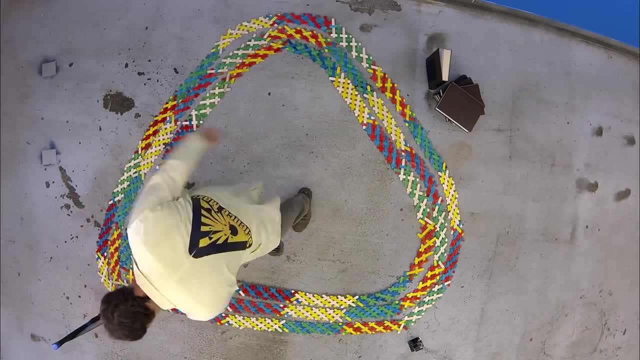 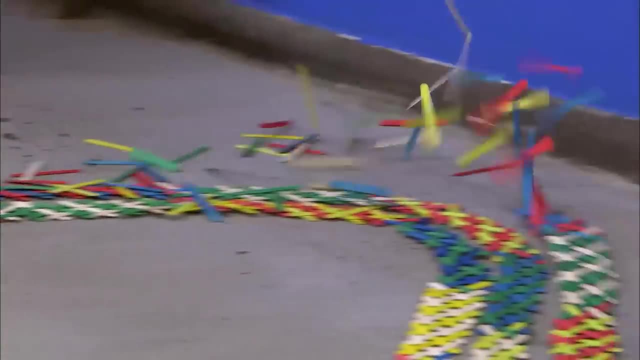 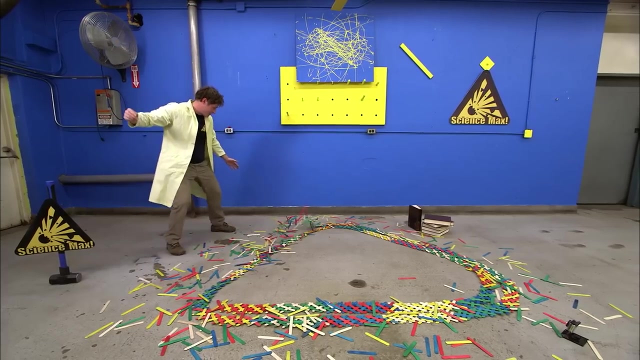 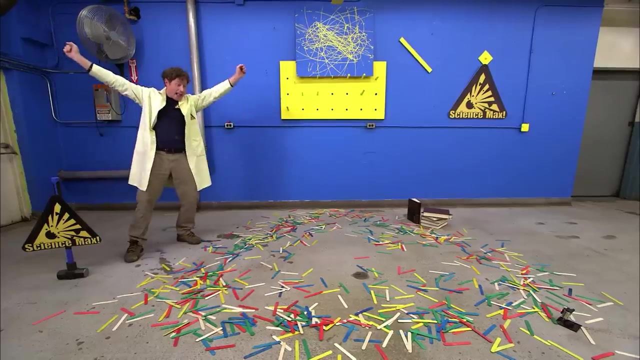 Fun and you can totally do it at home. Now let's max it out. Behold Almost 800 craft sticks in a long, nicely designed triangle. Ready, Two, one, Yeah, Craft stick chain reaction. I'm going to go get something to clean this all up with. 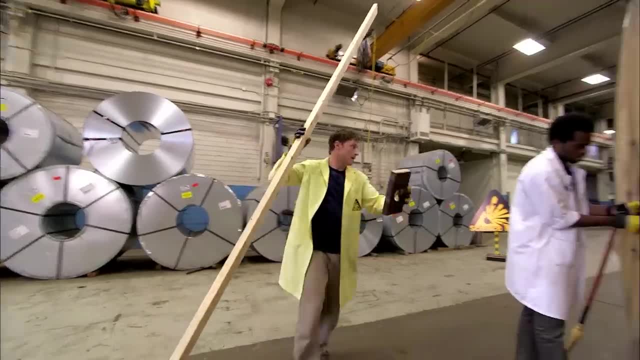 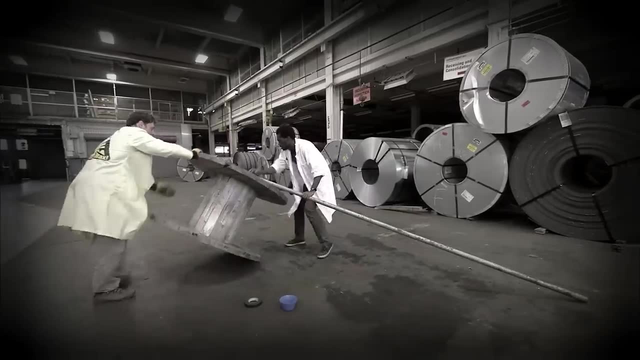 All right. so Anthony and I have built a giant spool racer and have taken it outside to try it out. In order to wind it up. we flipped over the last version on its side, But this spool weighs 200 kilograms. 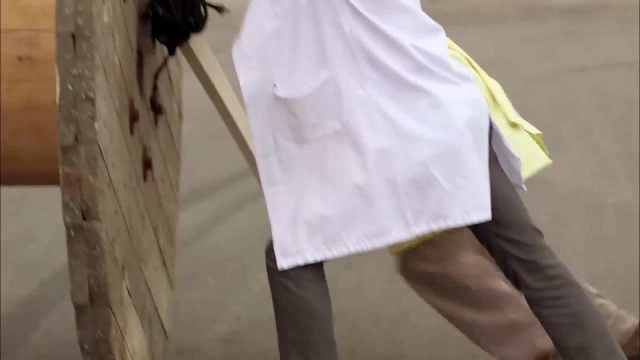 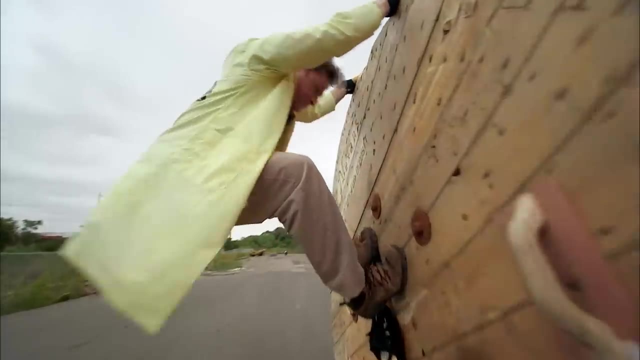 Easy to roll, almost impossible to flip over. Come on, get it. I don't know how to do it, but I'm going to try it. I don't know how to do it, but I'm going to try it. I'm going to try it. 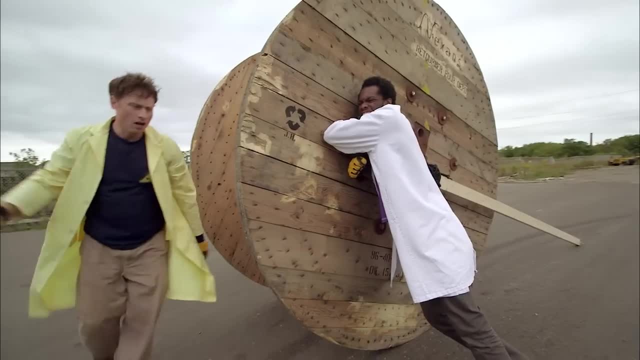 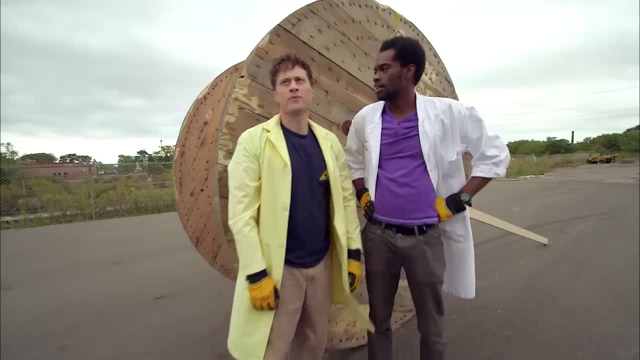 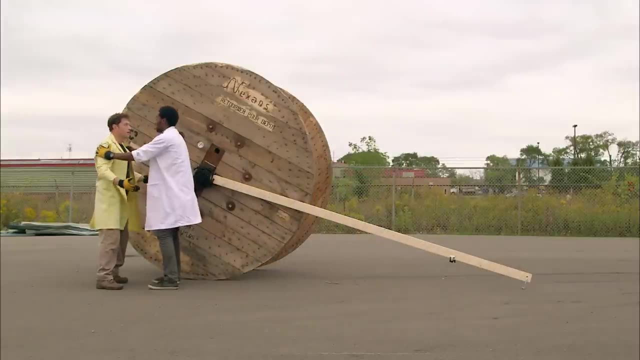 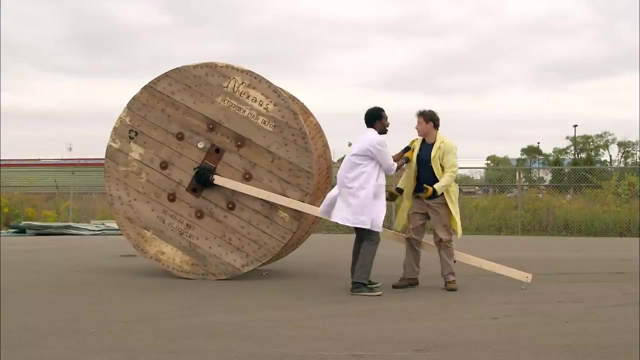 Yeah, We should have thought of that before. Well, I'm sure we'll think of something. Uh, So, Anthony and I thought about it. What? And thought about it, Oh And thought about it, I got it. What? 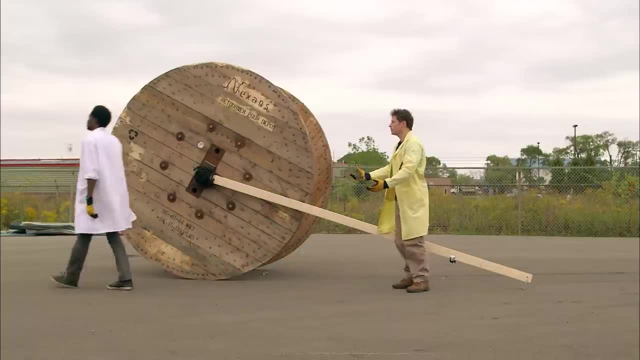 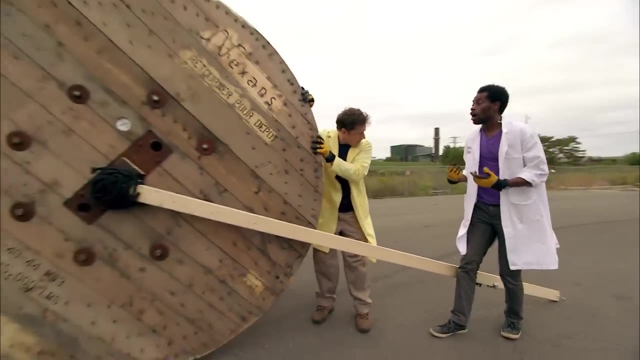 No, No, But you. And the answer finally dawned. What if we roll it this way? Because then that way it would wind it up. right, That's brilliant. By rolling it backwards, we wind up the bungee cord in one direction. 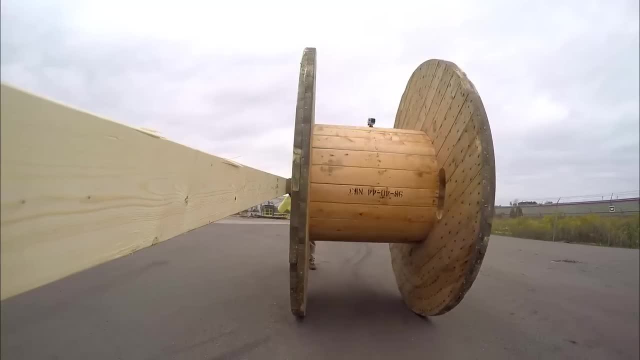 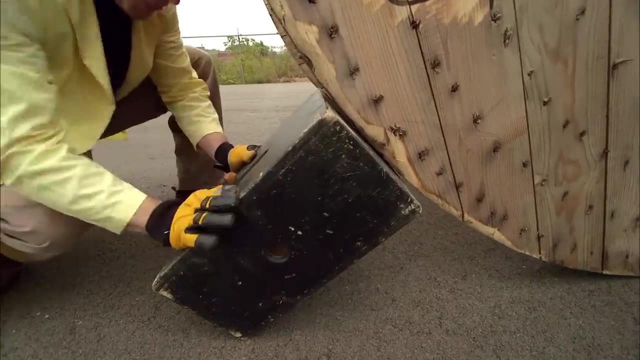 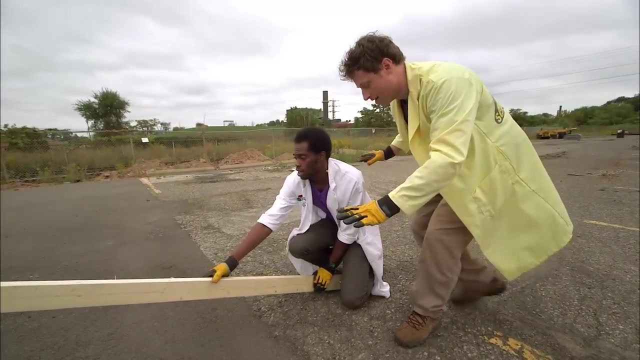 which will make it want to unwind in the other direction. Anthony and I roll it across the parking lot to get it wound up tight. I don't think I'm going to hold it anymore. Okay, Okay, Let go. Uh, Okay, it's wedged. 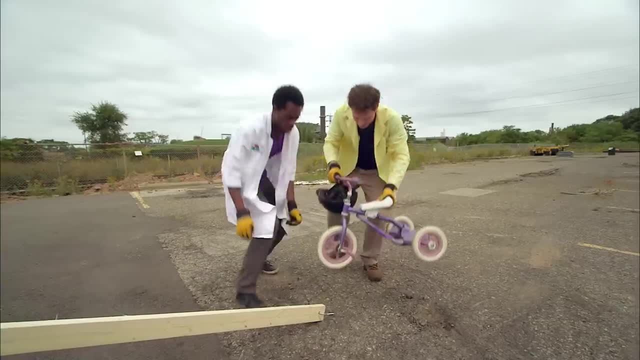 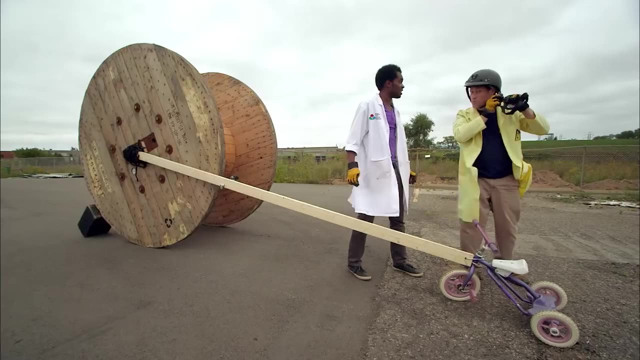 It worked All right. one more thing. I'm going to hook the trike up to this one as well, Okay, Okay. So right now it's all wound up, and when it gets moving, that potential energy in the coil. 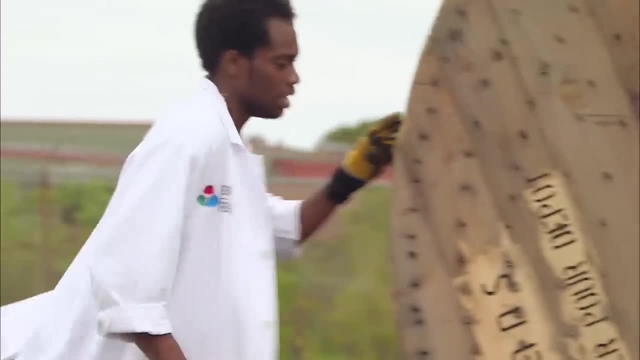 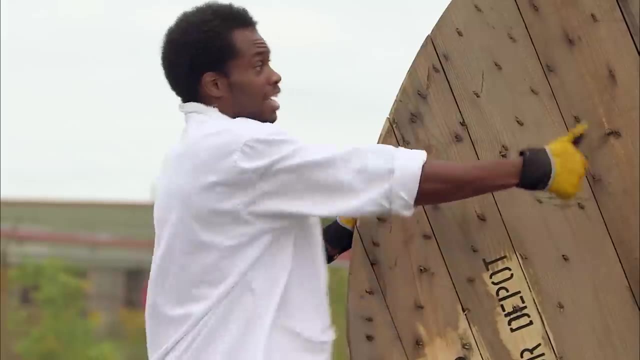 will turn into kinetic- Exactly, Kinetic- energy. Now, just in case you're tempted to try this at home, I need to tell you: do not try this at home. We're trained professionals, right? Uh, yes, Yes. 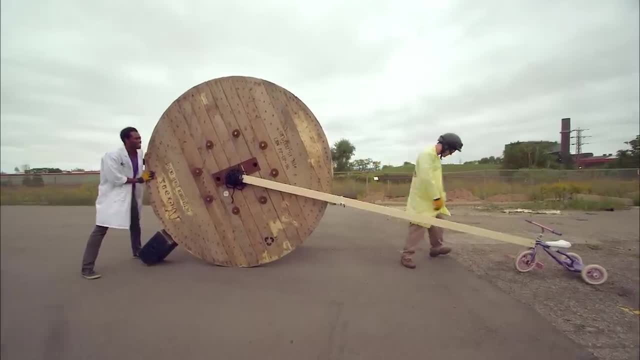 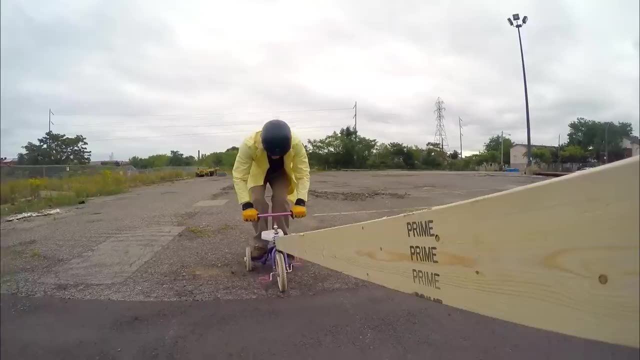 Well, as much as anybody can be trained for this, because no one really does this. Are you ready, Ready? Okay, here we go. Oh, It's working, It's working. Yeah, Sure enough. all the potential energy we stored in the bungee cords starts to unwind. 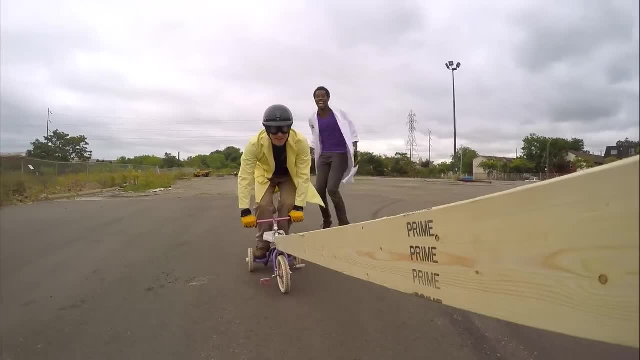 which rolls the spool and pulls me along behind it. What's more, that big, heavy spool has a lot of momentum, Yeah, So when it gets going fast, it just wants to keep moving. It wasn't long before I had to jump off. 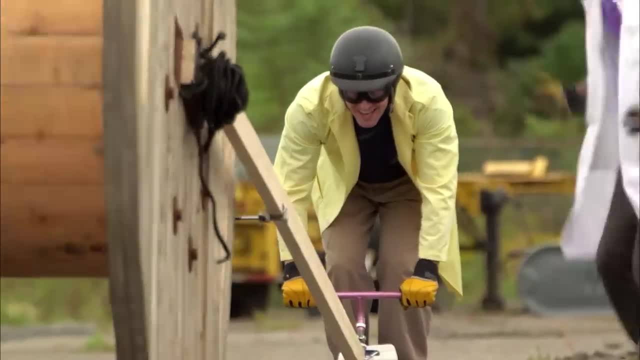 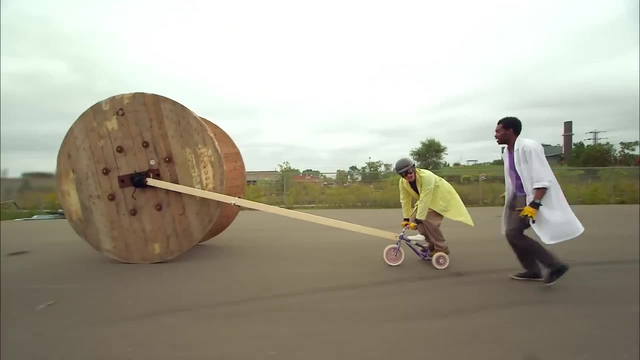 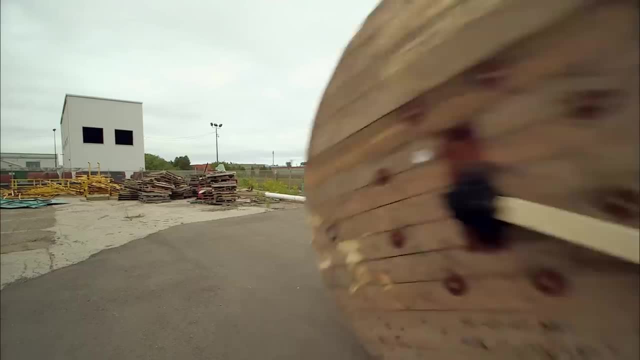 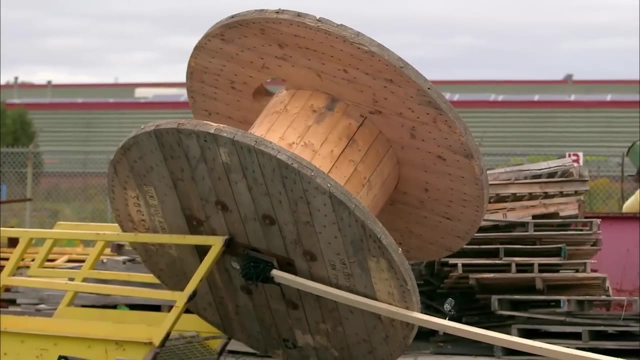 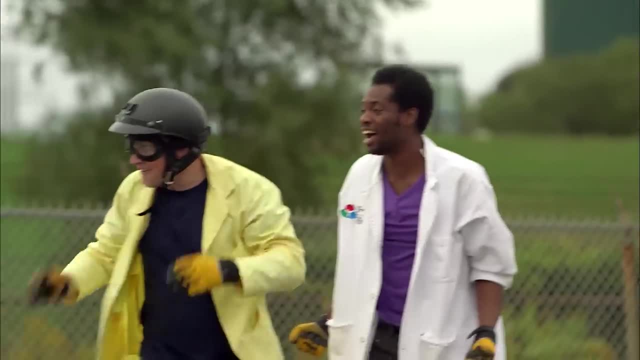 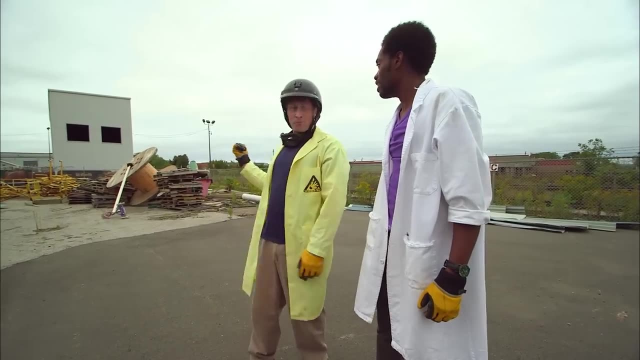 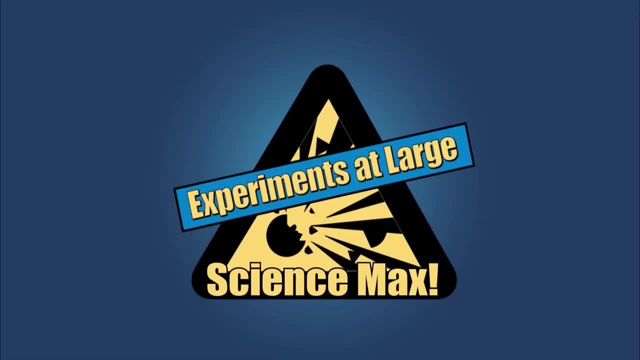 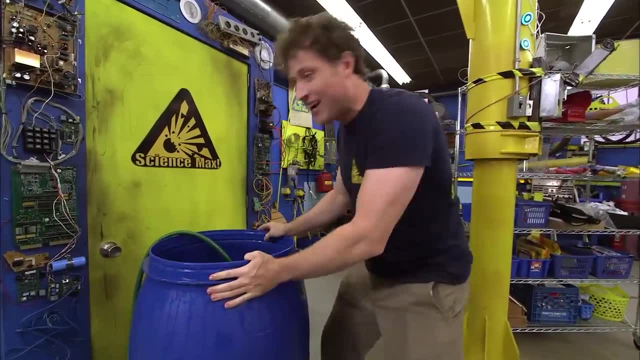 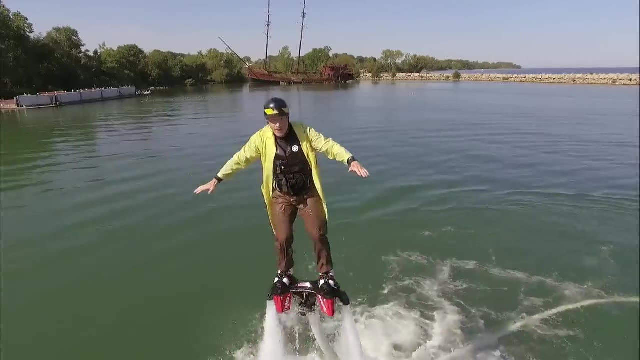 That was amazing. All right, That had a lot of kinetic energy. That was a ton of kinetic energy. There you go. Science Max, experience at large, massive spool racer- Your turn next. Yeah, Water is very heavy. Pressurizing water to make a water-powered car, water pressure pumpkin, carving, water flying and more. 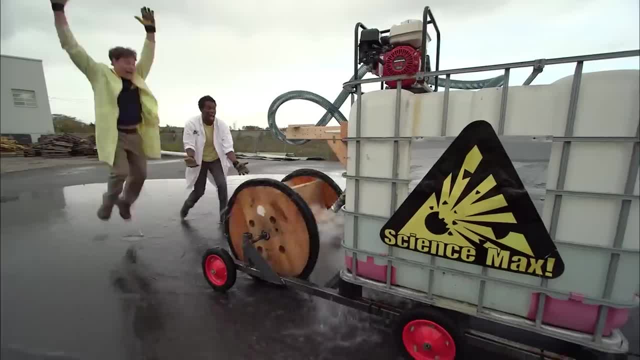 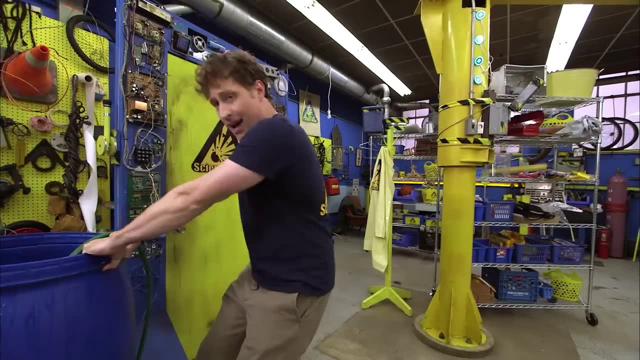 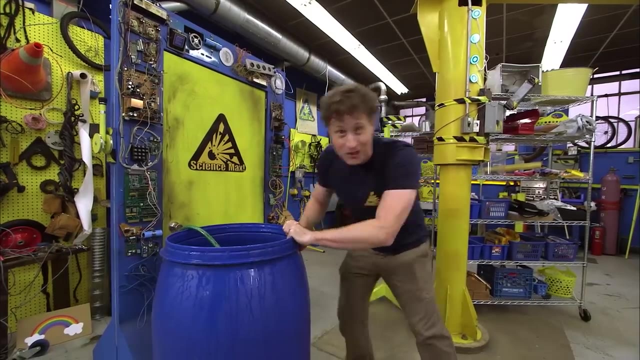 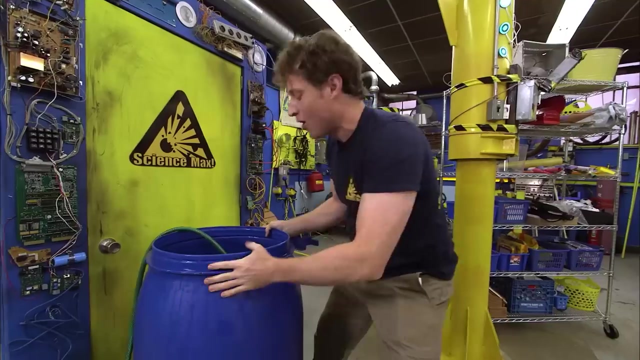 All on this episode of Science Max Experiments at Large. Greetings Science Maximites. Welcome to Science Max Experiments at Large. My name is Phil. Today we're going to be looking at water, but water is very heavy. 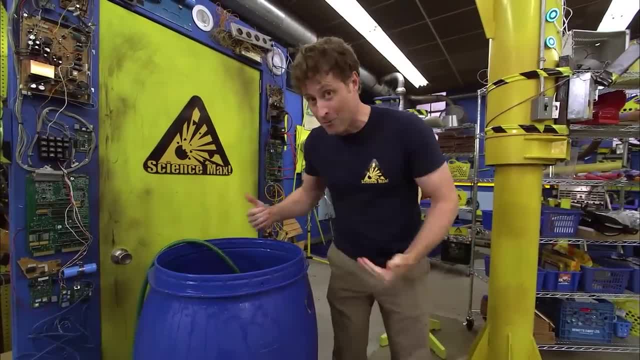 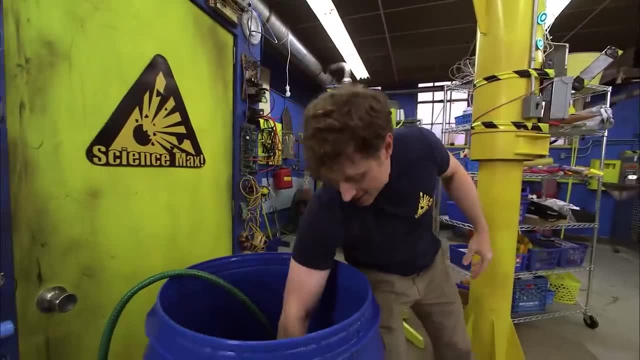 But that's okay, because we need it to be heavy for this experiment to work. I don't know if I need that much of it, though Maybe I can get. Oh, here we go. Yeah, that's probably all I need. 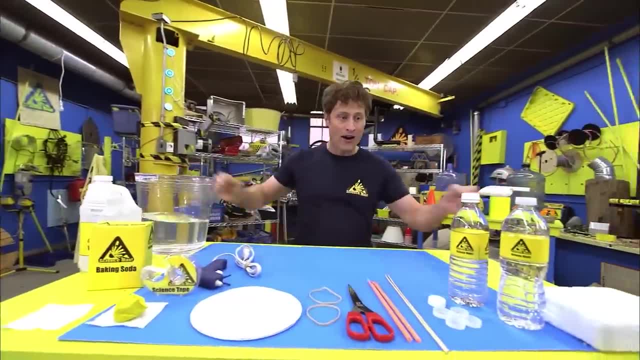 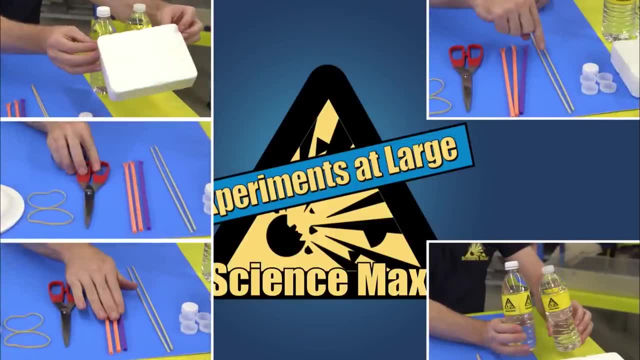 Today we're going to be building a water-powered car. You'll need a base for your car like this: Styrofoam, water bottles, shish kebab skewers, straws, scissors, elastics, paper plates, tape, a square of paper, towel, modeling clay, vinegar, baking soda. 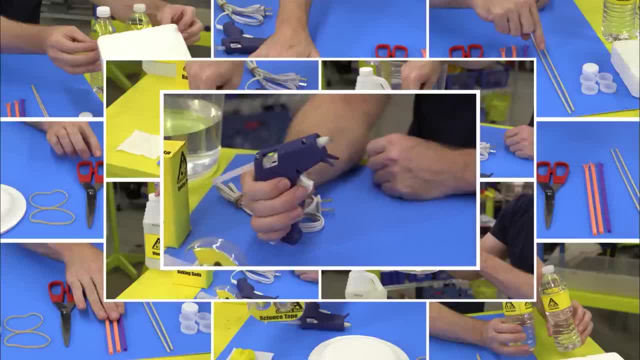 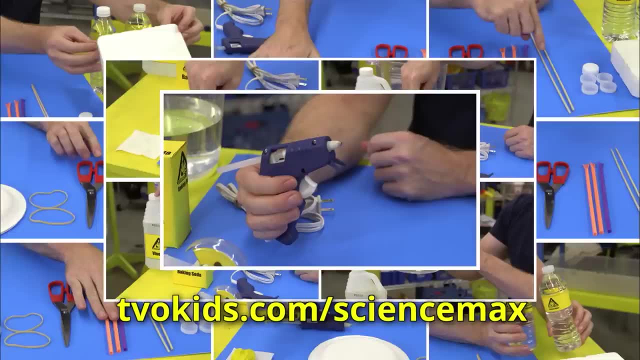 water and glue or a hot glue gun. if you have an adult to help you- and, Yeah, I know this one is pretty involved- That's why you should go to the website for step-by-step instructions. Take your paper plates and glue two together to make a wheel. 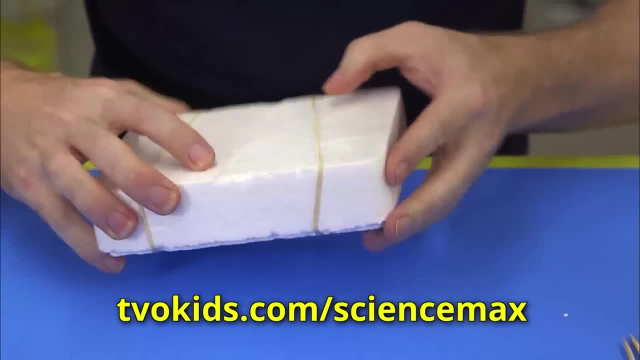 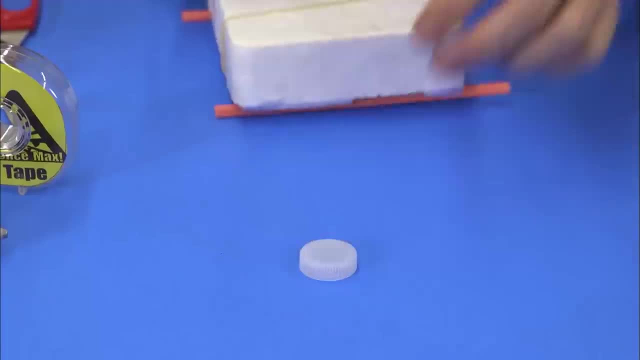 Then make three more. Wrap elastics around your base and then tape straws on the bottom. Trim them down, maybe about that much. Then take your shish kebab skewers and push it through a water bottle cap to make a hole. 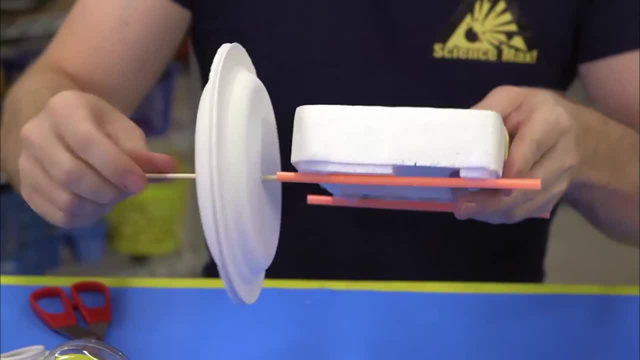 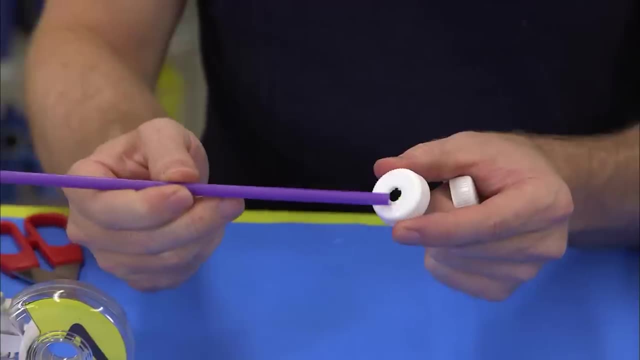 Then stick one wheel on, put the skewer through the straw and do the same thing on the other three sides. Then take the water bottle cap and get an adult to help you make a perfect hole in it so that it fits your straw. 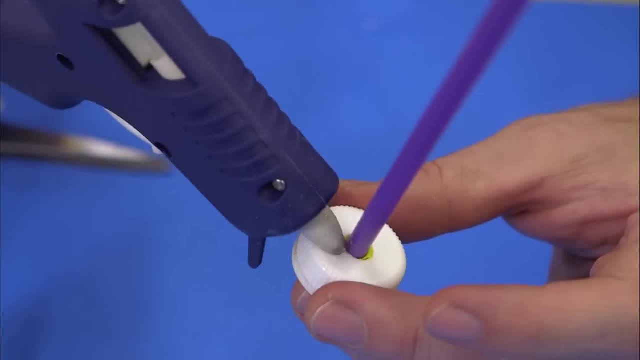 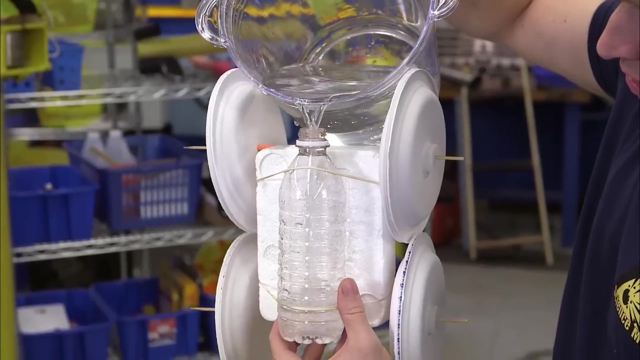 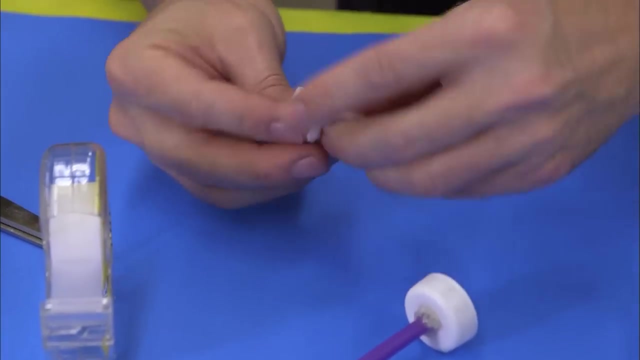 Then use some modeling clay and hot glue to seal the straw and the cap so it's airtight. Attach the water bottle to the base of your car, Then fill it with some water and vinegar. Next you'll want to wrap up a spoonful of baking soda in the square of paper towel, so you can make a little package. 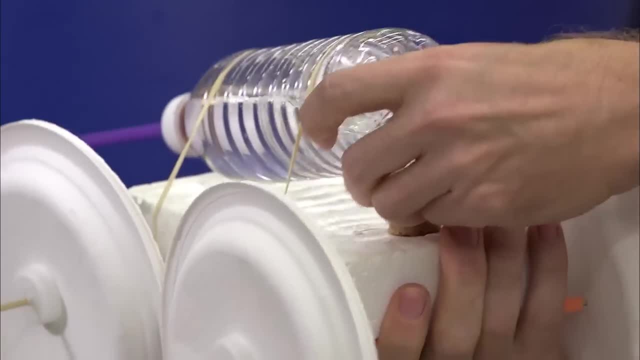 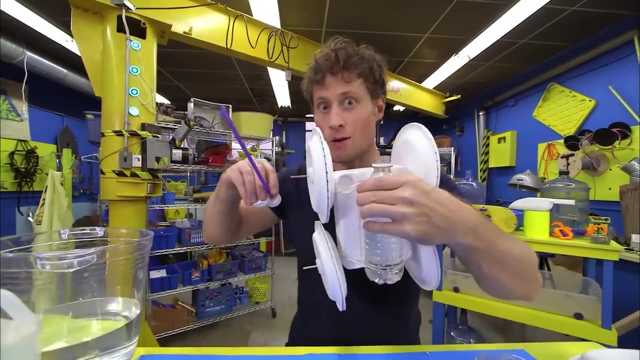 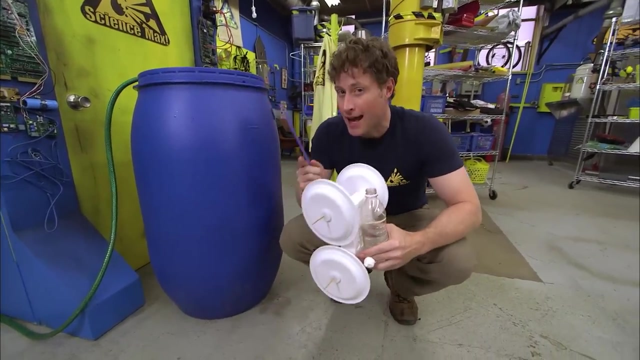 Finally stick something underneath the underside of the bottle to raise the end up off the base, Bring your cap and then go outside. Ah, here we are outside. Yeah, I know we're not really outside, but I have a science lab and you probably don't. 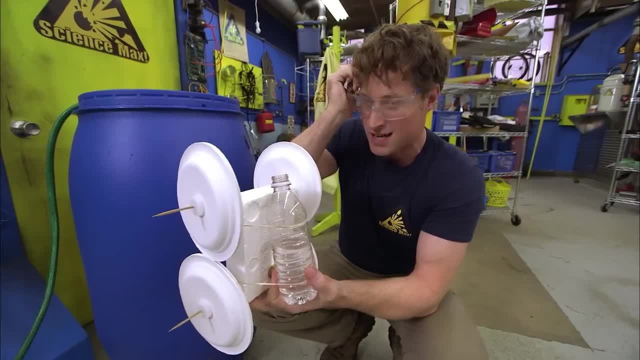 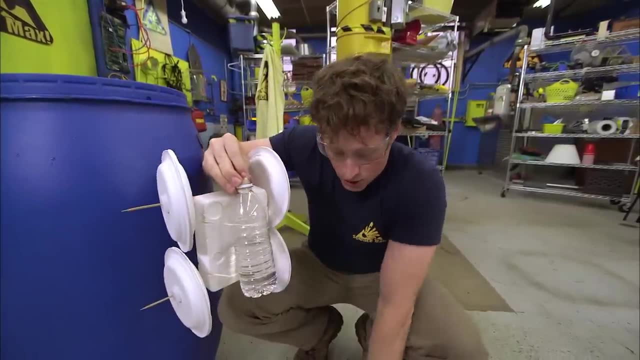 So I highly recommend you do this outside And don't forget your safety glasses. Now, this is why we make a little packet of baking soda, because we want to delay this reaction as long as we can. So I like to hold it there. 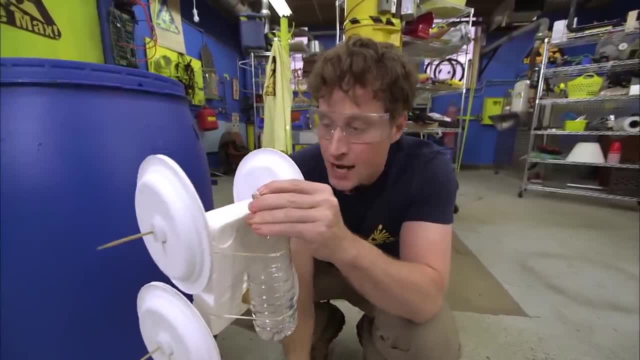 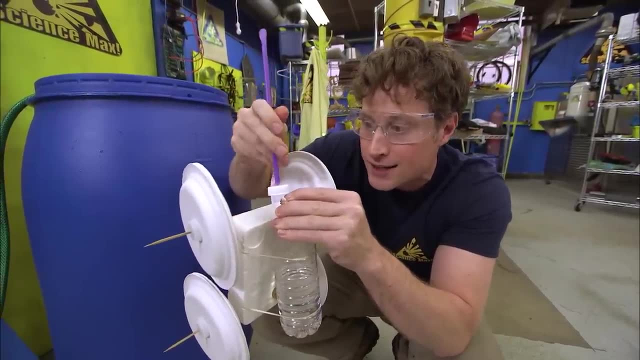 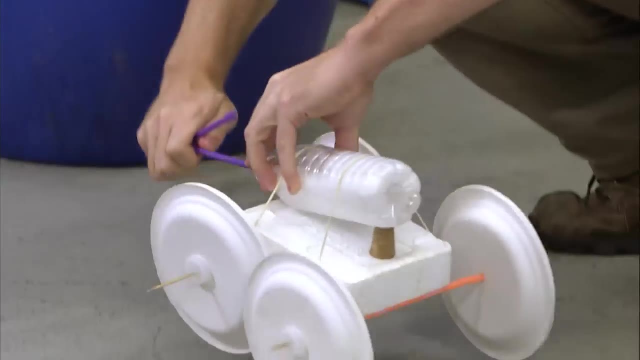 We'll hold it there with one finger so I can get the cap ready, because we don't want it to react until we can get the cap on and then kink the straw to keep the pressure inside until we're ready to let it go. Then, at the last second you'll want to drop that packet in and quickly cap it and kink the straw. 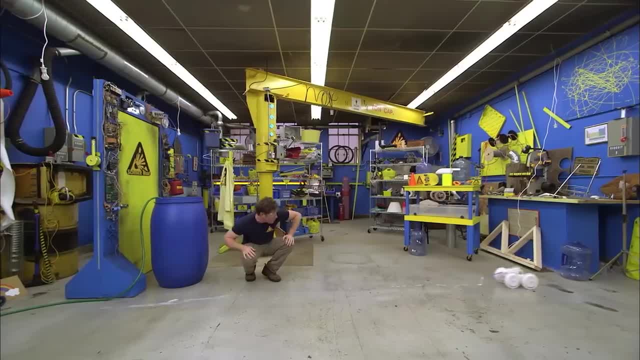 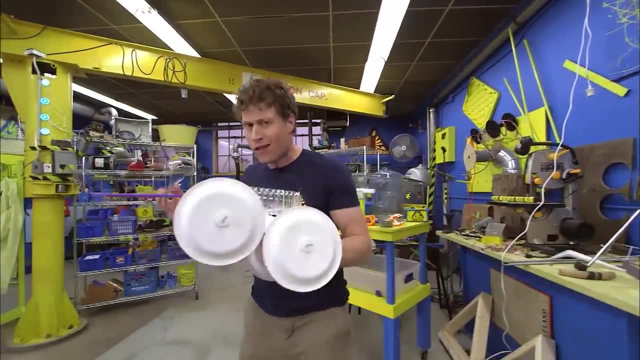 And Woo-hoo, Woo-hoo-hoo-hoo, Ha-ha, There you go, a water-powered car. Now I know what you're thinking. You're thinking, Phil, wait a minute, that's a vinegar and baking soda powered car. 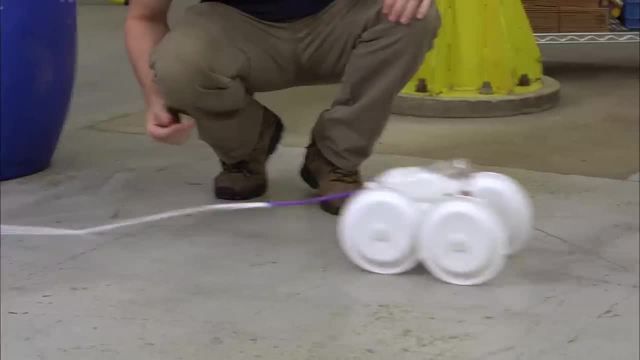 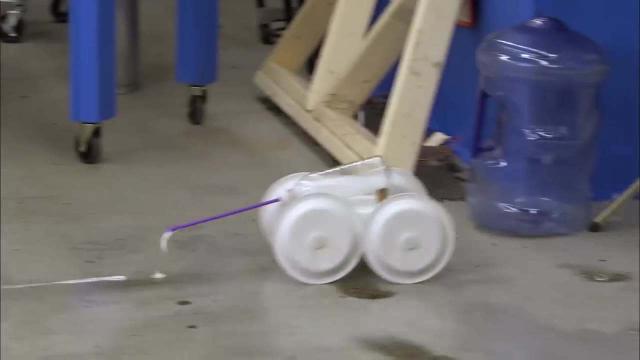 Well, kind of The vinegar and baking soda create a gas and that gas creates pressure in the bottle and that pressure forces the water out of the bottle. But it's the water leaving the bottle that creates the thrust. The water going that way pushes the car that way. 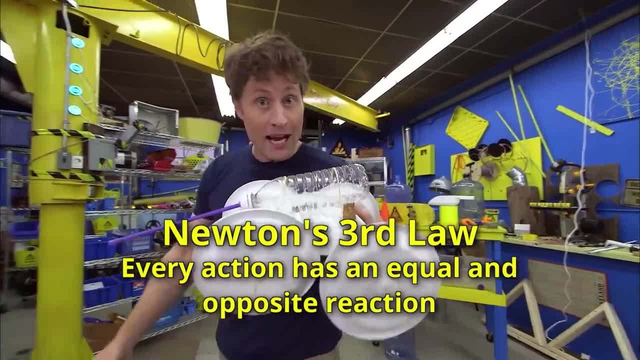 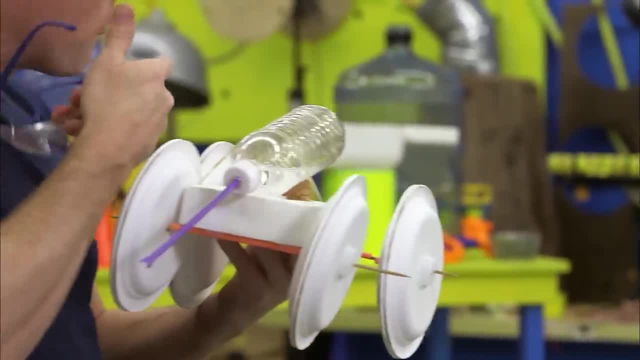 Newton's third law: every action has an equal and opposite reaction. So what we're going to do is max out the water-powered car, Figure out how to get water going that way so we can go that way. But we means me and someone else. 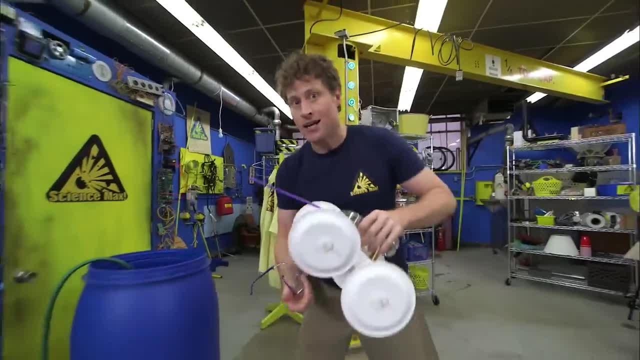 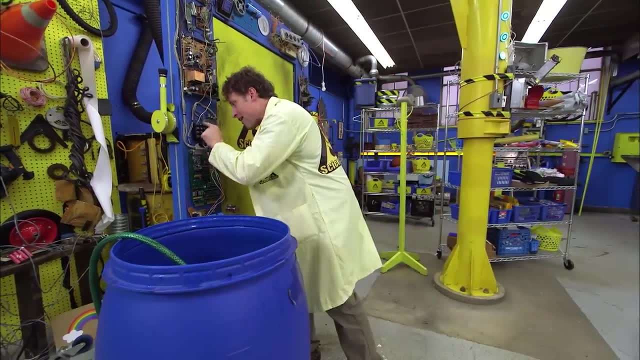 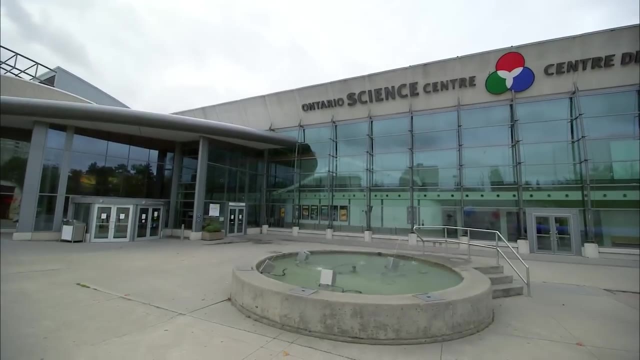 Who can help me? Oh, I know Anthony from the Ontario Science Centre. He'd be great at this. Hopefully he's not busy. We're going to max out the water-powered car. Ha, Anthony, Phil, Sorry about that. 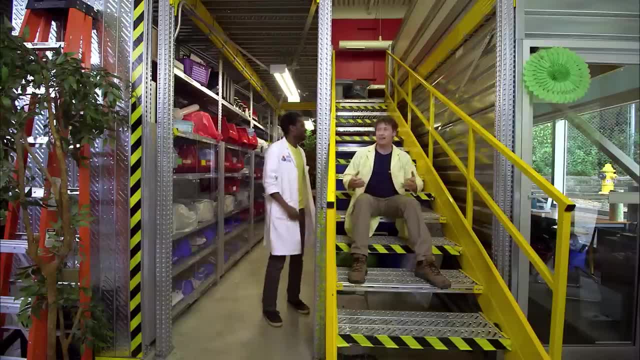 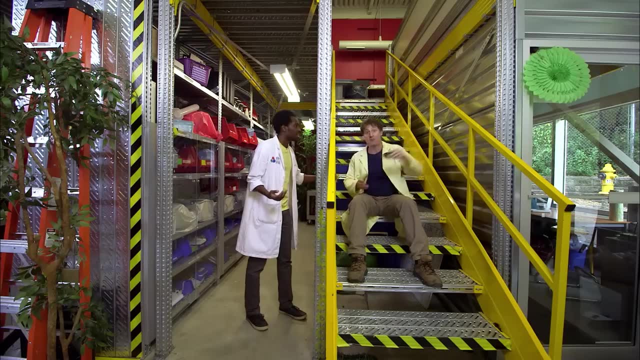 Did I scare you? Uh, don't worry about it. How you doing? Awesome thanks. I was wondering if I could get your help on an experiment. Yeah, okay, Which one? I'm building a water-powered car. It's going to be great. 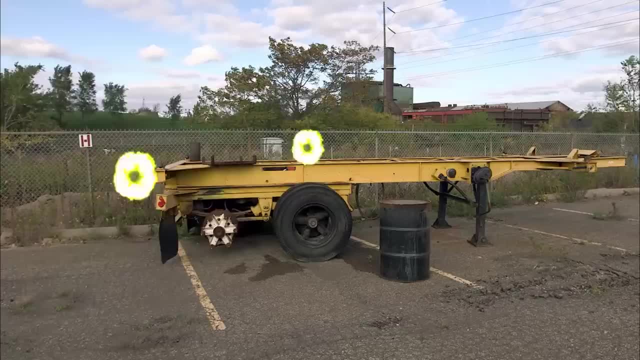 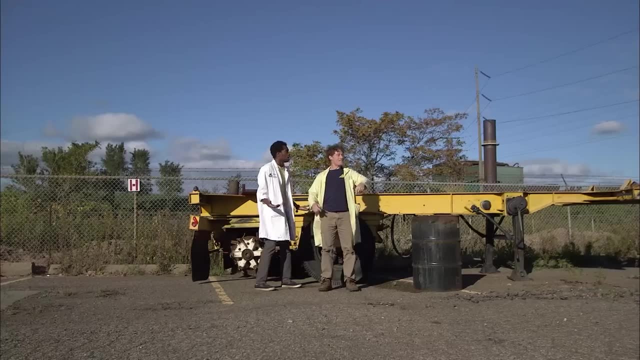 It's Science Max Headquarters. I'll show you, Phil. Phil, I'm here. What, Phil? where are we? Oh, this is the parking lot for Science Max Headquarters. So Okay, Today, Yeah, I want to max out the water car. 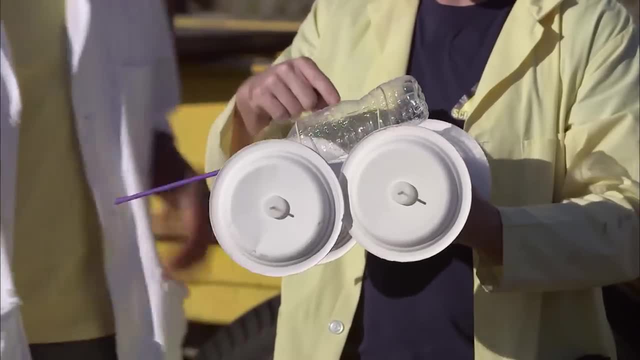 This thing is awesome, Yeah. so what you do is you use vinegar and baking soda, Yeah, And you pressurize this container, Okay, And the water shoots out that way. So the car goes this way: Ah, Newton's Third Law. 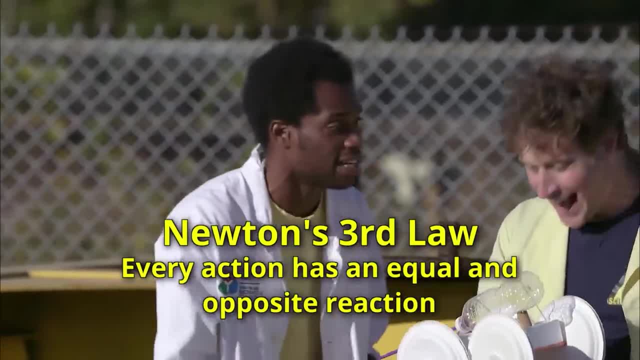 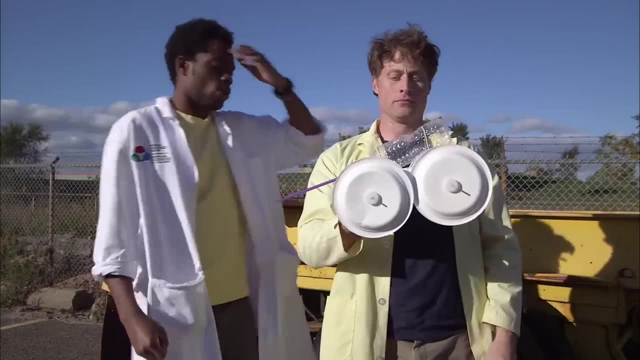 Every action has an equal and opposite reaction. Yeah, you know your stuff. Okay, This is why you're here. This is because I could really use your help and advice on how to make this bigger. Okay, so we're going to need a bigger tank to pressurize. 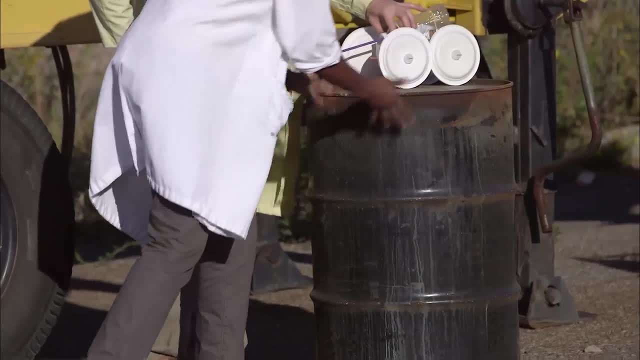 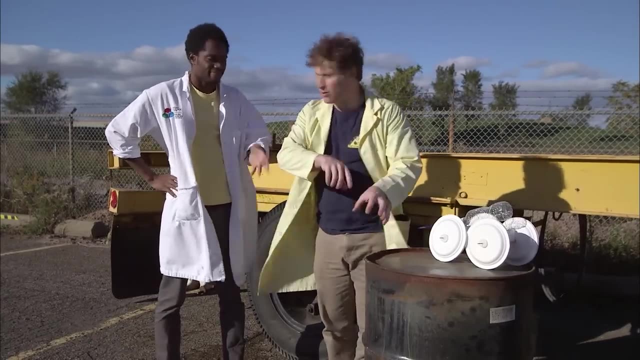 So this, what about something like this? Okay, This, So we need something that can hold pressure. Do you think this would work? I don't know if we'd want to And we'd have to put like pressure fittings on the barrel, like cut a hole and weld them. 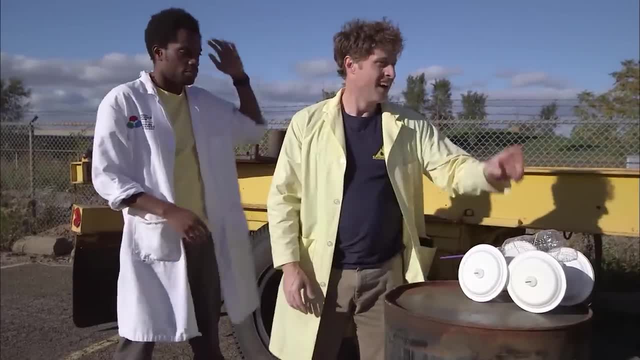 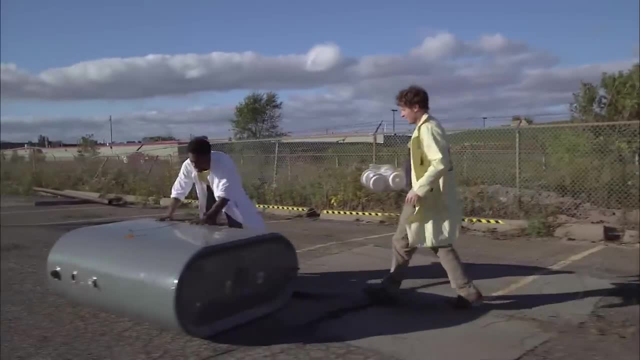 on. I don't know if that's Something tells me this wouldn't work. Okay, sure, I got some other stuff over there maybe that we could use. Oh, check this out. Yeah, I think this would work. This would work a lot better. 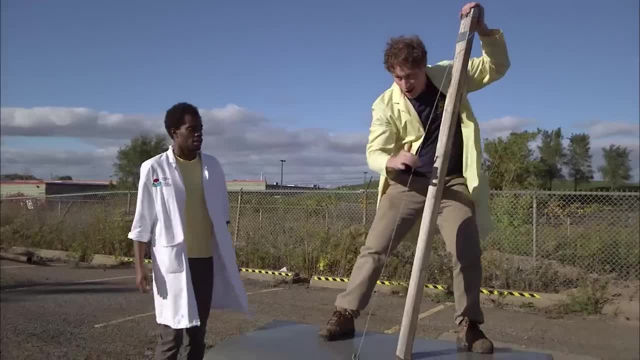 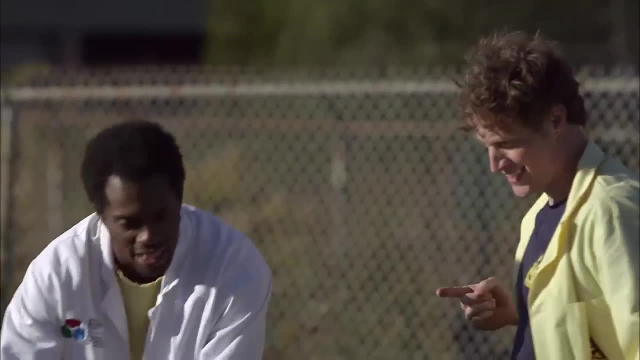 Well, this is my stand up: wash tub base Your what? So we'll reuse it. Yeah, Okay, So I know this. the problem is, I think this is like an oil drum- right It is. It's an oil tank from a house. 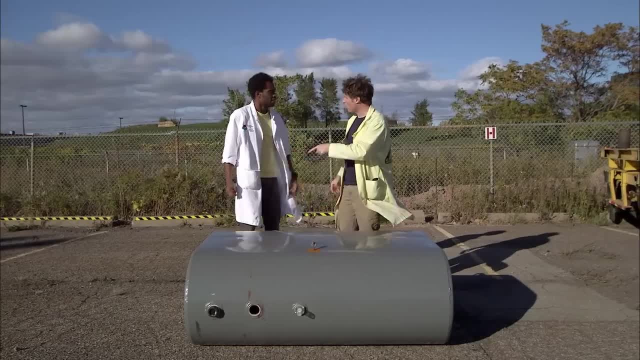 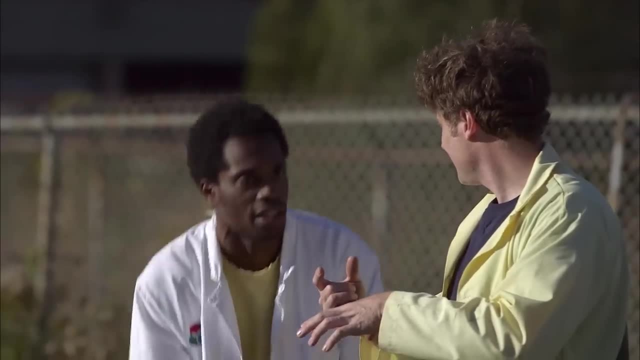 And these things are not built for pressure. You can get water tanks that you pressurize, Oh, like hot water heaters. Yeah, You can pressurize, They're built for that stuff. You pressurize them in your basement and then the water travels up to like your shower or 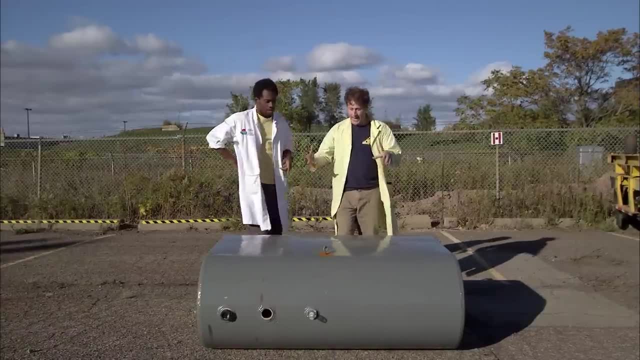 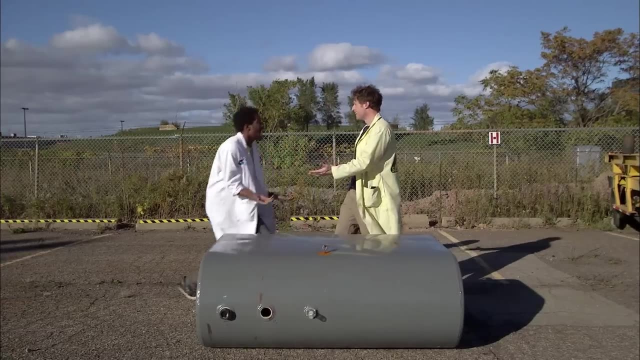 something like that To the top floor That makes. So all we need to do is get a pressurized water tank. Okay, Put water in it, Put pressure in it And put it on wheels, And then we open the valve and it goes right. 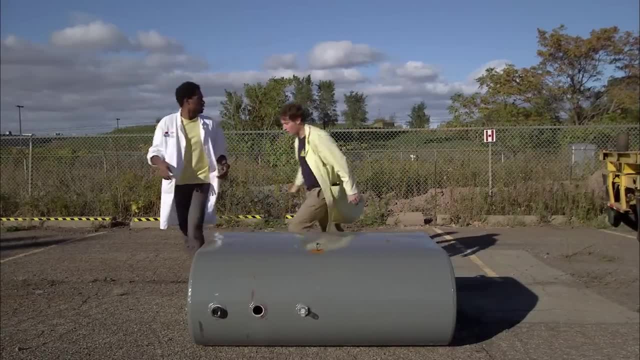 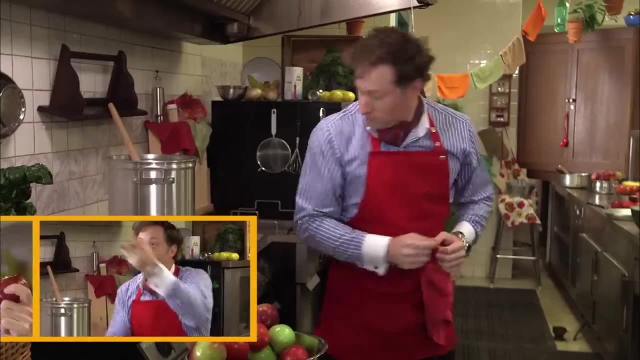 That sounds amazing. All right, Let's get to it, man, Okay, I got some water tanks over here in this corner of the parking lot. Seriously, Being a chef is my absolute passion and cooking up science recipes is my speciality. 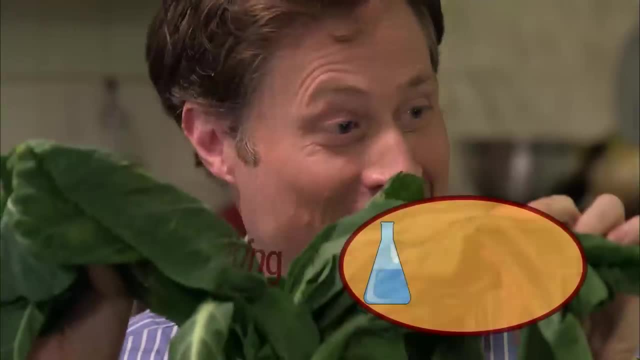 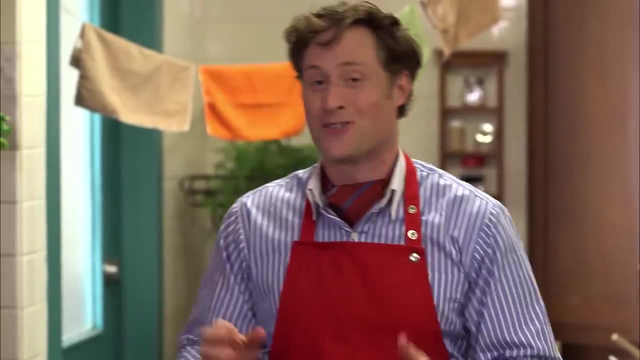 I'm Buster Beaker, and this is Cooking With Science. Oh hello. When you're a professional chef like me, you spend lots of time perfecting the perfect recipes. I know my way around the kitchen, and today I'd like to show you one. 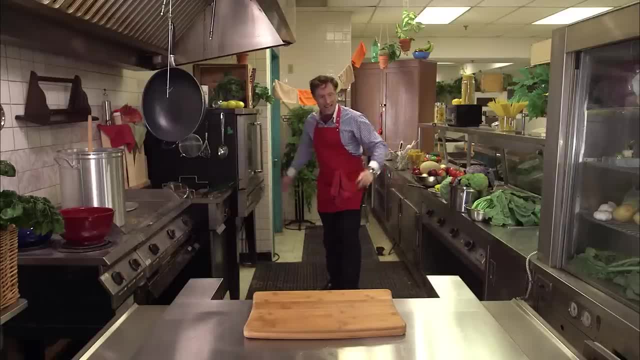 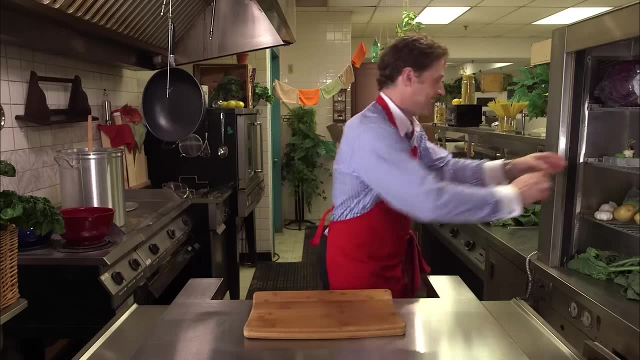 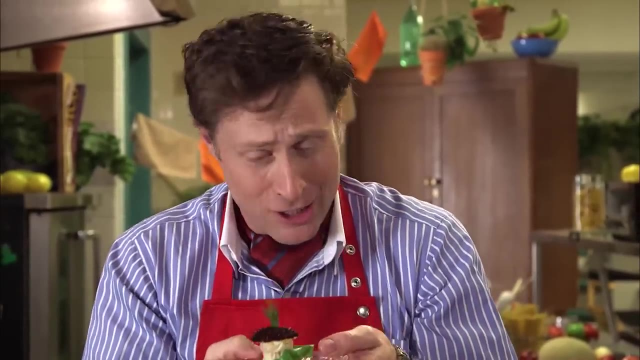 That's not the fridge. Oh, Today I'd like to show you one of my favorites: Quail, truffle gazpacho cakes on a plate of ice, Beautiful. And here's how to make it: Take some quail, some truffle and some gazpacho and put it into a cake. 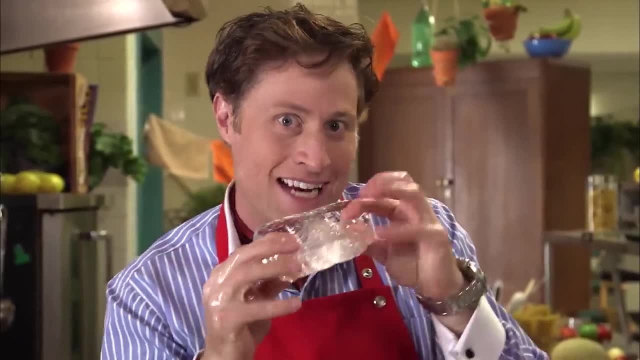 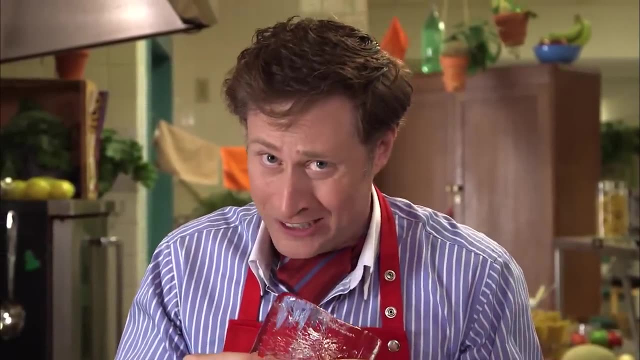 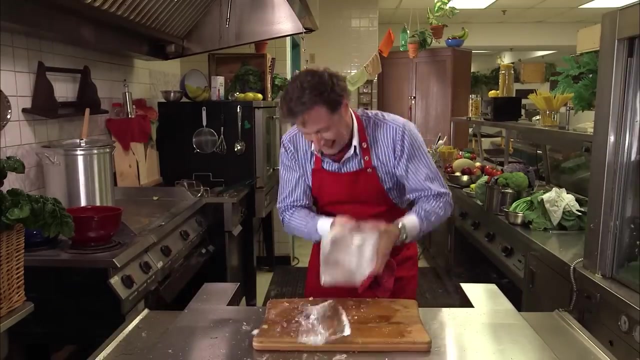 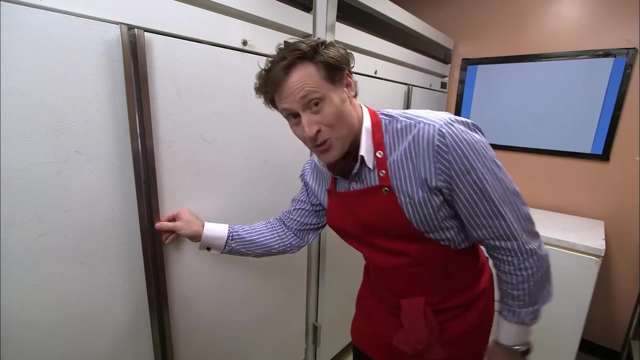 Delicious. And here's the interesting part: How to make the plate of ice. Ooh, How did I do it? Well, I tried many different methods and none were very successful, But now I let science do the work for me. So here's what I do. 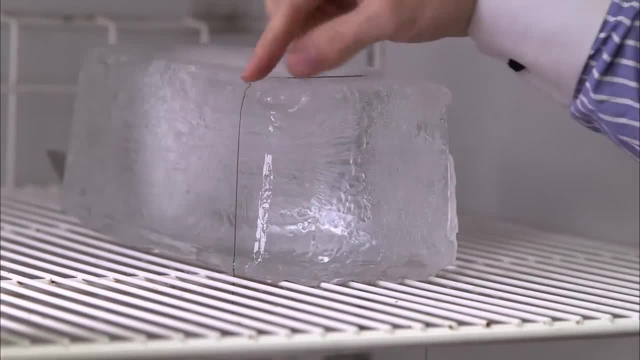 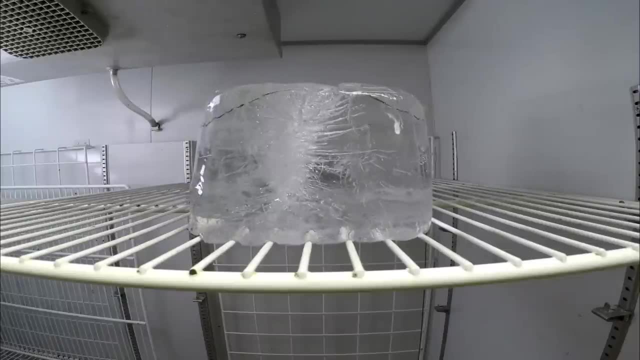 You see, I've got my large block of ice and I've got a fishing line over the top and on the bottom I've got two heavy weights. Now we wait. The heavy weights put pressure on the fishing line. This pressure melts the ice when it's pressing down. 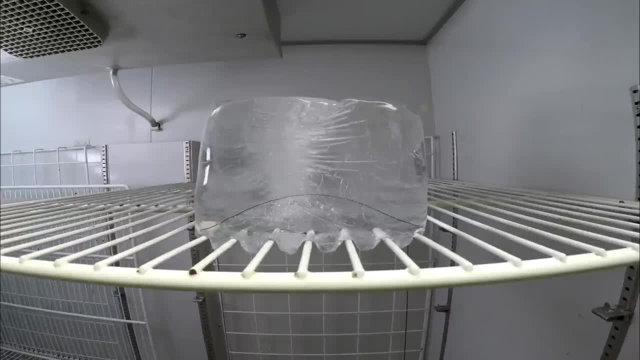 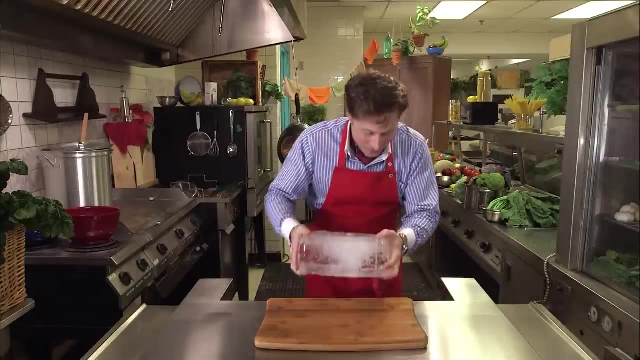 As the ice melts, the fishing line moves through the block of ice and eventually cuts its way through. There we are. My hours of waiting have almost paid off. You see, I've got a perfect line through the ice, and I stopped it just before it finished. 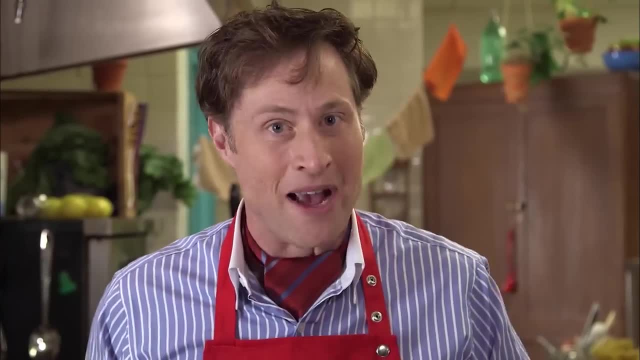 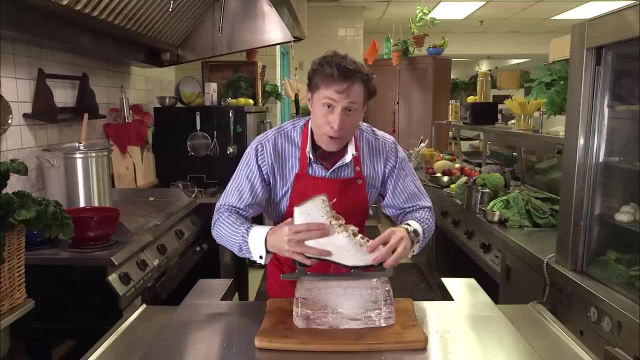 It's the pressure of the line on the ice that makes it work. The same thing happens when you use ice skates. You see, it's a very thin line and your body weight presses down on the ice, melts it a bit, and that allows you to glide across the ice. 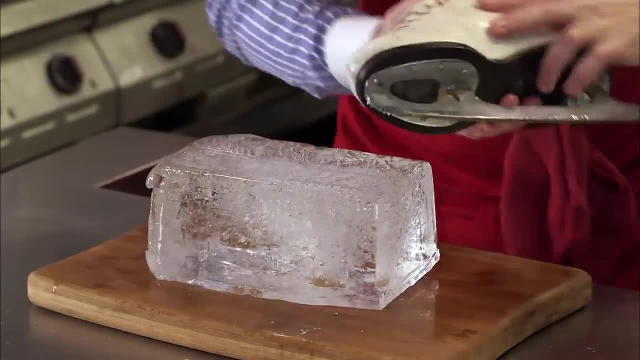 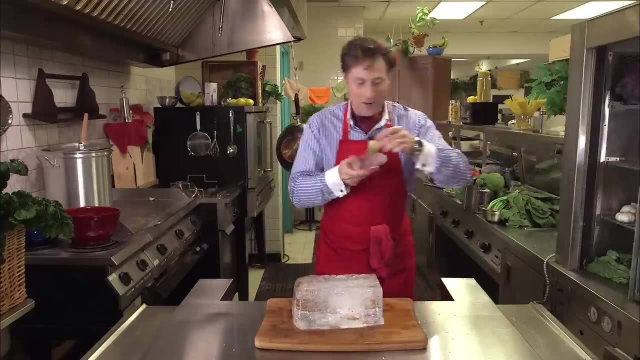 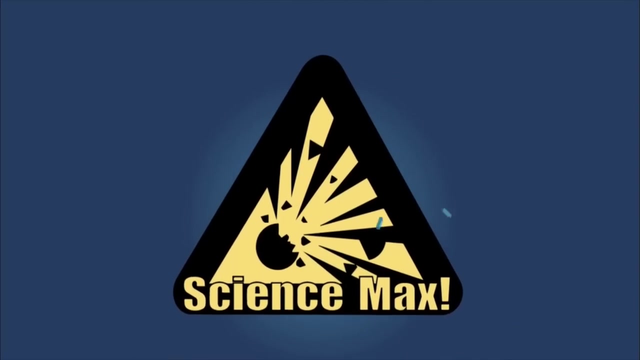 It also allows me to just pop this off. There you are, You see. Perfect plate of ice to put my delicacy on. Let's just try that now. There we Um. So I've joined Anthony and we're going to max out our water-powered car. 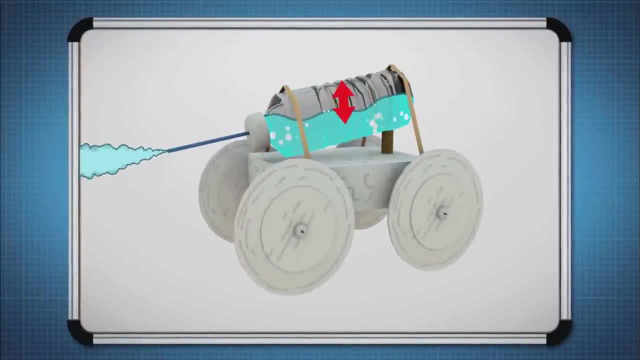 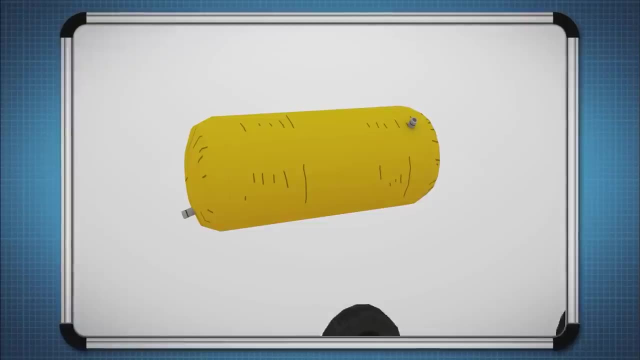 Our small design works by creating gas, which creates pressure, which forces the water out of the bottle, creating thrust. Our new plan is to get a water tank, put it on wheels and put water in it. Then we use an air compressor to pressurize the air inside. 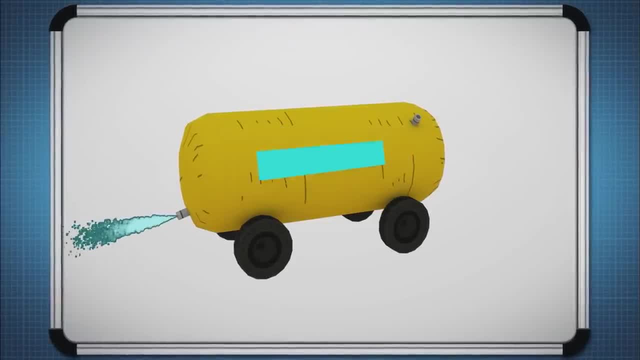 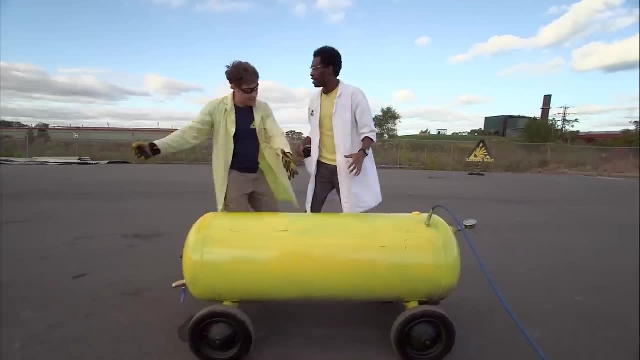 When we open the valve, the water is forced out this way, which causes our water car to go that way. Okay, Ha ha. So water car maxed out version Uh-huh, Huge Water tank And filled with lots of water and lots of uh. 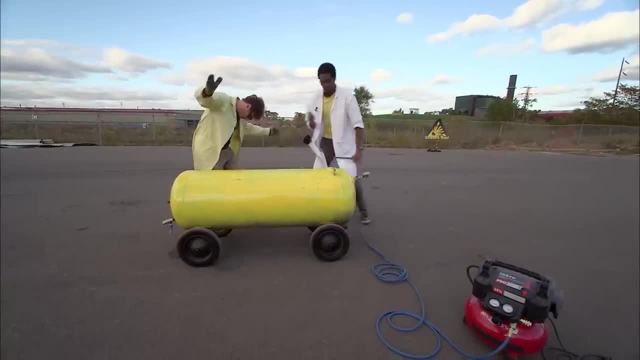 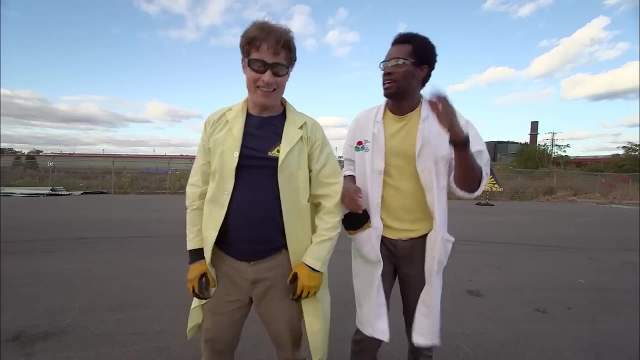 Lots of air too. Air, Yeah, Pretty good, right, Whoa, It's a lot of it. So Did it mess up? Did it mess up my hair? Uh, No, you look fine, You look great. 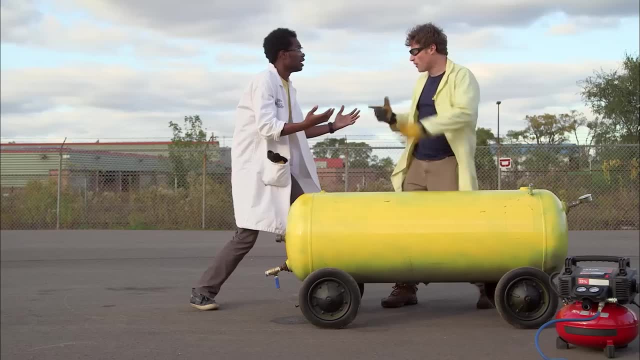 Okay, good, Now the only thing left is: we just got to open this valve here, right, Yeah, You want to do the honors? Uh, yeah, Yeah, let's do it. Okay, Okay, Let's do it. 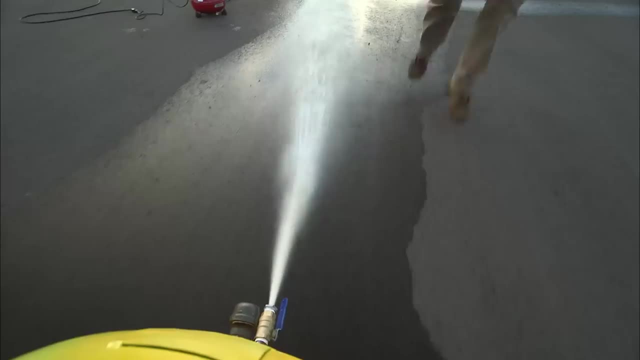 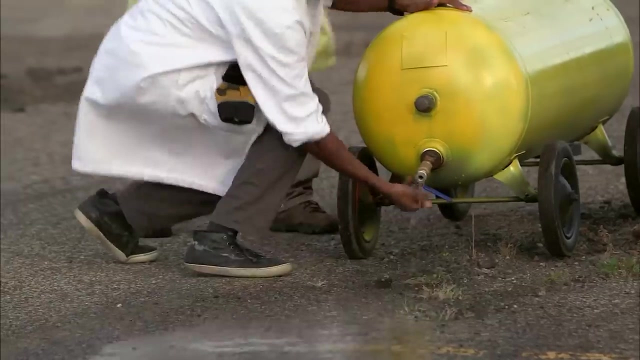 We open the valve and our pressurized tank moves forward. The air pressure in the tank forces the water out with enough force to move the tank. This is awesome. That was awesome. That was a great run. Yeah, It was amazing. 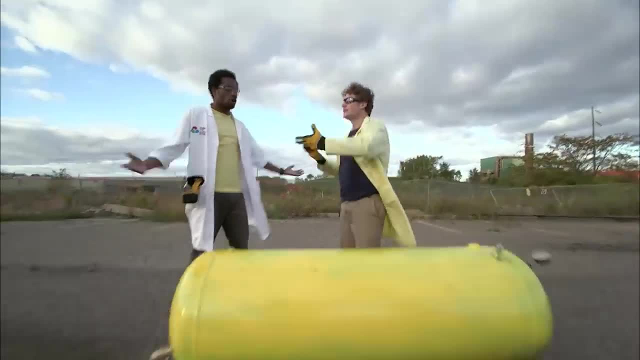 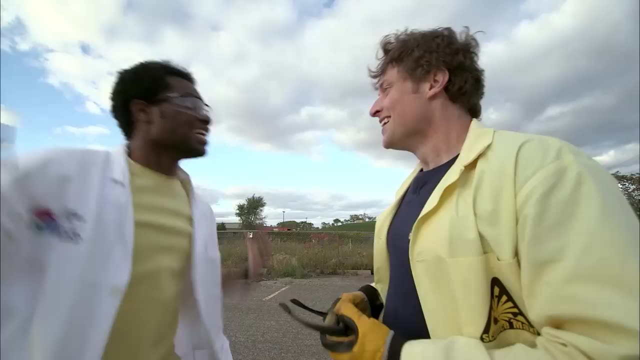 So pressurized water tank on wheels Totally works, Totally works, Total success, Yeah. Um so, because this is Science Max, the only thing we can do now is make it bigger, Right? Bigger, Exactly, Yeah. 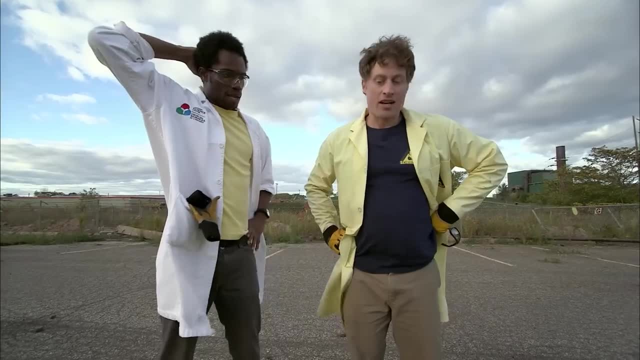 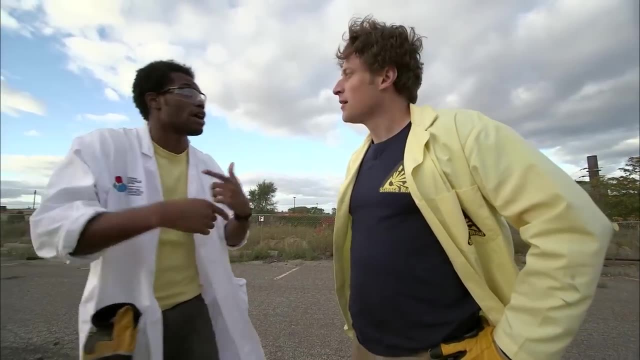 Okay, Bigger than this one, Yeah, Um, so, Because then it would be too heavy, right? Exactly, Way too heavy, Much bigger, Maybe. maybe what we can do is just get a lot more water, Okay, And then, and then we find a way to pressurize the water. 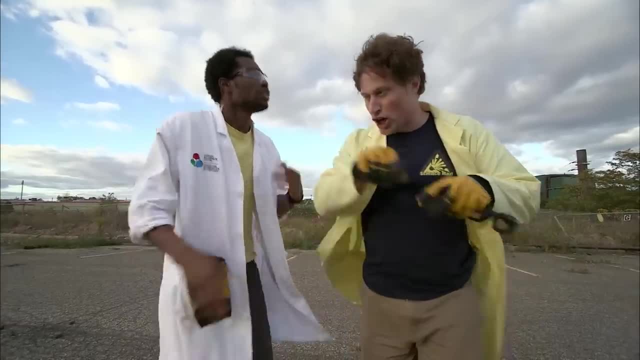 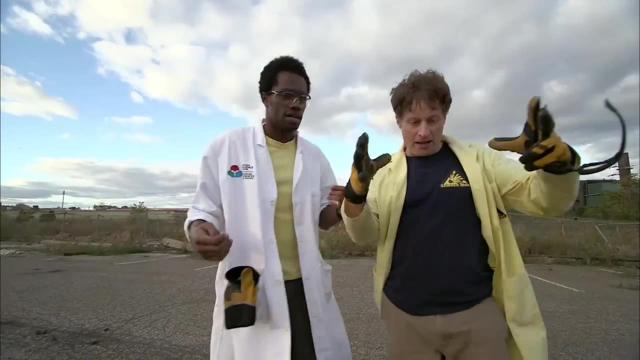 Oh, so don't pressurize the whole tank, Just just the stream of water that's going out of the tank As it comes out. Exactly Something kind of like a like a fire hose- A fire hose, Right. 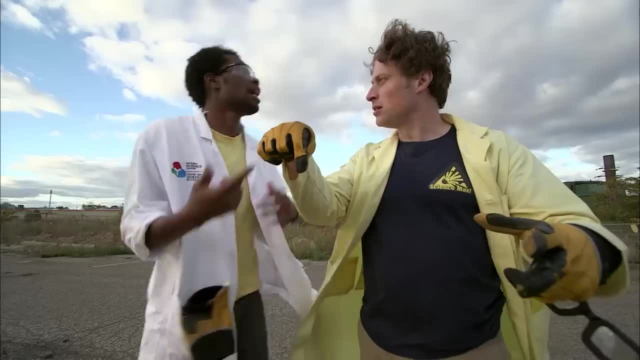 So So we take a big container of water Right And we I guess we would need a pump. Yeah, like a pump would be perfect. So then we, we suck the water out of the container, put it through the pump to pressurize. 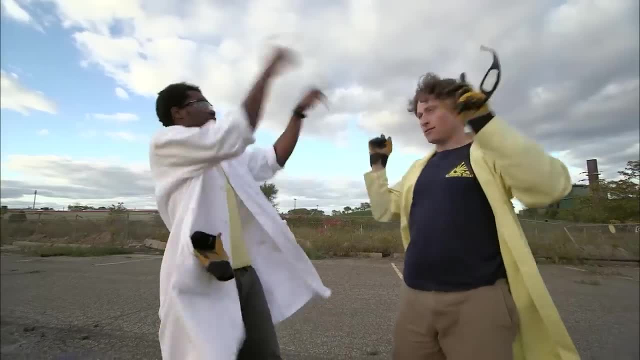 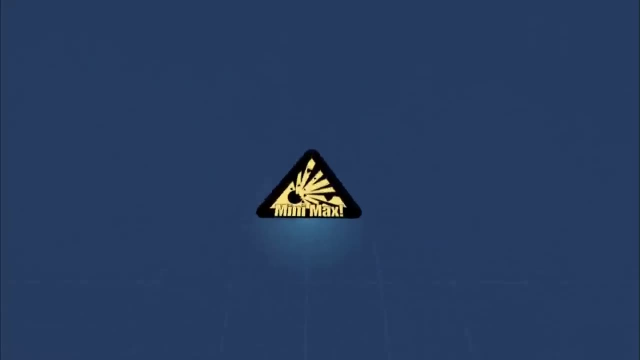 it, shoot it out of a fire hose, Uh-huh, And then our car goes flying, Goes flying. Okay, Yeah, let's do it. Yeah, All right. Amazing, When water is going fast, it has a lot of force. 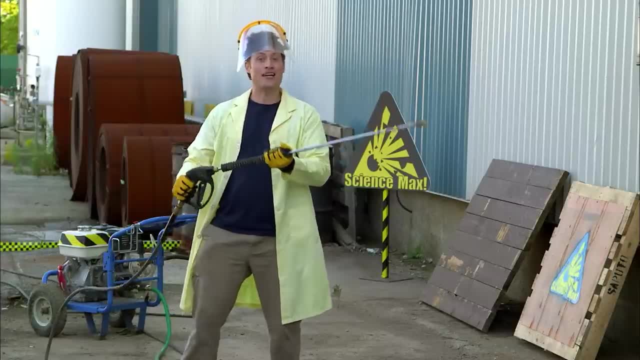 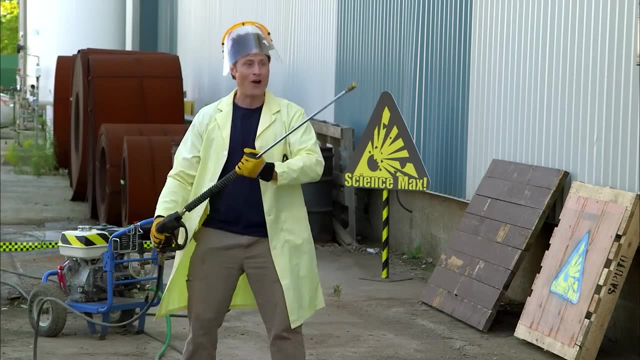 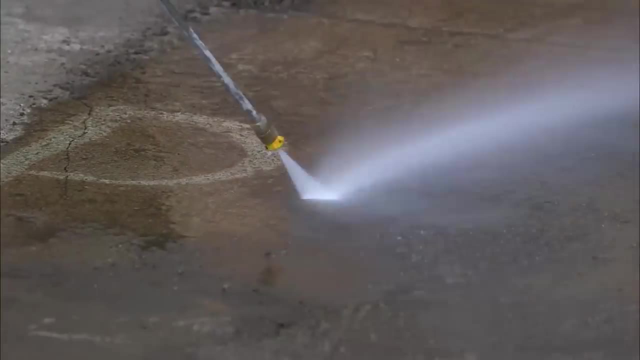 This is a power washer. It's made for cleaning concrete and wooden decks, but it doesn't use soap and it doesn't use heat. It only uses the power of water. Let's try it out. The power washer creates a stream of water that is moving really fast. 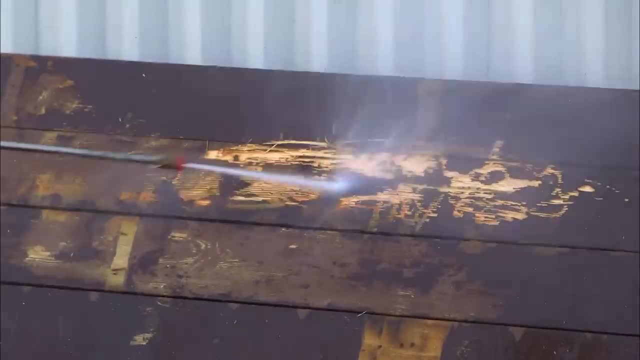 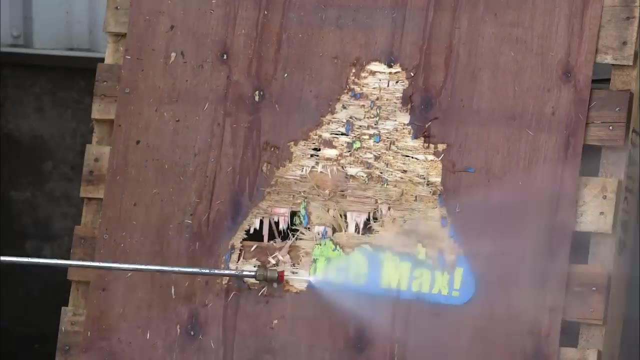 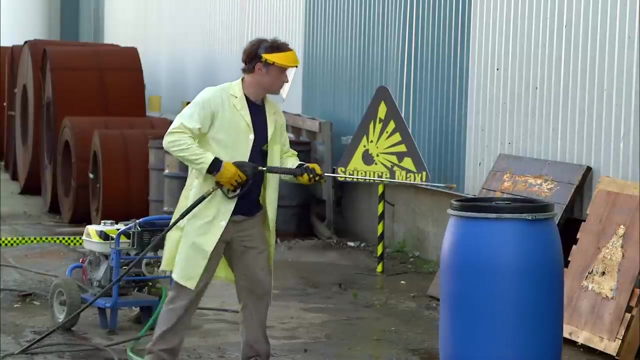 It has the force to clean concrete, strip the paint or even the Science Max logo off wood. But how do I max out the power washer? What's the most ultimate use? I can think of Power washer, pumpkin carving, Power washer, pumpkin carving. 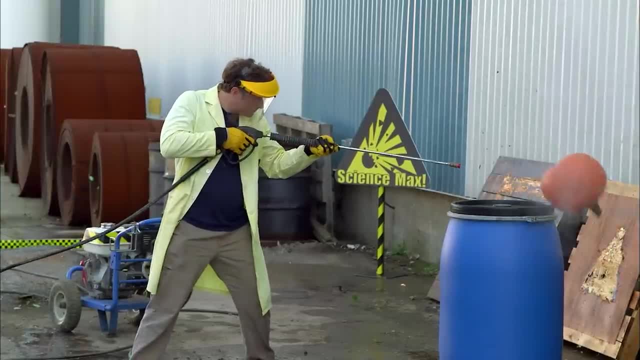 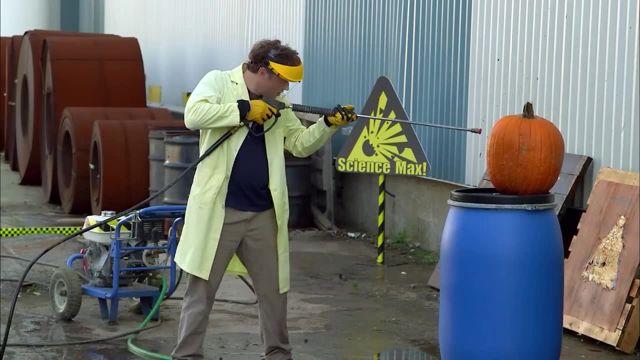 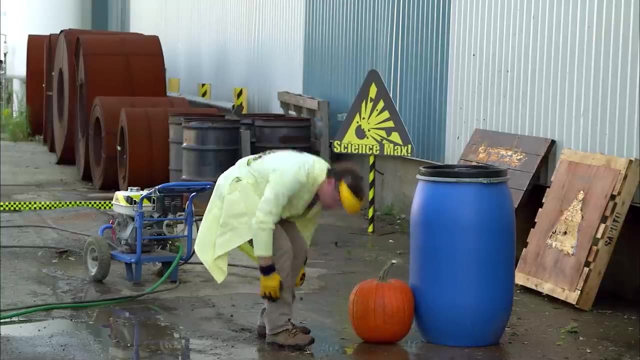 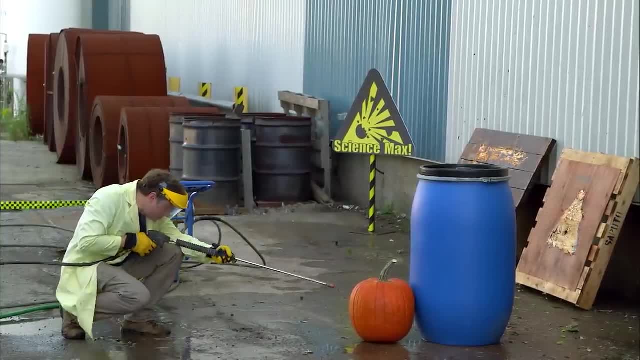 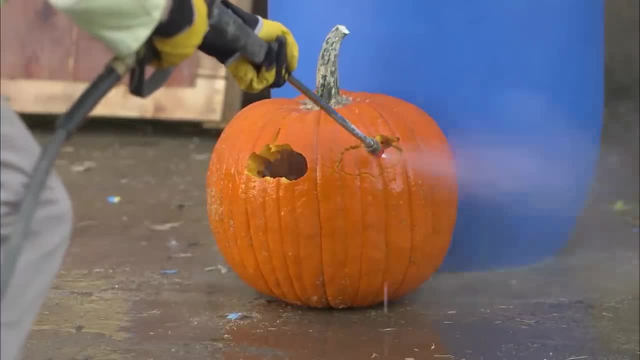 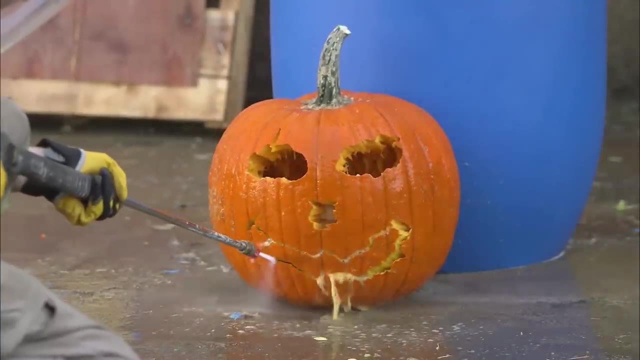 All right, Let's run it. The power of the pressure washer creates a stream of water strong enough to make short work of my pumpkin. Power washers may only shoot water, but they can be dangerous, so don't try this at home. 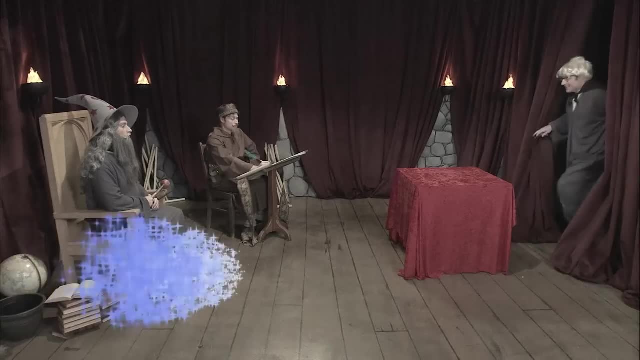 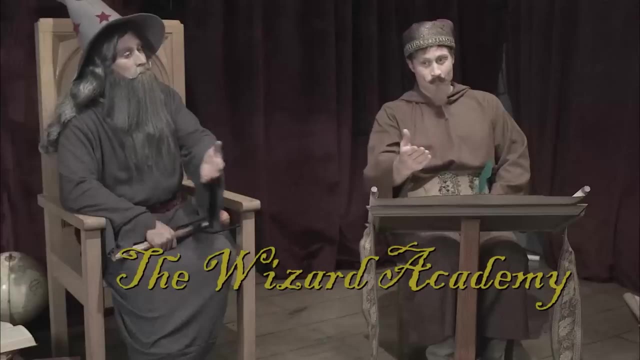 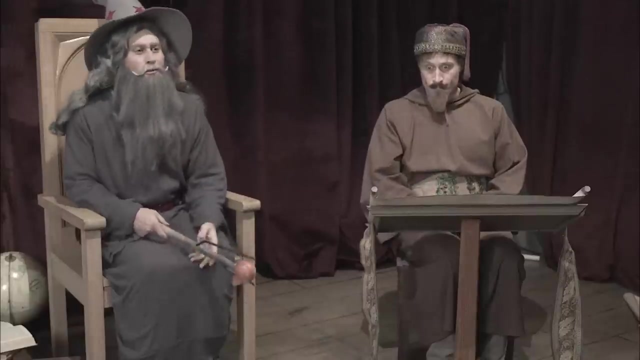 Yeah, Science, The Wizard Academy. All you have to do is demonstrate true magic And you'll be granted entry. Send in the next candidate. Oh no, not Over-Well-Mo. Did someone say Over-Well-Mo? 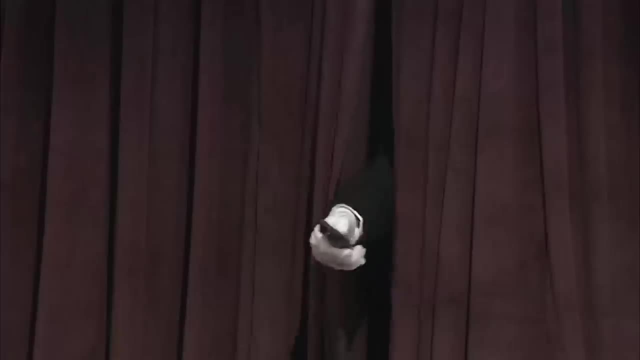 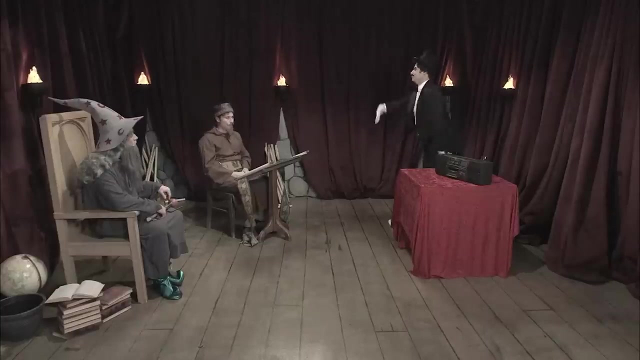 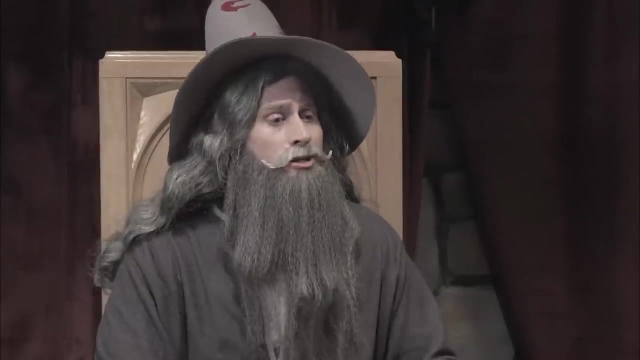 No wait, no, next, No, not that, Okay, okay, good, okay, Behold, it is I, Over-Well-Mo. Welcome back, Over-Well-Mo. If you can truly demonstrate magic, you may join the Wizard Academy. 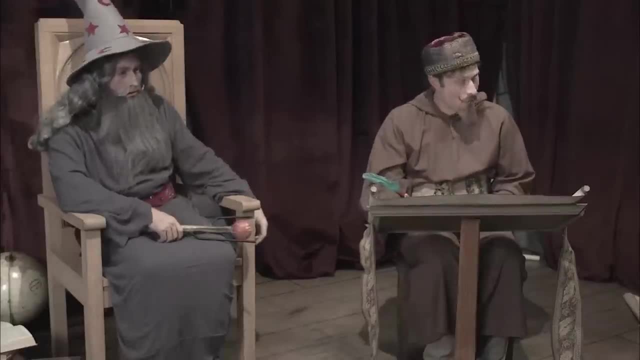 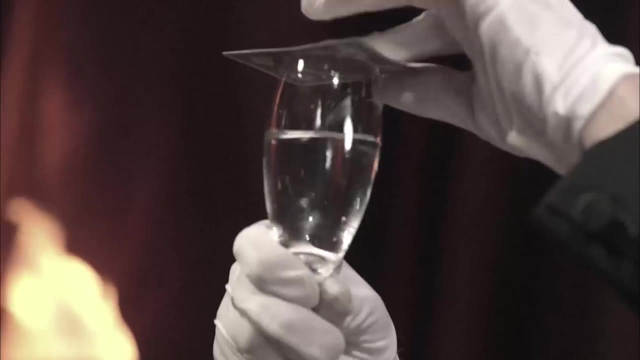 A glass of water. No, no wait, that is not the whole trick. Okay, hold on. Okay, and this a waterproof playing card. I put the card on the glass and flip it upside down, and then I say the magic word. 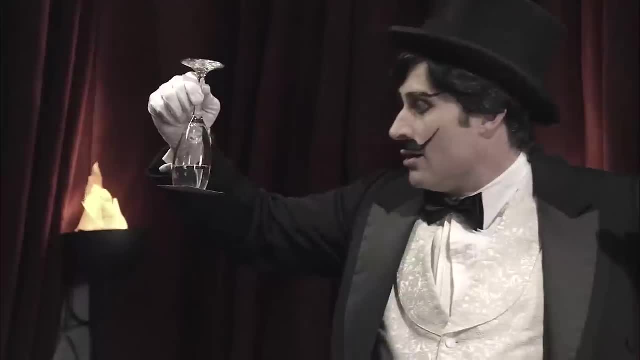 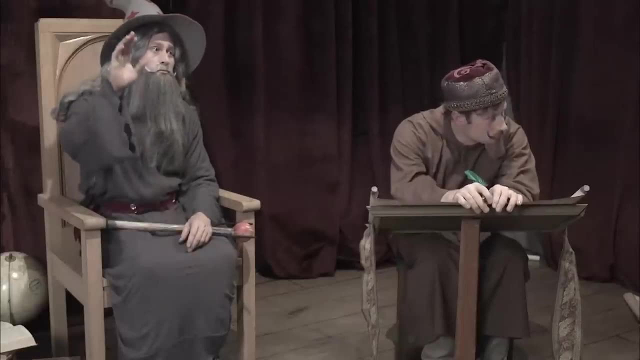 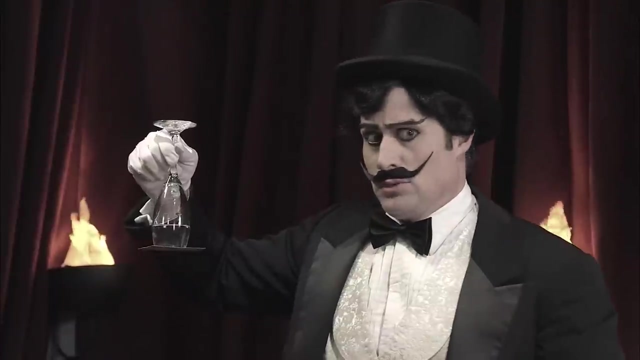 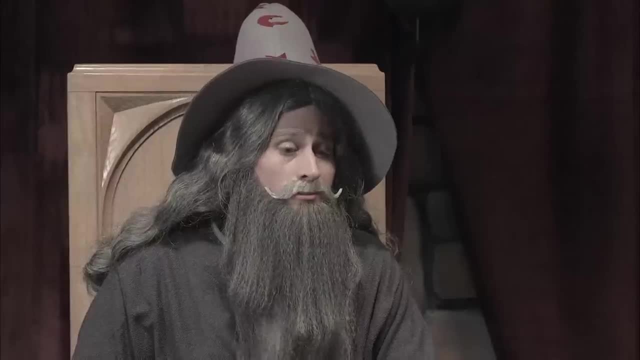 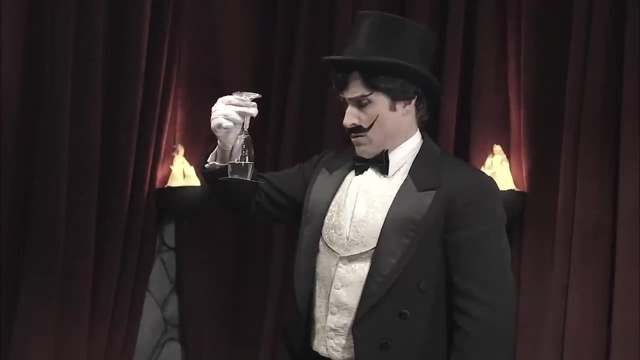 and the card would fall to the floor. It's not magic, This is magic. No, it's science. Horse feathers, Look. The reason the water doesn't come out is the air at the top of the glass keeps it held in by suction. 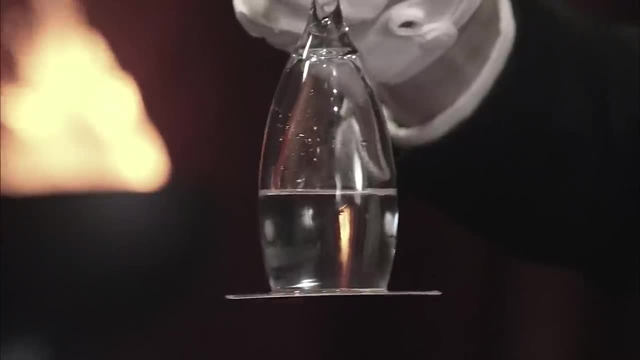 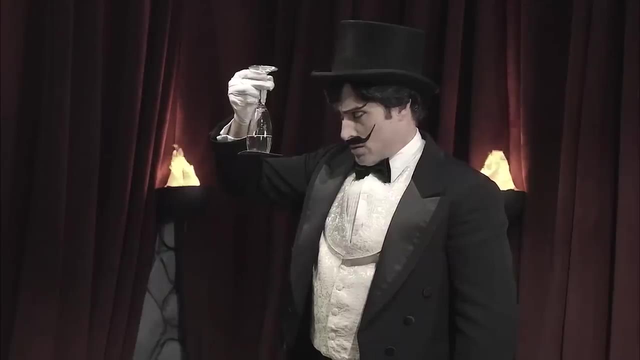 More air would have to get into this glass to decrease the suction. the suction, and because the playing card is keeping a seal on the glass, the suction of the air is holding the weight of the water up Walderdash. All right, look, let's do a little experiment then, shall we? 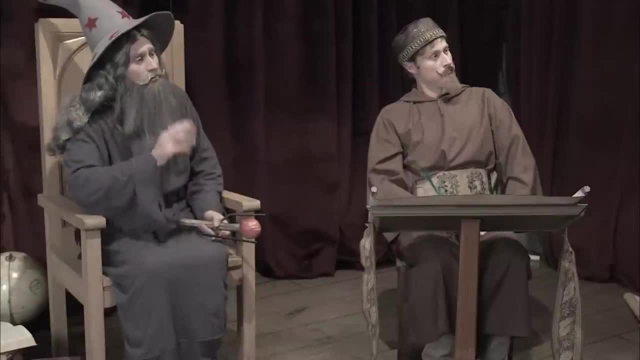 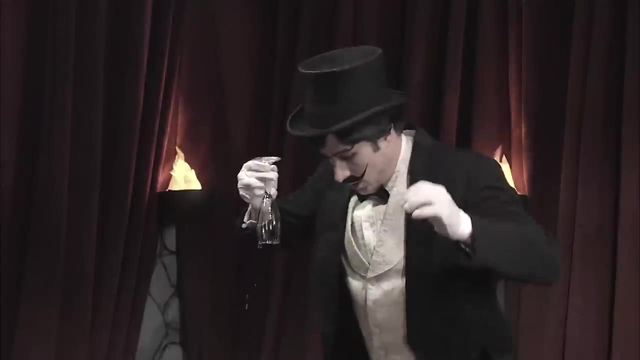 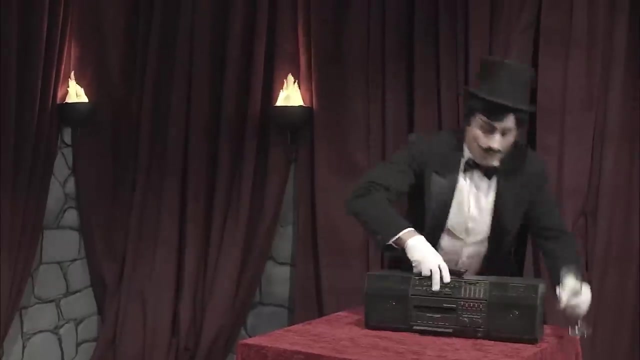 Let's move the playing card just a little bit from the edge of the glass. You see those bubbles. Yes, That's bad news. Ugh, Science, not magic. Well, I will return and then you will see. your mind will be melted by, by the no that's. 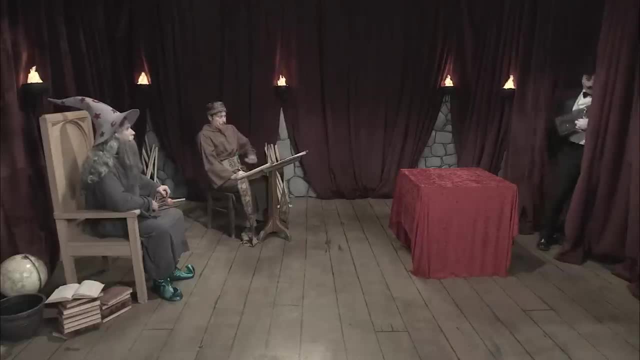 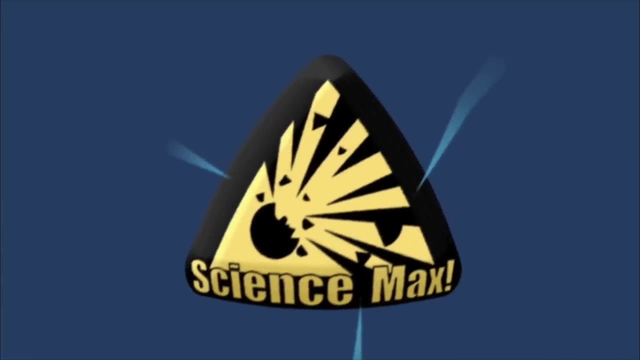 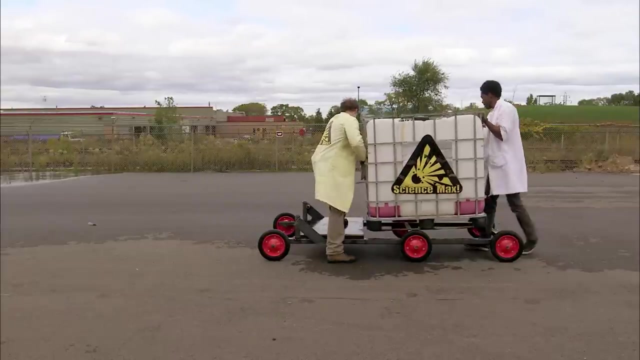 not my music. well, you will rue the day when that's not my music over. Wilma shall return. Our maxed out water car worked pretty well. Now it's time for something even more maxed out. We start with a giant tank on wheels. 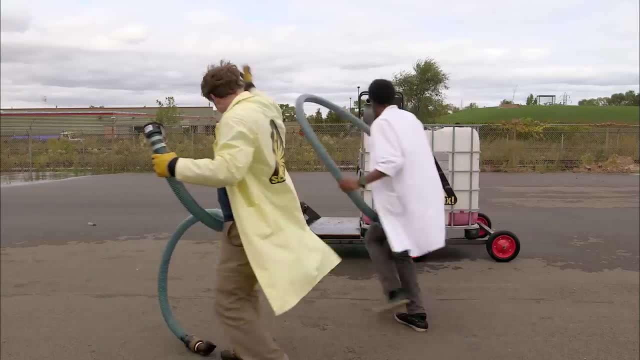 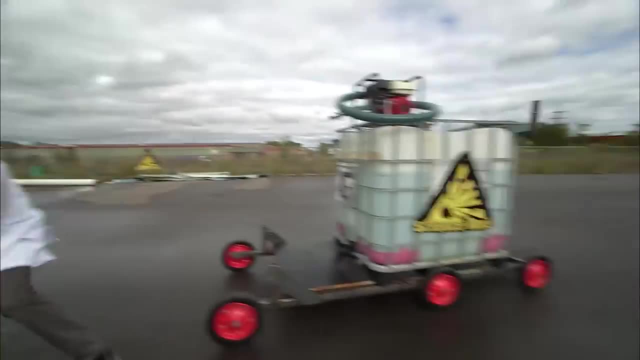 We add a pump to pressurize the water And a fire hose to shoot it out the back. What's more, this version is big enough for me and Anthony to ride Water car. Woo hoo. So this is the more super improved water car. 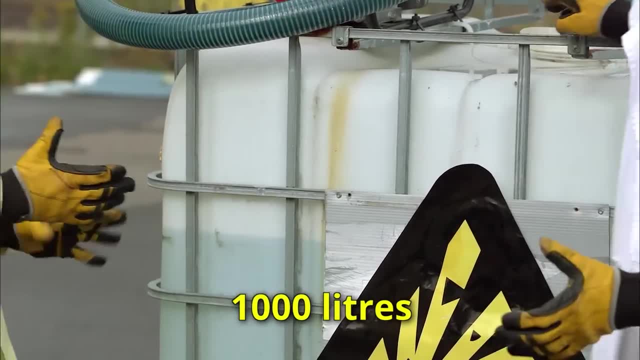 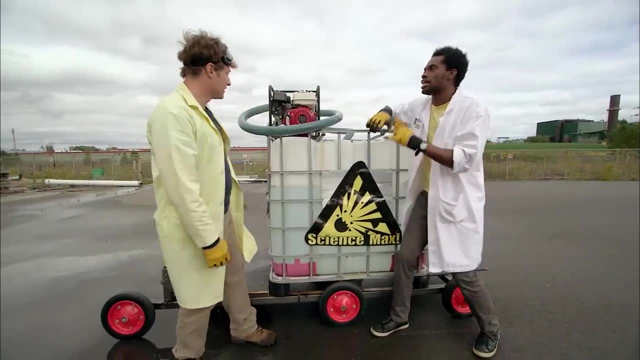 This tank holds 1,000 liters and right now it has 720 liters of water. We have a pump. A pump, That's right, our water pump. So the idea is we take the water from this container out through your hose, really pressurize. 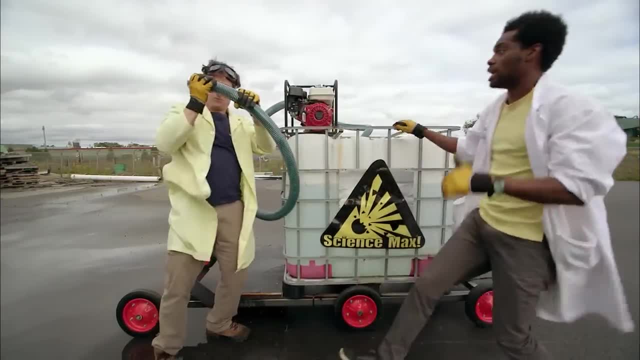 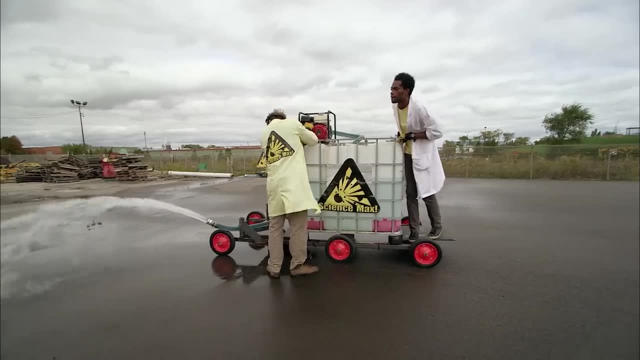 going really fast that way. Our car goes really fast this way. All we gotta do is just turn on the pump and we're ready to go. So we fire up the pump and the water stream comes out really strong, So strong I can barely hold onto it. 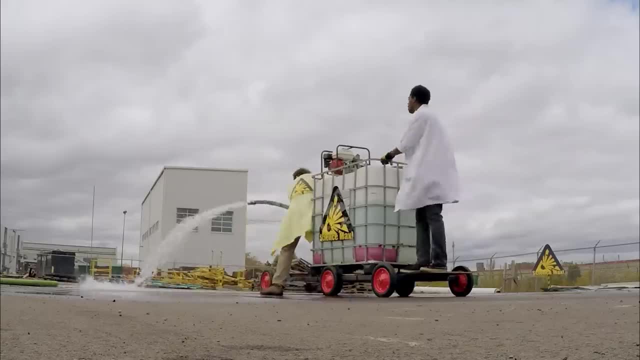 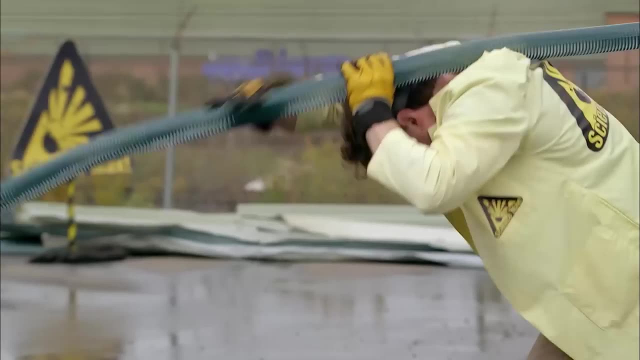 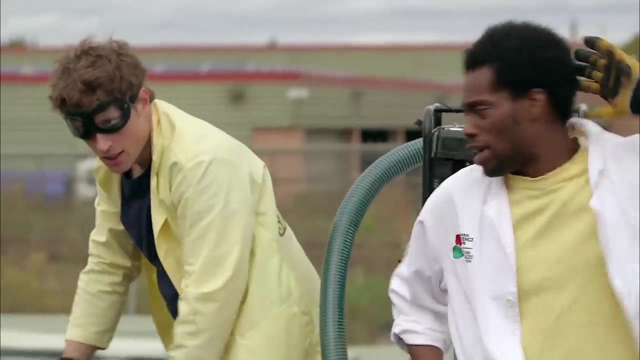 Here we go, But even so, there is a problem. What's going on back there? I got it, It's filling up. Yeah, Nothing happened. No, nothing really. Well, something happened. We got wet, but it didn't really. 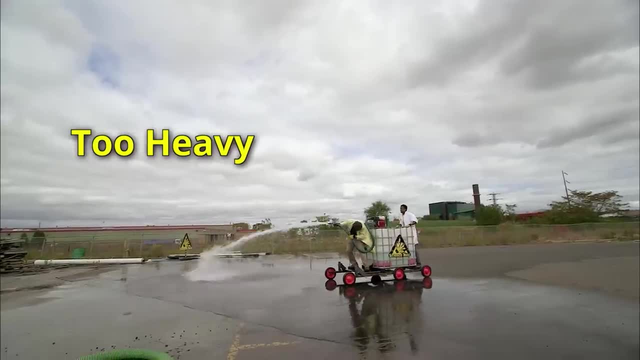 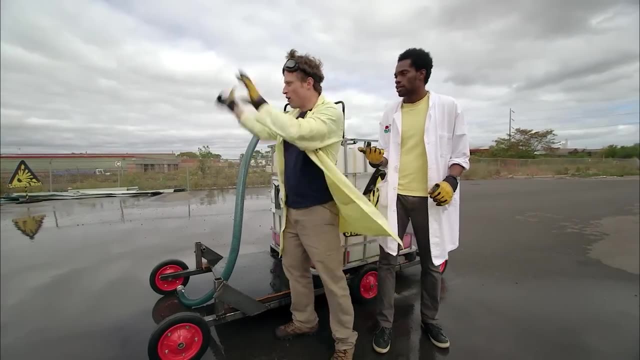 It's too heavy, Too heavy. So you're on it and I'm on it. That's a lot of weight. We don't ride it, That's something. Yeah, Also, this is kind of going crazy. Yeah, because if nobody's holding it, it's just going to flap around. 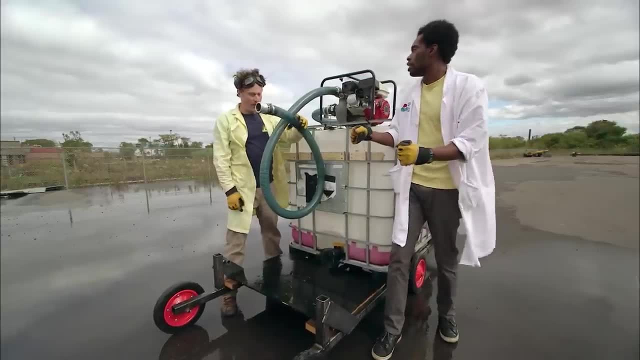 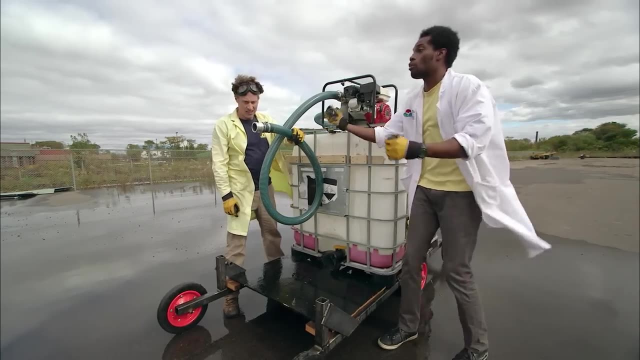 So we'll have a brace here, Yeah, Shoots it that way, That's good. And then we'll need- I feel like we'll, We'll need something to kind of propel it, Maybe a better propulsion system, Kind of like one of those steamboats. 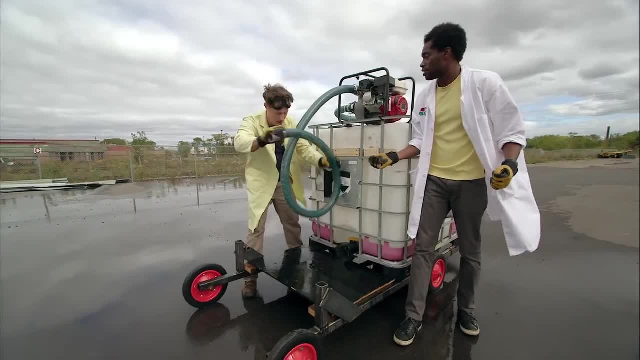 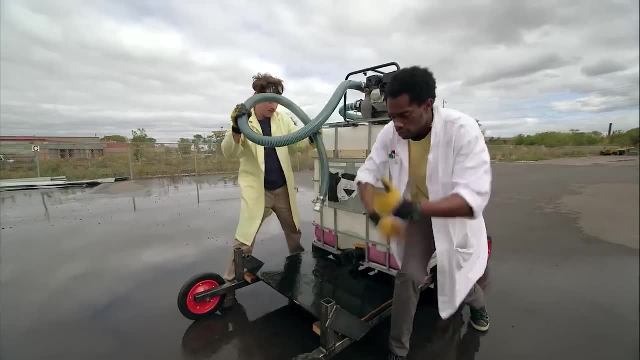 So we put a big paddle wheel here, Exactly, And we aim it. I guess we aim it down, Yeah, exactly Like that, And then At the paddle wheel, And then the paddle wheel spins and that propels the car. 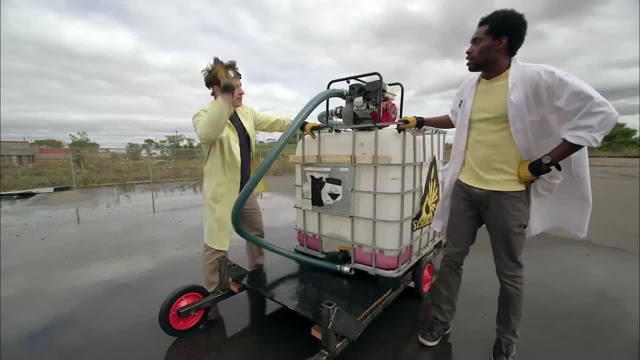 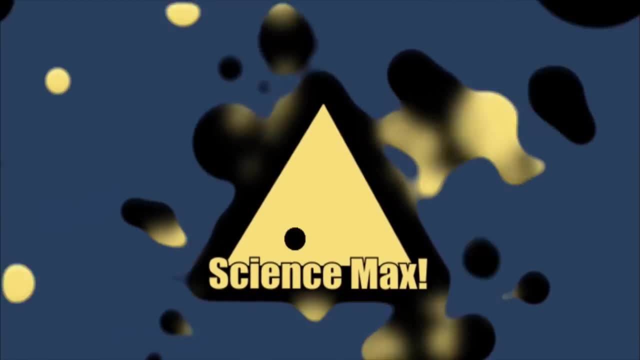 Exactly Right. Right, Okay, Okay. well, we can do that. Let's do. it Sounds good. Yeah, You know what? I have a paddle wheel because I had a failed hydroelectric. This is called fly boarding- Whoa. 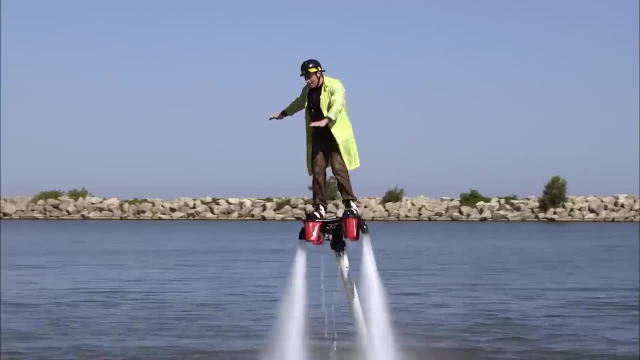 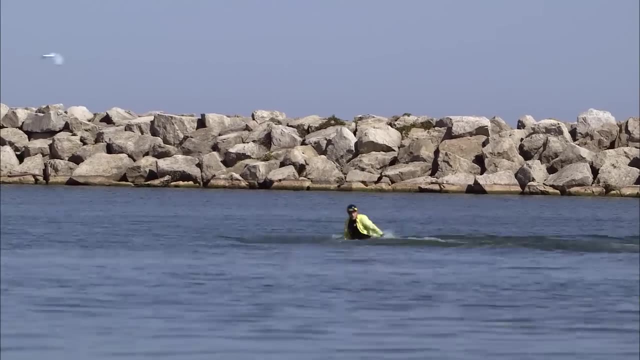 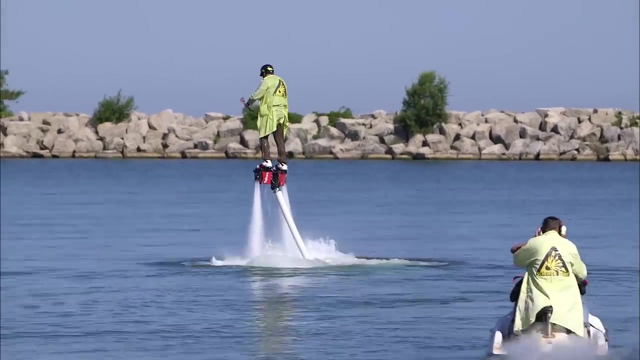 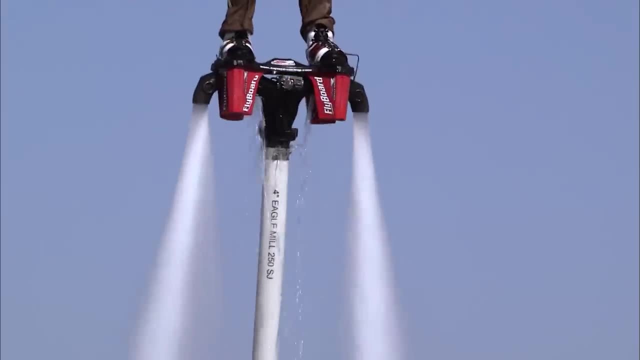 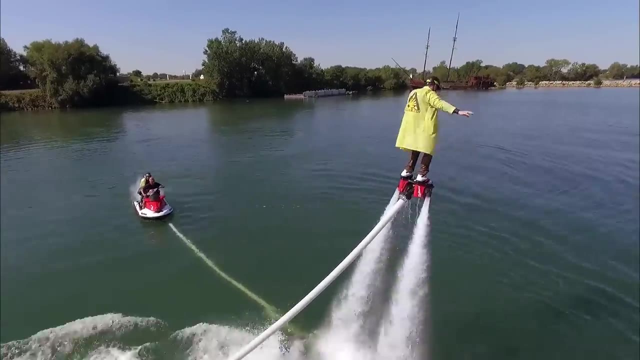 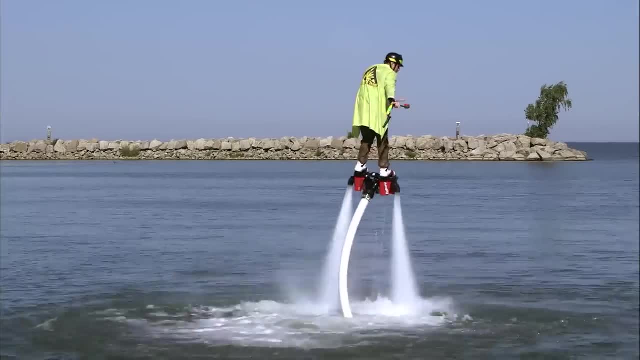 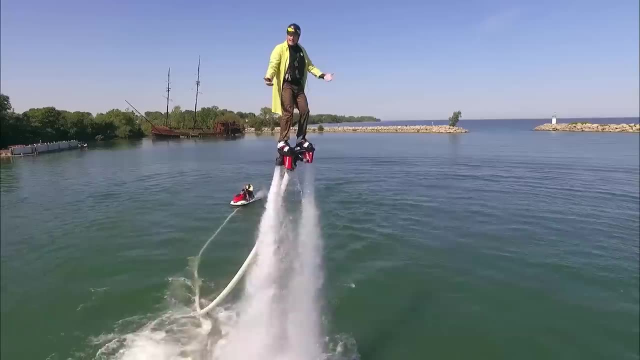 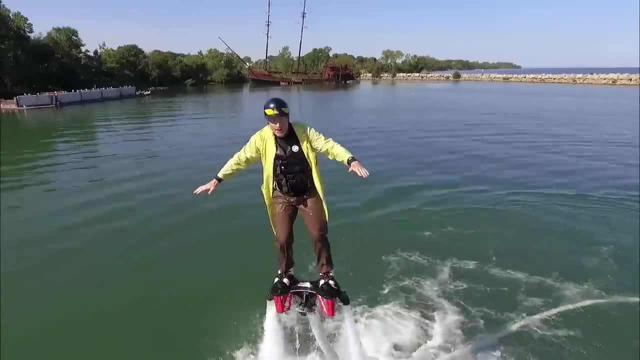 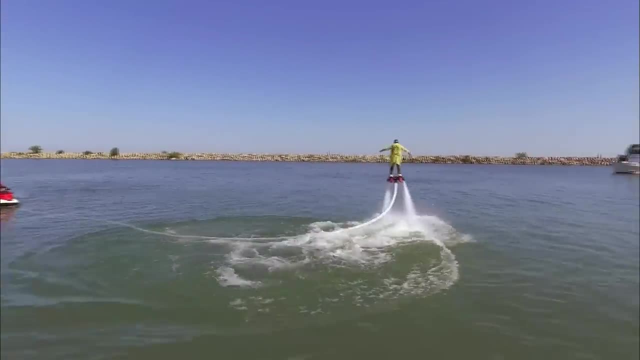 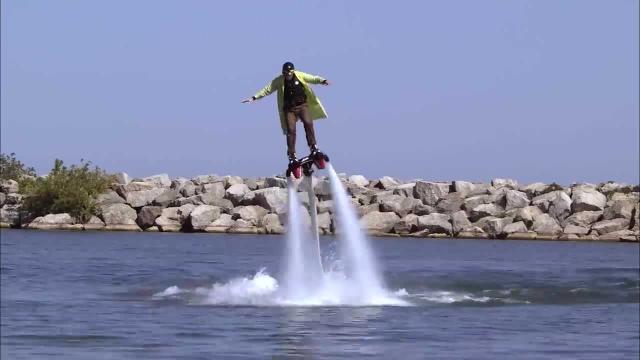 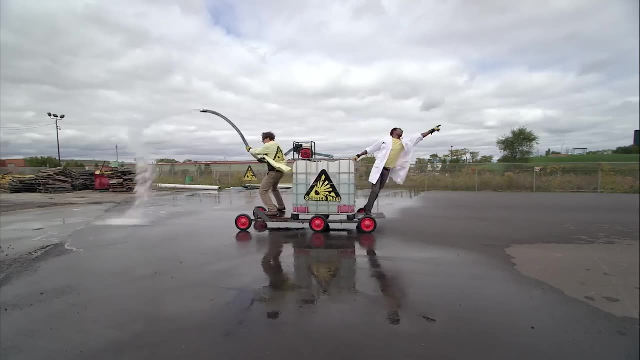 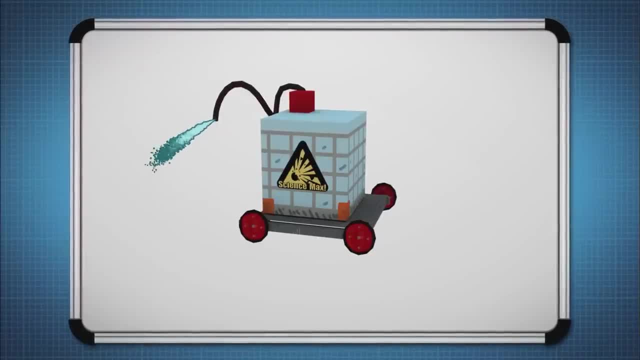 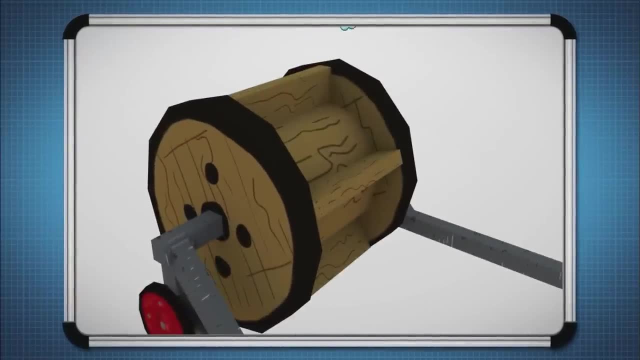 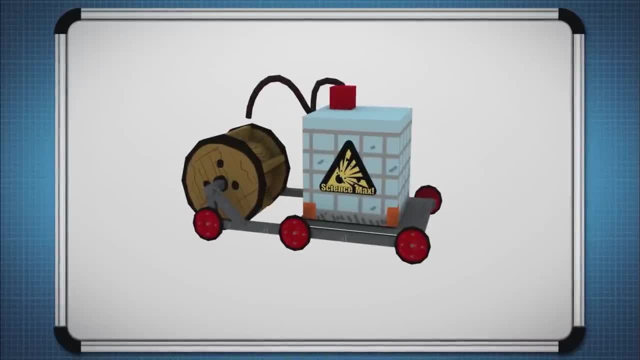 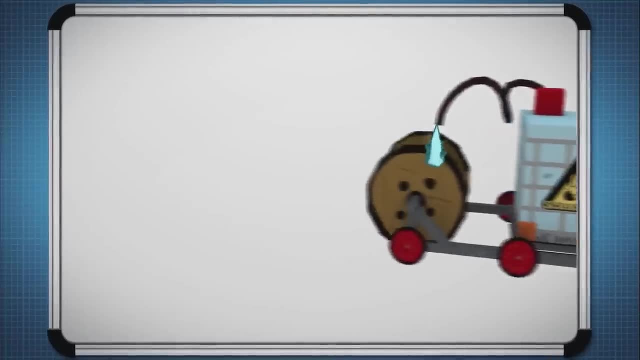 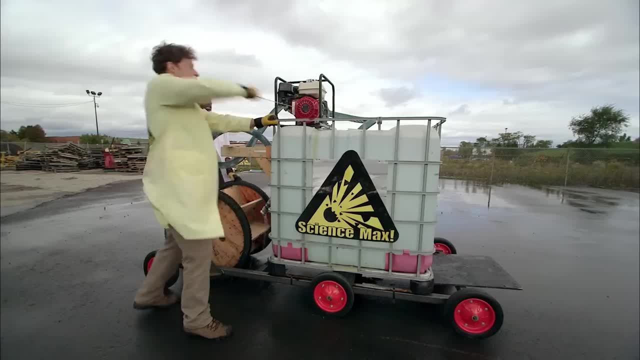 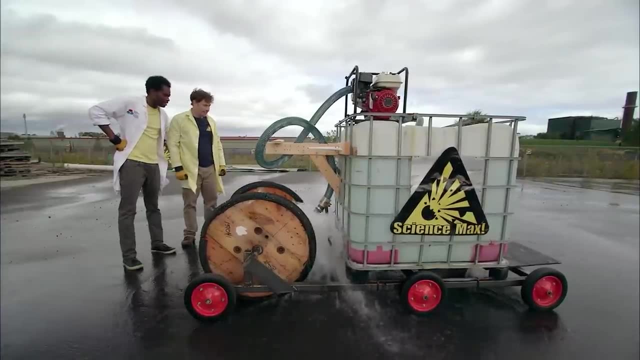 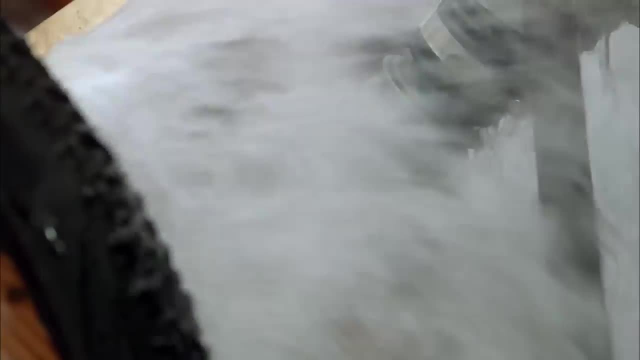 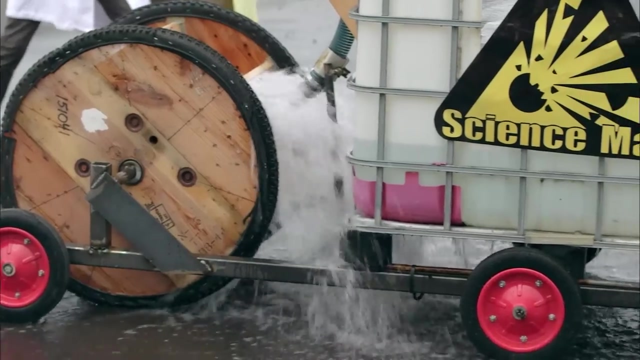 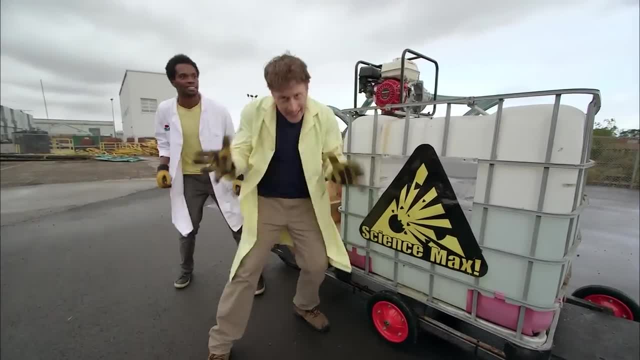 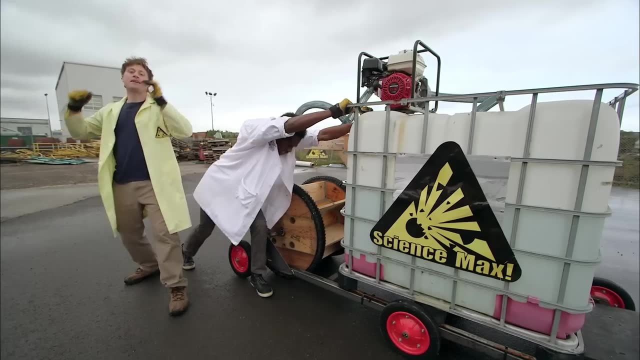 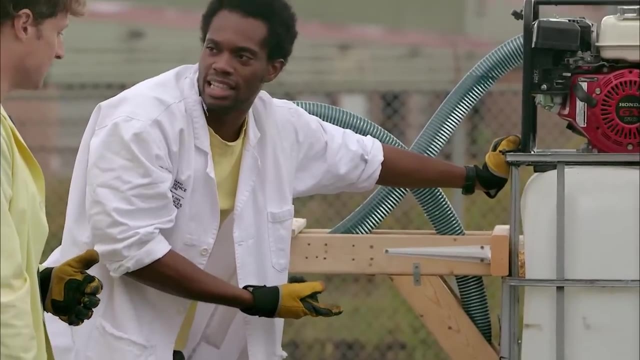 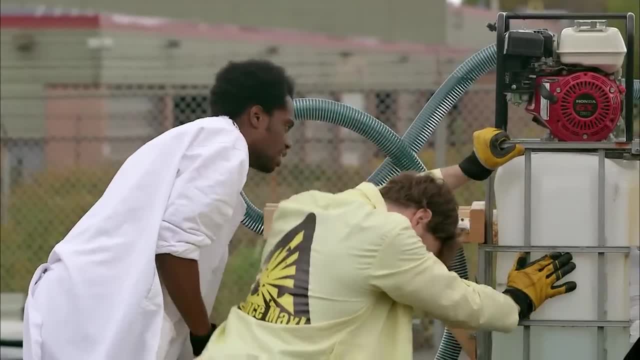 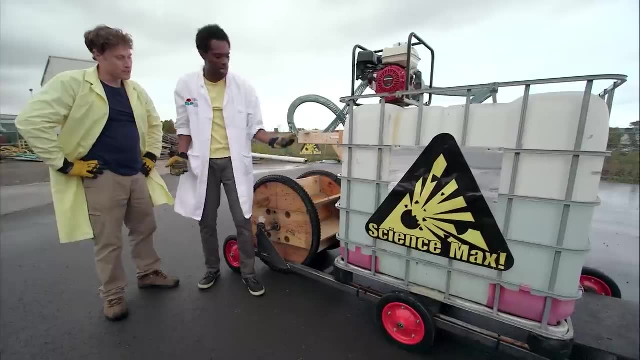 Whoa, Whoa, Whoa There's, Ah, There's. I can't. I can't even move this thing. What? I don't think. I think there's too much fuel, There's too much. Yeah, there's no way we can move this. 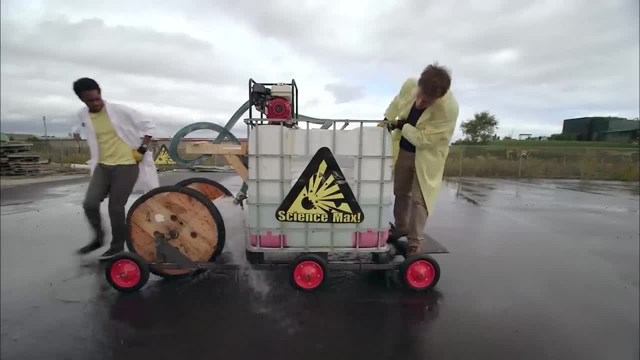 There's no way this is gonna be able to fly. so Even half full, you can't move. Even half full, I think we need less fuel. I mean we got to get it down to like maybe like a quarter or something like that. 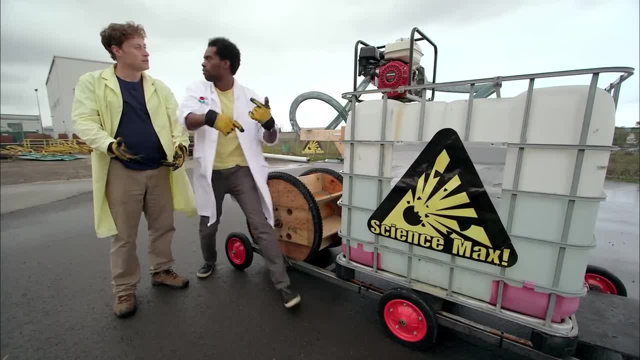 The thing is we ran it from the full tank last time and it never, it never moved at all. Okay, So What if we gave it like a push to kind of help it get over that little, like that little bump of energy? 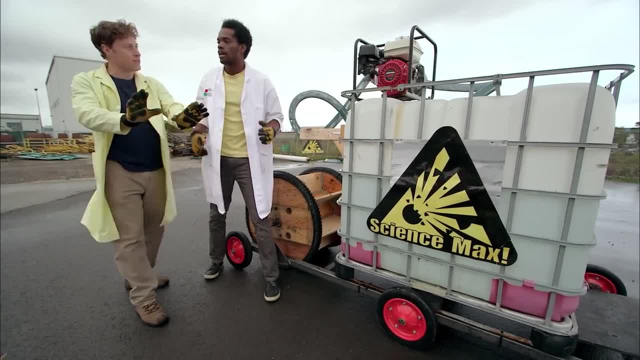 The first push, when it's still got a bunch of water in it. we give it a bit of a push and then maybe it'll go when it's done. Exactly, exactly, Okay, yeah, absolutely, let's do it. 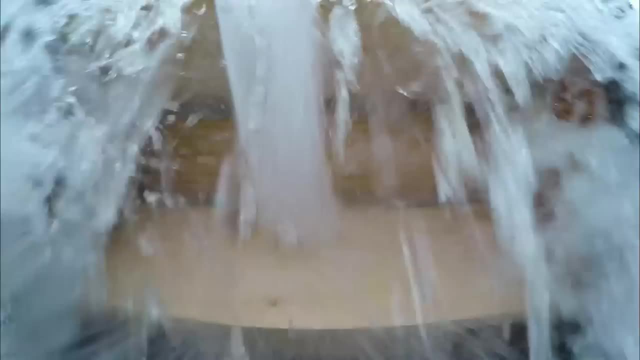 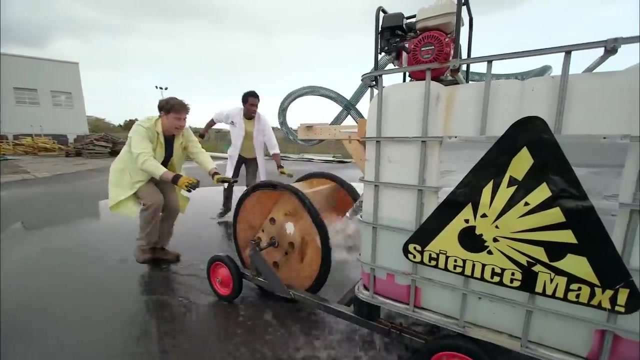 We start the pump and wait for the amount of water to get to just the right spot. Then we give it a push while it's still kind of heavy to start it moving. Sure enough, that push makes all the difference. Yeah, it's working. 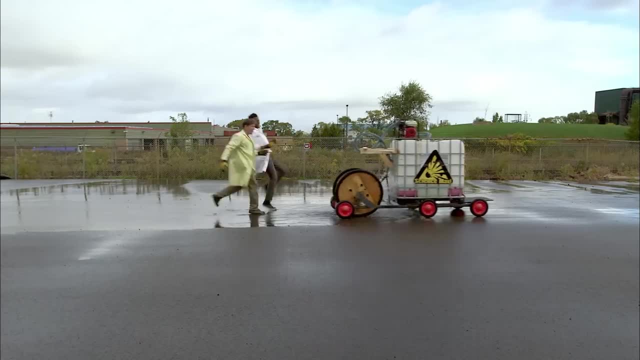 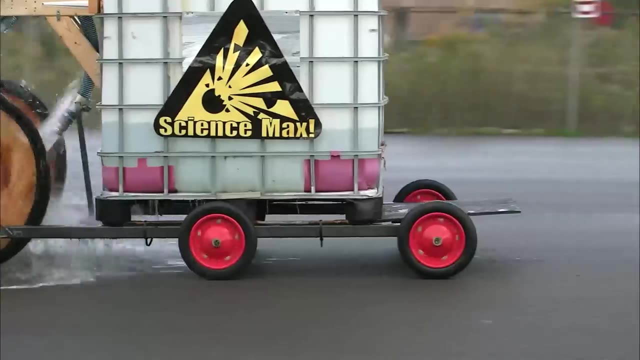 The water car is light enough to roll, has some momentum to keep it going and the force of the water coming out the pump is enough to keep it moving forward on its own. It's still going, Woo-hoo, All right, Amazing. 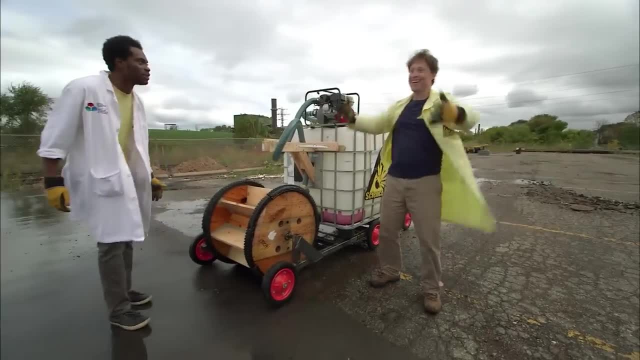 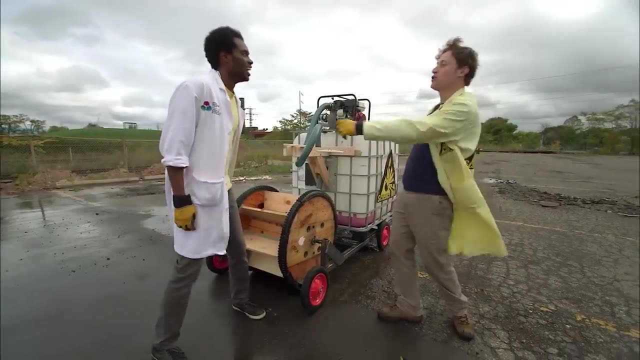 Yeah, Look at it, Man, this thing worked like a beauty. It worked all, it went all the way. Yeah, Way to go. The water car, finally a success. It was the push. It was the push. that's all we needed to get it going. 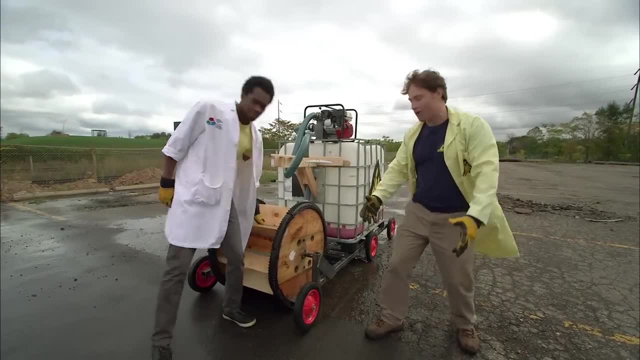 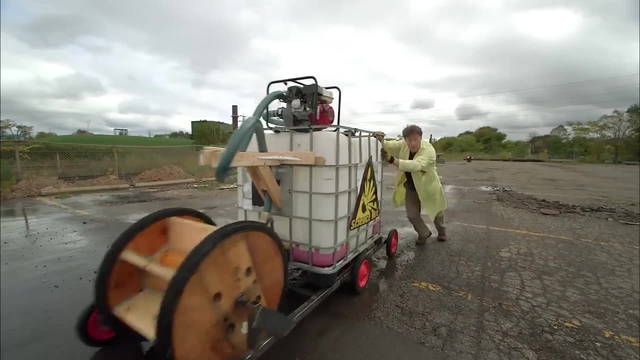 A bit of a push to get it going in a lot less water. and there you go, it totally works, All right. you want to do it again? Absolutely All right, here we go. Okay, See you next time on Science Max Experiments at Large. 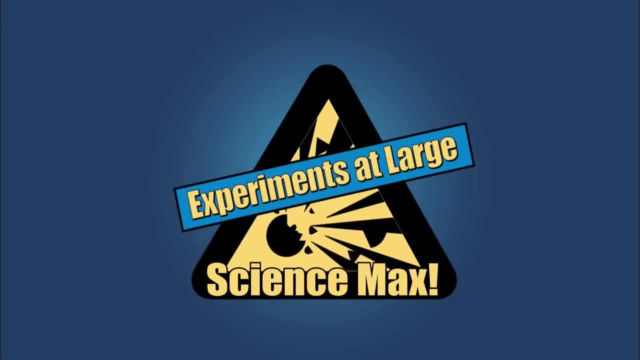 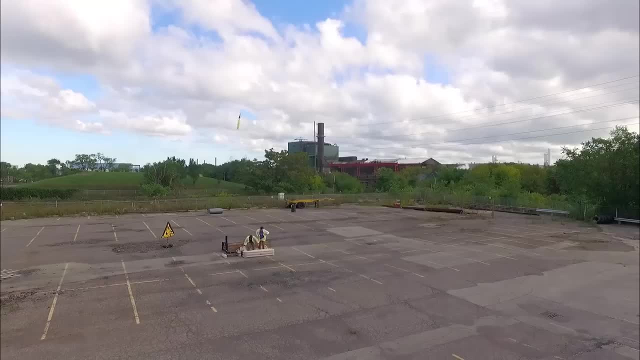 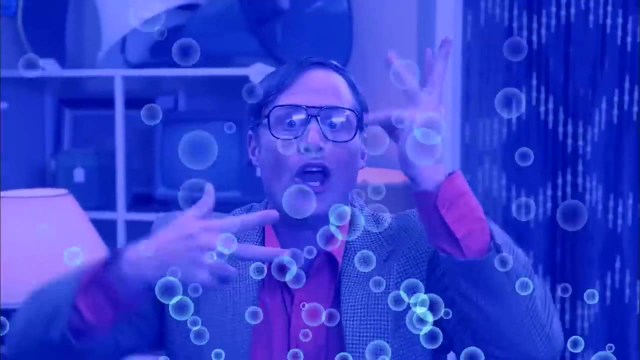 How much do you need to push it without any water inside it? Science Max. Today we're moving air. We're moving it through a tube to make a stomp rocket, vacuuming it out, turning it into a vortex and taking it with us underwater. 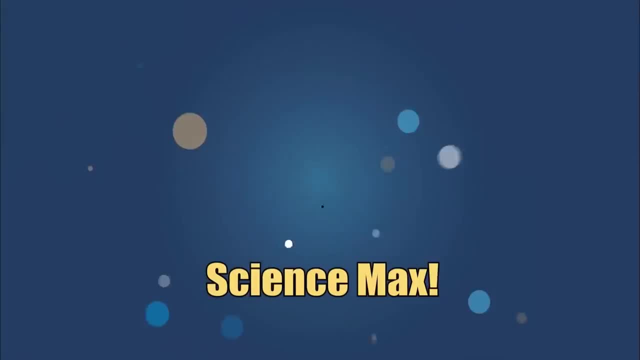 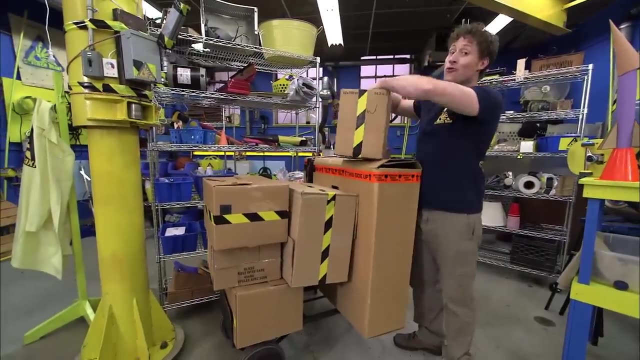 All on this episode of Science Max Experiments at Large. That was amazing. Greetings, Science Max-mites. My name is Phil and it's moving day today on Science Max Experiments at Large. Let's see where do I put this. 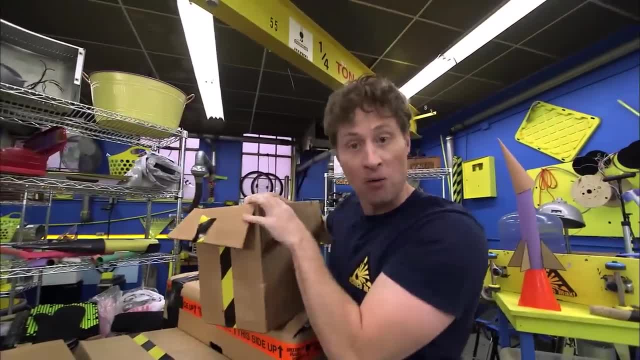 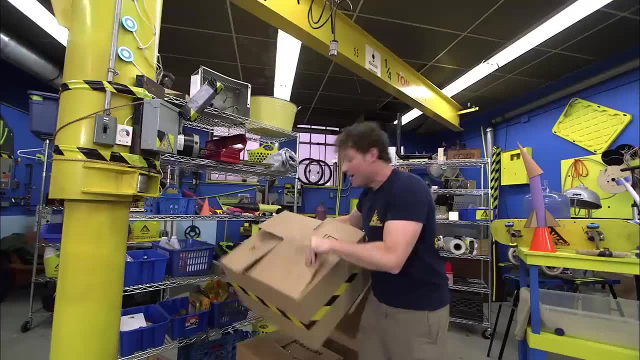 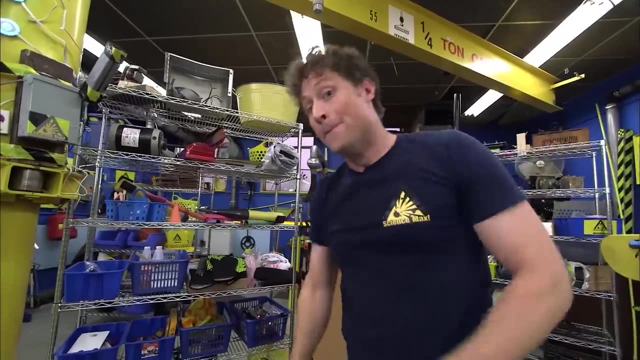 This is probably a good spot. Today we are moving air. You probably don't think that moving air will have a huge effect, but you'd be surprised what you can do by just moving air. But don't worry, we're not just going to move the air around in boxes. 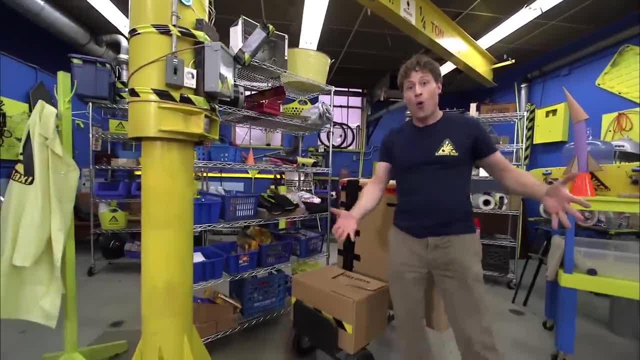 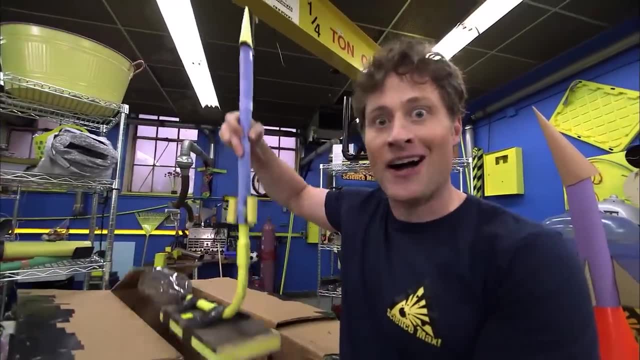 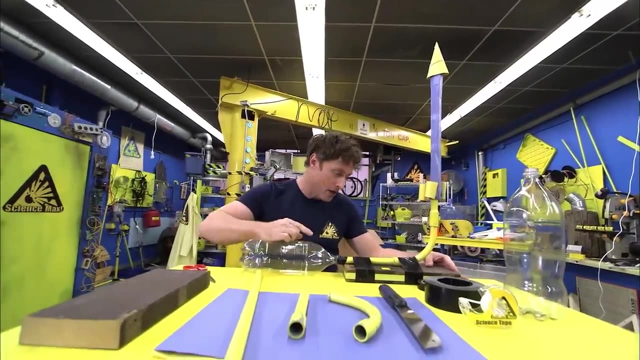 We are going to be moving the air around in boxes. We are going to be moving the air around in boxes. We are going to build a rocket, And this rocket uses the science of stomping on something with your foot. This is a stomp rocket and it works by stomping on this plastic bottle. 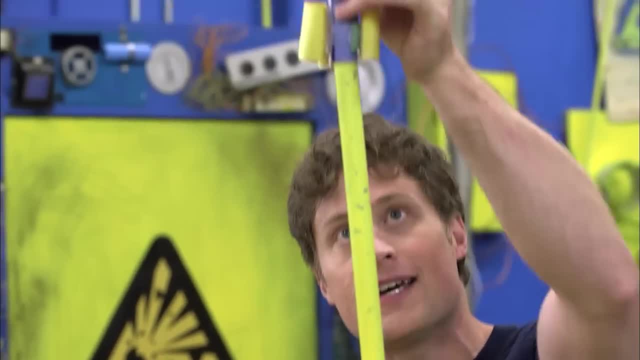 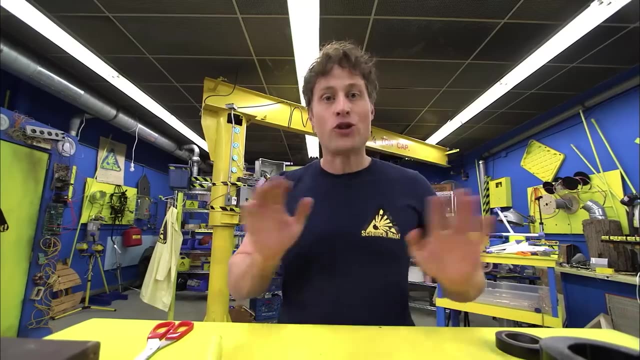 and air shoots through this tube and pushes the rocket up into the sky. And here is how you can build one of your very own. And remember, if I go too fast, don't worry. All of the steps are on the website, so you can follow along at your own speed. 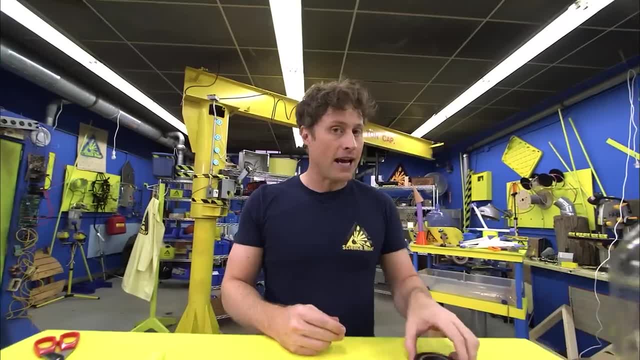 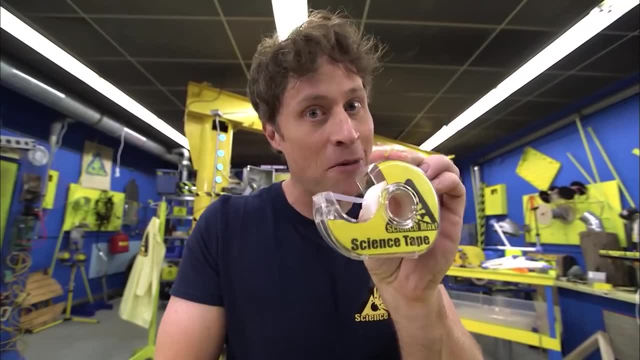 All you need is a two-liter plastic bottle, three kinds of tape: electrical tape, duct tape and science tape. Science tape is just the same as invisible tape, but I use this kind of tape for science. Then you want some plumber's tubing and some construction paper. 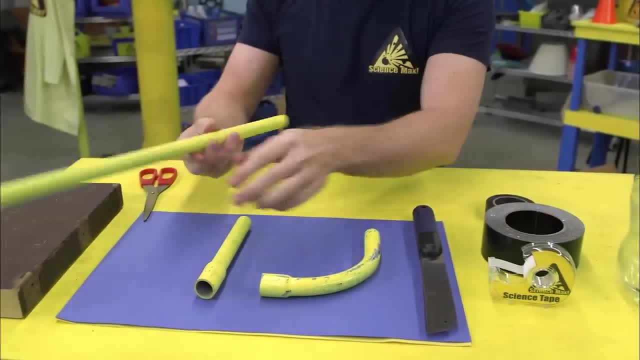 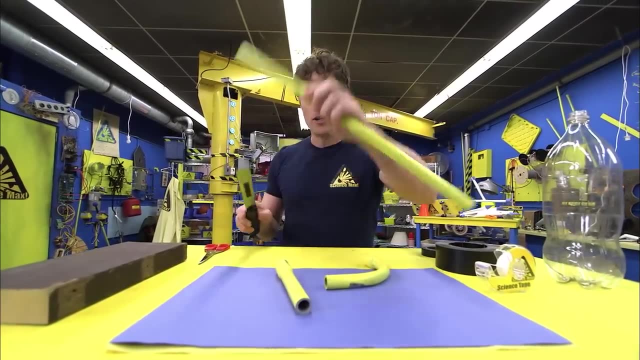 to make your actual rocket. First, you want to take your plumber's tubing and cut it into three lengths- And when I say you, I mean an adult, because you need to use a saw. So you saw it up into a long piece, a short piece. 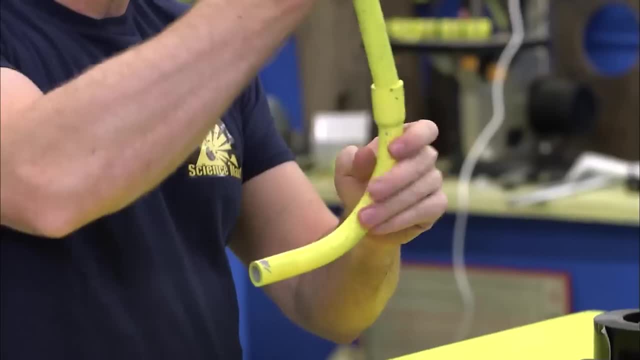 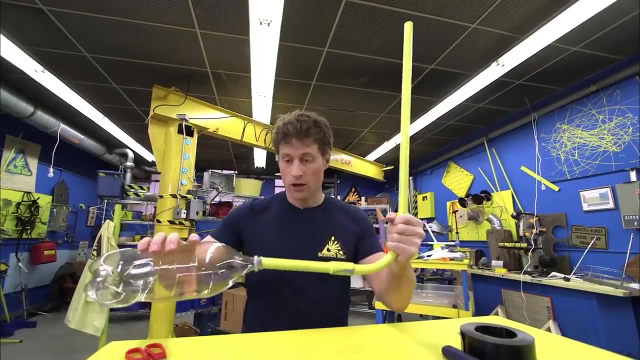 and an elbow piece. We want to make a long tube at the top, and then we also want to make a tube at the bottom so we can attach our two-liter bottle to. And there we go, Ta-da Ready to go, But of course it doesn't stay up. 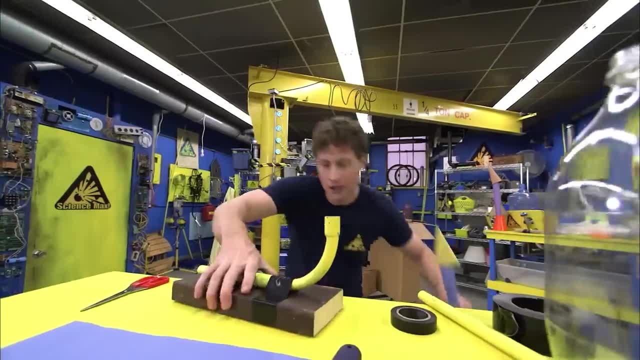 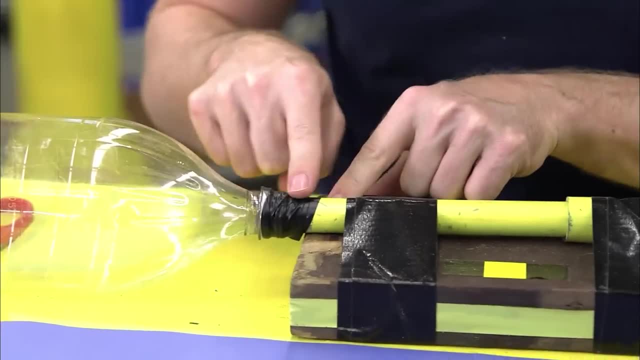 so we have to attach it to a base And it will look like this And you see, it's been attached with duct tape here and I've used electrical tape and I've wrapped that part around there. Now building the rocket. 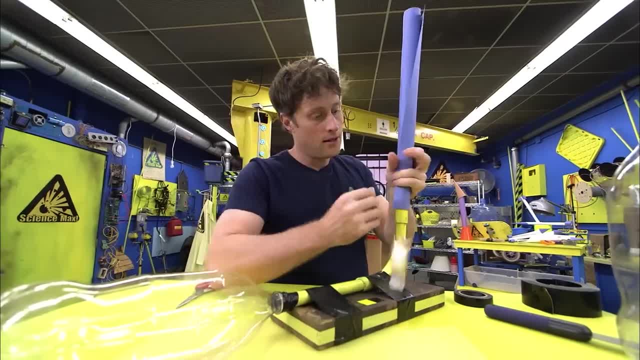 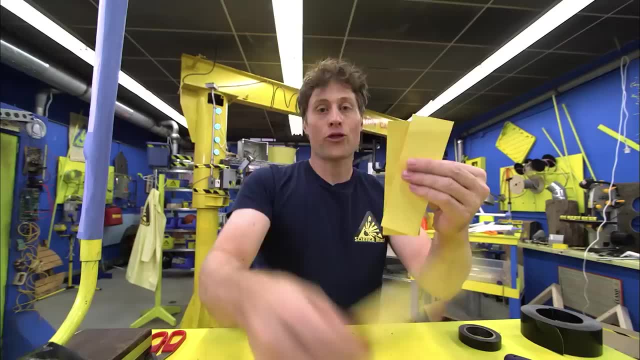 Wrap the paper around the tube and tape it with your science tape. Tape the top closed so no air escapes. Then cut a semicircle to make the nose cone and three hoops for thrusters and tape them to the bottom. There you go. 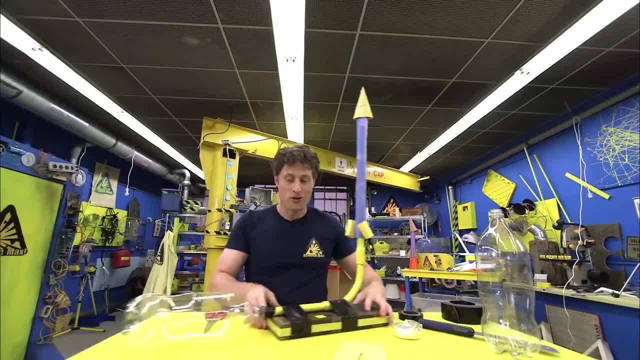 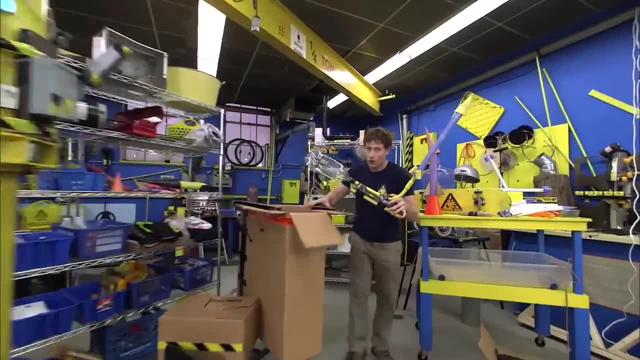 The rocket fits on the tube just like that, And when you stomp on this bottle, it launches. But here's the most important part, the one most important rule of launching rockets: You shoot rockets, You stomp rockets outside. Come on. 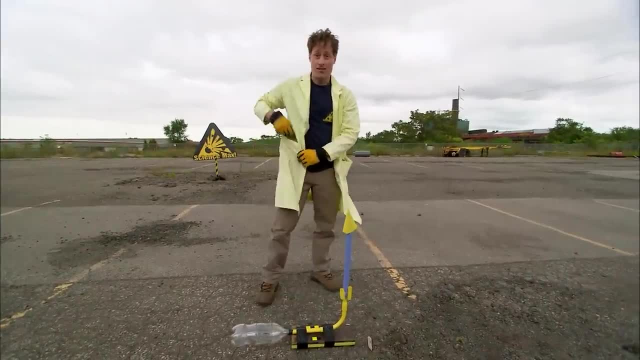 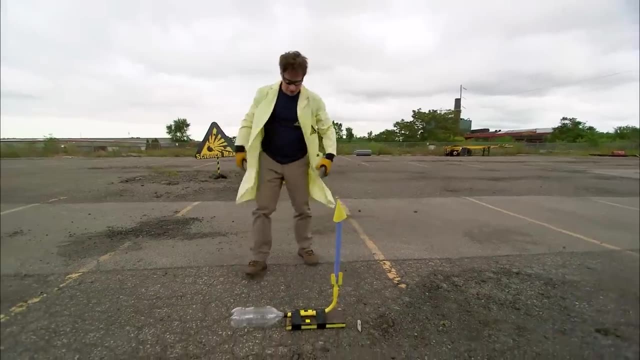 Once you get outside to a nice open area and you bring your safety glasses with you, all you need to do to make the stomp rocket work is, of course, stomp on it. You ready, Here we go. Three, two, one. 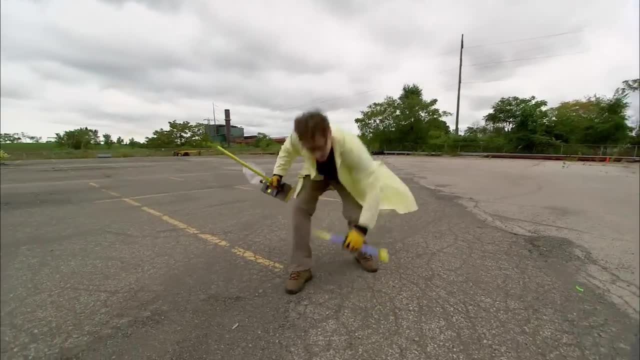 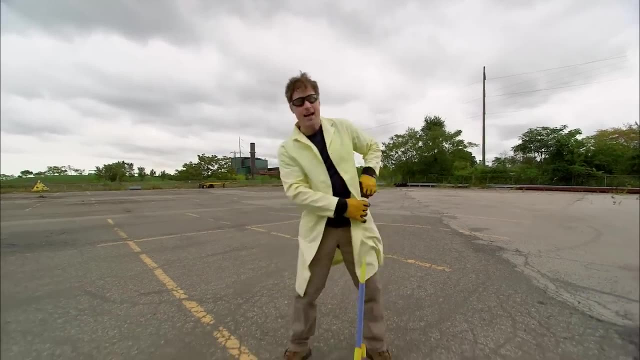 Whoa, Did you see that? That was amazing. OK, so this is where we're going to start with the stomp rocket. I'm going to meet Chris from Logics Academy and he's going to help me max it out. 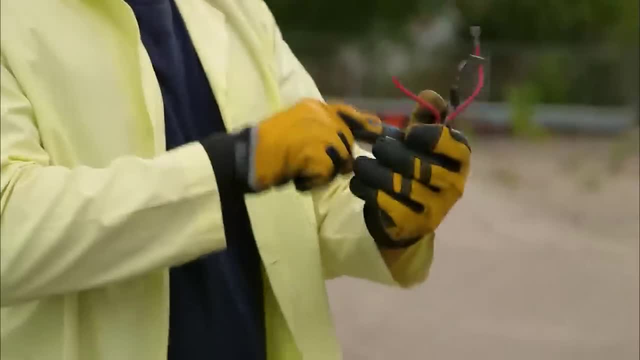 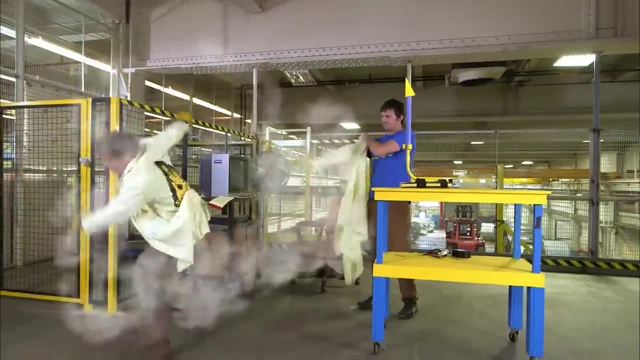 In fact, he's probably at Science Max headquarters already. I should get over there, OK, where is the? Oh, there it is. OK. How are you doing? It's good to see you. You too, Chris, is from Logics Academy. 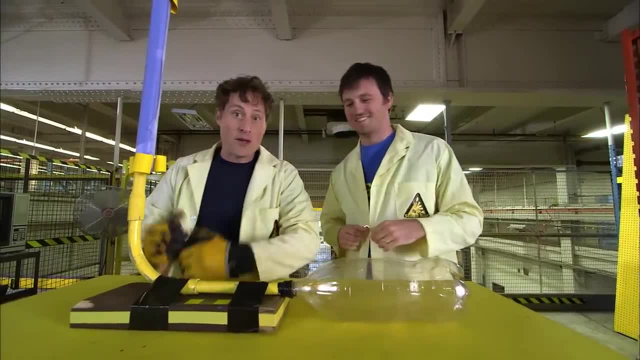 and you guys do in-class robotics workshops- right, That's right, we do Great. Well, I was hoping I could get your expertise to help me max out the stomp rocket. Yeah, Logics makes one of these. I totally think I can help you with that. 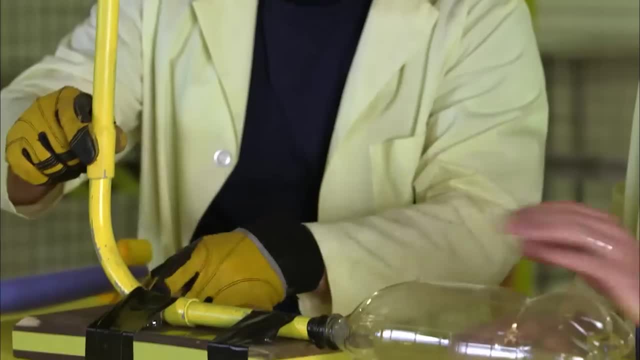 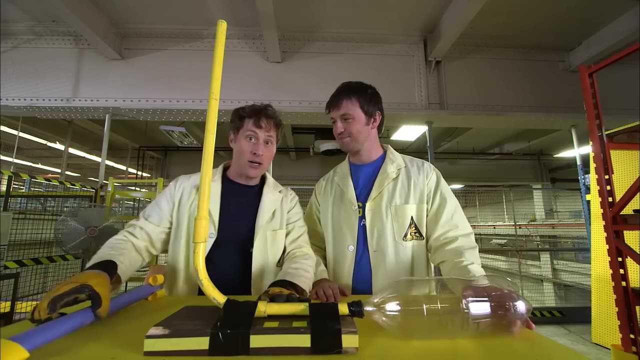 Fantastic. So it works great. Let's get bigger, better, more maxed out. First off, we can start by making this pipe a little bit bigger. so: larger pipe, more airflow, bigger launch. OK, let's do it. 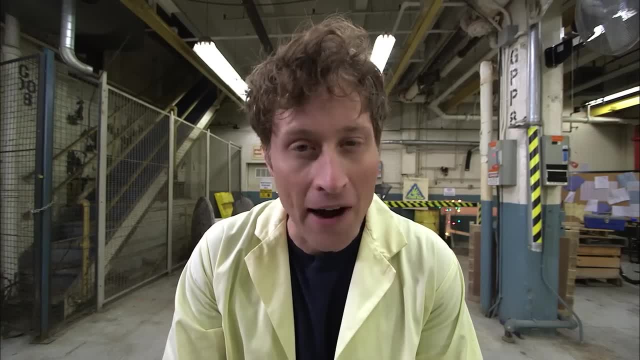 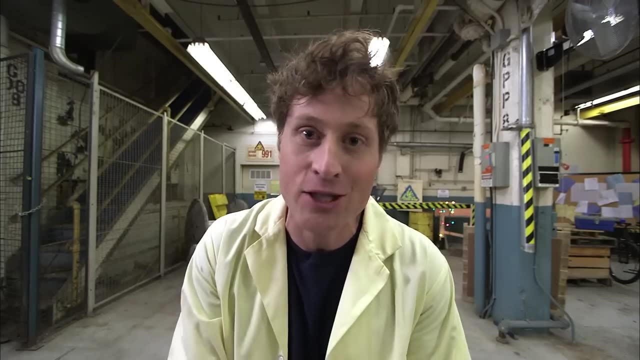 Cool. Moving air isn't that hard, right? I mean, air is super light. How hard can it be to move? Well, here's an experiment you can do that lets you measure how hard it is to move air. So what I'm going to do is I'm going to hit the ruler with the 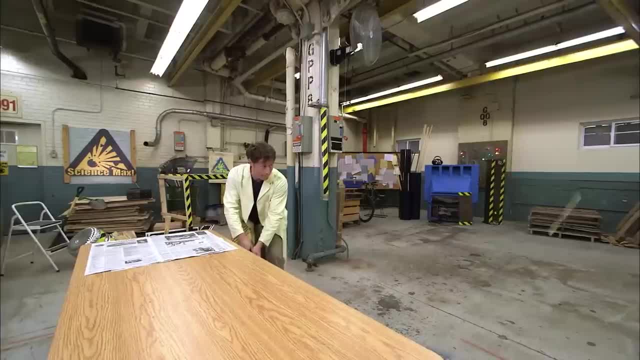 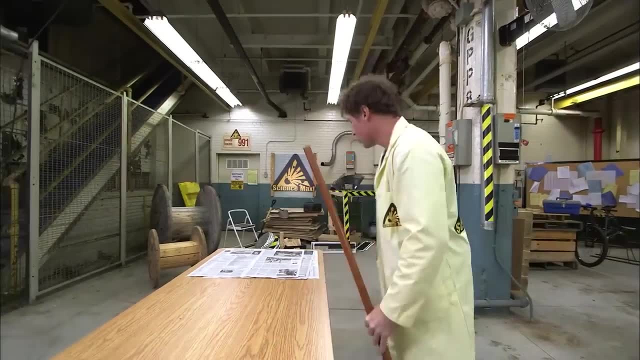 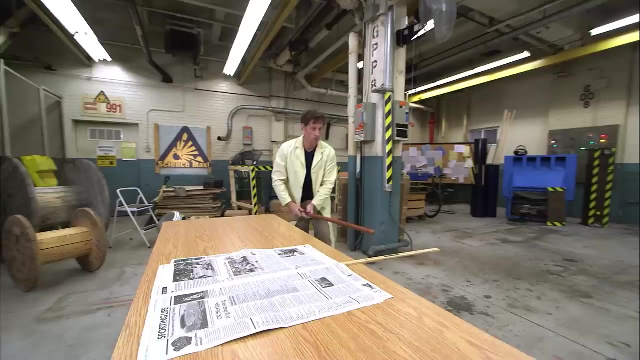 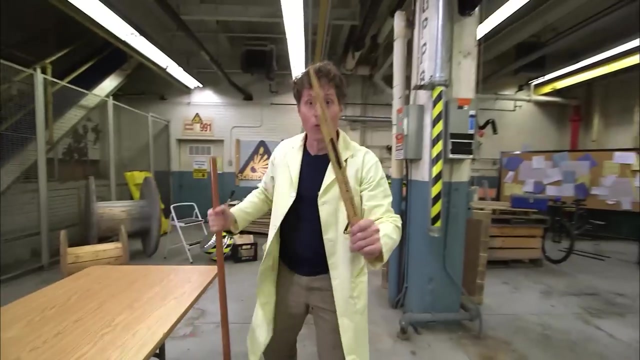 broom. It's going to go over there. I hit it and it moved, No problem. So we're going to do it again, except I'm going to add just a couple pieces of newspaper. All right, ready? Aha, the ruler broke because this time I wasn't just moving. 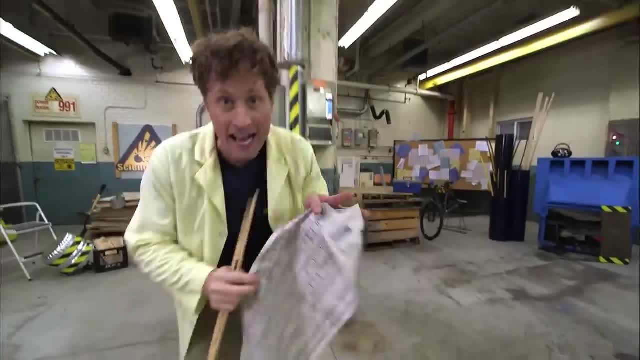 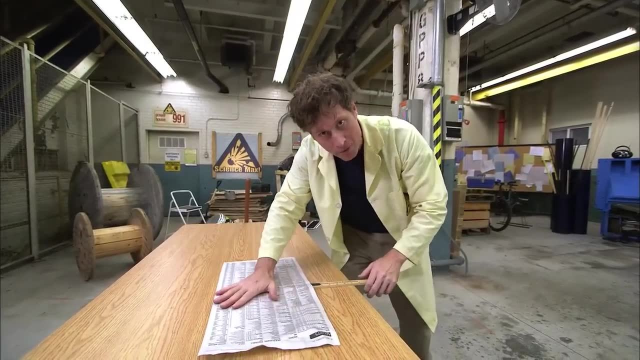 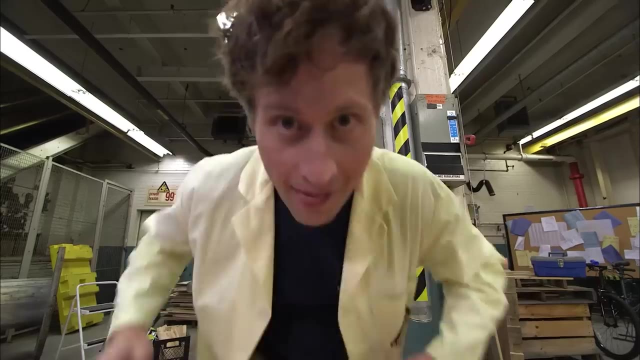 the ruler. I wasn't just moving the ruler and the newspaper, I had to move the ruler, the newspaper and all of the air that was on top of the newspaper, And that resistance was enough to break the ruler. Pretty good experiment, right. 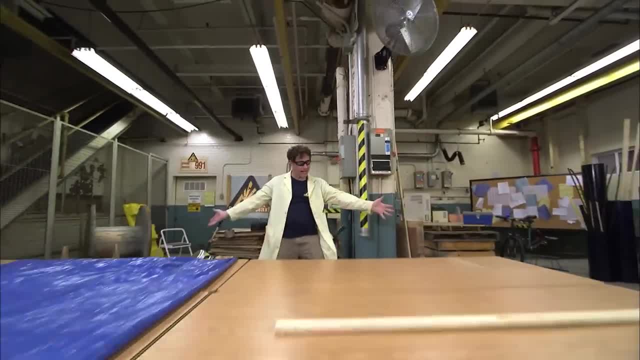 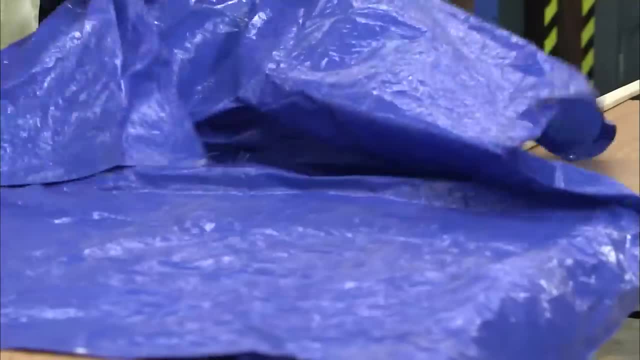 Let's max it out. I've got more table space, I've got a piece of lumber And instead of a newspaper, I have a tarp. Now the tarp is very light. It is not the weight of the tarp that is going to be the 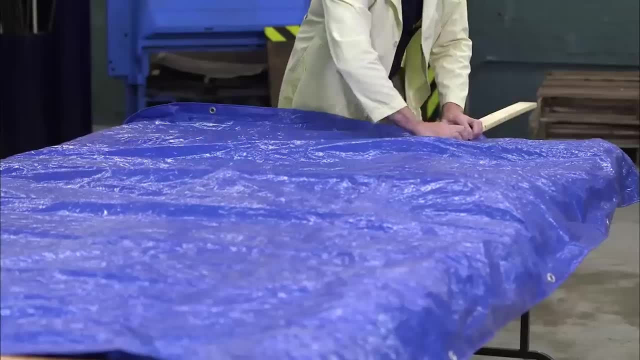 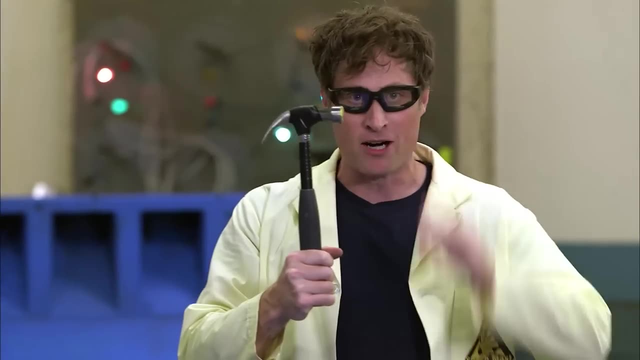 difference. It is how much air. All right, I need to move when I hit this piece of lumber And I've got a science max hammer. So, first of all, you're not going to try this at home, right Deal? 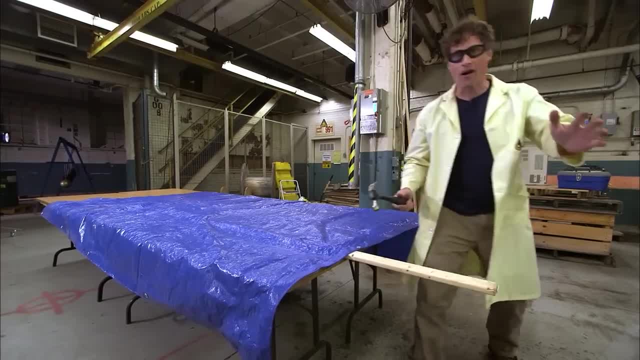 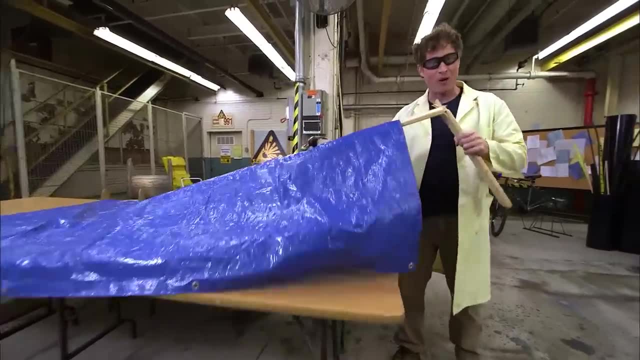 Okay deal, No trying this at home. Okay, here we go, Moving air test 2.0. It broke And it didn't even move. Did you see that? I wonder if we can max this out even more. 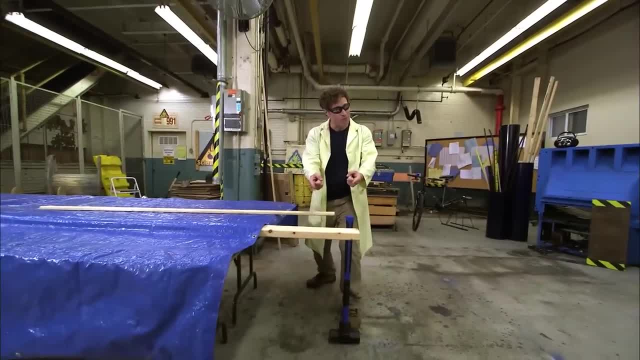 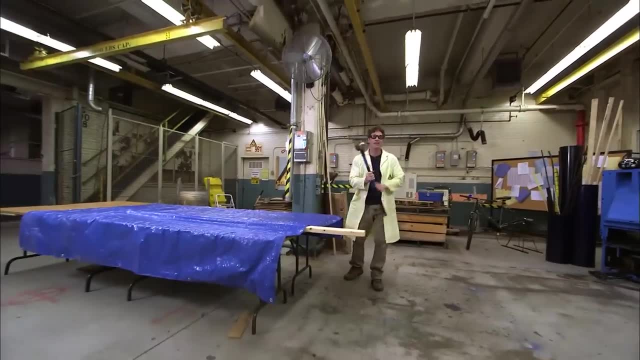 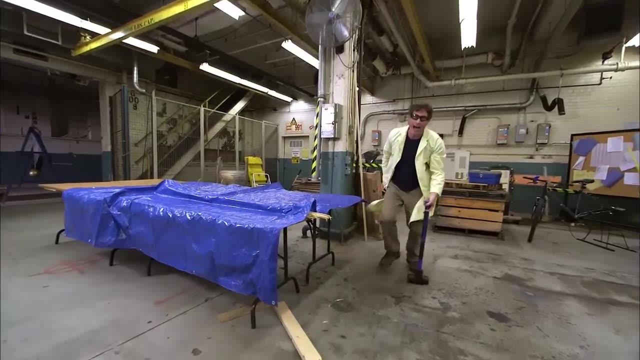 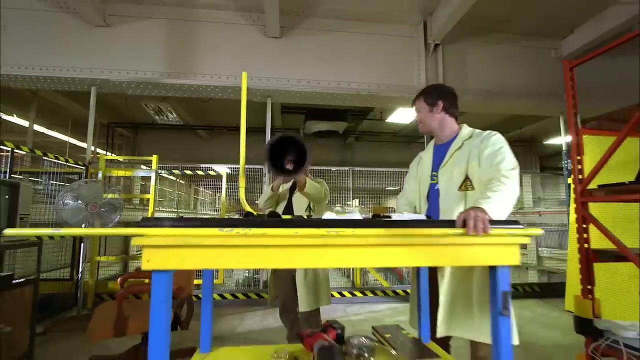 Two by four, which is much bigger than the piece of wood we used last time, And a sledgehammer. Here we go, Moving air experiment 3.0. Yeah, Science, Whoa. So I've joined Chris from Logix Academy and we are maxing out. 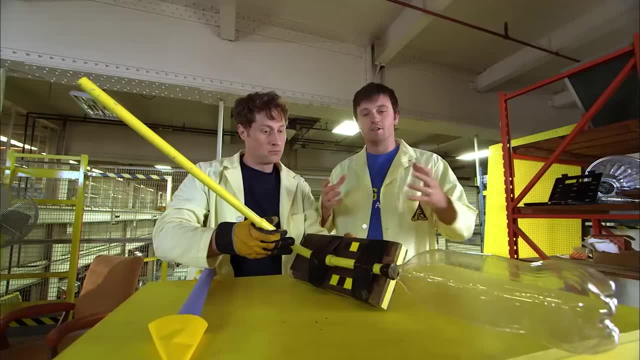 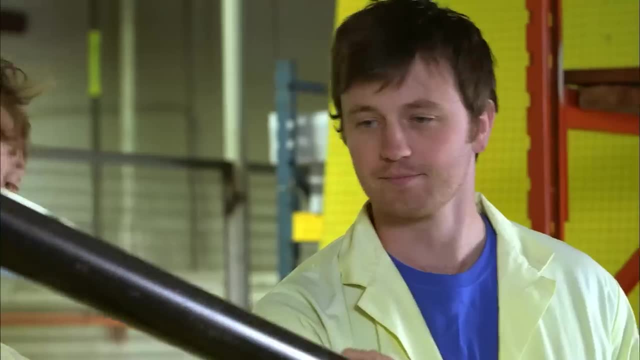 our stomp rocket. To do that, we're going to use Larger pipe, more air flow, bigger launch. The theory is that moving a larger volume of air through wider pipes will make our rocket work even better. So we get to work. 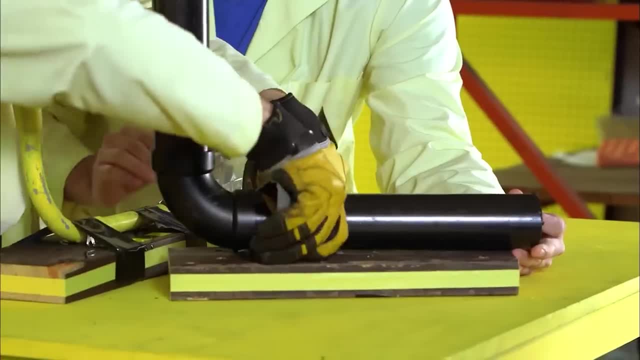 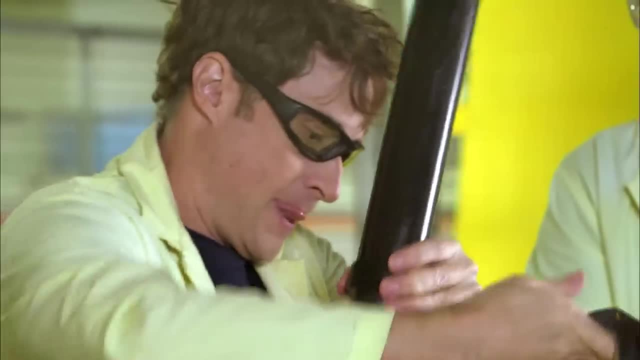 This version is built exactly the same. We cut and attach the pipes- a long piece, an elbow and a short piece- then secure them all down. We attach the plastic water bottle and tape it so it's air tight, and then the only thing to do is make a new rocket then. 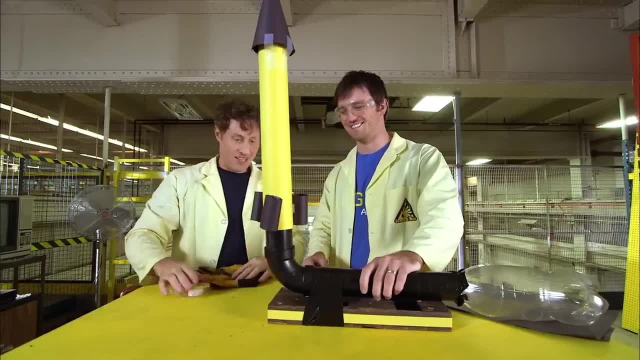 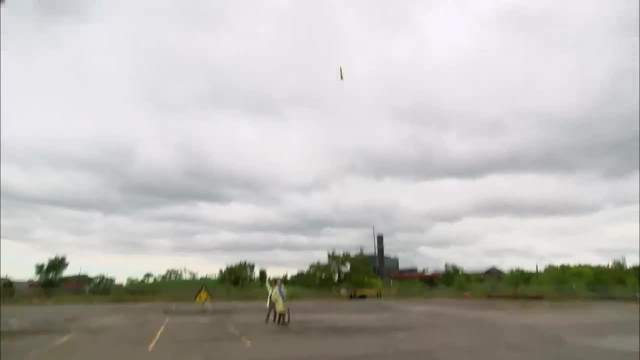 it's done. It's a rocket that fits over the larger pipe. Ready to try it? I'm ready to try it. All right, let's do it. Let's go. One, two, three go. Yeah, One, two, three go. 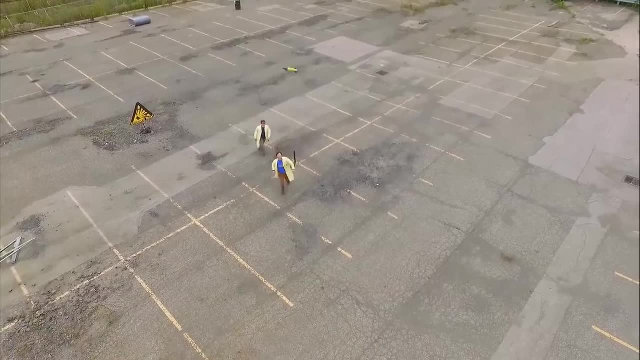 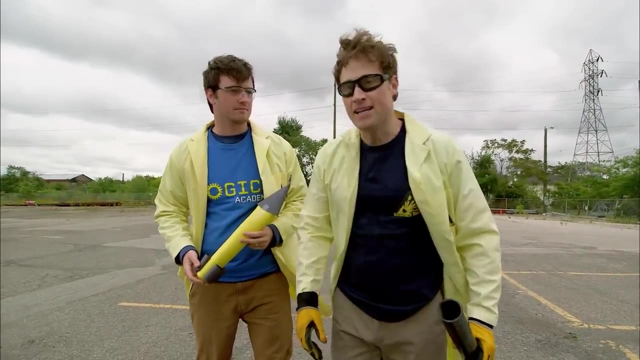 That was amazing. In the end, though, it worked. it wasn't much better than the smaller rocket. I think we could still do better, right? Oh yeah, This is Science Max, not Science Medium, Right, Okay, Let's go back to Science Max headquarters. 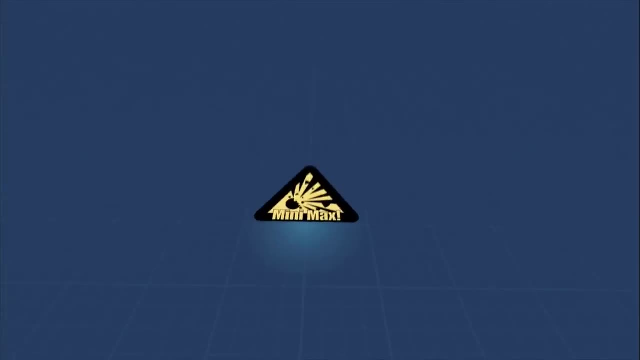 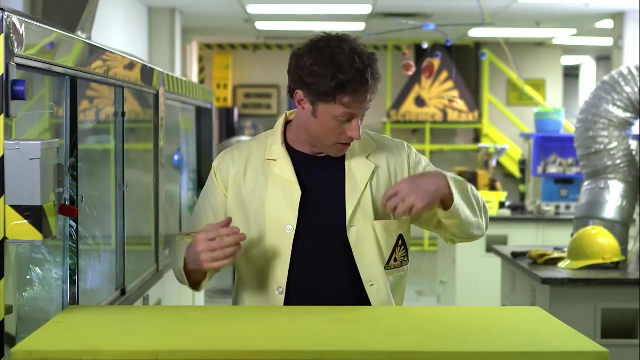 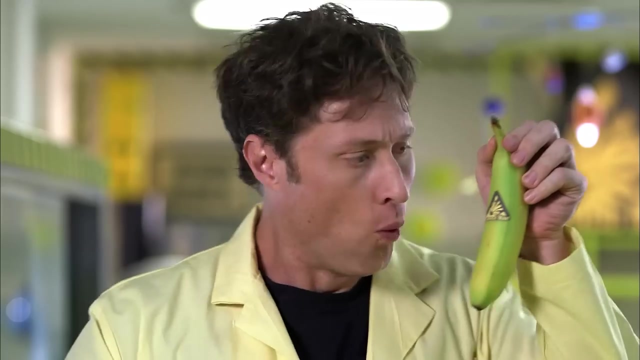 We're back, Let's go Mini Max. Vacuum sealing- That's what you call it when you take all of the air out of something, often a bag, to seal in the freshness of food. I will demonstrate using this Science: Max banana. 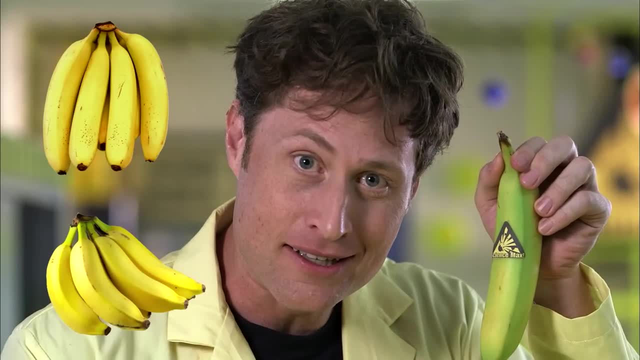 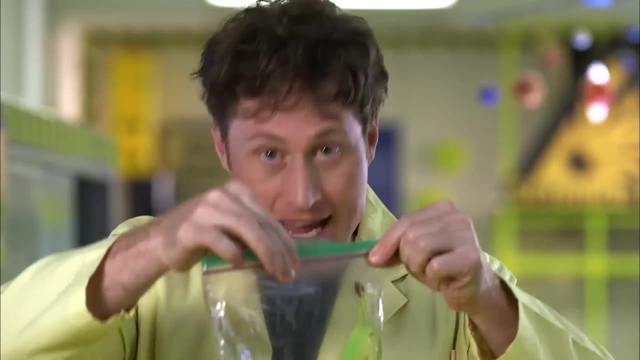 100% banana, but with added science. Not all bananas contain science. Here's how you can do it at home. Put your food in a bag, seal it most of the way, because we have the air from the bag, And we will do that with a straw. 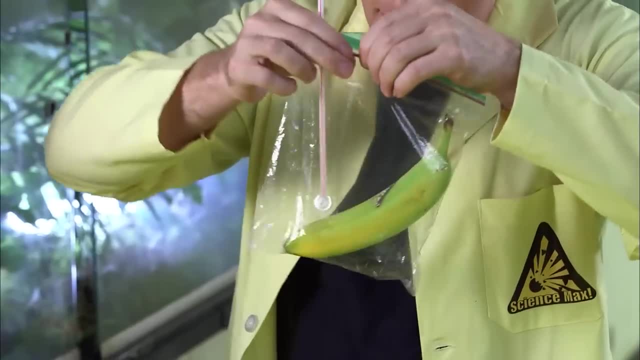 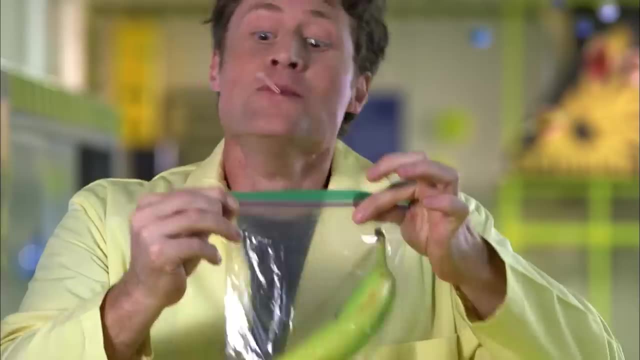 Put a straw inside the bag and then suck the air out of the bag and then seal it. at the very last second There a vacuum sealed banana. Now I know it's kind of hard to see that it's been vacuum sealed. 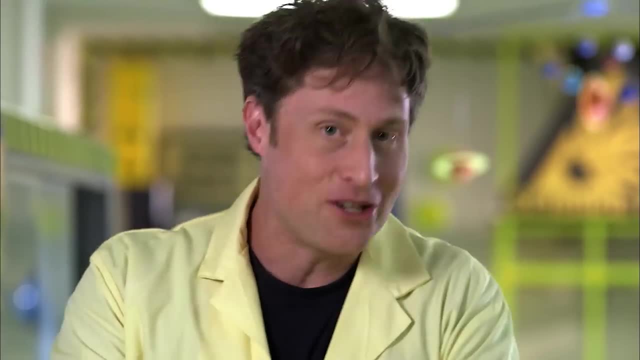 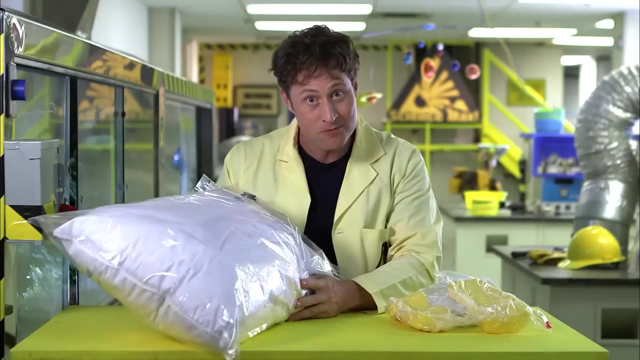 because bananas don't really crush much when you take the air out, So I like to use stuff that has a lot of air in it to begin with. In fact, there are special bags that are specifically for vacuum sealing that are supposed to store big and bulky items. 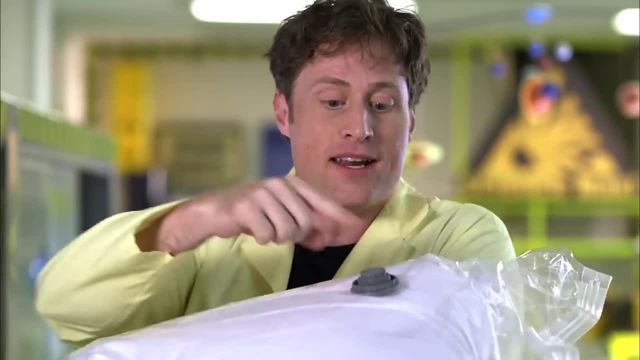 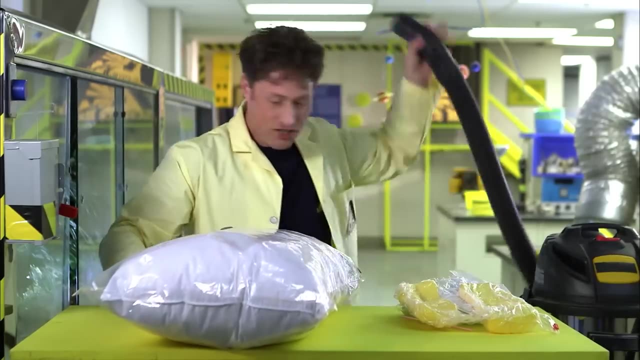 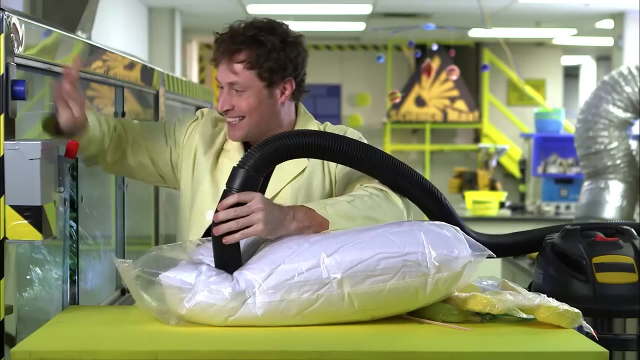 that have a lot of air in them, like this pillow. See this nozzle right here. It's designed to be used with a vacuum, So what you do is you put the vacuum on this nozzle, open it up and then you turn the vacuum on. 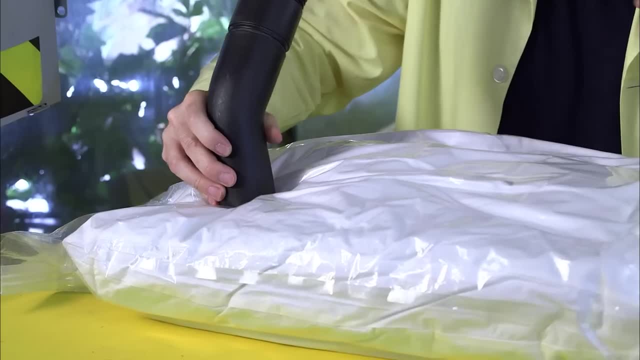 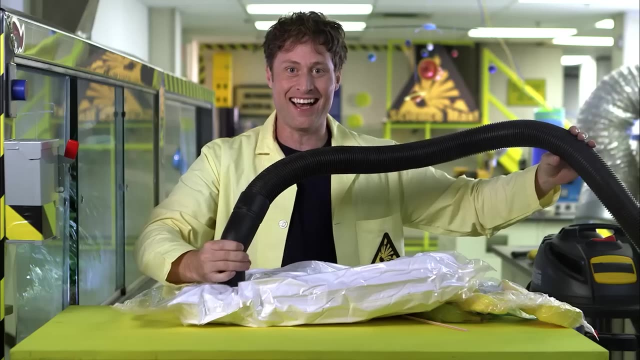 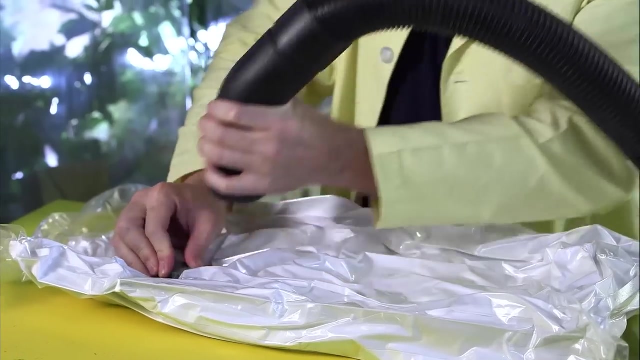 Oh, The vacuum is sucking all the air out of the bag, just like we did with the banana. But because the pillow is full of air as well, it starts to shrink and shrink. Then you pull off the vacuum and you tie the seal off. 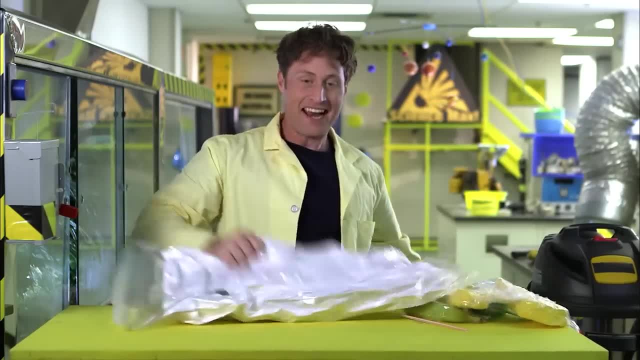 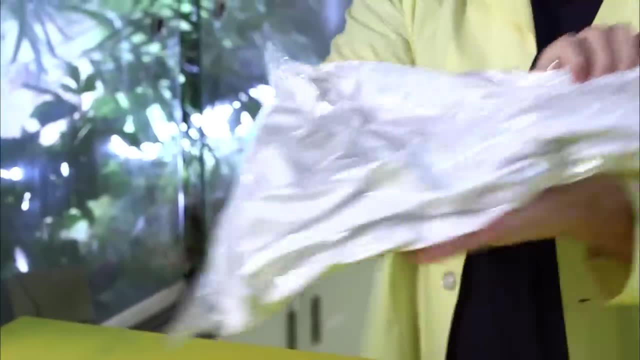 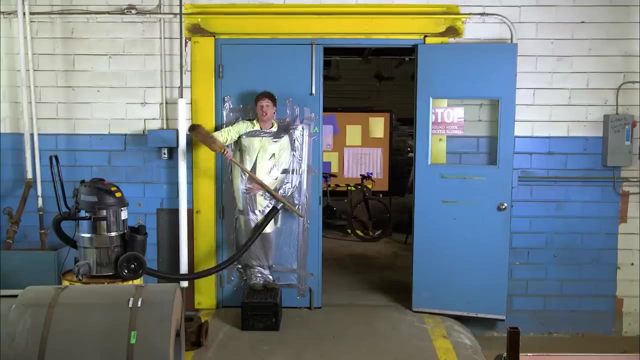 And all right and ta-da, a vacuum sealed pillow. Okay, let's max it out. What could possibly be more maxed out than a vacuum sealed pillow? Vacuum sealed fill- Okay, I put plastic bags against the door and then sealed the edges with duct tape. 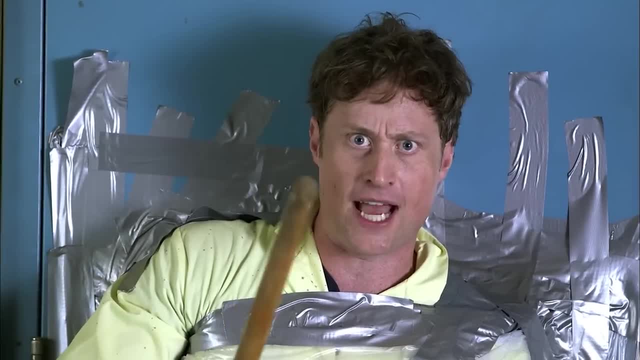 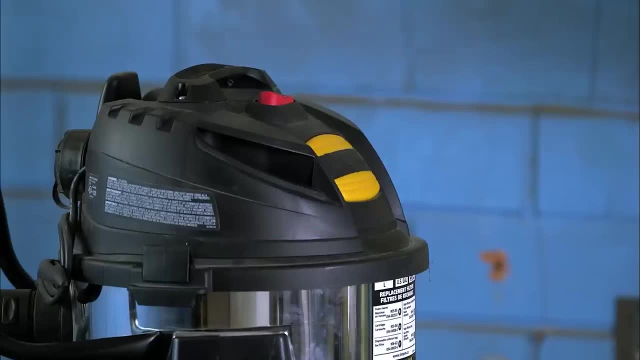 And, of course, I didn't put any plastic over my head, because you never put your head in a plastic bag, right? Well, let's see if vacuum sealed fill it works. Whoa, Hey, it's working, Ha-ha. 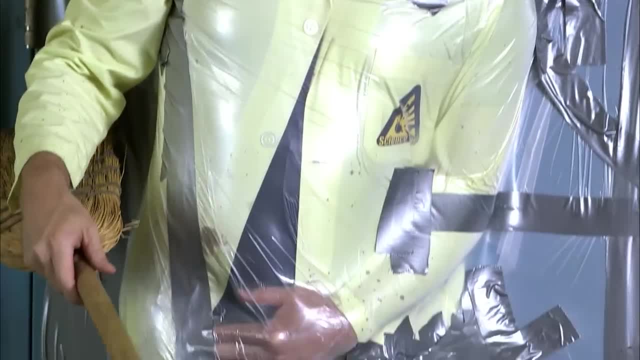 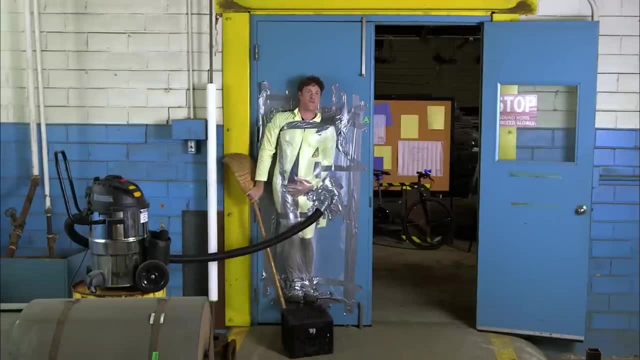 The vacuum sucks all the air from the bag, which seals the bag and me in it to the wall. That means Whoa. I should be able to knock this milk crate out from under me. Air pressure or the lack of air pressure. 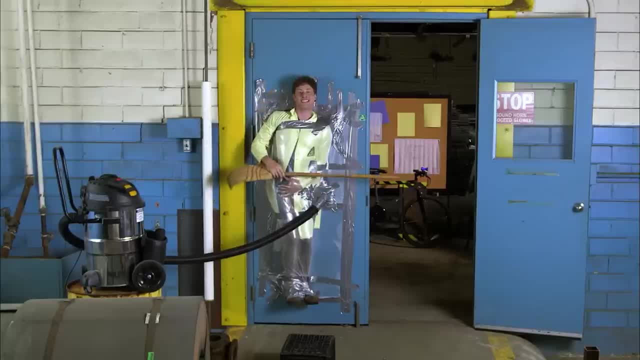 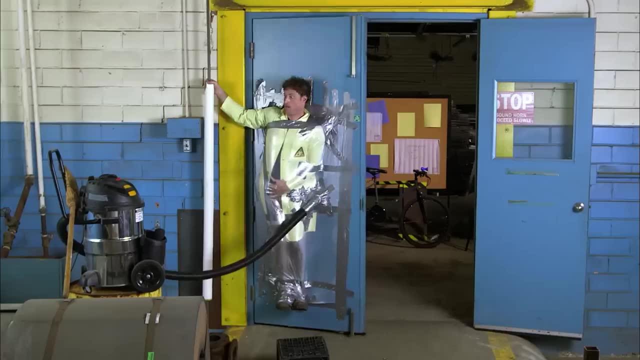 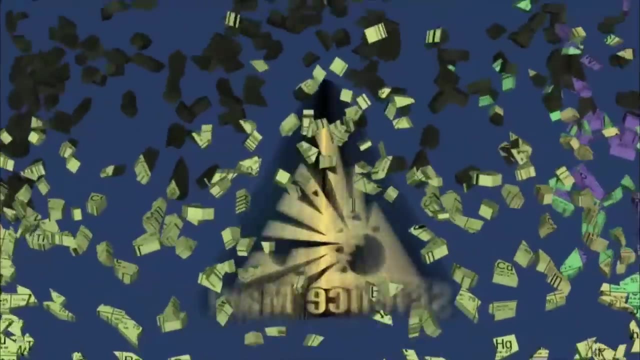 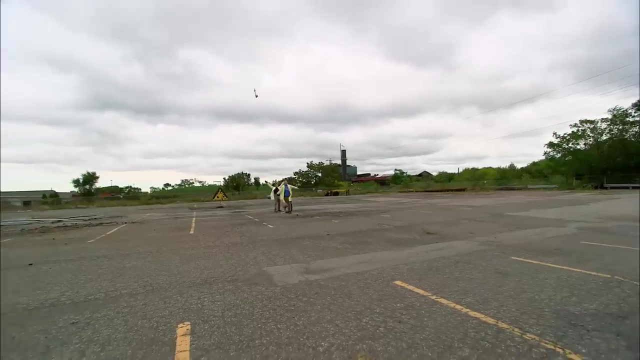 is keeping me sealed to the door. I'm completely suspended. Uh-oh, I shouldn't have done that. Whoa, Nope. So our larger version of the Stomp Rocket worked, but it didn't go as high as the first version. 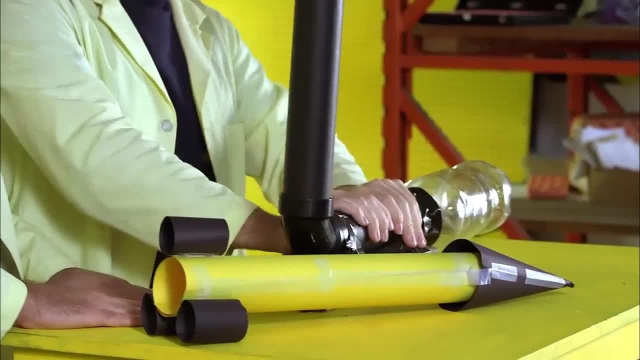 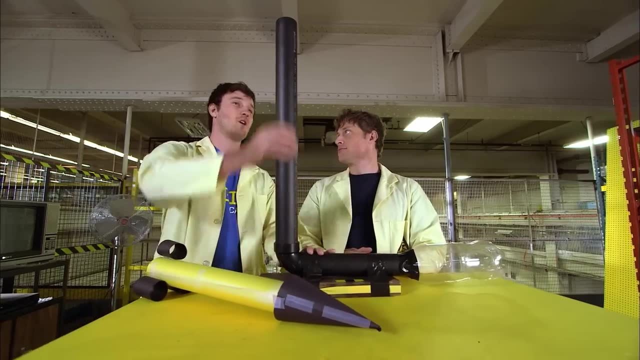 Chris and I see how we can improve the design. The larger pipe and the larger rocket works really well. It does work really well. I am afraid, though, that the larger pipe means that the same amount of air is flowing slower out the nozzle than it did before. 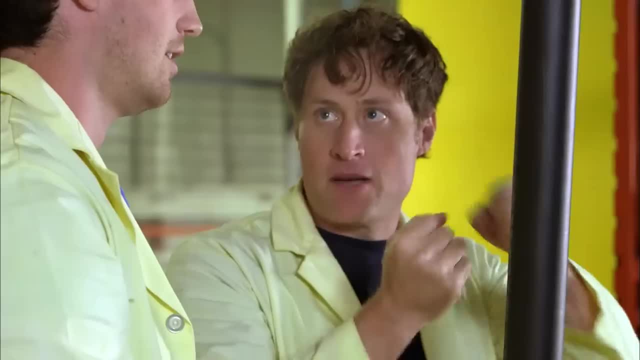 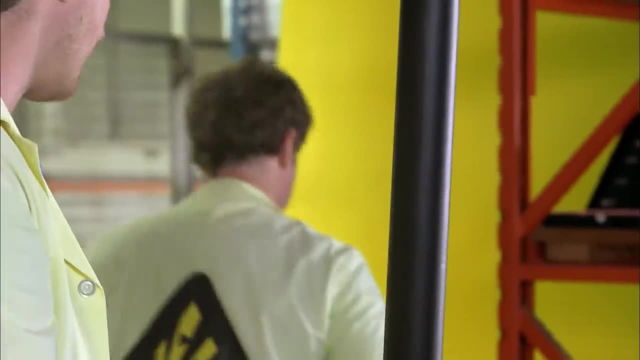 Oh, so because we're moving only this much air, it's not going to go as fast because this is a bigger tube. We need a bigger volume over here to match our larger. So a bigger bottle, That's right. I got a bigger bottle right here. 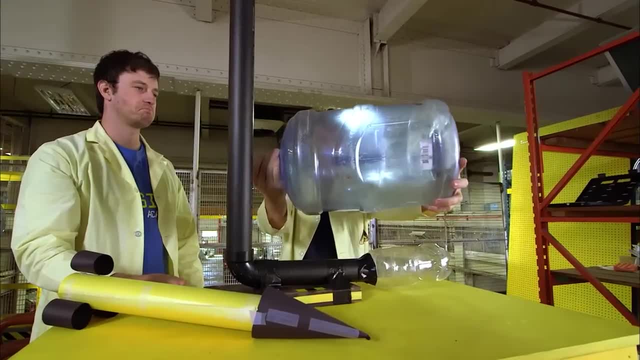 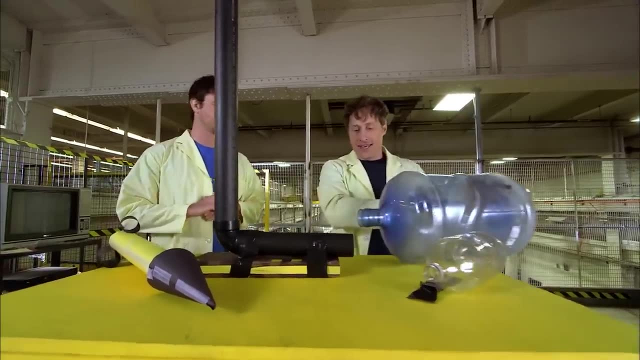 Ha-ha, Bigger bottle. So hold that, and then all we have to do is tape the bigger bottle on. I'm not sure if that's going to, Yeah, like this. Still, though, I'm afraid Yeah, so then all I need to do is tape it on. 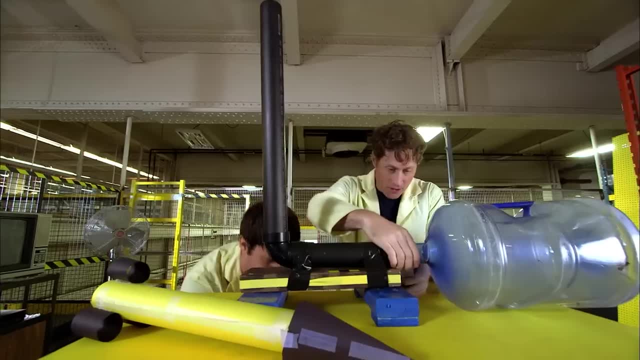 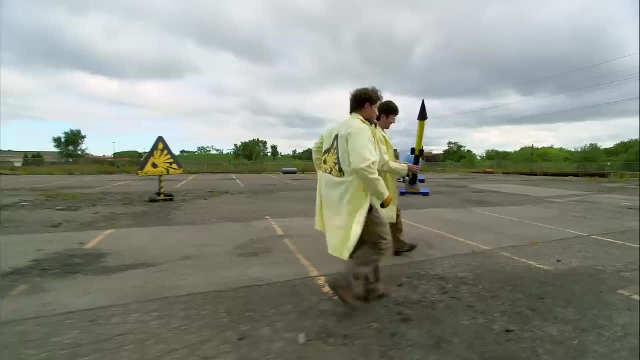 Chris and I attach a larger bottle to our tube. We just need some risers to adjust the height. then we tape it on and we're good to go. Everything else, including the rocket, stays the same. I still don't understand how you're going to step on this one. 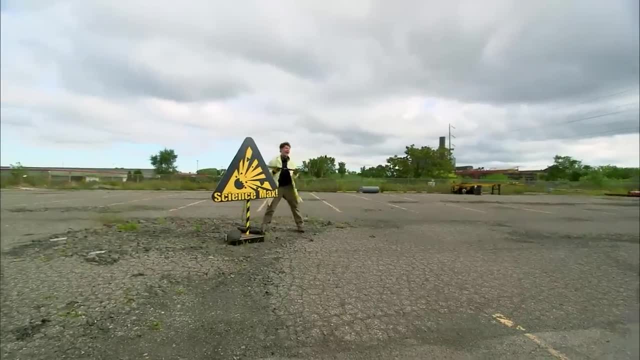 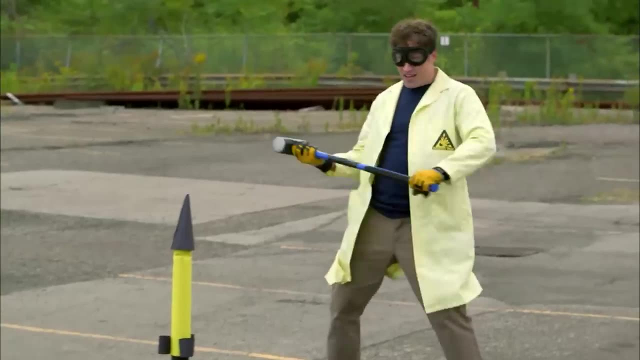 It's just too stiff. I have a plan. Ah, Sledgehammer, You ready? Yeah, I'm ready. Okay, One, two, three. It blew the top off the rocket, Right off the top. It also blew the bottom. 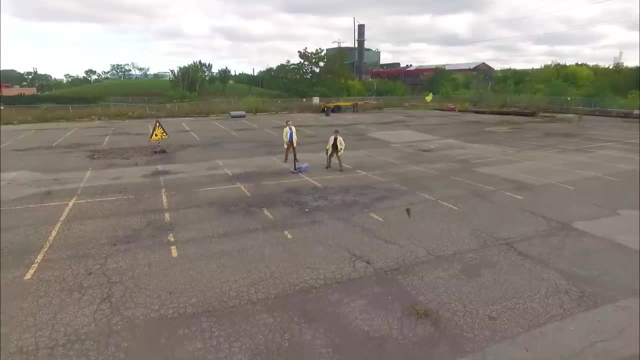 Looks like it's a bit rigid to change its volume so quickly, So it's kind of a one-time-use thing. huh, I think so. So why don't we try increasing the volume? Even bigger tube, Yeah, Even bigger container. 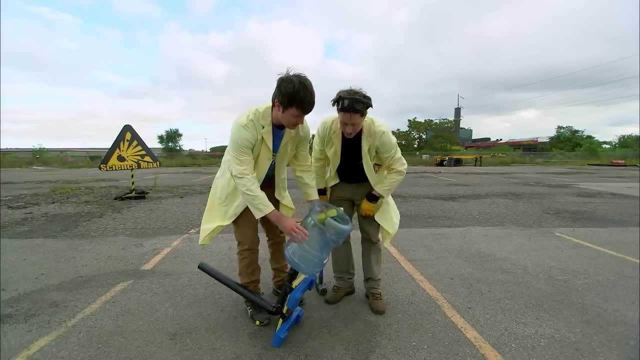 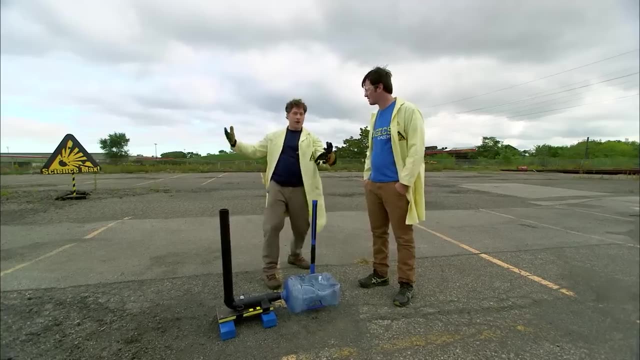 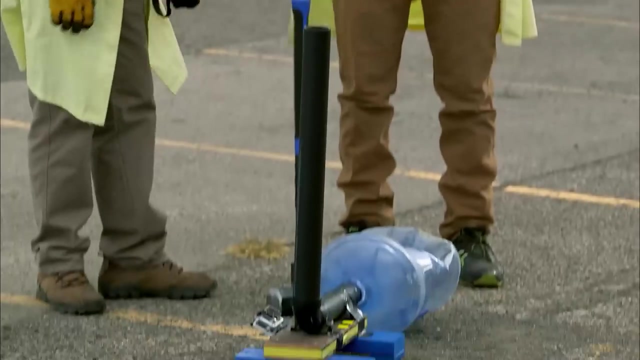 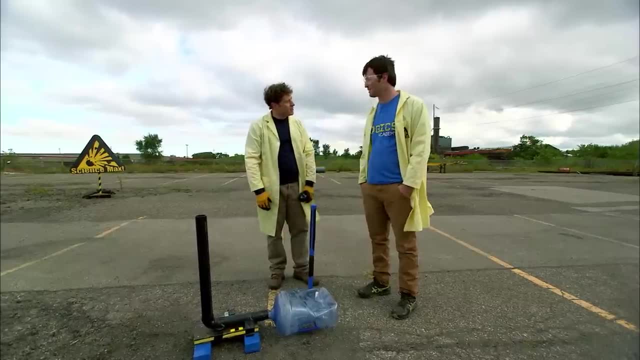 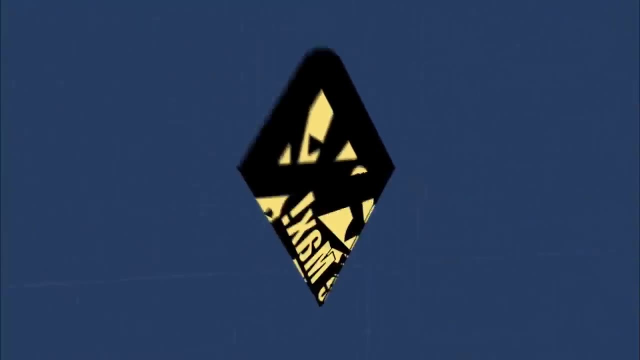 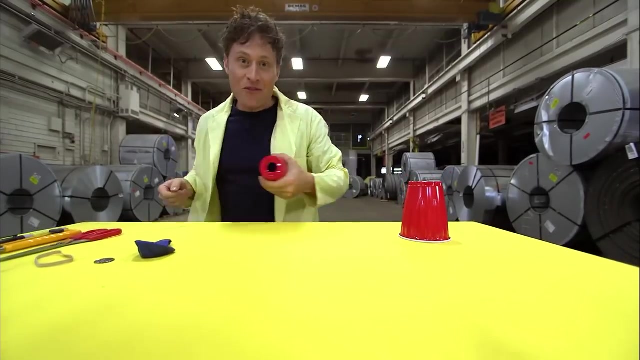 What about an air mattress? Do you think we could use an air mattress? I think we could. Yeah, A really big air mattress, Aw, Totally High five. Love that idea. Mini Max Moving air is a lot of fun, especially if you use one of these, a Vortex Cannon. 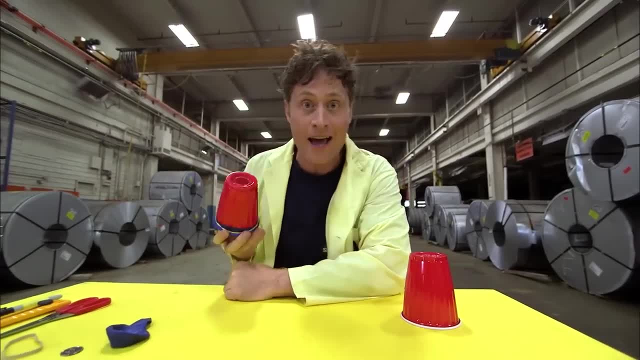 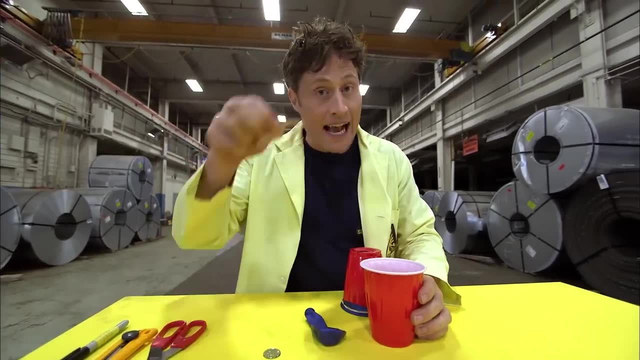 They're pretty impressive And they use some pretty amazing science. I'll show you how to build one. It's pretty simple. All you need is a plastic cup. You want a balloon, something round an elastic scissors or a craft knife and a pen. 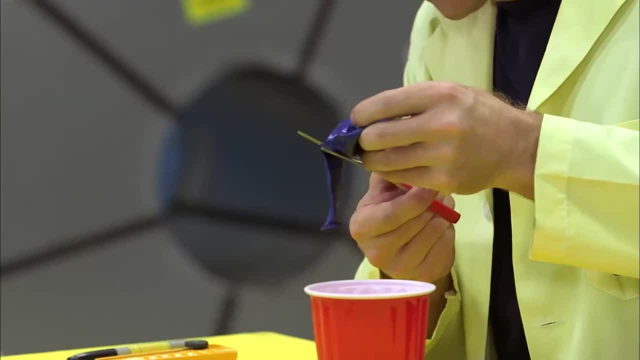 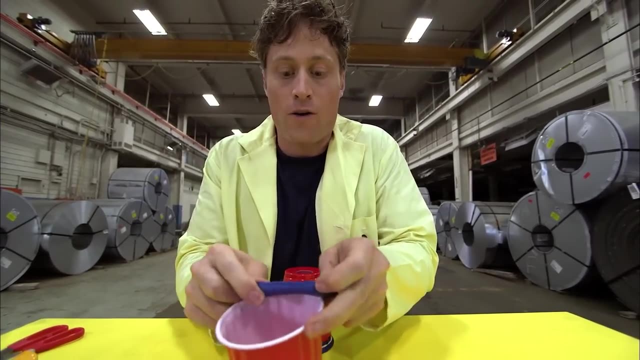 Here's what you do: Take your balloon and cut it just where it gets wide. You take the mouth of the cup right there and you have to stretch the balloon over the top, And then you want to put an elastic around it. keep it in place. 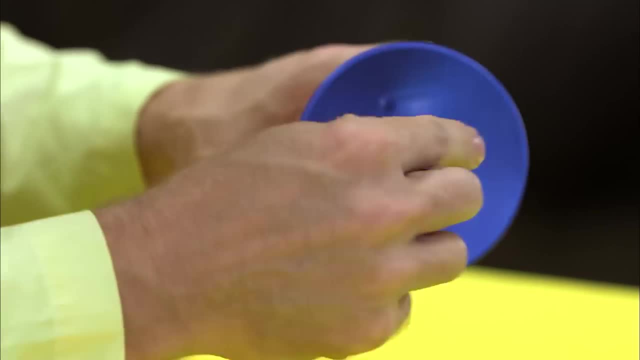 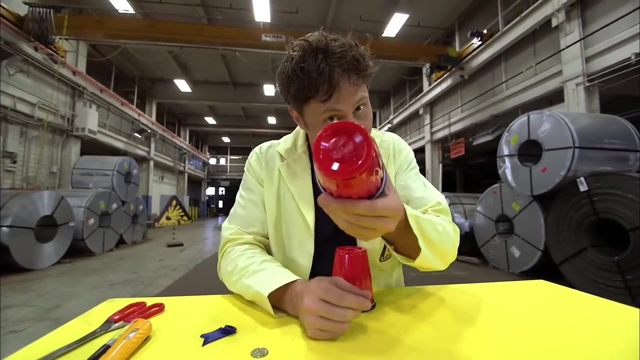 And this now is a surface on the top and that's what you're going to use to pull back and create your burst of air. But of course, the air's not going to go anywhere until you make a hole in the bottom. So here's what you do. 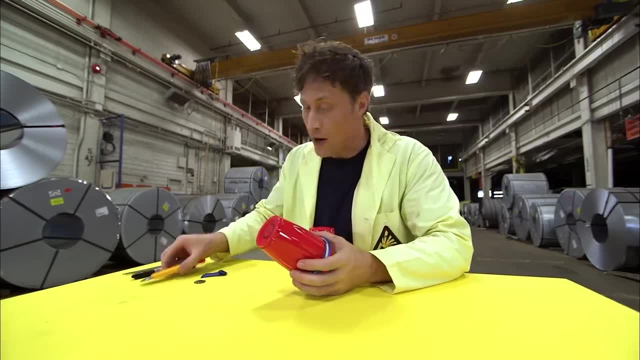 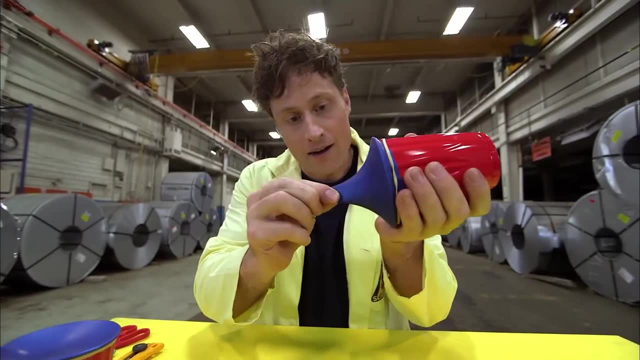 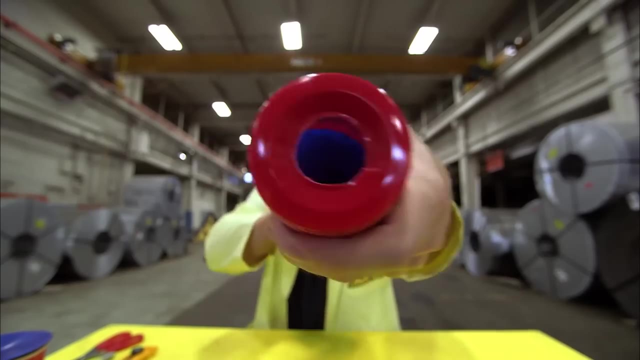 You take your round thing and draw a circle and take your craft knife or scissors and an adult and get them to help you cut out a hole And when you pull back on the balloon, A burst of air, A burst of air comes through the hole. but the air has an interesting shape. 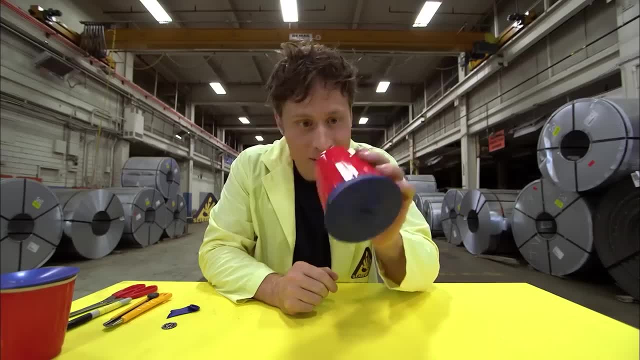 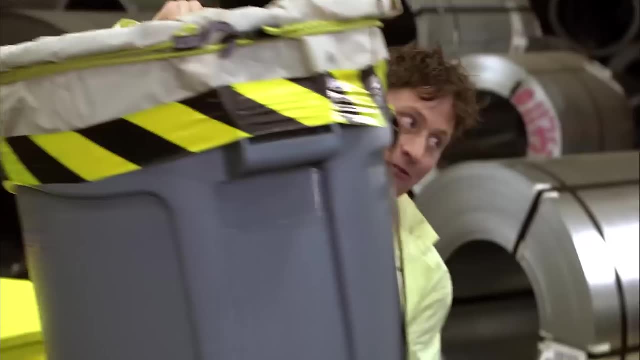 Now I know what you're thinking. You're thinking, Phil, air is invisible. You can't tell what shape it is. Well, I can show you. Come on, This is my maxed out vortex cannon. It's made out of a garbage can. 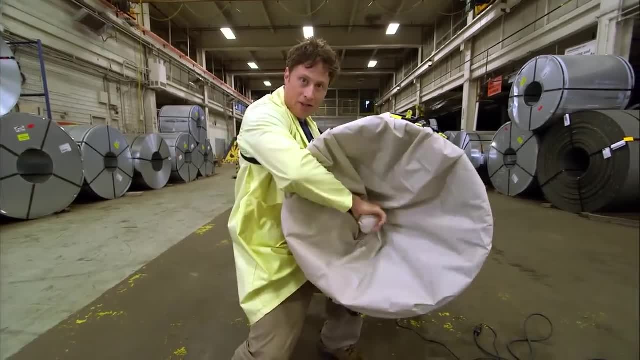 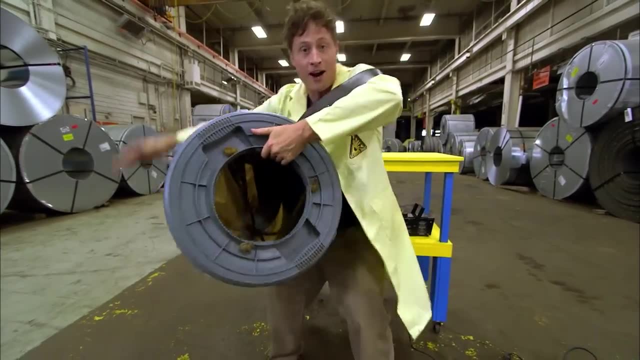 I've got a hole in here and this is a shower curtain with a ball that I can get a grip on and pull, And then it shoots forward like this. Now it makes a big puff of air, But again the air is invisible. 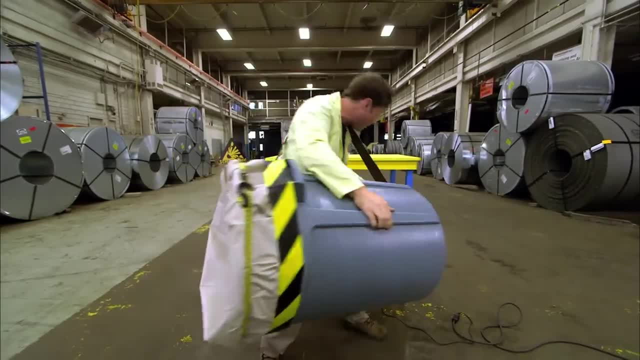 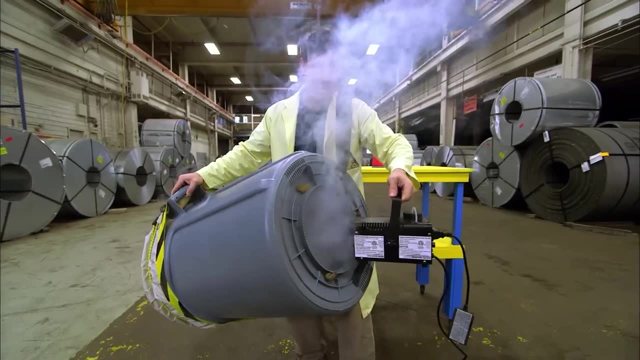 So we don't know what shape it is. But I can help with that because I've got this, a fog machine. I fill the inside of the garbage can so we can see what the air is doing when I fire the vortex cannon. Okay, come on over here. 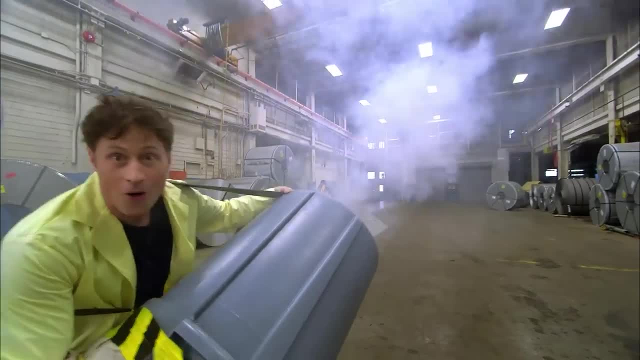 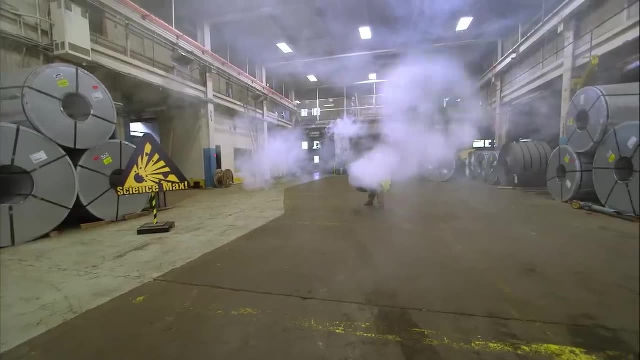 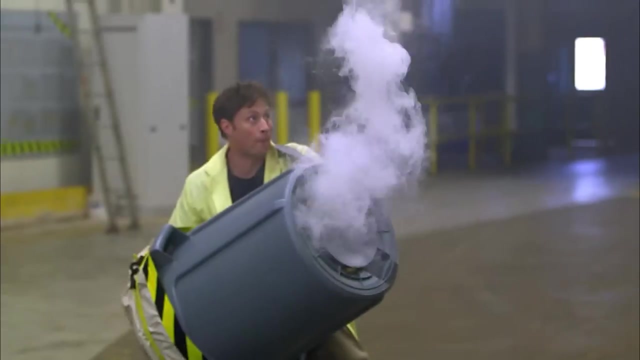 Ready, Whoa, Okay, ready, Check it out. The vortex cannon shapes the air into a ring called a vortex. It makes a ring Well, actually sort of a donut. Because of its shape, the air in a vortex can move much farther than air that doesn't. 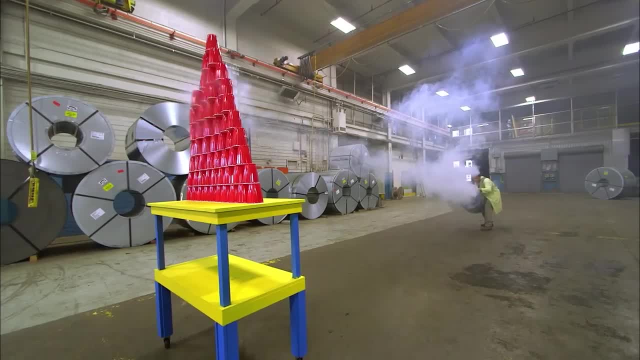 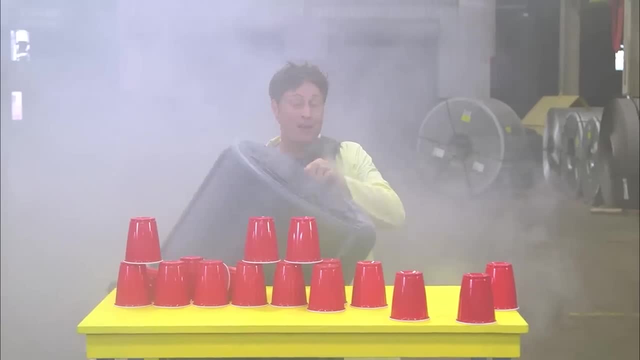 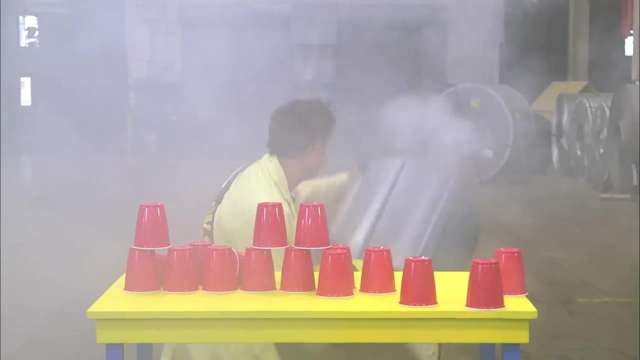 have a shape. Vortex cannon Air that has a shape goes a lot further than air that doesn't have a shape, And it's also way more fun. Woo-hoo, A little to the left, A little to the left: Remote it. 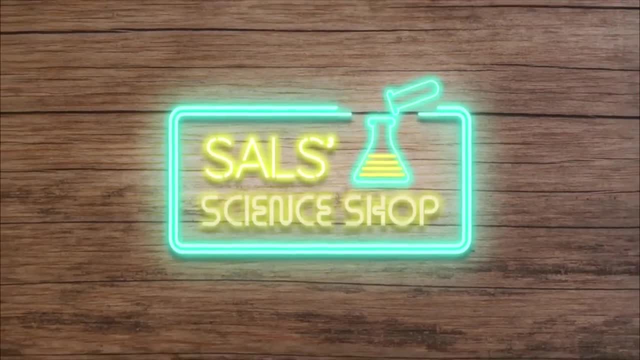 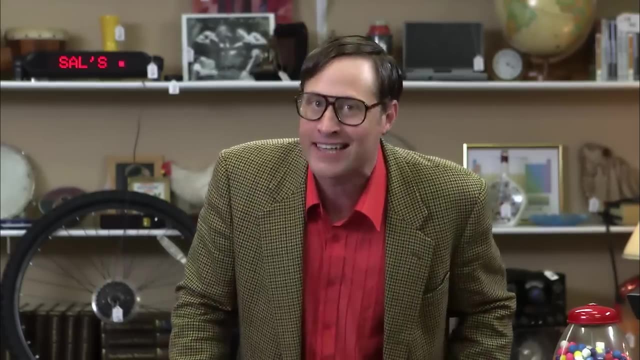 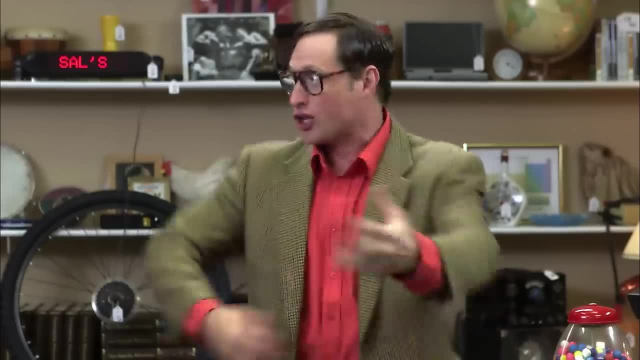 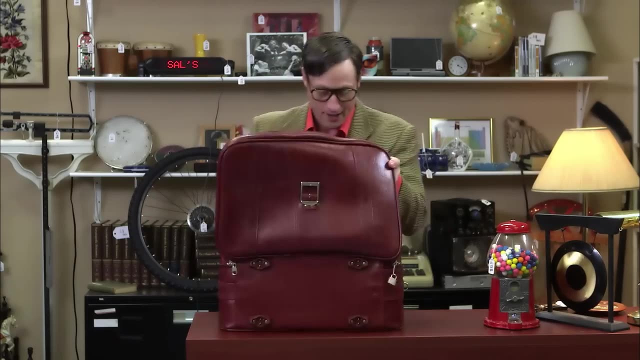 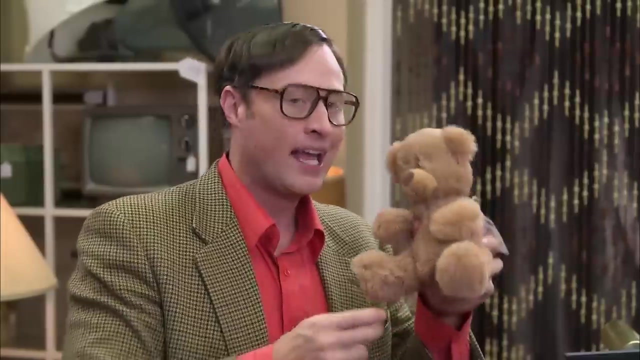 Well, if you haven't decided where, may I suggest underwater? But don't forget to pack the most important thing when you go: Hat Nah, Ukulele Nah, forget about it. Chicken, No Sunscreen, Forget about it. 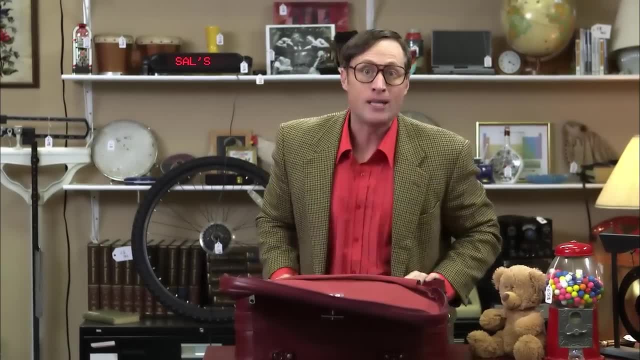 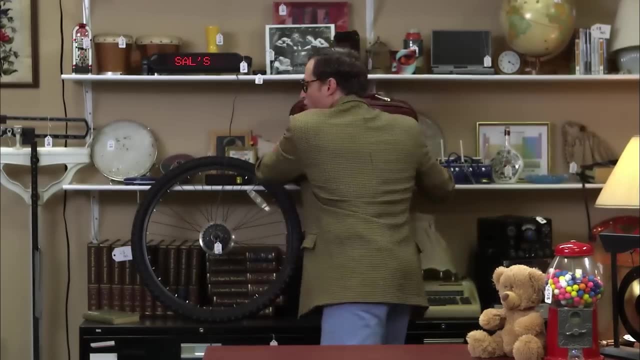 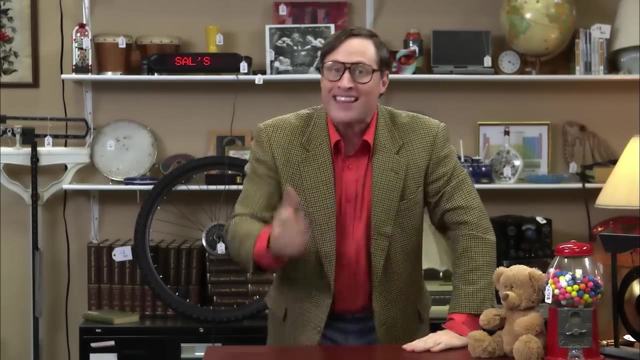 Teddy. No, If you're going underwater, the most important thing you've got to pack is air. Okay, All right, You know, you see, human beings have been coming up with ways to go underwater for a long time. but the thing is you've got to bring air with you because you know breathing. 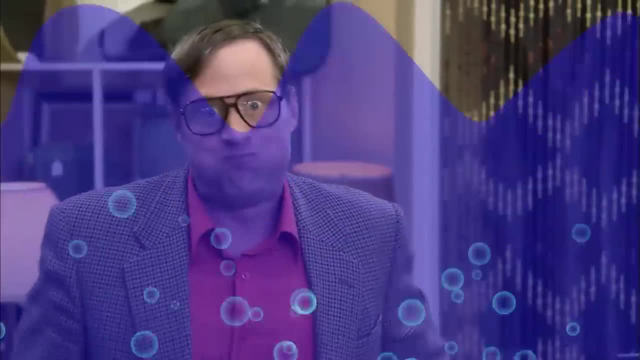 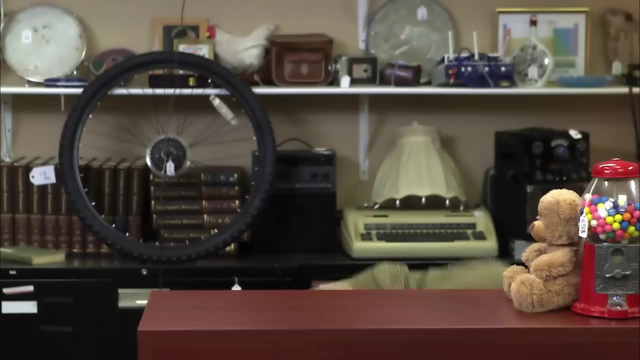 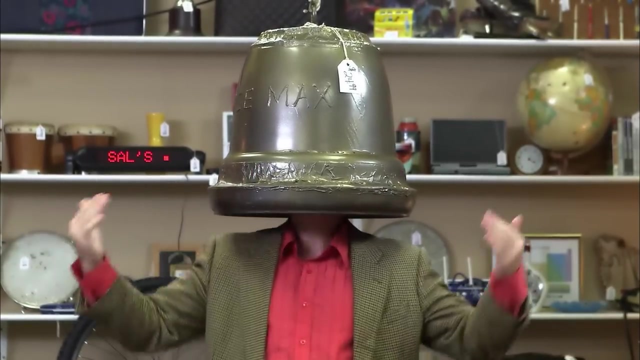 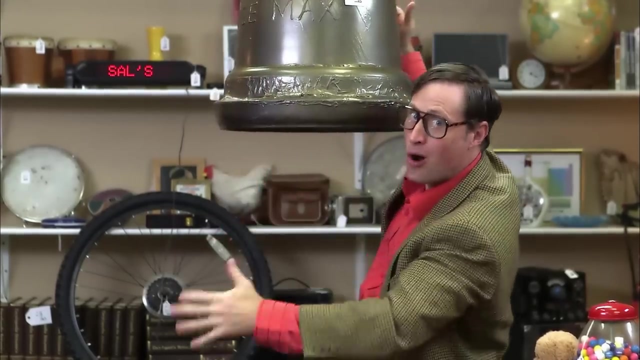 is is good. Check this out. It's a diving belt. One of the first ways human beings could actually dive used to be able to take air with them when they went underwater. you see, it's a big, heavy bell and it's lowered from a ship above on a rope and when it gets lowered into the water it traps a. 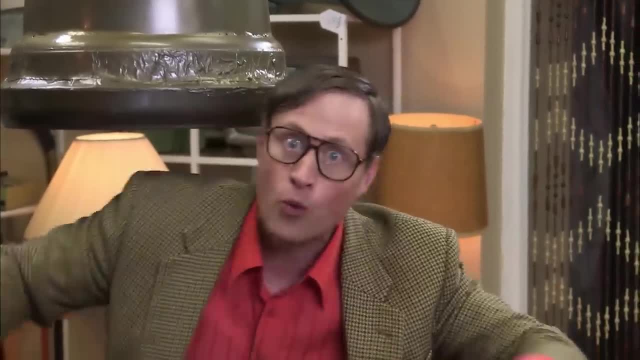 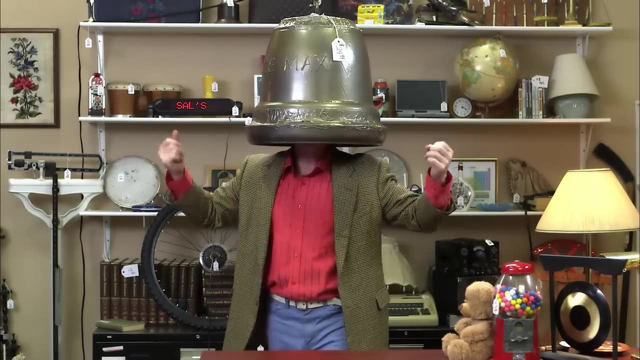 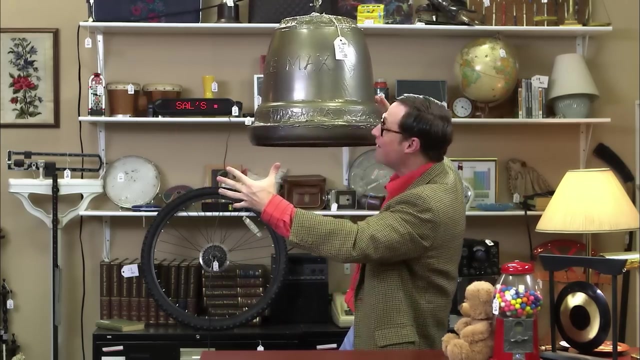 bubble of air underneath so you can swim around underwater. but then when you need to breathe again, you don't have to go all the way back up, you just pop under the bell and take another breath. bells like this were actually much bigger when they used to use them for diving. 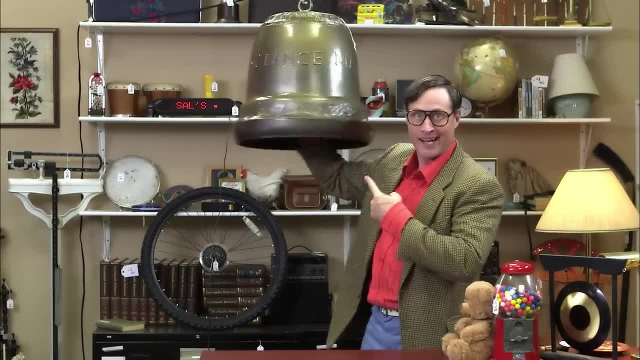 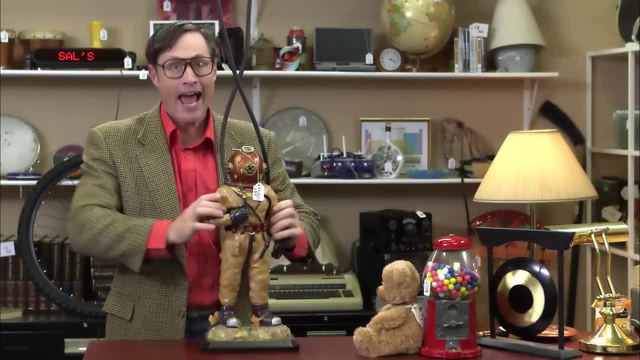 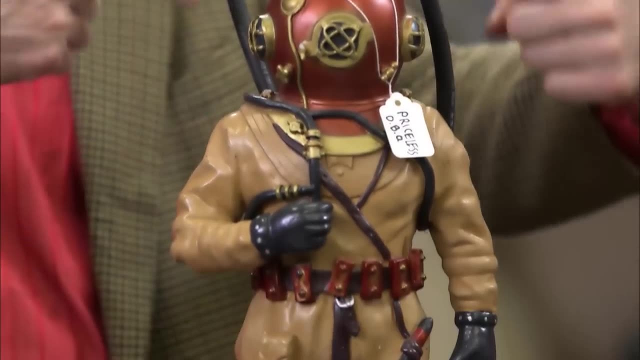 to hold more air. huh, ring-a-ding-ding, what do you think you want this? no, it's okay, i got something else. hold on, check this out. it's an old-timey diving suit. air is pumped in through these hoses here, which means the diver has a constant supply of air, which means he can stay underwater longer. 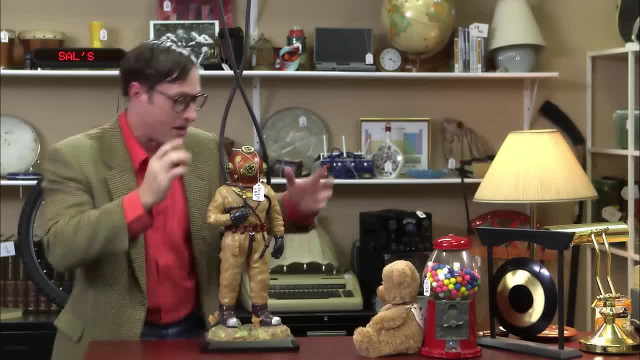 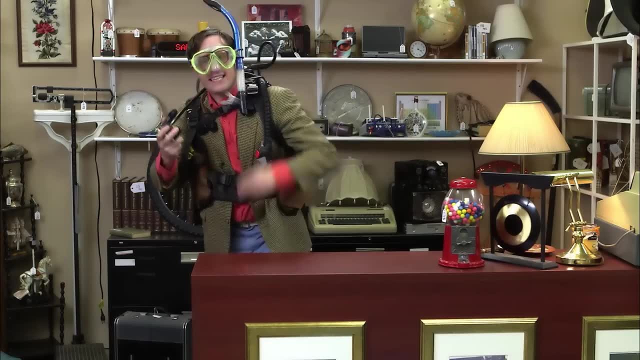 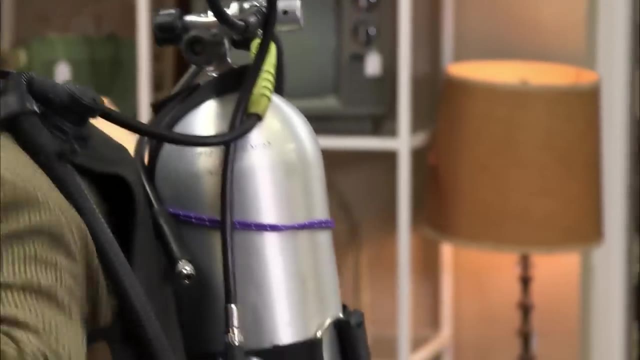 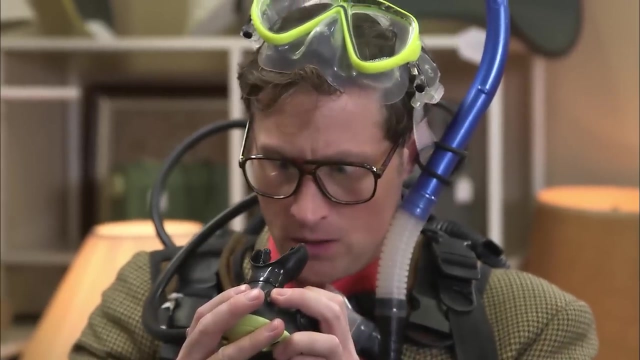 what do you think? like: no, okay, hold on, i got something else. i got something else. um, yeah, this is it, the ultimate: bringing air with you, the scuba suit. this tank holds compressed air, which means it can carry a lot of air with you, which means you can stay underwater for longer. so i'll tell you what. 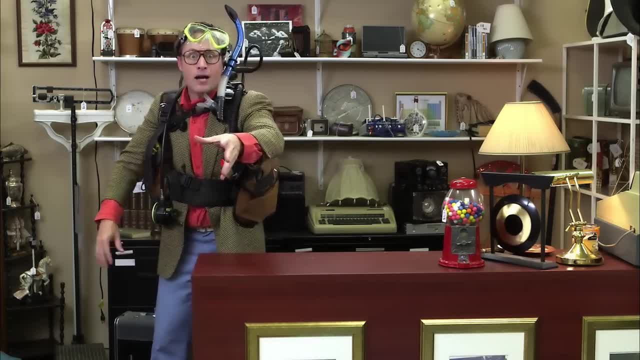 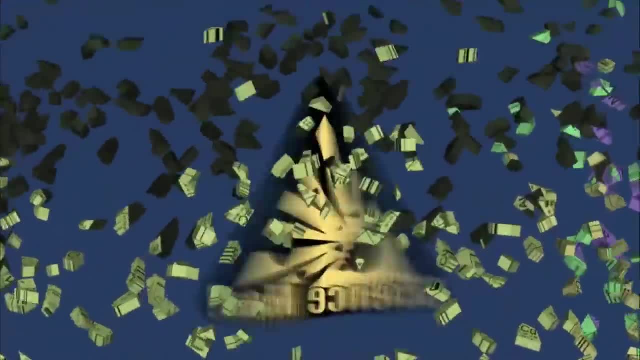 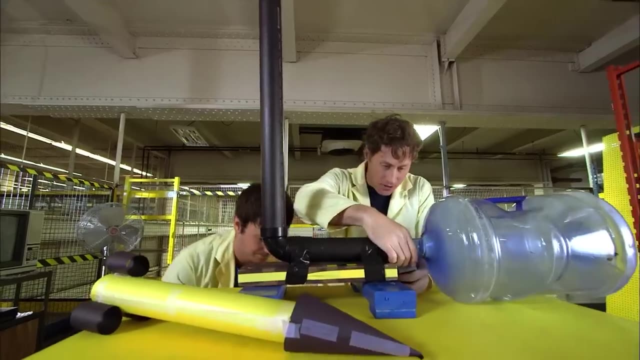 i'll wrap up all three things. what do you say? yeah, you'll take them. okay, great, let me just wrap them up for you. come on, teddy, let's go find the bag. so our large stop rocket hasn't worked perfectly, but our larger bottle was too rigid to stomp and when i used a sledgehammer it was so sudden. the 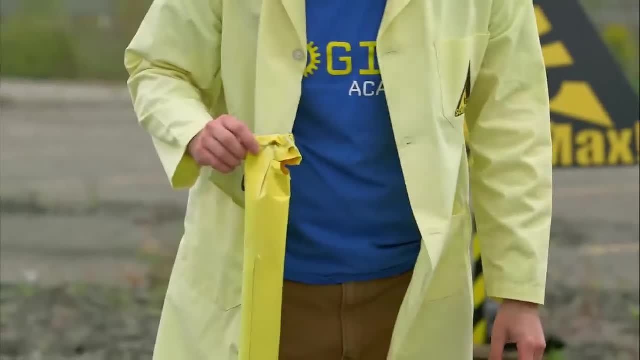 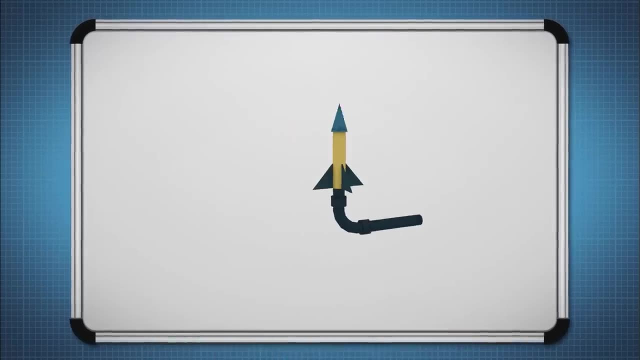 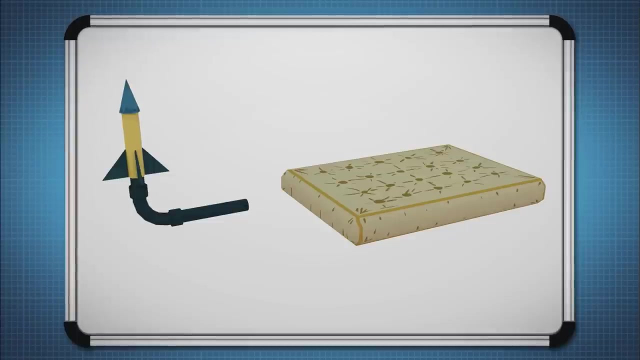 bottle broke and also it blew apart the rocket chris, and i need a large container of air that is soft enough to change its shape easily. so here's the current plan: an even larger pipe, an even larger rocket, and we use an air mattress. we make two holes in the air mattress, one to fill. 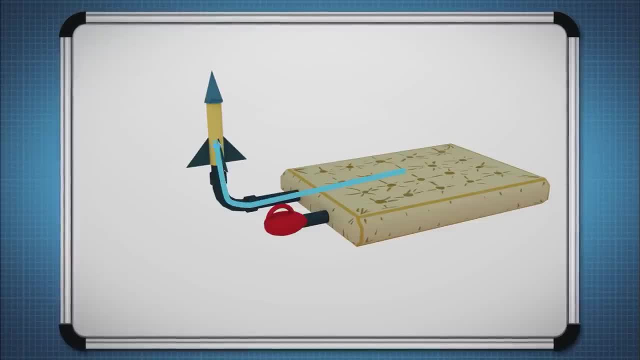 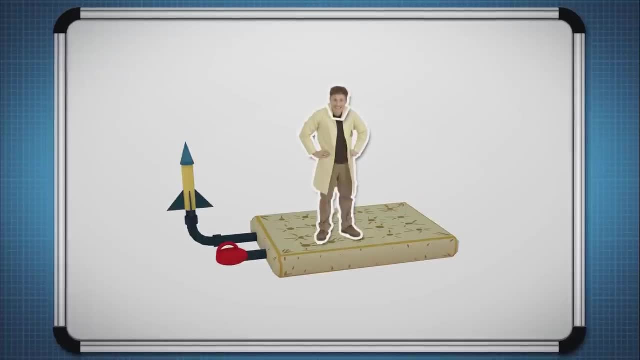 it up with a leaf blower and the other hole to go out the tube to the rocket. since an air mattress holds lots of air and is very easy to change the shape by jumping on it, we figure it'll be a great way to get lots of air through the tube to launch our rocket. okay, let's do it. let's do it. 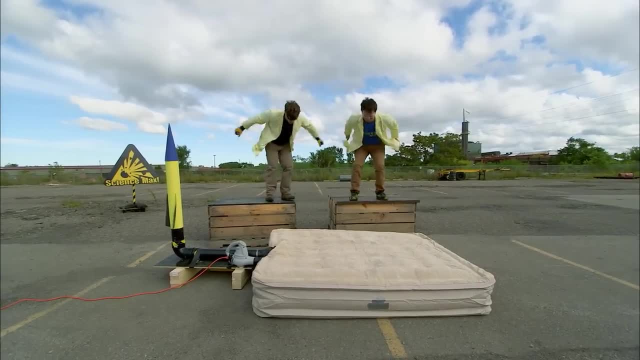 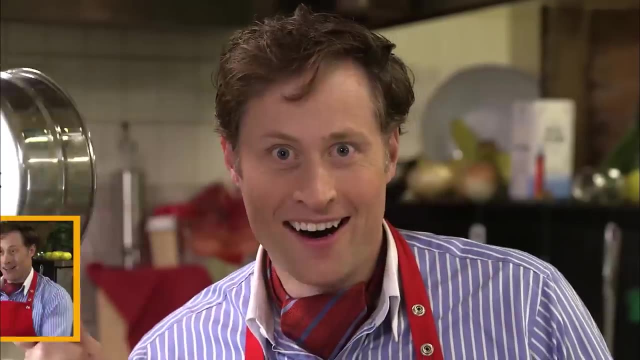 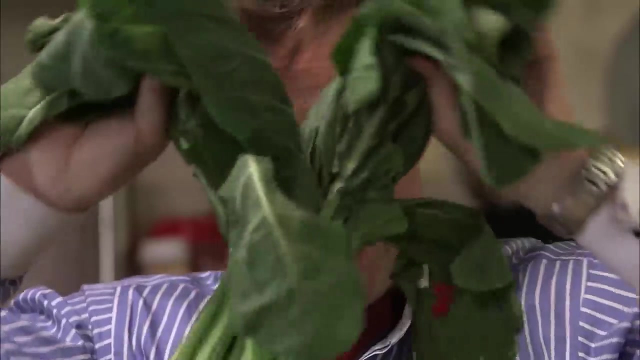 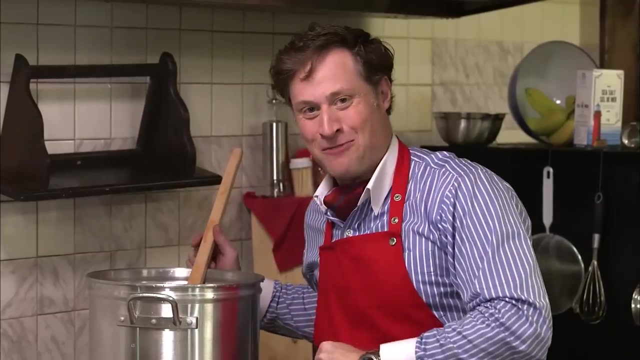 all right, we're gonna go one, two, three, jump right. yeah, one, two, three. being a chef is my absolute passion and cooking up science recipes is my speciality. i'm buster bika and this is the rocket rocket show. this is cooking with science. oh, hello, welcome to cooking with science. i'm buster bika whenever. 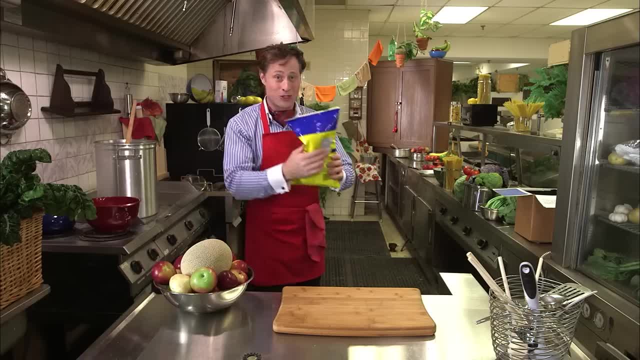 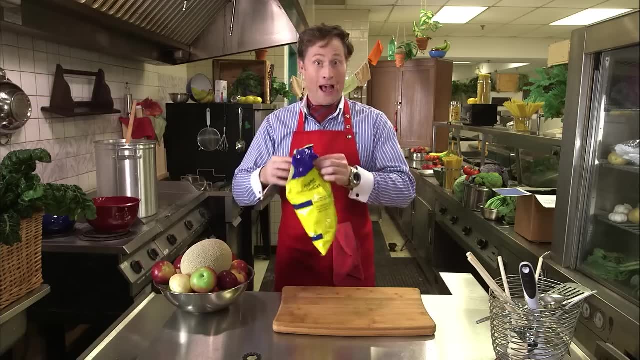 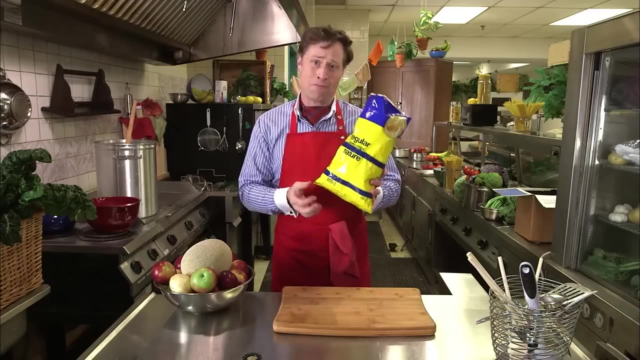 friends come over. i like to make my famous potato chip recipe. and look at this bag of potato chips quite large. there must be a lot of potato chips in here, right? well, let's open it. what this potato chip bag is? mostly air. why do potato chip bags have so much air? well, to tell you the 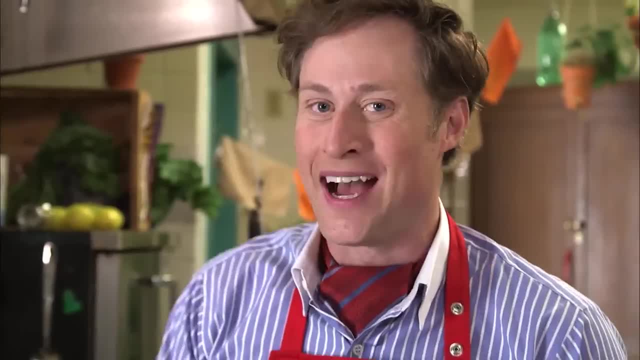 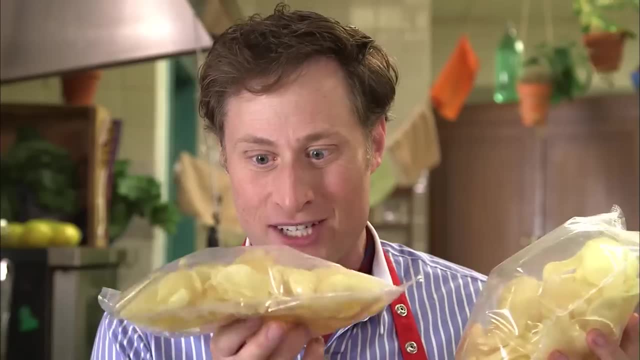 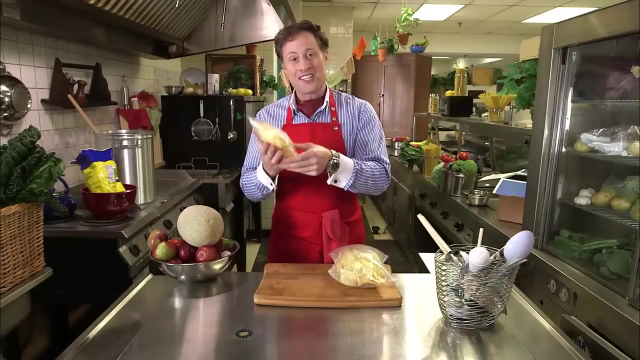 answer to that, i have to tell you the story of two bags of potato chips. here they are: this one full of air, and this bag of potato chips there's not much air in it at all. why don't they make them like this? well, let's find out. the first thing that happens is the. 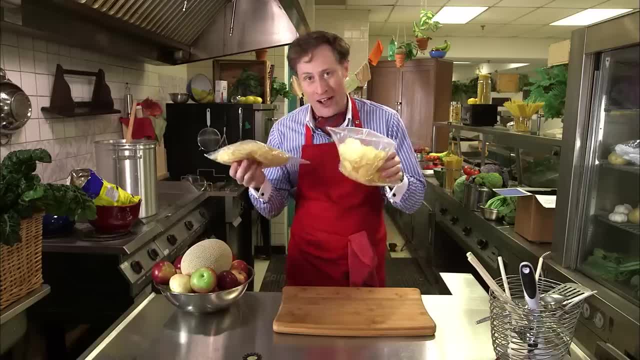 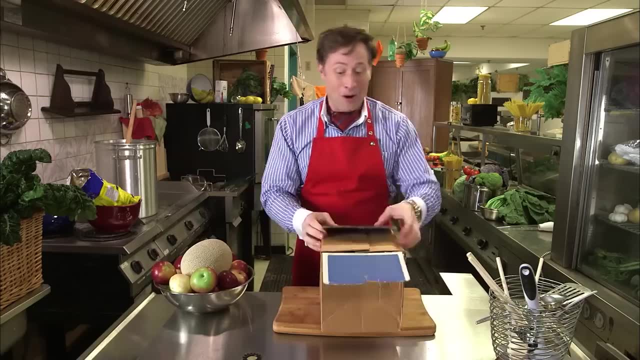 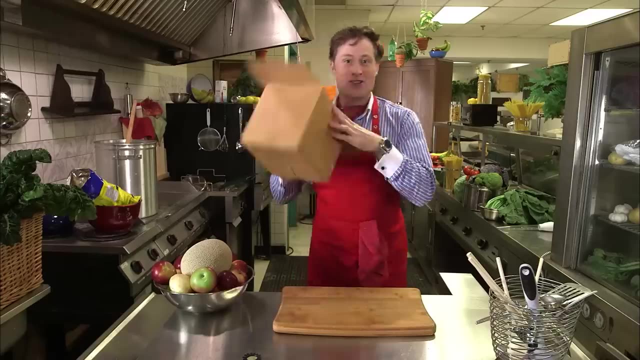 potato chip bags come off the conveyor belt at the potato chip factory, where they get packed into a crate- here's a crate here, so let's really stuff them in- and then the crate gets boxed down up and shipped off to the store. oh, it's a bumpy ride to the store today. now we're at the store. 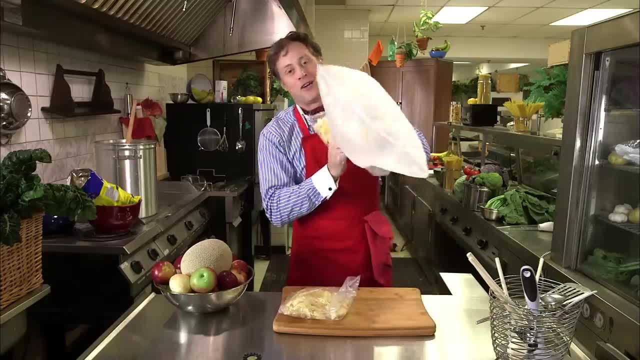 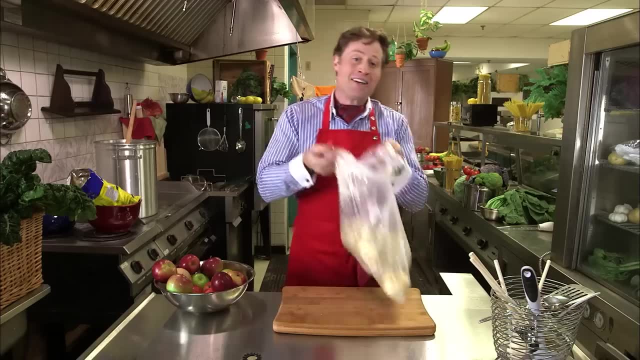 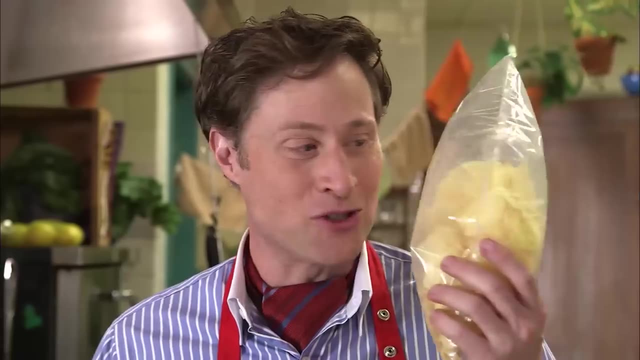 and then you come along: ah, bags of potato chips. what else should i buy today? oh, i know how. about a cantaloupe, very nice. some apples, yes, and take it home. walk along and you get to the kitchen. you have a choice: this bag of potato chips, where all the potato chips are light and fluffy, or this bag. 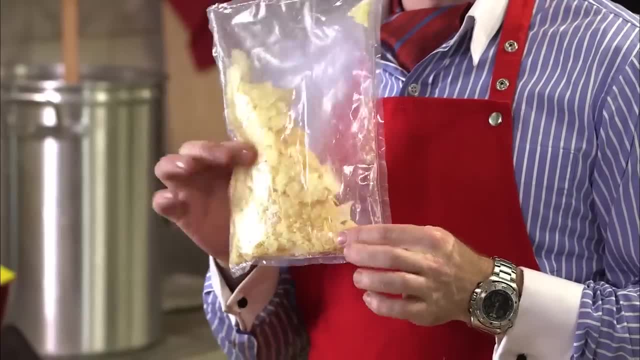 of potato chips are all potato chips that are light and fluffy. all the potato chips are light and fluffy potato chips, which is not exciting at all, And that's why potato chip bags have so much air to protect the potato chips from getting crushed. 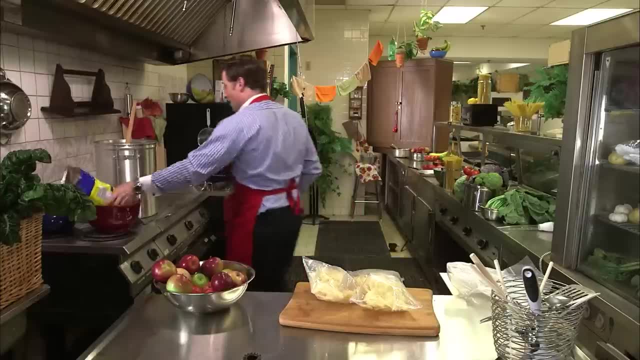 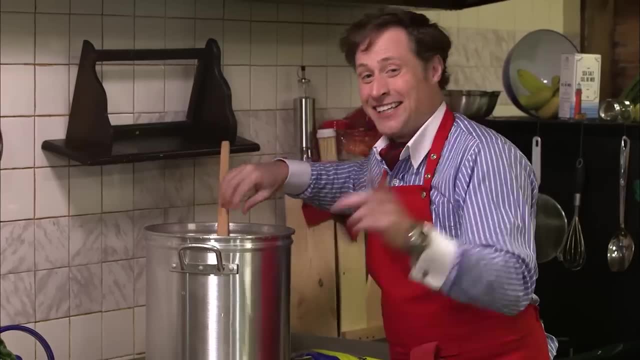 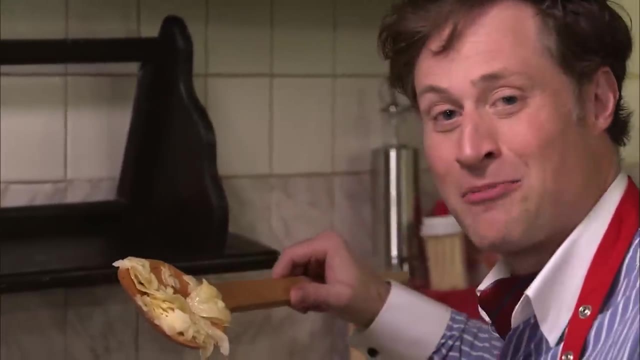 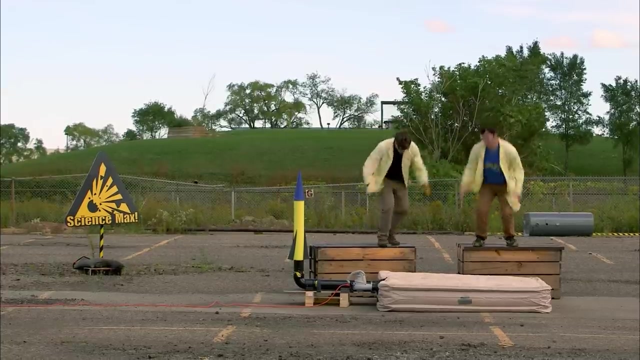 Speaking of potato chips, time to get back to my recipe. What is it? It's potato chip soup. Well, I'm Master Beaker, and thanks for joining me on Cooking with Science. Perhaps a little bit more cooking, Okay. so where were we? 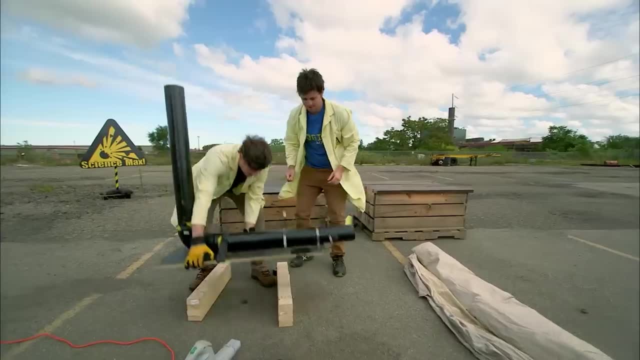 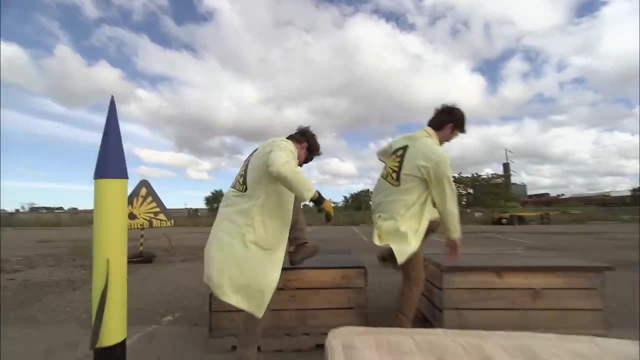 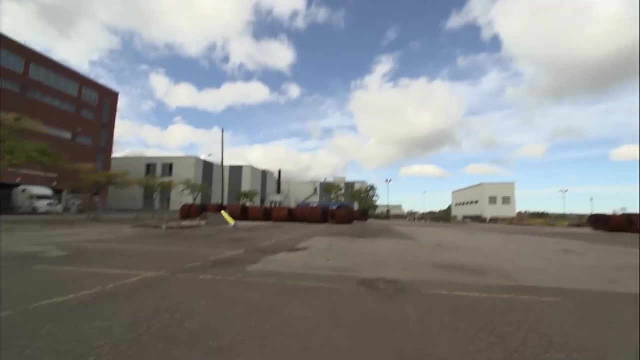 Oh right, our maxed out rocket: A much larger pipe, a large air mattress and the largest rocket yet. Let's see how it goes: One, two, three jump. One, two, three. Yeah, there you go. 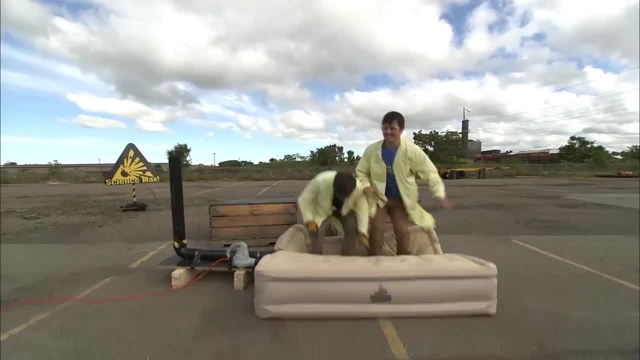 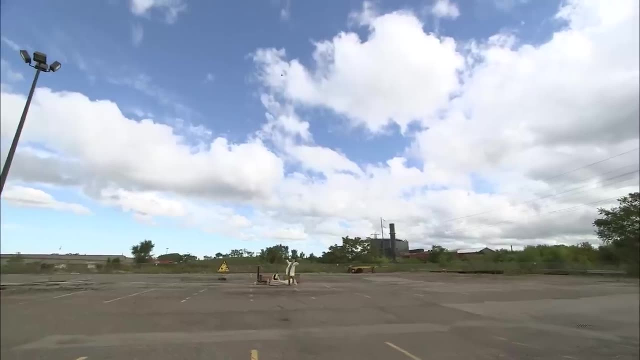 All right, let's do it again. One, two, three. It works amazingly well. The large volume of air Chris and I can move by, both jumping on the air mattress- gets transferred through the large pipe, and even though it's a giant rocket. 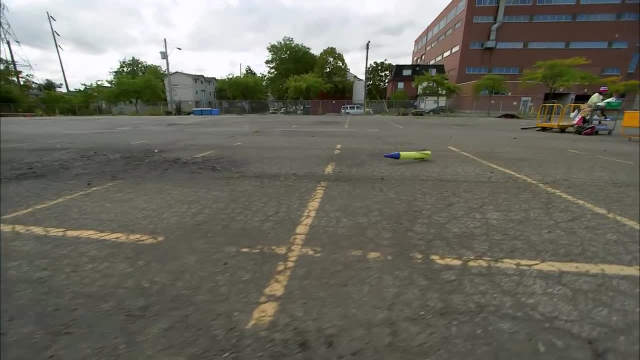 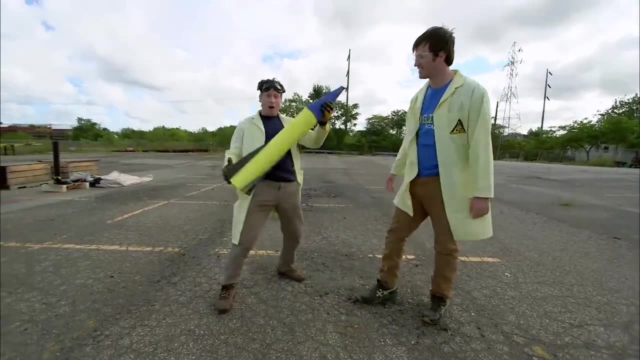 it sails higher than any other version. That was great, That was amazing. All right, There you go. Science Max: experiments at large, moving a lot of air. That has to be the biggest stomp rocket ever. Biggest stomp rocket ever. 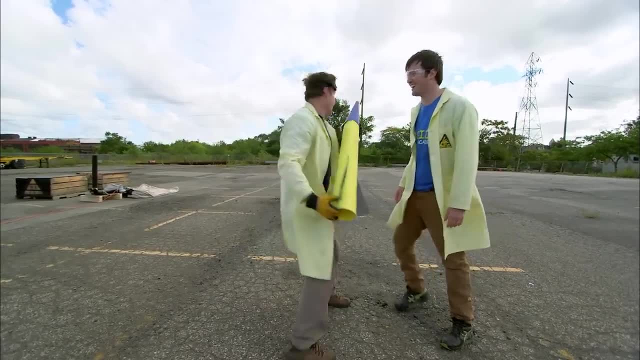 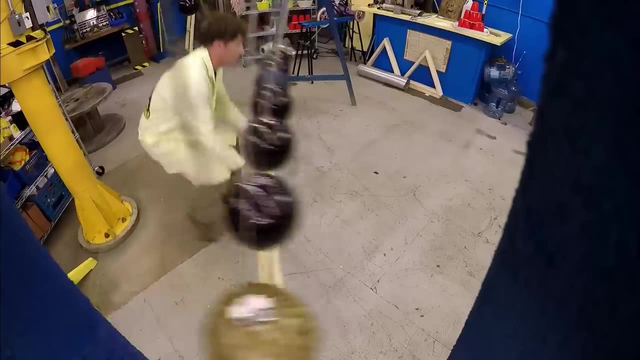 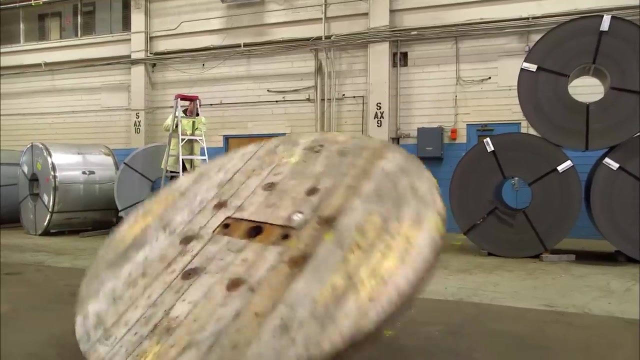 Let's do it again, Okay, Okay. Science Max. This episode of Science Max is all about vibration and frequency. Frequency and vibration: What's the difference? We build a maxed out vibrobot, spin a giant disk, suspend water and play with lasers. 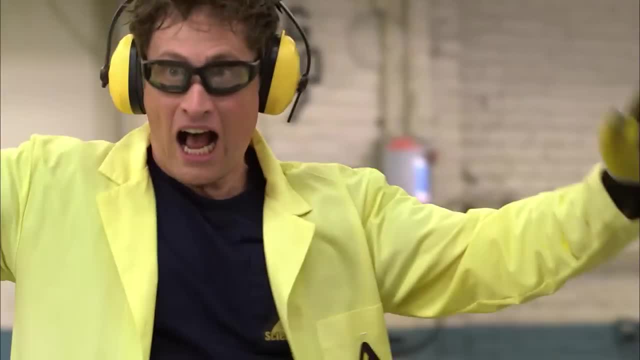 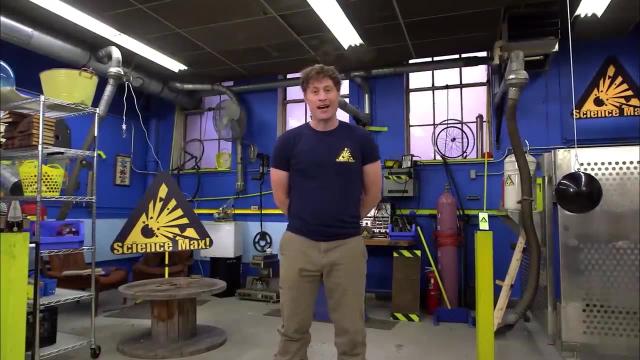 All on this episode of Science Max experiments at large. Greetings, Science Maximites and welcome to Science Max experiments at large. My name is Phil and I'm your host, Chris And I'm your host Chris, And today on Science Max experiments at large. 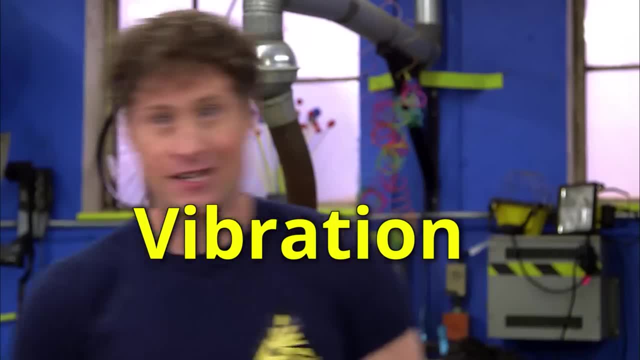 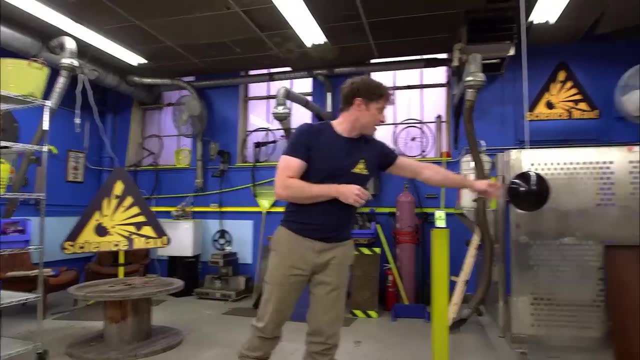 we're going to be looking at vibration. Vibration is when things go back and forth, back and forth and back and forth. All kinds of things vibrate, like pendulums, Pendulums, Wait, wait And pendulums. 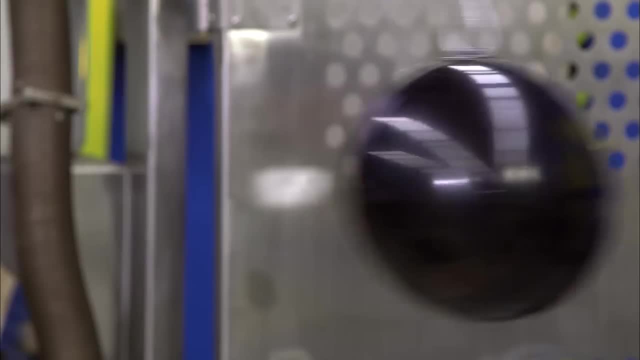 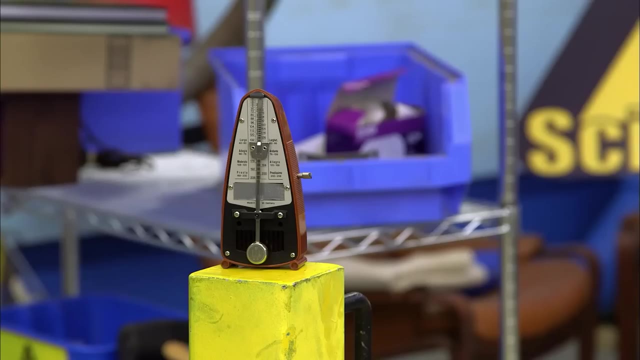 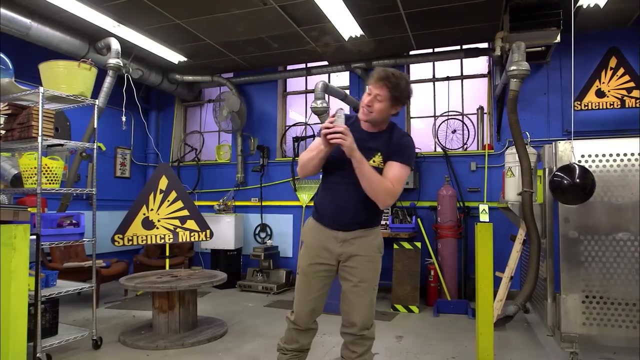 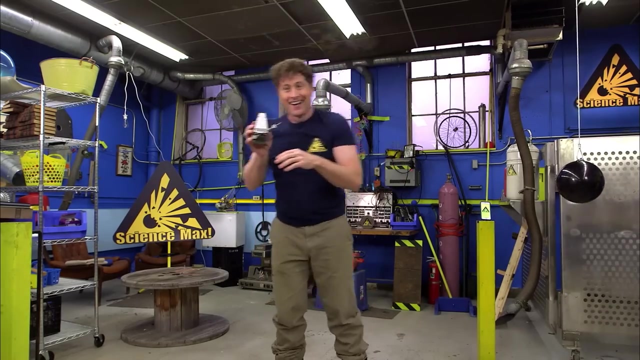 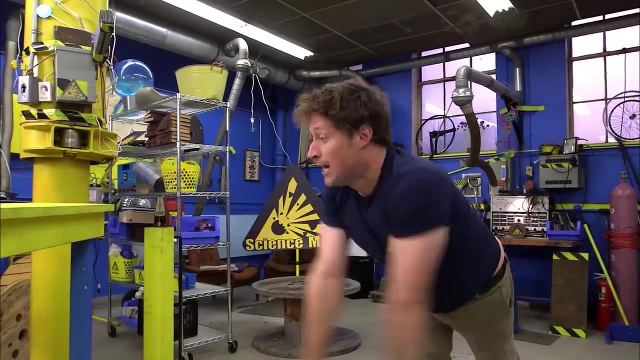 Pendulums are designed to swing back and forth. Stop that. Also, metronomes: Oh, Metronomes are used by people when they're practicing music to keep accurate time. Yeah, OK, Putting it back And we're going to be building. 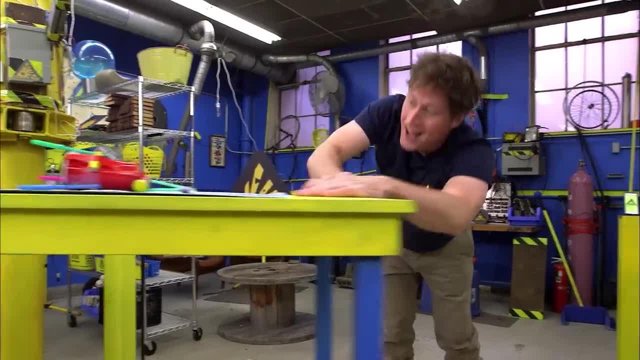 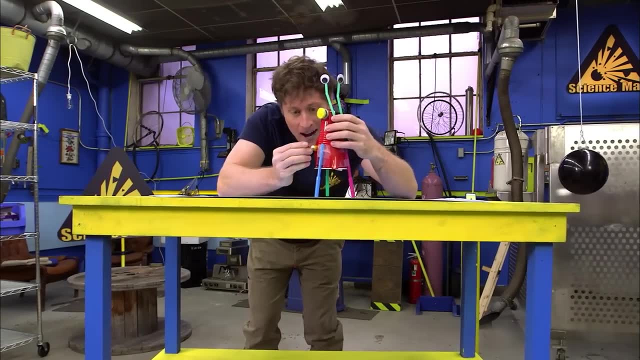 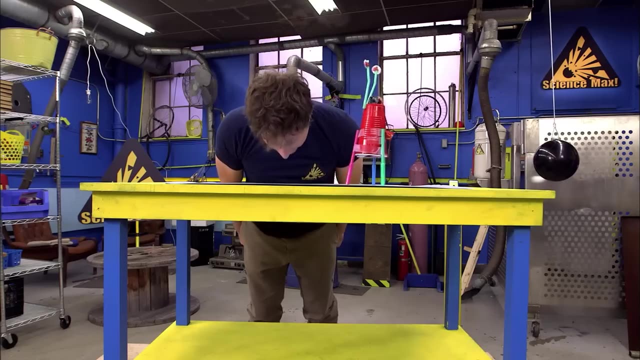 OK, We're going to be building this little guy. This is a vibrobot And he vibrates and he skitters around on the paper And if we take the caps off the markers, he makes interesting patterns on the paper. OK, 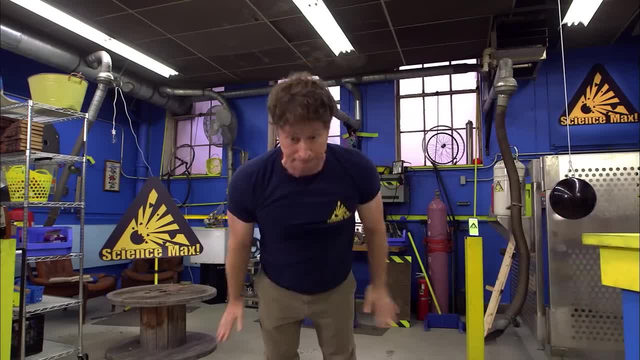 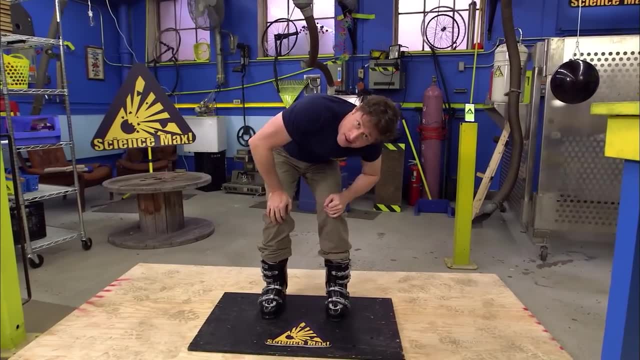 So let's get started. Let's build a vibrobot. Oh yeah, You know what? Maybe it's time to take off the ski boots. huh Whew, There we go. That's better. So today, like I said, 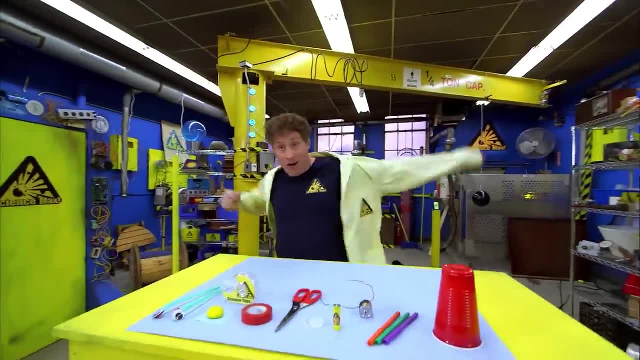 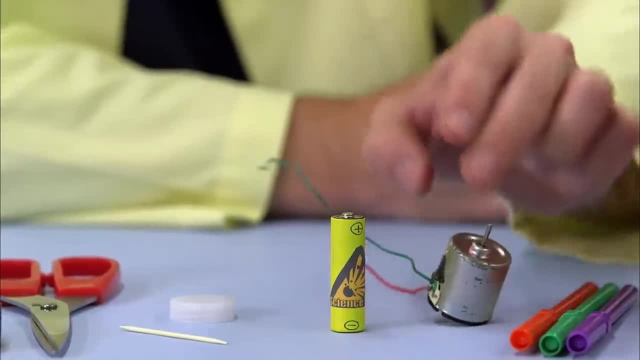 We're going to be making a vibrobot, And here are all the materials you need to make your own Plastic cup, three markers, an electric motor- Just make sure you ask an adult first- A battery, a plastic drink bottle cap, a toothpick. 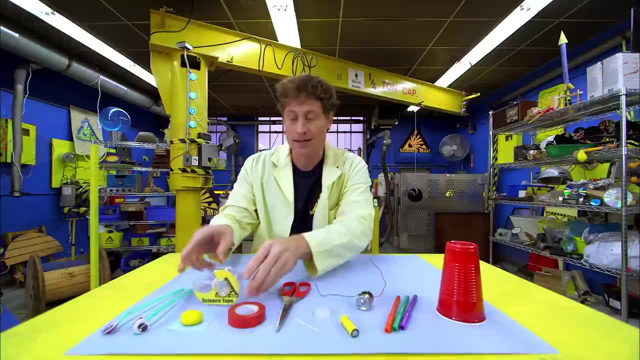 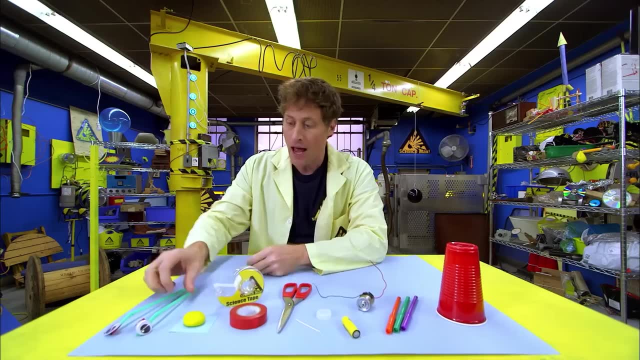 scissors. This kind of tape is called electrical tape, Science tape, which is the same as invisible tape, But of course I use this tape only for science And some modeling clay, And these are two bendy straws that I've taped googly eyes. 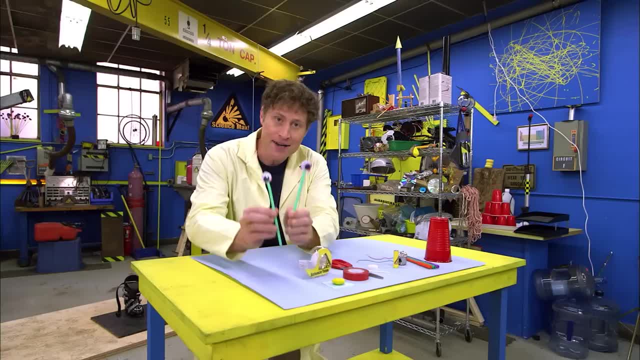 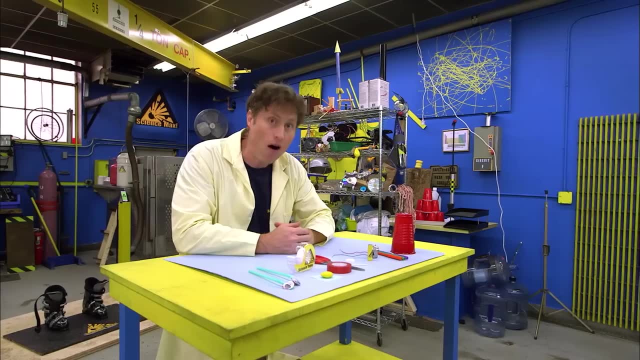 And I'm going to use this tape, And I'm going to use this tape to make these googly eyes too. These are not necessary, I just like them for decoration. Now remember, if I'm going too fast here, which I probably- 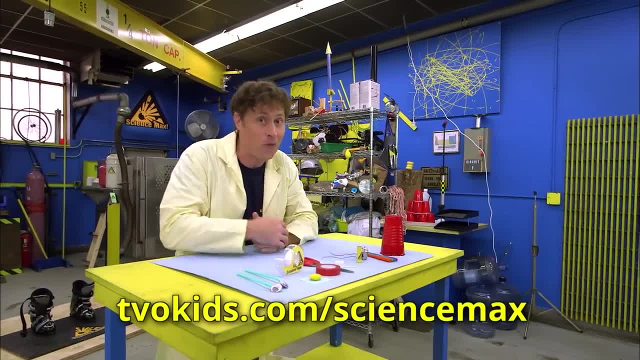 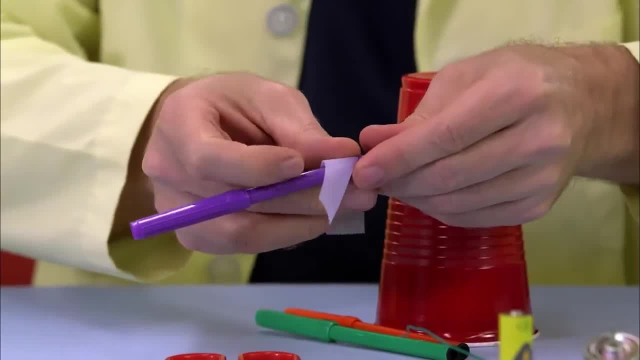 will be. you can get all of the steps on how to make your very own vibrobot on our website. OK, So here's how you get started. First, you're going to make the feet for your vibrobot, So I attach some science tape to the markers. 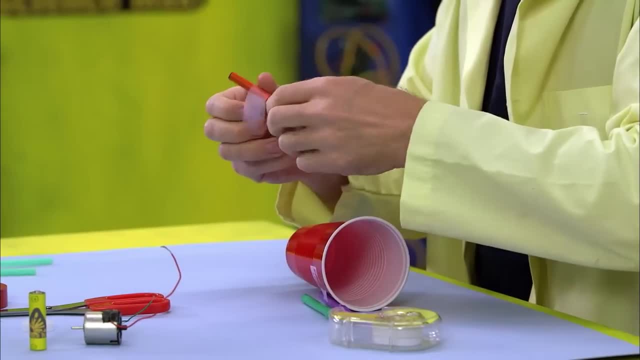 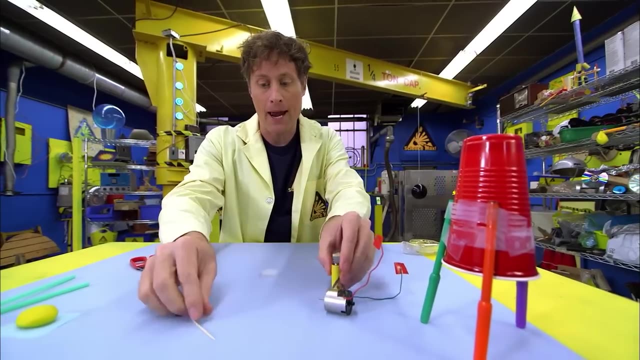 And then I put the marker on the bottom of the cup, And then I do that again to the next marker, And then the third Balance it, And there Next thing you want to do is take your plastic drink bottle cap and make a hole with a toothpick. 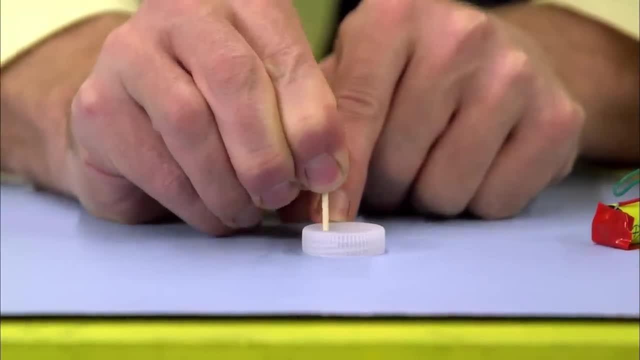 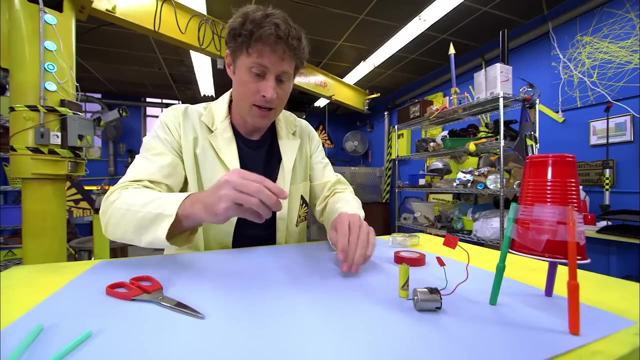 You want to make it off to the side, right about there, Just like that. That's so when it turns it will be off-center. That's what's going to give us our vibration. So once you've made that hole, take some modeling clay. 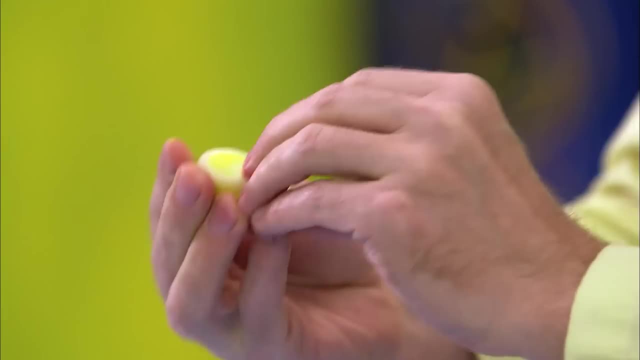 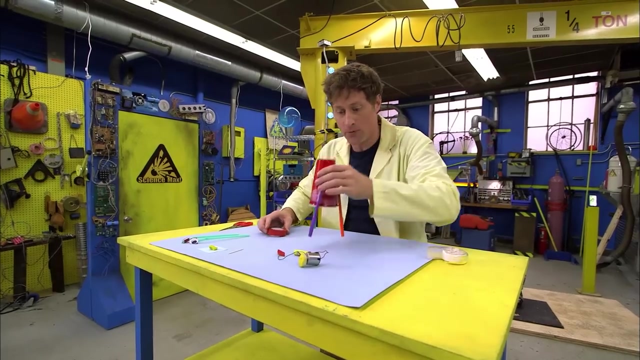 and stick it in the cap to give it some weight. When you've done that, stick it onto the shaft of your motor like this- See how it's off-center there- And then you attach it to the vibrobot. I just put it right here on the top. 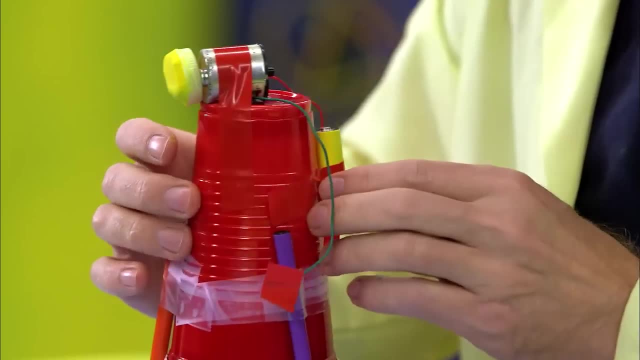 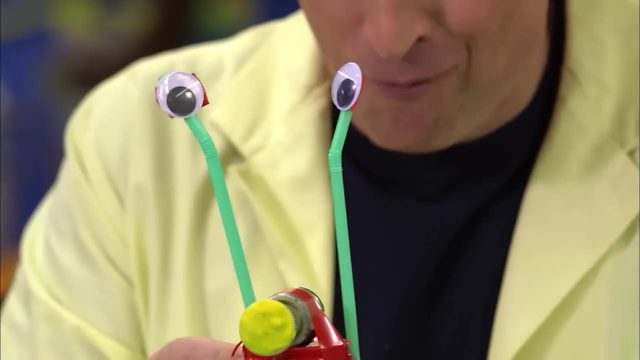 And I like to attach the battery to the back of the cup, And now, finally, we're going to attach the eyes. We take some science tape and we put the straws over. here I am vibrobot. I am here to vibrate. 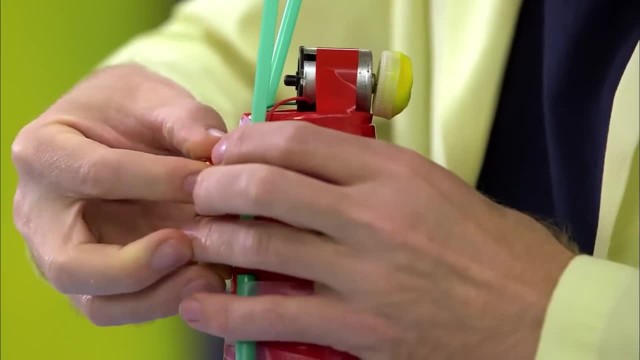 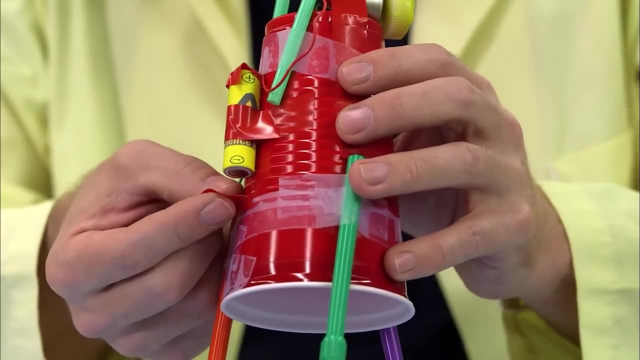 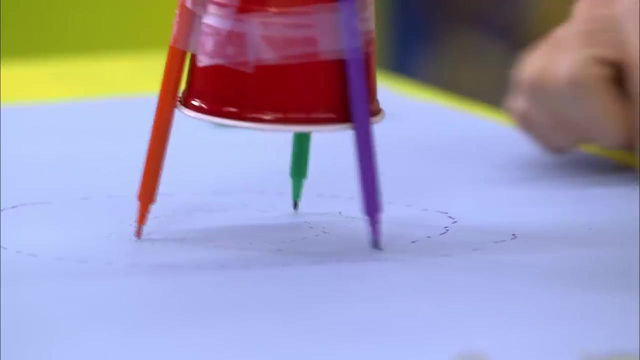 Take me to your leader. So then you attach your tape with the wire to the top of the battery there, And then the other wire to the bottom of the battery, just like that, And let your vibrobot make some art. Ha ha, ha ha. 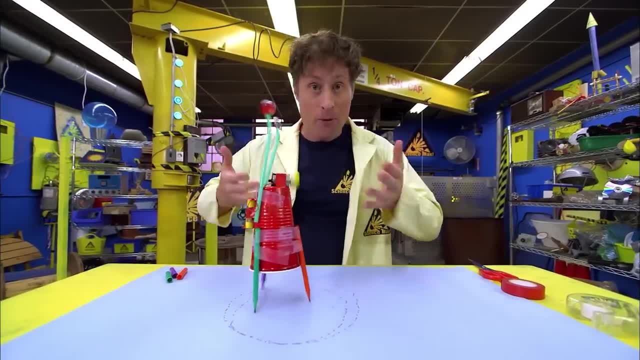 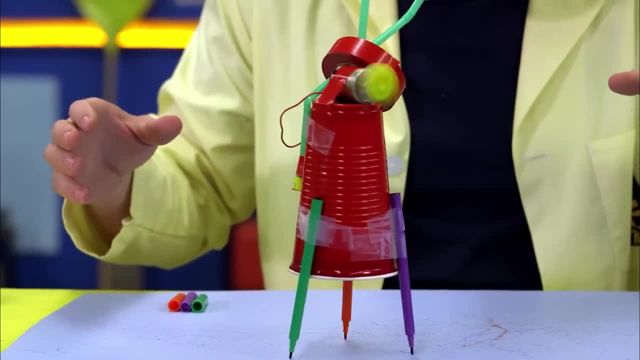 Now, if the battery is new, your vibrobot might be jumping up and down quite a bit, So you can do what I like to do and add some more weight, And then you make better lines with your vibrobot And your vibrobot makes art. 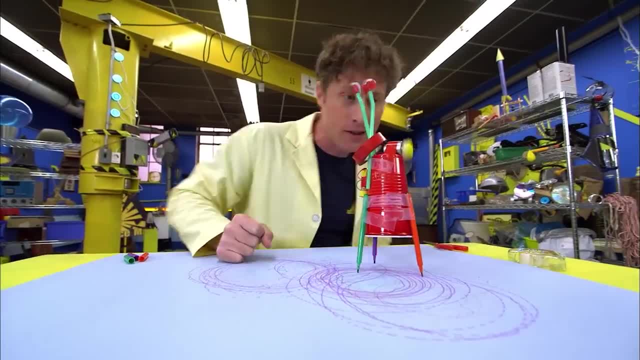 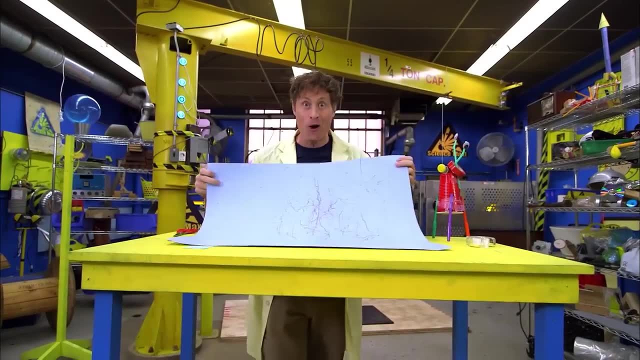 How long will he last? Probably till lunch. And there you go: Vibrobot art- Art made by a robot. How cool is that? So that's what we're going to do today. I'm going to meet Chris from Logix Academy. 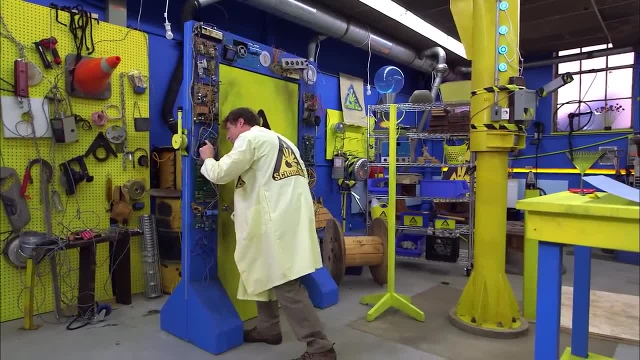 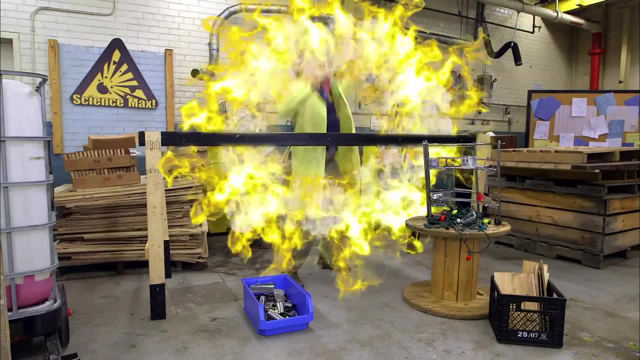 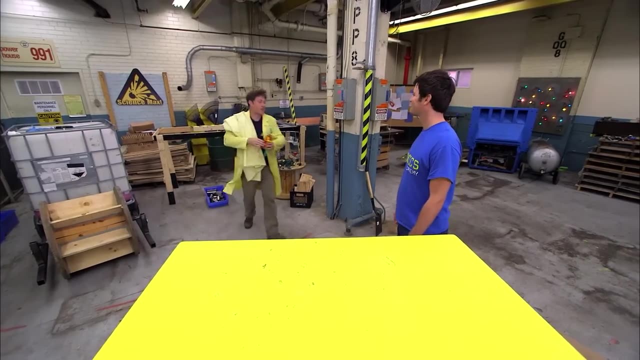 And he's going to help me max out the vibrobot Plus. we're going to learn a little bit more about vibration. Come on, Oh hey Chris, Oh hey Phil. Thanks for coming My pleasure. OK, here's your Science Max lab coat. 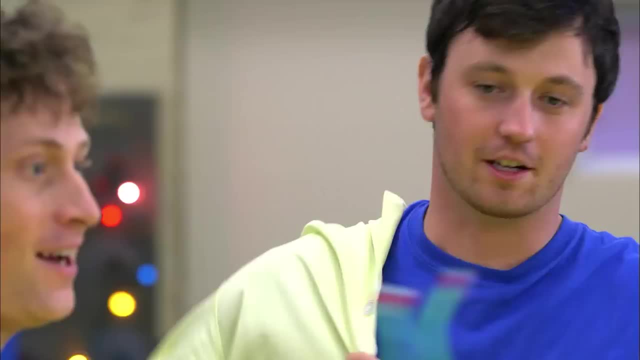 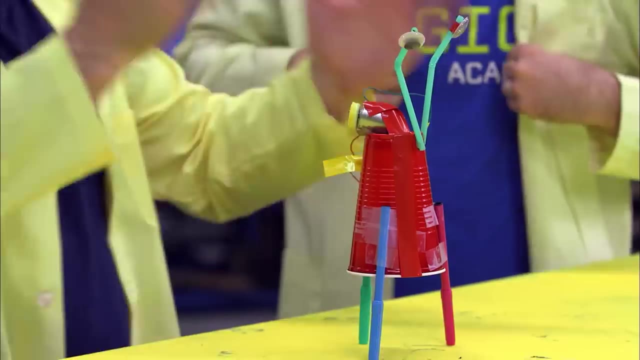 Thank you. So you guys at Logix Academy, you also build a vibrobot, right? That's right We do. This is mine, And it works pretty well. That's awesome, So I want to max this out, Cool. 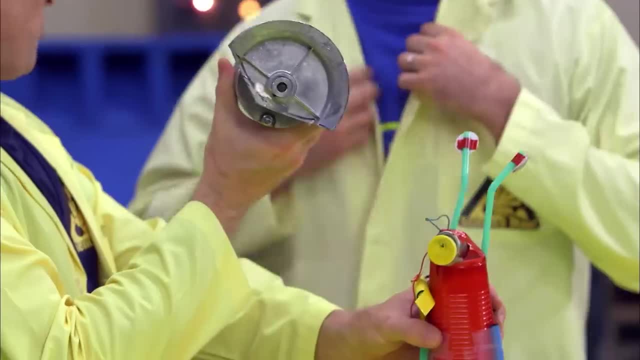 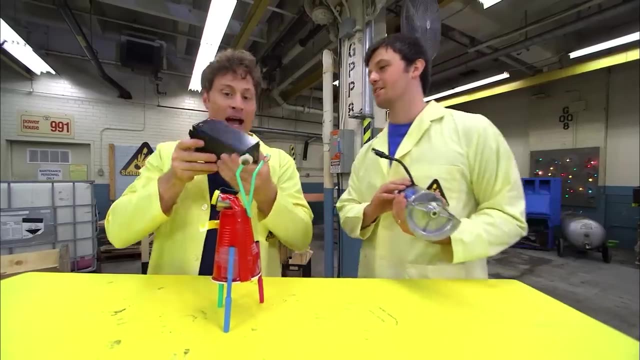 So I thought we would start with, instead of this motor, we would start with this motor. Wow, It used to be a round circle, But I cut it off so that it's off center. Perfect, I've also got. this is our battery. 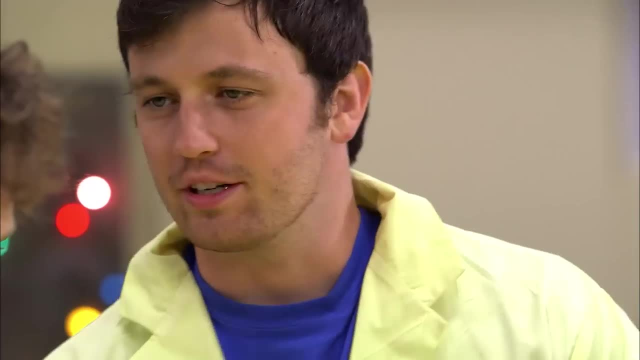 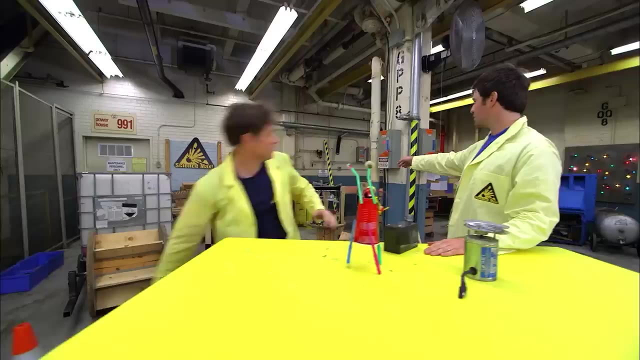 Fantastic. That's as far as I've gotten so far. Well, it looks like we need a frame next, Right, something to be the cup. That's right. So we just need some sort of larger cup. Ooh, how about that metal shelf over there? 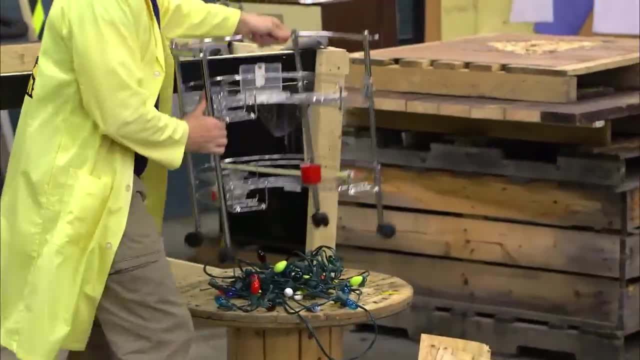 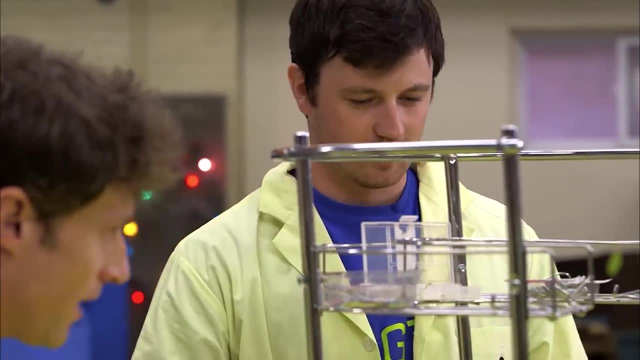 Oh, this thing. Yeah, This is just something I keep my parts on. It's perfect, Really. Yep, the shelves will house everything that we need And it looks like it'll be strong enough to hold everything together. Now, the vibrobot had markers on the bottom of it. 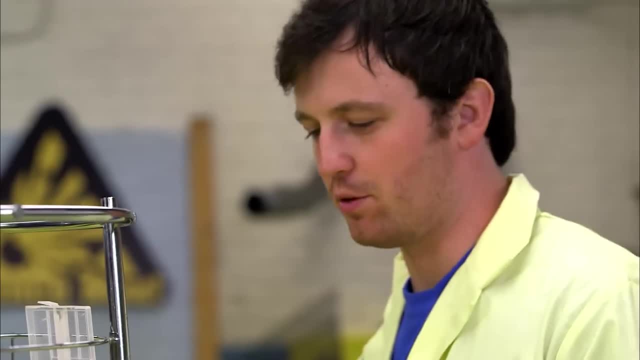 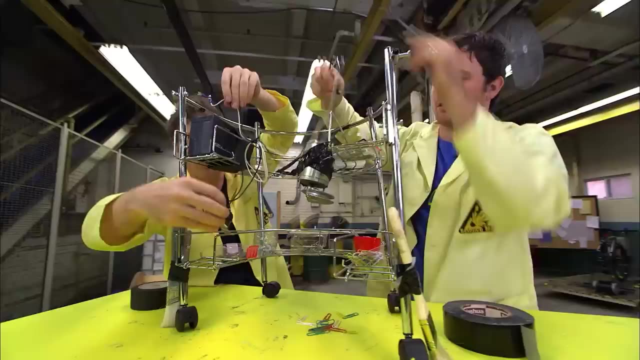 That's right To make a little pattern. Should we try that with this, Because we're going bigger? what if we use paint and paint brushes instead? OK, sure, We could attach paint brushes to the legs. Pass me one, All right. so now all we need to do 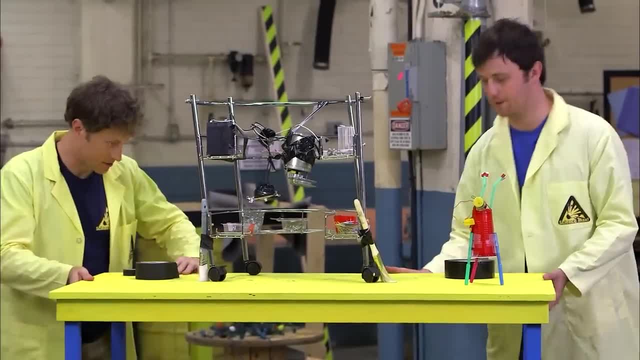 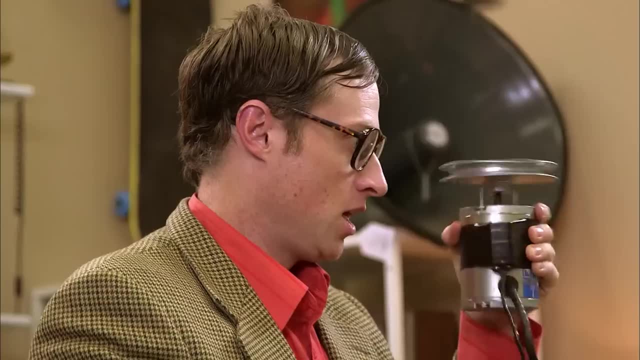 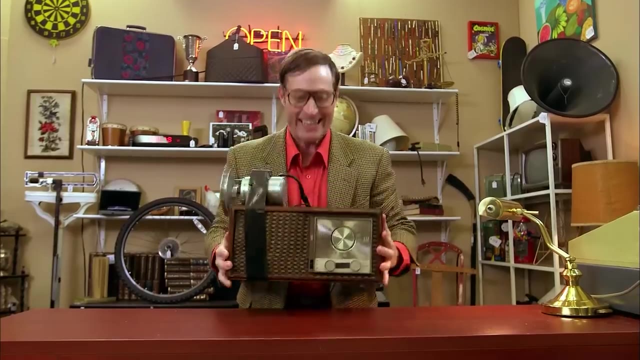 is: get some paint and some paper. That's right, And we can fire it up. OK, let's move it over this way. Let's go. Vibration and frequency- what's the difference? They're all connected, Ta-da. 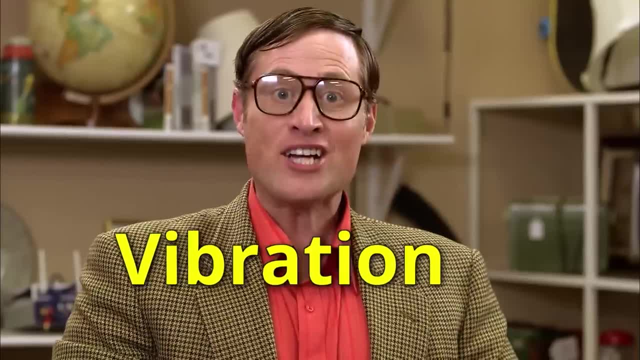 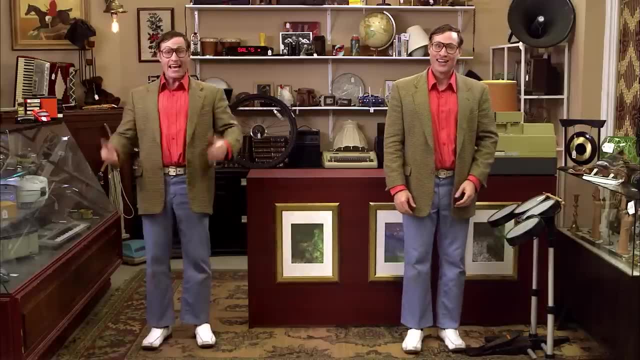 Now we can. whoa Vibration is things going back and forth, back and forth, and back and forth? It's a cycle Cycle 25 bucks. Oh yeah, it's the wrong kind of cycle, Never mind. 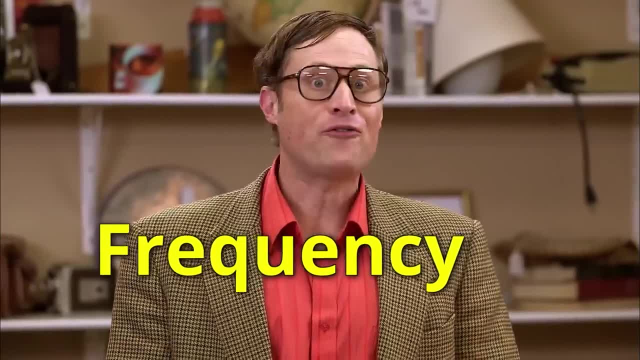 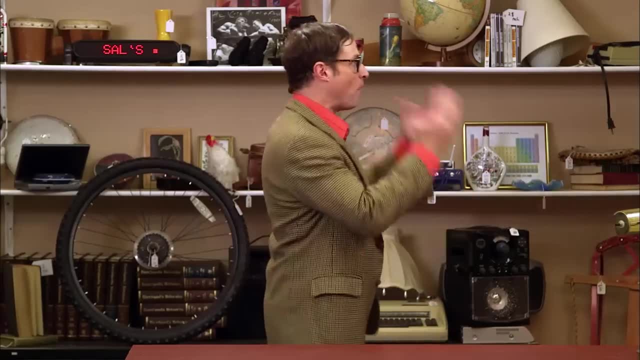 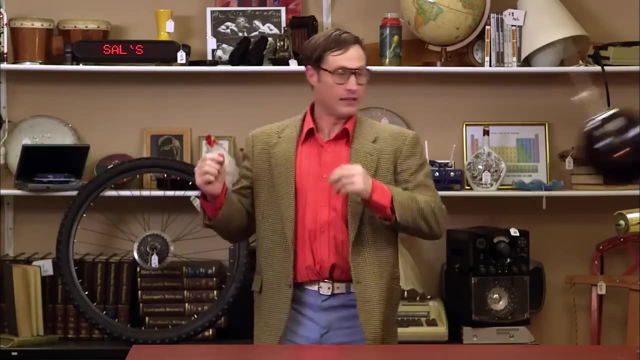 Well, if that's vibration, then what's frequency? Well, frequency is a measure of how fast or slow, how frequent those vibrations happen. Look at this bowling ball. It is swinging back and forth, but not very fast. You could say it has a low frequency. 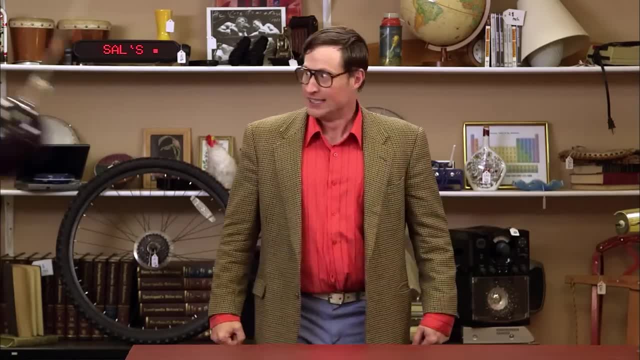 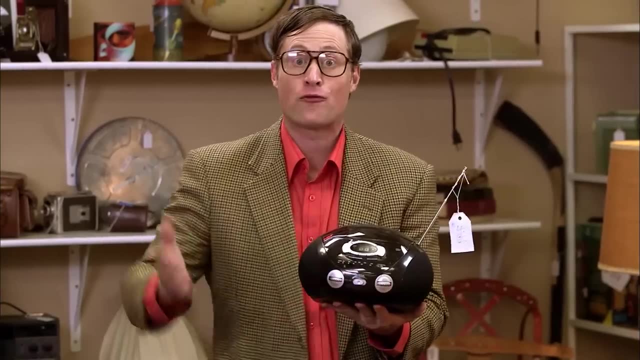 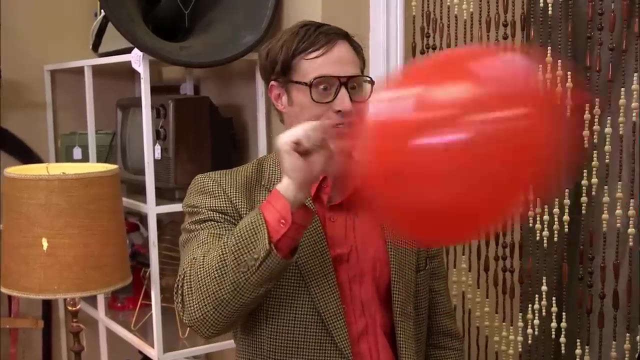 We measure all kinds of things by the frequency. This thing is terrifying. When you turn the dial on your radio, you're tuning in to different frequencies of radio waves. Hey, look at this punching balloon, It's going very fast. You could say it has a high frequency. 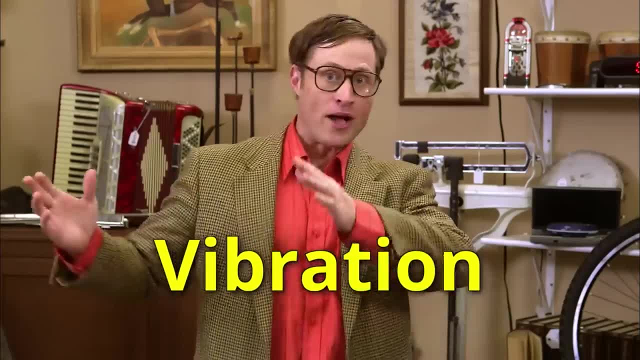 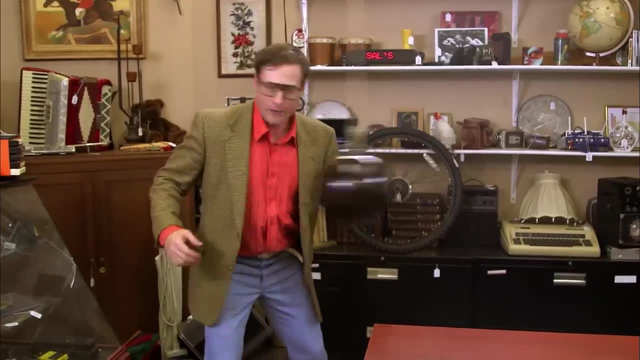 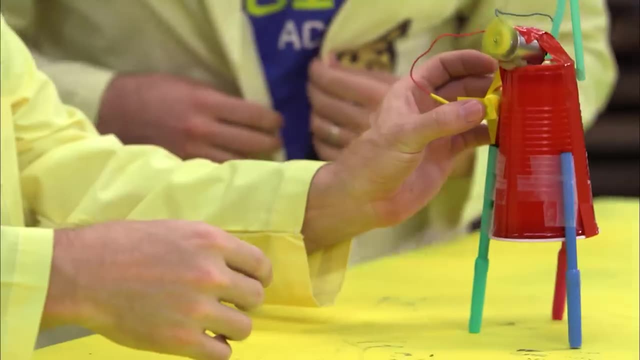 So now you know, Vibration is something going back and forth and frequency is how quickly it does it, Ramona? the bowling ball keeps coming through everything. How do you turn it off? Okay, back to our main experiment. Chris and I are taking a vibrobot and maxing it out. 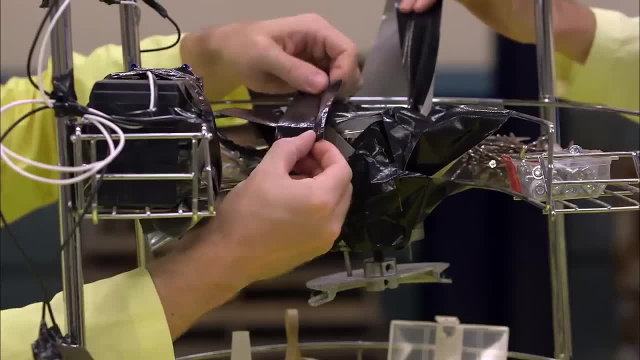 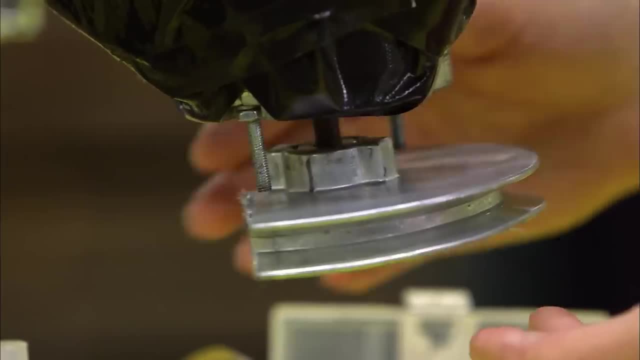 We have a large motor and a battery and we're taping it all to some shelving, Just like our small vibrobot. our motor needs something to make it unbalanced when it spins. That's what will cause the vibrations. It's just taped. 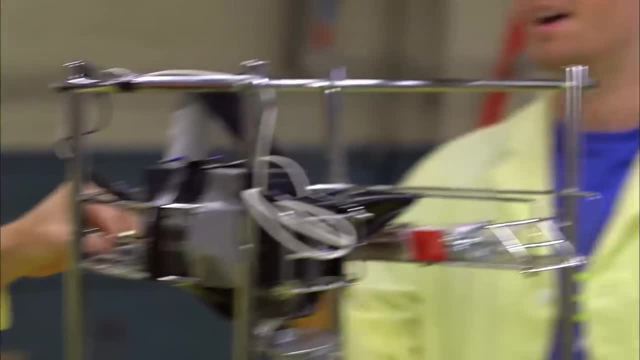 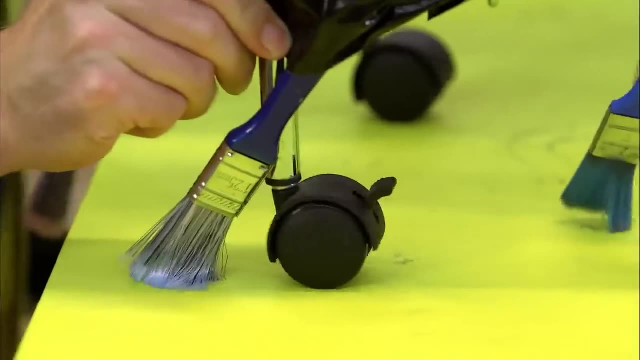 I haven't attached it in any other way. Do you think that's okay? As an engineer, I have superior faith in duct tape. Okay, well, that's good to know. We're also adding an on-off switch and some paint brushes on the bottoms of the legs. 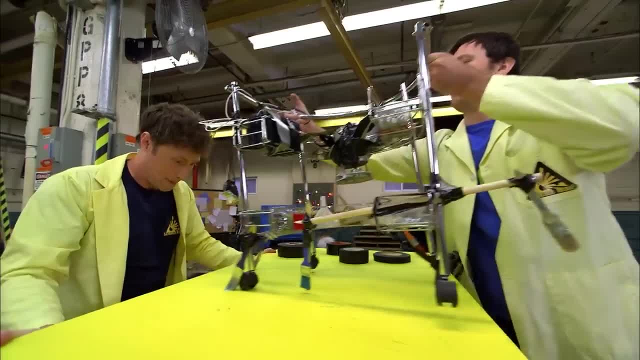 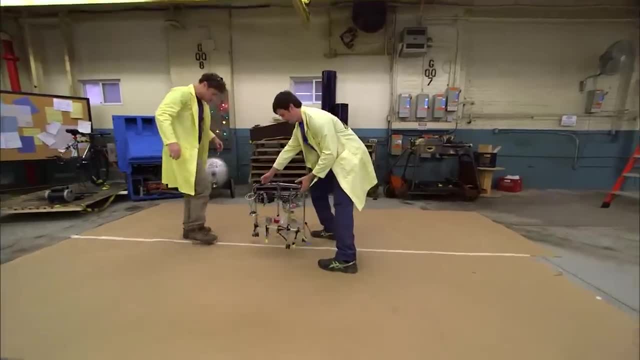 so our maxed-out vibrobot can make art just like the small one. The final step: dipping the brushes in paint and setting it on a big piece of paper. We fire it up and it immediately shakes everything off the shelves. Oh, 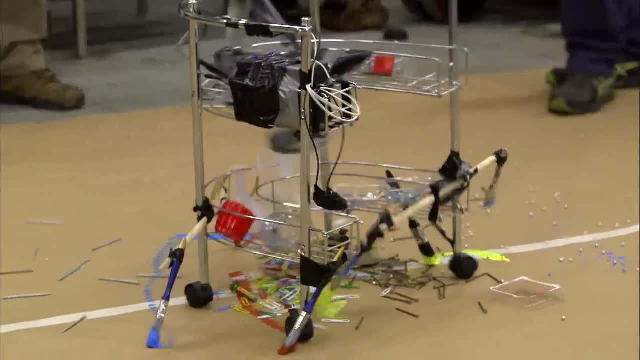 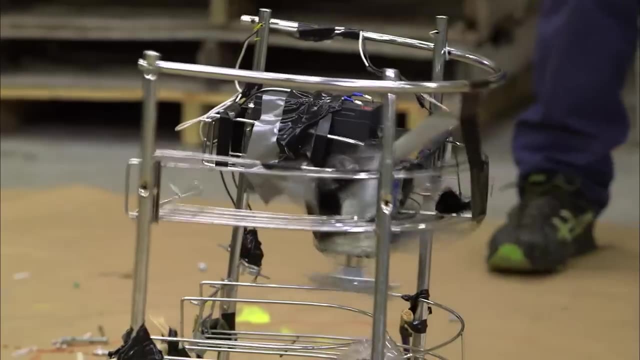 It totally spilled all the stuff on the shelves. The motor shakes the vibrobot a lot, But there's a problem. All that shaking is starting to take its toll on the shelves. The wheels come off, The screws come out And finally, 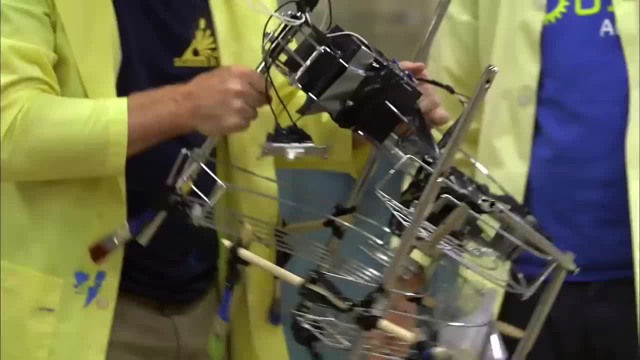 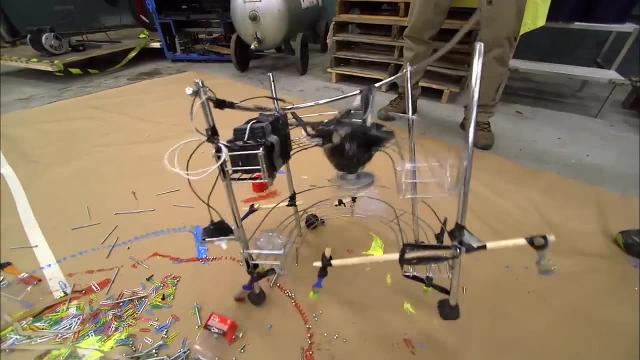 It totally shook itself apart. It destroyed itself. The shelving unit just completely falls apart. when it's being shaken, Vibration is really hard on the structure of an object. We need something more sturdy, Something that can take weight Steps maybe. 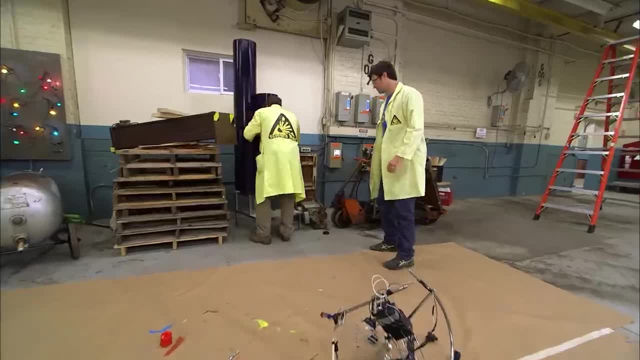 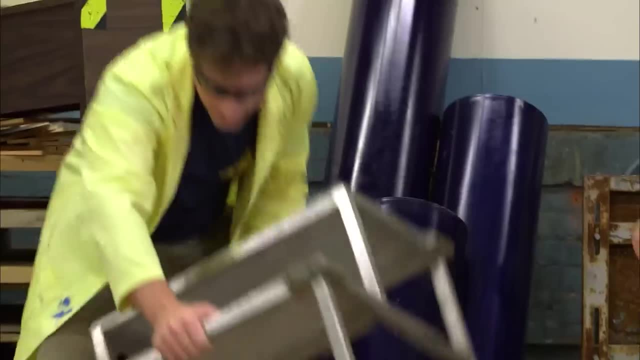 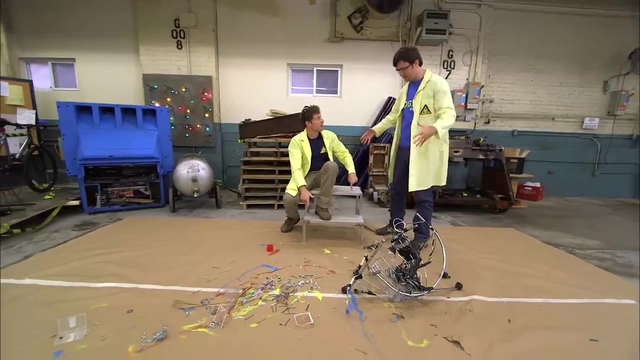 Yeah, Okay, hold on, Okay, Yeah, this looks much better. Okay, great, So we build the new vibrobot out of this. So more paint brushes, Bigger motor, More paint, More everything, More everything. 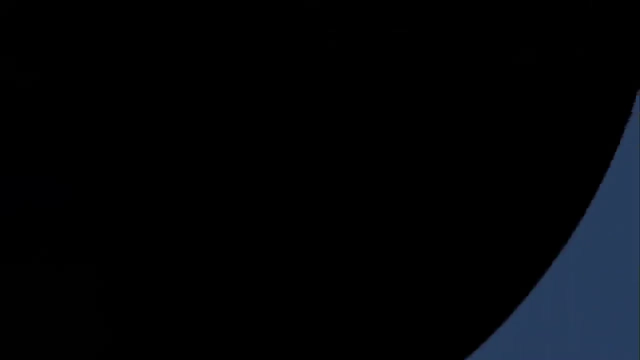 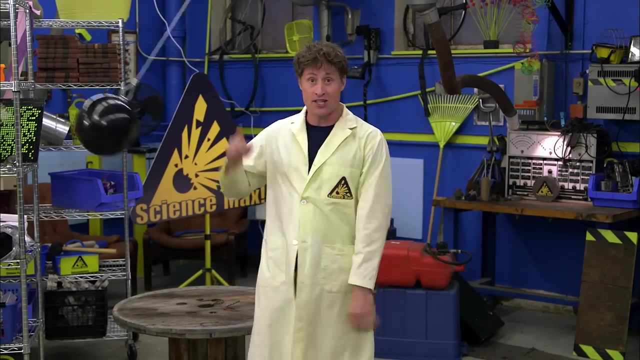 All right, good, This is a pendulum. It's just a weight suspended on a line and anchored from above. Pretty simple. Pendulums were used for hundreds of years for all kinds of reasons. It's just a pendulum. It's just a pendulum. 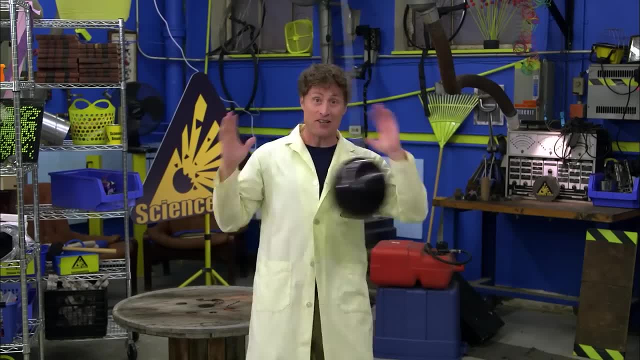 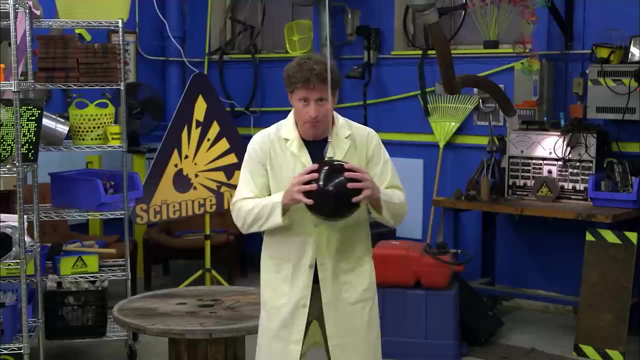 It's just a pendulum For all kinds of reasons, But most famously in clocks. Why were pendulums used in clocks? Well, here's why Let's mark every time the pendulum hits the bottom of the swing, Right here. 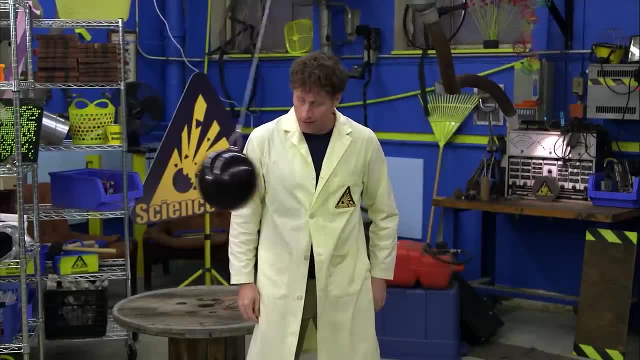 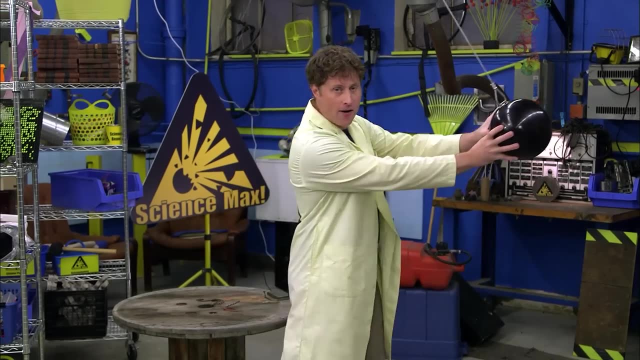 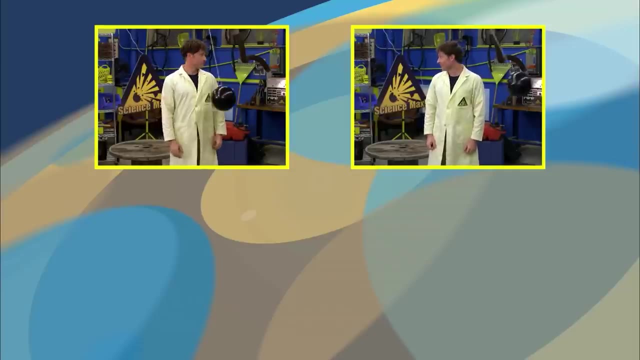 Okay, watch All right. now here's the question: How fast will the beeps be if I swing it from much higher up? Let's find out. No matter how high the pendulum swings, it keeps the same frequency. That's why they were used. Because it could swing for a long while and, even though it would lose energy, it would still keep perfect time. The frequency of a pendulum doesn't change no matter how high it swings or how much weight is on the bottom. The frequency comes from how long the line is. 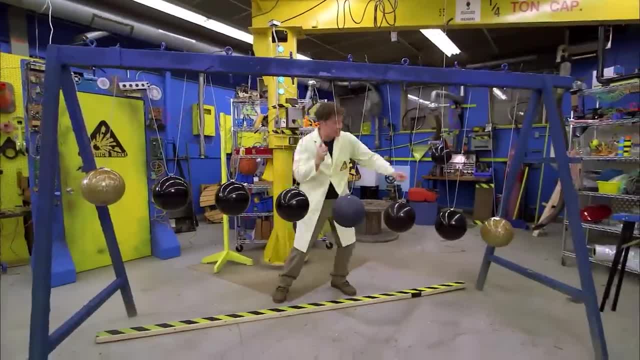 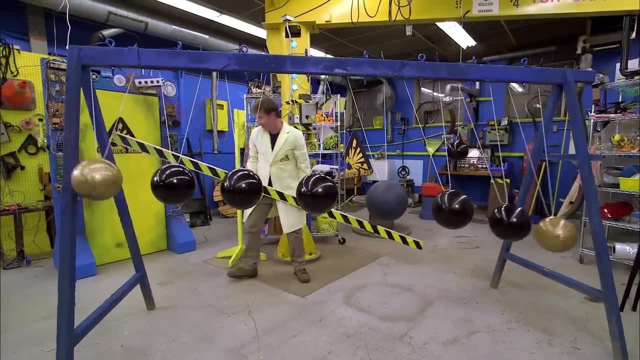 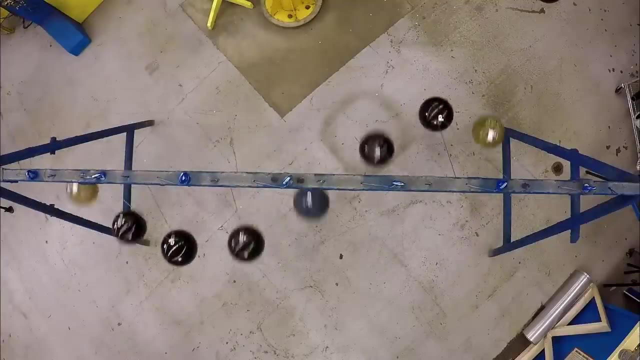 Now, this is a pendulum weight, Because each bowling ball has a line that's a different length. they have a slightly different frequency. They start out swinging together, but soon they start to make interesting patterns. Remember, each pendulum is keeping its own perfect time, even if it's slowing down. 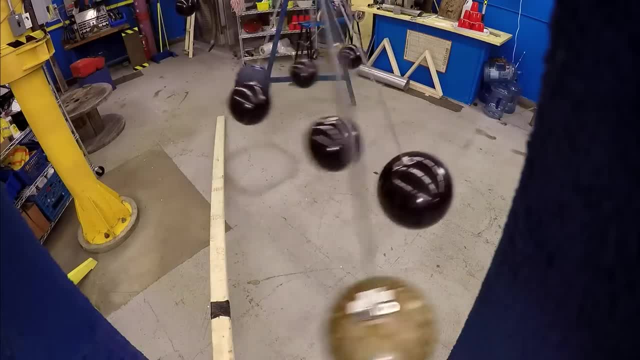 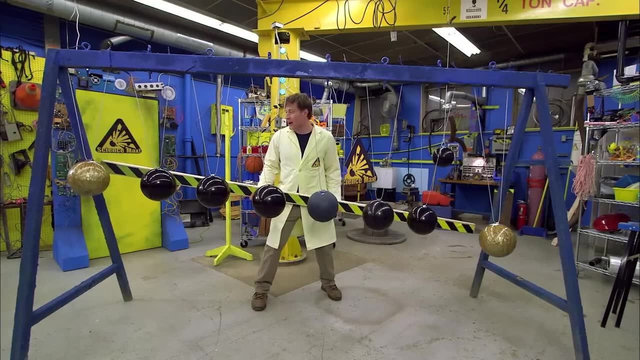 It's only the length of the line that gives each pendulum a different frequency. And now we're going to max it out with: um, well, I guess these are already bowling balls, so this is already pretty maxed out. I'm just going to leave that there. 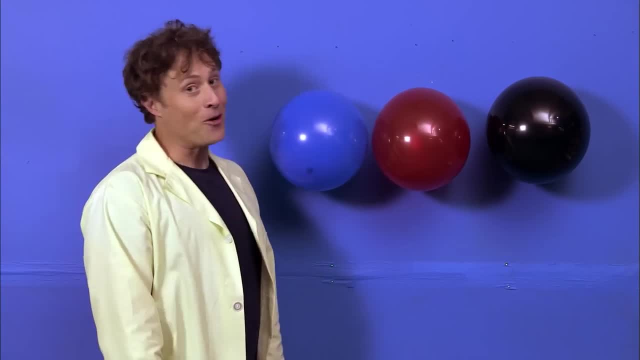 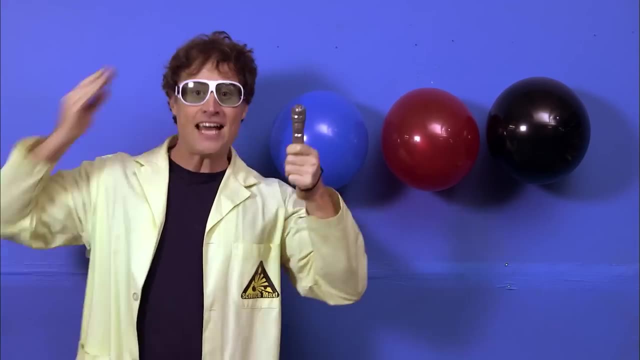 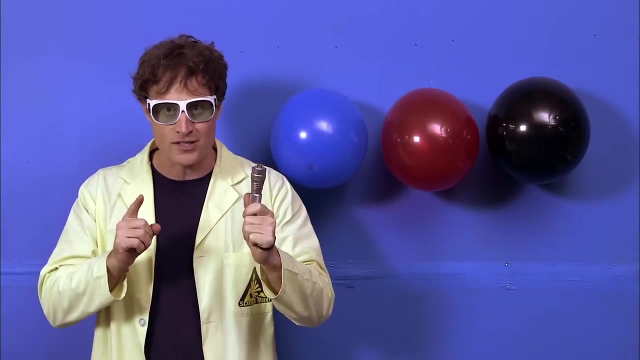 These are balloons. This is a laser and these are awesome laser safety glasses. Now, lasers are made of light, and light has a frequency. In fact, each color of light has a different frequency. This is a red laser. Check it out. 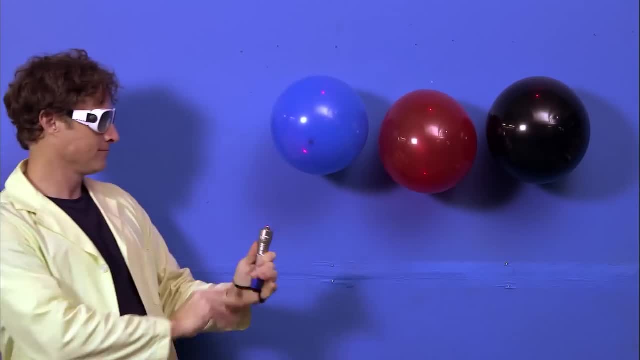 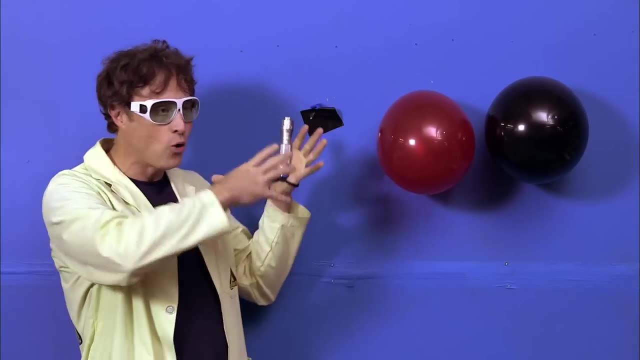 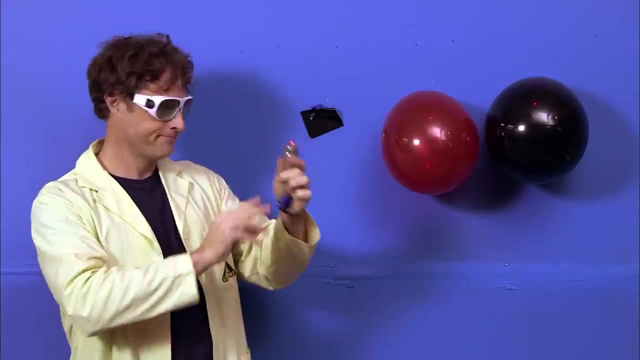 Yeah, cool, This is also a very powerful laser. Oh, I can pop the blue balloon with the red laser, because the blue absorbed the red light from the laser and then it heated up and the balloon popped. But here's the cool thing. 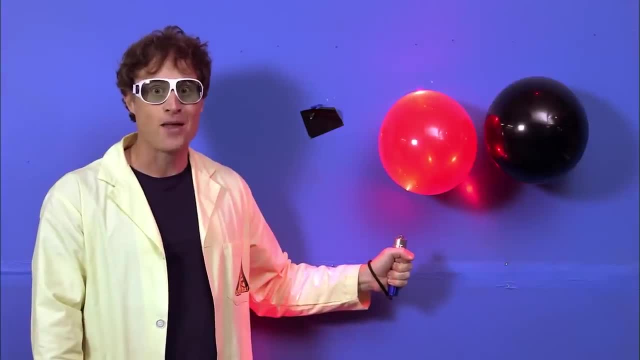 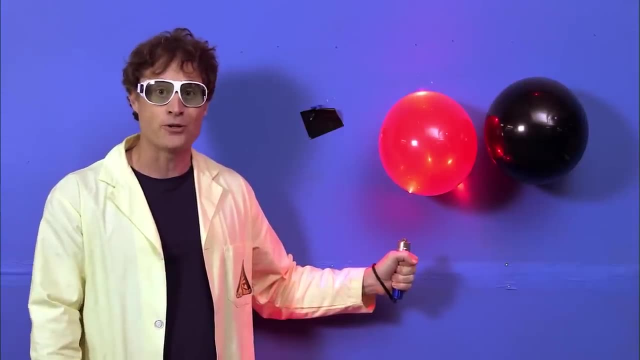 I cannot pop a red balloon with a red laser because the red balloon reflects the red light from the red laser and I can't pop it. If I wanted to pop a balloon with a red laser, I need to use a darker balloon. 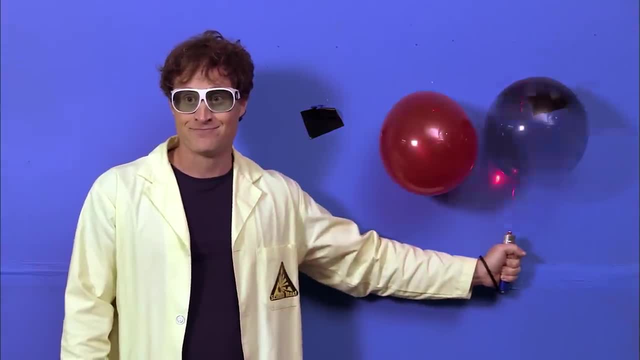 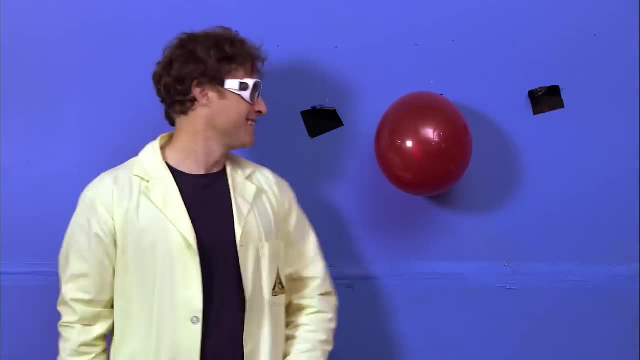 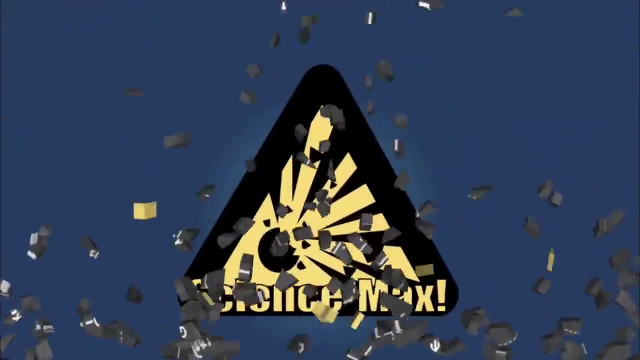 One that absorbs the red light like a black balloon. So there you go: Lasers, frequencies of light. I'm going to keep this red balloon, because it's always nice to have a balloon. Chris and I are maxing out the Vibrobot, but our last version shook itself apart. 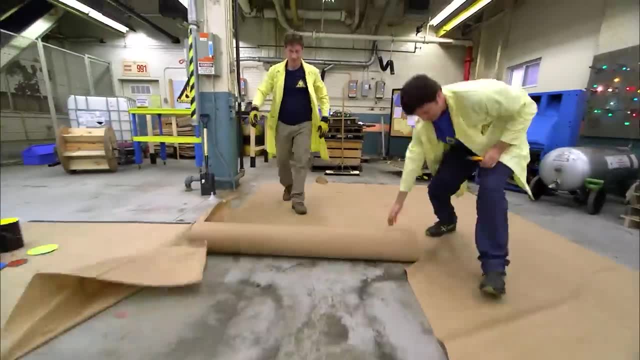 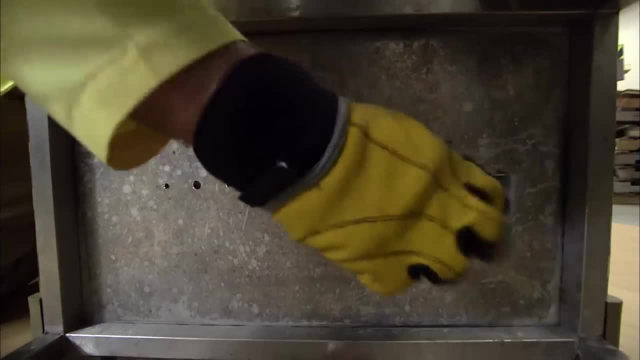 Now the plan is to start with something more solid and try again. We found some very solid steps and added an even bigger motor, an even bigger battery and attached a half-circle wheel to make the vibrations when the motor spins. We add some paint brushes and fire it up. 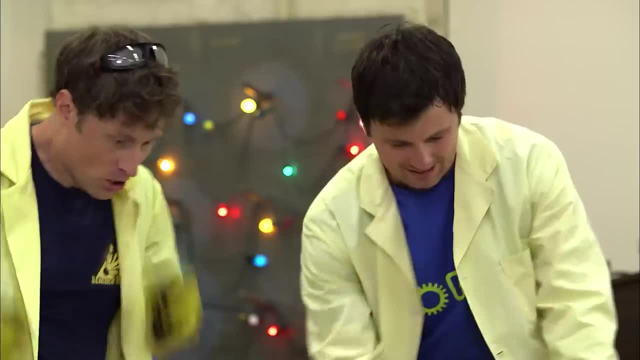 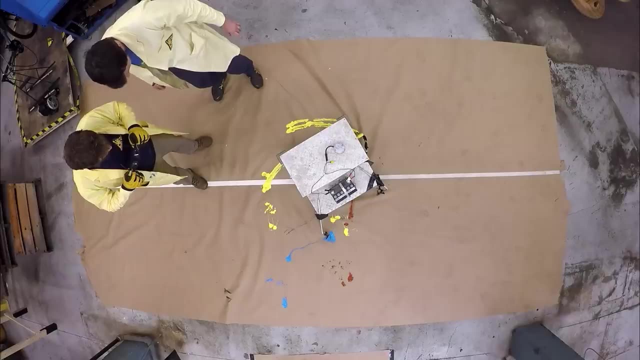 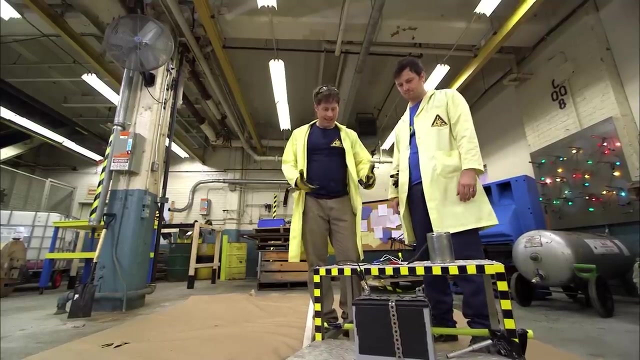 Here we go. Come on Go, Vibrobot. It wants to move. Is it moving at all? Hmm, Hmm. So it's still not working. It's already getting caught in the paper and it's on the paint brushes. 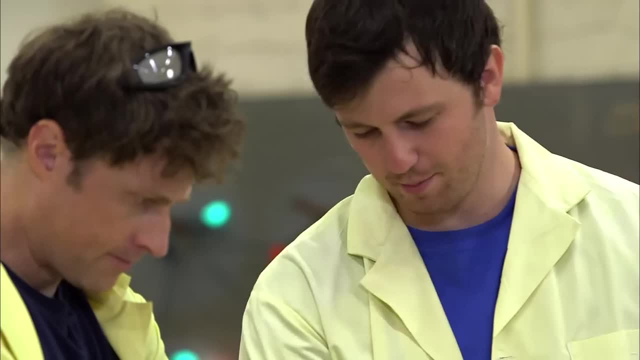 Yeah, the paint brushes seem to be absorbing too much vibration, and then the paper's stopping it as well. So why don't we remove the paint brushes? Yeah, And we might as well remove the paper if we don't have any more paint brushes. 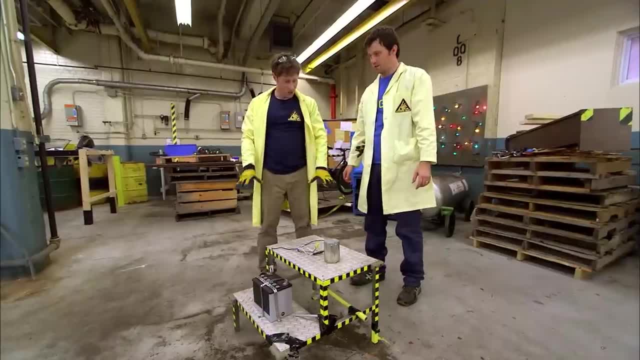 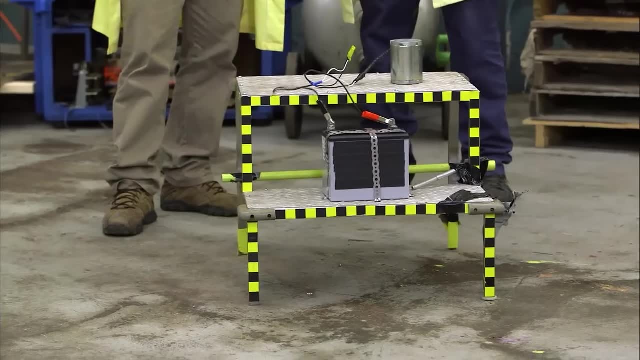 Yes, And we'll see what happens. We'll see what happens. Okay, No paint brushes, no paper. Okay, Now let's try it. Three, two, one go, Yeah, Aha, It's moving. Not bad. 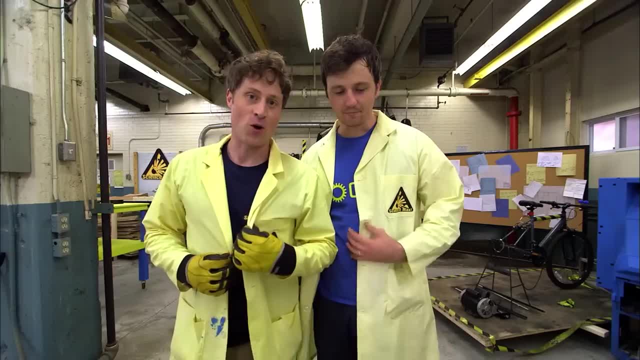 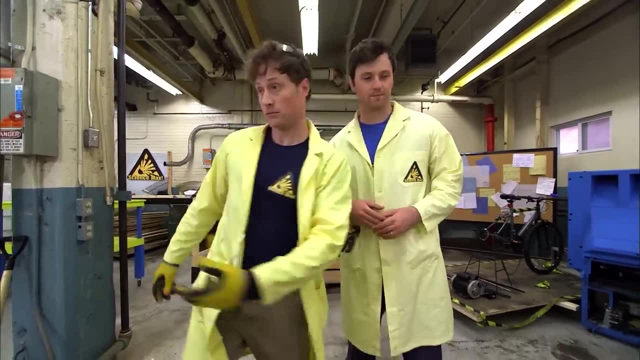 The shaking is good, but I don't know if the shaking is enough. So what do we do? Well, we could add another battery, Another battery which would give it more power. That's right. Okay, let's try that, Okay. 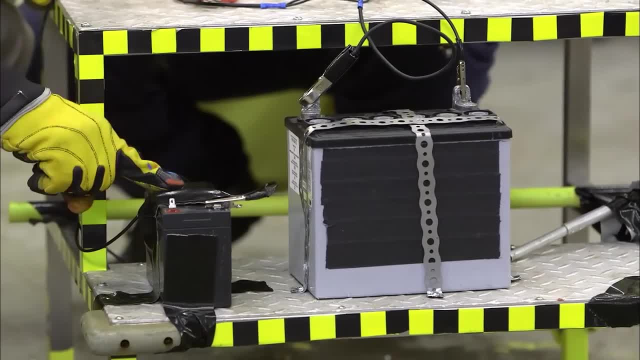 Okay, so it wasn't working before. No, Not enough power. And now we've got a second battery here. That's right. We've wired them up so that one power feeds into the other, so we've got twice as much juice as we did before. 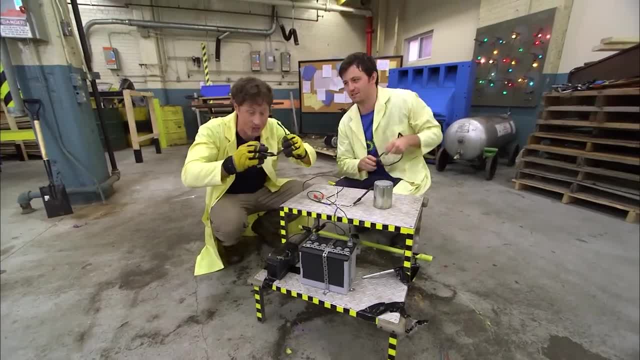 So it's just a matter of clipping this onto there. That's right. Yeah, Safety glasses, because now we don't know what's going to happen anymore. Ready, Three, two, one, Whoa. The extra battery makes a big difference. 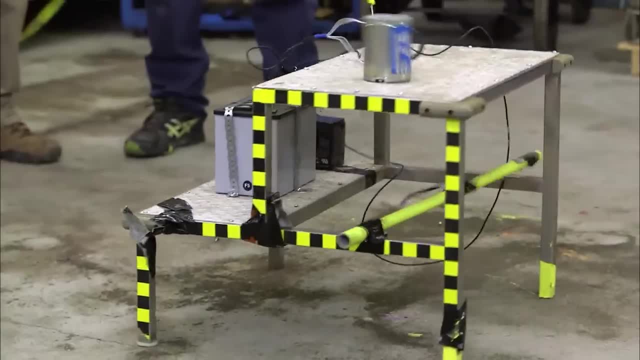 The new Vibrobot shakes around, and only shakes itself apart a little. All right, Whoa, That was amazing. Okay, so all we needed was more power. That's right. I think it didn't have enough power to vibrate up and down and that's why it wasn't moving. 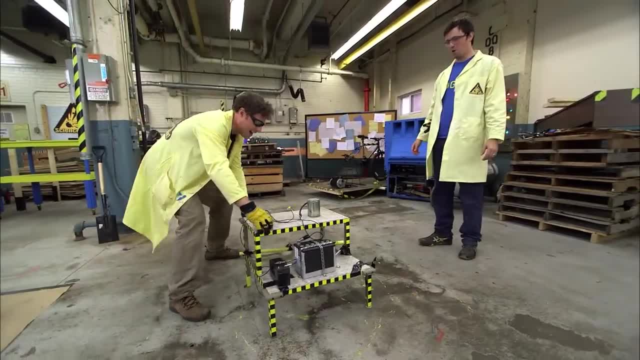 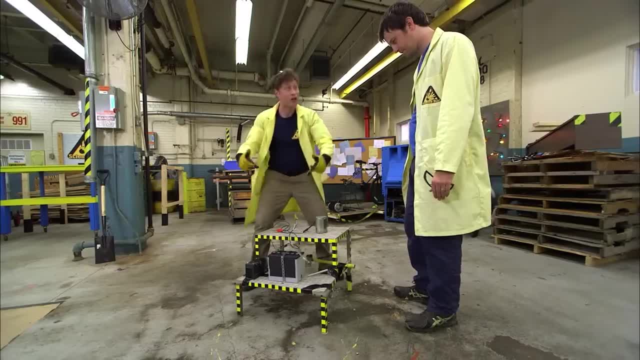 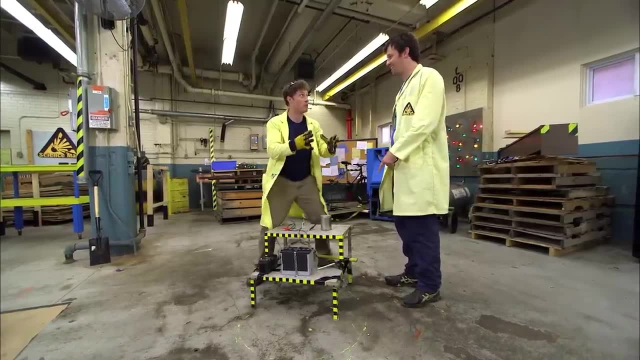 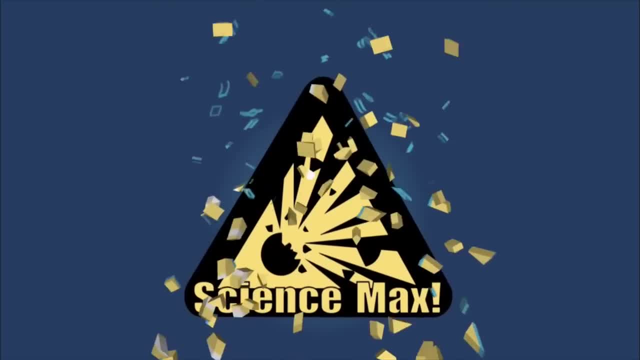 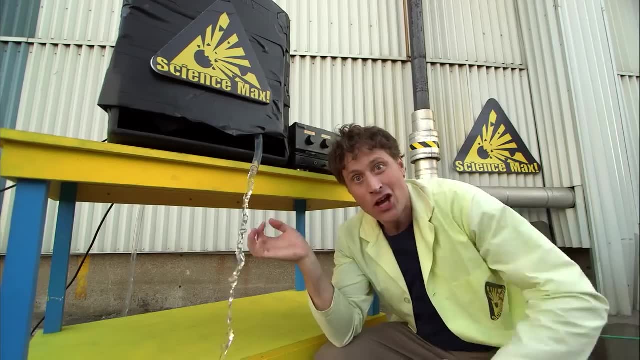 All right, All right, Oh boy. Well, there it is. There it is. I think we need to build it again. Okay, Build it even stronger and with a bigger motor, Yeah, And more power, And then maybe I ride it. 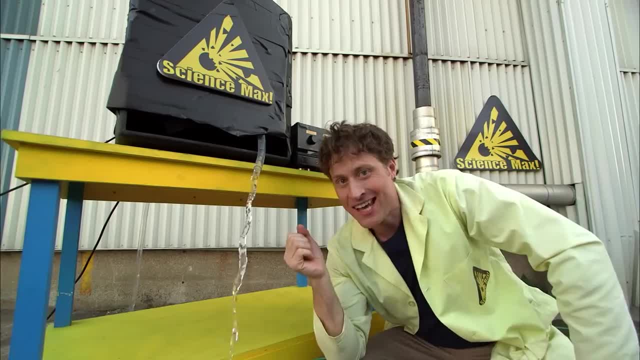 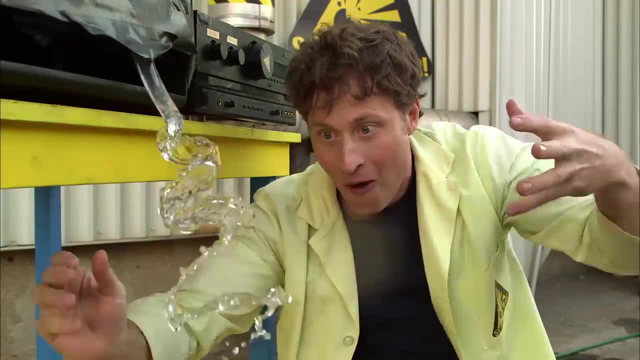 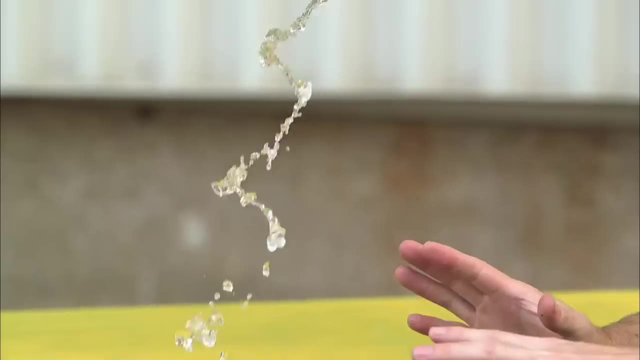 You think we could build that? Of course, Of course. Okay, Let's do it. You want to see something cool? I can make this water levitate Gravity defying water. I can even make the water go very slowly, or I can make the water go back up into the. 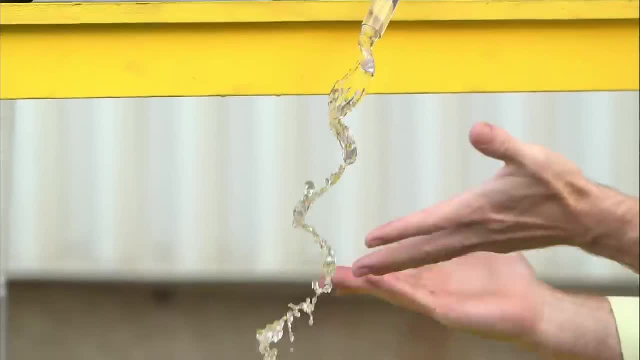 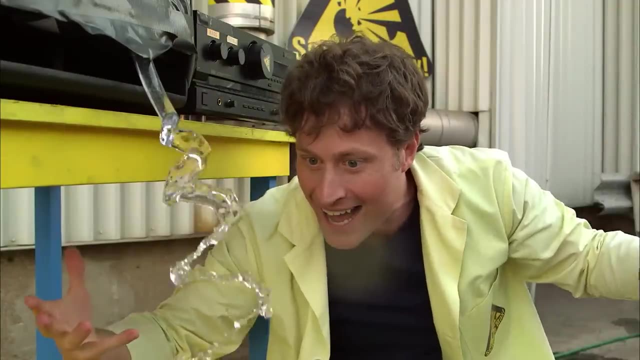 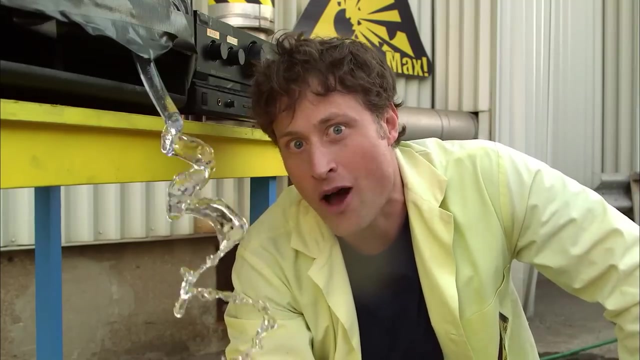 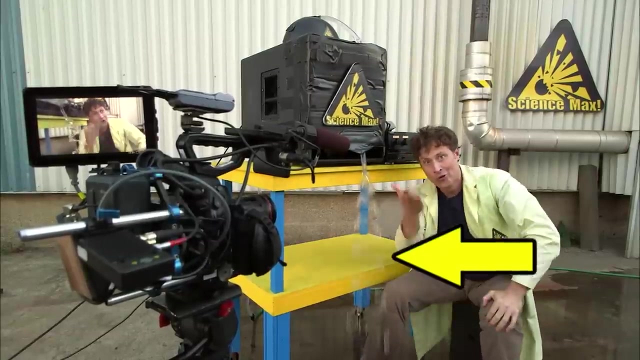 hose or I can make the water completely stop. You know what's interesting? The water does not seem to be stopped. for me, You see, stopped water because you are looking at it through a TV camera. See Real life TV camera. Real life TV camera. 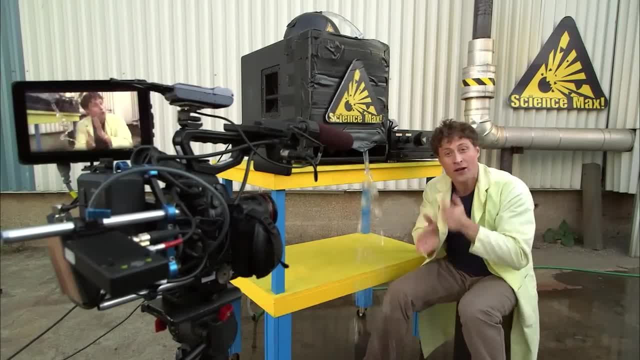 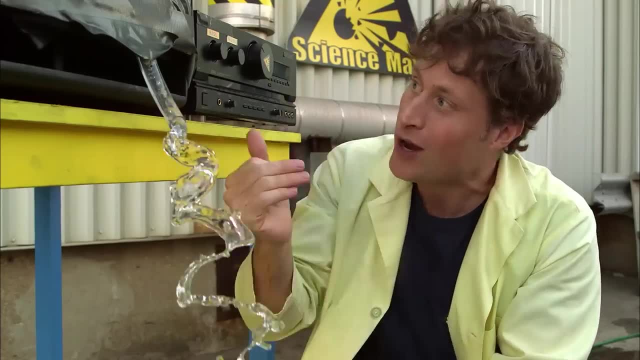 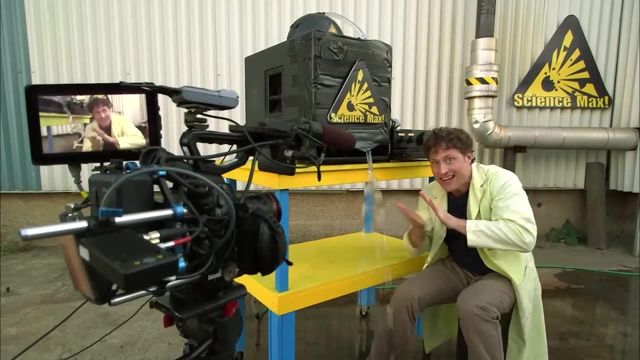 You see, movie cameras and TV cameras take a whole bunch of still photos and then run them together really, really fast, 24 times a second. for our TV cameras, I have created a device that drops water at 24 times a second And what happens is everything lines up. 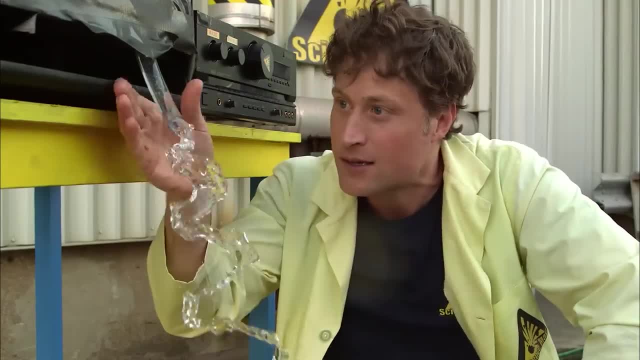 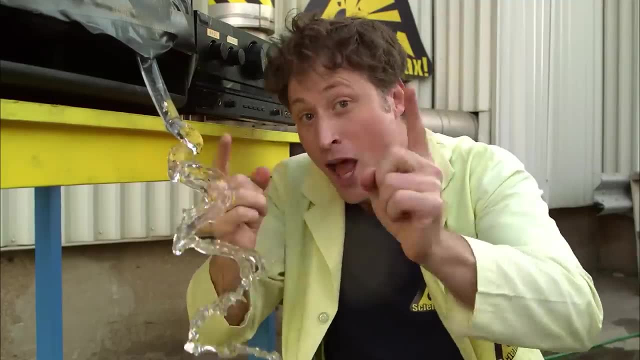 So it looks like the water drops aren't moving. But watch this. I grab the hose and it's fine, But I let it go and the hose is vibrating back and forth. at exactly the same time, the camera shutter is going back and forth and everything looks like it's stopped. 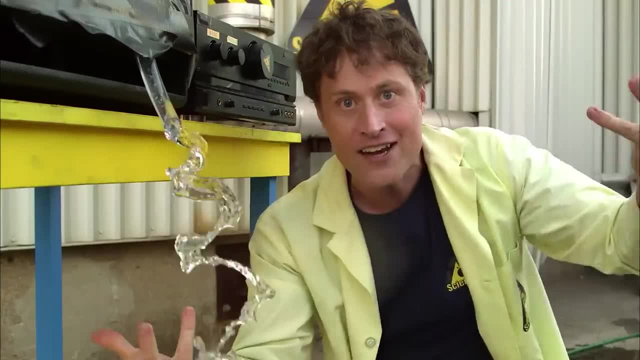 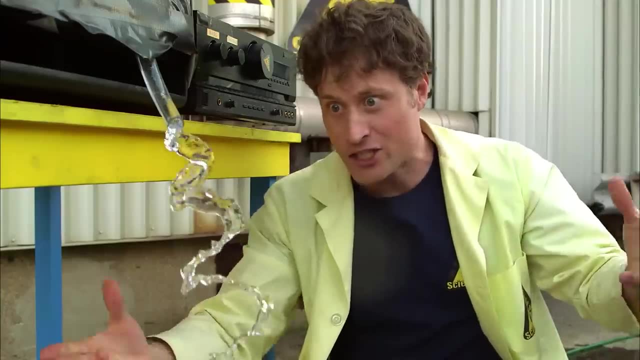 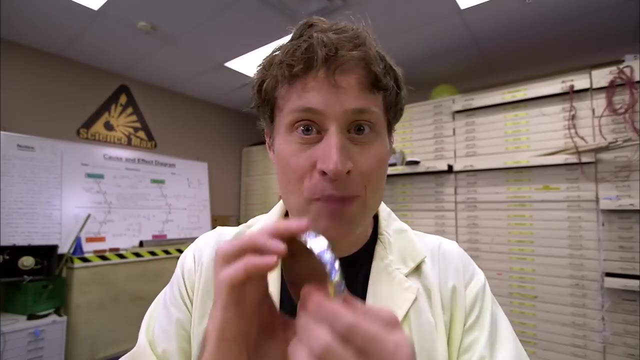 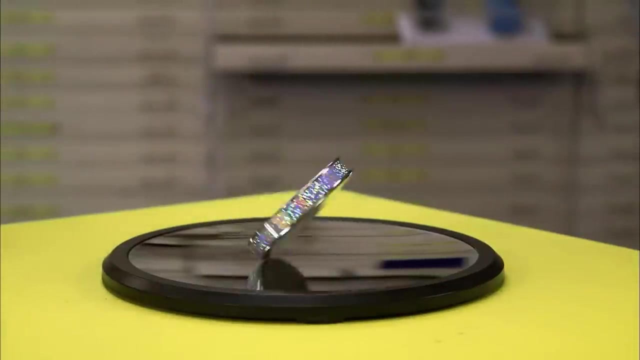 The power of frequency has defied gravity. Okay, so not really. It's kind of a camera trick, But I prefer to call it science. Science. Here's a fun way to play with things going back and forth. This is Euler's disc and it's designed to spin like this. 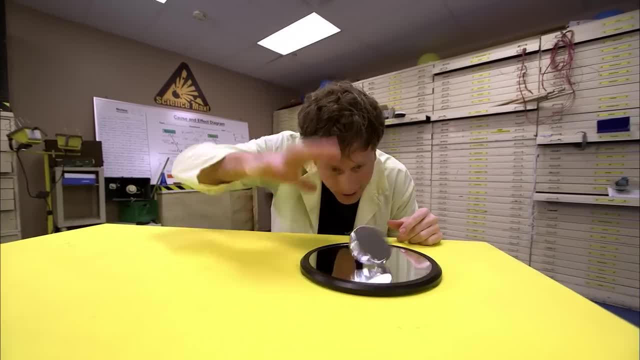 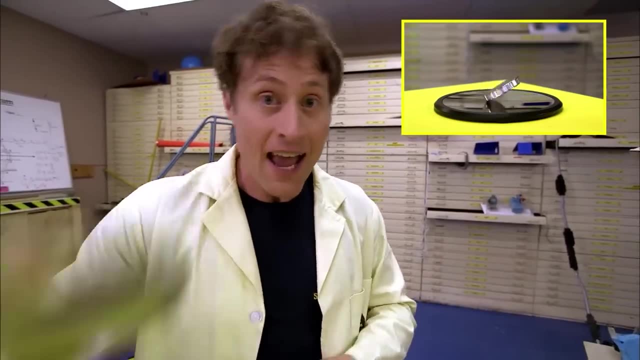 What's going on is friction and gravity are slowing that down and pulling it towards the earth. Now, you don't need a fancy disc like this to do this at home. All you need is a pot lid. Check it out. When the pot lid spins, friction and gravity start to slow it down. 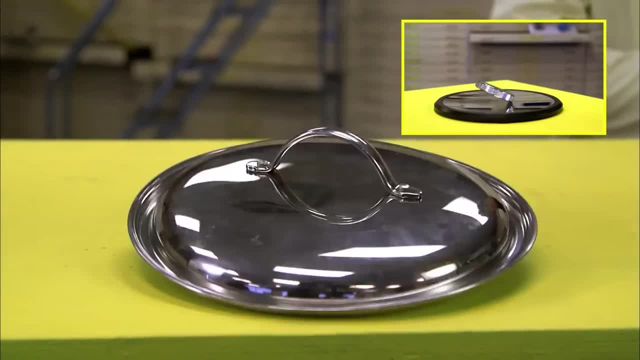 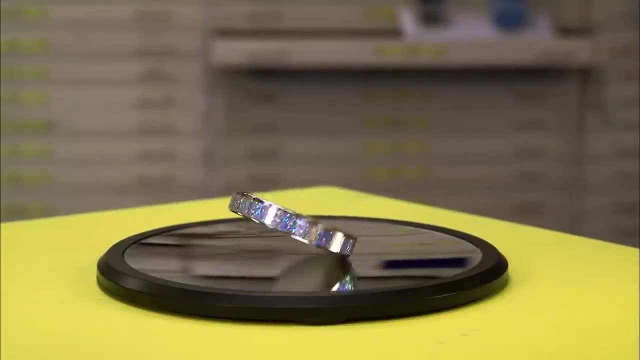 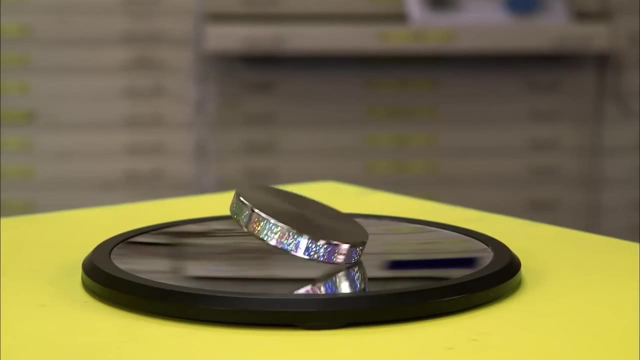 Which means each spin gets lower and lower and the frequency gets higher and higher. But the difference between a pot lid and Euler's disc is: Euler's disc is made to go for as long as possible. The heavy puck has a slightly rounded edge and sits on a glass surface that is slightly 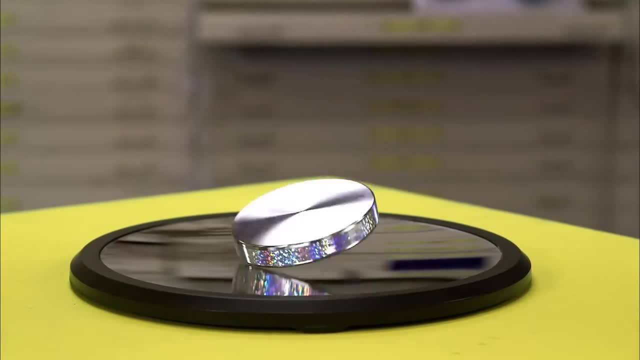 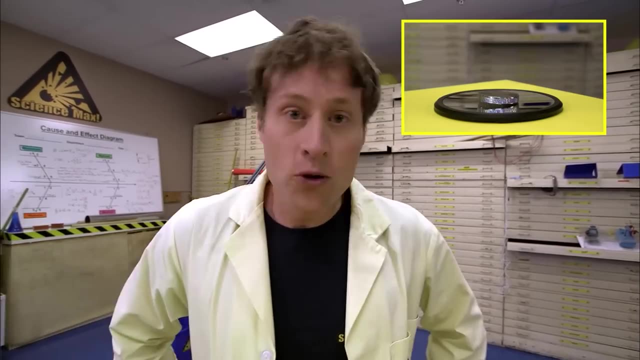 concave Like a bowl. All of this is designed to make Euler's disc last a really long time, Which is Which is Which is quite a while, But eventually friction and gravity pull the disc down and finally, 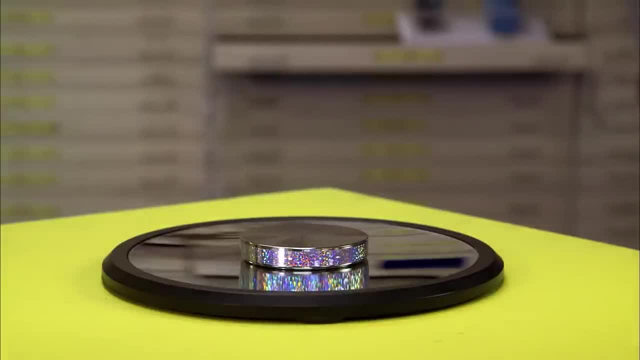 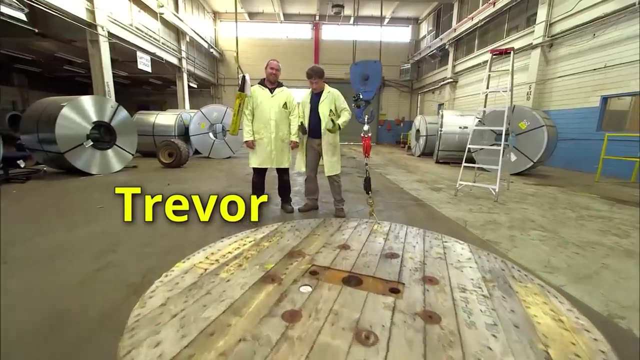 It stops. Pretty amazing, right? Well, Wait til we max it out. This is Trevor, head of the science max build team. Hey, Thanks for setting this up, Trevor. So what is this? This is a giant side of a spool. 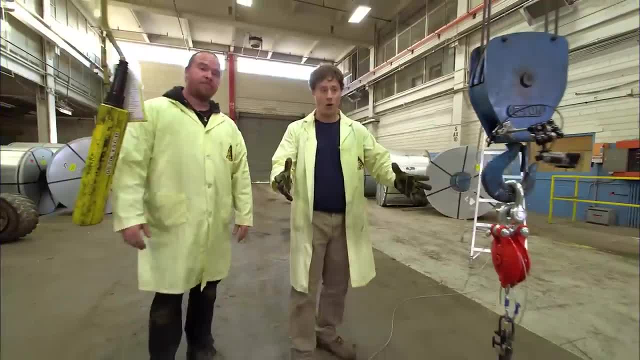 Big Hydro-. spool. Ok, so this is the largest disc that we could totally find And we've got it all hooked up here. We lift it up, we spin it and then you pull town thing and it will drop down. We lift it up, we spin it, you pull the thing and 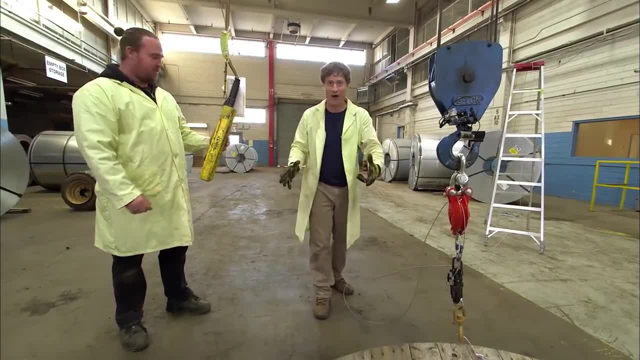 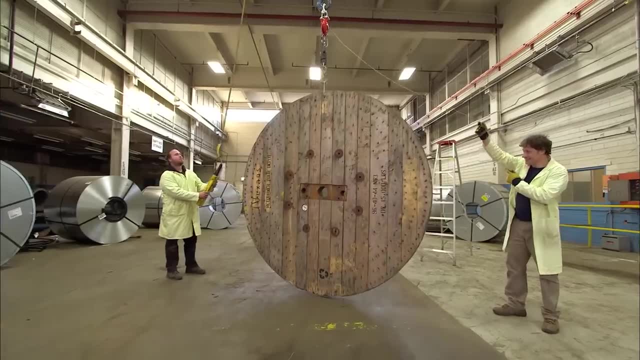 It drops down down and spin like a coin, because it's the only way we can do that with something this heavy. Yeah Ready, I'm ready. Okay, Trevor, and I hoist it up and get it suspended above the ground. Then I start to wind it up. 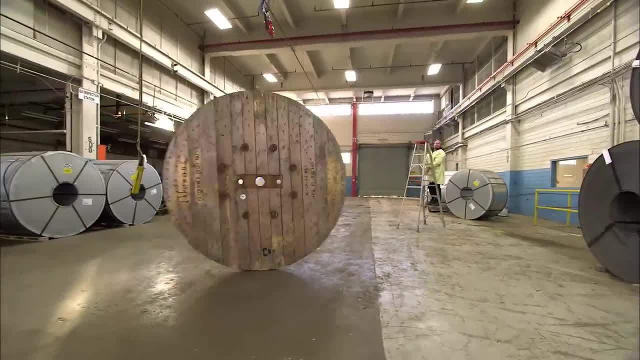 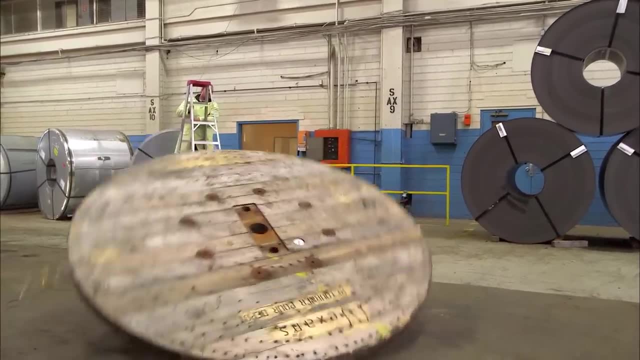 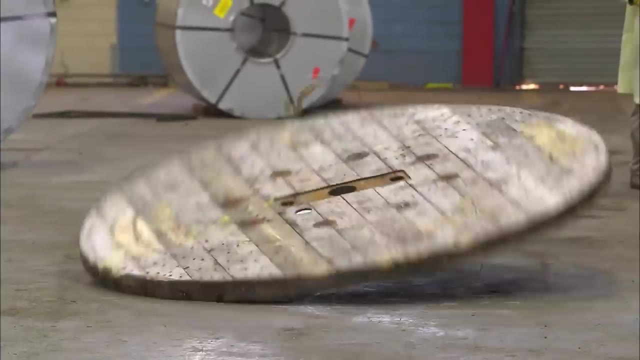 Ready When it's going fast enough. go Trevor. Trevor pulls the release and it turns out a 200 kilogram spinning disc. works exactly the same As it spins and rolls: gravity and friction work on it and the frequency speeds up as it gets closer to the ground, until 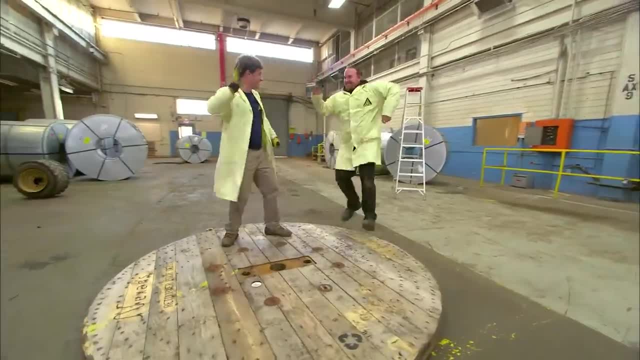 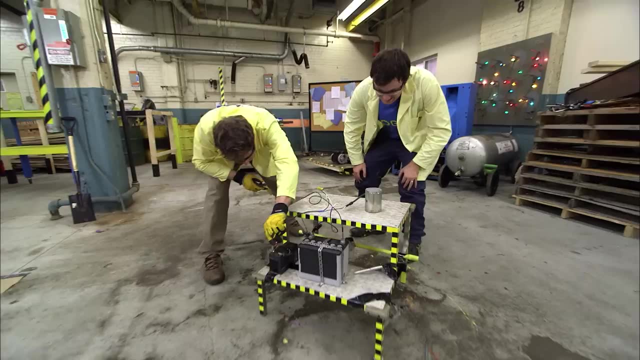 it stops Giant oiler's disc. Nicely done, Trevor. That was awesome. That was great. Let's do it again. All right, Our vibrobot was working well, so that means it's time to make a new one. Let's do it again. 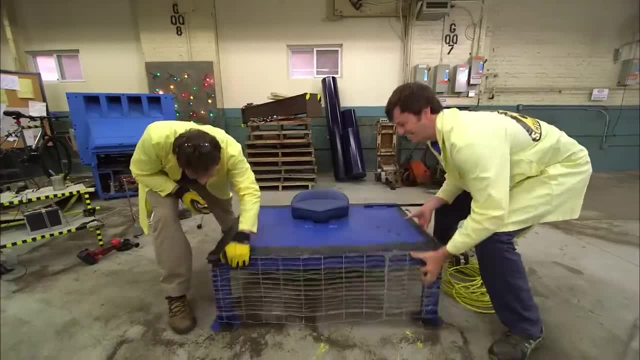 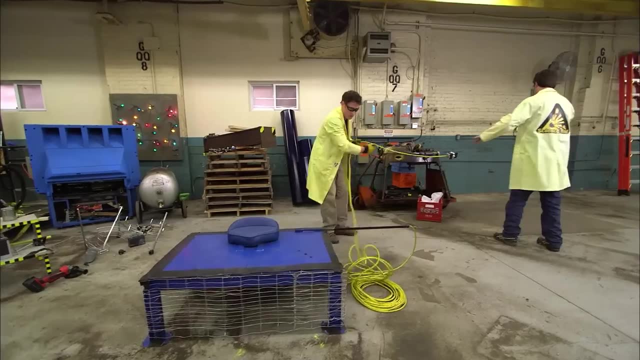 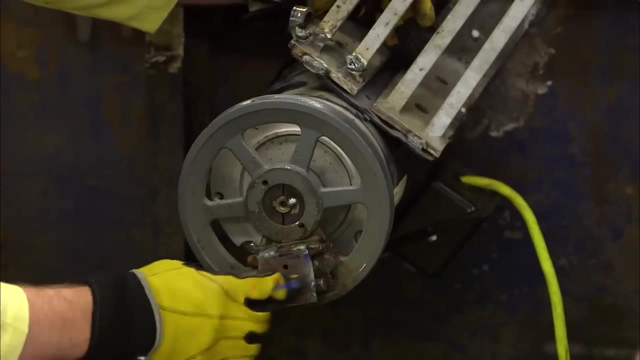 Let's make it way bigger. We started with a big metal table and added a huge motor, one 20 times as powerful as the last one. Instead of batteries giving us 12 volts of power, we're going to use a plug which is 10 times more power. We've added an off-center wheel for 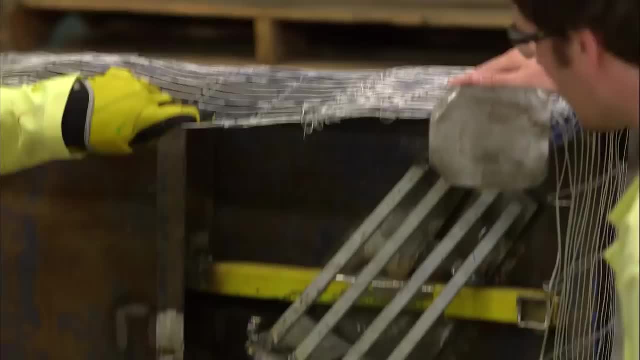 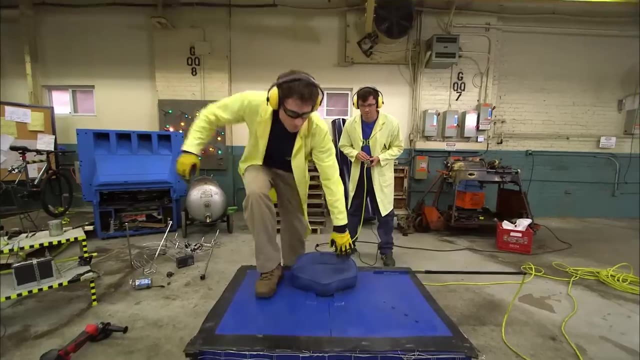 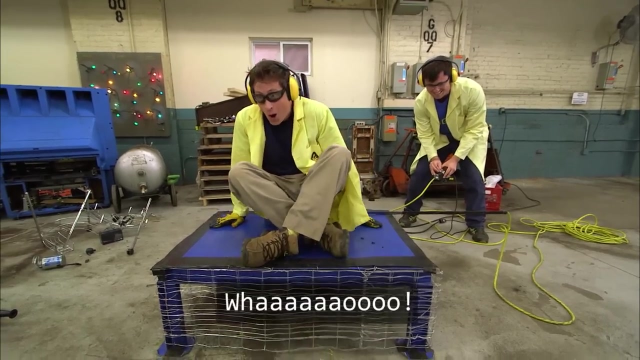 vibration, bolted the motor to the frame and added a protective cage all around to prevent anything from flying off. It even has a seat for me to ride. Okay, Okay, You ready, Ready, Here we go. We fire it up, and it's very shaky. 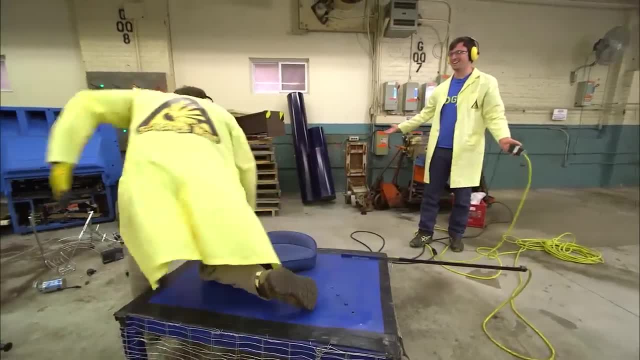 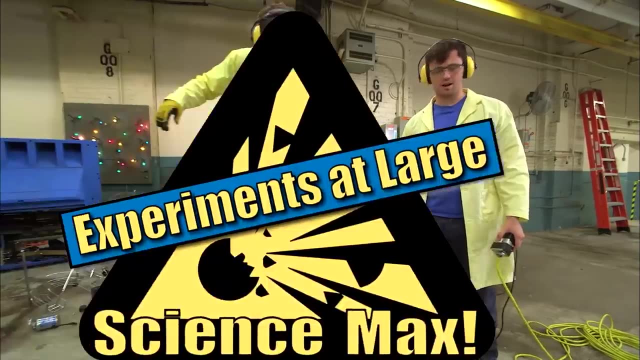 Oh, wow, Wow. That was really uncomfortable. It was like very bangy even with the seat. Yeah, Can I? I'm going to try standing on it. All right, When I try standing on it, the vibrobot lives on. 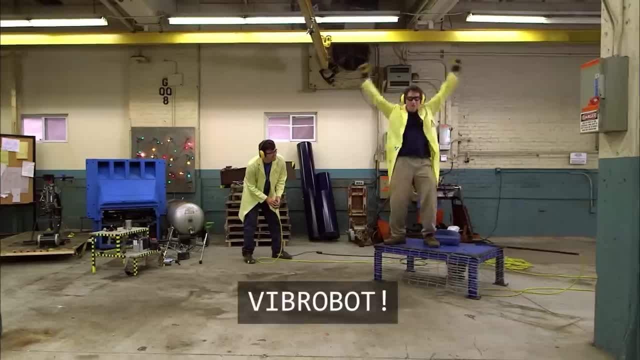 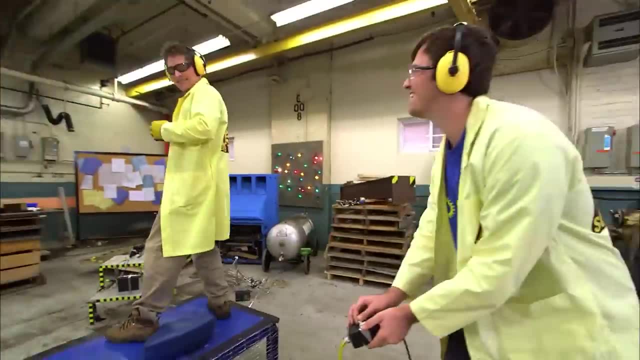 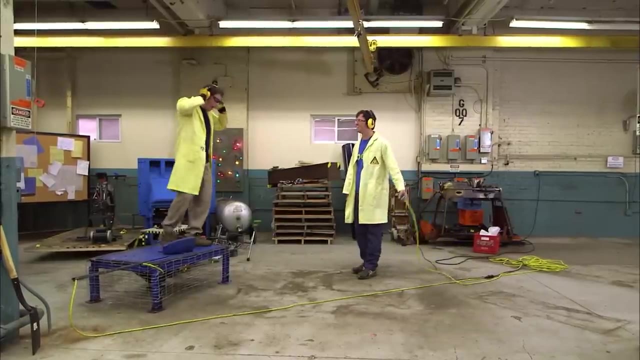 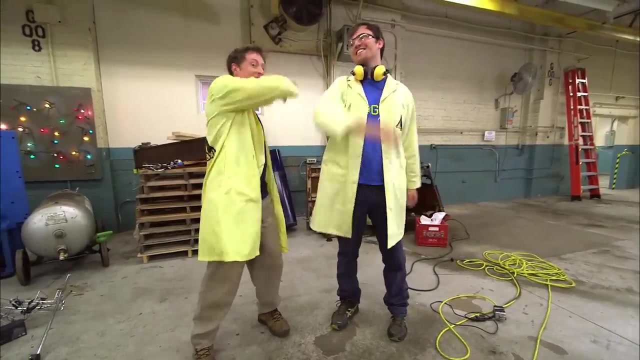 It lives up to its name. It vibrates all around the lab. Oh wow, My legs are numb to the knee. I'm not surprised. Vibrobot, All right, Yeah, that worked really well. That was awesome. I can't- I really can't feel my feet right now. 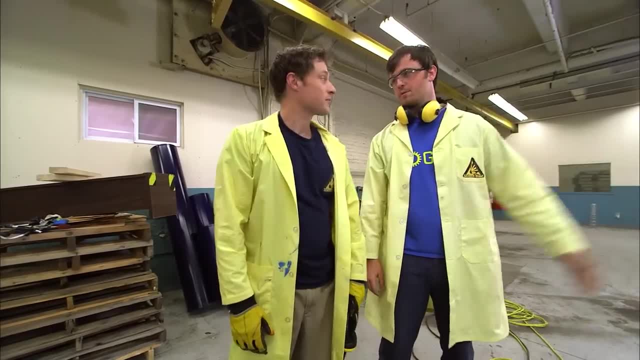 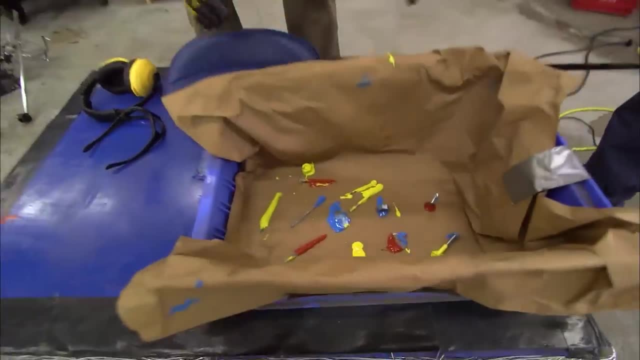 And it held together, which is impressive. That's right. The more power and the stronger structure paid off. Yeah, The only thing I regret is not getting a chance to Wait a minute. Wait a minute, Come with me. Okay, So I achieved my dream of riding the vibrobot. 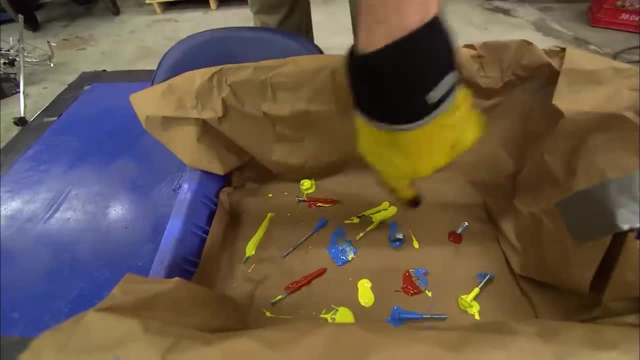 You did, But we never got a chance to make art. So we've dipped a whole bunch of nuts and bolts and heavy things in paint, Yeah, And now we're going to turn on the vibrobot and see if we can make some art. 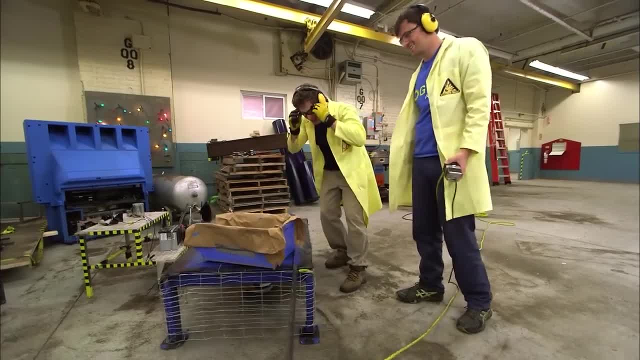 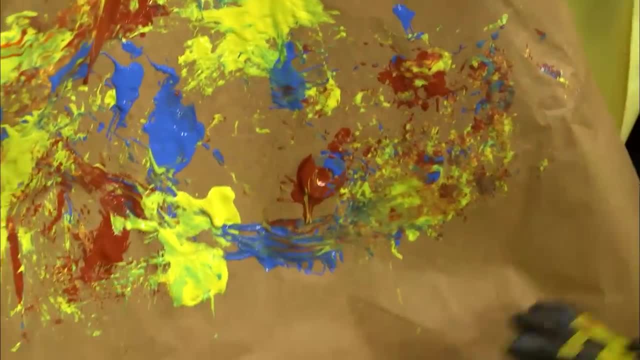 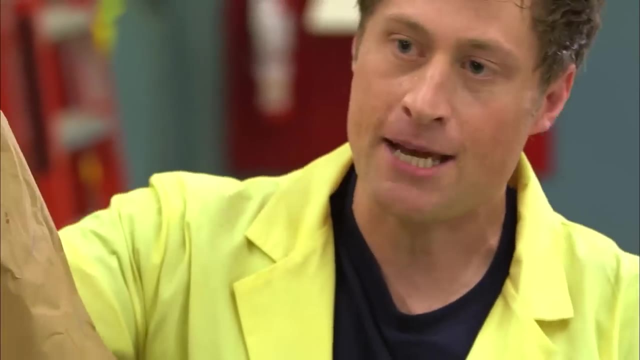 Let's see how it looks. Oh wow, Ta-da, Vibrobot art. Vibrobot has been a huge success and we've got some art to keep. High fives, Well done. Science max Experiments at large. Who gets to keep the art? 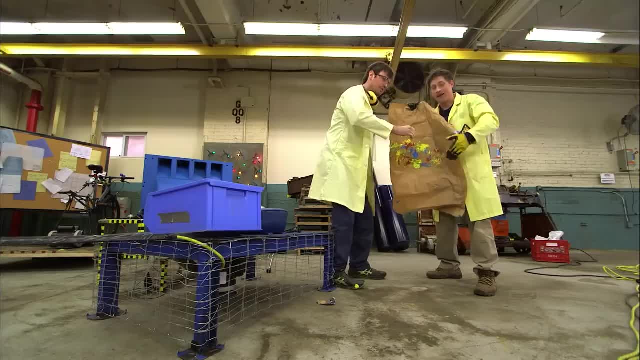 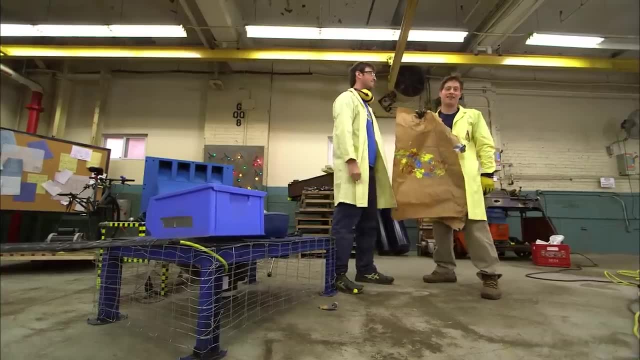 Rock paper scissors: Okay, One, two, three. Okay, Tie One, two, three. Tie One, two, three. One two, three. Wow, One two, three. Ah, tie One, two, three. 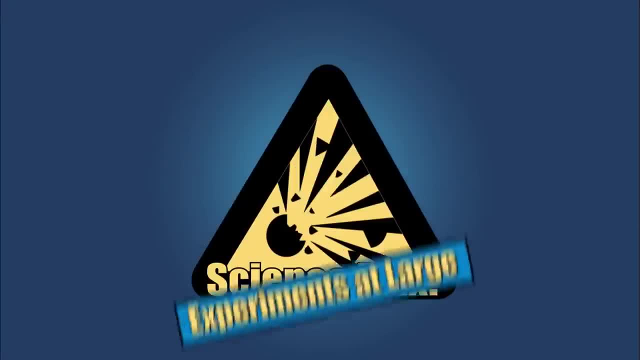 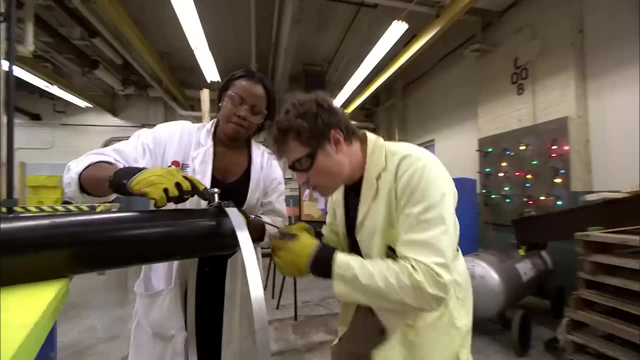 Man, Science, max, Gravity, Gravity, Gravity, Gravity makes things fall, But on this episode I'm doing everything I can to defy gravity. You win this one gravity: From a hoop glider to an egg, drop to a hover balloon. 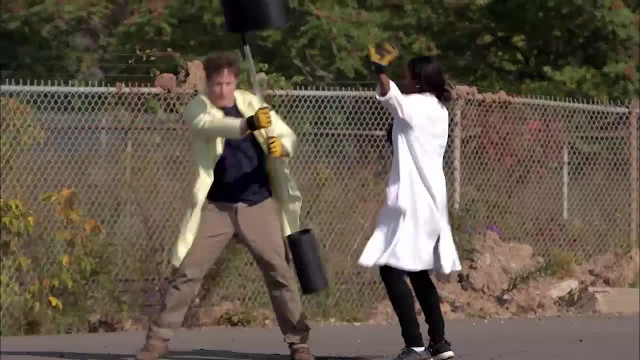 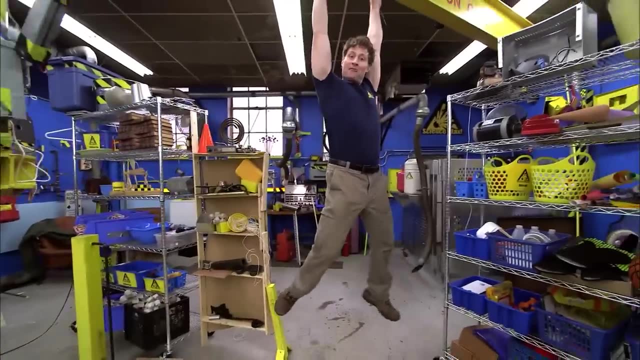 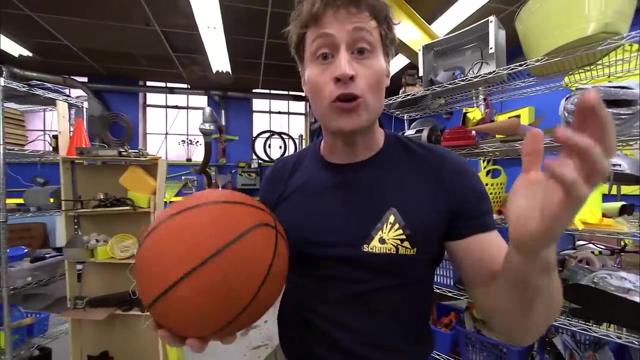 it's a gravity-defying dance party. All on this episode of Science Max Experiments at Large. Greetings Science Maximites. Welcome to Science Max Experiments at Large. My name is Phil And today on Science Max, we're going to be looking at gravity. 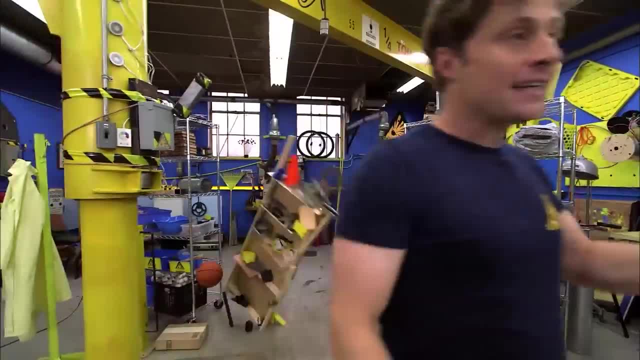 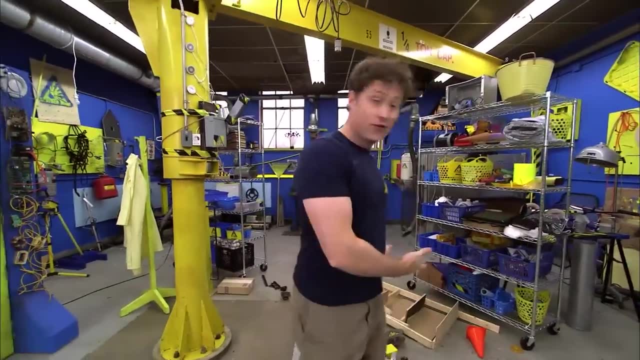 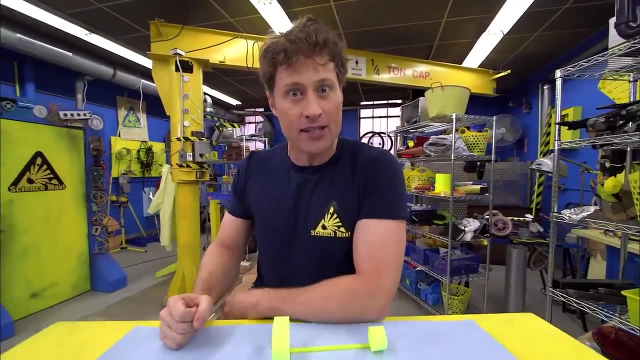 What goes up must come down. Today, Gravity is the force that makes things fall Towards the ground, But just because it's a force of nature doesn't mean that we have to listen to it. No, No Today on Science: Max Experiments at Large. 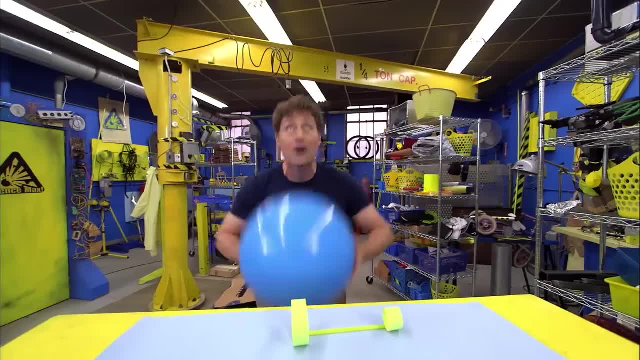 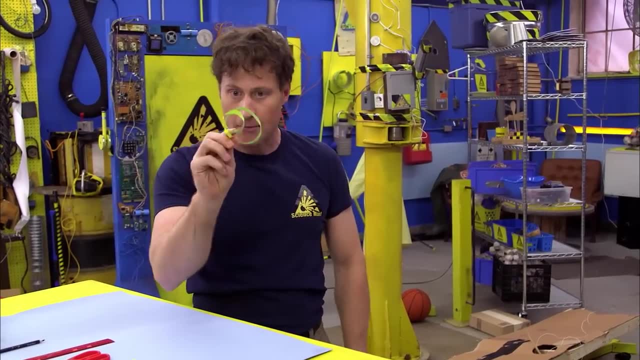 we're going to use everything in the power of science to defy gravity. Ha-ha, We are going to be making a hoop glider Now. hoop gliders may not look like much, but they fly just like paper airplanes, Woo-hoo. 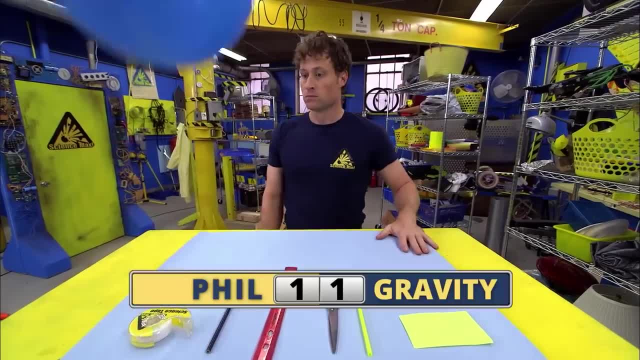 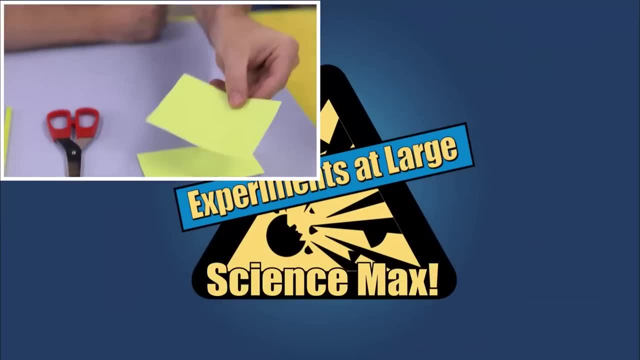 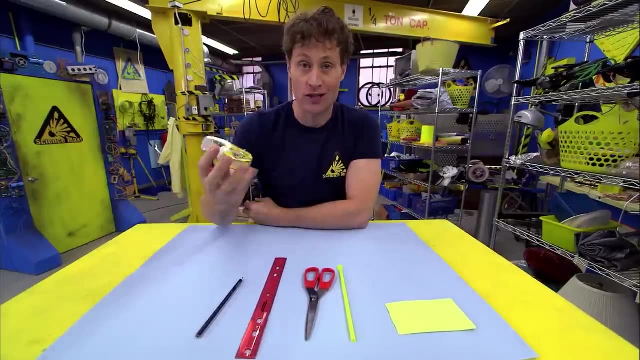 And here's how you can make a hoop glider. Here's how you can make a hoop glider all your own. This is what you need: Index cards, Scissors, Straw, Ruler Pencil And, of course, science tape, which is just like regular tape. 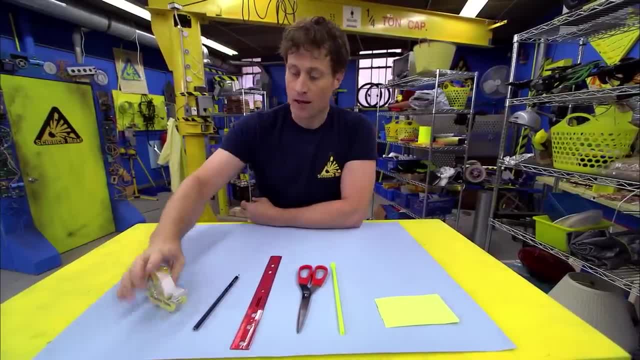 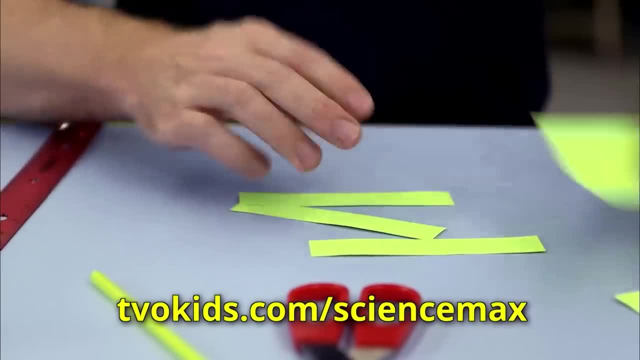 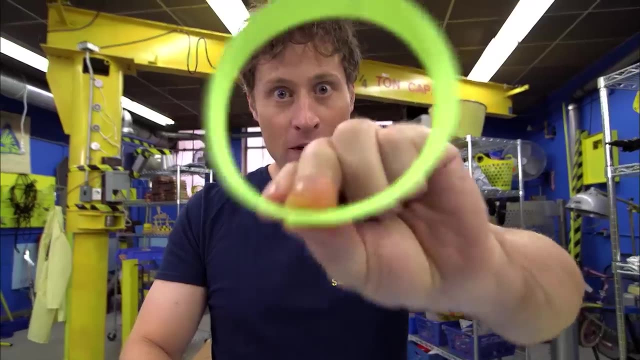 except you use this kind of tape for science. So here's how you do it: Take your index card and cut it into three equal lengths, Take two strips, and you take your science tape and you tape those two strips and make a hoop out of it. 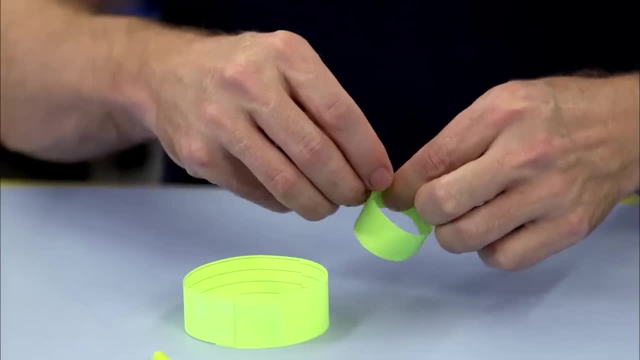 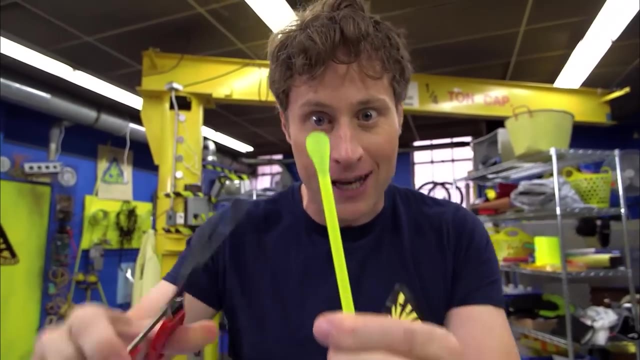 And with the small strip, you want to make another hoop. Now, what you want to do is take your straw. Now this is a little bit of a challenge. Now, this straw has a little scoop at the end and that's not very aerodynamic, so we're going to get rid of that. 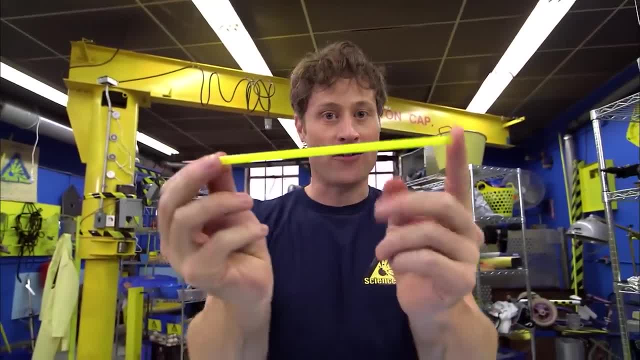 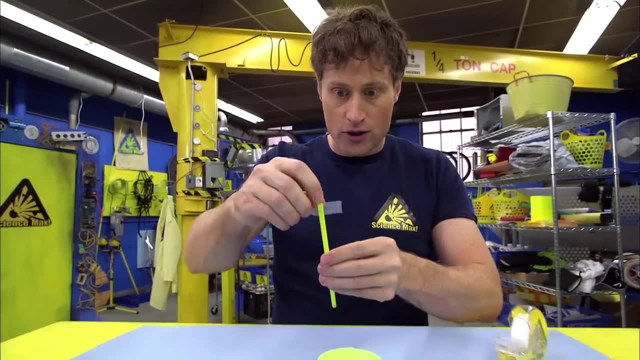 Ooh, Maybe it was kind of aerodynamic. All right, now that we've got the straw, you have to align the hoop and the straw together. So here's what I like to do: Take some science tape and stick it on the straw. 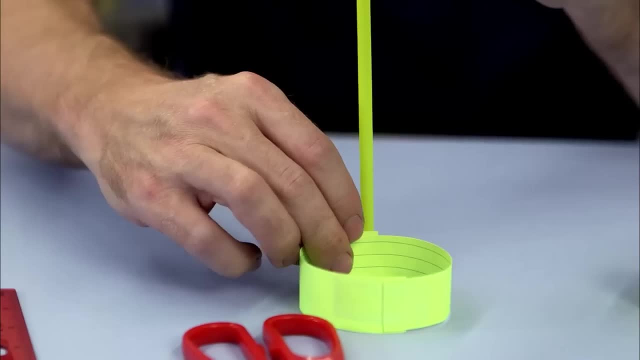 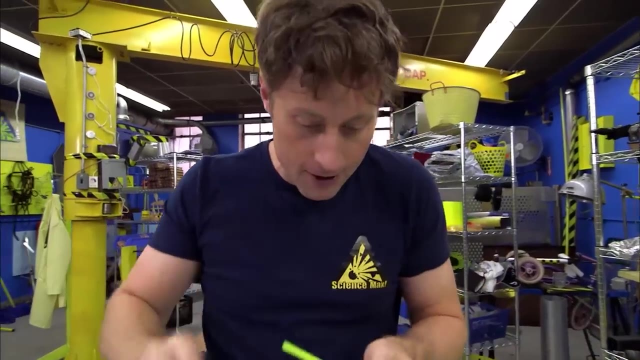 and then align it so that it's perfectly straight and then stick it on. Looks straight to me. All right. The small hoop also has to be perfectly aligned with the first hoop. So again, put the tape on the straw First, then align them up. 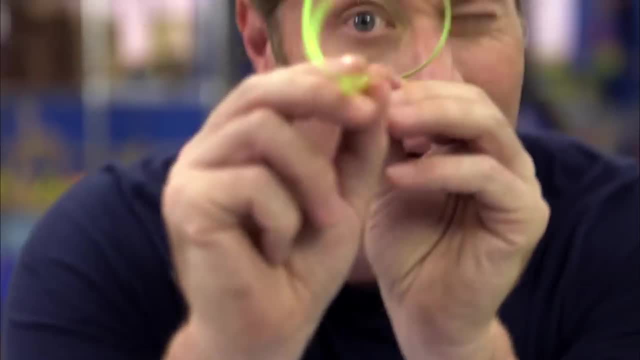 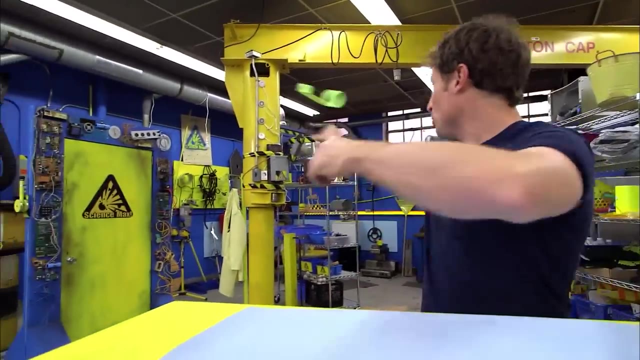 and then start looking down through it to make sure it's aligned There. Once you have it all taped together, you're done. You're a hoop glider and it flies just like a paper airplane- Pew, Awesome. So that's what we're going to do today. 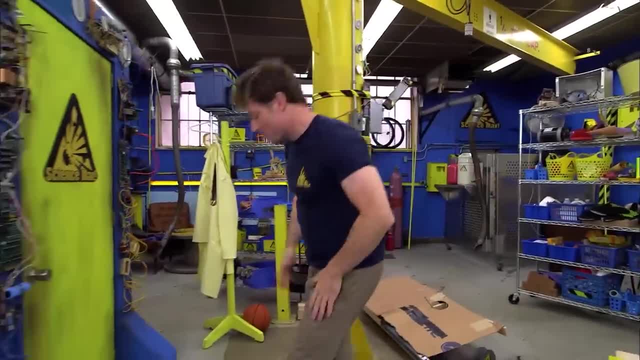 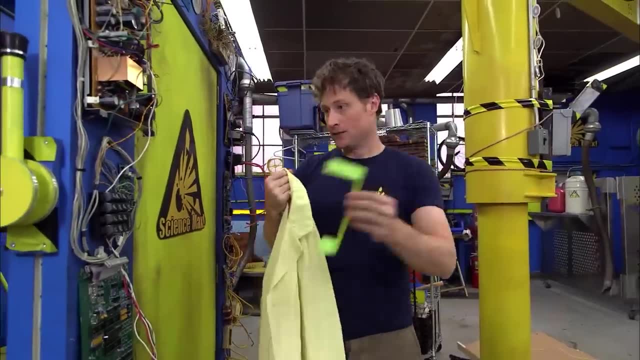 We're going to- Oh yeah, I've got to clean that up- We're going to max out the hoop glider. I'm going to go meet Sonia at the Ontario Science Centre and we are going to max out the hoop glider into a giant version. 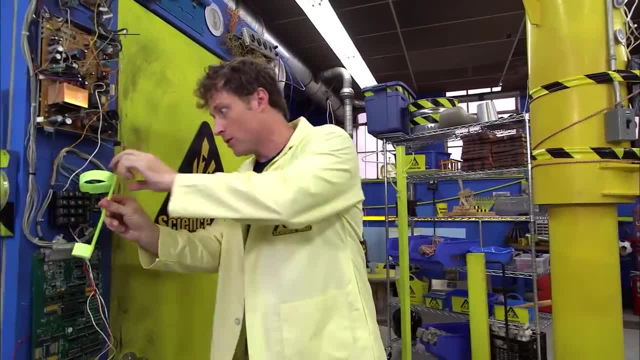 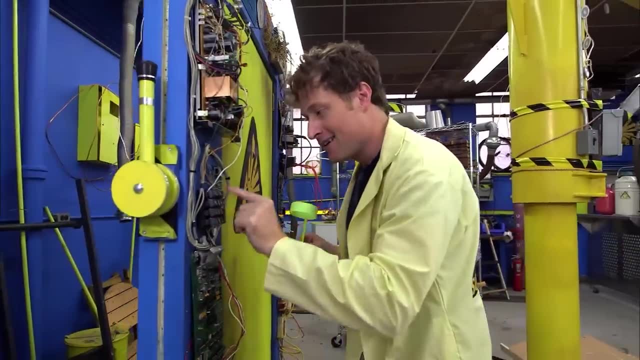 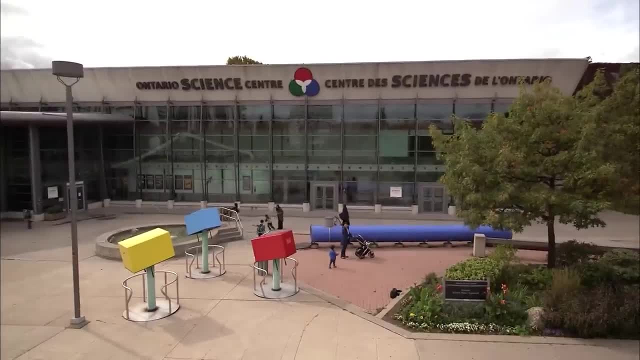 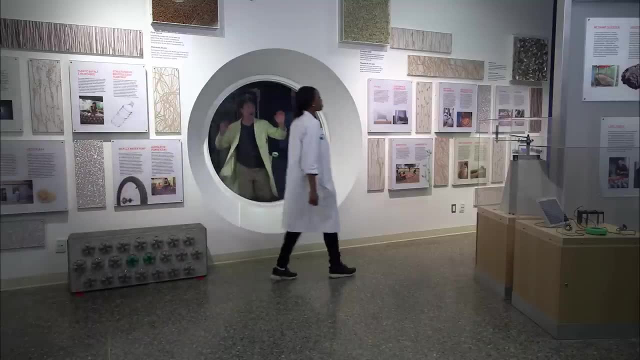 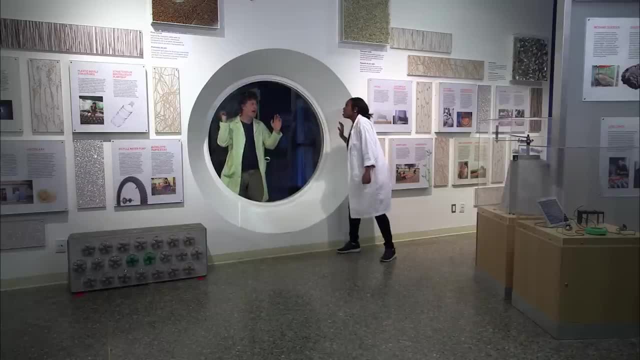 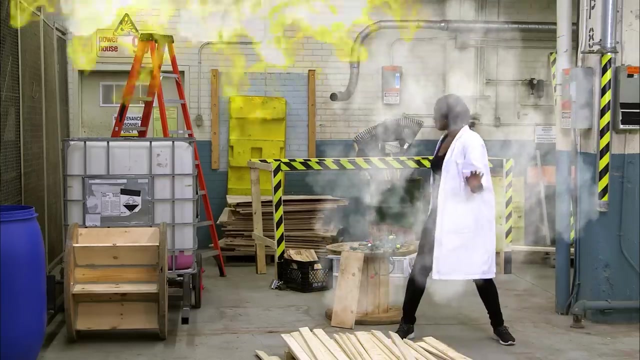 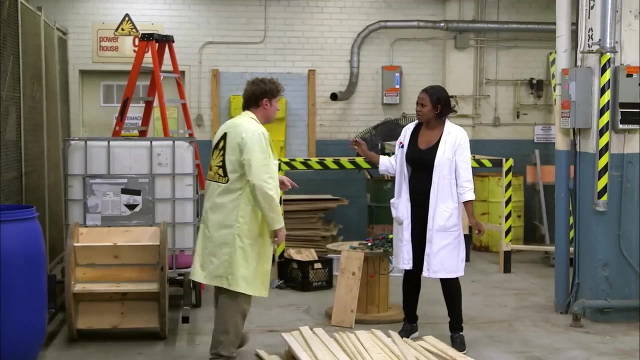 Pardon, You want me to help you with an experiment. Okay, All right. Ha-ha, Oh, Sonia, I came in. You came in here, Are you okay? Are you okay? Yeah, I'm fine, Come on, let me show you. 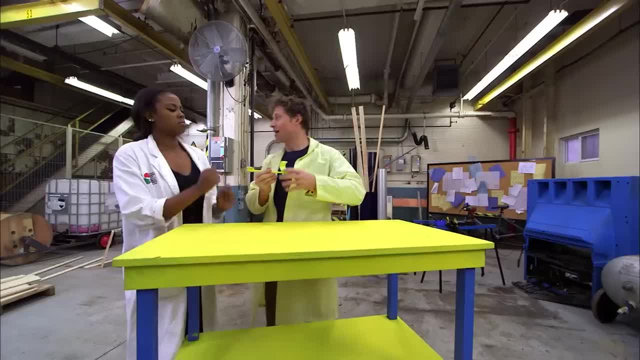 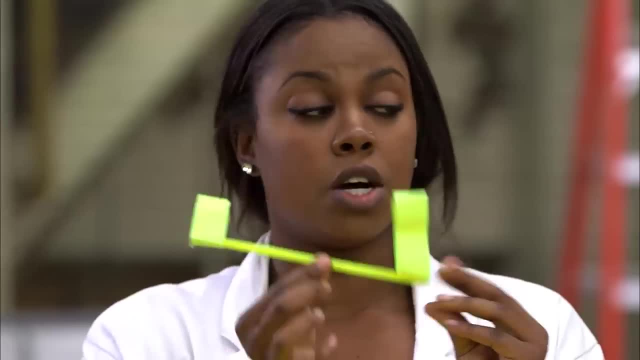 This is what I would like to max out. It was in my pocket when I fell, so What is that? It's a hoop glider. It was a hoop glider. So how do we max this out? First, we're going to need a larger tube. 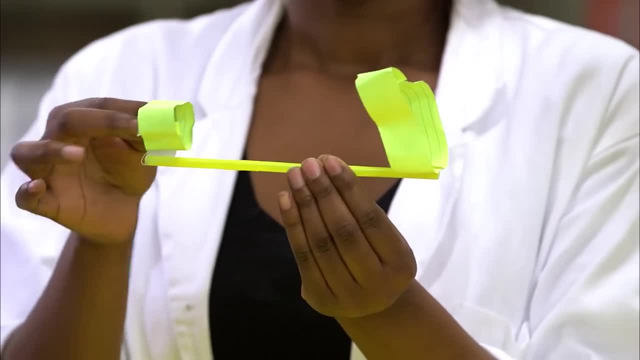 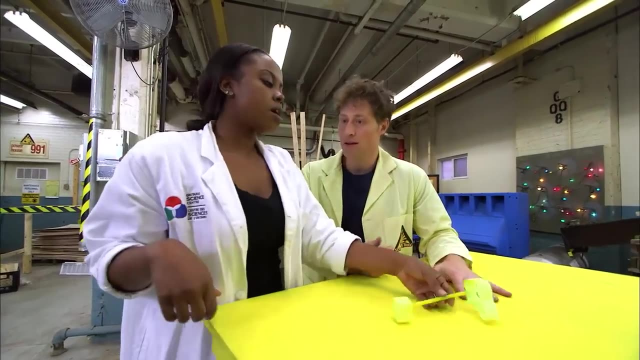 To replace the straw. yeah, Exactly, and we're going to need two hoops. We need something that's flexible, that will convert into a hoop. Okay, that's great, So why don't we get started? Sounds good, All right, high fives. 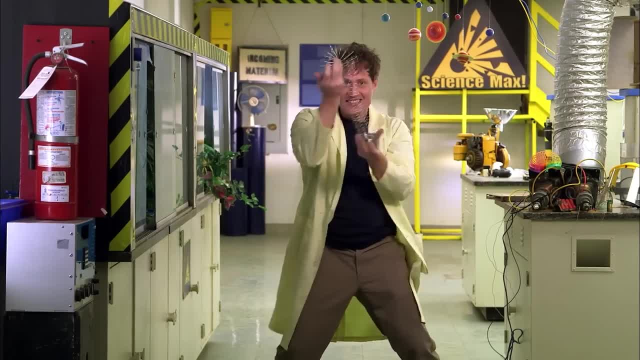 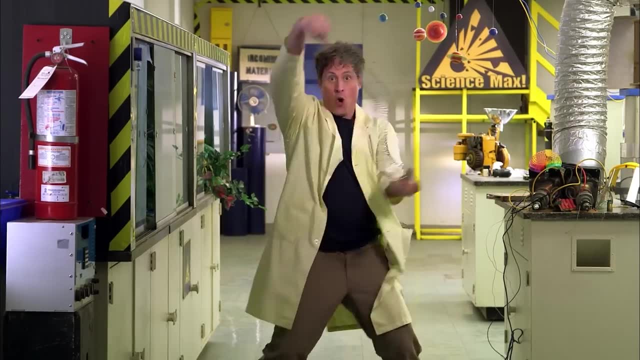 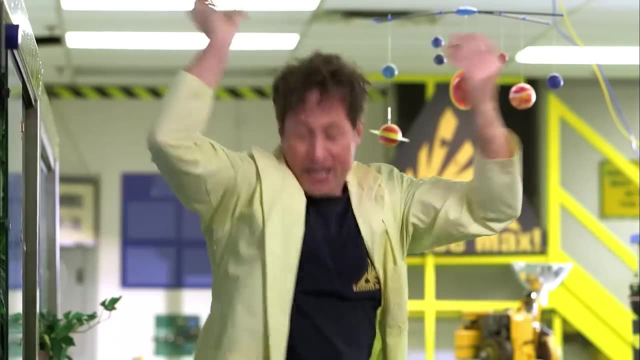 You may recognize this: It is a spring. Yes, good for you. But did you know that springs can defy gravity? Whoa Gravity defy. What Gravity defy, Gravity defy. Look at it fly Defying. Okay, not exactly. 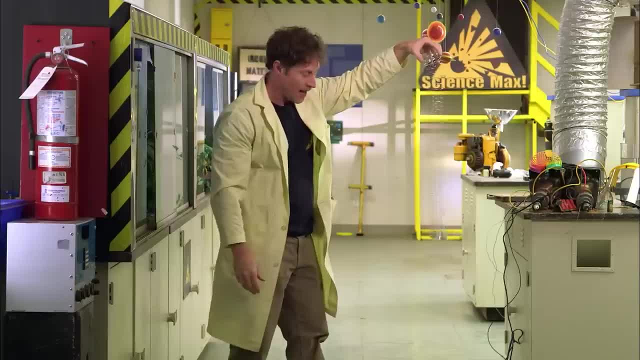 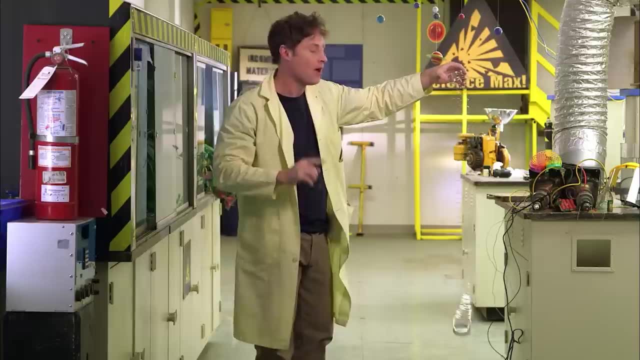 But what if I was to hold the spring like this and let it go? What'll happen? It'll fall. Yes, it'll fall, That is true. But while it's falling, what happens to this end? Does it stay in one place? 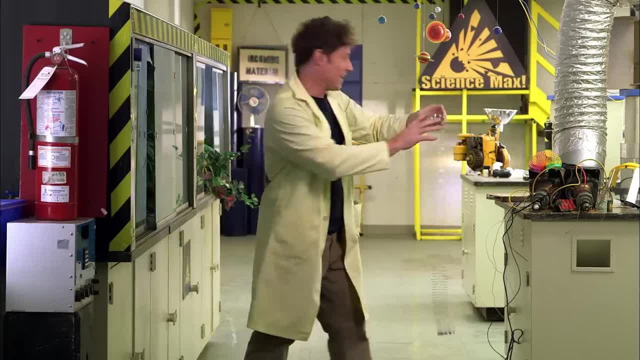 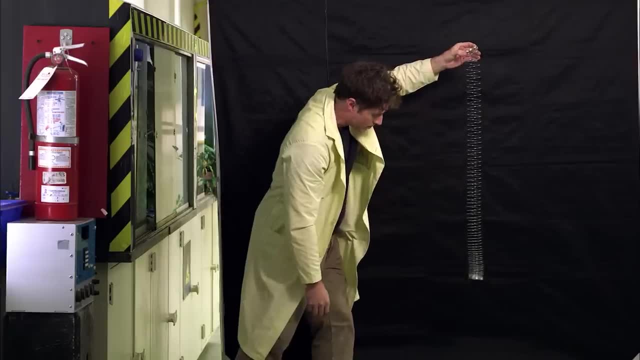 Does it go up or does it go down? Let's find out. I'll bring this in so you can really see it. Okay, ready, Watch close. Did you see? No, Okay, tell you what. Watch it again, this time in slow motion. 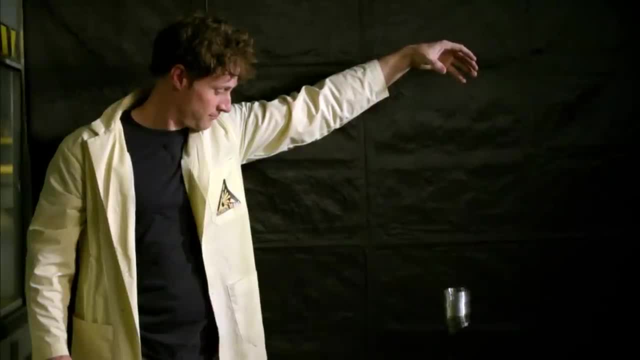 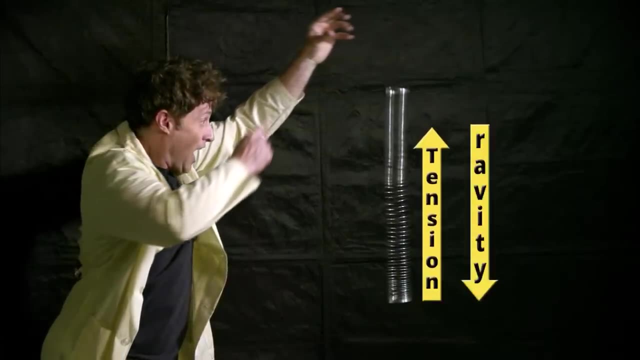 See, The bottom doesn't move, And here's why, When the top of the spring is released, gravity and the tension of the spring are pulling on it. The bottom of the spring is being pulled down by gravity and up by the tension of the spring. 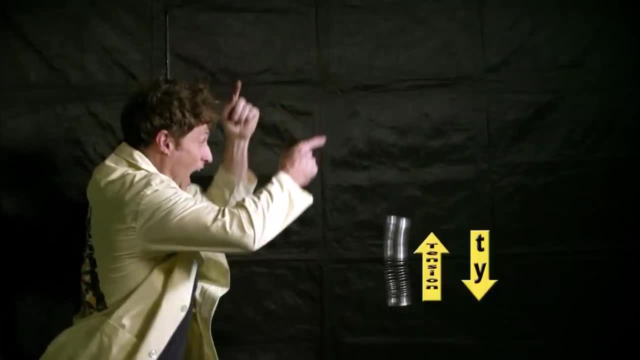 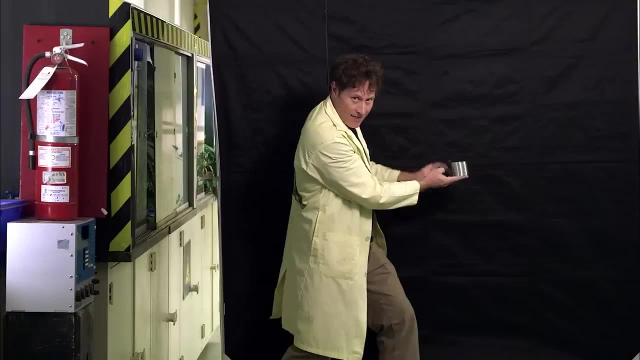 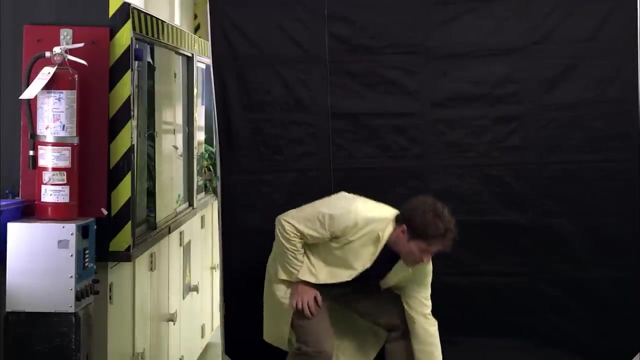 These forces cancel out, stopping the bottom of the spring from falling until the top reaches it, Until there's no more tension, and then the top passes the bottom and the whole thing. That is how it works. But here is the real question: Will it happen differently with a longer spring? 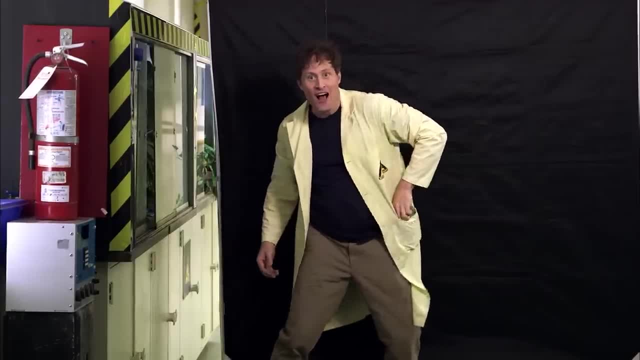 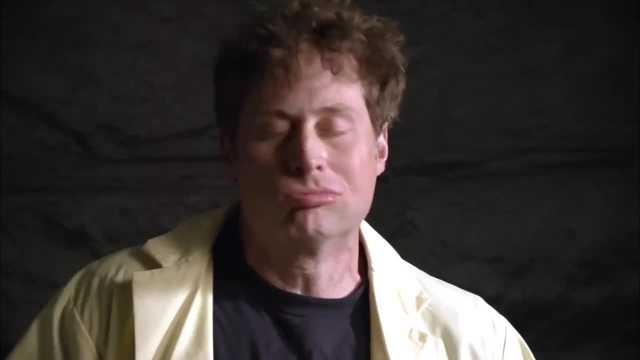 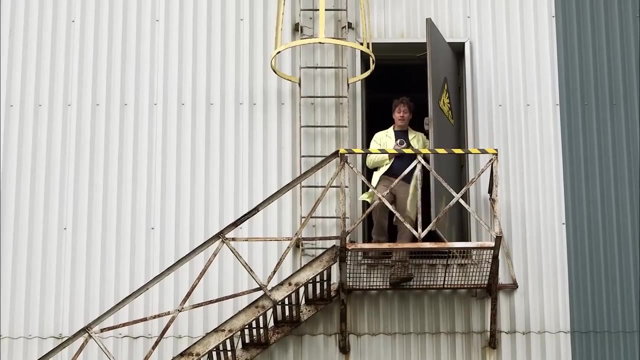 Huh Well, I just happen to have a longer spring. Let's not waste time. Let's find out, Let's max it out, Bring it, Don't tangle it. So now that I'm up high on this fire escape, 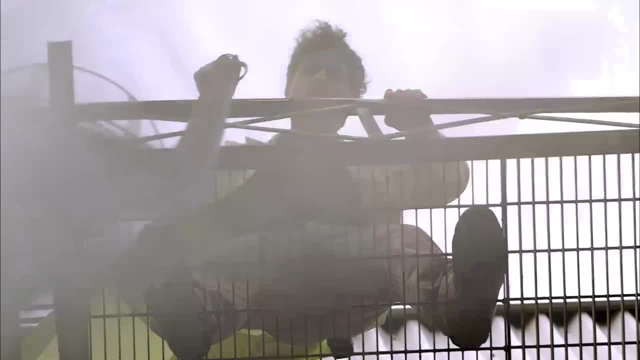 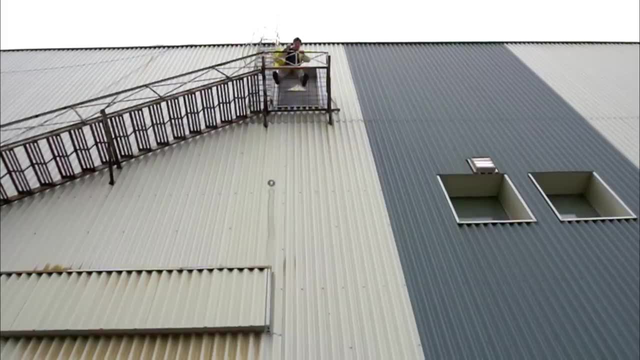 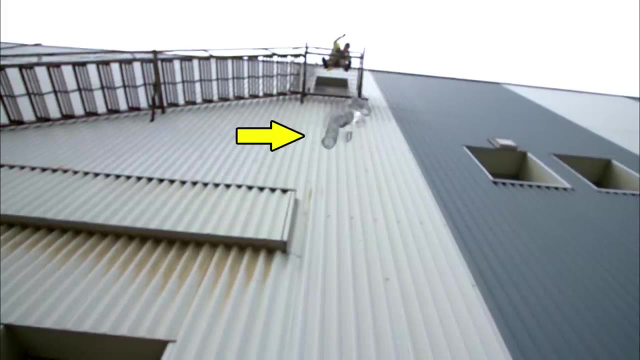 let's test it out. Okay, Three, two, one go A longer. spring still has the same forces working on it: The tension of the spring pulling it up and gravity pulling it down. No matter what size of spring, these forces cancel out for the bottom of the spring. 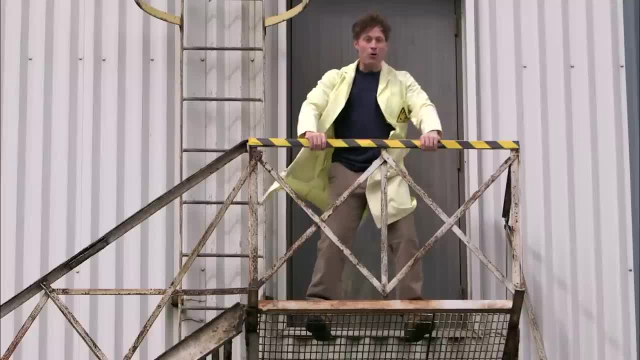 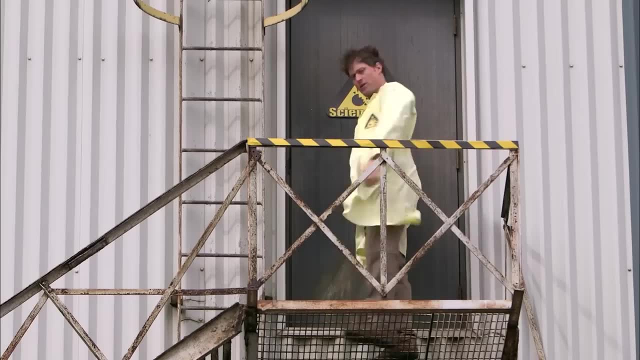 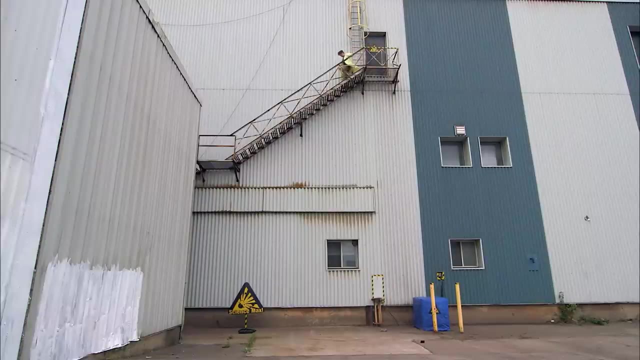 until the top meets up with it. So there you go, An almost gravity-defying spring, Ha-ha. Uh, hey, There's no door handle on this door. I guess I have to take the stairs. Whoa, Sonya and I are maxing out the hoop glider. 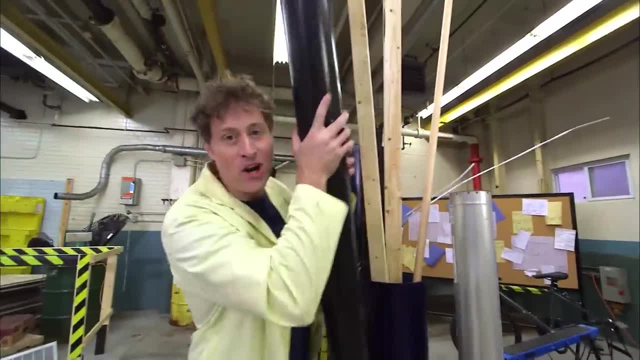 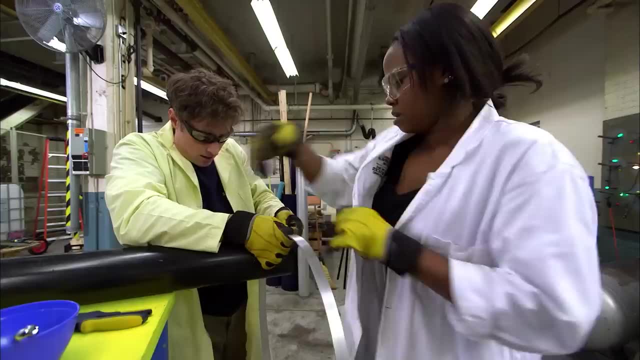 out of bigger and better materials. This is the largest tube I have, Right, A giant ABS pipe and some bendable metal to make into hoops. Then we attach them all together and, Okay, big hoop is done And little hoop is also done. 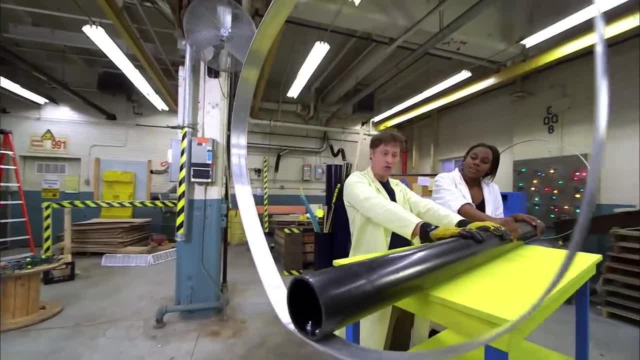 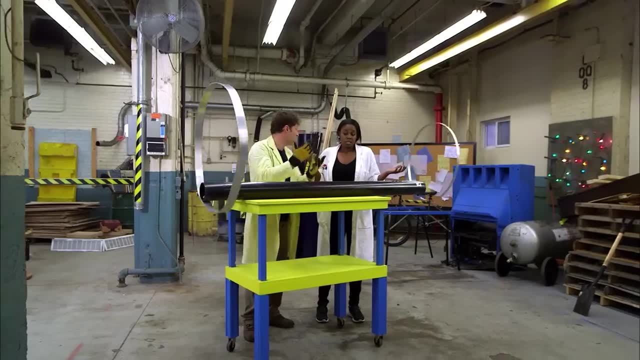 Awesome, Not bad, Not bad at all. Super solid, And that's the thing. We have pretty heavy material, so it might not fly as well as we'd like, But something heavy can always be good, right? Oh no. 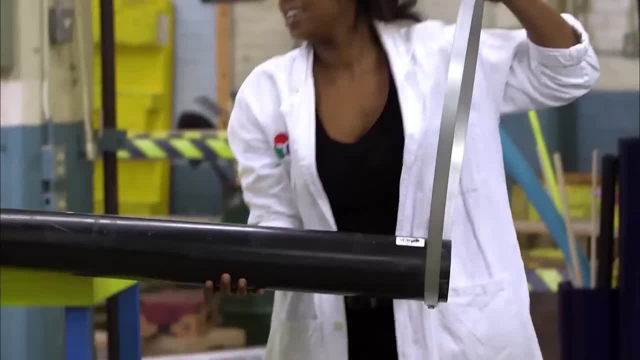 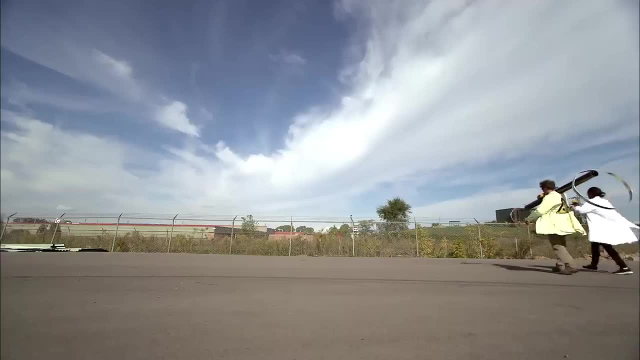 That's what I'm talking about. See how solid it is. It's pretty solid, No damage whatsoever. You want to test it? I think we should. Okay, I'm excited We take our plastic and metal hoop glider outside to test it and 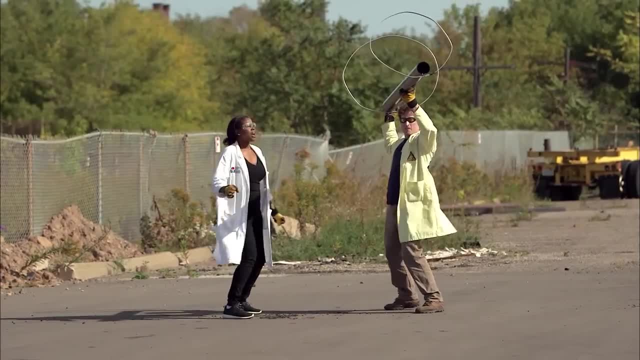 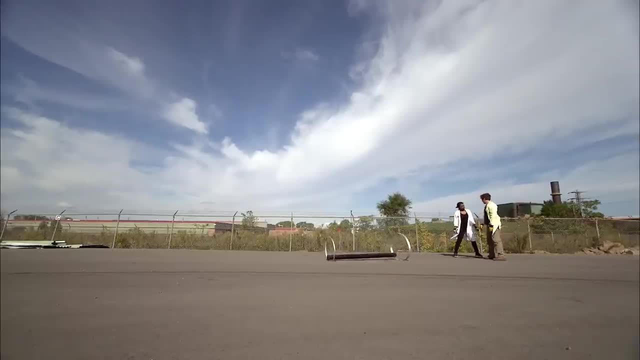 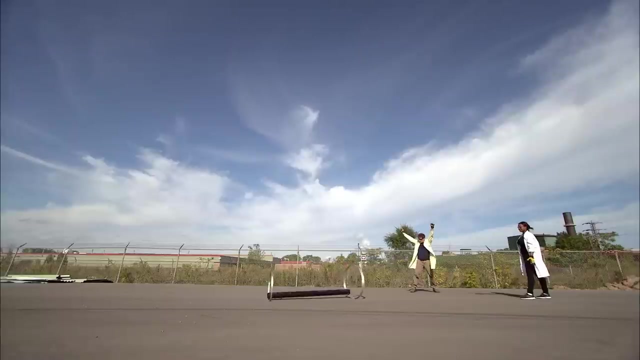 Ready, Ready. One, Two, Three, Huh, It didn't really fly, did it? Sonya and I have been trying to figure out what's going on. Sonya and I made a very solid design, but the problem with it became pretty obvious. 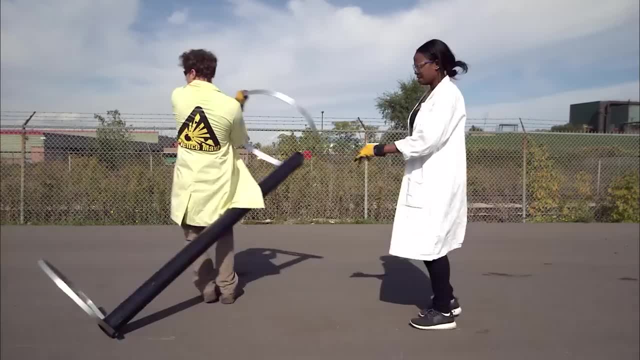 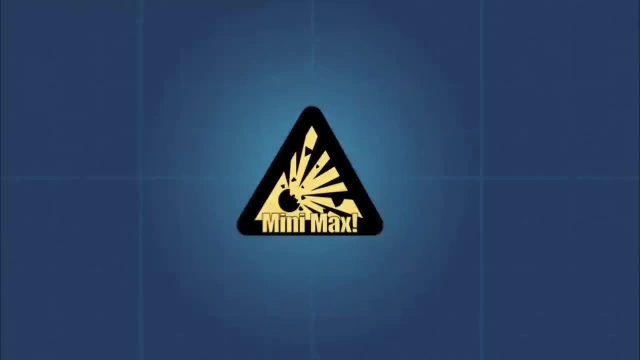 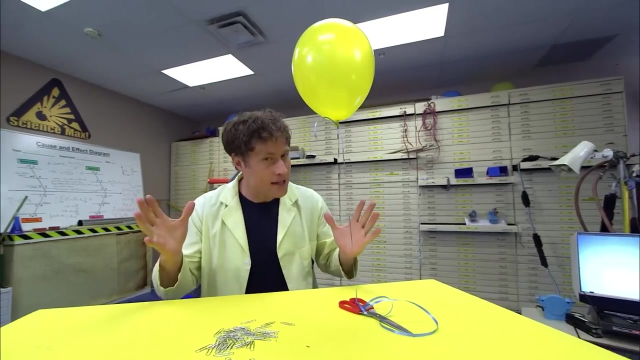 Yeah, It's just too heavy. Well, that's what science is. Back to the drawing board. Here's something fun you can do if you ever get your hands on a helium balloon. Now, helium balloons float up, not because they defy gravity. 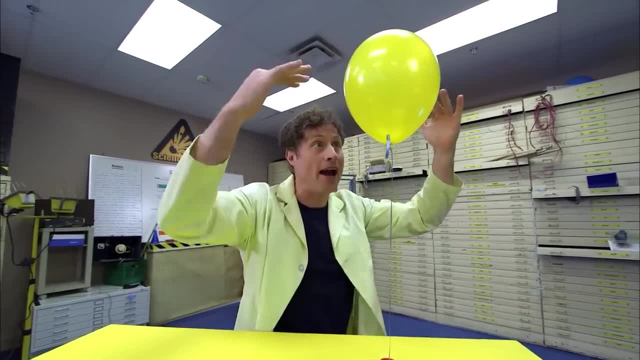 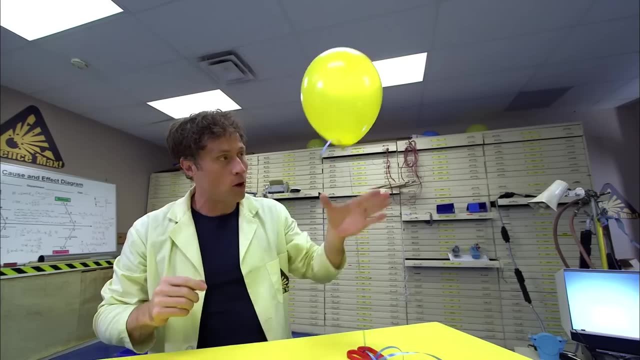 but because they're lighter than air, It's because the heavier air around it actually falls past the balloon, and that ends up pushing the balloon up. But what if this helium balloon wasn't lighter than air or heavier than air? It was exactly the same. 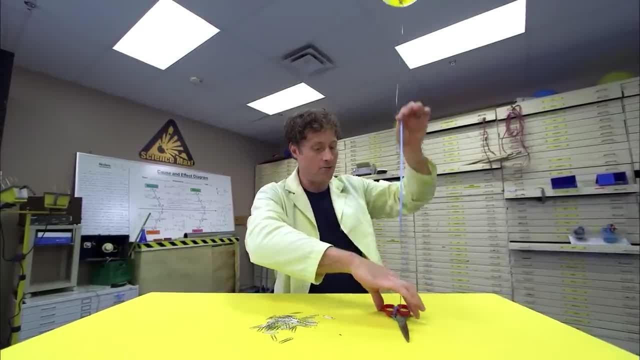 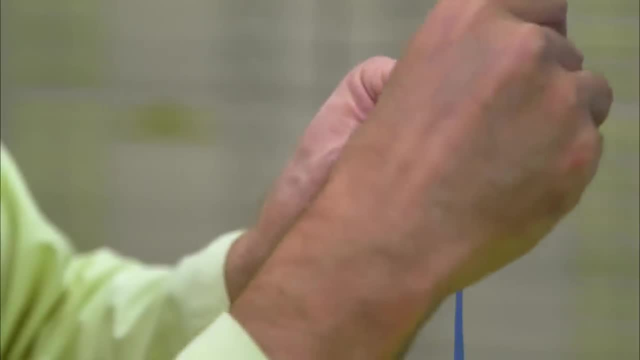 This is what I like to do. Just take a helium balloon with a long ribbon and a bunch of paper clips and adding a little bit of weight every time, And what we want to do is make this balloon neutrally buoyant. That means it won't go up or down. 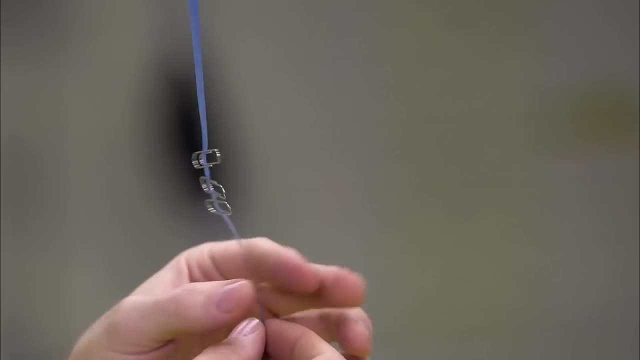 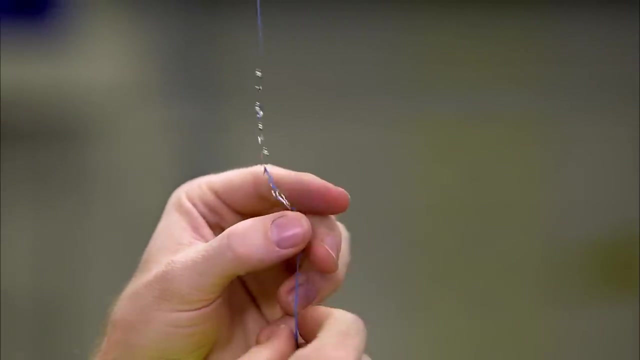 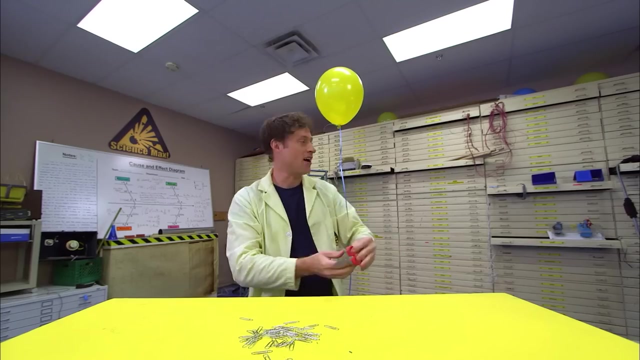 but it will be neutral. You want to check it every once in a while. Let's see, three paper clips is clearly not enough. Five paper clips is Ooh. five paper clips is pretty close. It still might float down. So you want to take off just a little bit of weight. 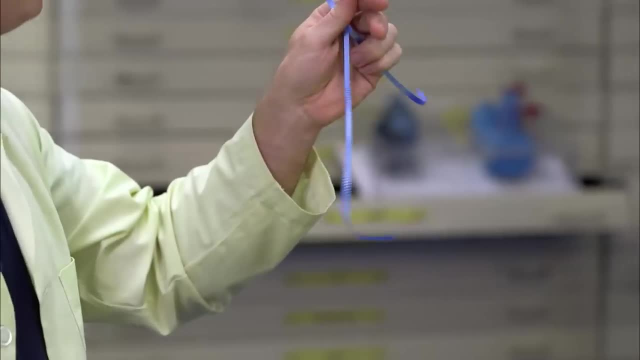 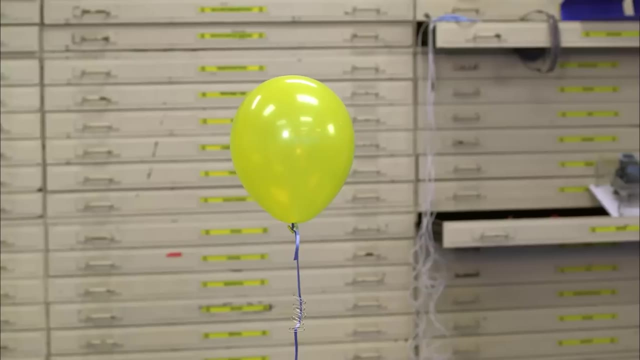 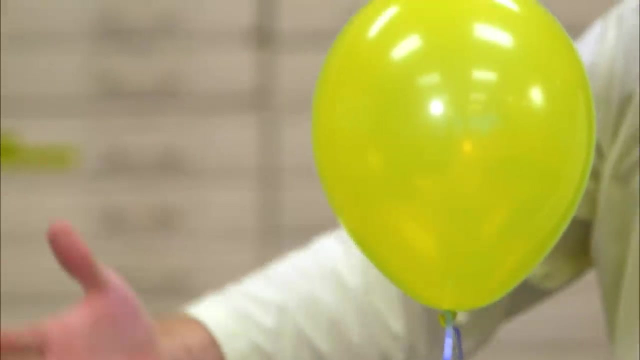 maybe about there? Watch this: You just take the balloon and you put it somewhere and it stays. It stays put. It doesn't go up, It doesn't go down, It's attached to nothing. Now let's max it out. 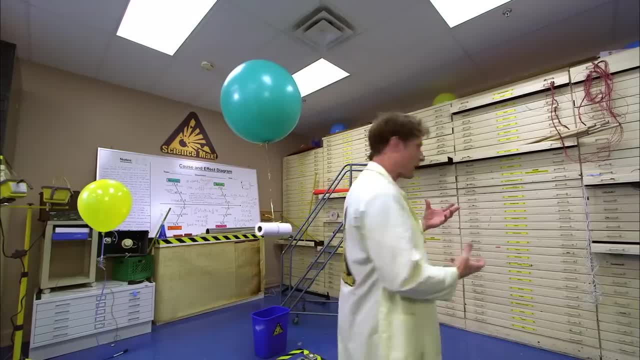 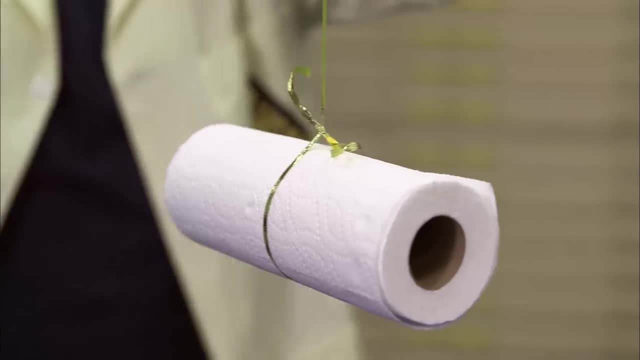 Huh, I had a big balloon and it was a. It had a. Oh There, Ha ha, ha, ha ha. A giant balloon And look, it's a great paper towel delivery device. Say, did you want some paper towel? 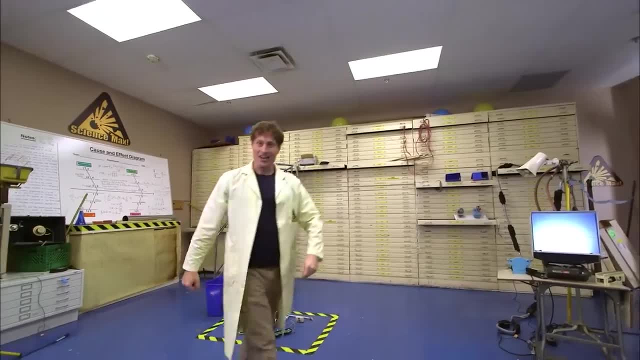 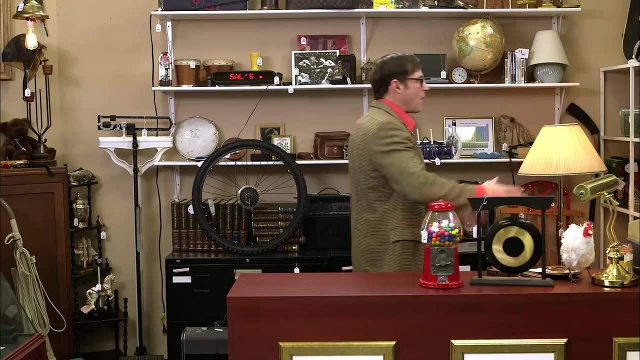 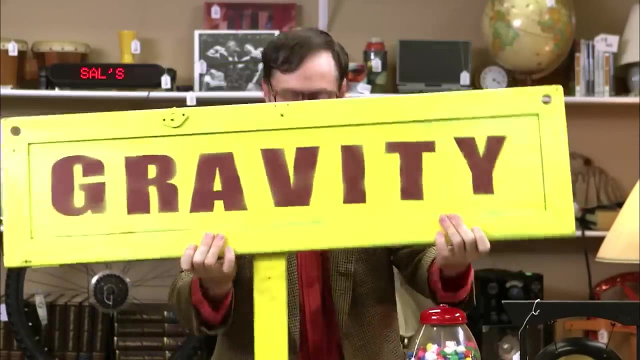 Here you go, Science. Yeah, don't worry about it, Ramona, Just put them up high. Put them up, Yeah, higher. Good, Hey, Gravity, Gravity, Huh, Gravity makes things fall, But where do they fall? 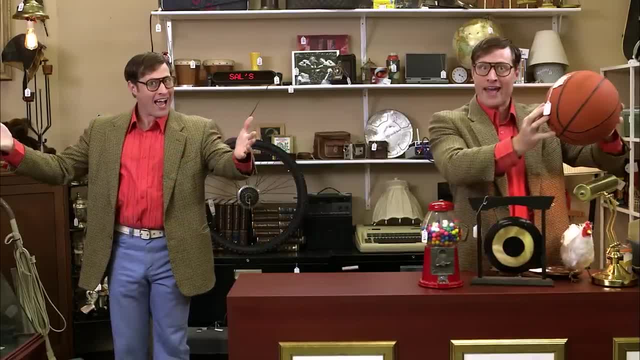 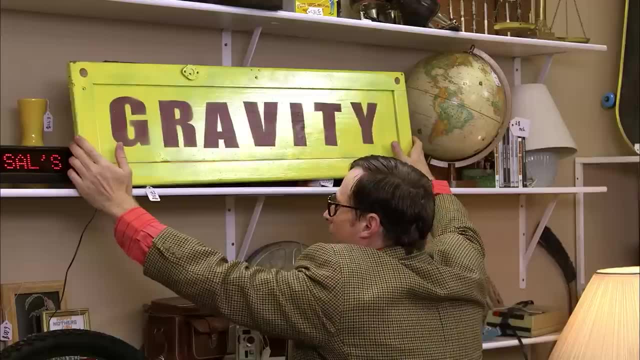 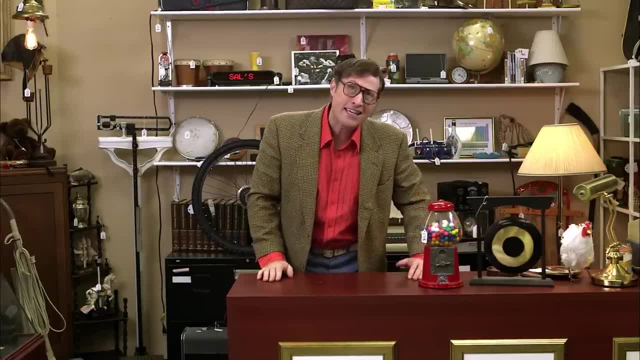 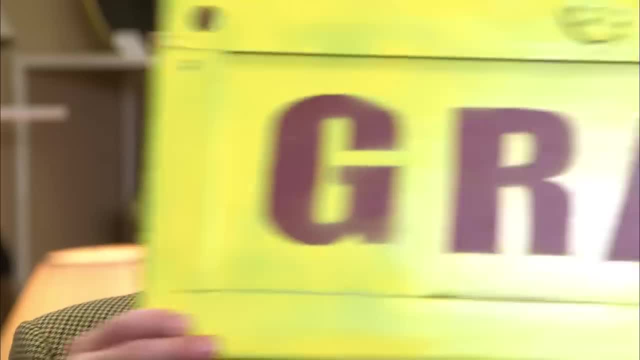 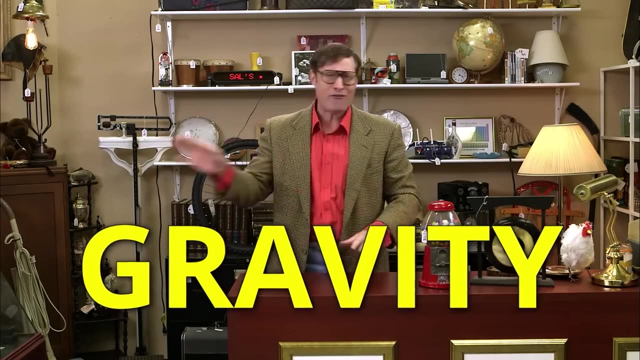 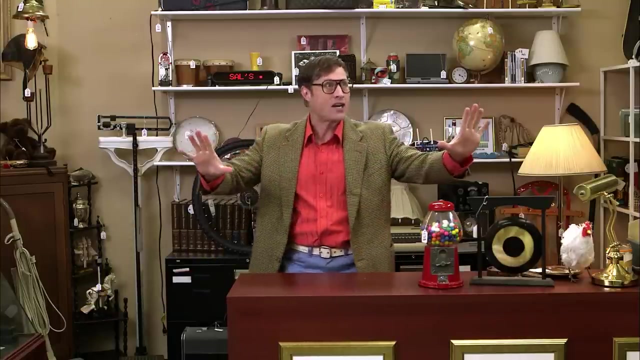 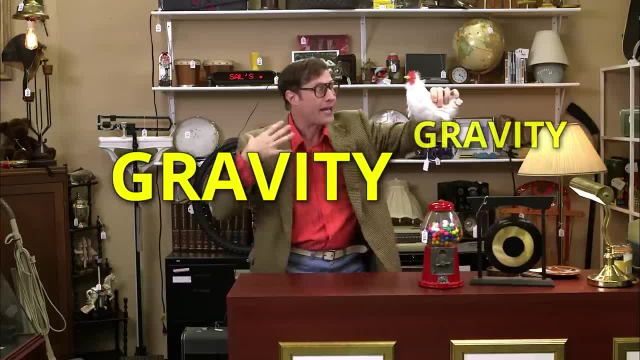 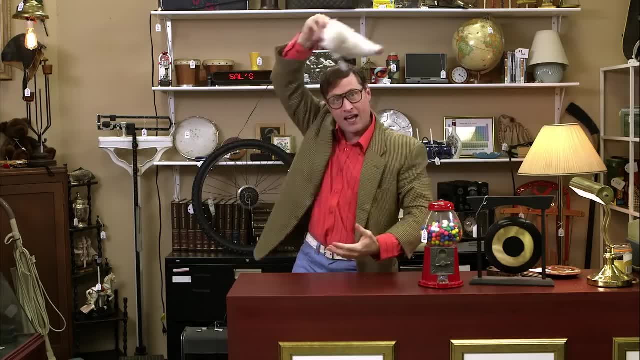 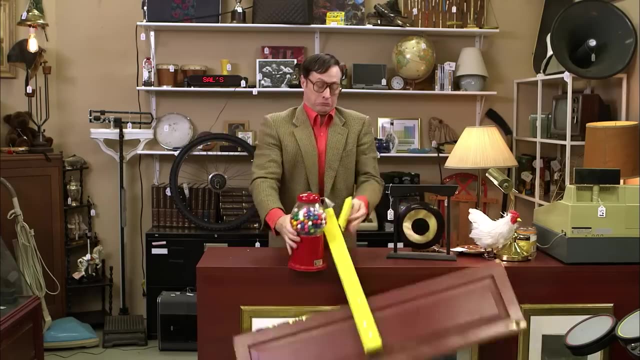 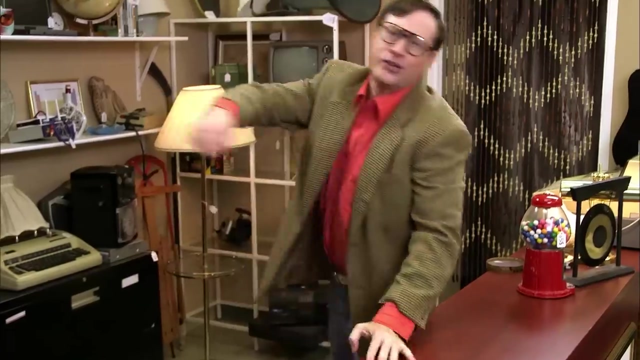 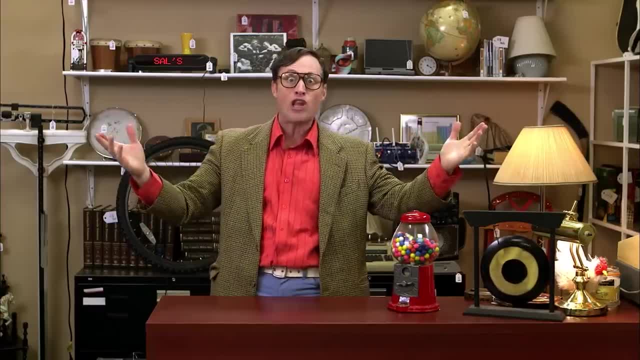 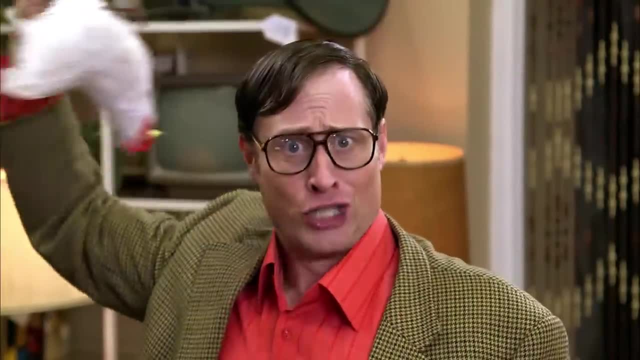 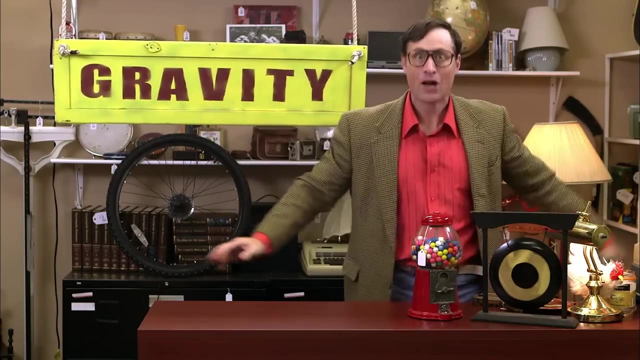 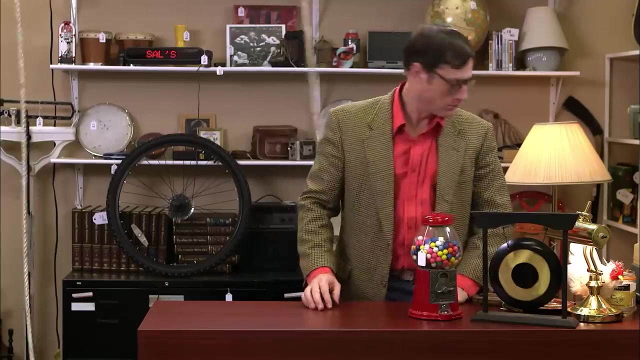 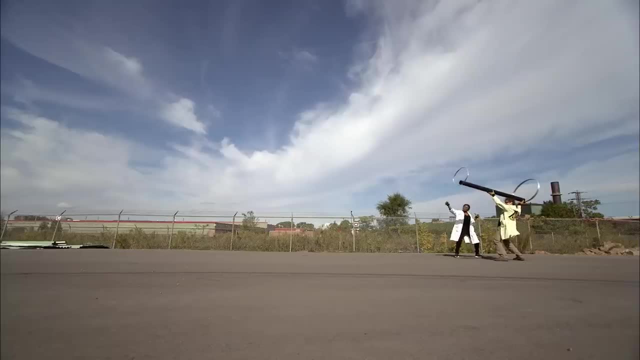 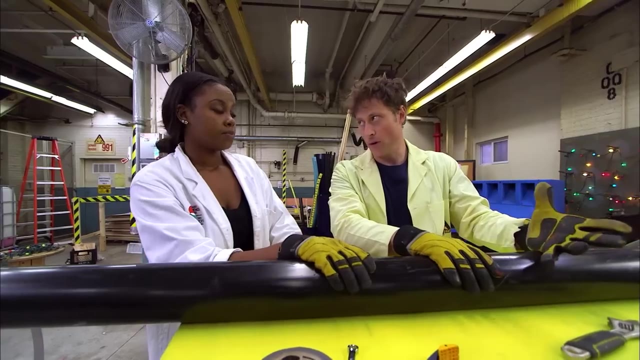 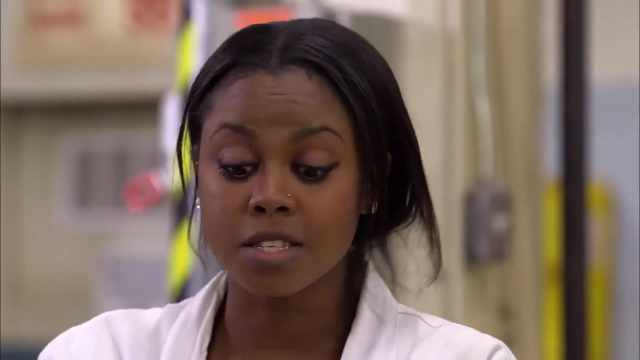 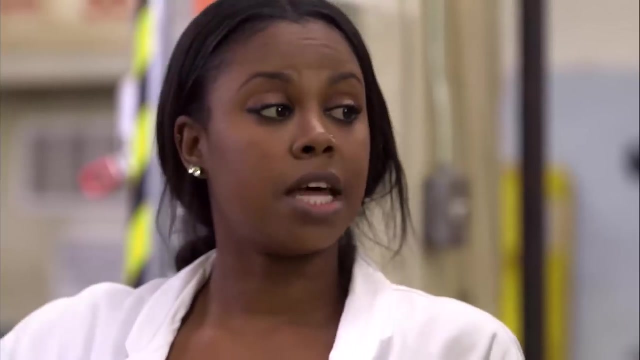 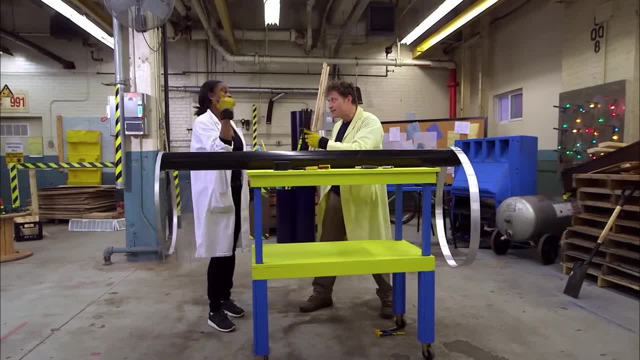 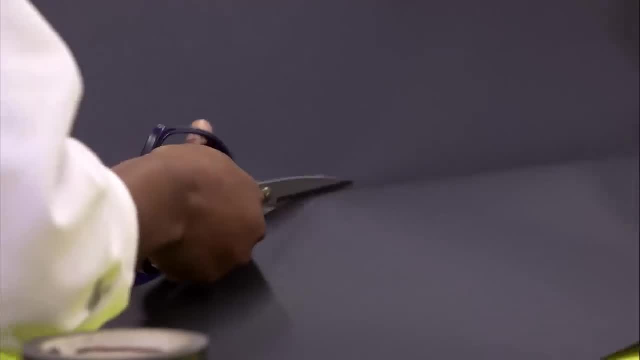 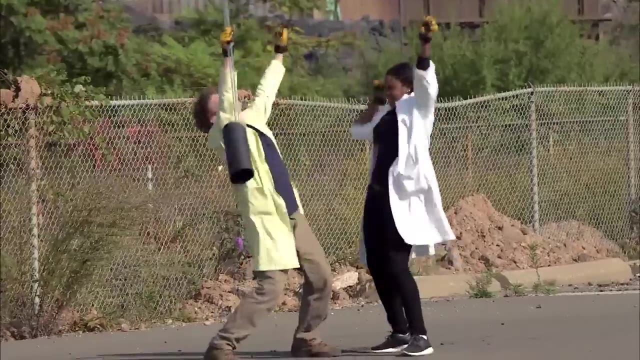 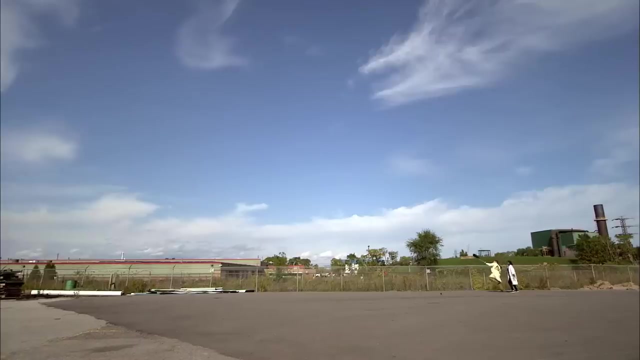 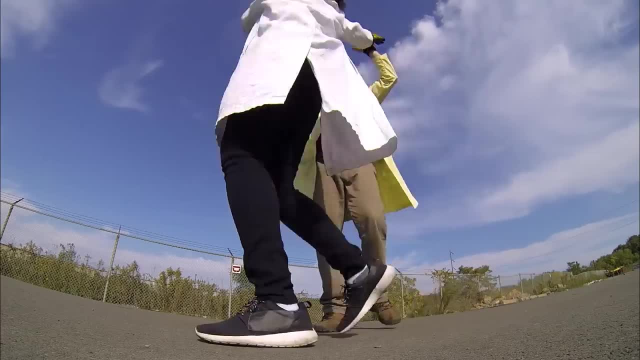 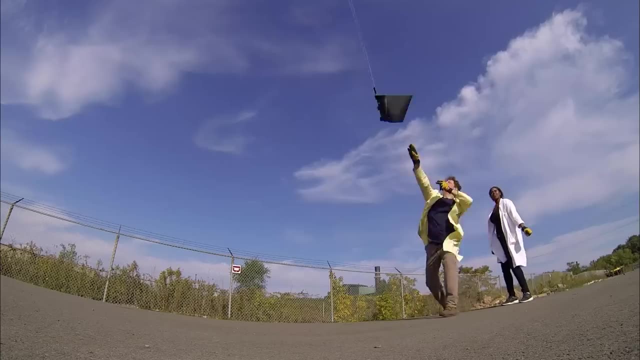 Yeah, Woo-hoo, That's pretty good. That was amazing, Pretty good. Let's try that again. Here we go, I throw the hoop glider and although it doesn't keep flying forever, it goes much further than our first version. 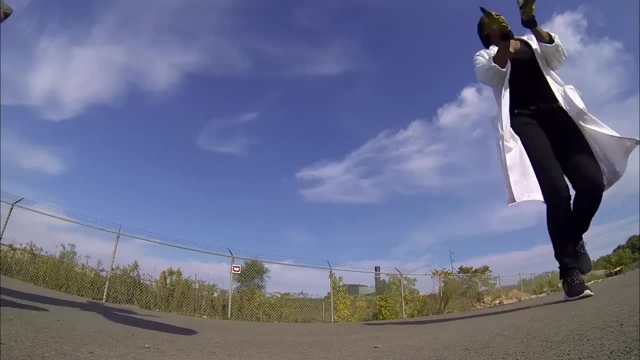 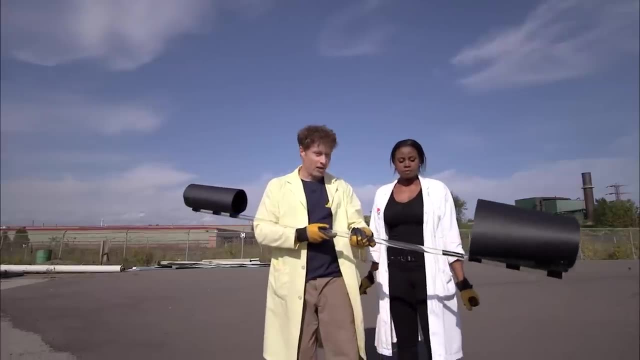 and also further than I could have just thrown the pipe by itself. That's pretty good. So we've done a good job of making something that flies. Why don't we make a couple different kinds out of different materials and we'll see if we can get one? 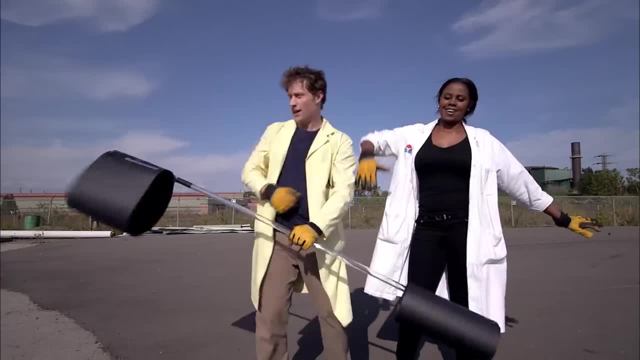 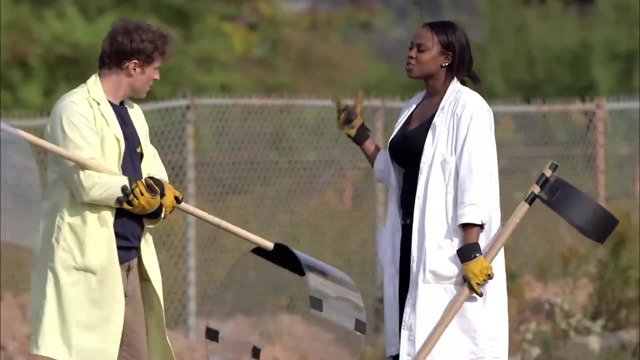 that flies even better than this. I think that's a good idea. Yeah, okay, let's do it. Sonia and I have created a pretty good maxed out hoop glider, but we wanted to see if different materials would make an even better one. 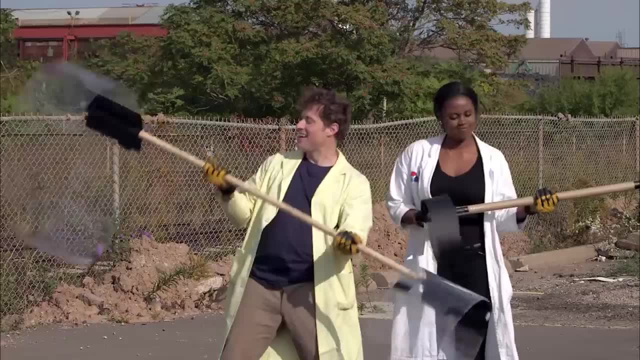 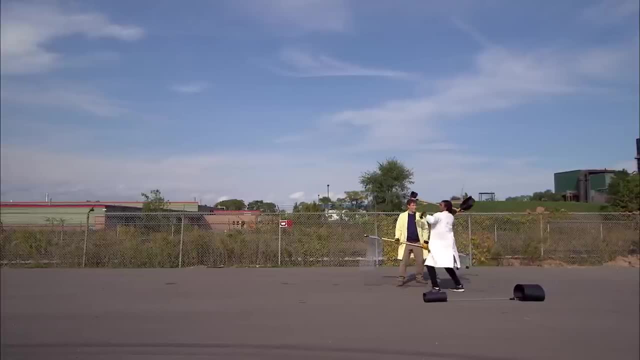 Sonia made a much lighter version. This time I used cardboard And I- I made this- Made a slightly heavier one. Let's do it. Okay. Three, two, one go. Not bad, My turn. Here we go. 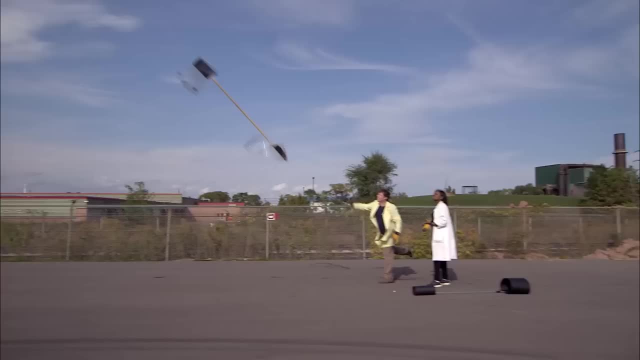 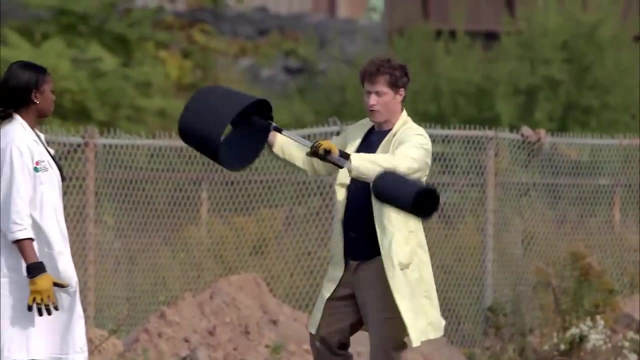 Okay, That didn't really go very far at all, did it? No, Okay, so now we can measure it against the one that we threw before, And that went pretty far. This went pretty far to see if we've got a better design here. 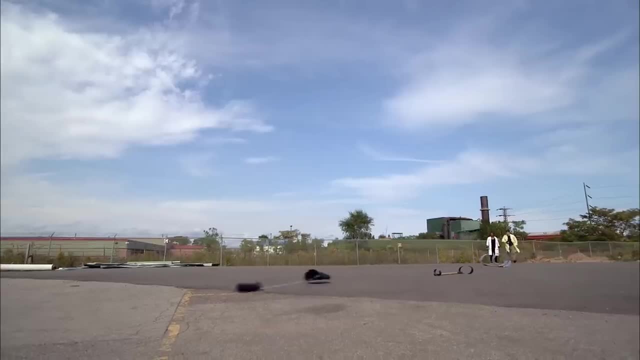 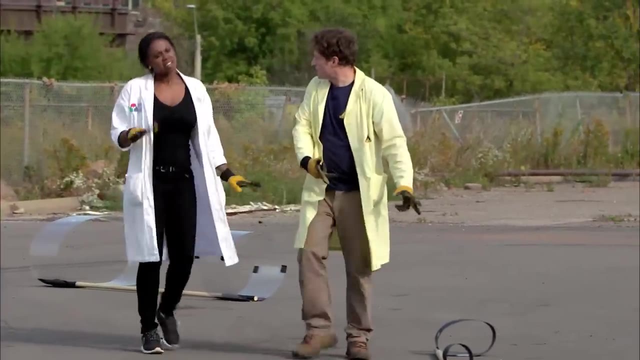 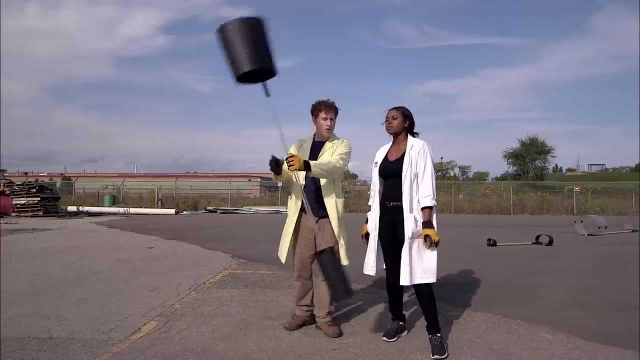 Here we go, Ready, Wow, Awesome. So heavy one no. Light one no, Interesting, Uh no, This design seems to be the best one. I keep thinking about how you were talking about thrust, Yep, All the thrust that we can put in. 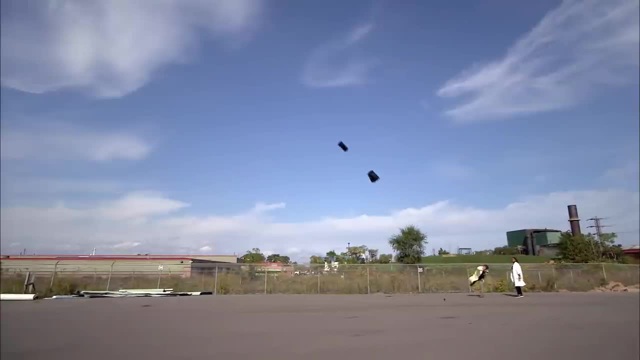 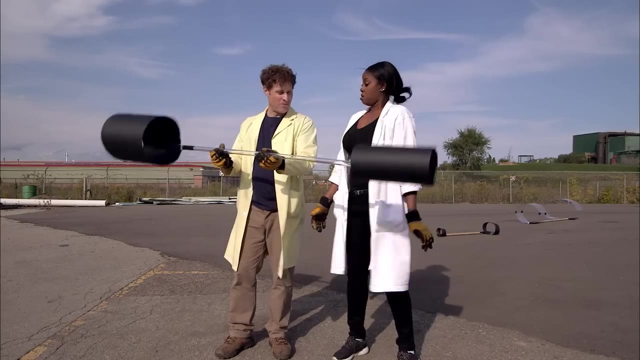 is just what we can put in with one throw. Yeah, What if we could give it more thrust than that? How can we do that, I don't know, like some sort of slingshot or something Like it'd have to be a pretty big slingshot. 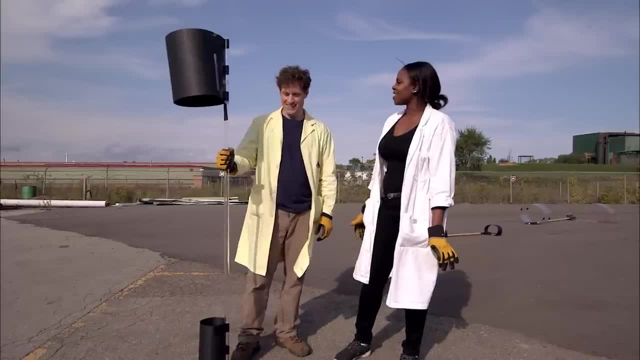 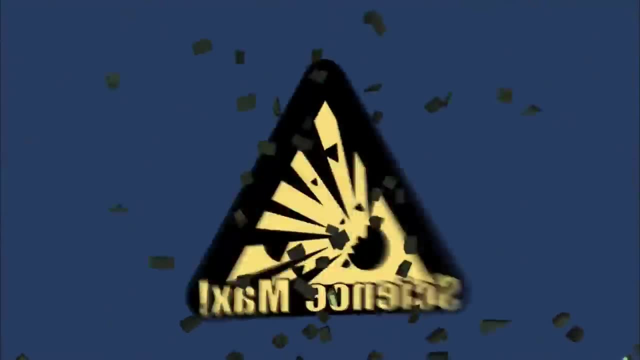 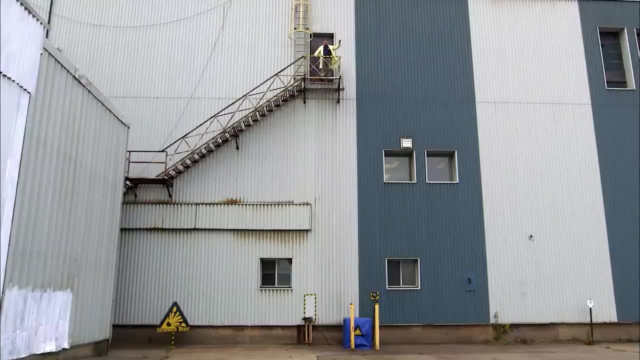 A pretty big slingshot, But I think that sounds great, though. I think we can make a big slingshot for this, Why not? Okay, high five, Let's do it. All right, This is an egg. Eggs do not like to be dropped. 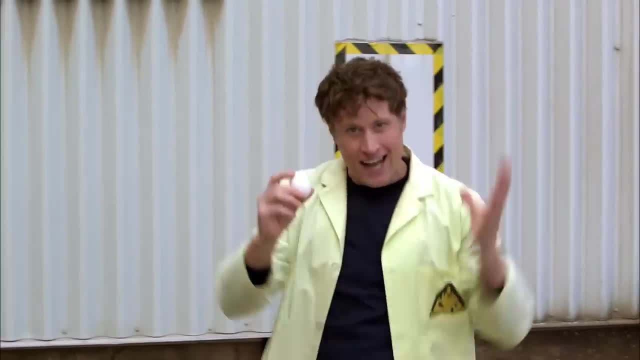 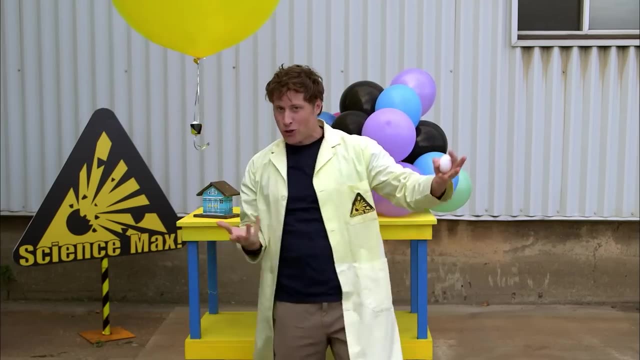 Oh, fortunately we can use the power of science to design something that'll keep the egg safe as it falls. Behold my egg drop contraption. Behold my egg drop contraption. Behold my egg drop contraption. 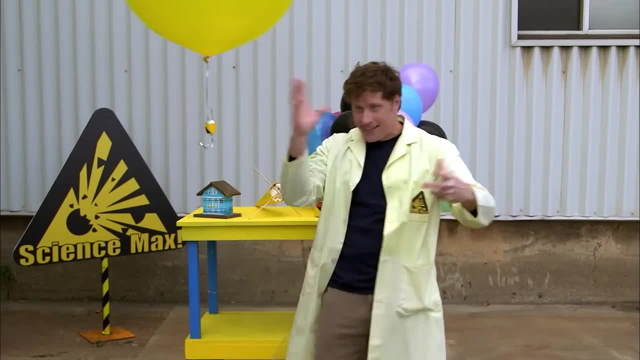 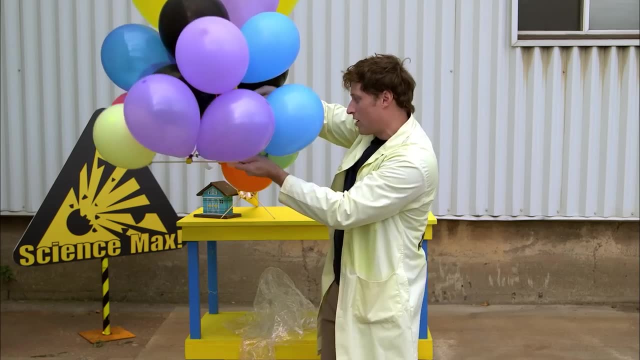 The thing I really like about this experiment is there's no wrong way to do this. You can come up with any design you want and see if it works. This one here is a bunch of helium balloons. This structure is just to keep the helium balloons on. 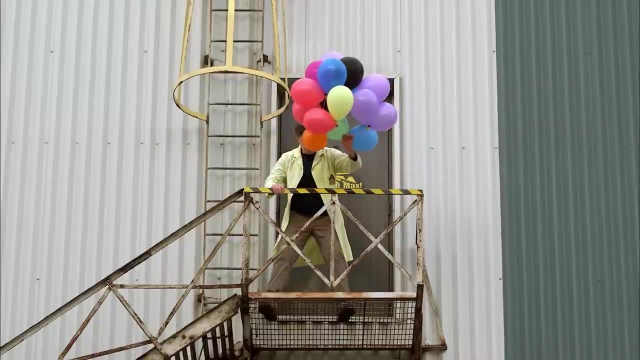 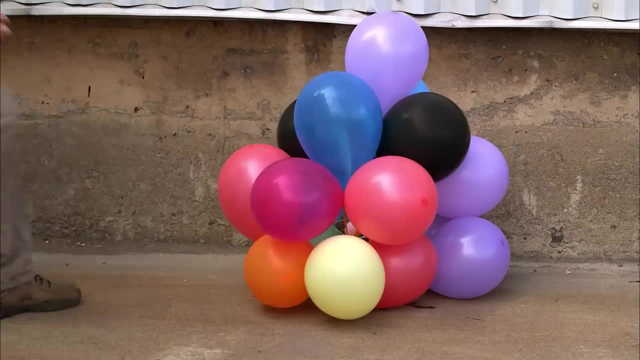 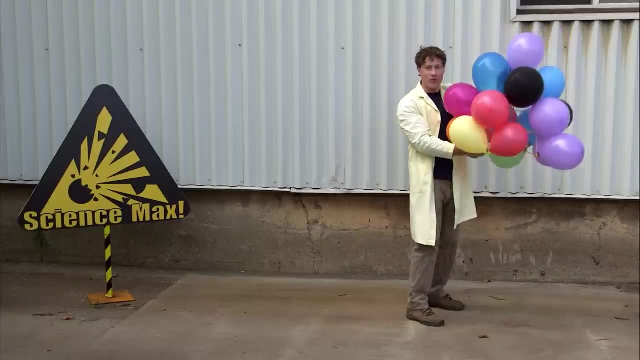 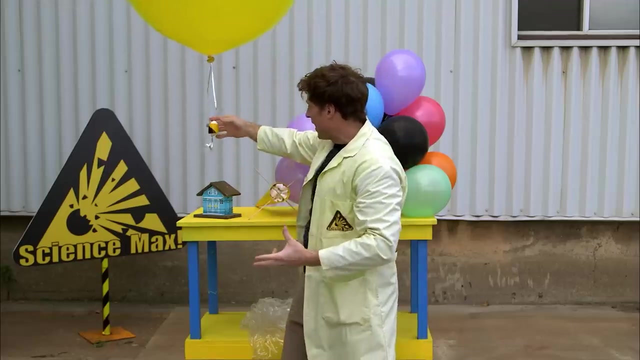 so the egg can touch down very gently. Here it goes, Whoa And, and the egg is unharmed. Miraculously sound. That one worked really well. Success. This is a giant helium balloon that I think will work pretty much the same way. 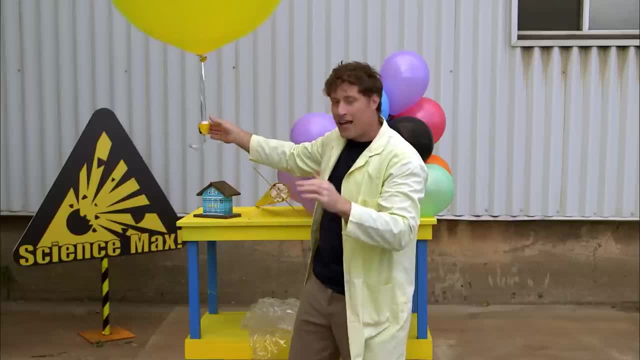 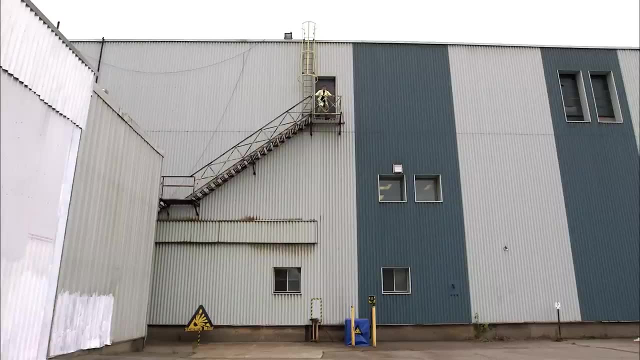 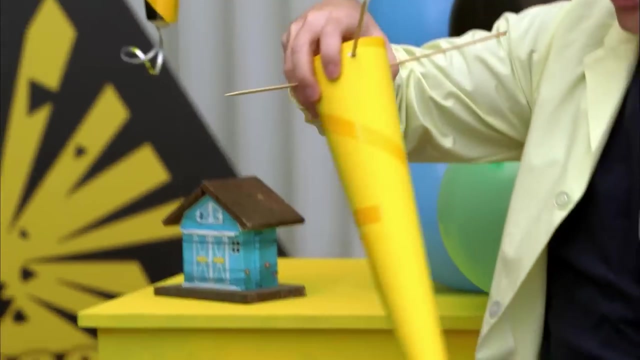 because I think this balloon will drop just slowly enough that the egg can actually just touch and nothing will happen. Um, so that didn't work. And then there's this one, which has no slowing at all. It's all designed to just absorb the impact. 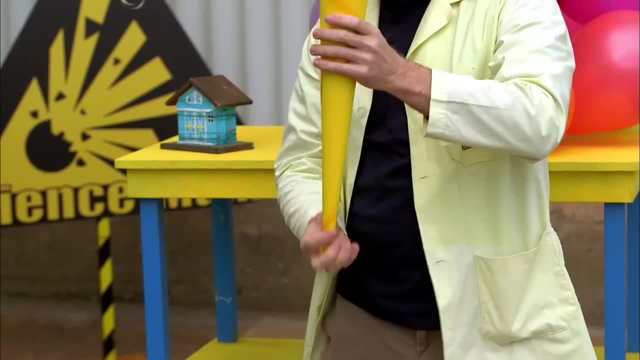 And the idea is that the current balloon is going to be the one that's going to absorb the impact. And the idea is that the current balloon is going to absorb the impact And that cone will crumple and absorb the force when it hits the bottom. 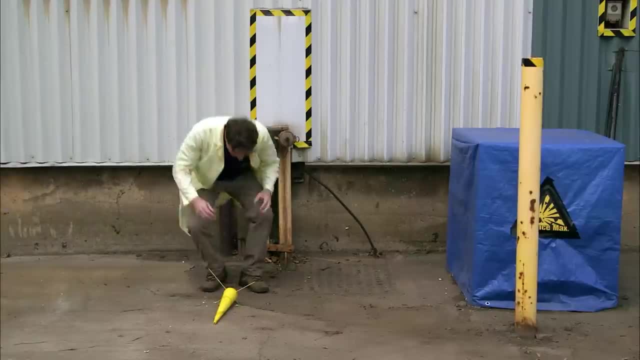 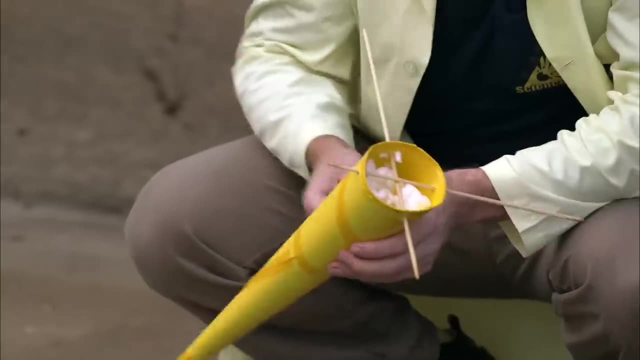 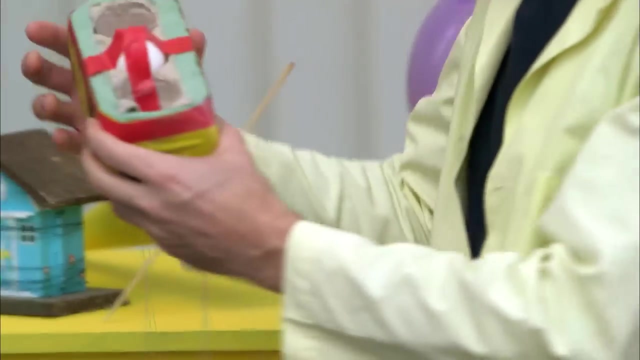 Oh no, Oh no. I think it would have worked if it hadn't turned in the air, but it did, and well, I guess the egg is completely broken. So I'd call that one a fail. This one is the parachute. 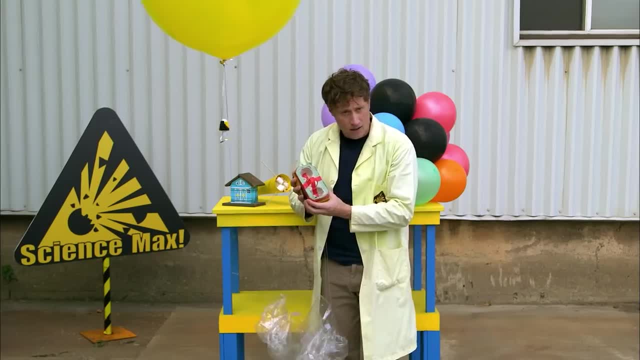 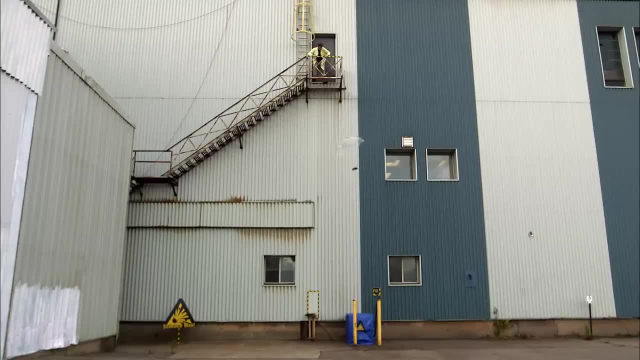 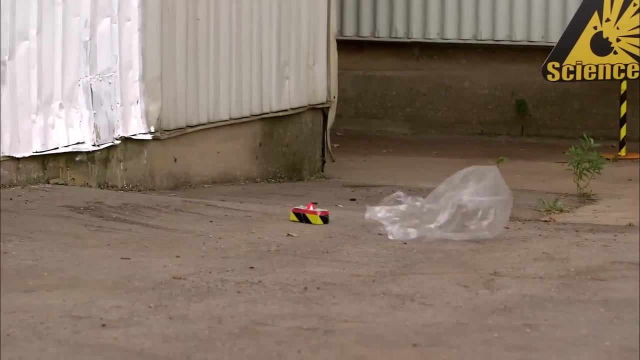 You see, the egg has been nestled into this foam container And this is a parachute that will hopefully slow- Let's slow- the egg down, Whoo, Uh-oh, Whoa, Over, Over, Good, And That one seemed to work well. 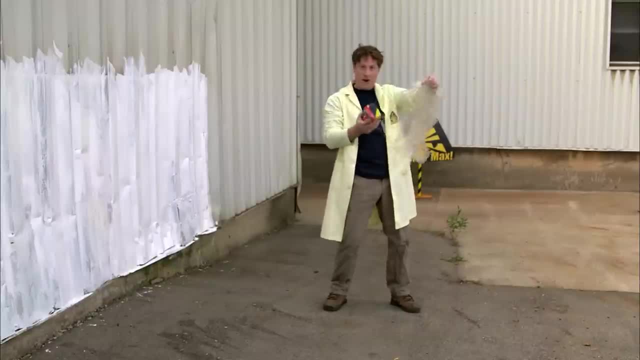 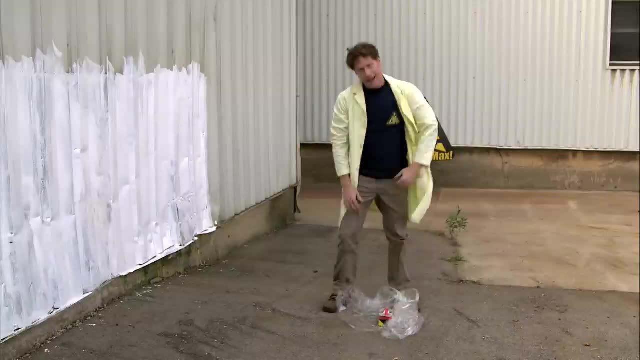 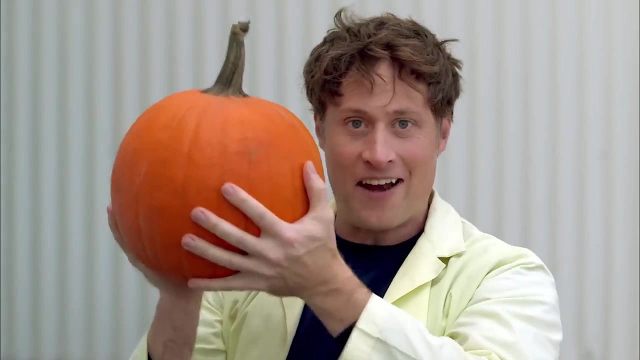 Yep, The egg is totally fine, The parachute worked, All right. Egg drop experiment: Totally fun experiment to do. But the question is: how do we max it out? And the answer is: Pumpkin drop. Same thing, except with a pumpkin instead of an egg. 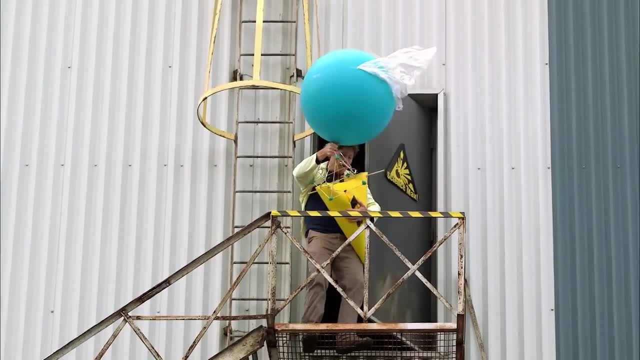 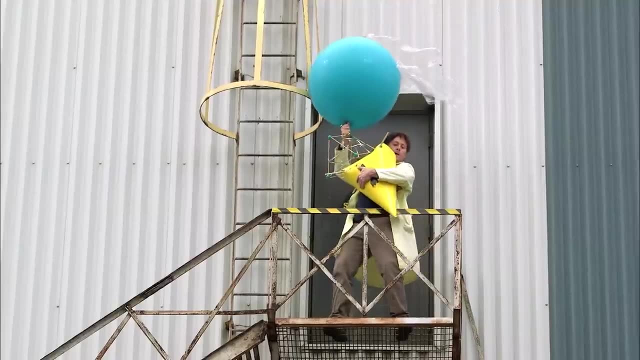 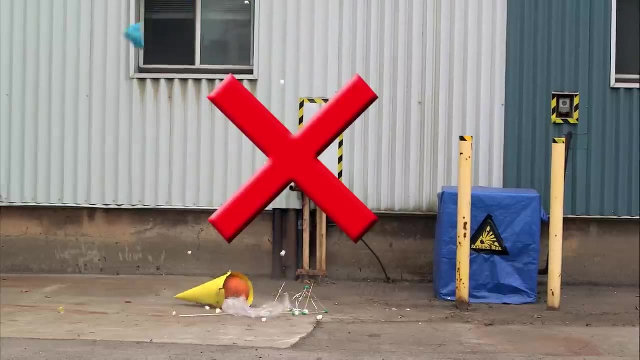 Come on, Okay, All right, Pumpkin drop with everything attached all at once. Okay, Here we go, Ready: One, Two, Three. So what we've learned from this is: the heavier something is, the more force is acting on it from gravity. 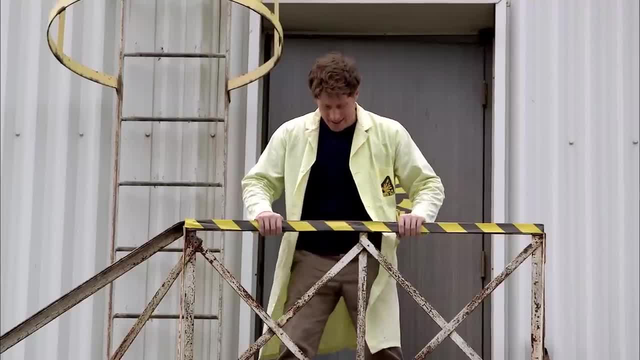 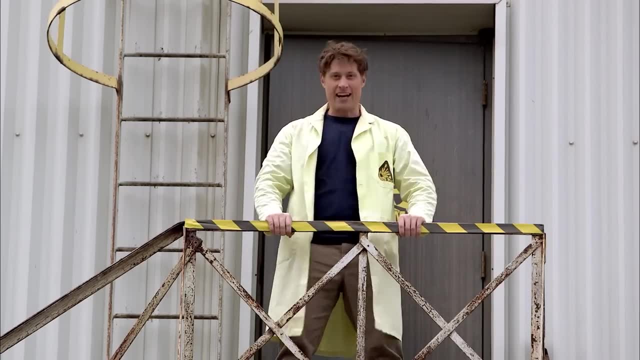 which means the harder it is to slow down when it's falling. Okay, Fair enough, You win. You win this one Gravity, But I'll beat you. next time I'm I'm gonna get a broom. Being a chef is my absolute passion. 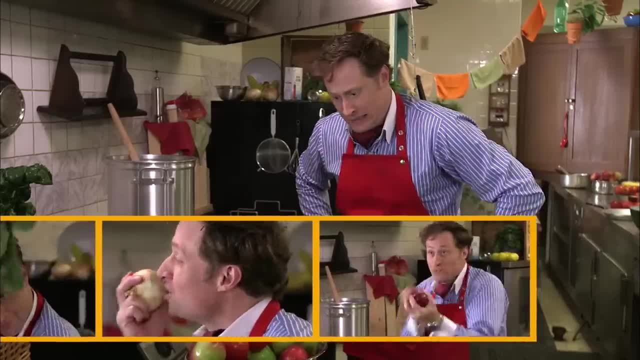 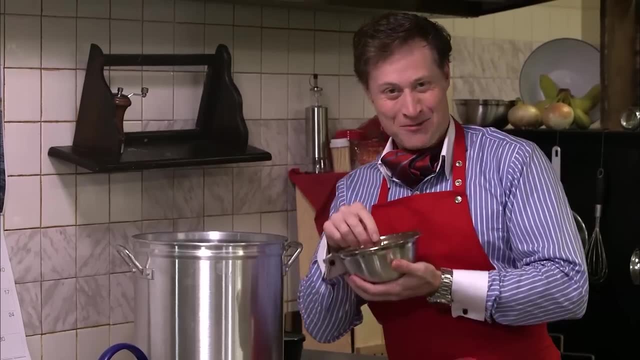 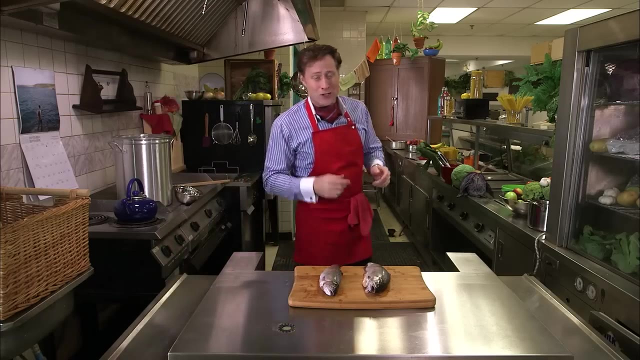 And cooking up science recipes is my speciality. I'm Buster Beaker and this is Cooking With Science. Oh, hello, Welcome to Cooking With Science. I'm Buster Beaker- Delicious. Nothing is more important to have fresh than your seafood. 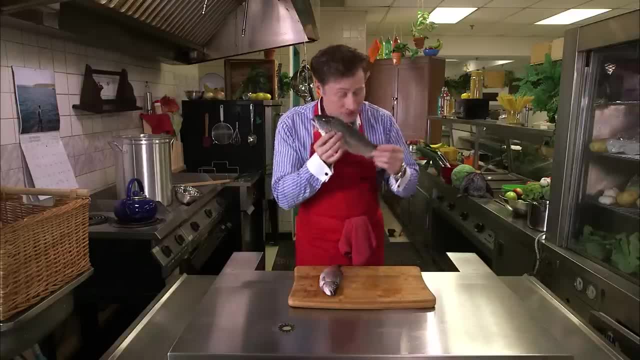 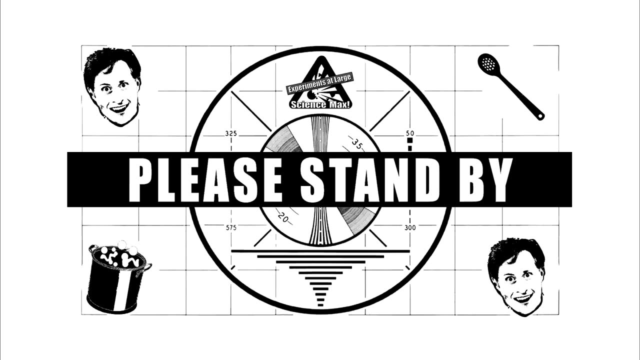 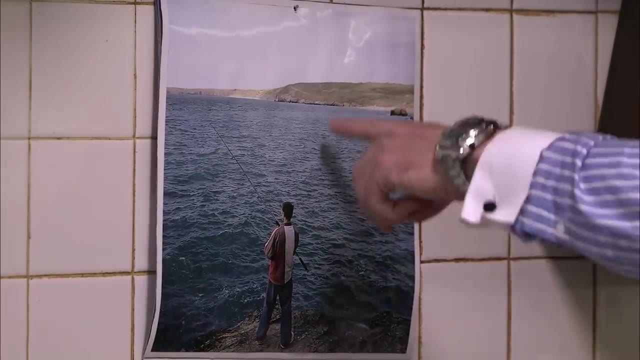 It's what makes the difference between a fresh fish and one that isn't so fresh. If you live by the ocean, you probably know that the water gets high tide and low tide. Look closely, It's the same location, Amazing. 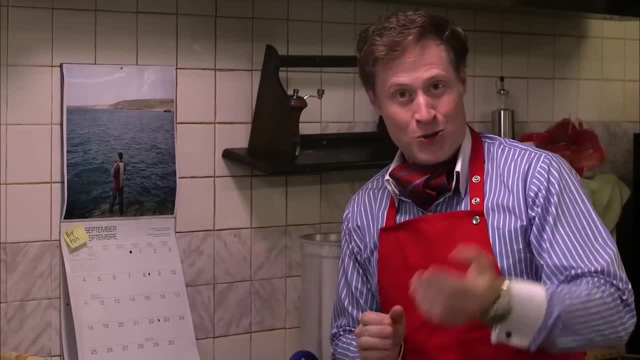 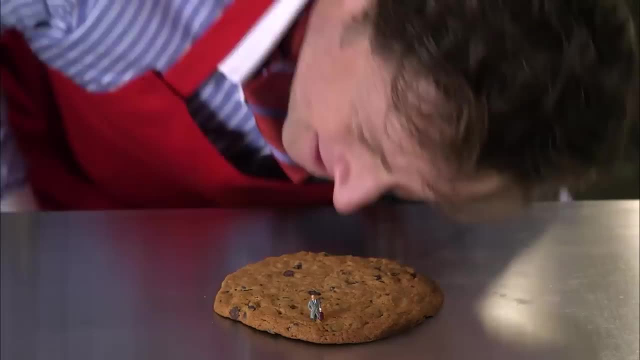 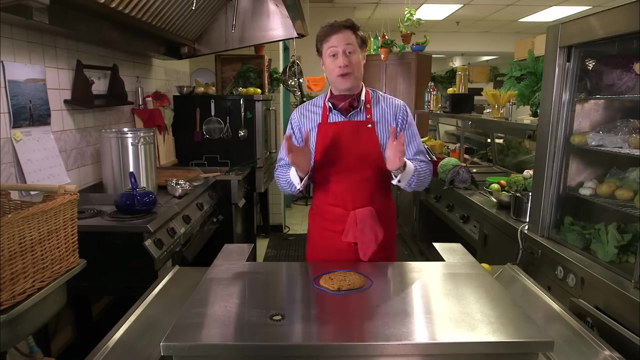 But did you know that this is caused by the gravity of the moon and the sun? See, this cookie is the Earth and this little happy fellow is me. Hello. And this string represents the water around the Earth. If we didn't have gravity to worry about, 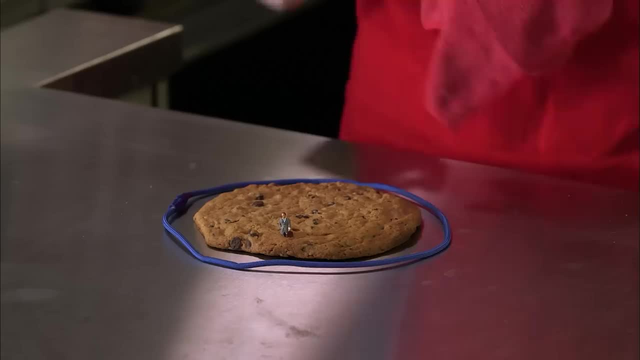 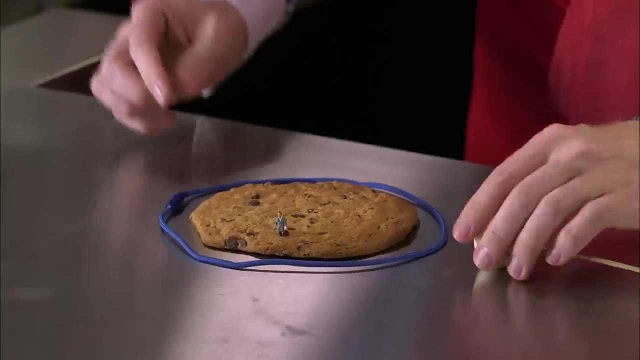 the water would all be equally deep around the Earth. But here comes the moon, this mushroom. Now the moon has gravity and that pulls the oceans towards it, a little bit like this, And that creates high tide there and low tide here. 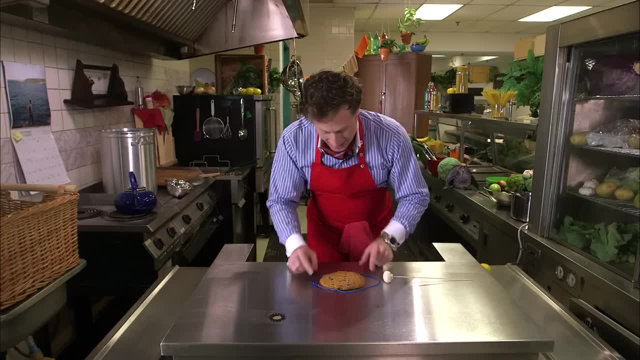 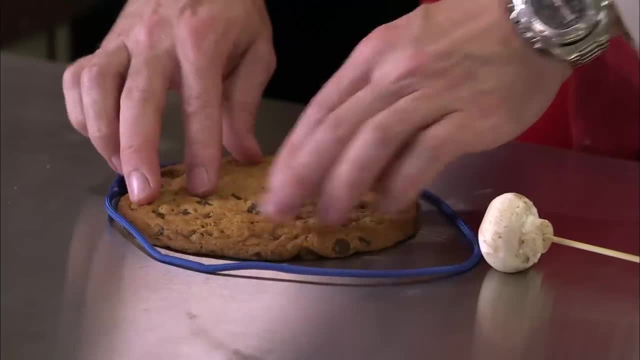 and a little bump of high tide on the other side of the Earth. And as the Earth rotates and I'm on it, I experience low tide and high tide and low tide and high tide- Very interesting. But there's another factor. 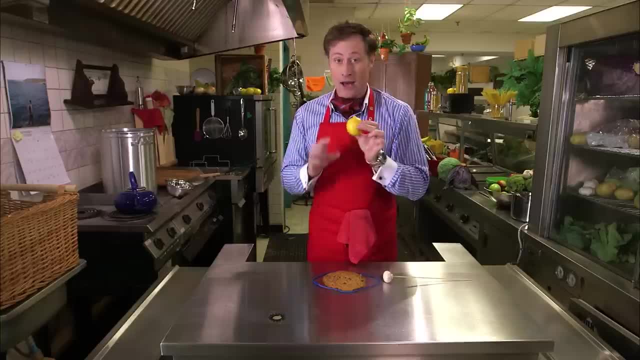 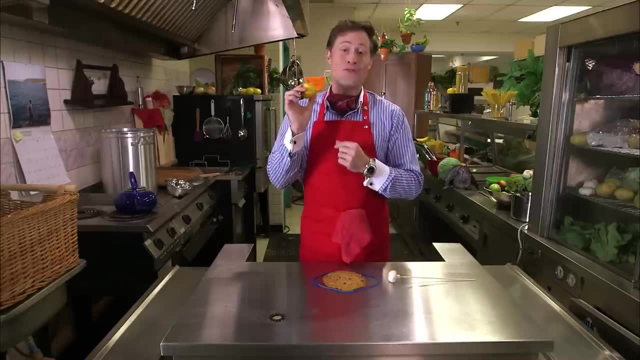 The sun, or this lemon. Now, the sun also affects the tides, but not as much as the moon. Now, the sun does not affect the tides as much as the moon because it's much further away, But it still has an effect. 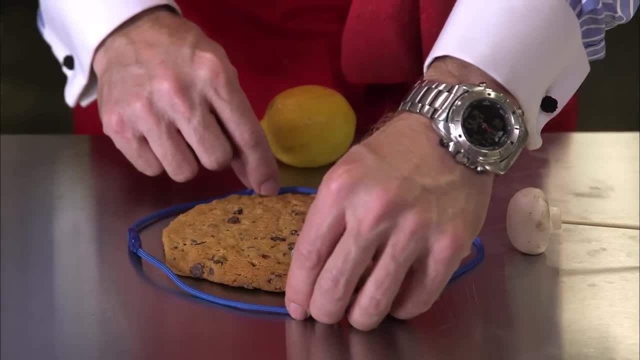 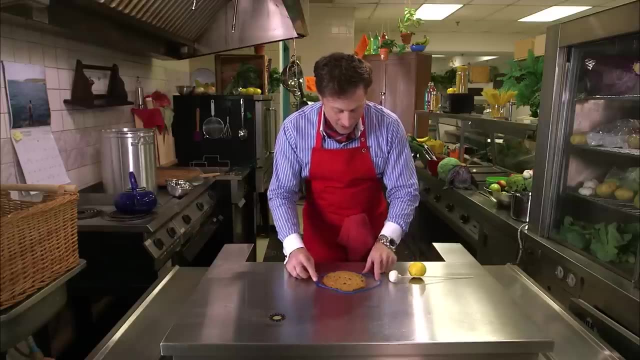 If the sun was here, then the tides would be pulled away a little bit like that, and the tides would be less severe. But if the moon and the sun line up, like over here, you'd get a very, very high tide. 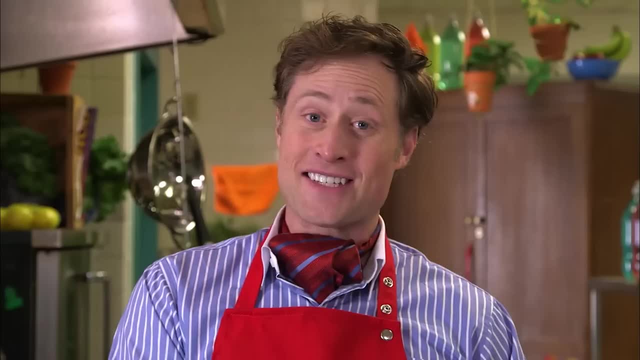 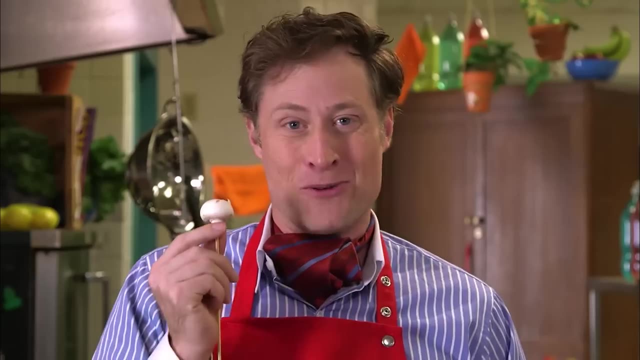 and very, very low tide. So there you are. That's how the tides are affected by the gravity of the moon and the sun. Mmm, delicious. I'm Pastor Beaker, and thank you for joining me on Cooking With Science. 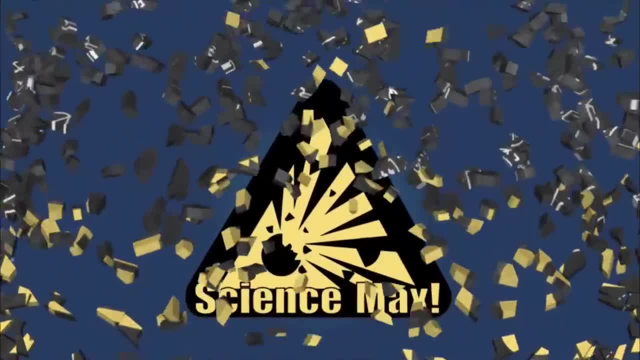 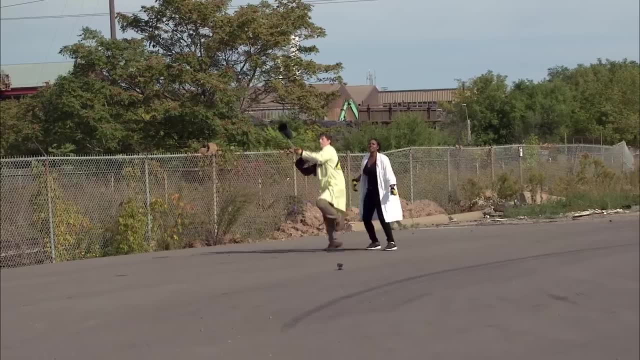 Oh, Our maxed-out hoop glider was working pretty well. That was amazing, Pretty good. Here we go, But we could only give it so much thrust by throwing it. Oh yeah, So we came up with the perfect science max solution. 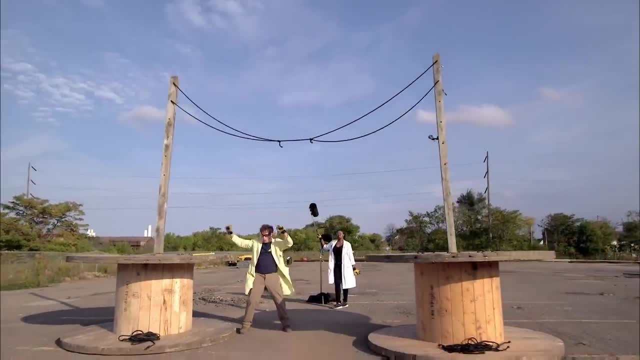 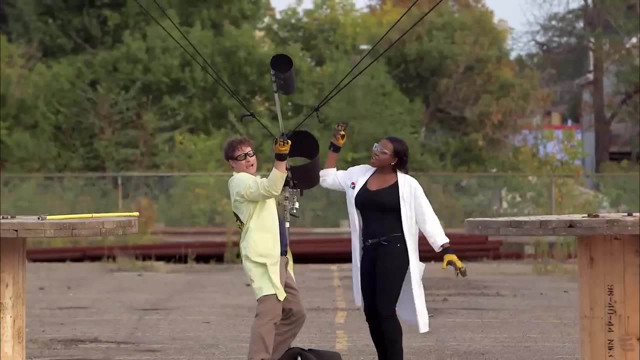 Our giant slingshot. We pull the bungee cord back and hook it onto our hoop glider. I am ready to fire. Count me down Three, two, launch it. Whoo-hoo-hoo-hoo-hoo. 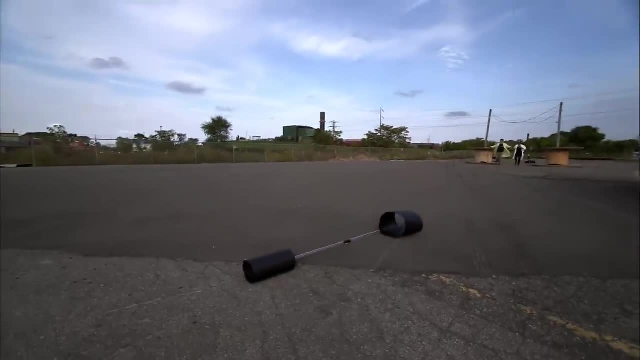 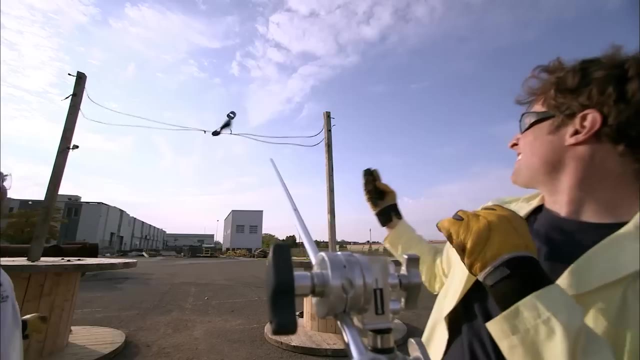 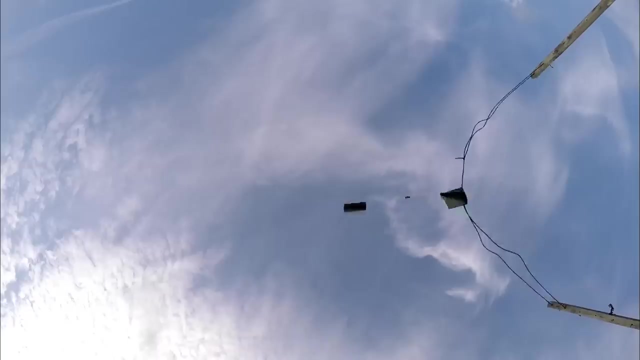 Whoo, Very nice. Our slingshot is amazing. By giving the glider more thrust, that is, more energy at the beginning, so it's going faster. when we launch it, the glider soars through the air and flies a long way. 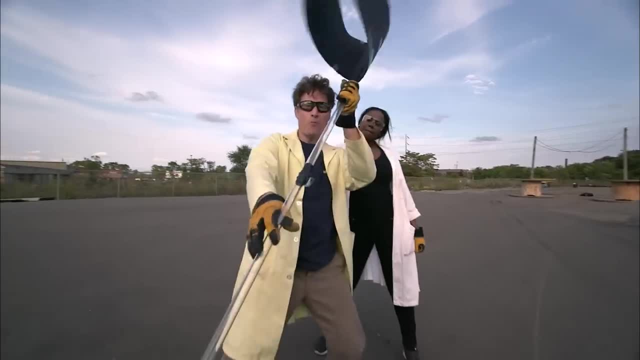 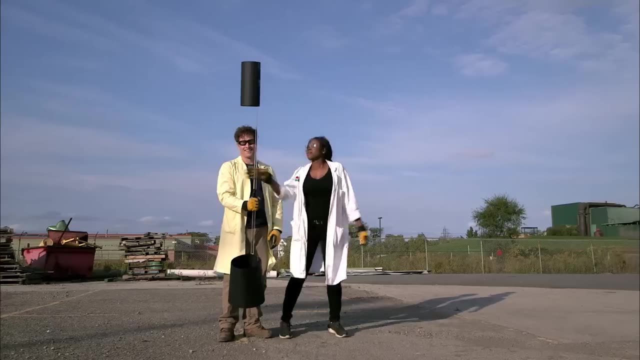 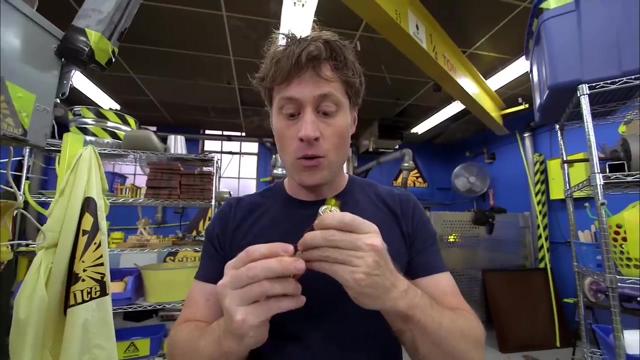 That was great. So there you go, Giant hoop glider, Yeah, Science max. Experiments at large. Nicely done. What more could you ask for? Well, my turn. Hey, see you next time. Science Max. This episode of Science Max. 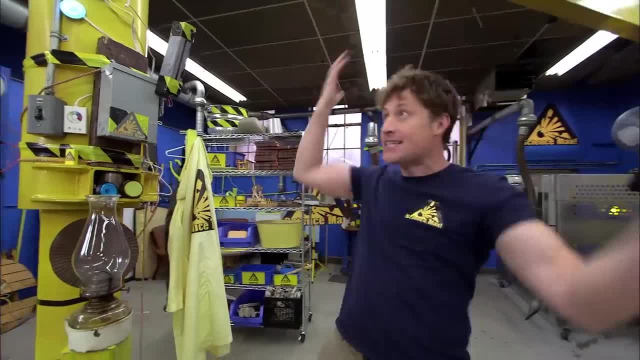 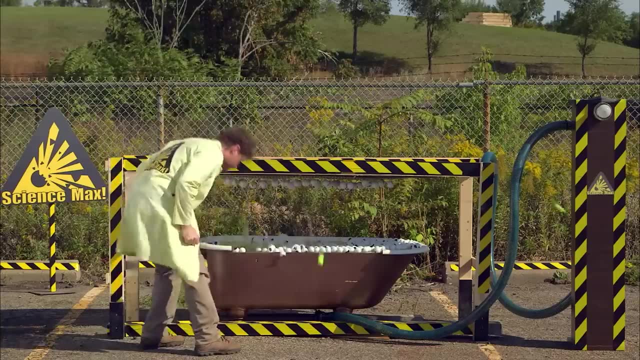 is all about generating electricity. Where do we get this electricity that we use all the time? We try to generate as much as we can using human power, Plus solar energy, tidal energy, wind energy and more. All you need to do is: 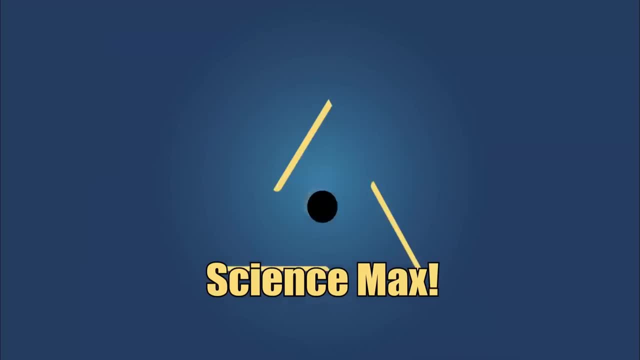 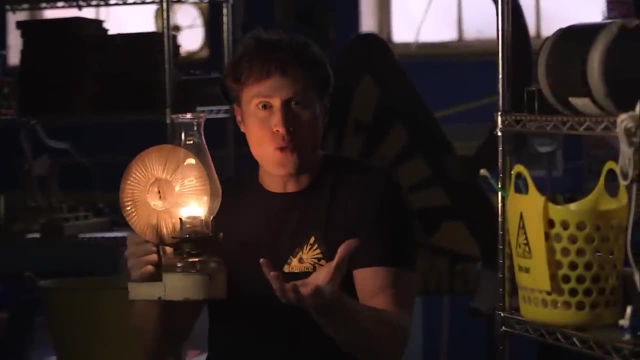 Turn the generator. All on this episode of Science: Max Experiments, Experiments at Large, Greetings, Science Maximites. Take a moment and imagine with me, if you will, a time when the only way to light your house was with candles or oil lamps. 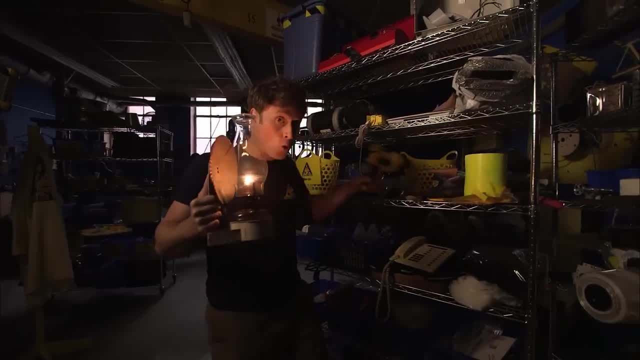 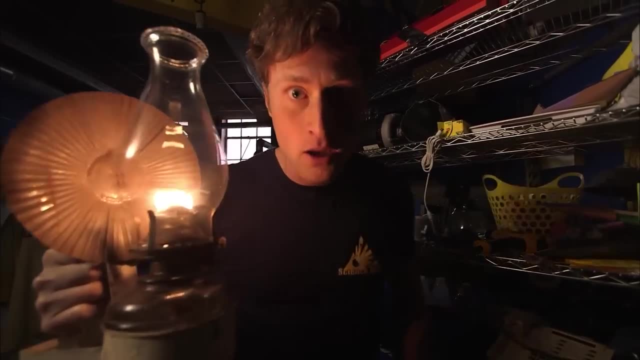 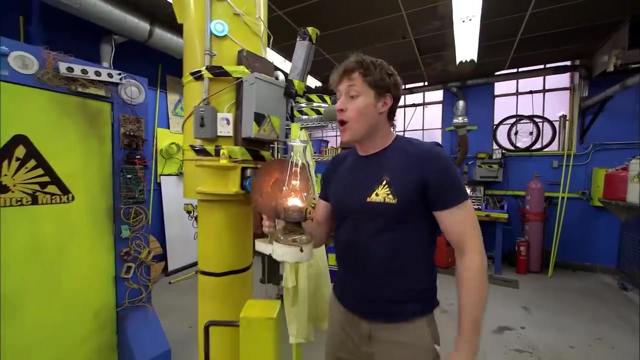 There was no electricity, That meant no power tools, no video games, no telephones and, worst of all, no TV. Fortunately, we live in a world of electricity. If you've ever lost power in your city or neighbourhood, you know how hard it is to get by. 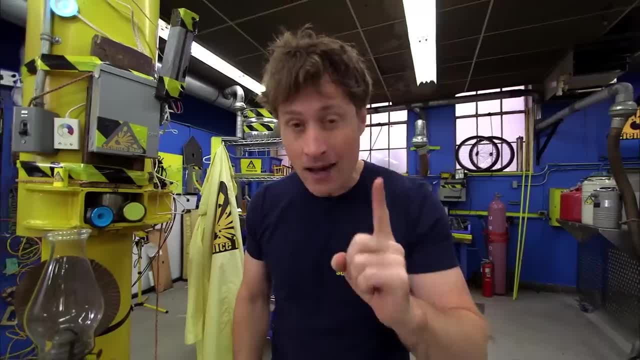 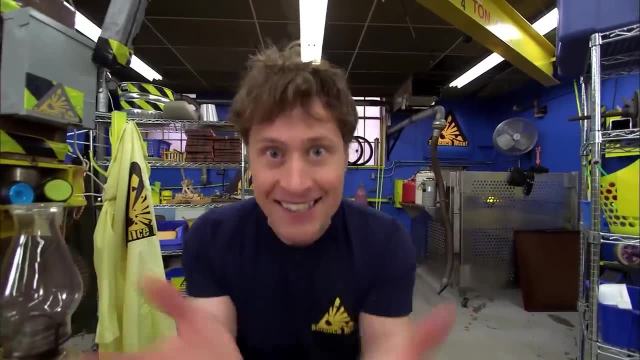 without electricity even for one day. But where does it all come from? Where do we get this electricity that we use all the time? We make it. That's the cool thing, And I can show you how to make it as well. 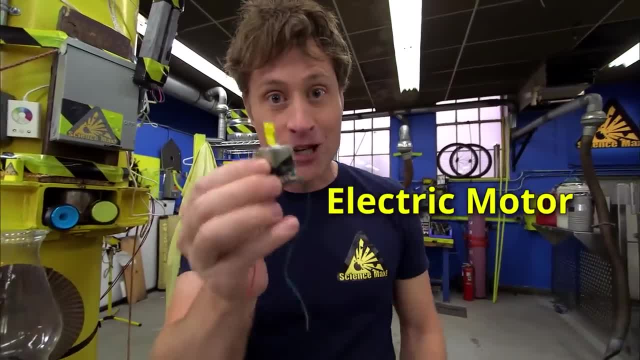 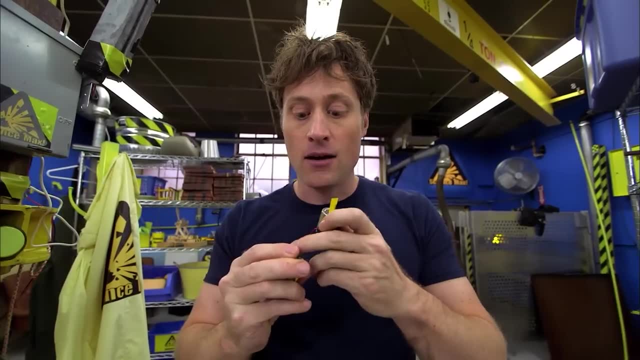 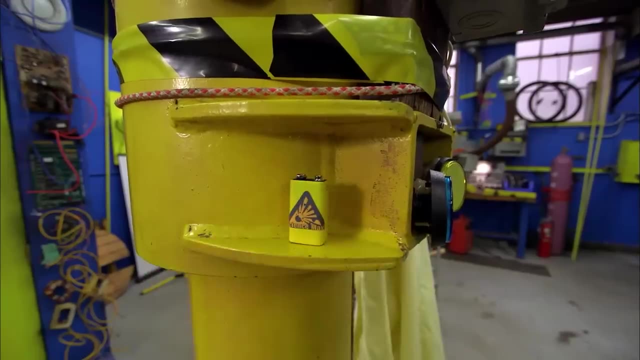 Check it out. All you need is an electric motor. Electric motors are pretty simple. All you do is get a battery and you attach it to the electric motor and that makes it work. There we go. Attached to the battery, it spins. 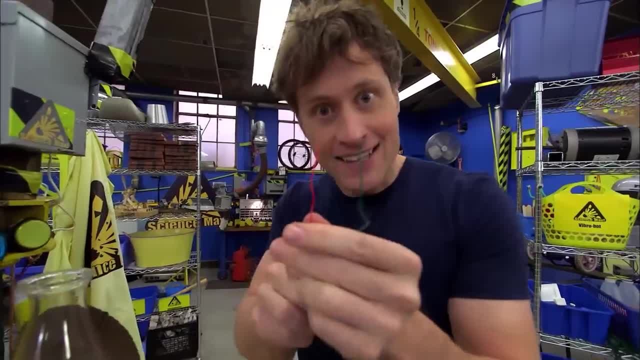 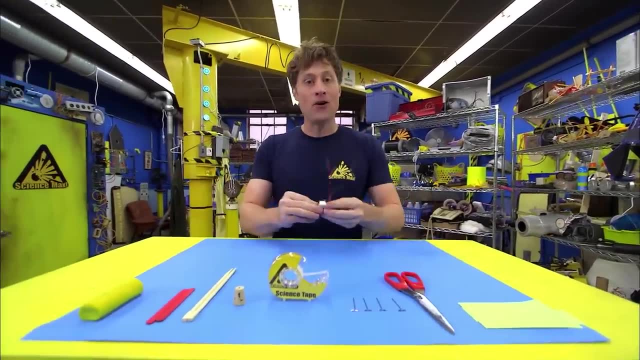 But if you spin the electric motor, it creates electricity, And that's what we're going to look at today: Creating electricity. We're going to build a wind turbine, But first you need an electric motor And you can probably get one. 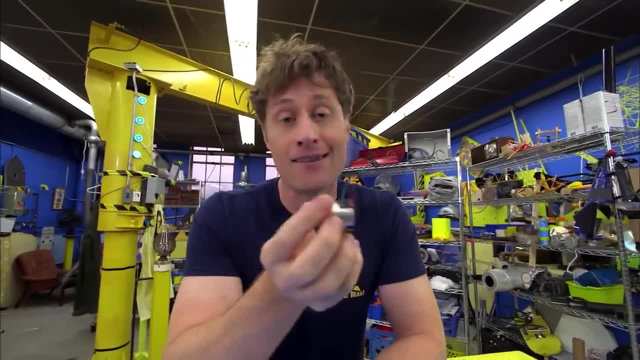 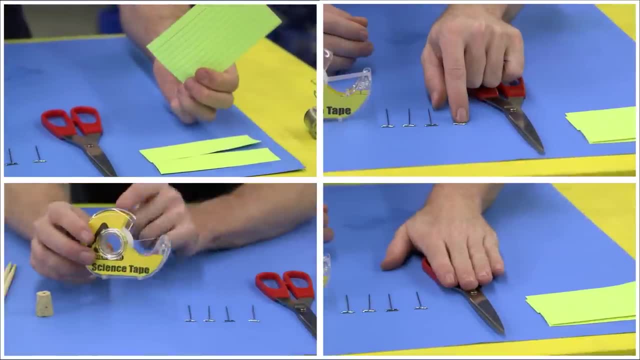 from a broken toy. Just make sure that the toy is broken and that the broken part isn't the electric motor. Here's what you need In December. you'll need index cards or construction paper, scissors, push pins, science tape. It's the same as invisible tape. 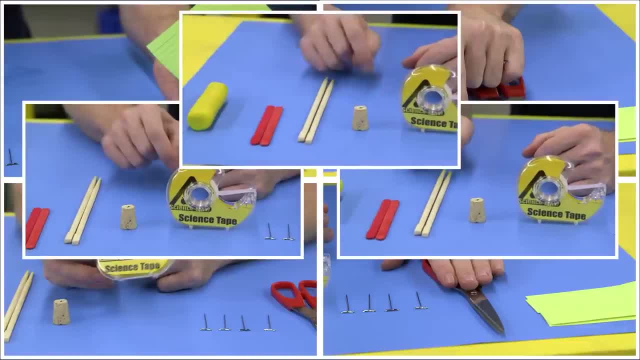 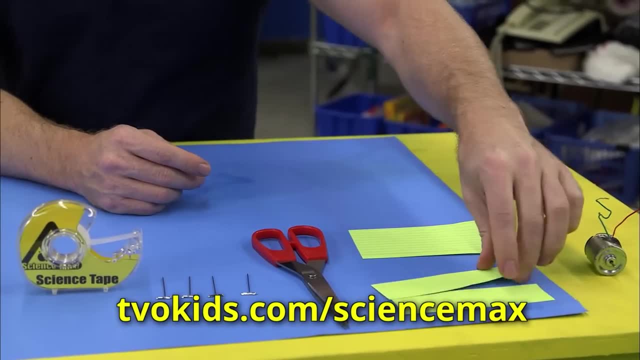 except I use this one for science- A cork chopsticks, craft sticks and modeling clay. And remember, all the steps for this experiment are on our website. To begin, cut the index cards into strips and tape down a push pin so it sticks out. 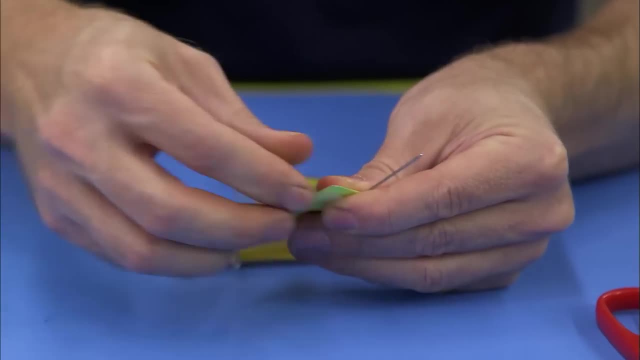 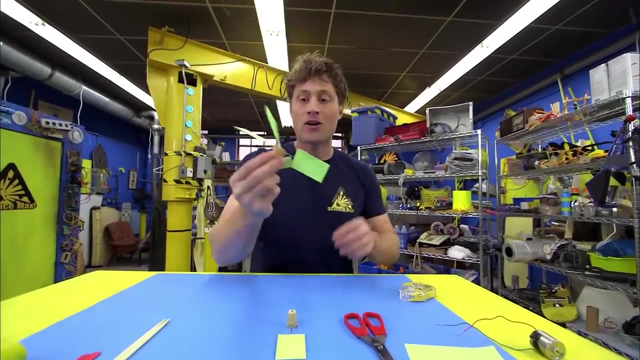 Then fold over the index card and tape it together. Then stick the pin into the cork and repeat that step. If you want as many blades as you can get on your fan, you are welcome to do that. Next, take your modeling clay and stick the chopsticks in. 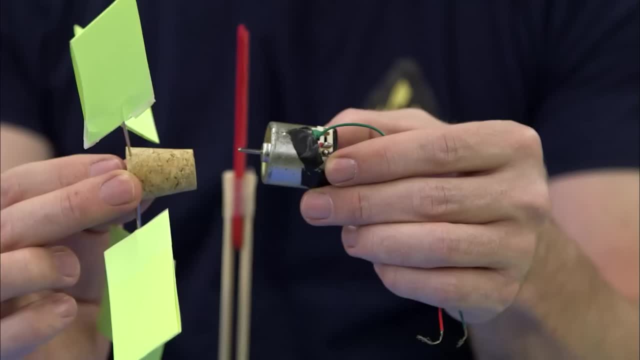 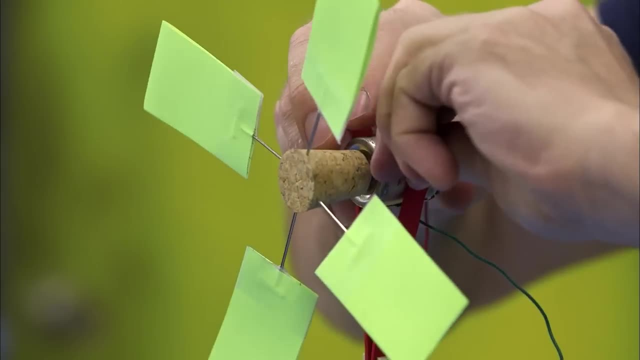 Then tape the craft sticks in between with science tape. Then take the motor and stick the cork on the end. Then wedge the motor in between the craft sticks and tape it down so it stays put. And there you go- a fan that will spin in the wind. 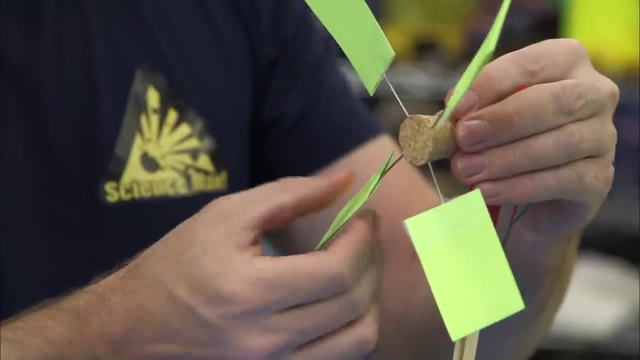 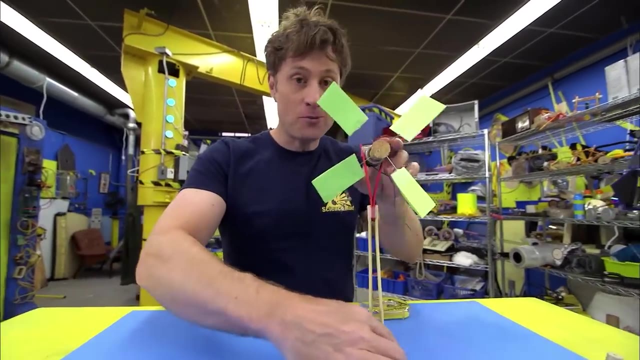 You want to adjust the fan blades so they all face on a bit of an angle. That way they will catch the wind and spin. There we go Now. when it spins, it will create electricity. I'll show you with this: It's a multimeter. 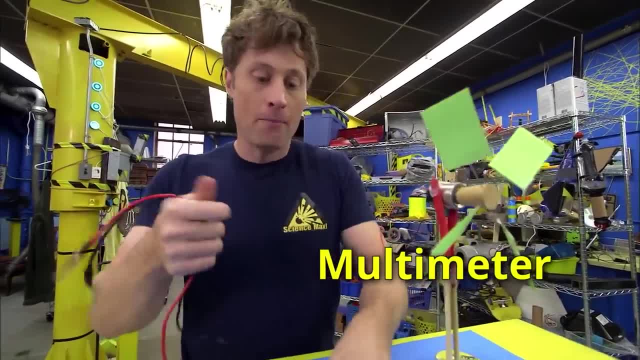 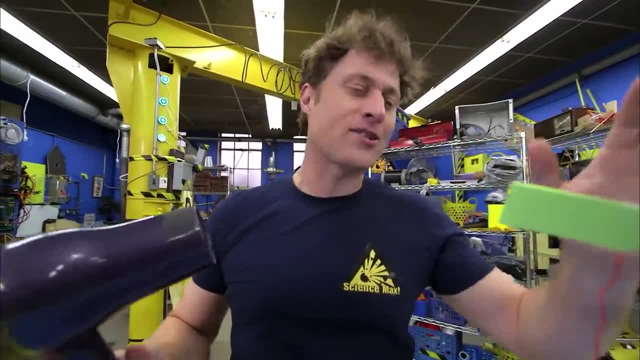 And a multimeter measures little amounts of electric current. There, The hair dryer makes wind, Spinning the fan blades, and we are creating electricity. Now, pretty much all electricity that you make comes down to turning a generator, A small motor like this. 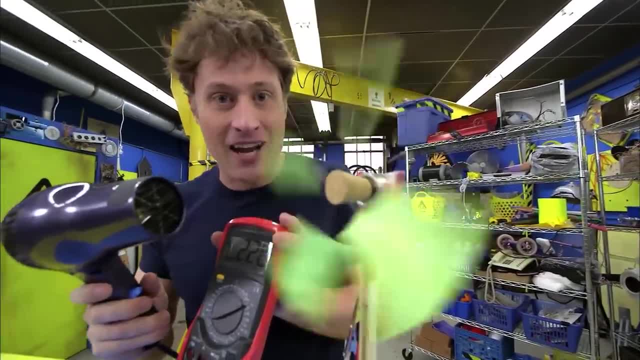 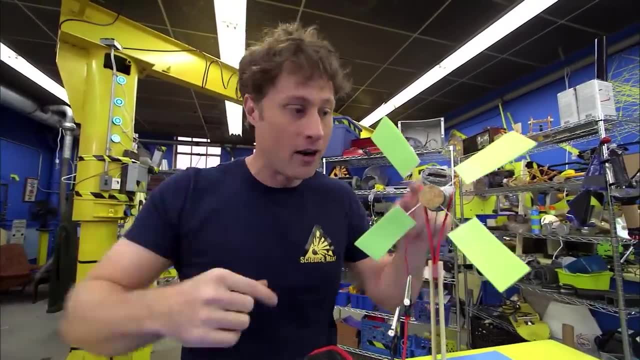 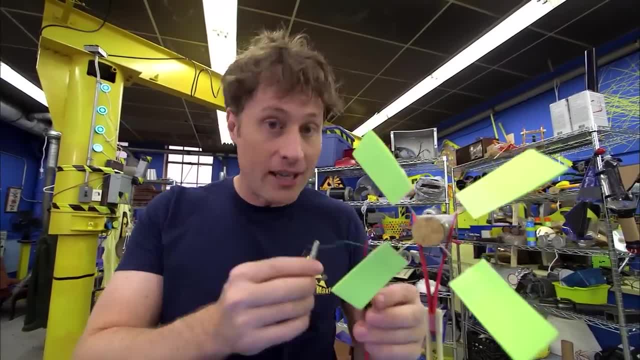 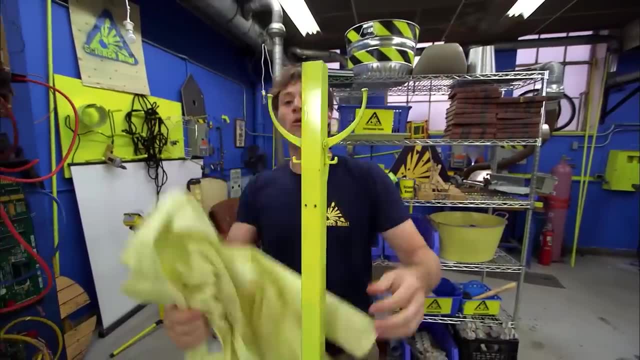 a lot of noise. Now it's going to make a lot of electricity- Barely enough to power one tiny little LED. But it's a start, And a good start is all we need, Because Today, on Science, Max Experiments At Large. 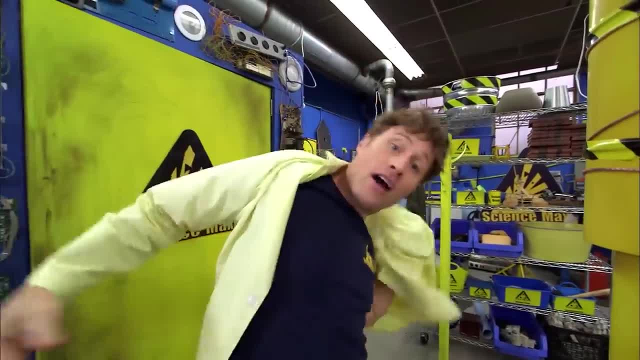 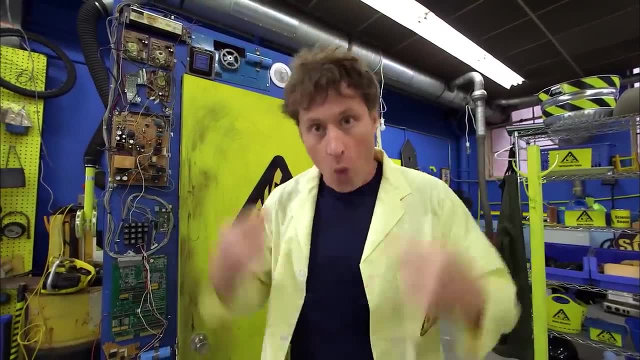 we're going to look at all kinds of different ways of generating electricity. Plus, I want to find out just how much electricity one human being can generate. Although one human being is going to be kind of lonely, I'm going to need an expert. 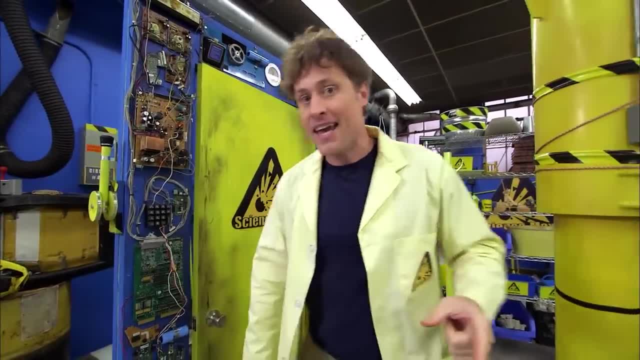 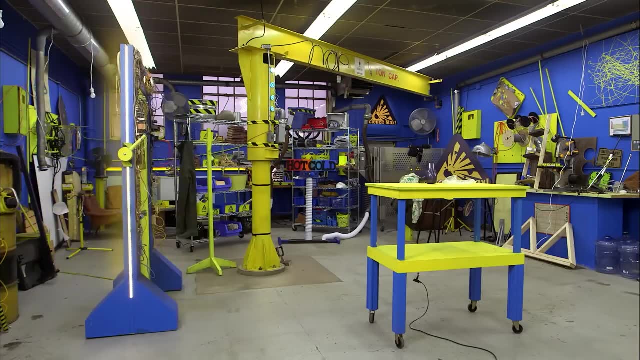 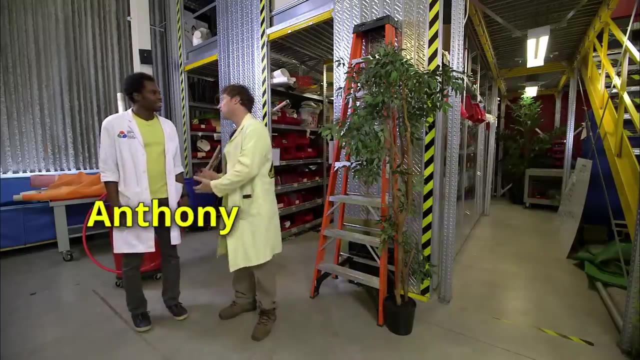 Oh, I know Anthony from the Ontario Science Centre. He could help. I wonder if he's busy. Well, come on. Oh, Anthony, Bill. So I was wondering if you could help me with an experiment I want to generate. 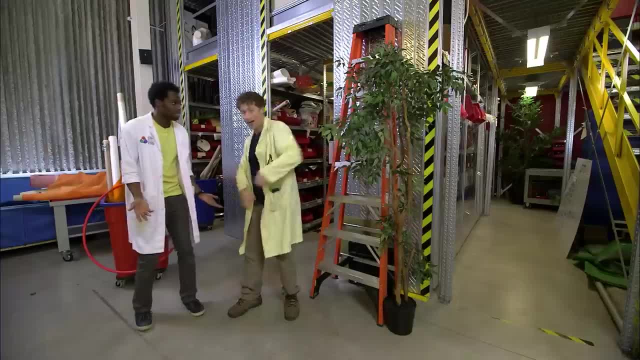 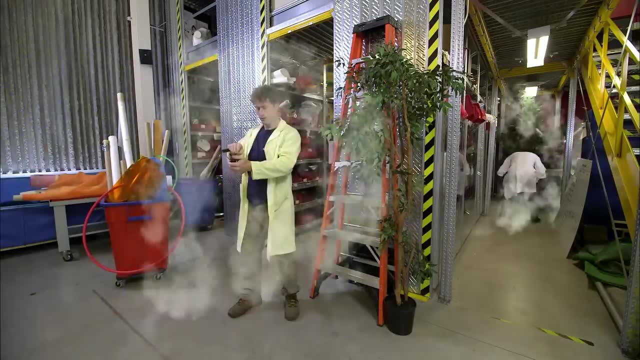 as much electricity with human power. What do you think? I think that sounds awesome. Okay, great, Let's go back to Science: Max headquarters- Is that the portal? Yeah, Don't worry, I'm going to show you how to do it. 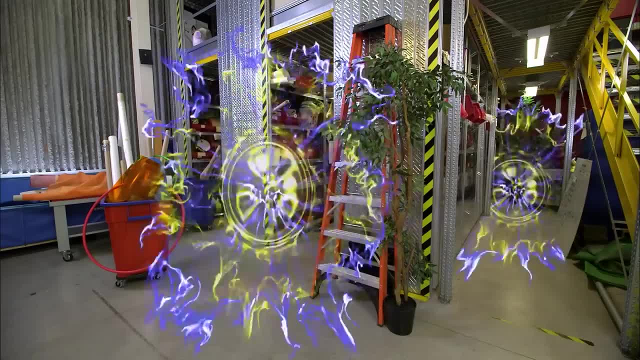 I know what it is. It's this: Where did you end up? I was in the vents. Oh, I ended up in the bathroom. All right, Well, now that we're here, Okay. so this is what I started with. 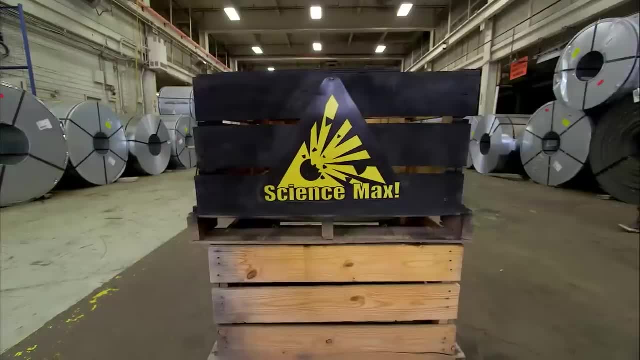 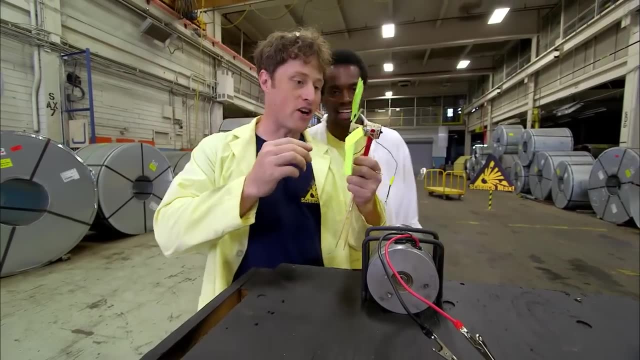 And this is just, you know, an electric motor, right, Right, So you can generate electricity. You spin it, So I figured, in order to generate electricity. you spin it, So I figured, in order to generate electricity. 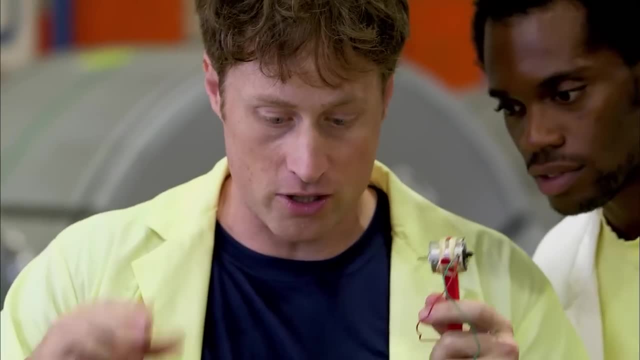 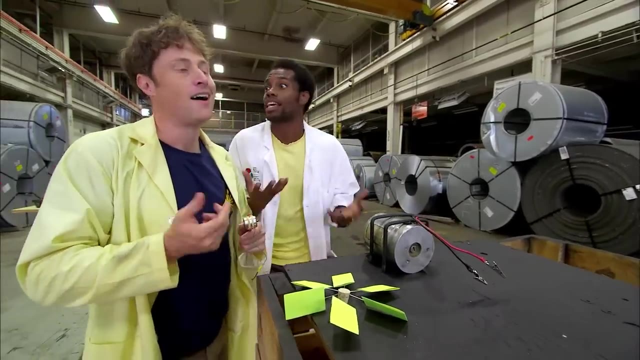 you spin it. So I figured, in order to generate more electricity, you get a bigger generator. Exactly yeah, The bigger the generator, the bigger the magnet, the more the copper, the more the electricity. Oh well, you know. 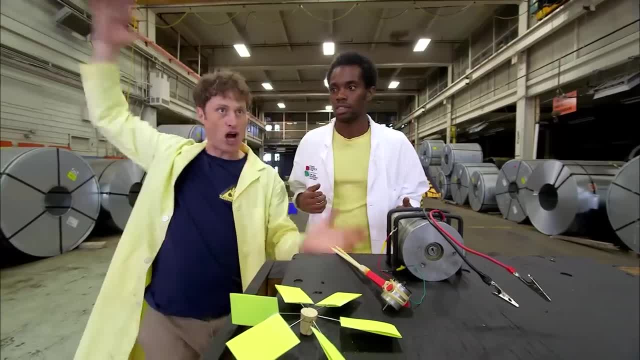 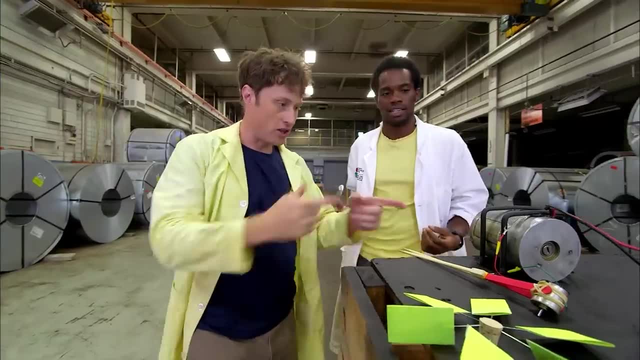 what we should do is we should just get an even bigger one, like a giant one that they use in like a power plant or something Not quite. That would be too big for a person to be able to turn. It would just be impossible. 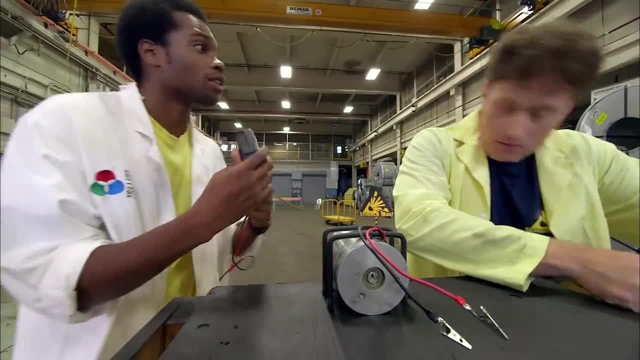 So you think this is a good size. I think this is a great size. Okay, so that's good. This is called a multimeter. We're going to hook up the wires. I will do black to black, Black to black. 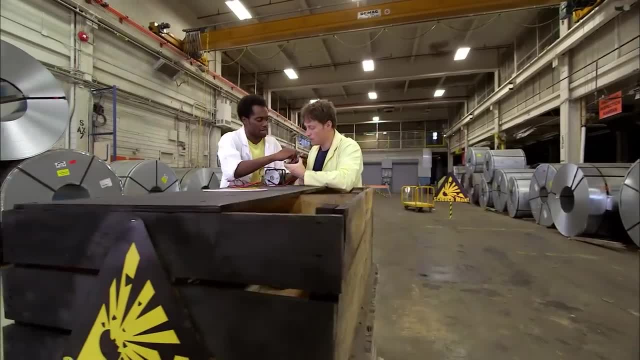 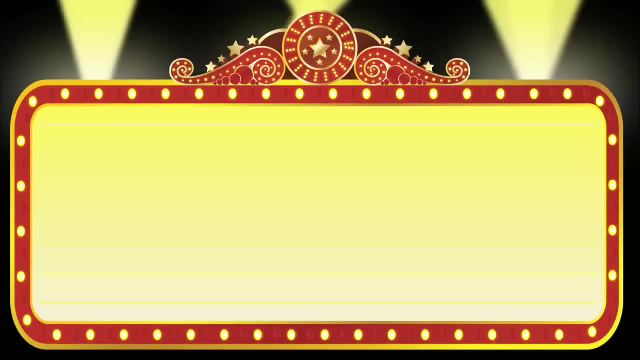 Red And as you turn you can see just how much electricity we're generating. Okay, so Here you hold onto that And I'll turn the generator. Now it's time to play. How Much Electricity Did They Make? 2.4 volts, yeah. 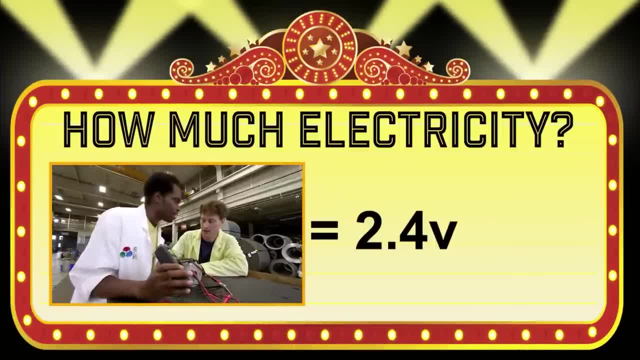 it's not bad. Oh, 2.4,. yeah, it's not great. That's just enough to power a small LED flashlight. Better, keep trying, boys. I got some handles here that we're going to attach to the end of the generator. 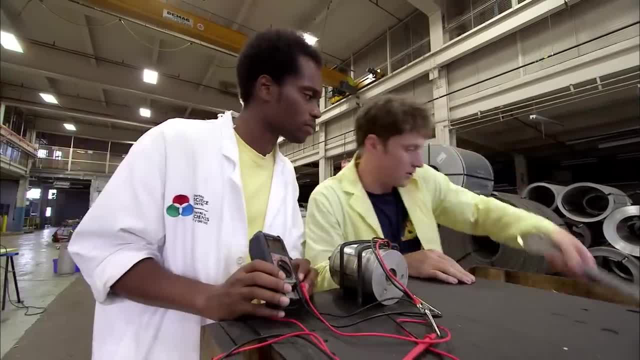 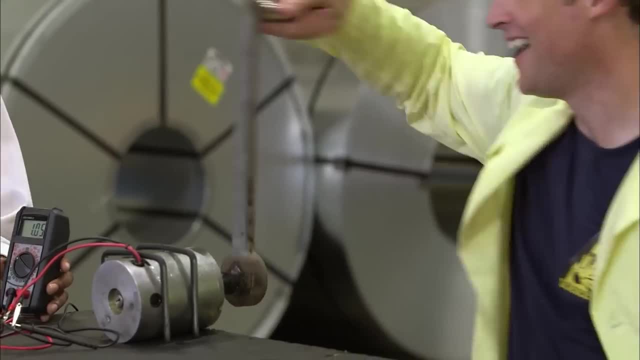 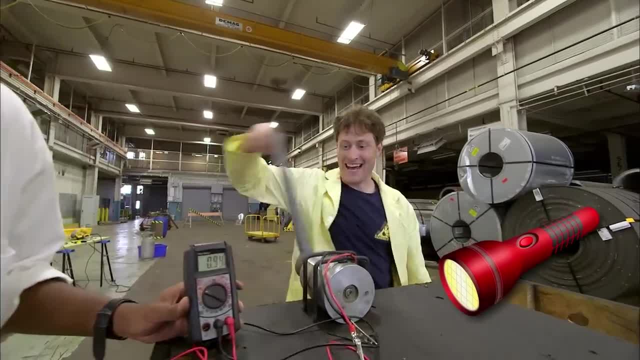 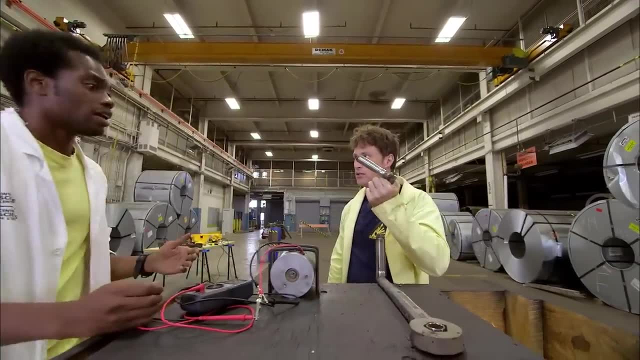 No matter how fast I crank the large handle, I couldn't make any more electricity than before. Okay, let's try something else. I bet it's a smaller handle. Perfect, okay, yeah, That's good. Yeah, well, maybe. 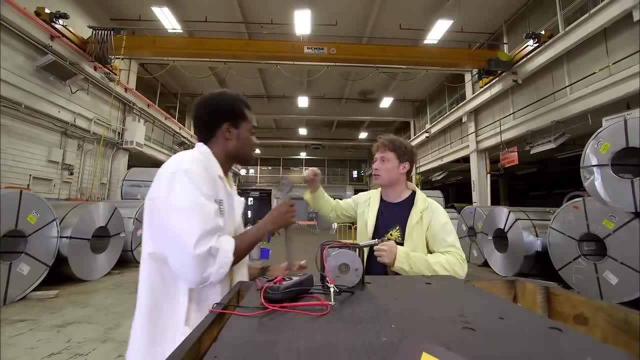 it'll let us get more spins in. Oh yeah, because I don't have to make as big a circle. Exactly Yeah, it's working already. We're up to like 3.5.. Now how much electricity is Phil making? 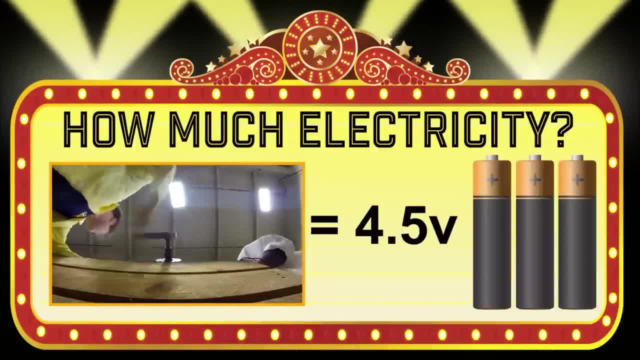 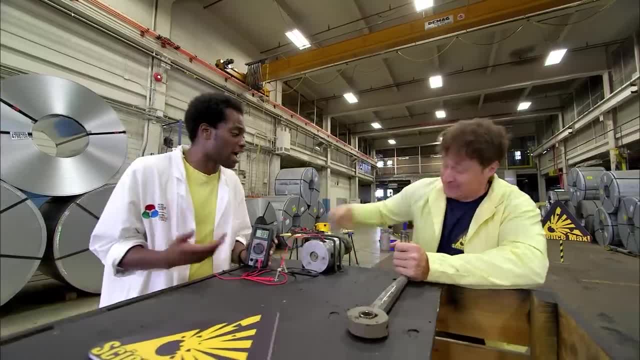 4.5.. That's the same as three double A batteries. Maybe enough to power a toy car. Still a long way to go. Yeah, it's a lot higher with the fastest spins. Oh, all right, all right, You okay. 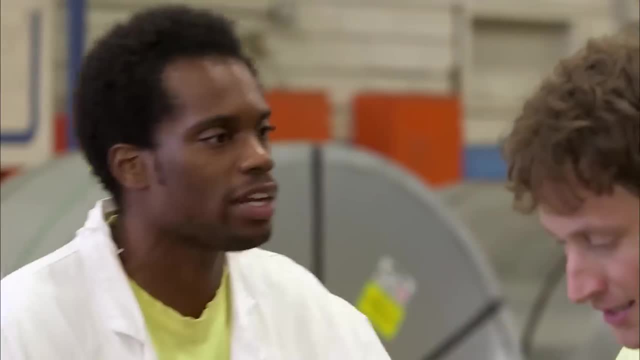 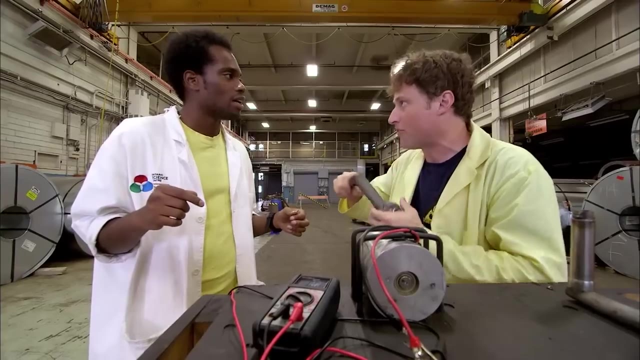 I'm okay, Maybe we could use, like, some gears or something like that. Oh yeah, you know that's a good idea, because the circle that I'm making here I can only go so fast. Yeah, So maybe with gears. 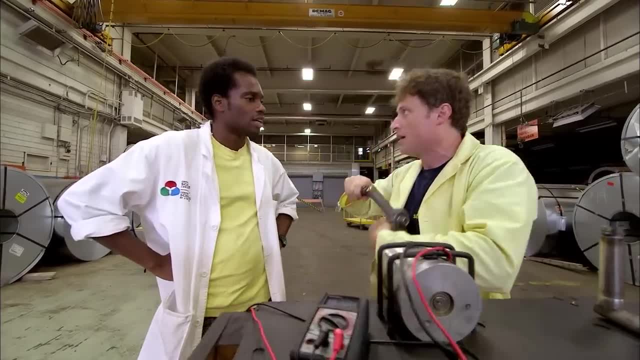 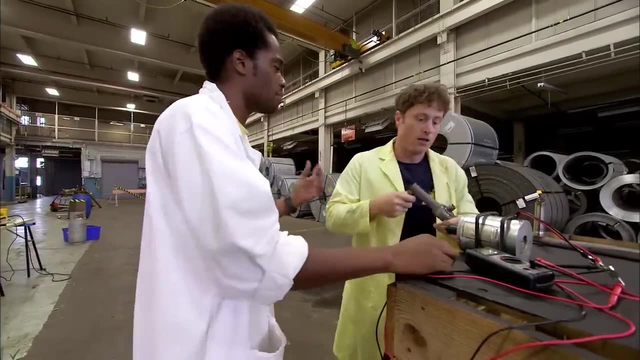 you can do. one circle here equals like ten circles on the other gear. Exactly, Yeah, Okay, so kind of like the gears on like a bike, Yeah, the gears on a bike or something like that. Yeah, Okay, All right. 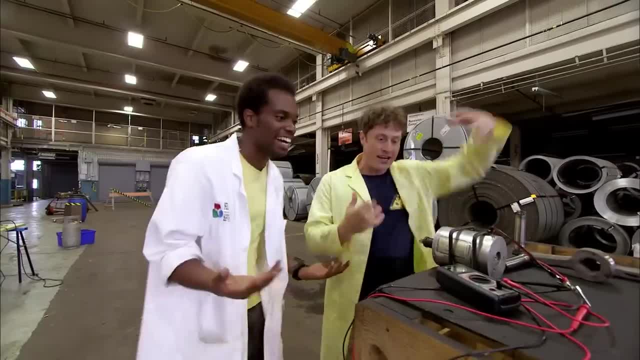 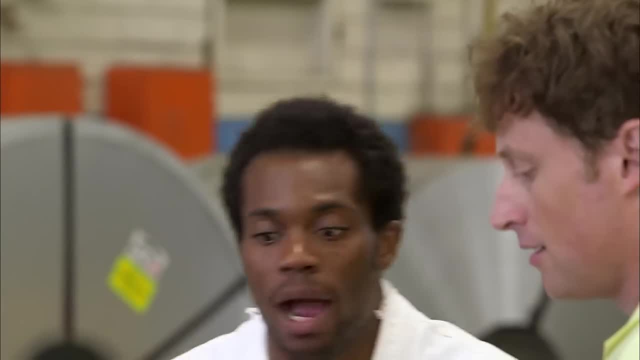 Let's see A bike, Of course. Yeah, so, okay. so we get a bike and we attach the back tire to the generator, The generator, and then you can use the pedals of the big gear to power the small gears. Okay, great. 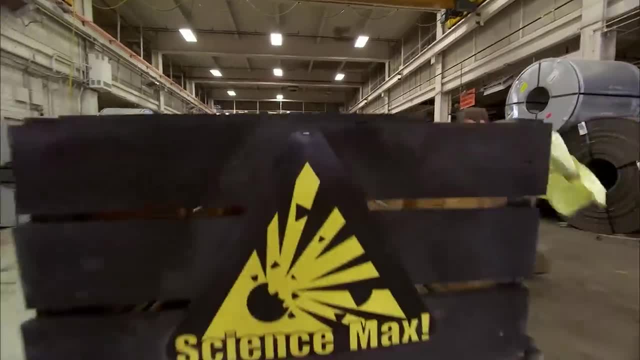 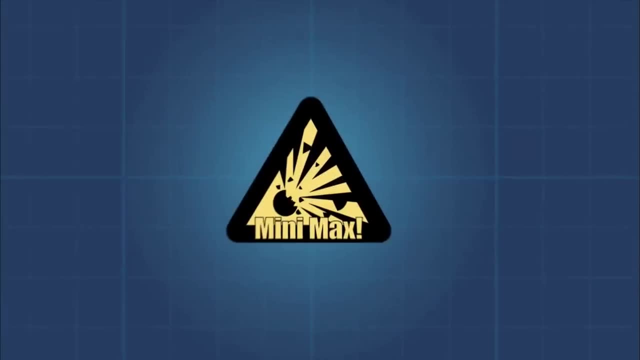 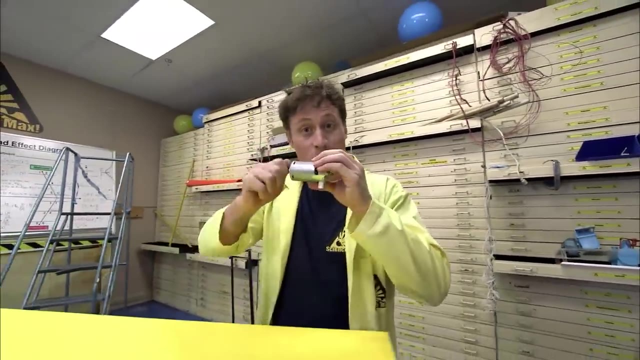 We'll go get a bike. Yeah Yeah, high five, All right, All right, Oh right, they're over here. This is a generator. It generates electricity when you spin it, But how does it work? What wizardry is inside? 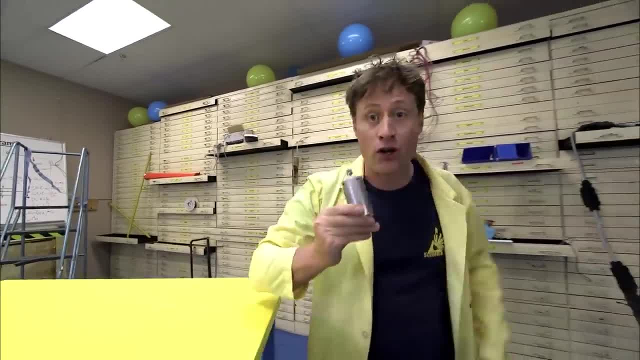 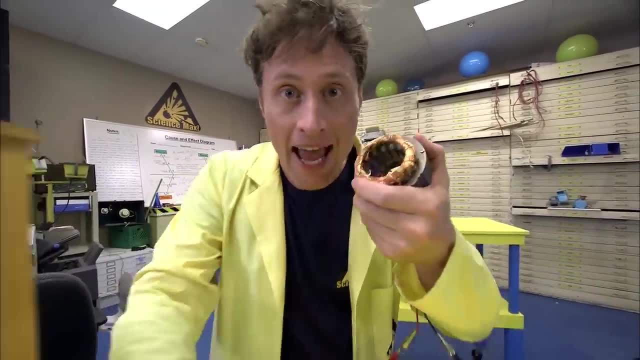 Well, actually generating an electric current is fairly simple. All you need is two things. First, you need a conductor, like this coil of copper wire, and you need a magnet. Now, this is a galvanometer. It measures small amounts of electric current. 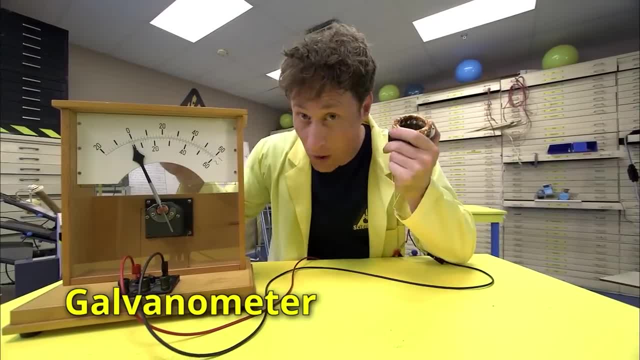 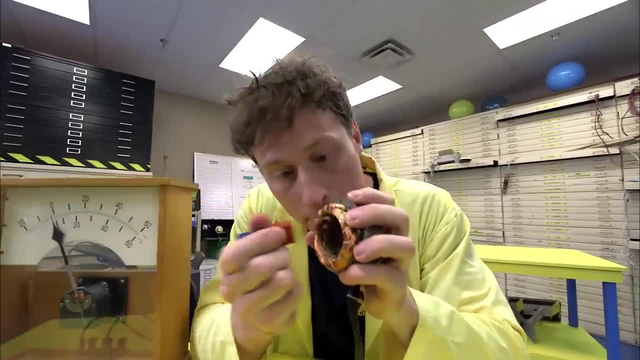 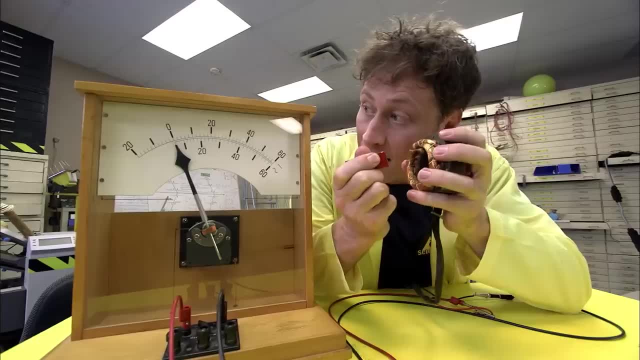 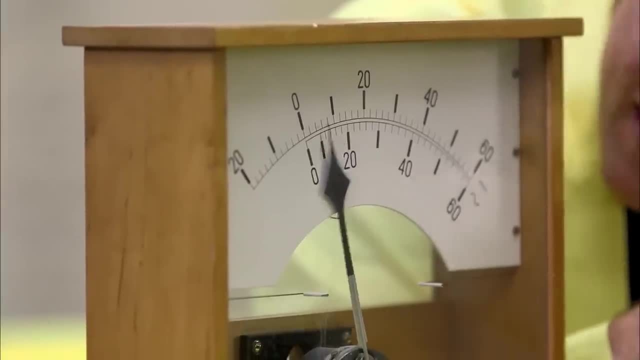 and out. it goes in the other direction A little bit going this way, and then I take it out a little bit going that way. Positive negative, Positive negative. This kind of current that goes back and forth is called alternating current or AC. 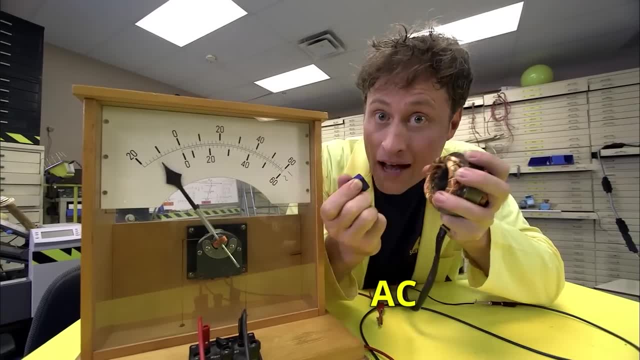 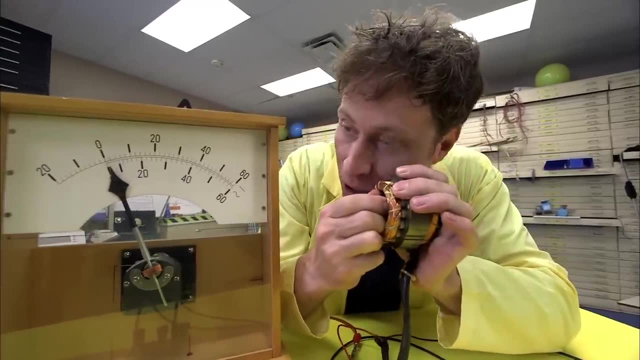 It's the same kind of electricity you have in your house. But here's the cool thing. Watch this: I put the magnet in and I leave it. It goes back to zero. You only get electricity when you move the magnet. All right. 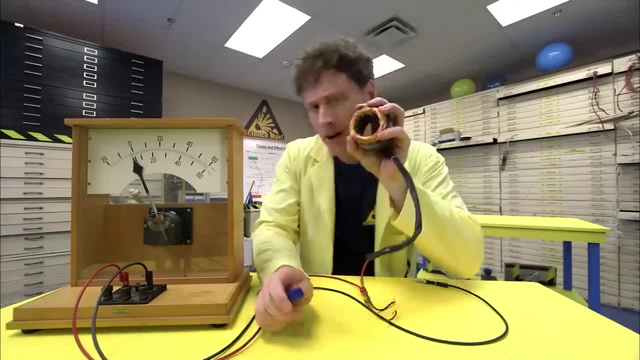 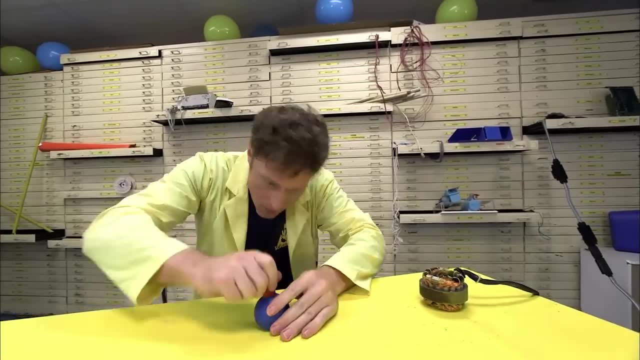 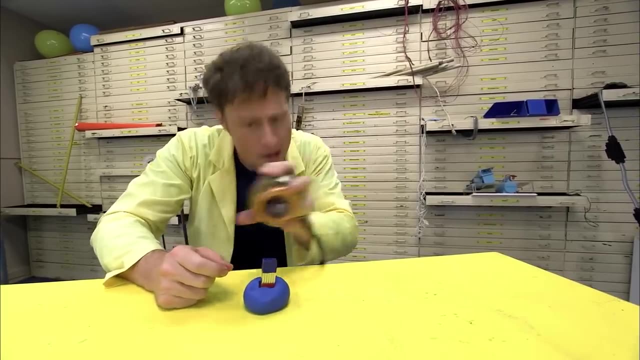 So let's create our generator Instead of starting with a copper coil like this. what if we just had the magnet and we have it staying still like that and we move the conductor past it like spinning? hmm, It's good but not great. 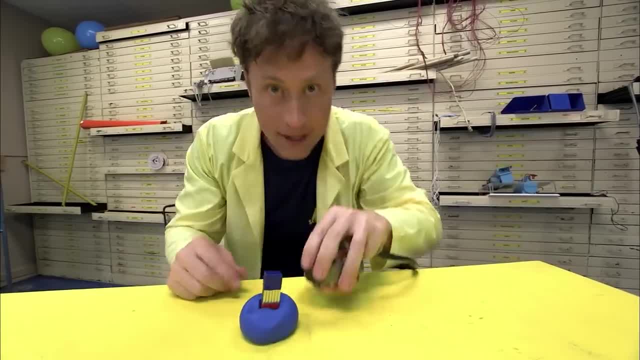 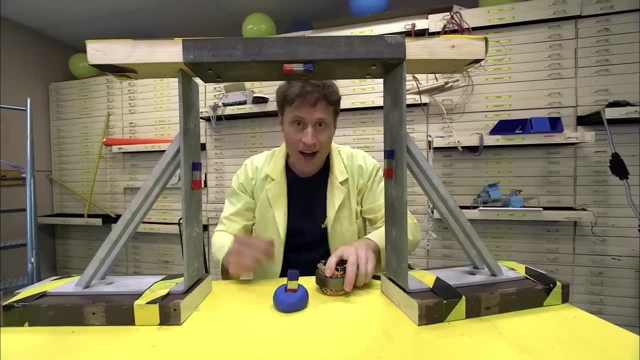 because we're only getting a little bit of electricity as it passes. so let's make it more efficient. Let's put in some more magnets, One on either side and one on the top- And now when we spin it, it goes past all of these magnets. 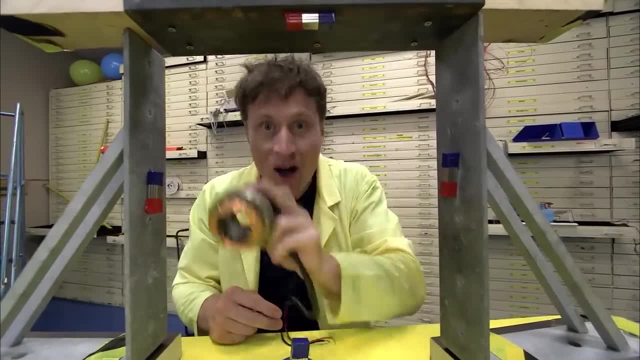 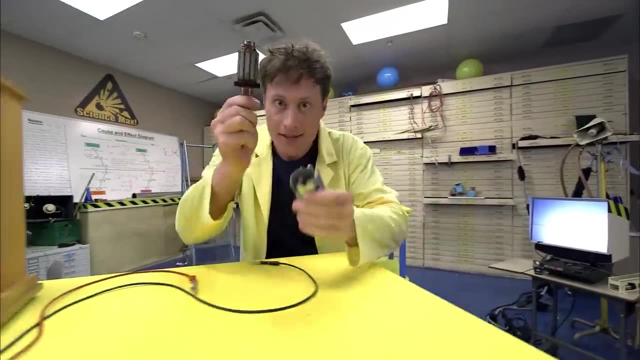 and every time we get a little bit of electric current. Well, this is how a generator works. If you take an electric motor or a generator apart, you can see there's a coil of copper wires on the shaft and it spins around like this. 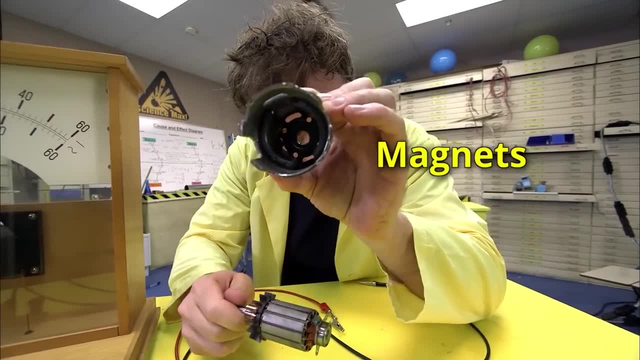 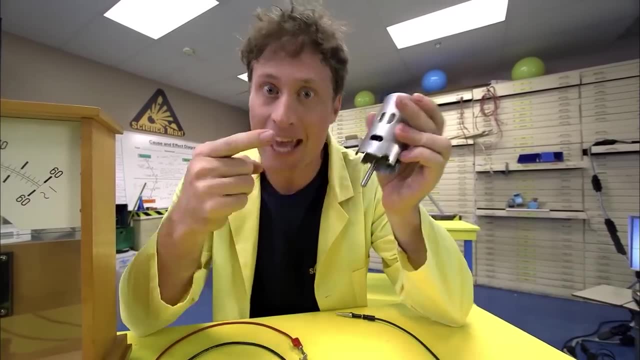 And on the inside there are magnets. so there you go. When you put it together and spin it, you get an electric current. Or if you put an electric current in it, it will spin just like an electric motor. And that is how a generator works. 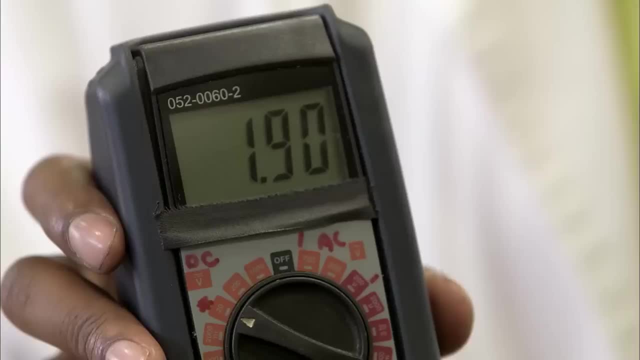 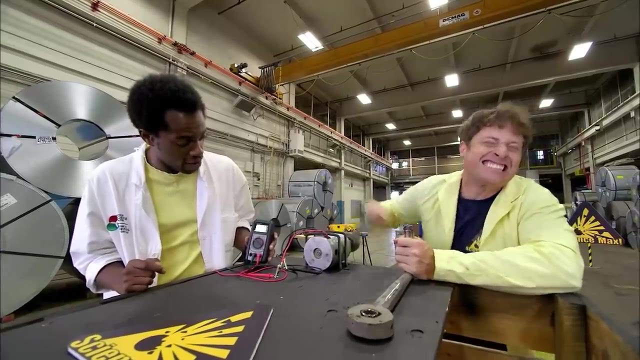 Anthony and I are trying to create as much electricity as we can using just human power, but so far it hasn't been going so well. It all comes down to how fast we can spin the generator. Maybe we could use like some gears or something like that. 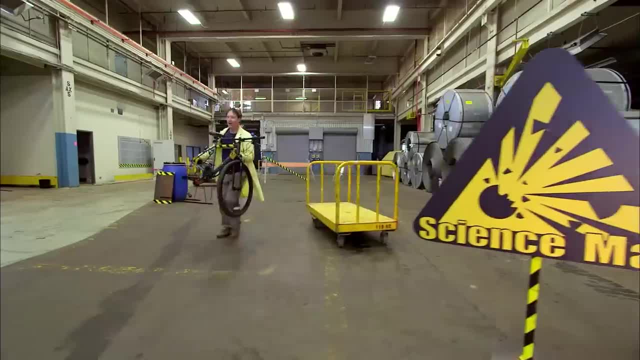 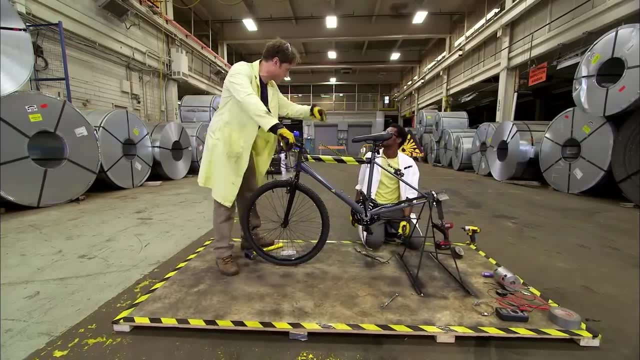 In order to get it spinning really fast, we're going to use a bike. It's just a matter of getting a bike, taking off the wheel, putting it on a stand and then putting it on a stand. It is now a stationary bike. 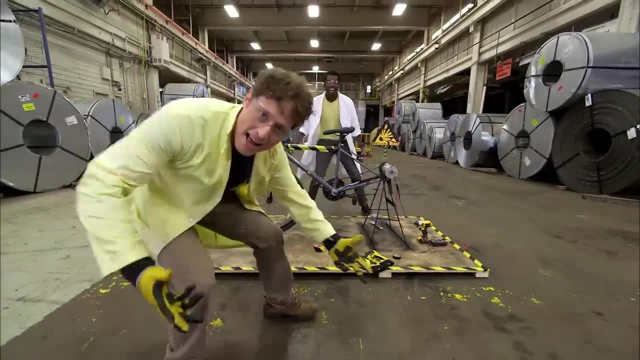 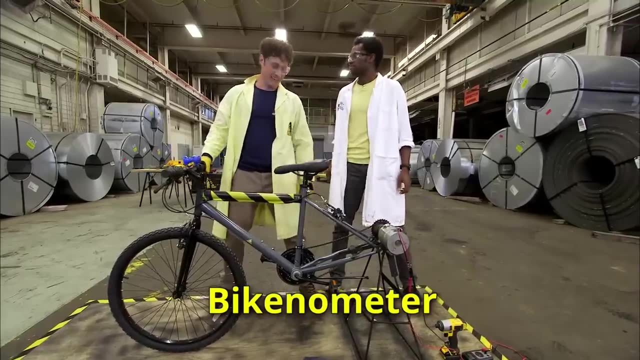 It'll be even more stationary once we screw it down And attaching the generator. All right, the bike generator, bike-er-ator- What should we call this thing? Bike-na-nator, Bike-no-mator- I like it. 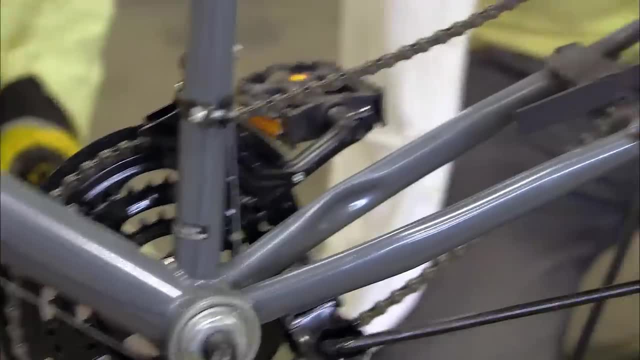 So, okay, let's go over what we've got here. Okay, so we've got two gears. We've got a big one, we've got a small one. We turn our pedals and the big gear turns the small one. 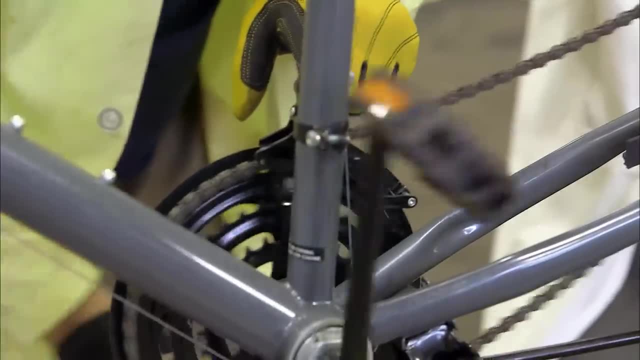 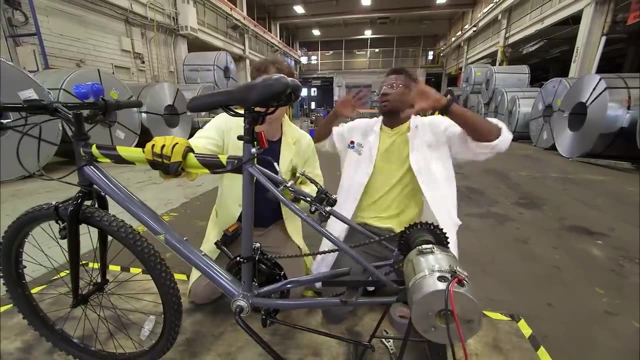 So this is the whole point of this build- is so that we can get one revolution here and we can get a bunch of spinning here. Exactly The more we get here, the more our generator spins and the more electricity we get. 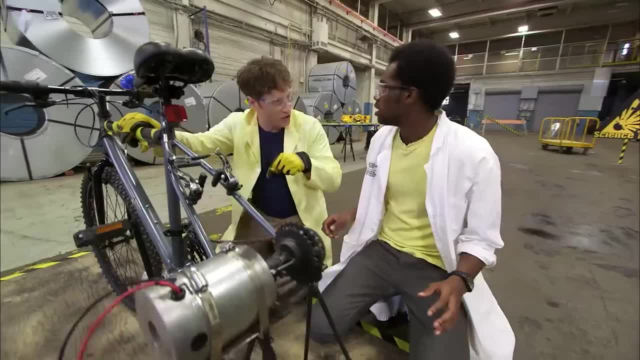 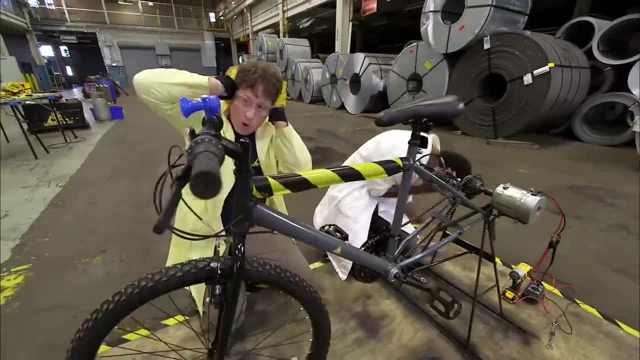 We get tons Awesome And obviously, using bike, because you're using your legs, Uh-huh, The strongest muscles in your body- Awesome, Uh-huh. Okay, so now what's with this horn? No, no, no, no, no, no, no. 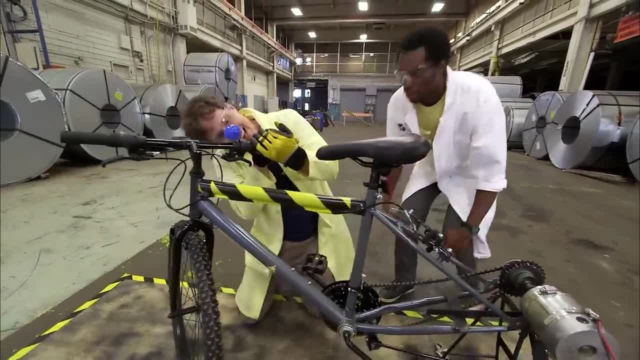 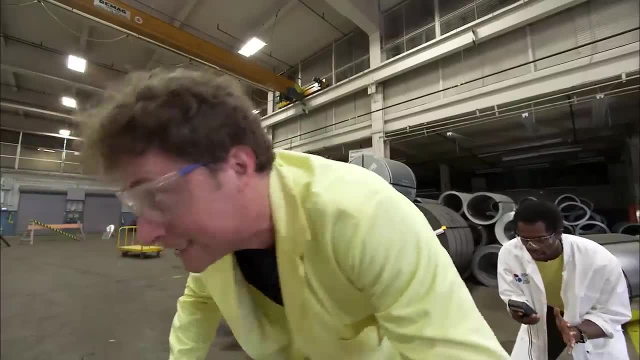 Oh, that is a loud horn, I know, I know. I tried to warn you. That is great, I love that. So Anthony and I hop on and give it a pedal. We pedal as hard as we can and we produce a pretty good. 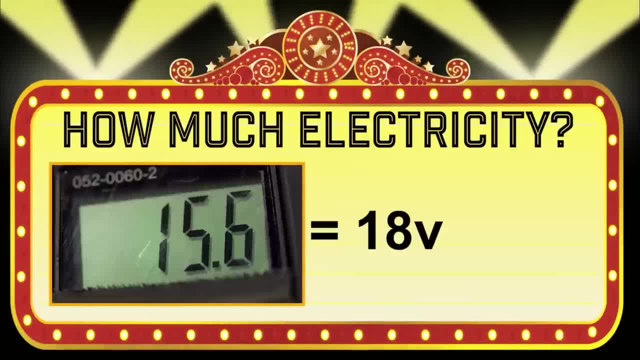 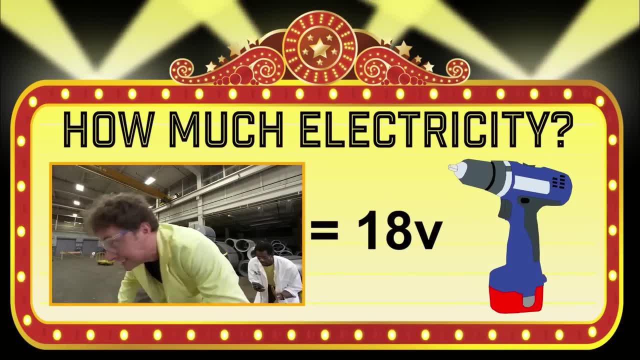 amount of electricity. How much electricity did they produce? We got up to maybe like 18 there. We did a pretty good job. That's enough for a power tool like a drill. It's good. You know what This works well, I think. 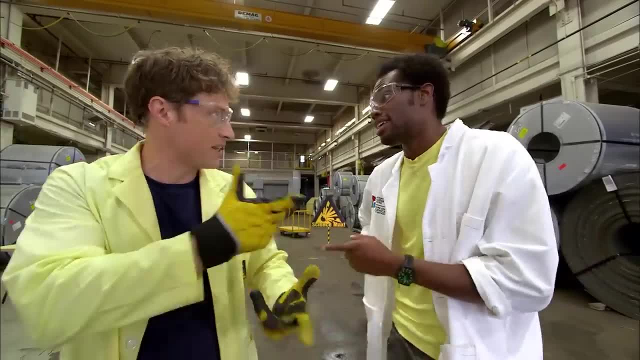 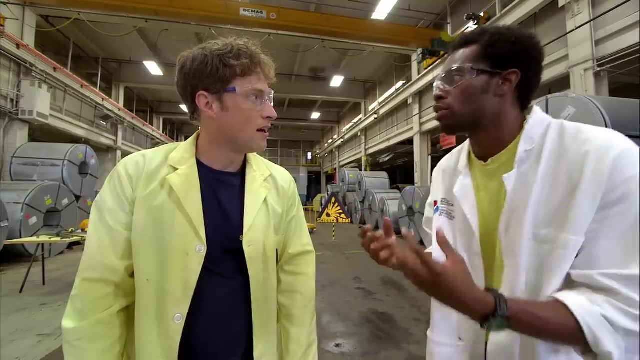 for keeping a good number for a long period of time. Yeah, So we can get up to like 18,, 20, but it doesn't, We can't really get any higher than that. Yeah, you know, what we need is like one really hard pull. 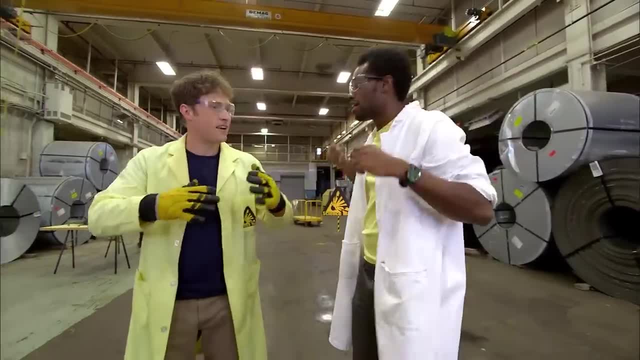 like all of a sudden. That way you can get like a spike. Yeah, you're right. You're putting all that effort into going for a long time. You put all the effort into one quick motion, Exactly. Yeah, good idea. 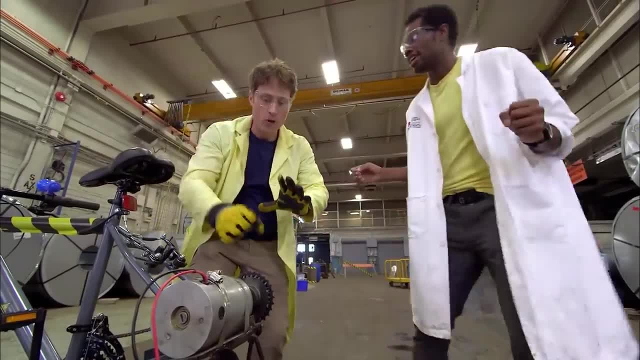 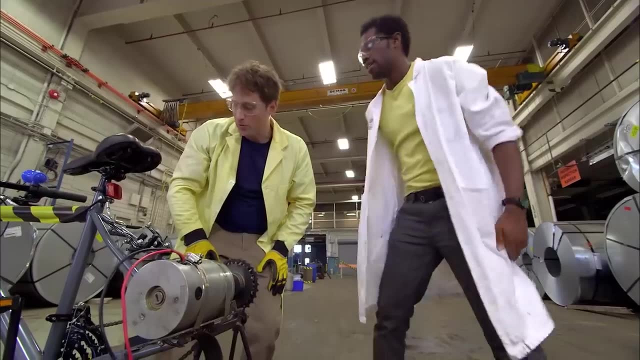 So you wrap a rope around here and then you just pull it Exactly, exactly, And that would be a really fast motion, Spin it really quick and get a very high number, High spike, exactly. Okay, You know we're gonna have to take the bike apart, though. 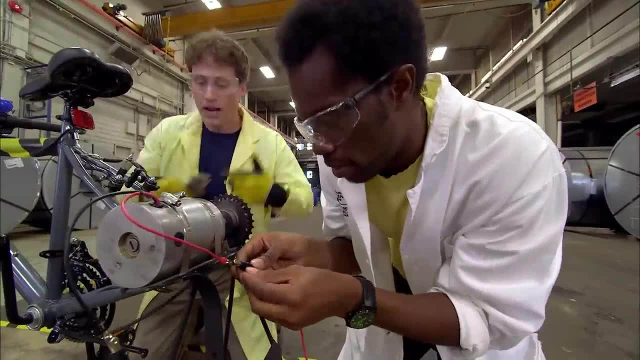 Okay, well. Well, it's science, Okay cool. Oh, you know what? We actually don't have to take the whole bike apart, We just have to take the generator off. Oh right, Okay, hang on a sec, I got it. 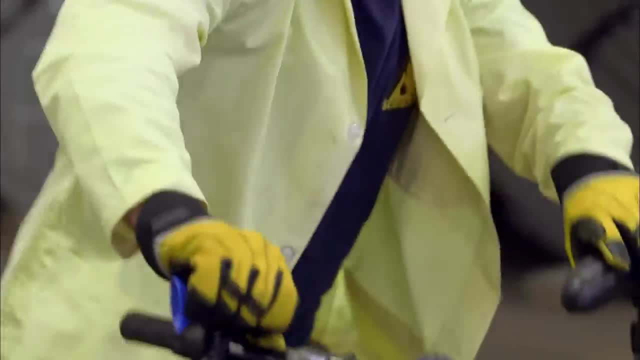 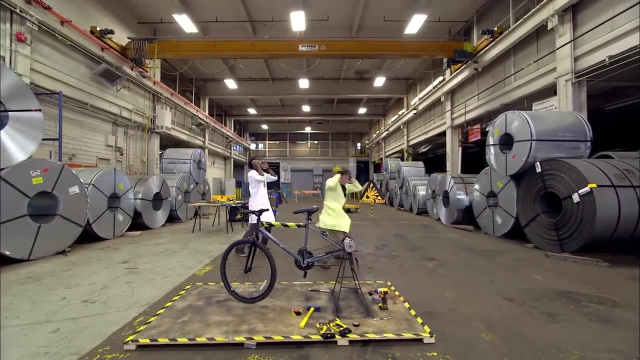 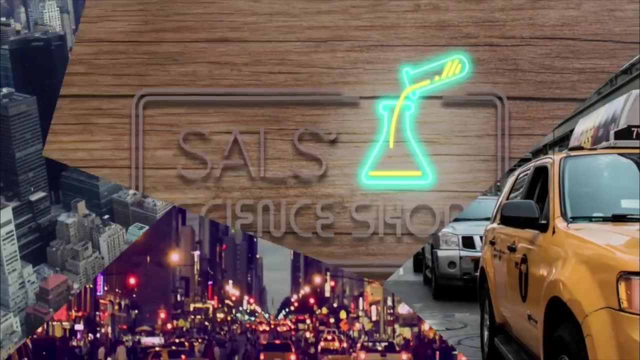 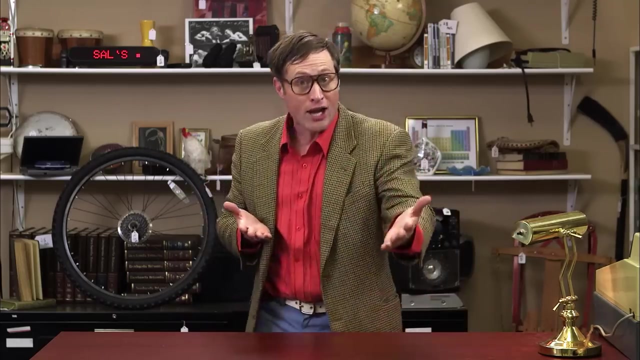 And maybe we should attach the horn to the next thing too. Oh, what are you? No, turn it off. Oh, you're great, It's so loud. So you want to generate some electricity. but what do you choose to generate that electricity? 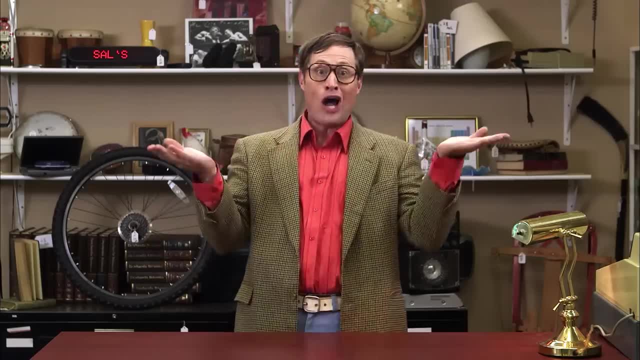 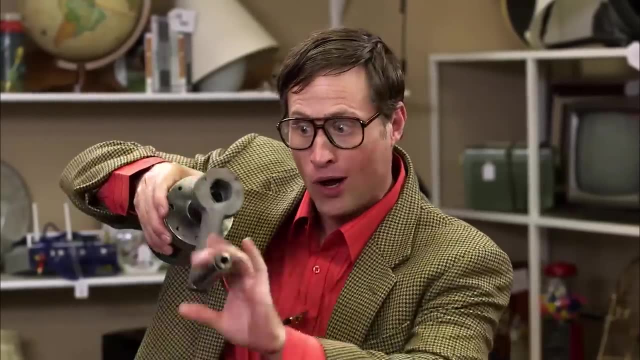 Hydro, nuclear, coal, solar. Who knows? I do, I know, And soon so will you. In order to generate electricity, you need to turn the generator. Turn the generator, One of the most common ways to turn the generator. 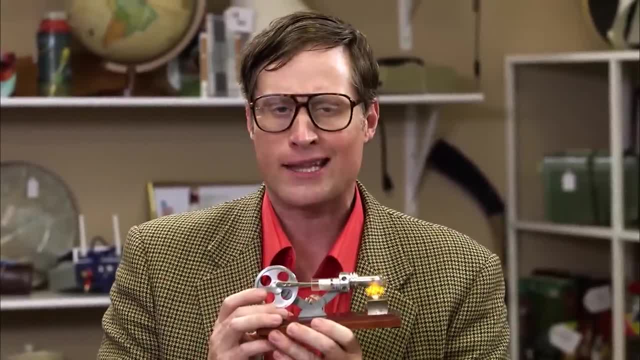 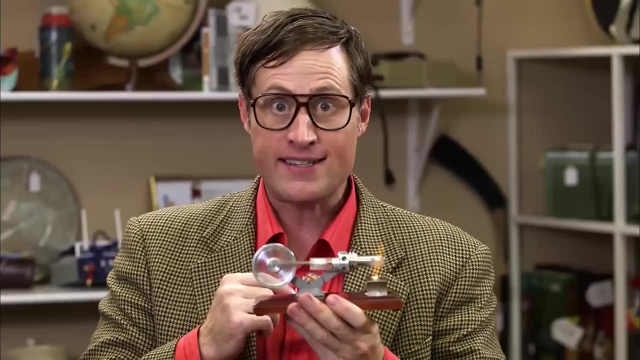 is to use one of these. It's a steam engine. Usually they're a lot bigger. You see, you heat the water to boil it and turn it to steam which works. a piston which turns the generator. Huh, Pretty amazing right. But what it really boils down to is heating water to make steam, Boil water to make steam to turn the generator. Coal power: Burn the coal to boil water to make steam to turn the generator. Natural gas, That's different, right. 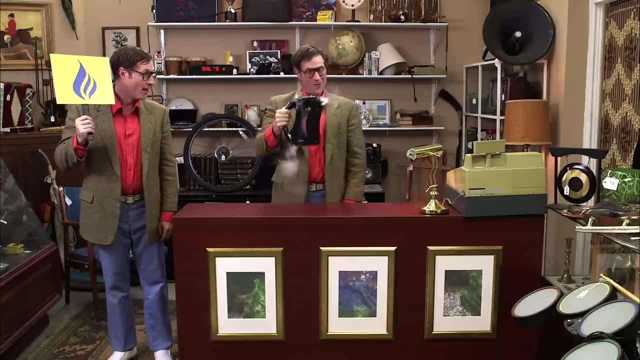 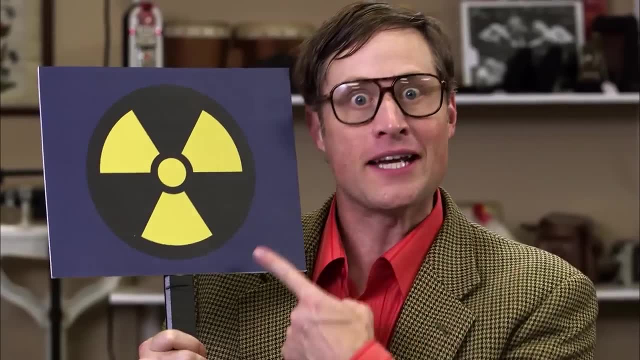 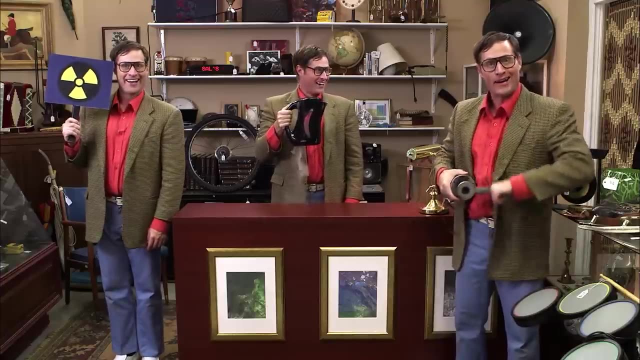 Nope, Burn the gas to boil water to make steam to turn the generator. Nuclear power: That's different, right? Nope, It creates heat which you use to boil water to make steam to turn the generator. Wind power: We don't even need heat for that. 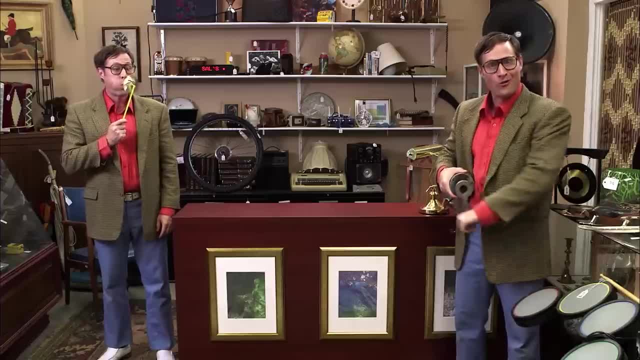 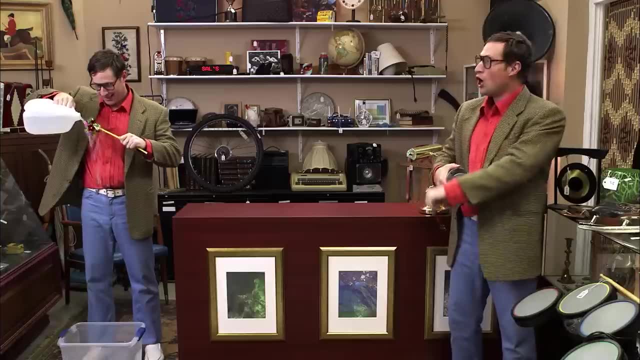 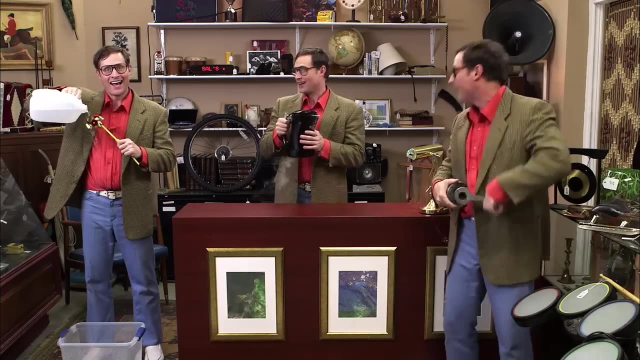 Just use the wind to spin the fan to turn the generator. Hydro power: Just pour water across something that spins to turn the generator. No matter what, making electricity always comes down to turning the generator. It's always yada, yada, yada yada. turn the generator. 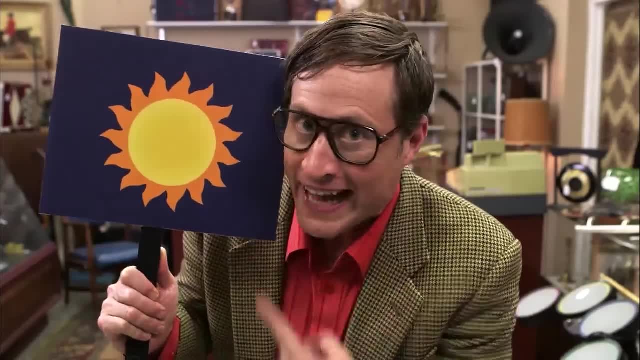 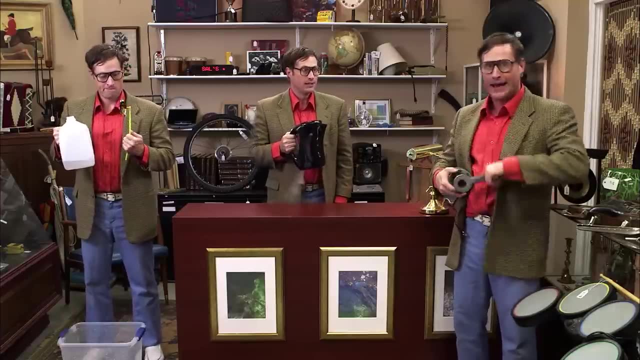 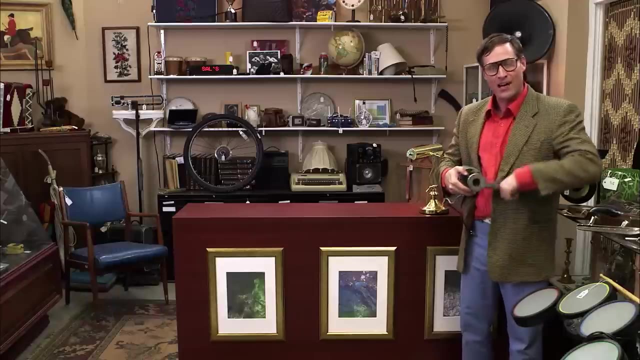 Except for solar. Solar does not work like that, But other than that it's always yada, yada, yada yada to turn the generator, And now you know your electricity generation. Hey, Ramona, you want to come and give me a hand over here? 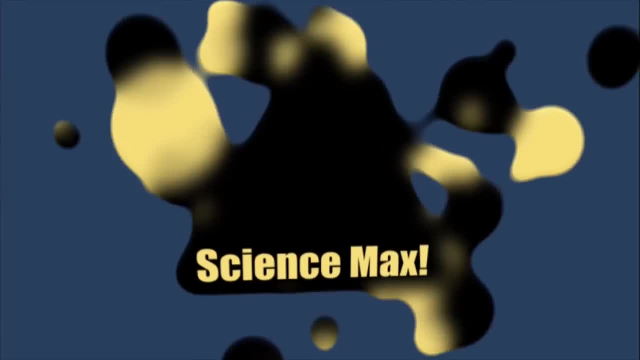 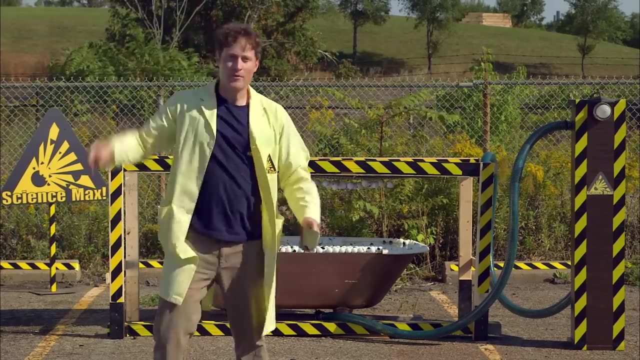 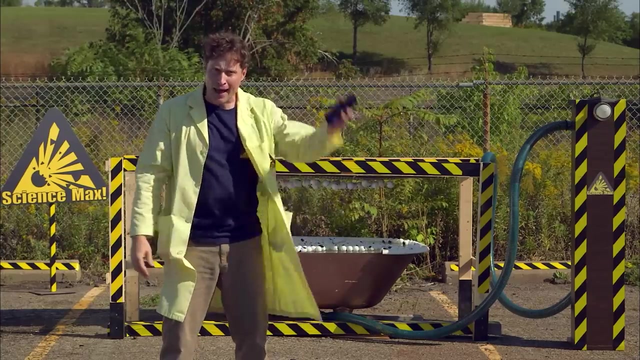 My arm is getting tired. Whew, it is hot out here. In order to generate electricity, you need to spin a generator. Most forms of electricity generation work like that, but not solar. Solar panels like this one generate electricity from the sun's energy. 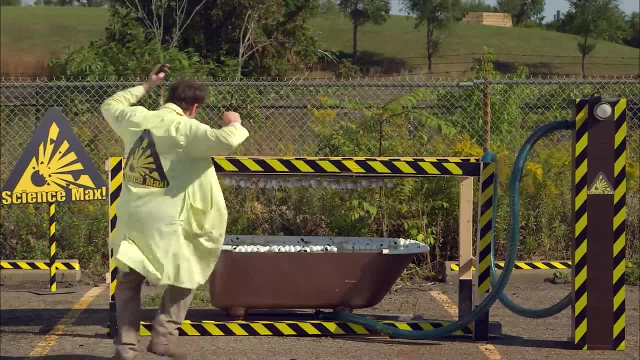 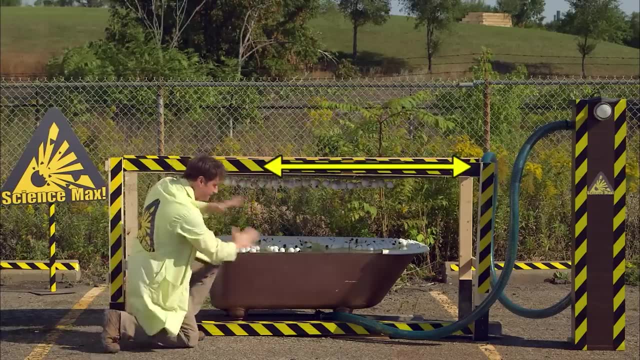 So how do they do it? Well, this is a solar panel. Okay, it's not really a solar panel, I just sort of put this together, but it works the same way. There are two plates, and on these plates are electrons. 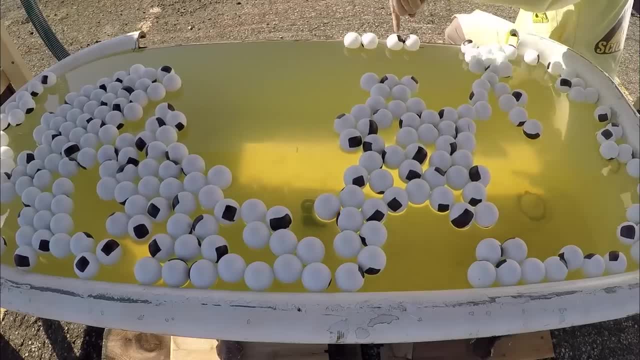 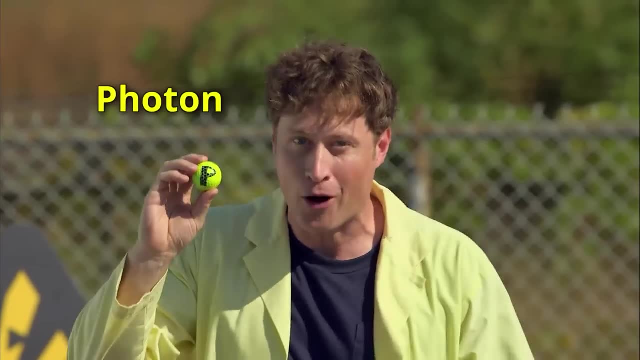 I've got golf ball electrons up here, ping pong ball electrons down here, but they're all the same thing. Now, this happy little fellow is a photon energy from the sun in handy-dandy particle form. What happens is photons come from the sun. 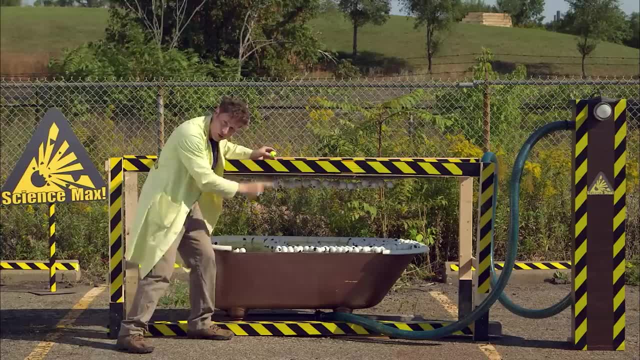 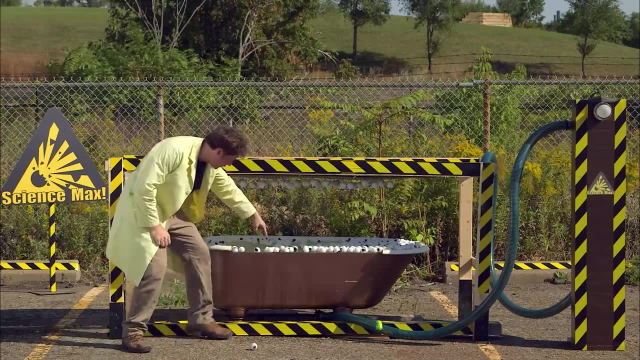 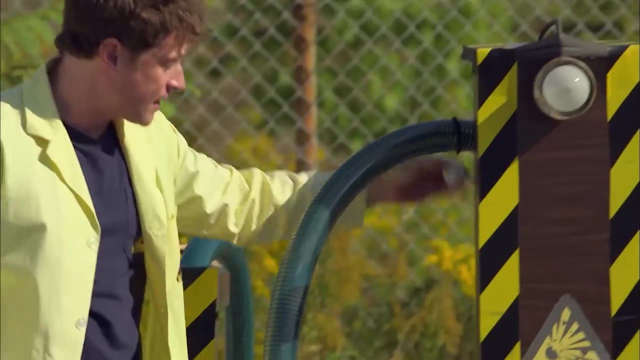 and hit the top plate and knock some electrons from one side to the other like this, And that knocks over some electrons. Now these extra electrons travel up a wire in the form of electricity and we can use them to do work for us. 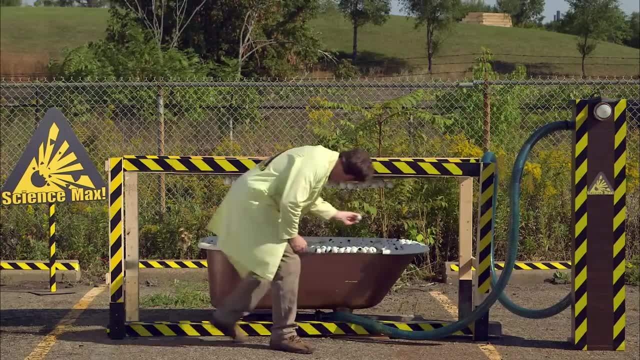 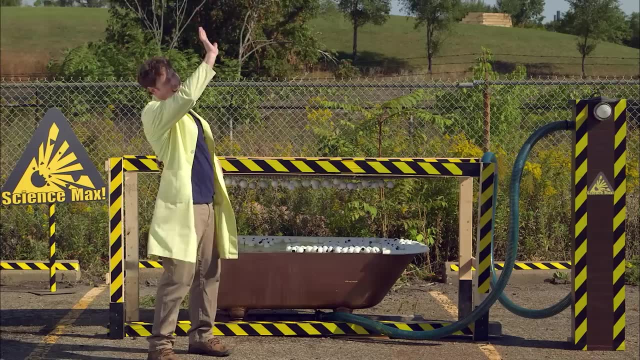 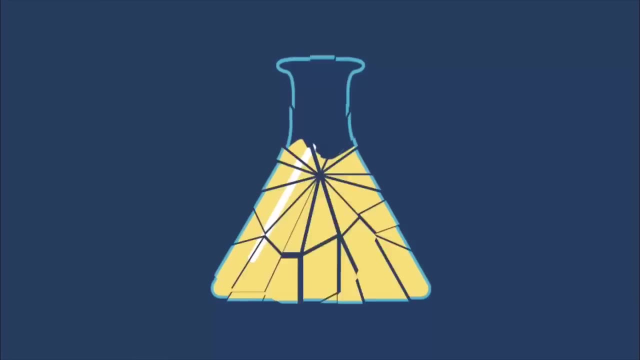 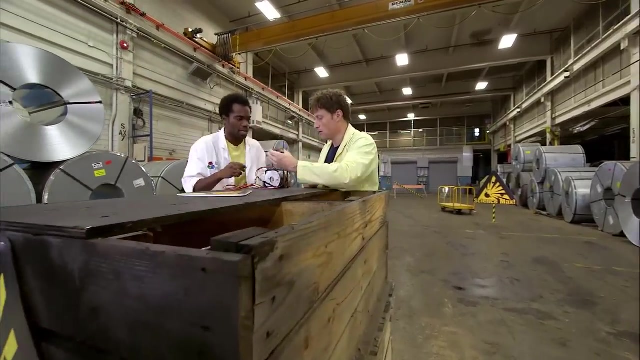 Then they change to the other charge, go back and we start the process all over again. That is how solar panels work, But remember it only works when there's sun and photons. Anthony and I are trying to generate electricity using human power. 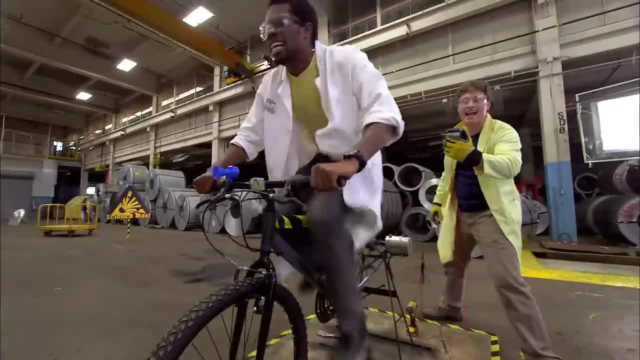 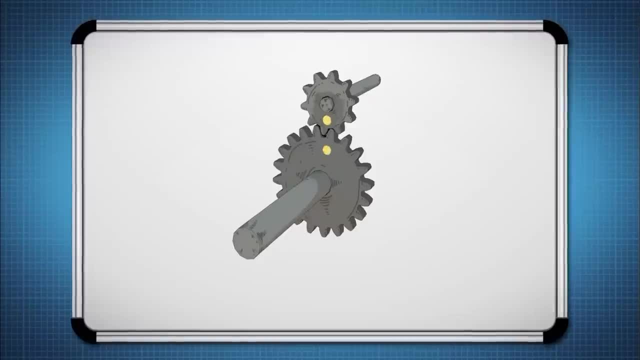 Spinning the generator didn't work too well, but we found if we use some gears like those on a bike, it worked better. You know, what we need is like one really hard pull, like all of a sudden Using gears is a great way to get work done. 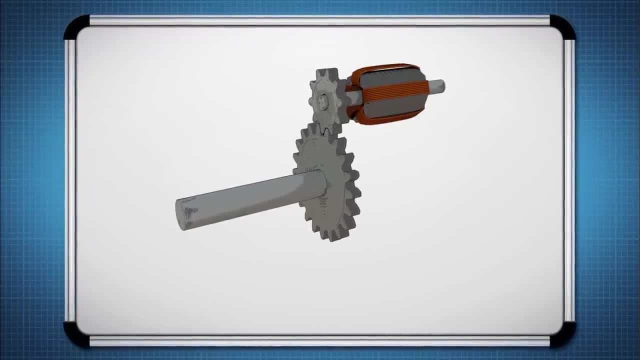 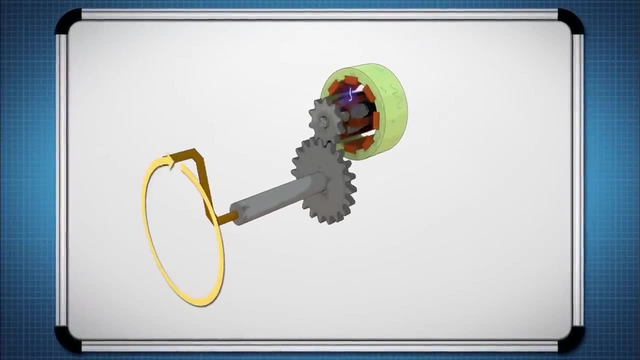 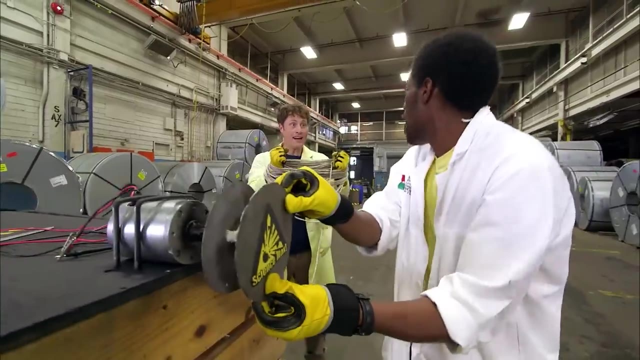 The good news is there are generators with gears already in them. That means if we can turn the spindle once, the gears inside will spin the coil a lot of times. The only downside: Turning the spindle gets harder the higher the gear. Anthony and I attach a spindle. 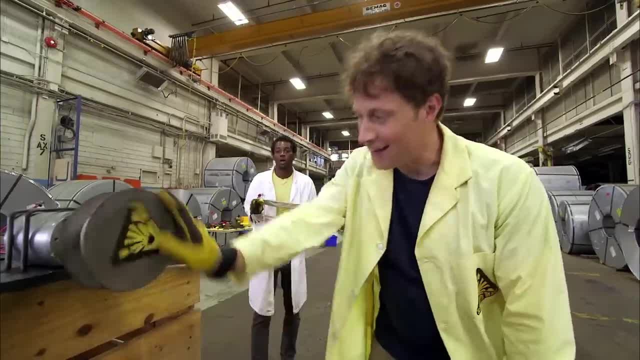 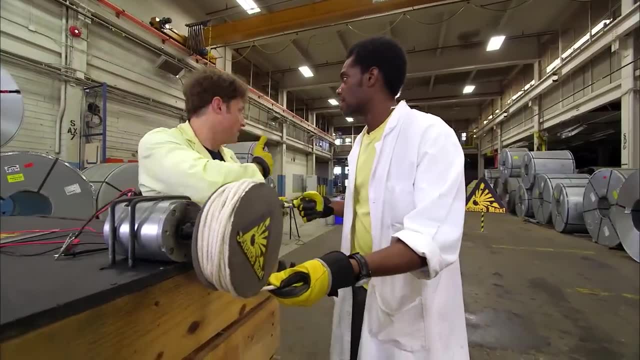 and then we wind up the rope, which takes a while. Okay, so the plan is: it's on a big spool now and you just run as fast as you can, Got it, And we'll hopefully get as many revolutions as we can. 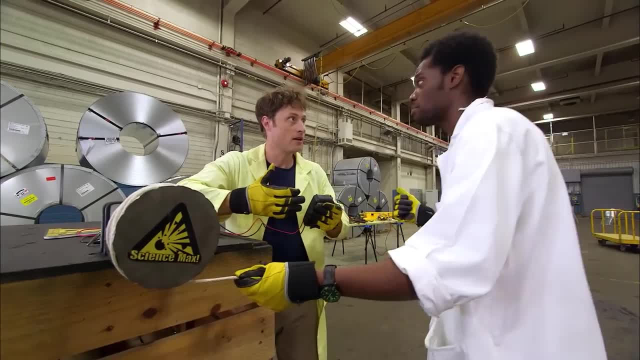 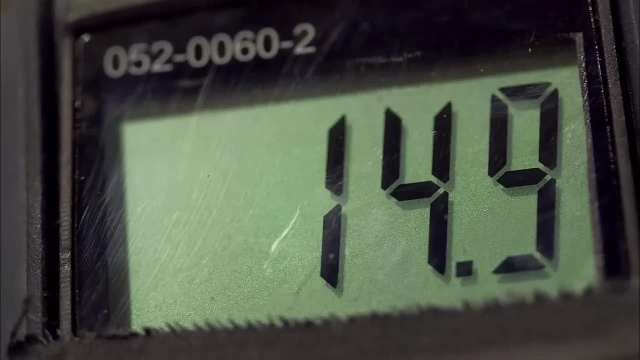 depending on how fast your top speed is. Okay, sounds good, Sounds good, I can be pretty quick. Okay, good, all right, Ready On your mark. Uh-huh Get set, Uh-huh Go. How much electricity did they create? 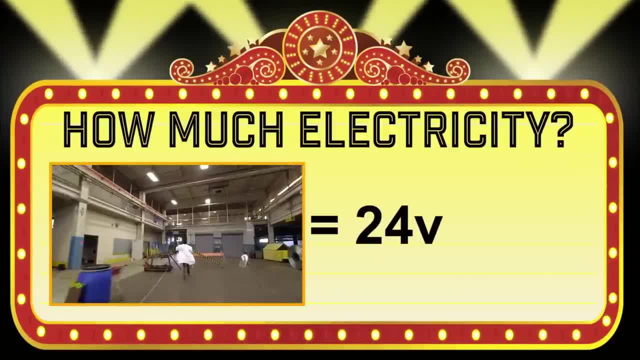 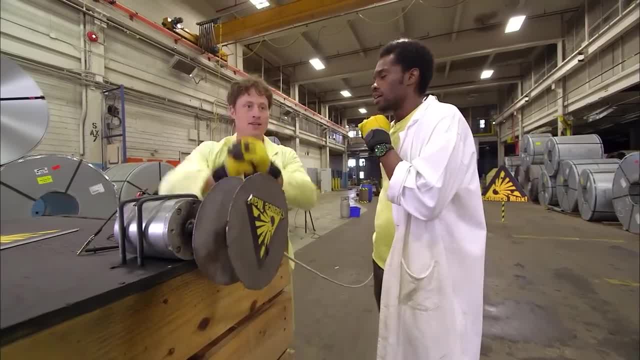 24 volts Actually not bad. That's enough to power their own personal scooter. Not too shabby boys. We need like a hard pull all at once. Yeah, something like really big. What if we could get like really high? 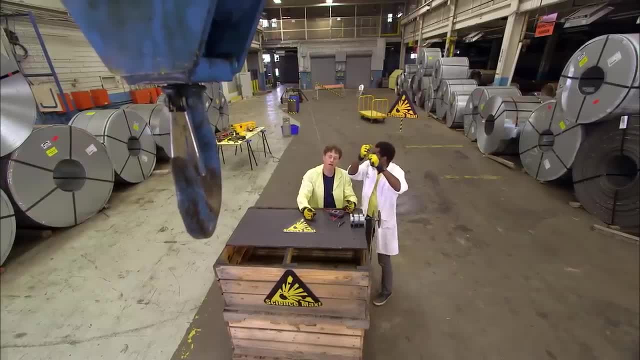 Okay, Like up there, Could we attach the generator up there? You could jump down from there, Um, and I would hang on the rope. Yeah, Yeah, that's good, but I don't want to jump from up there. 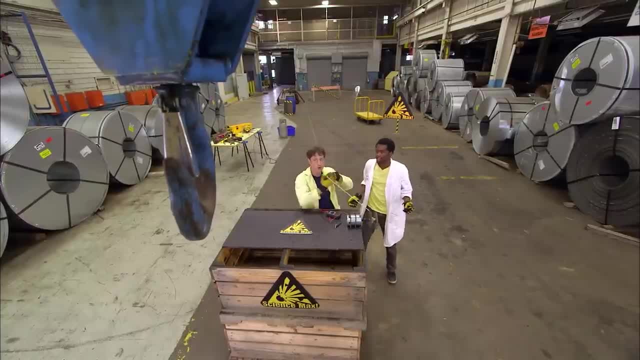 Um, oh, what if we put a pulley up there? That would work. And then the rope goes through the pulley and then back down, and then I jump from somewhere much safer, like just on top of here, And then the rope goes through the pulley and then back down, and then I jump from somewhere much safer, like just on top of here. 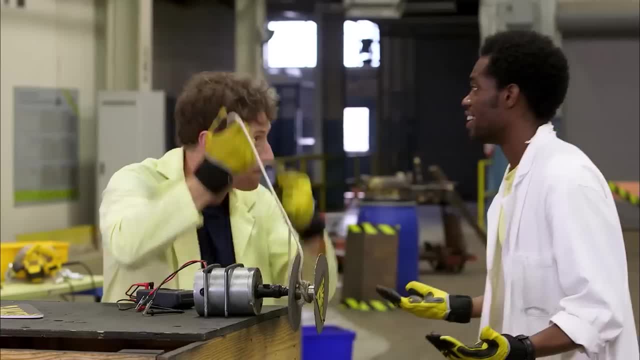 and then the rope goes through the pulley and then back down, and then I jump from somewhere much safer, like just on top of here, onto a crash mat or something. That sounds great, And that's my full body weight on the rope. 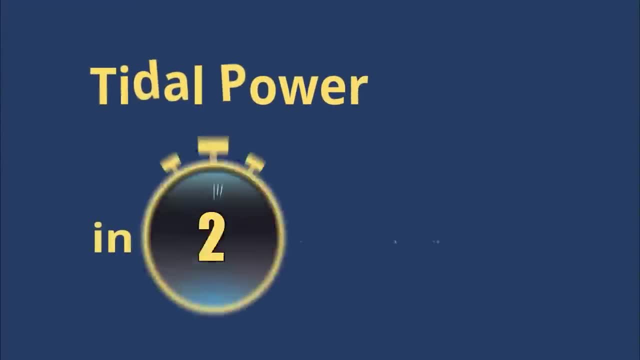 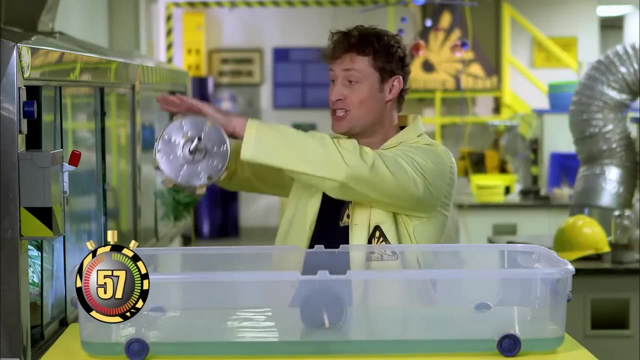 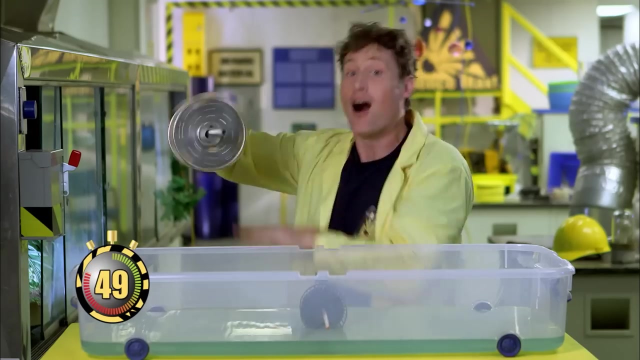 That sounds great. All right, high-fives, Yeah, Tidal Power in 60 Seconds. By now, you know that in order to create electricity, you need to spin a generator. Scientists and engineers are always coming up with lots of new ways to use natural forces of the Earth. 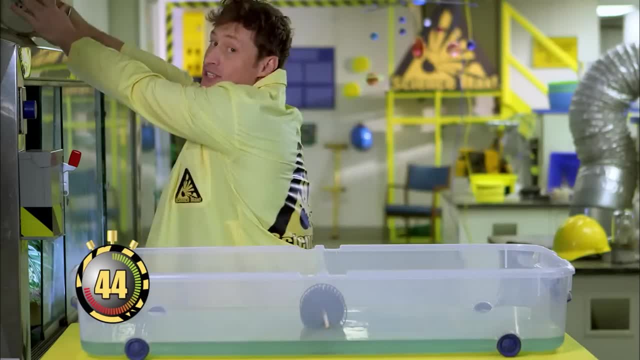 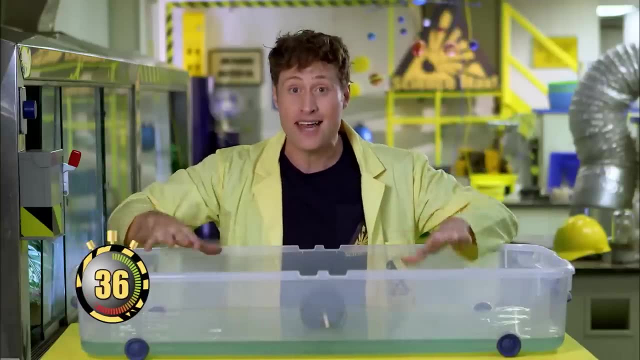 to spin a generator and create electricity. One of those natural forces. One of those natural forces. One of those natural forces is the power of the tides. You see, the water in the oceans doesn't stay still. Every few hours, the water or the tide goes out. 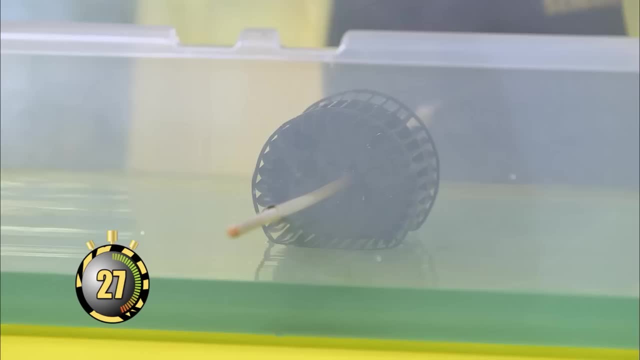 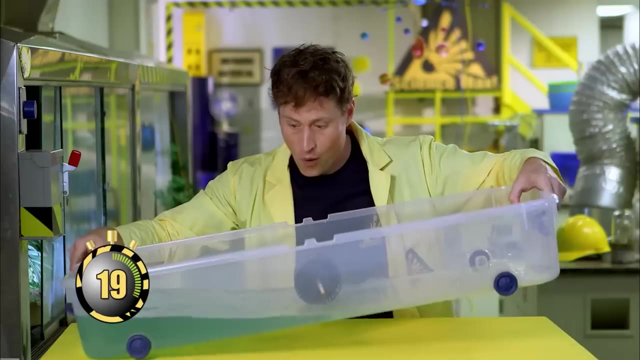 And then a few hours later it comes back in. So if you attach a paddle wheel in the water and attach that to a generator, when the tide goes out it creates electricity. When the tide comes back in, it creates electricity. That is how you create electricity. 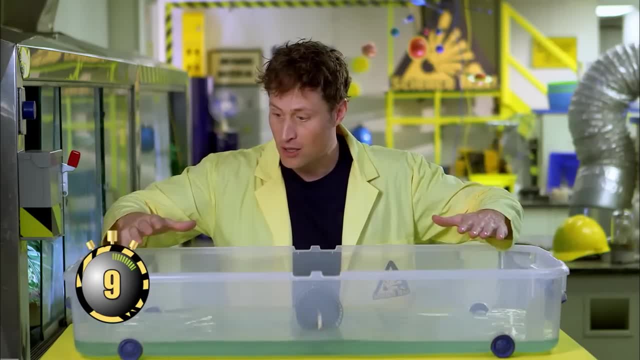 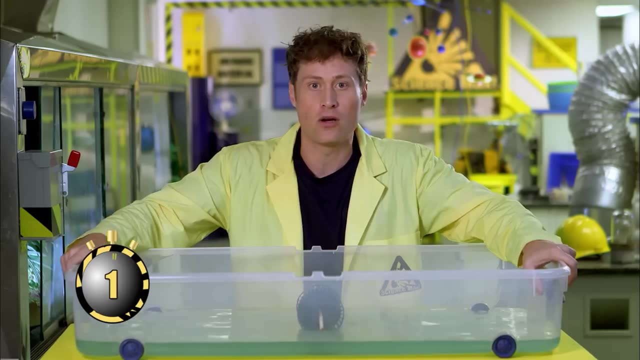 using the power of the tides. It's water power. Hydroelectricity is also using water power. Do we have time to talk about hydroelectricity? We don't have time, We don't. Okay, come back, come back. 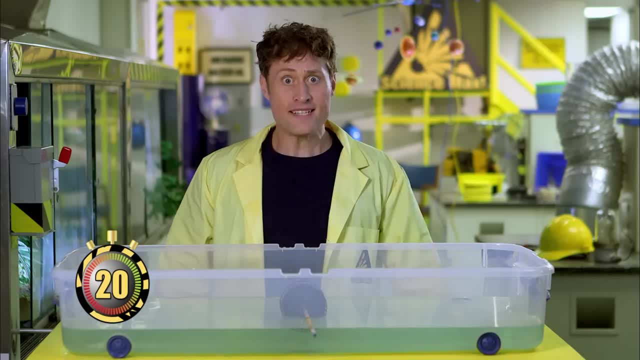 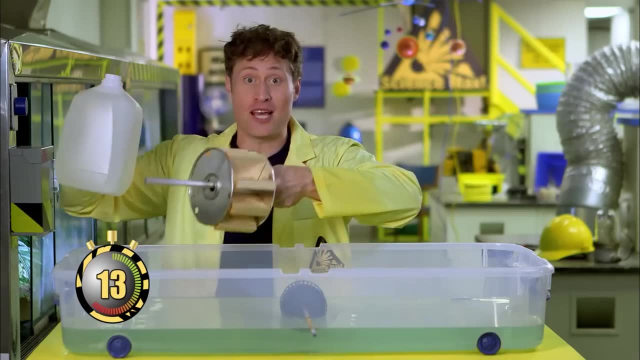 Hydroelectric Power in 20 Seconds. 20 seconds, Okay. hydroelectricity comes from water. Hydro means water, So all you have to do is find a place where water pours down from a height and you can put a generator in there. 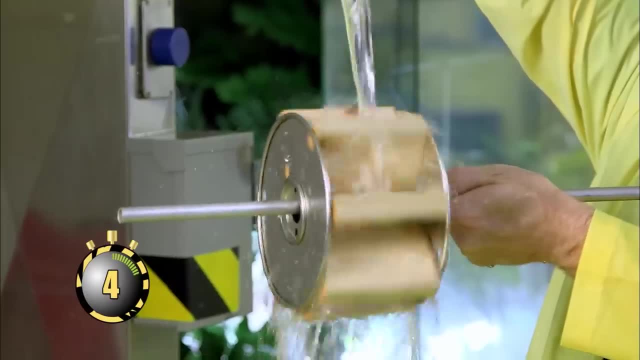 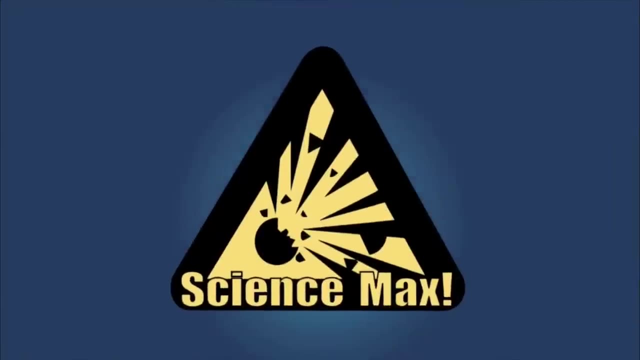 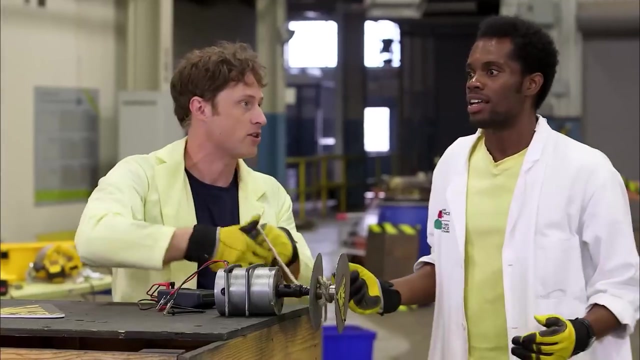 and ta-da, you're creating electricity with the power of hydro. Ha ha ha, I did it. Anthony and I have pulled and pedaled and now we're going to hang onto the rope and use our whole body weight to spin the generator as fast as possible. 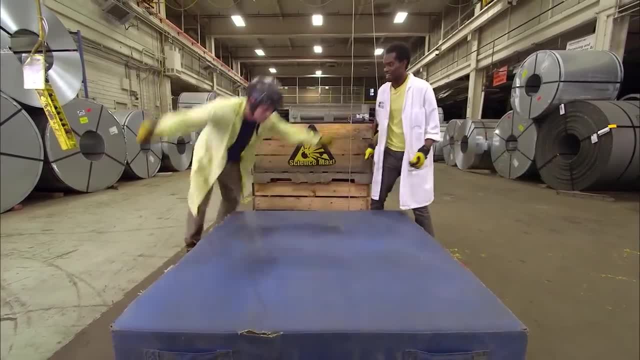 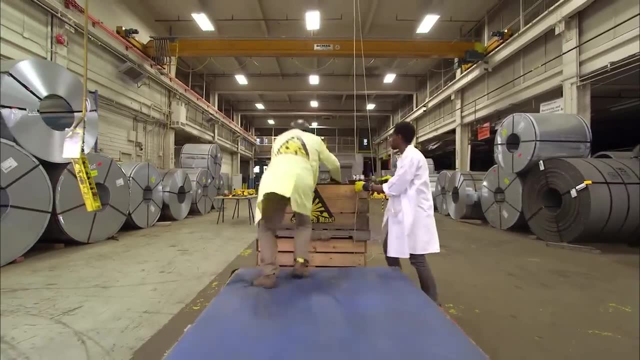 Okay, Okay, Crash mat. Uh-huh, Let me test it out. Looks good. Yep, it's good for crashing. So I go up here. Uh-huh, Okay, I go up here. Climb on up, We'll get you the rope. 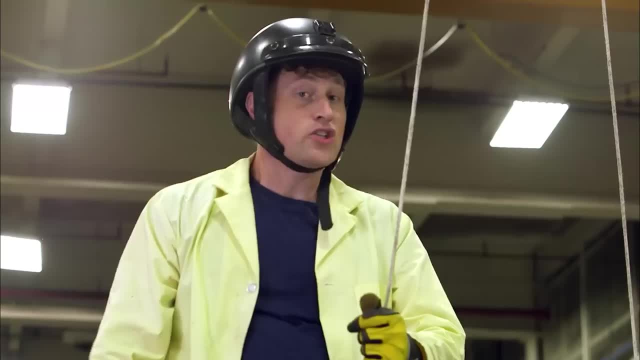 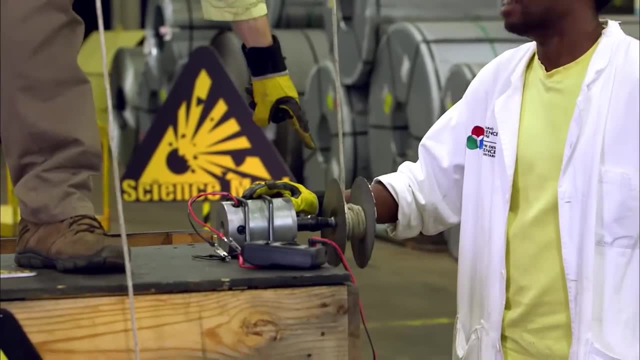 Got your helmet for safety. Helmet for safety, Crash mat for safety. So we have the rope and it goes up through that pulley and then back down to our generator with a spindle on it And as I fall, the spindle will turn. 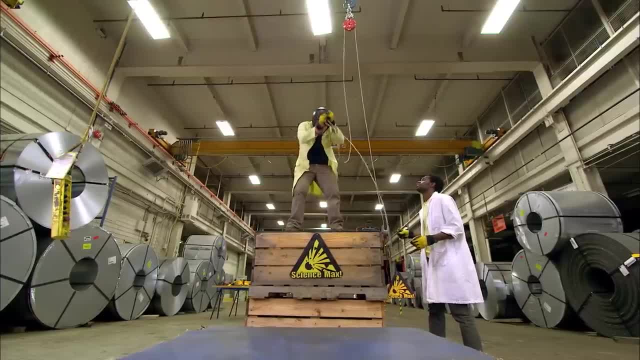 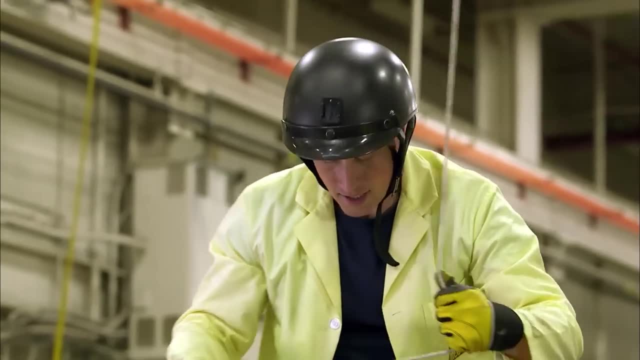 Exactly, And hopefully the speed of me falling and holding it and yanking it down as hard as I can will be the biggest spike of electricity yet. That's right, we'll be measuring it on our multimeter here. Okay, Okay, Ready. 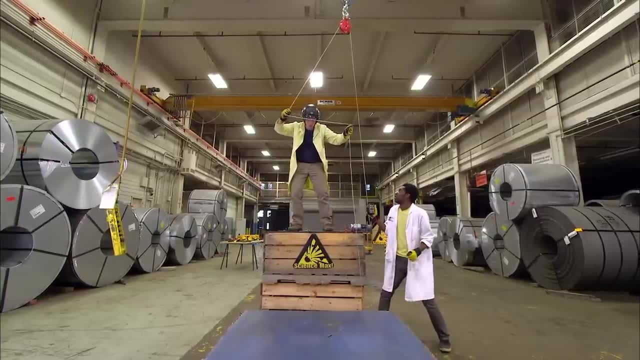 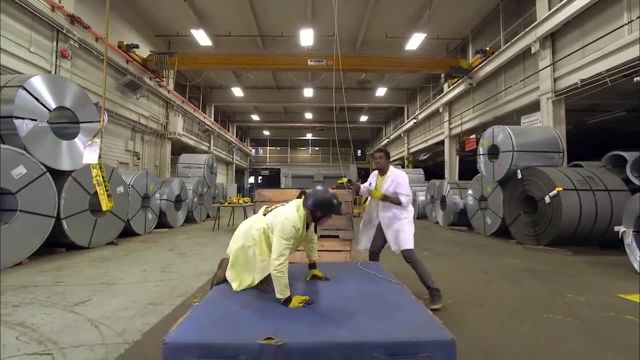 You ready? Yeah, Here we go. Three, two, one. I jump down and my whole body weight pulls on the line. Oh, that was awesome. That was like our biggest spike ever. That was amazing. All right, high five. 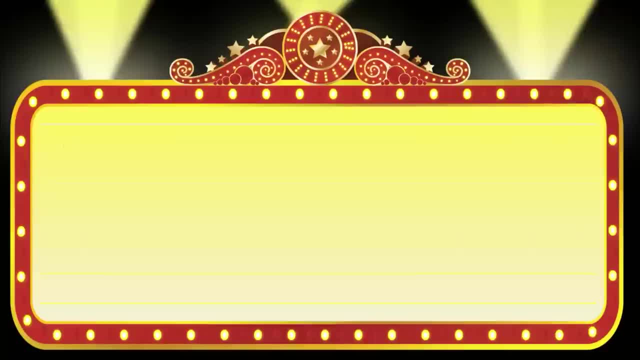 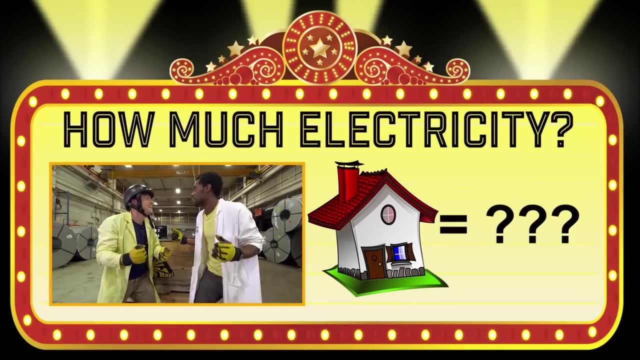 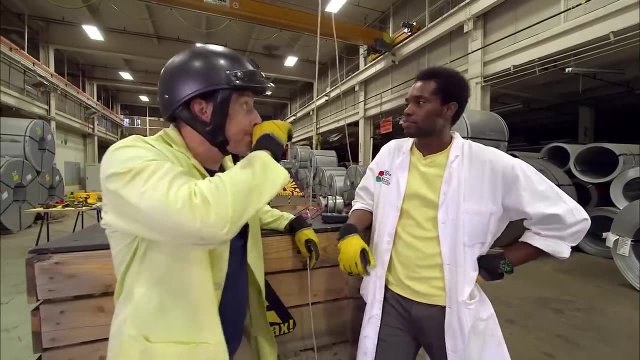 Biggest spike ever. Is it enough to power my house? Nope. How much electricity did Phil generate? Almost 30 volts. How much does he need to power his house? 120 volts. He's still off by quite a bit. Well, we've learned something: nuclear wind. 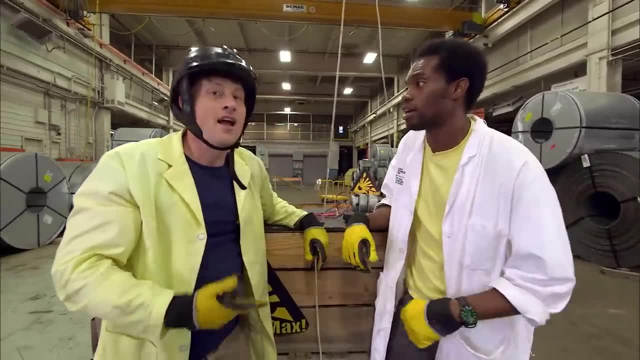 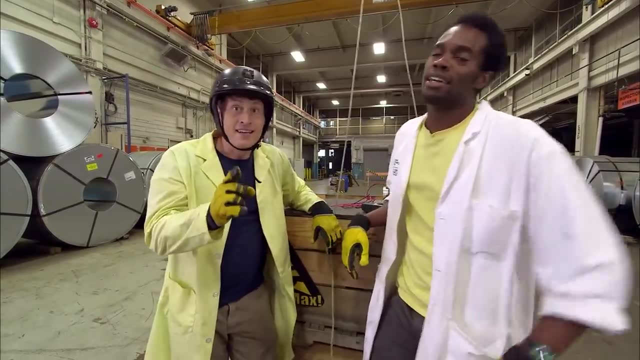 Hydro, Solar, Natural gas, Coal power- It's all great ways to generate electricity, Yeah, And human power not so much, Not as good, but human power is more fun, Yeah, way more fun, Yeah. so your turn. 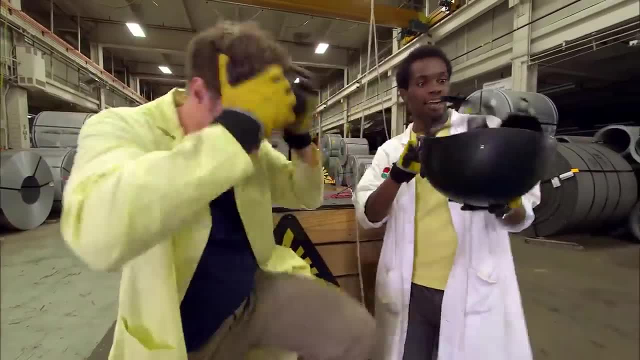 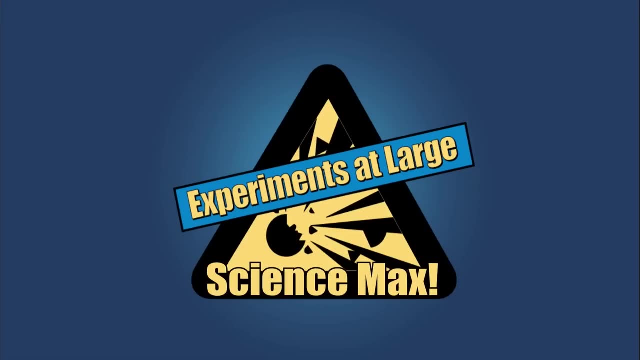 Yes, Okay, okay, You take the helmet and I'll take the multimeter, Okay, And then we'll go and we'll do it again, Okay, Okay, Wait, I gotta wind it up. Science Max. This episode of Science Max is all about hot and cold. 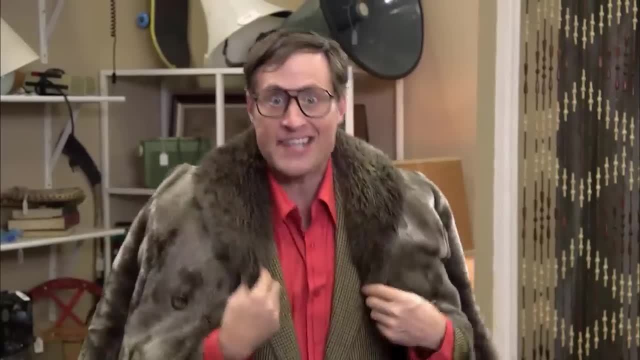 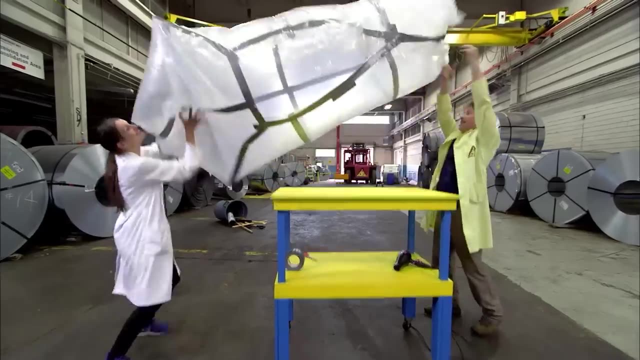 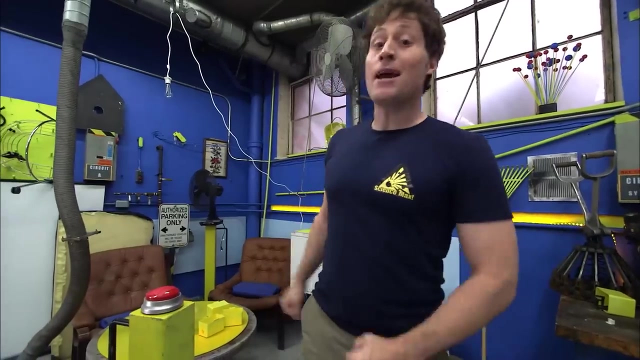 Hot air balloon, Dry ice, The coldest temperature possible, Absolute zero And whatever this is Blubber suit. All on this episode of Science Max: Experiments at Large Greetings, Science Maximites. My name is Phil and welcome to Science Max. 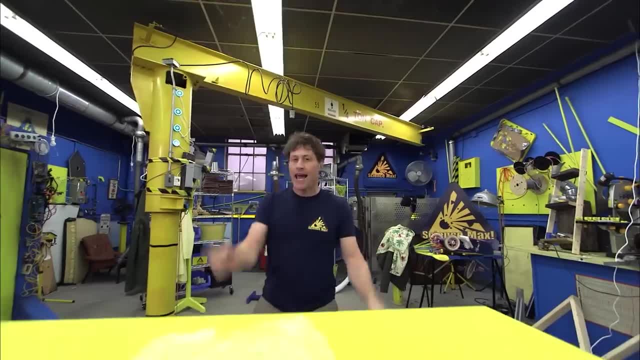 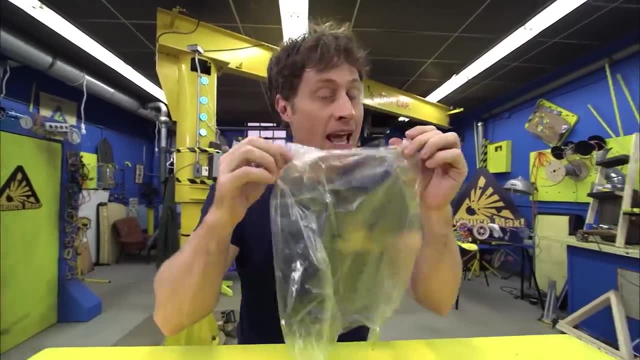 Experiments at Large. We're gonna be making one of the easiest and one of the hardest experiments to do. Here's what we're gonna make: A hot air balloon Pretty easy to make. That's why it's one of the easiest experiments. 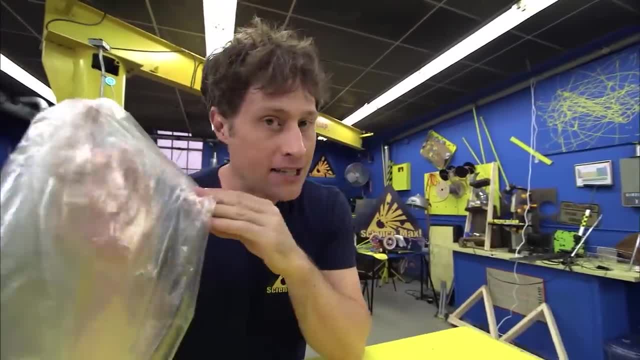 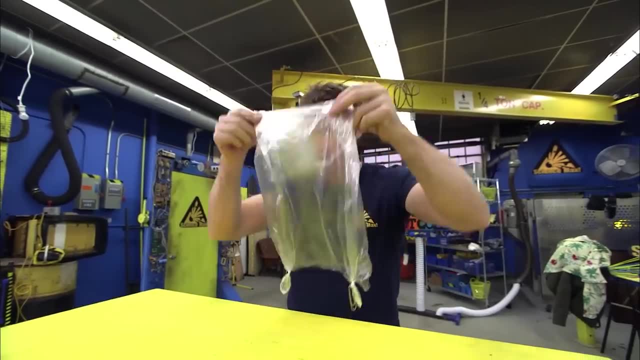 All you need is a plastic bag, but not any plastic bag, The kind of plastic bags you get at the grocery store to put your fruit in. That kind of plastic is very thin, very light, Good for hot air balloons. And you just wanna put two paper clips. 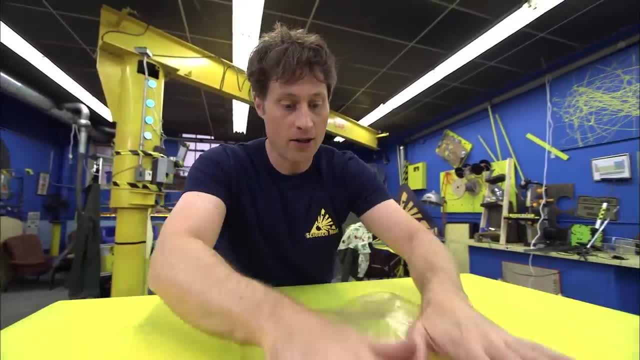 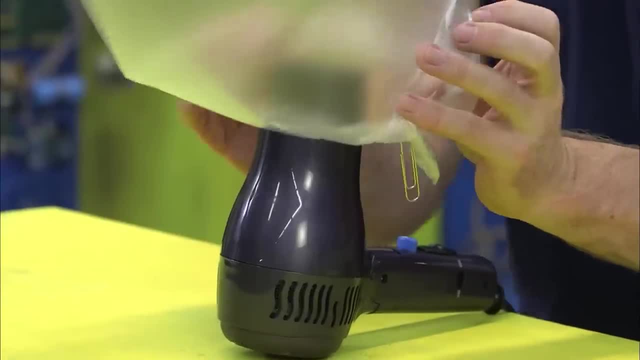 on the bottom of the bag to hold the bottom down. Now here's the other thing you need. You need an adult and a hair dryer. Turn the hair dryer on, Put the heat on the highest setting and the fan on the lowest setting. 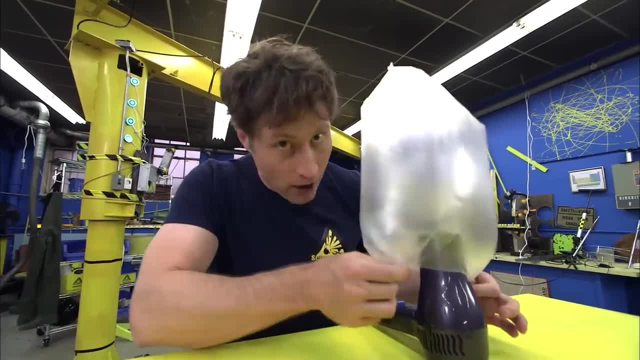 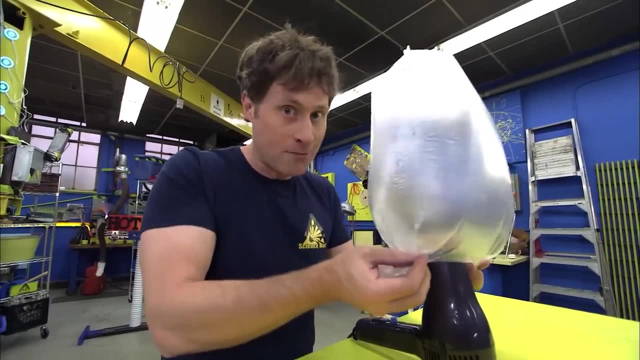 The air inside the bag is getting hotter, which means the molecules are moving faster and they're getting further apart, which means there's going to be less of them in the same space. Less molecules means less weight, and that means it's going to be lighter. 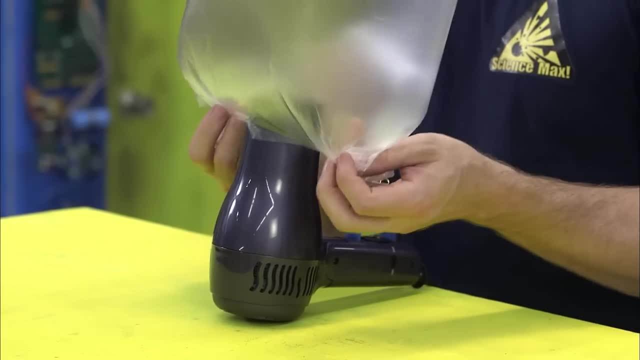 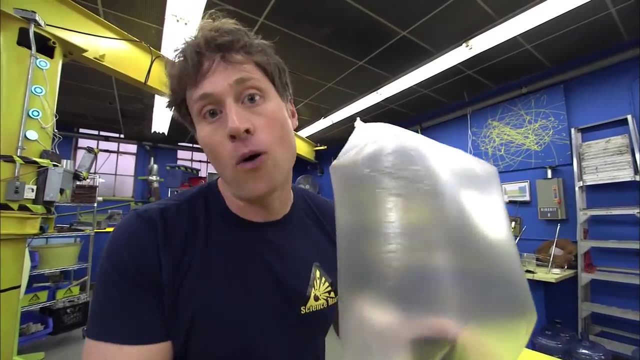 The bigger the difference in temperature between the air inside the bag and the air outside the bag, the better it's going to work. So I recommend doing this outside actually, on a cold day. When it's been long enough, turn the hair dryer off. 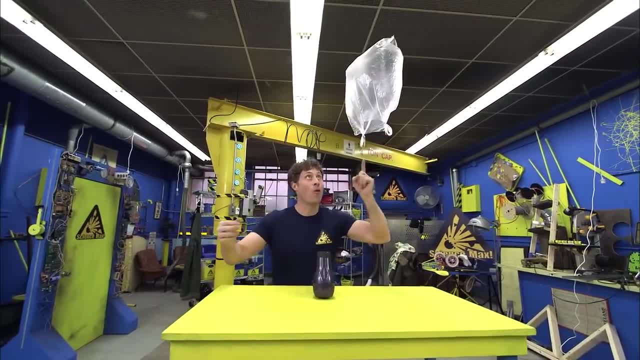 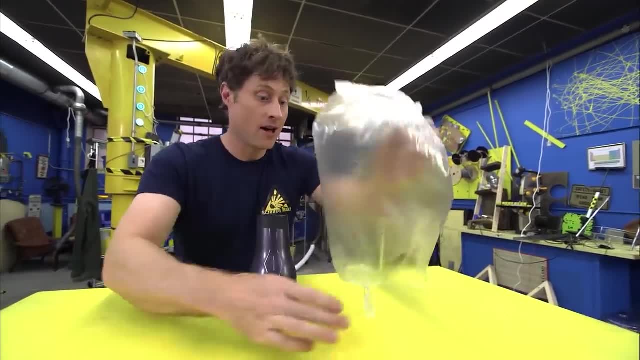 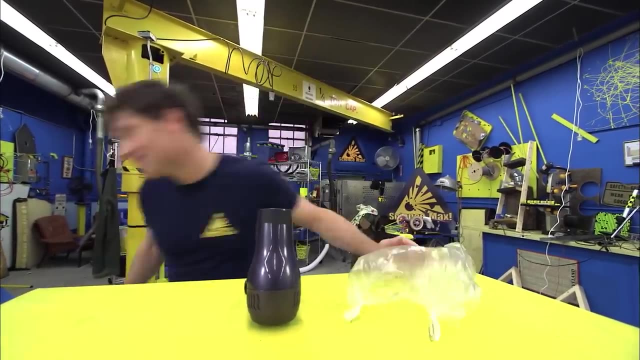 and it will work. It will float, Ha ha. Now, it won't float very long because the air inside the bag will quickly return to its original temperature and it will no longer be any lighter than the air outside the bag, But it's definitely fun to fly for a while, while it lasts. 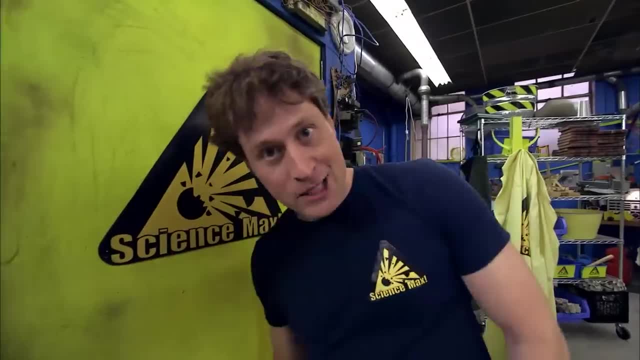 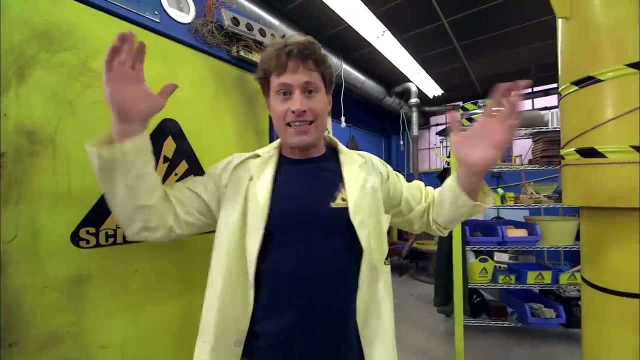 So that's what we're gonna do today on Science Max Experiments At Large. We're gonna max out the hot air balloon and make a giant hot air balloon. Yeah, I know what you're thinking. You're thinking, Phil, hot air balloons already exist. 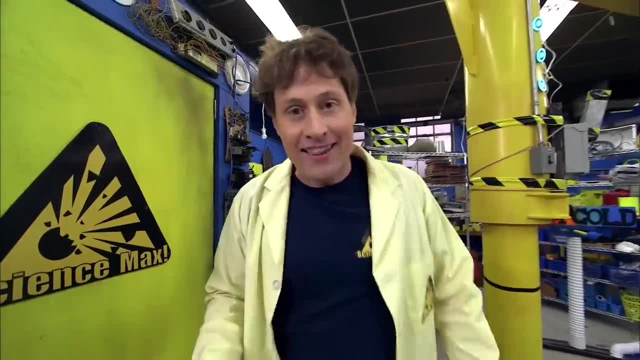 Why don't you just get a giant hot air balloon? I mean, they're big and you No, no, no, no. there's no fun in that. I want to make one I built myself. I don't think I'm gonna be able to fly in it. 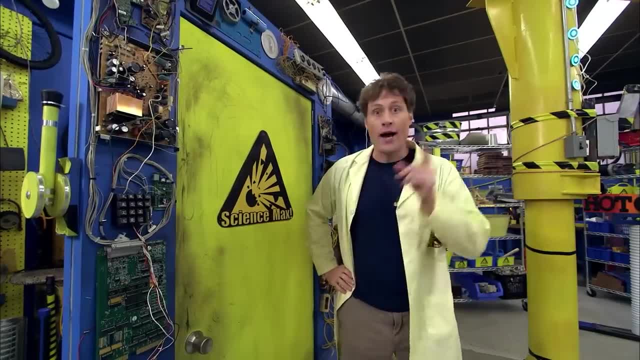 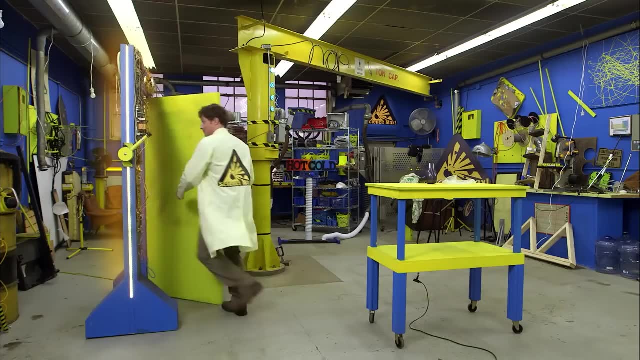 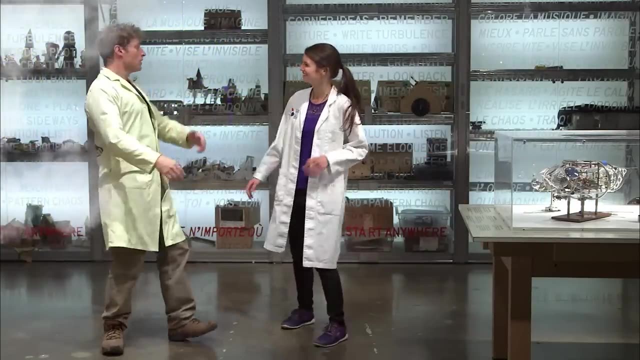 but it'll still be pretty cool. I bet I just need someone to help me. Um, oh, I know Michaela from the Ontario Science Centre. Hopefully she's not busy. Oh hey, Phil, How's it going? 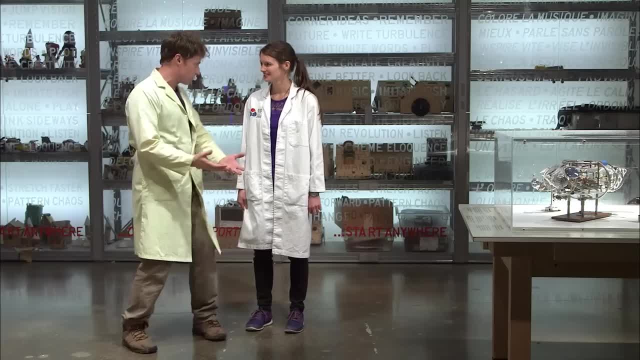 Michaela, how are you Good? how are you Good? I was wondering if I could get your help with an experiment. Do you have some time? Yeah, I'd love to help out, Awesome. Okay, let's go back to Science Max headquarters. 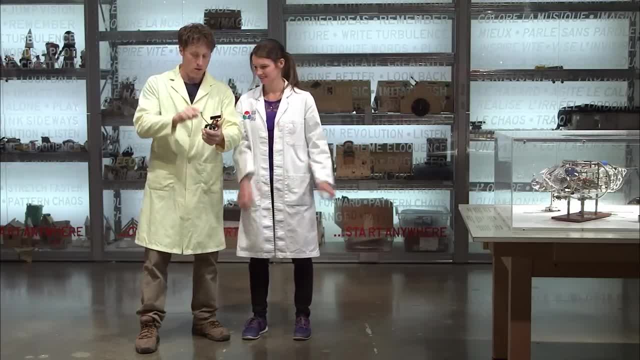 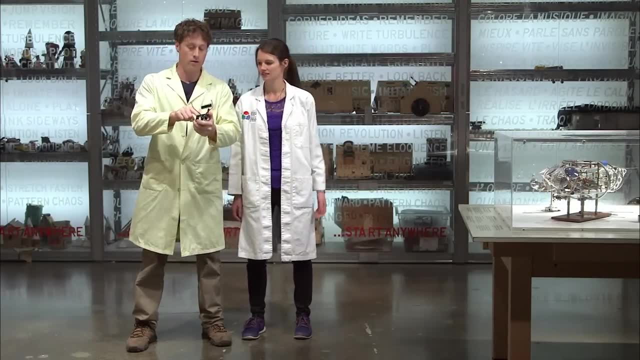 and I'll show you what we're gonna do. Okay, so ready, Here we go. Oh no, still here, still here. Why are we still here? That's weird. Okay, I know, I know, I know. 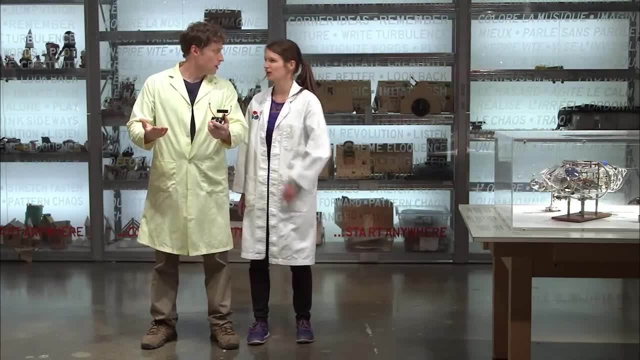 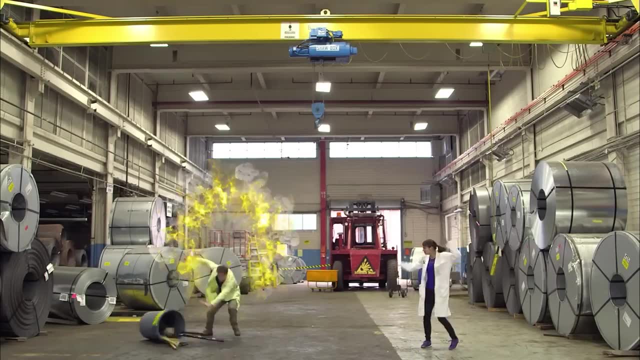 No, Why is the code not working? I think it's the Science Centre code. Try the, try the other code. Oh, it's the lab code. Right, Okay, Phil, are you okay? Yeah, Are you okay? Yeah, no, I'm fine. 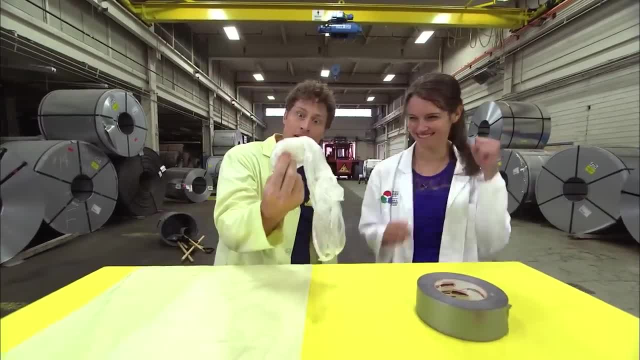 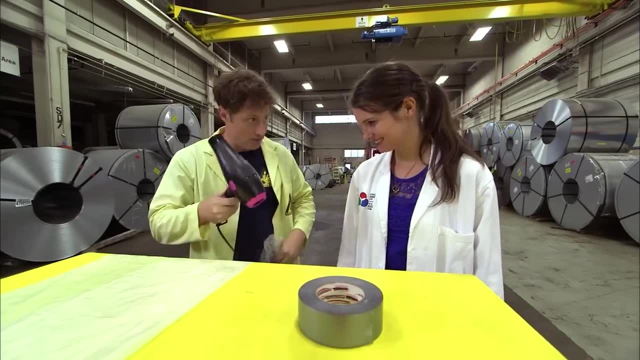 So, Michaela, I'm glad you're here, because today I want to max this out. This is my hot air balloon. It was better before I smushed it in my pocket, But what I did is I used a hair dryer and then I put it in and I heated the air. 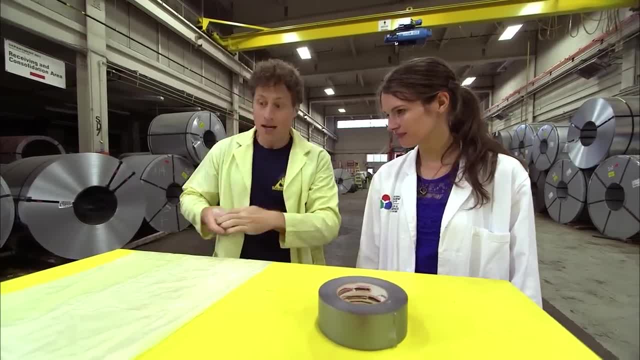 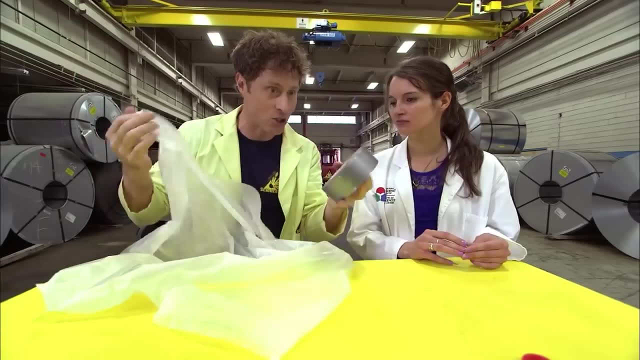 and it rises up. So in order to max it out, pretty simple, I just get larger bags right and then I thought we could cut them and tape them together to make a much larger balloon. It's a good idea, but you know. 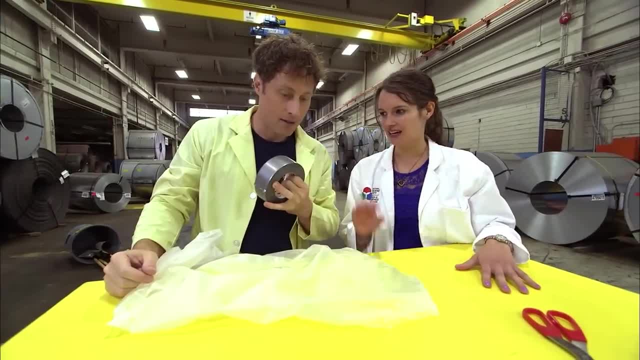 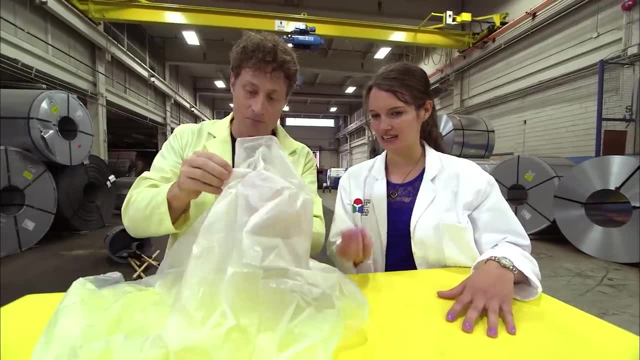 if we're making a hot air balloon, we need to make sure our materials are really light. The duct tape seems a little heavy. Even this bag seems a little heavy to me In terms of, oh you mean, the kind of plastic it is. 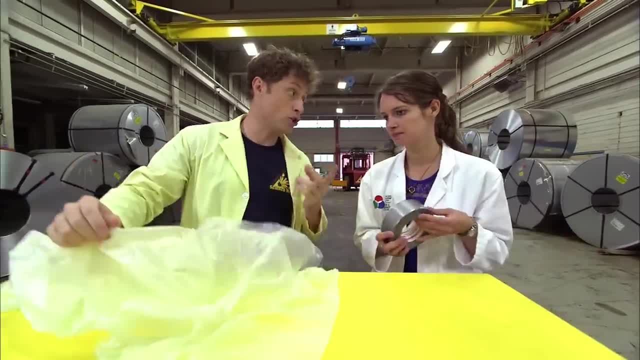 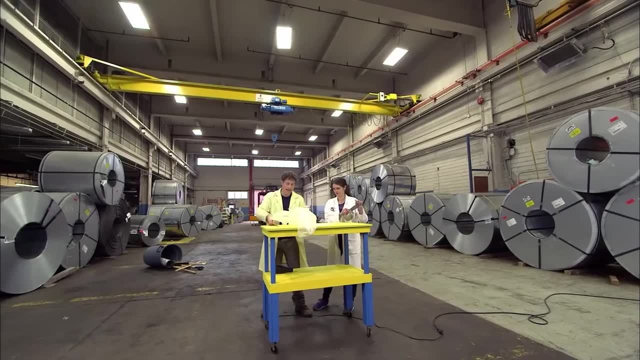 Yeah, it seems really thick, this one. Well, do you know for sure? I've never tried it before. All right, well, that's science. We should try it and see what happens. Let's try it. Okay, so I'll cut along the side of the bag. 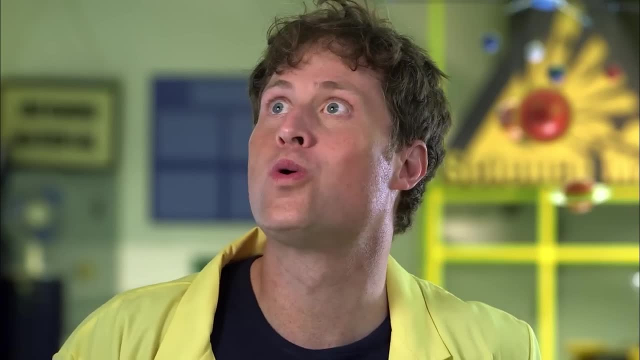 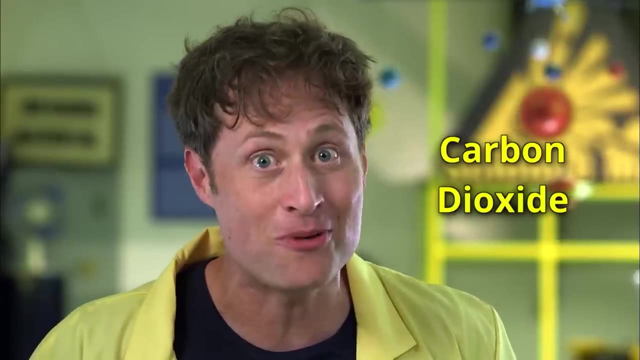 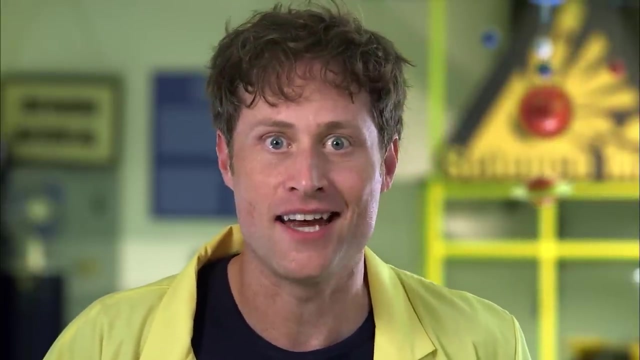 You see that Carbon dioxide gas. Our bodies breathe in oxygen and breathe out carbon dioxide. Did you see it? Take another look. How about now? No, you didn't see it right, Because carbon dioxide is invisible unless you freeze it. 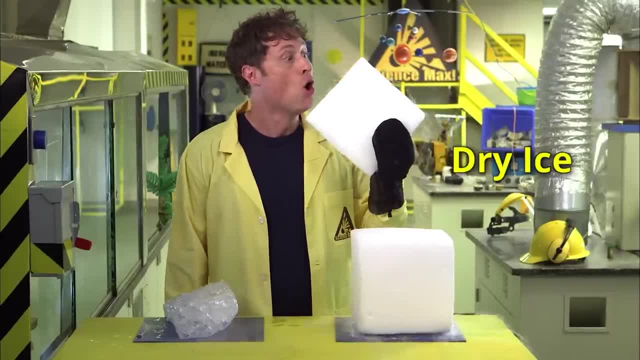 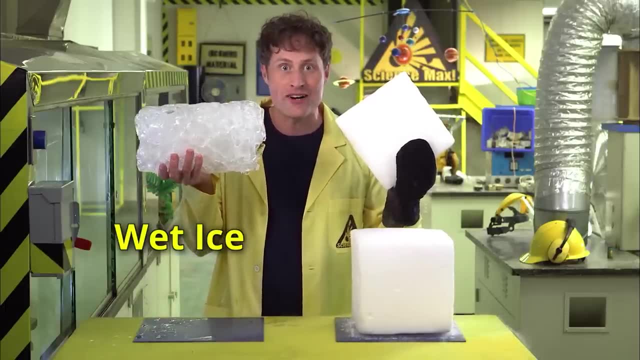 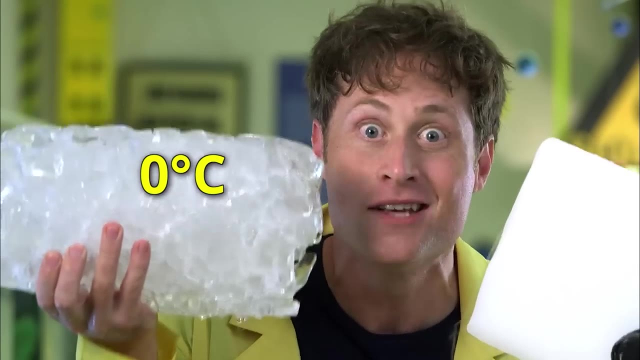 This is dry ice, frozen carbon dioxide, And this is wet ice. It's not really called wet ice, It's frozen water. Now you know what temperature water freezes at. Starts with a zero, ends with a well, it's actually zero, zero degrees Celsius. 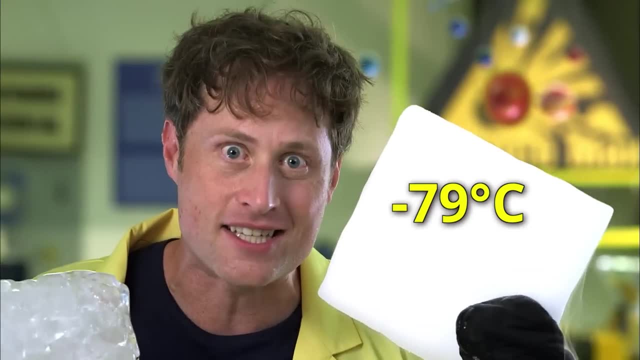 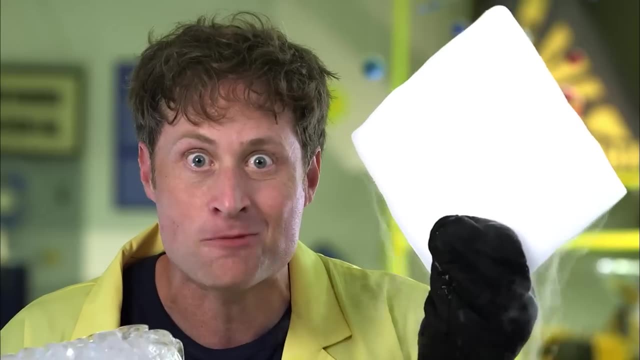 And this freezes at negative 79 degrees Celsius. It's much colder. I have to hold onto it with a glove, because if I held onto it with my bare hands I'd get frostbite. So here's the experiment. If I pour some liquid water on the dry ice, 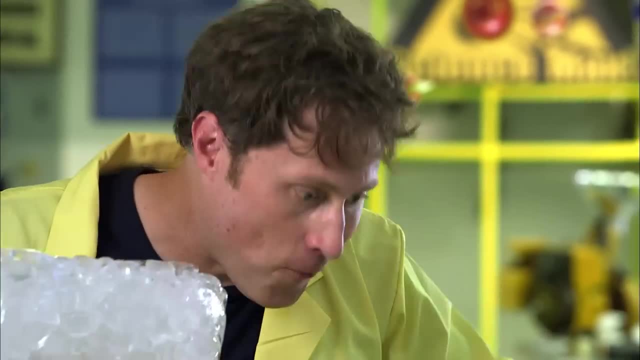 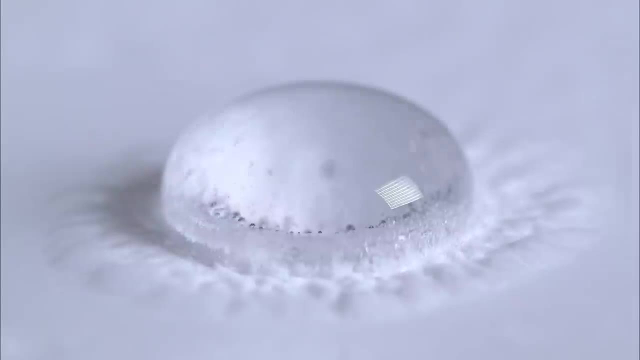 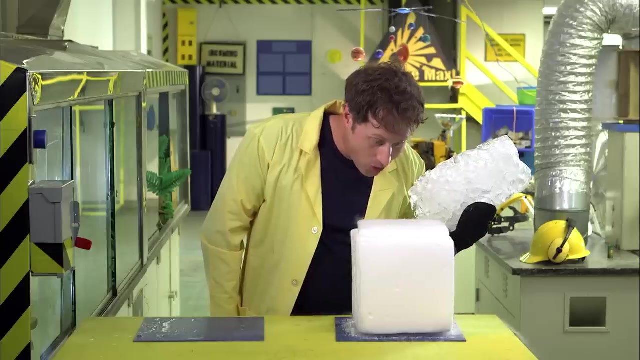 will it freeze again? Let's find out, Because the dry ice is so much colder than the freezing point of the water, the water begins to freeze from the bottom up in room temperature. air right before our eyes. Whoa, totally frozen Cool. 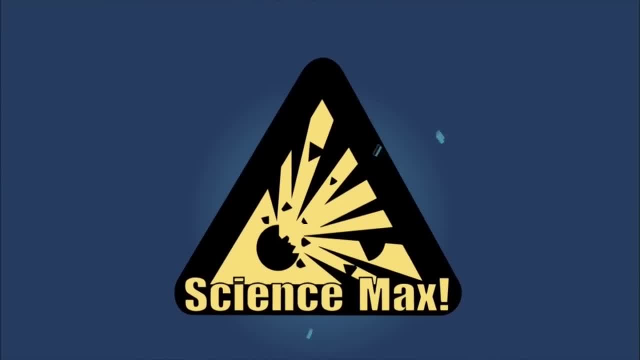 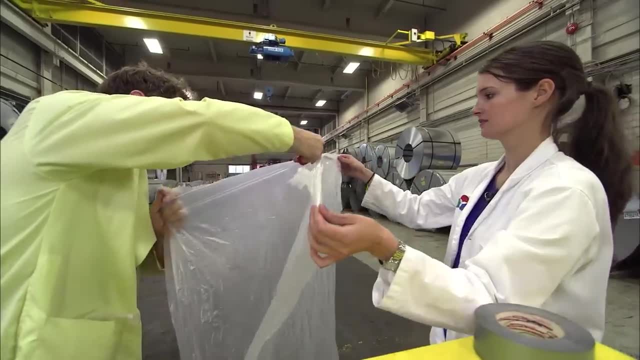 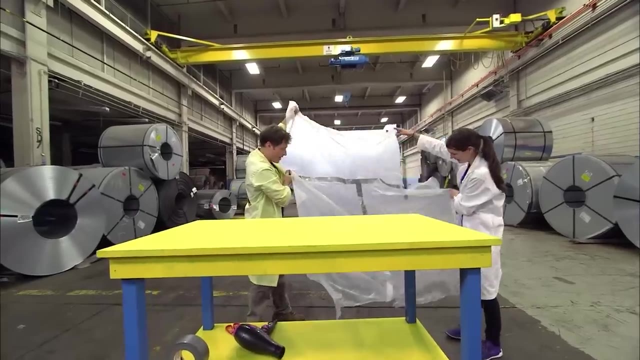 Cool. In order to build our hot air balloon, Michaela and I are taking clear garbage bags, cutting them along the seams so they end up as one thin sheet of plastic, and taping them all together with duct tape into a balloon. Okay, so that's how many bags, is that? 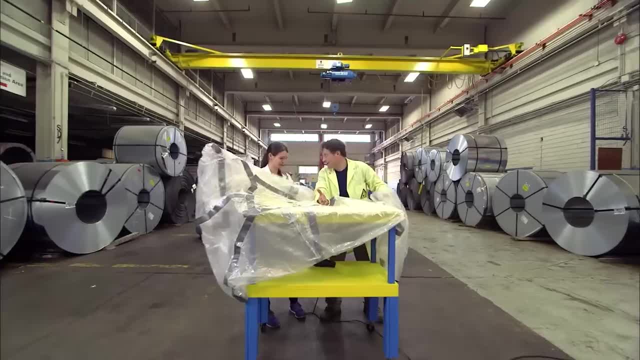 It's like 12 bags, 12,. so you think that's big enough. I think so it's pretty big. Okay, I think we can stop there, Okay. so where's the? where's the opening? again, I think it's on your side. 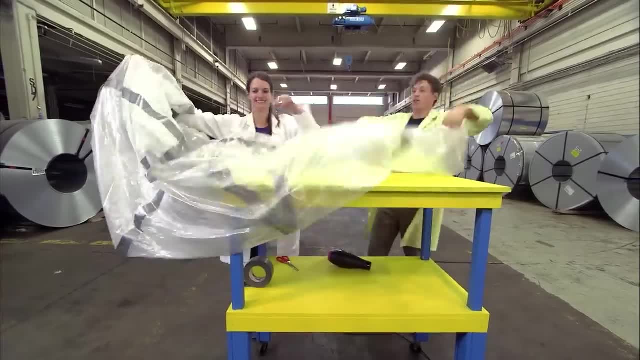 Hope you didn't duct tape it, Chloe. Okay, no, we're good, we're good, So, so it's going to inflate. It's going to inflate like this: Wait a minute, let's, let's okay, let's make sure it works. 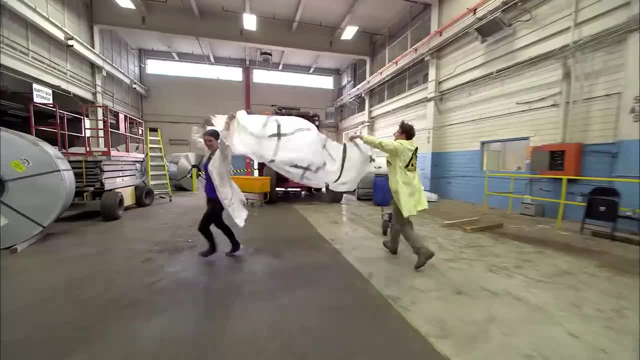 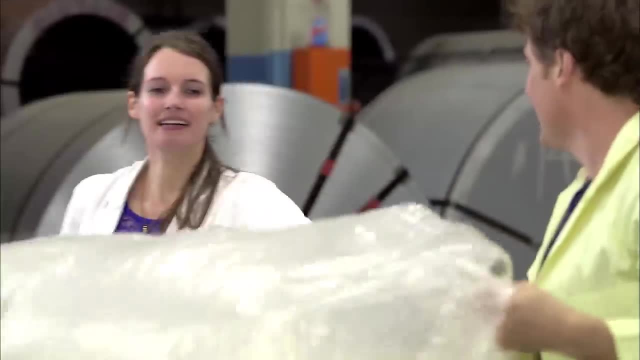 Is it working? Uh, kind of, Ooh, I don't know. if it's inflating, Okay, good, so it does inflate. It does hold air, Yeah Right, So should we try it? Yeah, let's try it. 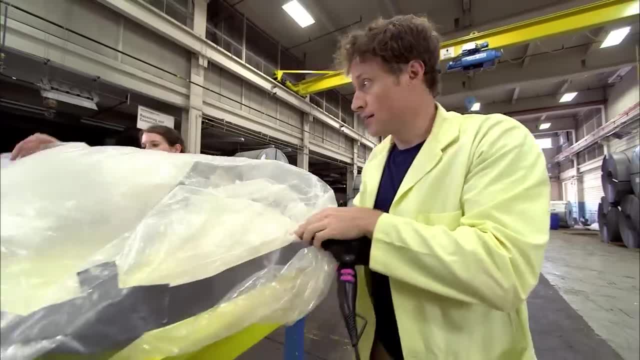 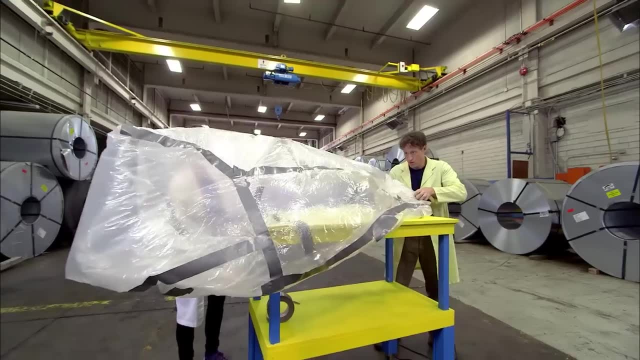 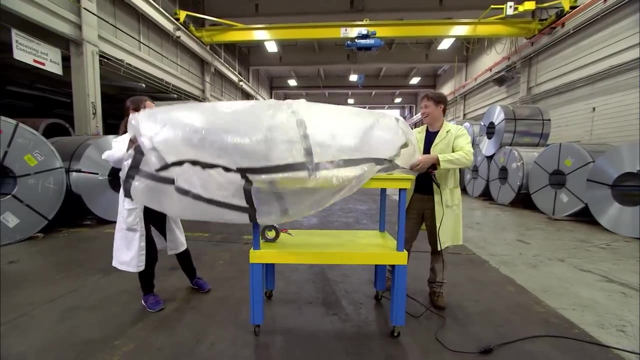 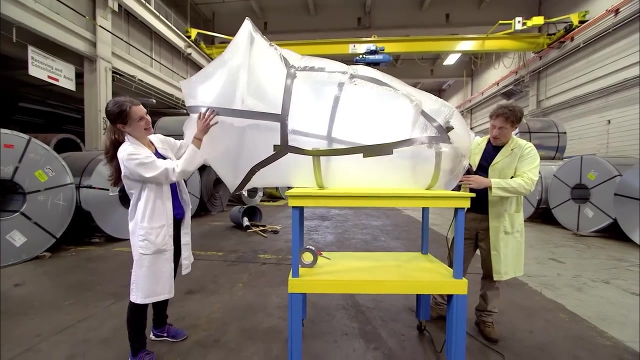 Okay, so we're going to use a hair dryer, right, And now we wait. It's working Kind of Oh yeah, Woohoo. Okay, it's almost inflated, All right, Okay, what do you think? 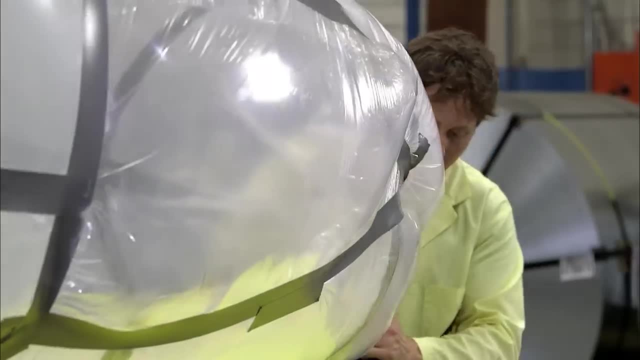 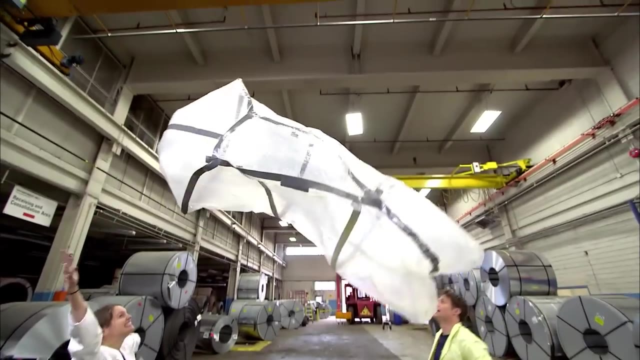 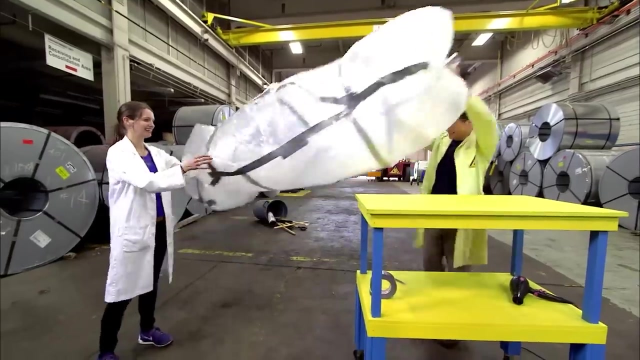 Yeah, let's try it. Okay, on the count of three, we'll throw it okay. Okay, All right. One, two, three. Yeah, It didn't quite, it doesn't. it doesn't quite float huh. 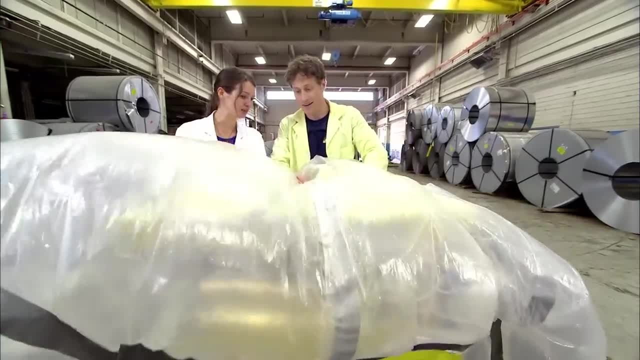 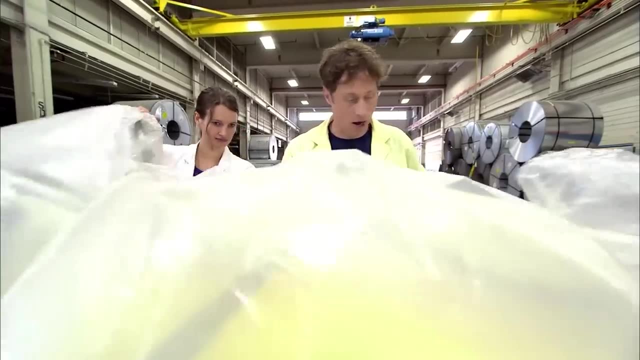 It's still too heavy, Phil. I think we've got a couple problems here. The duct tape is really heavy, Yep. Also, these bags themselves are really heavy. Okay, well, if we want to fix the duct tape problem, we could use lighter tape. 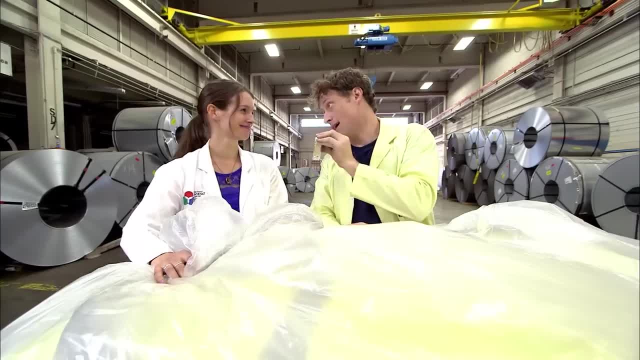 Like: what if, haha, we used invisible tape, or, as I like to call it, science tape, Science tape Which would be lighter than duct tape. That's a good plan, But what do we do about the bags? Have you ever seen the? 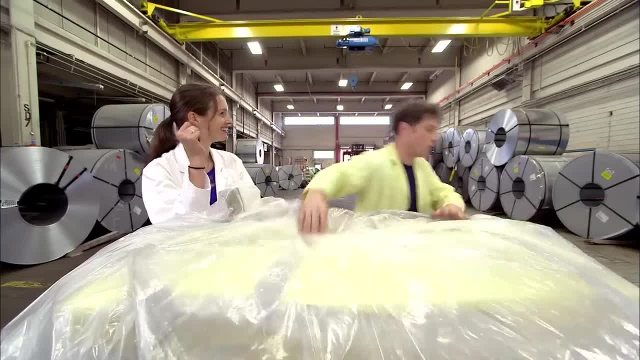 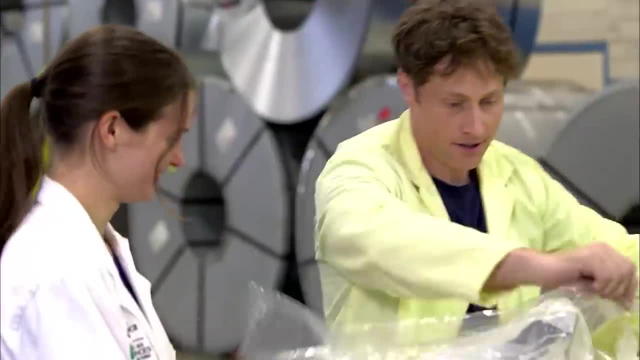 you know those dry cleaning bags. Oh wait, I've got one. I've got one here, Cool, Perfect. Haha, Yeah, perfect, Because you know when I get my lab coats dry cleaned. So let me see here. 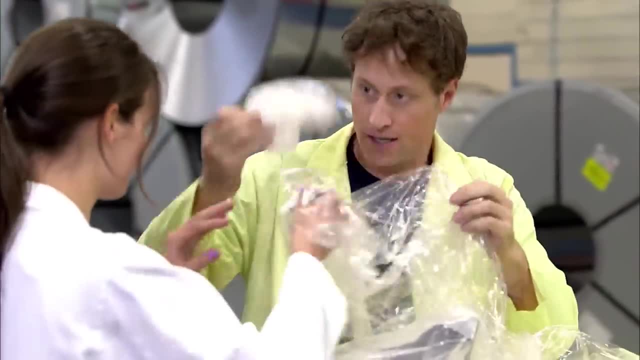 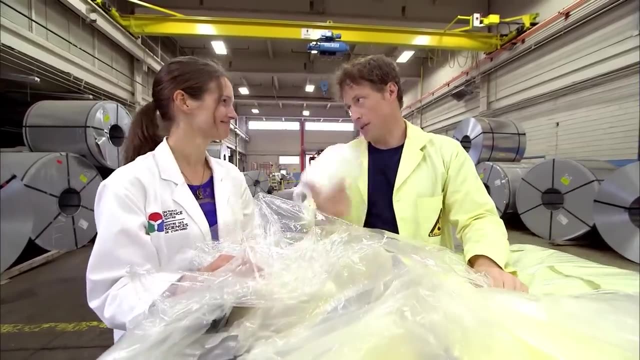 Oh yeah, this is much lighter. This is kind of the same material as the as the grocery store fruit bags. right, I have a better feeling about this one. So lighter tape, lighter bag means a much lighter balloon. Okay, well, let's try it. 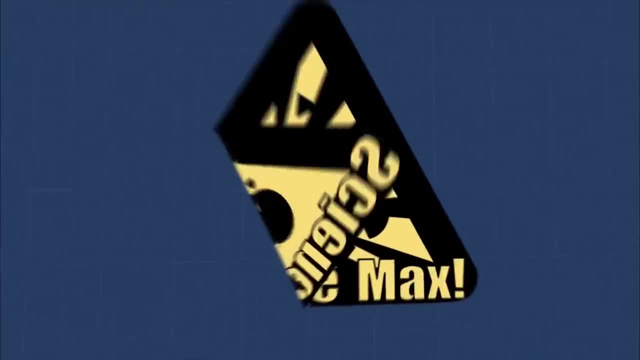 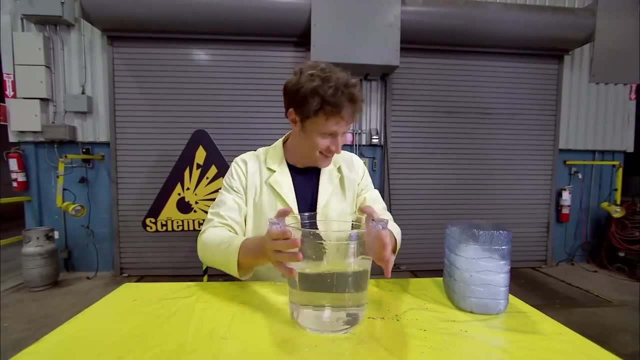 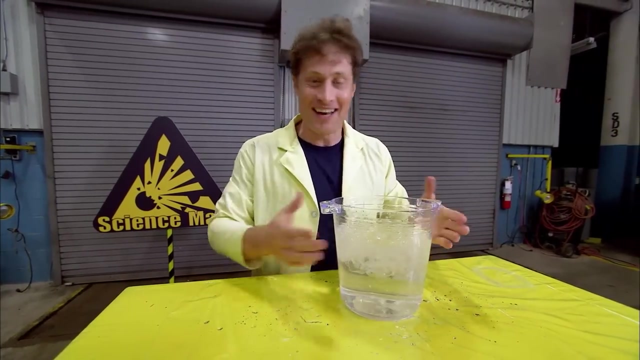 First I should probably take my lab coat out. Okay, Now there you go, baby. This is water. Now it's ice water. haha, Science, okay, no, that's not the science part. Here's something you can do at home. 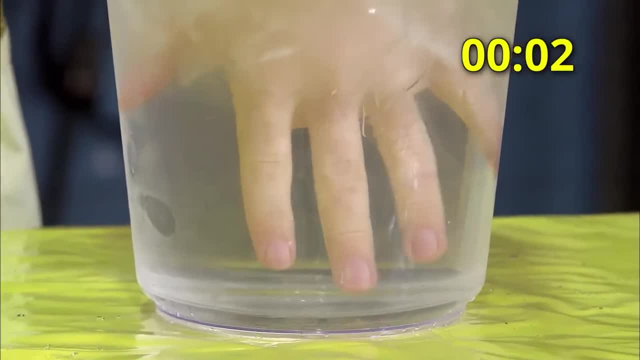 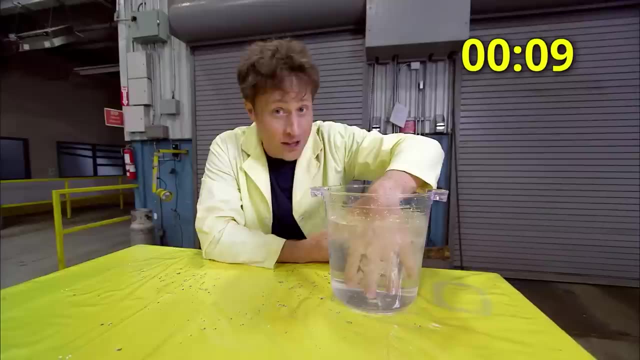 Get some ice water and a way to time yourself and stick your hand in the ice water. It's a little hard to stick your hand in ice water for a long period of time, But don't worry. the pain that you're feeling isn't actually because you're damaging anything. 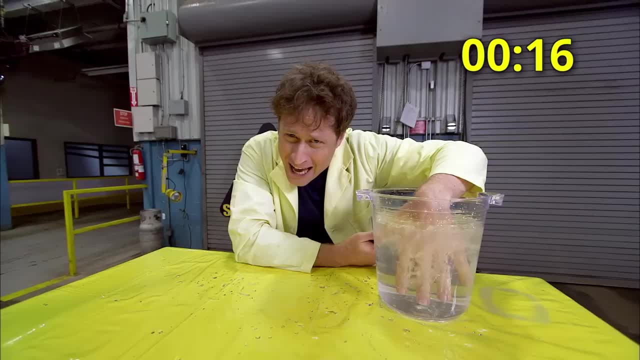 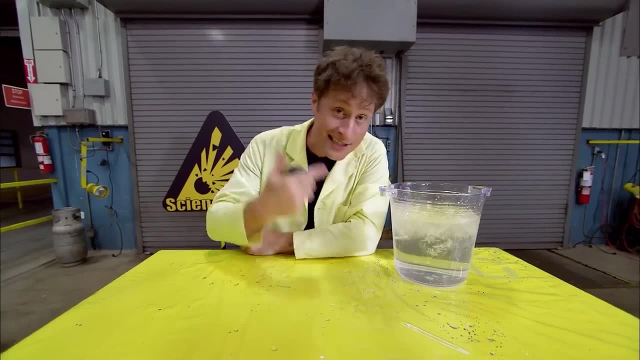 it's just your body's way to tell you that you need to take your hand out of the cold water. Yeah, you usually can't do it for very long, But some animals like seals and whales- they live in ice water all the time. 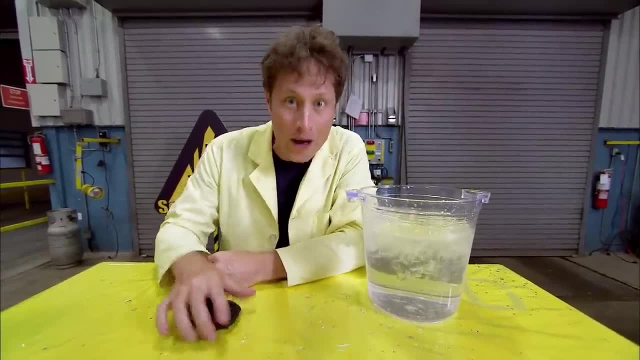 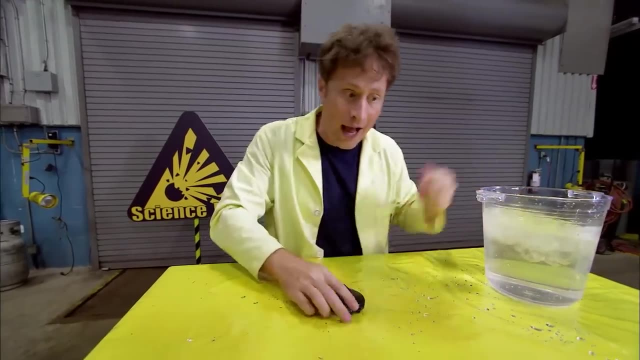 They live in the Arctic. so how do they do it? One word: blubber. Blubber is a layer of fat that protects you from the cold or protects a seal and a whale. We don't have blubber, but we are, today, gonna have some blubber. 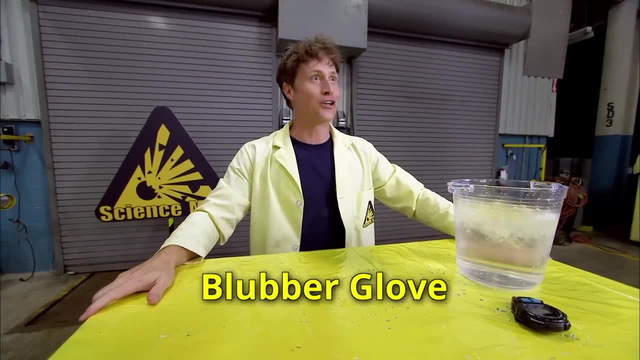 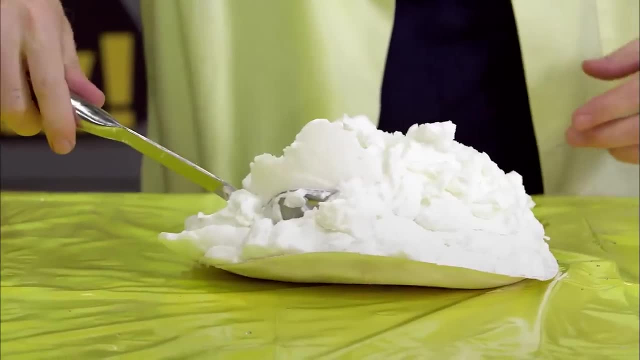 because we're gonna make a blubber glove, Blubber glove. I love saying that. Here's how we do it. First, we want blubber. Okay, this isn't blubber, this is lard, which is actually animal fat. 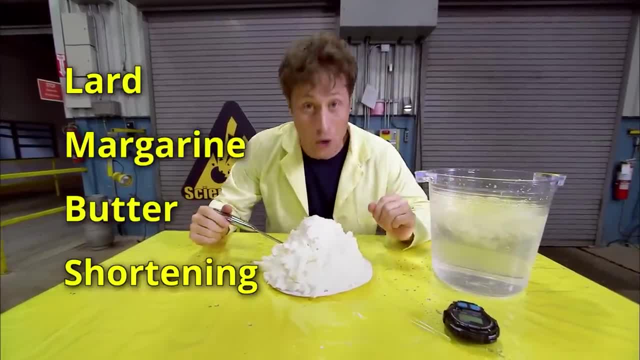 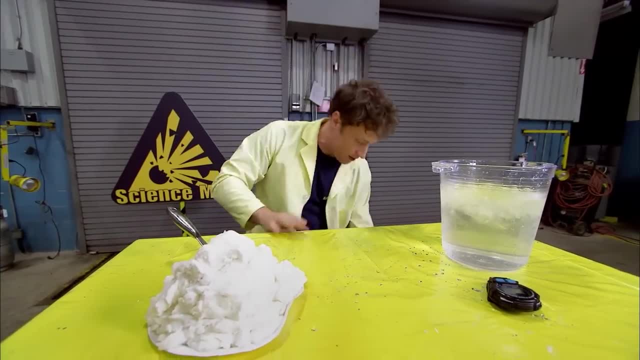 You can use lard, you can use margarine or butter or shortening- anything with a lot of fat in it. And remember, this is messy, so definitely get an adult to help you. So we've got our lard and we need a bag. 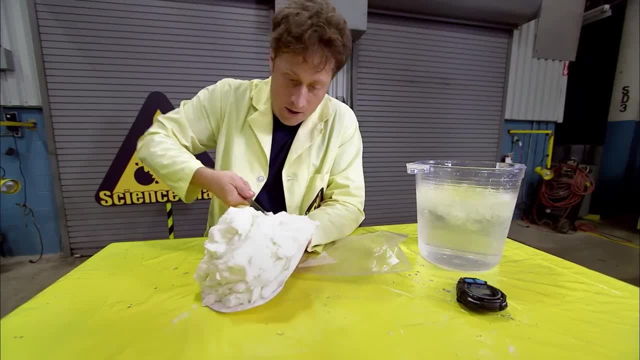 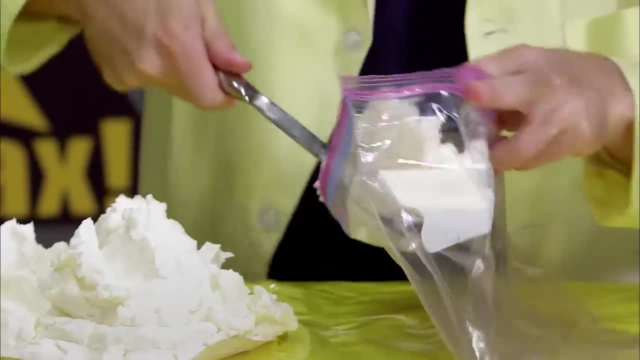 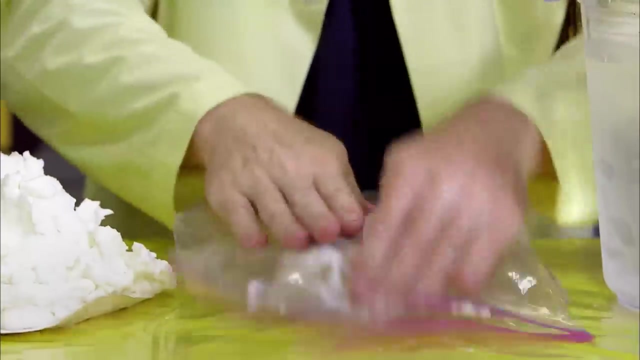 So what you're gonna do is you're gonna take a scoop full of lard like this And you're gonna put it in the bag like so, Mm-hmm, Like that. There we go, And then you're gonna start smoothing out the blubber. 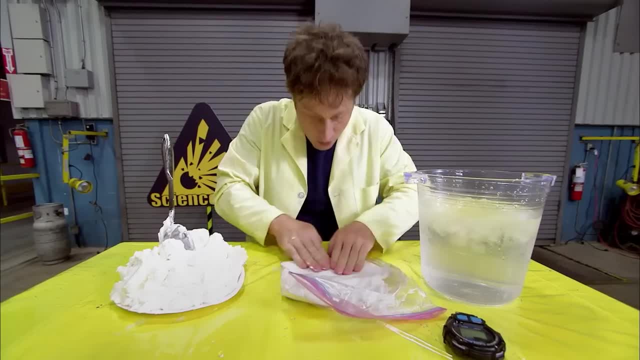 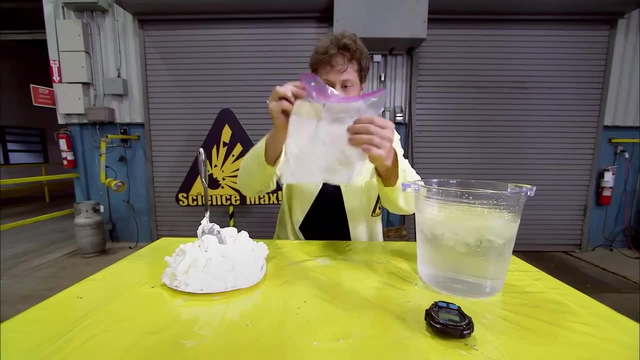 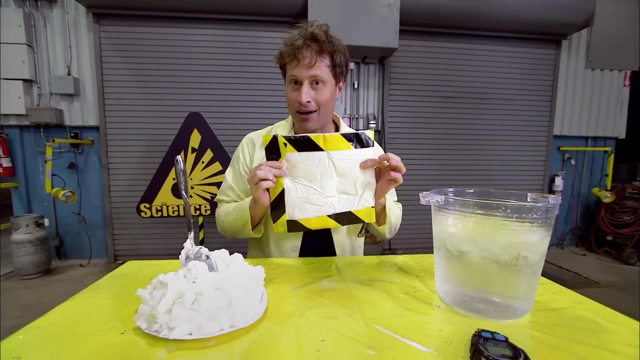 or the lard like this, Because what you wanna do is have a nice thin layer all the way around. See Starting to work. Yeah, Then seal the bag and tape the edges. huh, A square of blubber. 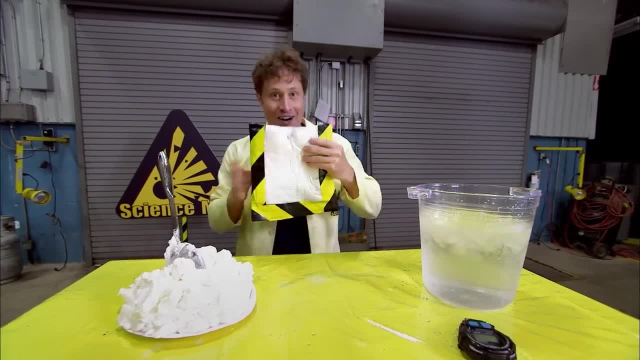 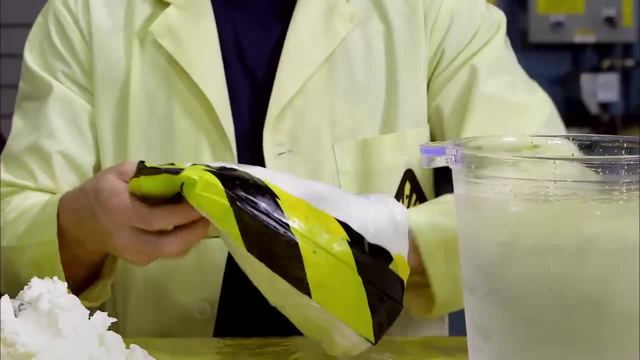 Then do it again. Here I have two bags of blubber and I've taped all the way around the outside. So I have, ha-ha, a blubber glove. Check it out. So let's try it out. 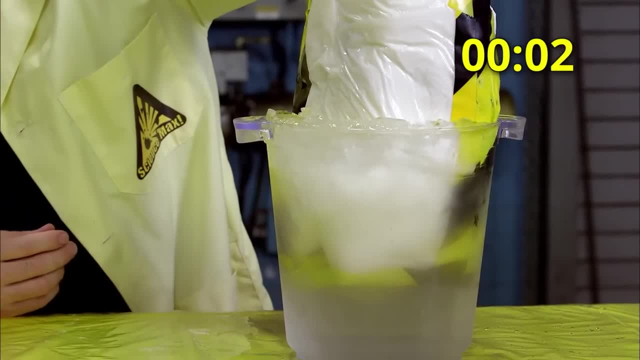 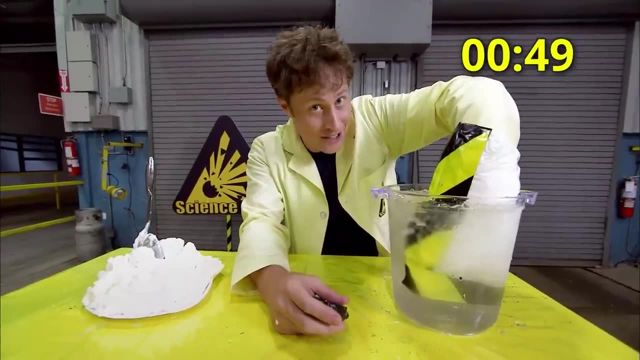 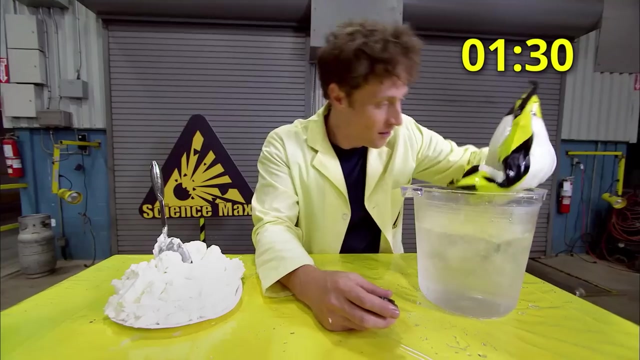 I stick the blubber glove in the ice water. It's completely working. It is not even cold. The blubber is completely protecting my hand from the ice water. I'm not even remotely cold at all. That is very fun, So try it yourself. 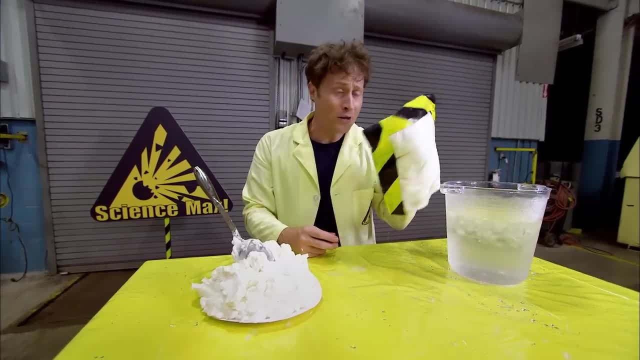 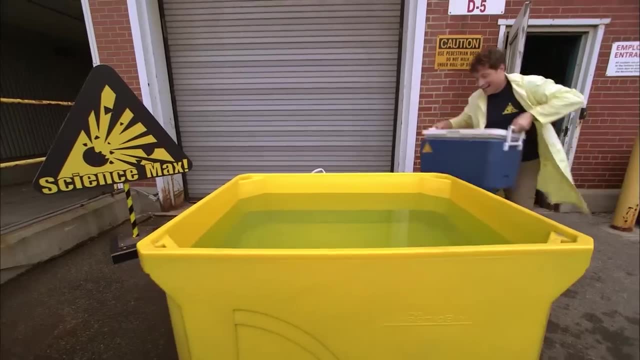 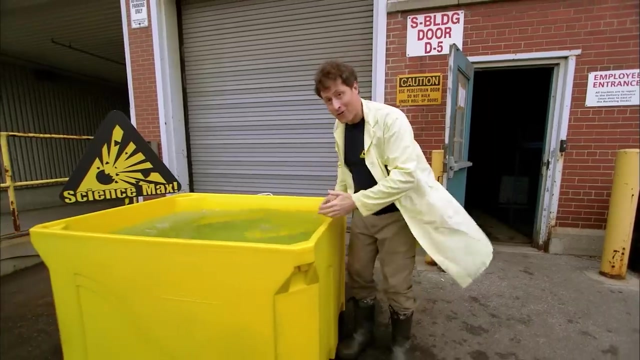 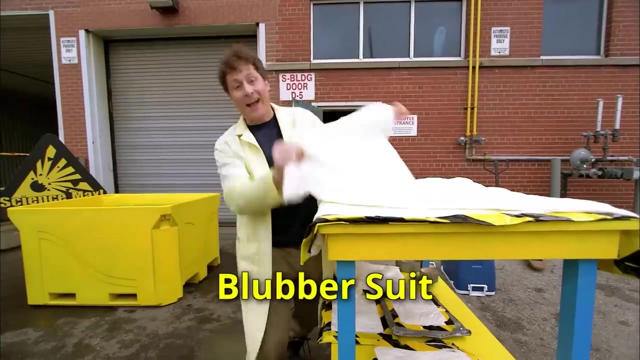 A blubber glove. Now, how do we max out a blubber glove? Watch Water, Ice water. I know for a fact that I wouldn't last more than 10 seconds in here without my blubber suit. I'm going to make an entire outfit of blubber. 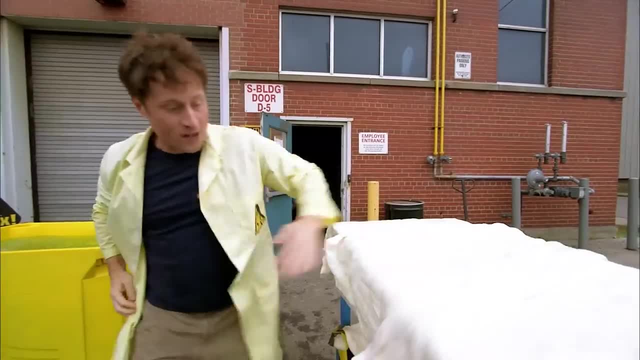 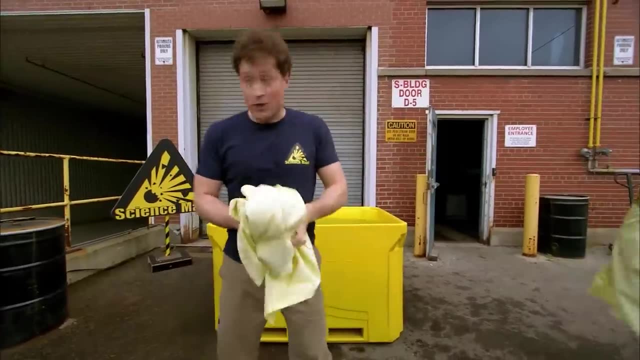 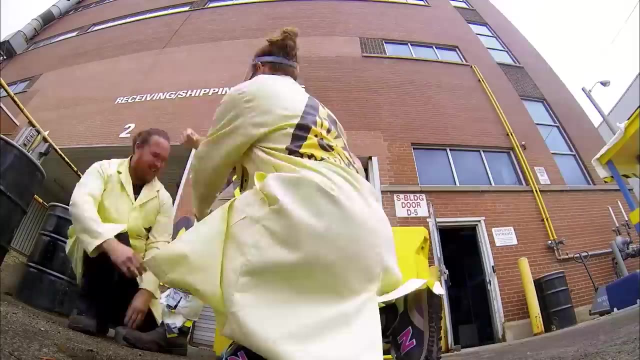 I've got them in large plastic bags and I'm going to get completely suited up in blubber with the help of Trevor and Stephanie. OK, guys, suit me up. It's very heavy. This is going like this, Oh, OK. 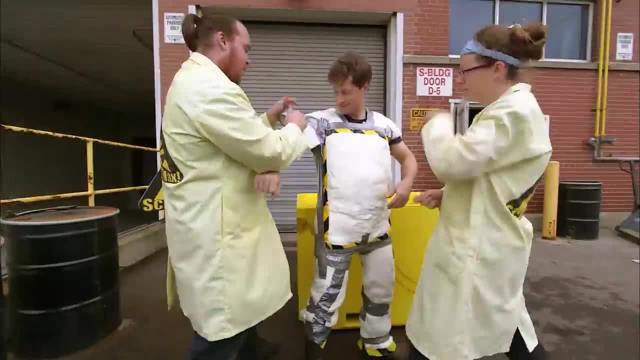 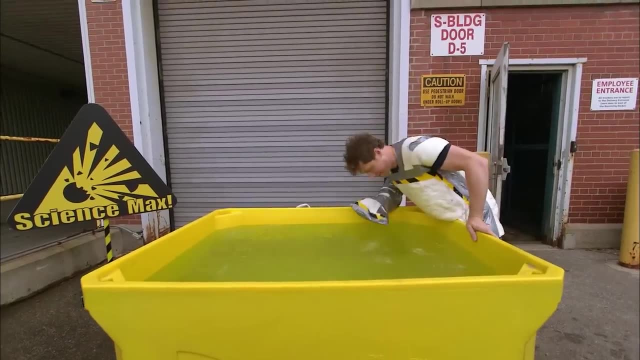 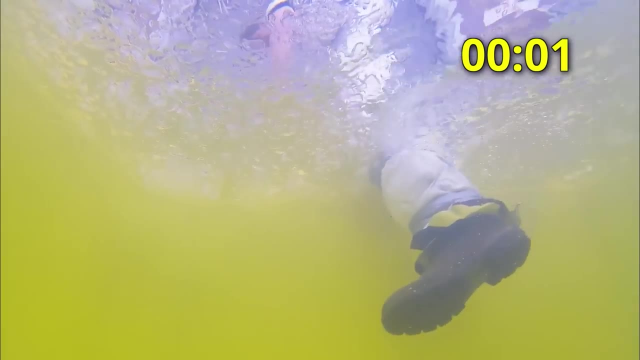 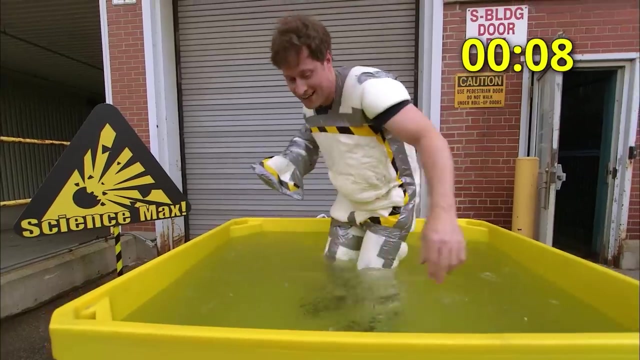 OK, Time to cut back on the cookies. All right, let's do it. All right, Blubber suit go. OK. Oh, here we go, And OK so far. Oh, Ha, ha, ha, ha, ha ha. 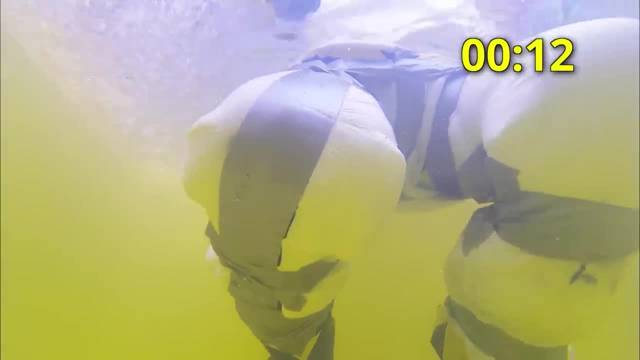 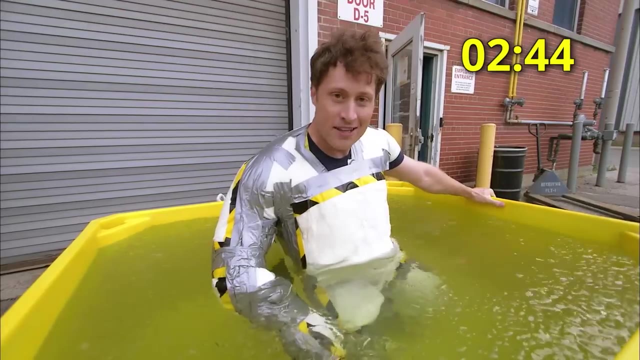 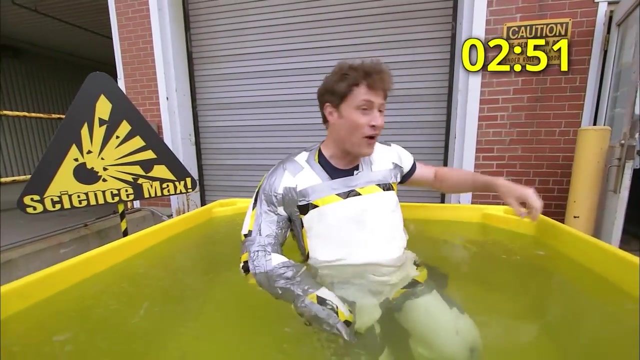 The legs are warm And oh, Blubber suit, Ha ha ha, I am in seals, Actually. here I am in the ice and I don't feel too bad. Blubber suit works. Ha, Blubber suit's refreshing actually. 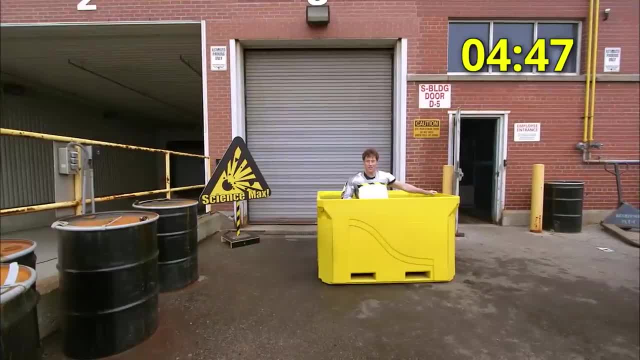 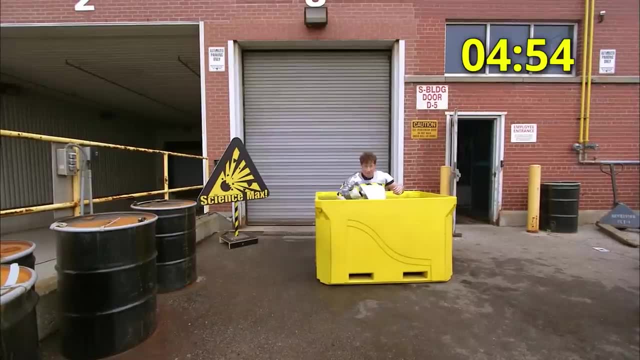 You just sit back and chill out. Well, there you go. Blubber suit success. Seals and whales are able to stay in ice water for their whole lives because they have protective layers of blubber, just like I do. OK, so now all I have to do is get out. 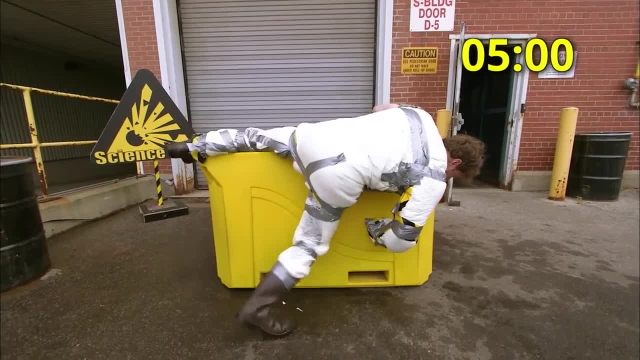 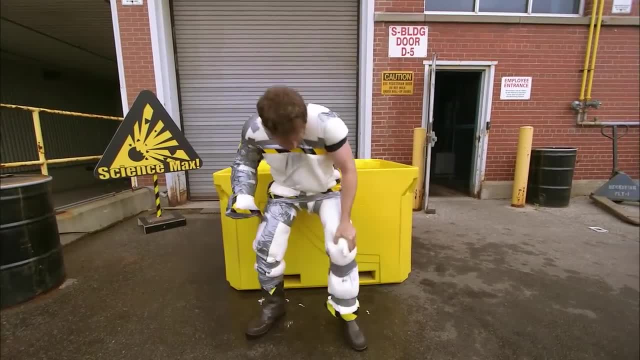 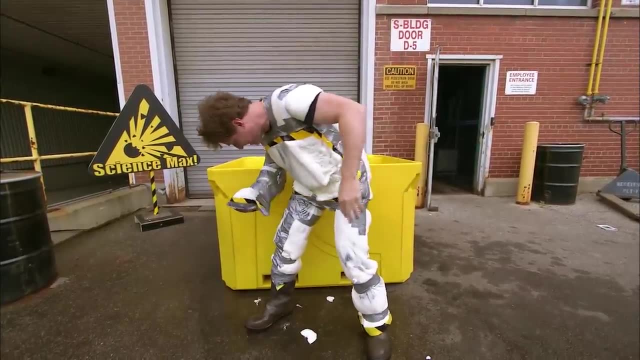 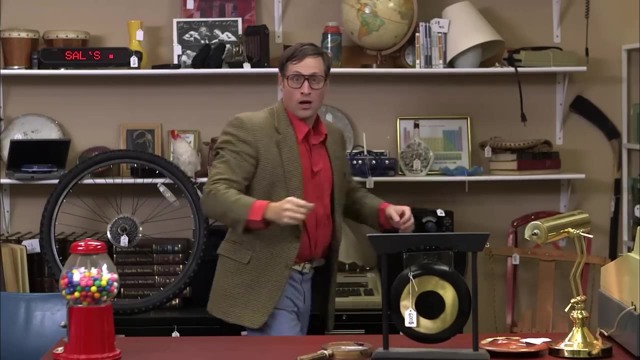 Oh no, My blubber is leaking. Ah, I've sprung a leak, My blubber. Oh, my precious blubber. No, What a world. Oh hey, How you doing. Ugh, shut the door. It's cold out there. 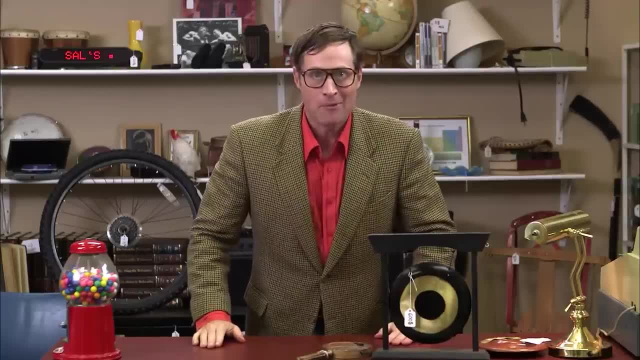 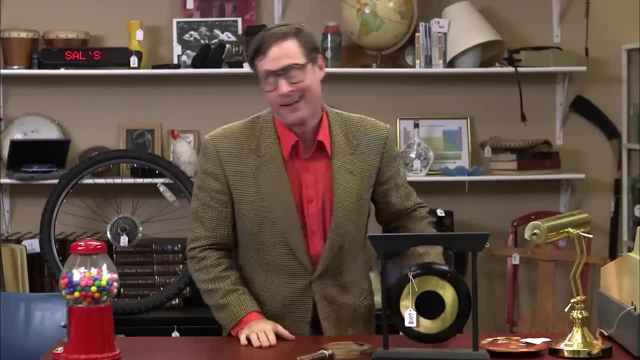 Whoa, cold enough for you? huh Well, that's nothing. Let me tell you, You know what temperature? water freezes at, Yeah, 0 degrees Celsius. But even that is nothing. Let's say it's winter in Winnipeg. 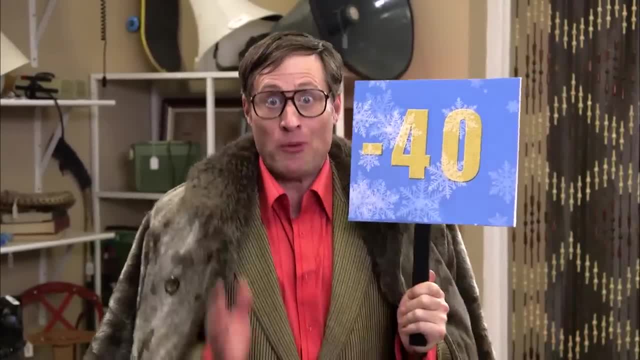 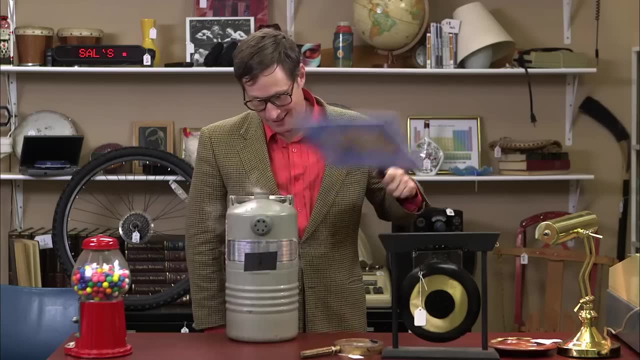 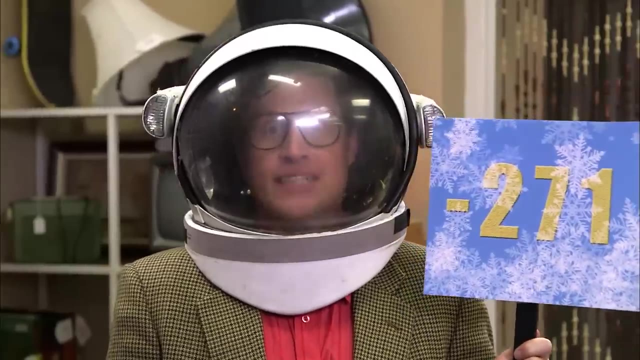 It could get down to minus 20,, maybe even minus 40. But even that's nothing. Liquid nitrogen: minus 196 degrees Celsius, But even that's nothing. The vacuum of space: Minus 271 degrees Celsius, But even that's nothing. 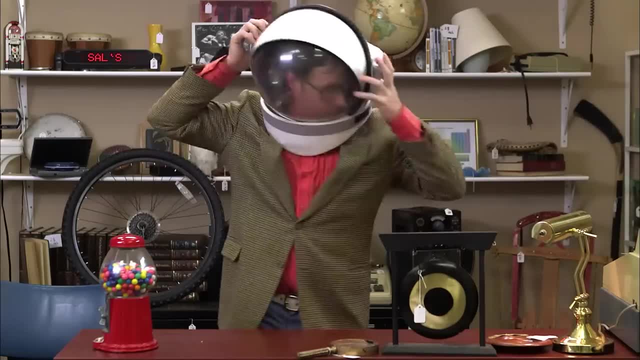 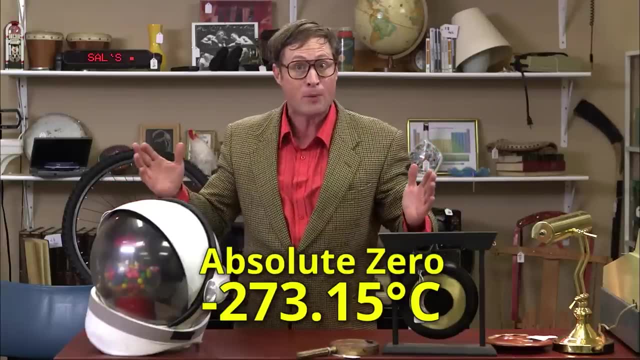 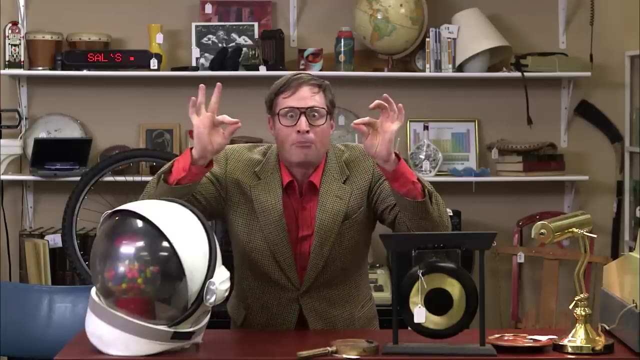 So what's the coldest temperature you can have? It's called absolute zero Minus 273.15 degrees Celsius. At that temperature, all the little wiggling that particles do comes to a stop. Everything is frozen. No more movement. 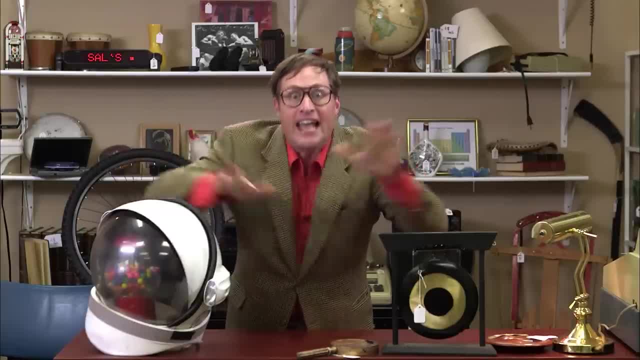 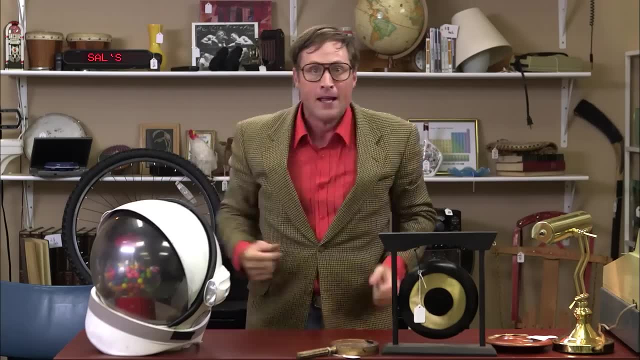 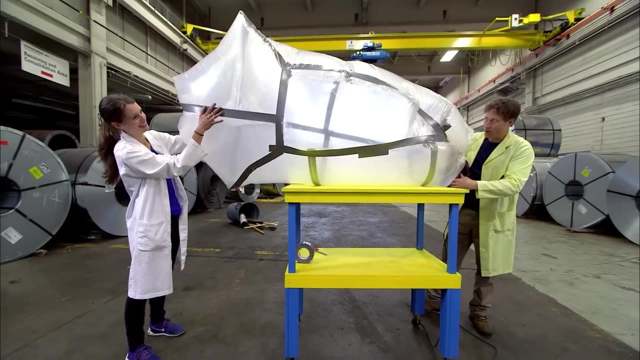 No more energy. Everything stops. It doesn't get any colder than that. Absolute zero is the ultimate nothing. Time to get your mittens on. Our first hot air balloon didn't float very well. It's still too heavy, though. I think we've got a couple problems here. 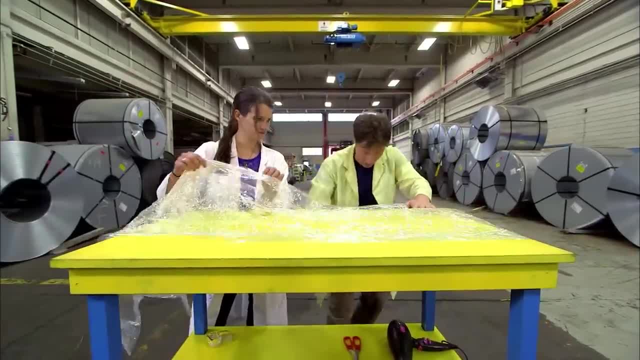 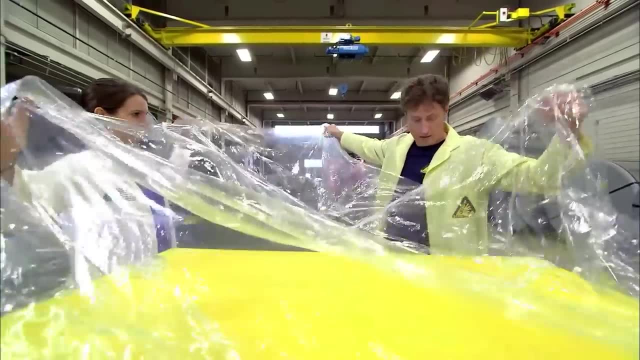 So we're making a lighter version out of dry cleaning bags and science tape, Both lighter materials than our last version. We also went for more of a square shape than our last version, which kind of looked like a sock. Once we were done assembling, we got the hair dryer and tried it again. 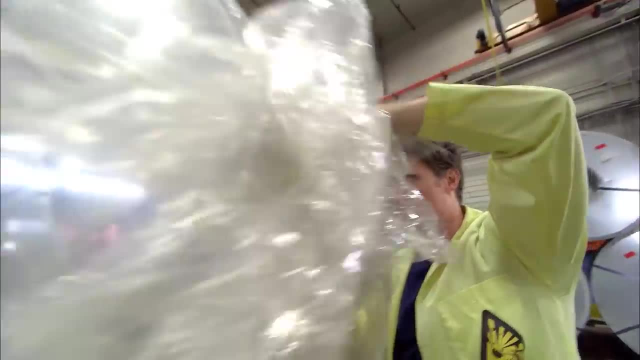 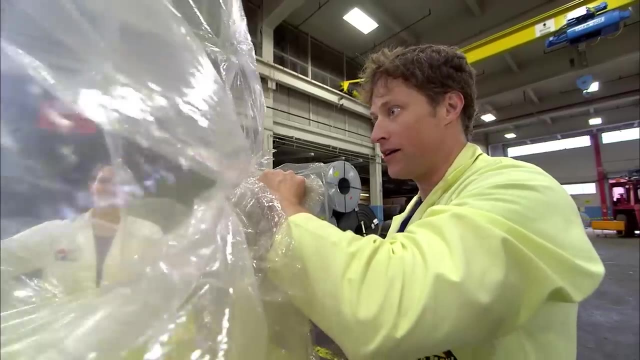 It's sort of working, Kind of It's inflating, That's something. Yes, Let's start. It feels warm, like the hair dryer is actually making a lot of warm air in there. Yeah, This is definitely working better than the last version because it's so much lighter. 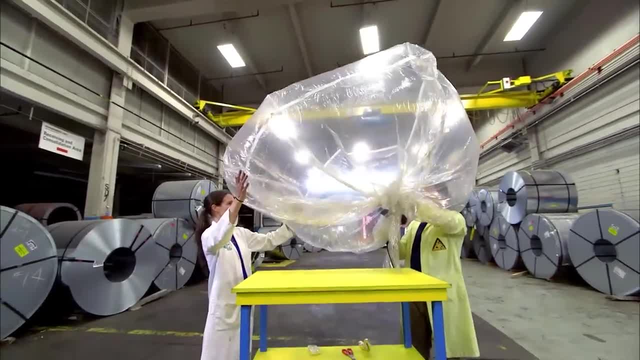 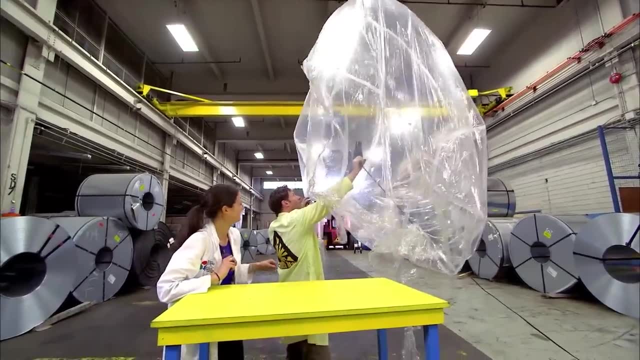 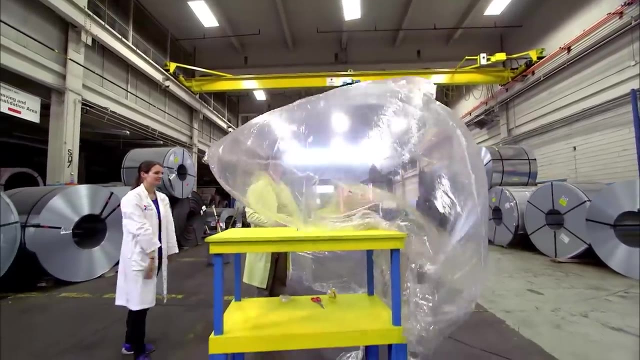 Yeah, Wait a minute, Almost got it. Whoa, Yeah, It's sort of working right. Cool, Kind of Okay Ready. Are you testing it Turning off the hair dryer? Huh, It kind of collapses the moment we turn off the hair dryer. 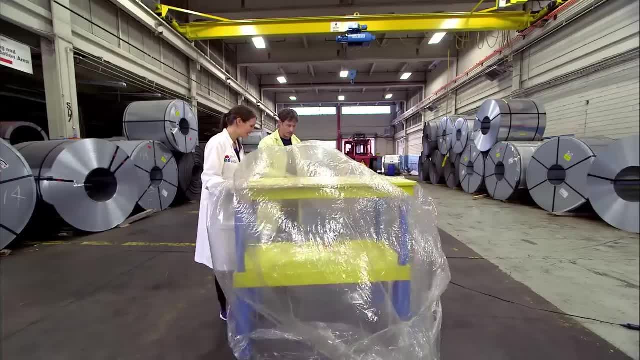 Not what we expected, was it? Yeah, I mean it sort of works. The thing is, our balloon is so big that we need to heat up all of the air that's in there. I don't know if this hair dryer is strong enough. 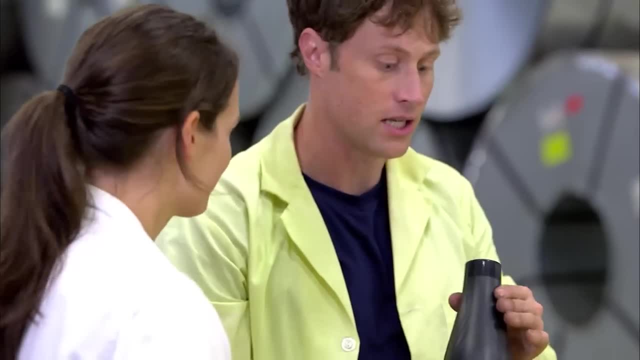 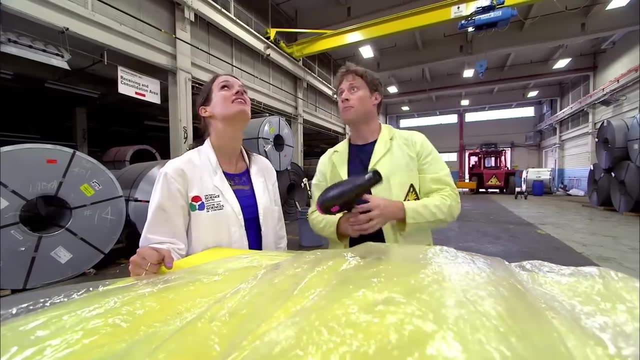 I think you might be right. So we just need something else that pushes heat. Yeah, more heat, More power, So like a heater of some sort. You know, we've got some heaters up in this room actually and maybe I could just tear. 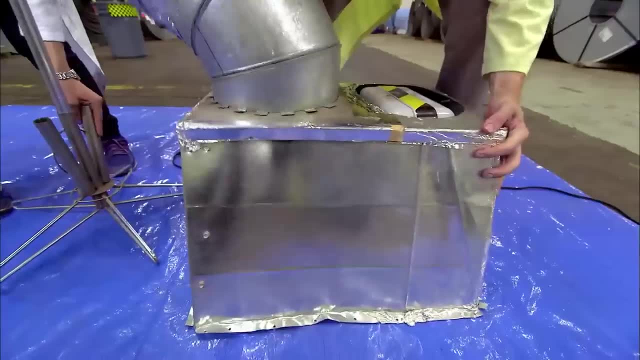 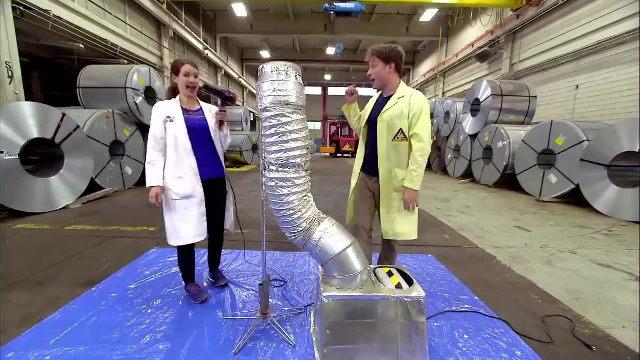 one out. We can use that. I like it. Okay, All right, There Got it An industrial heater, And this is going to work just the same as our hair dryer. It's going to blow a lot of hot air up here, but this is way more effective than a hair. 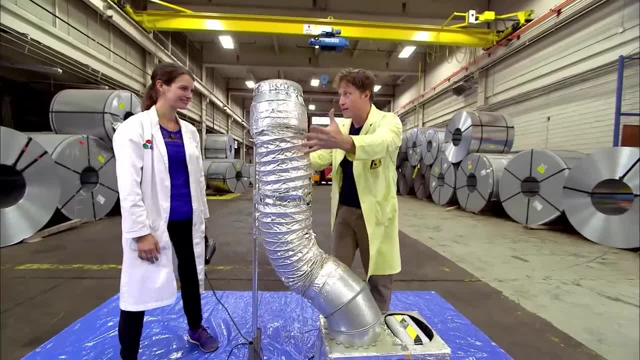 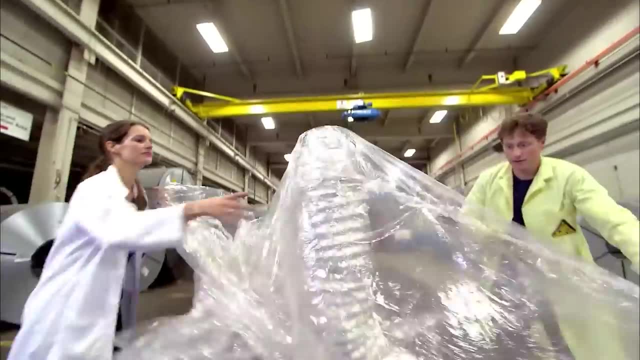 dryer, right, Yeah. So we put the balloon over here. hot air comes up, the balloon inflates and hopefully it flies, Hopefully. All right, Let's get the balloon. So we put the balloon on the heater and turned it on, but it doesn't seem like much is happening. 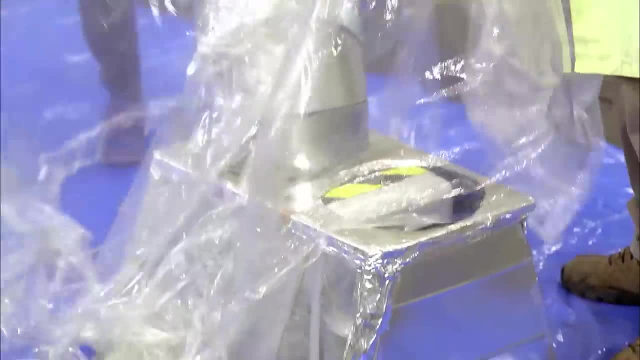 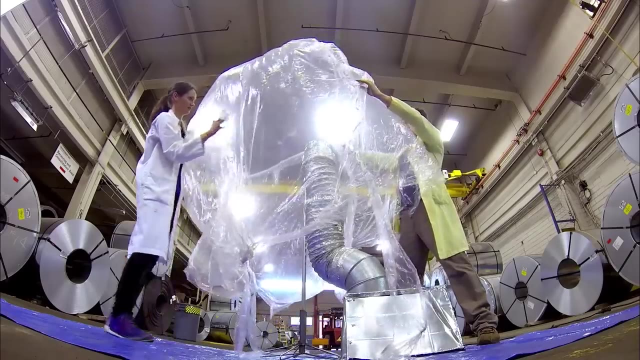 That's because the heater pushes less air, but the air is much hotter, which means it took longer. Should we have brought a book? But soon it was inflating. Definitely a better result than the hair dryer. Okay, You ready. 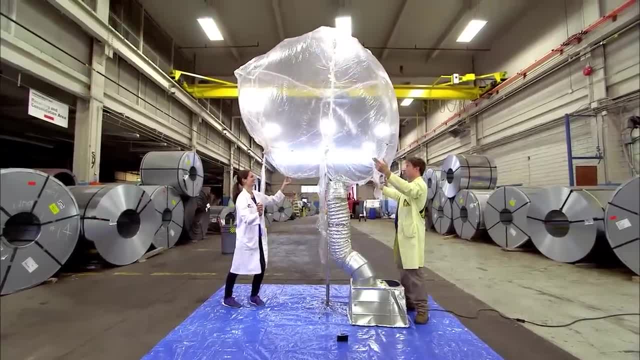 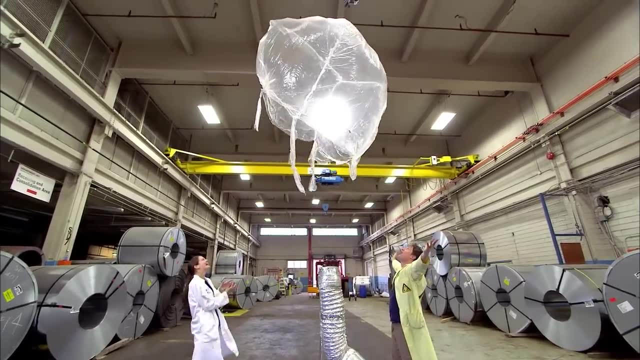 Let's do it All right. Yep, One, two, three, let go Blister. Yeah, It's like a giant jellyfish, It's huge. Uh-oh, Uh-oh, It's tilting, It's tilting. 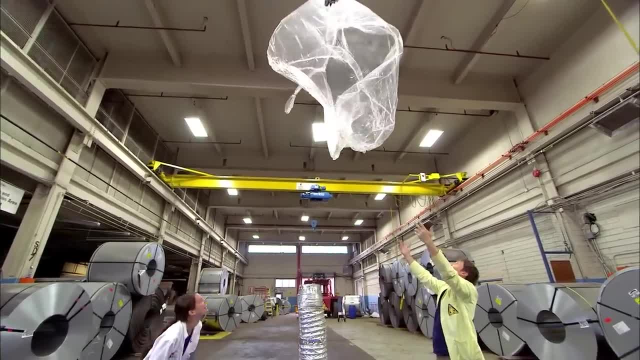 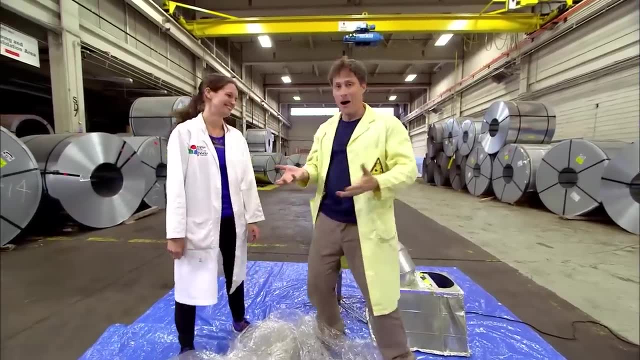 No, No, Oh no, It's going back down. Okay, So the balloon flies, which is great, Awesome. The problem is it turns over in the air. Yeah, I noticed that. I noticed that. And if it turns upside down, then all the hot air comes out. 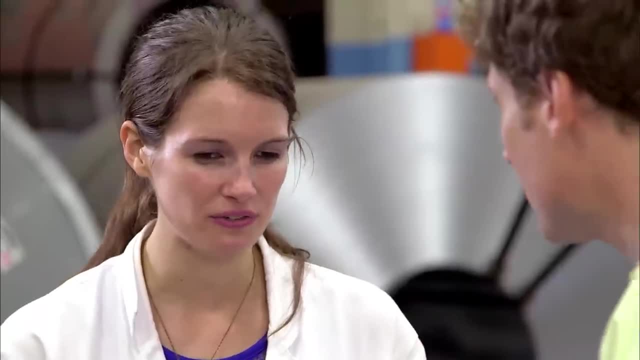 And it doesn't fly anymore. I know I was thinking: next time, if we make it bigger, what if we had a little weight at the bottom just to keep it stable? Oh yeah, Okay. I've seen balloons that have sort of an X, like a very light wood that goes across the 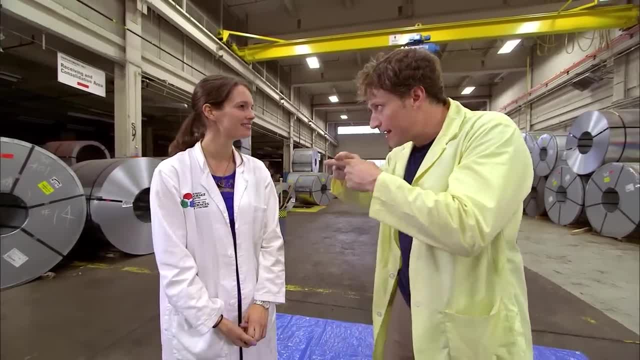 opening at the bottom. Oh wow, Maybe we could tie a piece of rope to that to keep it weighted, And if the bottom is heavier then it won't flip over upside down. right, Love that idea. So we're going to weight it at the bottom with a little X so that it doesn't flip over. 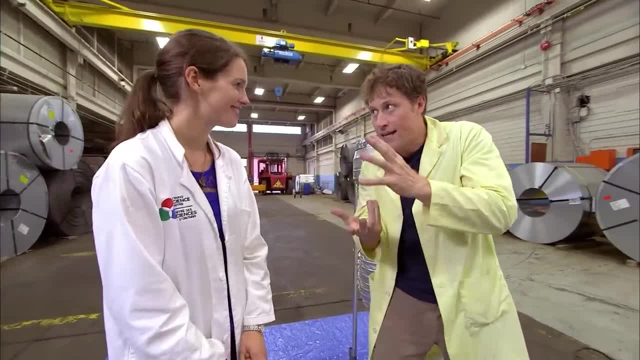 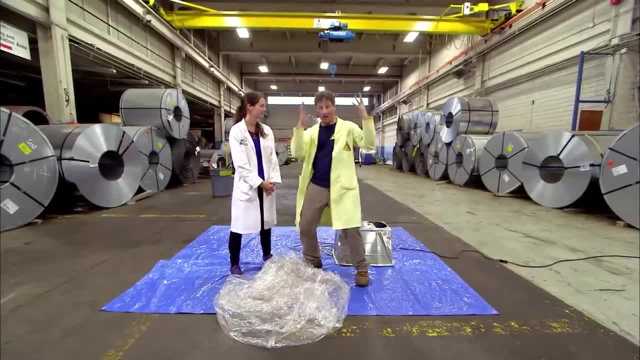 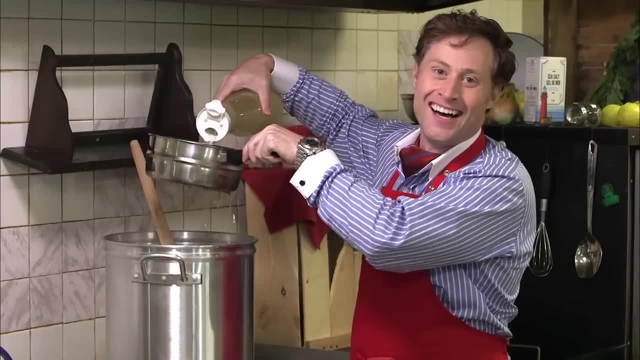 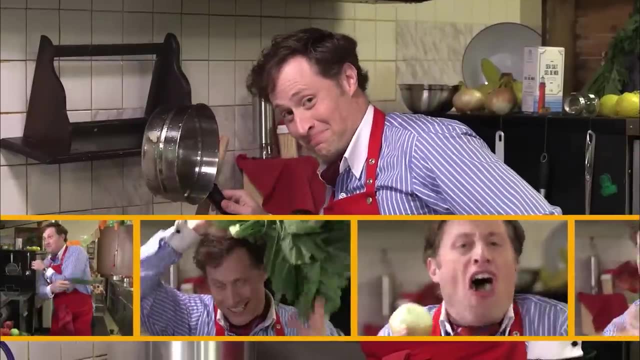 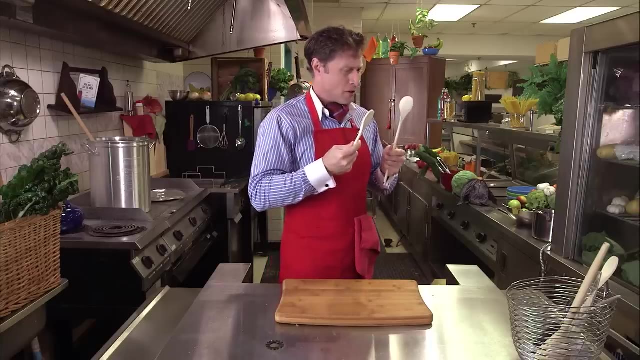 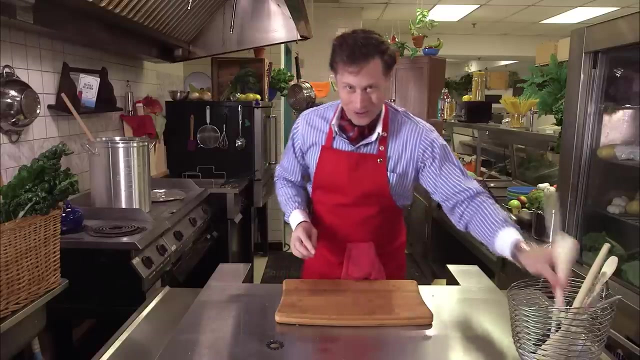 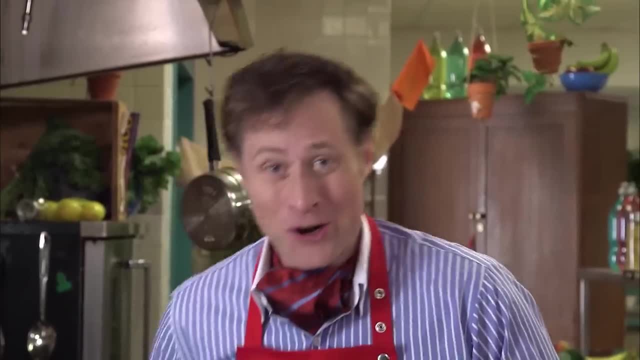 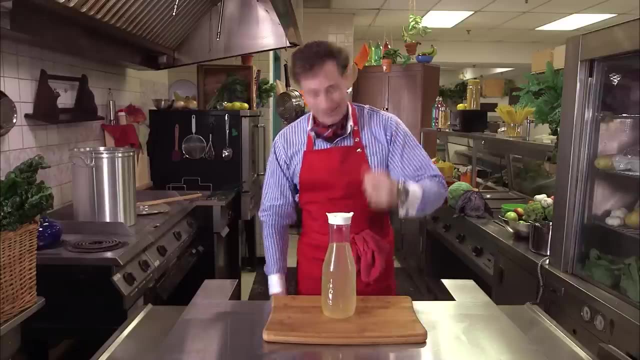 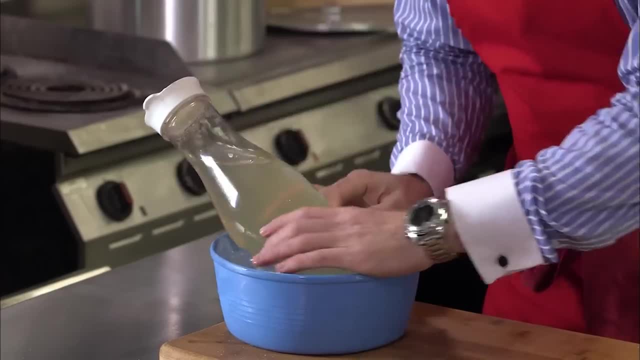 Look at this bottle of lemonade. It's warm right now and not very refreshing, So what's the best way to cool this down? We put it in ice, right, But did you know? there's an even better recipe than ice: You can make ice colder. 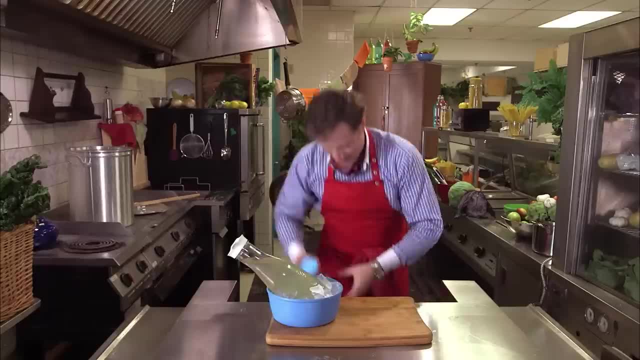 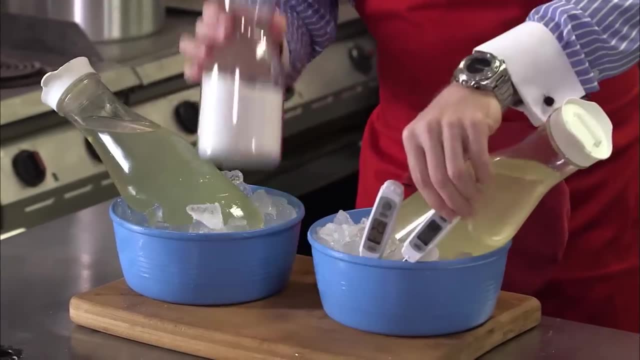 It's made of pure water. We're going to use some water, That's true. All you need to do is add salt. I've got a second bowl of ice and a second jug of lemonade, and I've got two digital thermometers. 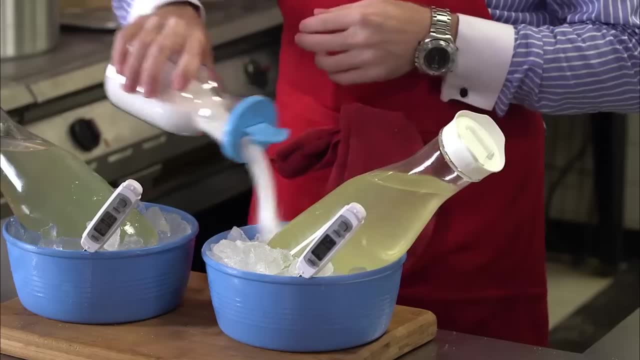 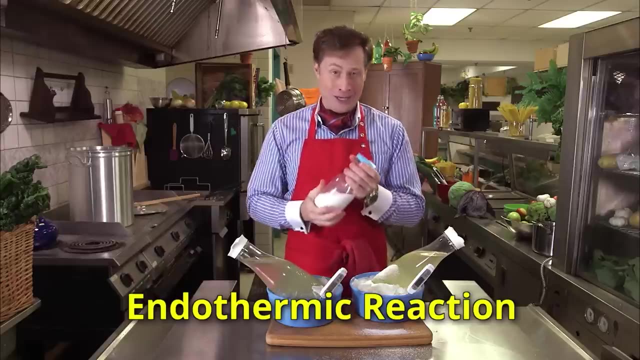 What I'm going to do is add salt to this bowl. What the salt does? it starts to melt the ice, and that actually consumes heat. This is called an endothermic reaction, and it absorbs heat, which makes the ice colder. 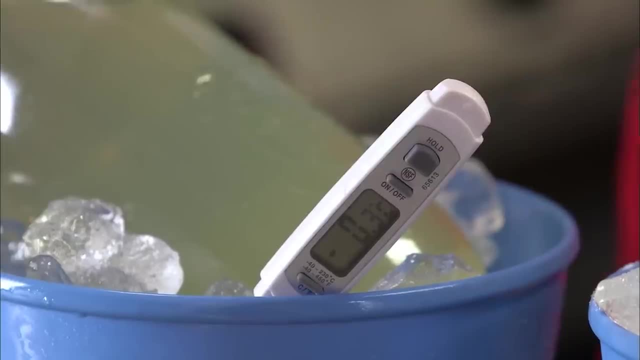 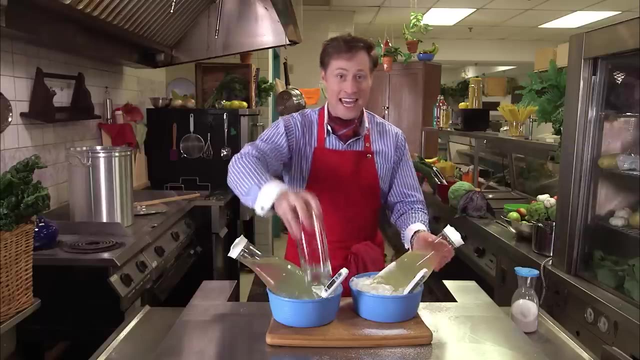 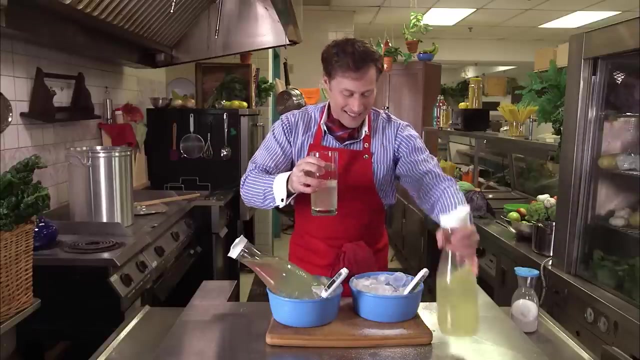 And, as you can see, this bowl of ice still sitting at around zero degrees Celsius, but this bowl minus eight and falling Wow. So there you have it, making something even colder than ice would normally make it. That is a way to make a refreshing glass of lemonade. 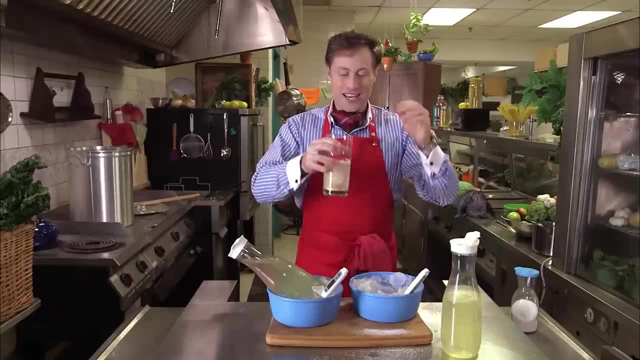 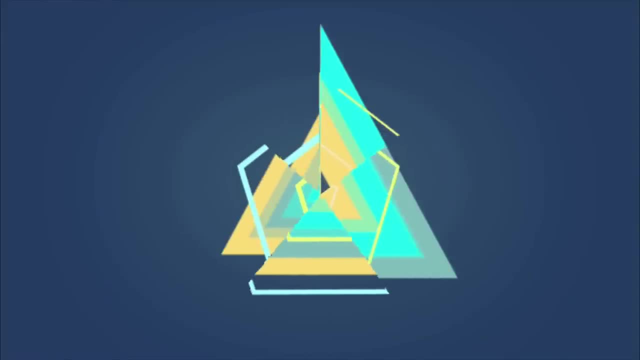 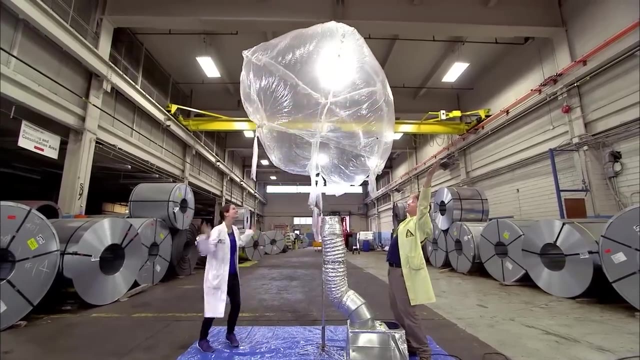 I'm Boss Nobika and thank you for joining me on Cooking with Science. With our new heater and lighter materials, our hot air balloon was floating free, That is, until it tipped over. When that happens, all the hot air inside escapes. 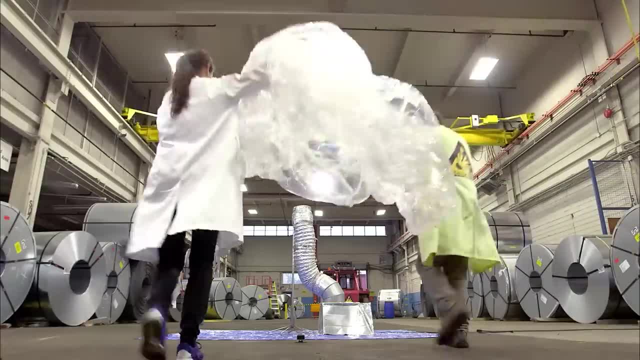 But Michaela and I have a solution. so we decided to build an even bigger hot air balloon and add a way to keep it upright. So, the process aside from that, we're going to make a hot air balloon. So, the process aside from that, we're going to make a hot air balloon. 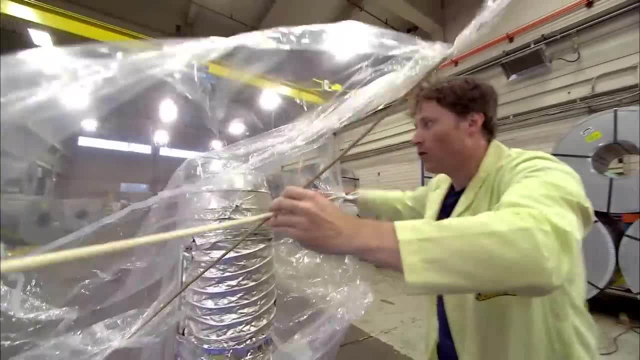 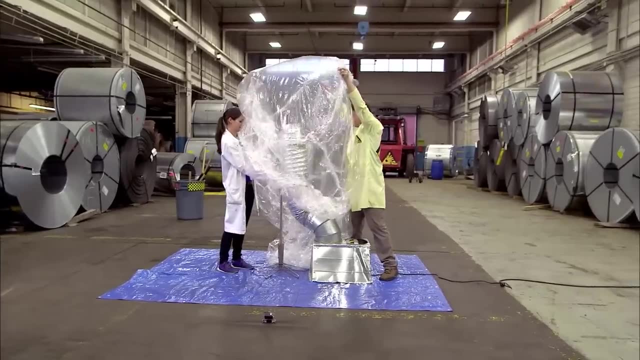 So the process. aside from that, we're going to make a hot air balloon. It's pretty much the same. We put the end over top of our industrial heater and I will plug it in. Get that hair dryer again, for good measure. 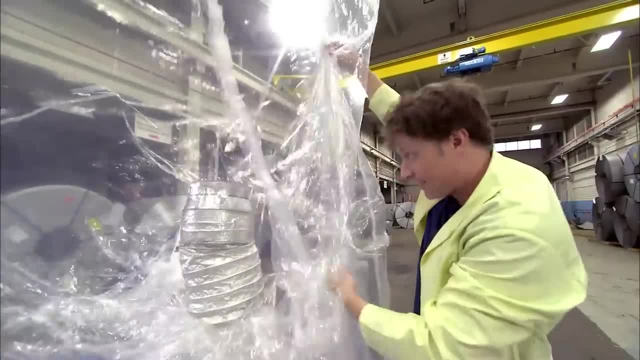 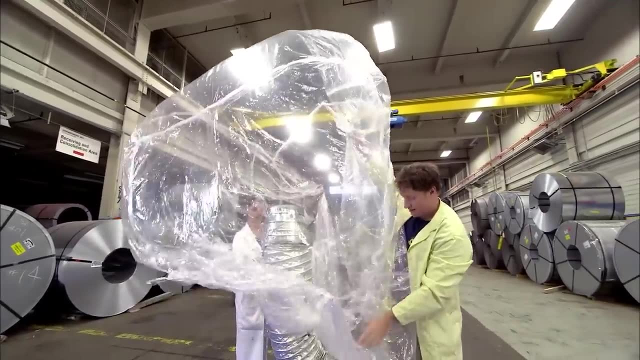 It's working. It's inflating, but we got to keep fluffing it up, otherwise it just sort of sags. But you can see the top of the balloon is definitely working. It's a lot bigger than the last one though. 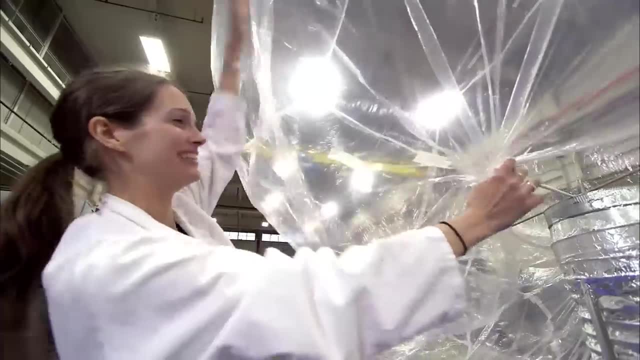 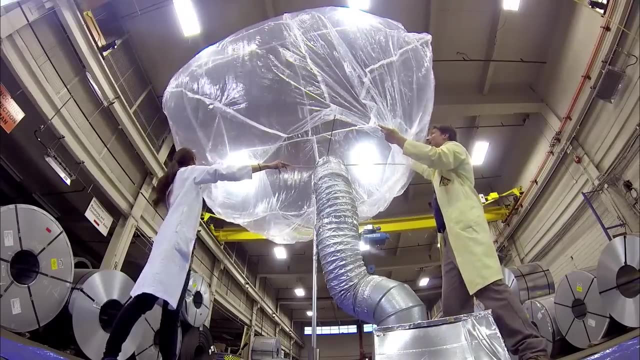 Do you think we made it too big? Michaela? It's really big. I think it's working. It's definitely working. Uh-oh, Pull your side, Hold it. Oh, it's totally working. I'm so surprised that this works so well. 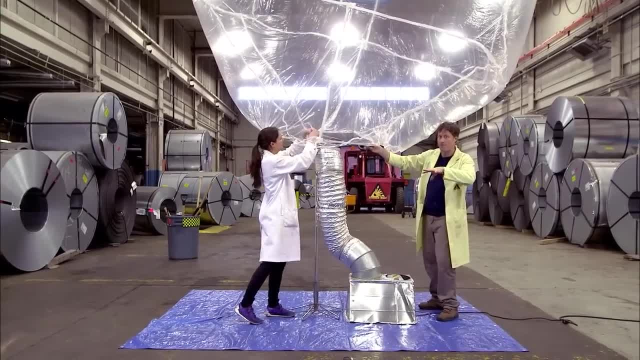 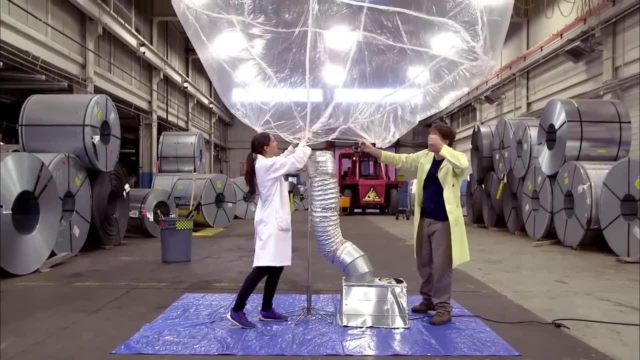 So the stick is going to keep it balanced. so the bottom faces down, but Michaela's going to tie a string to the stick so that when it goes up we can keep it centered. Okay, this looks good. You want to let it go?